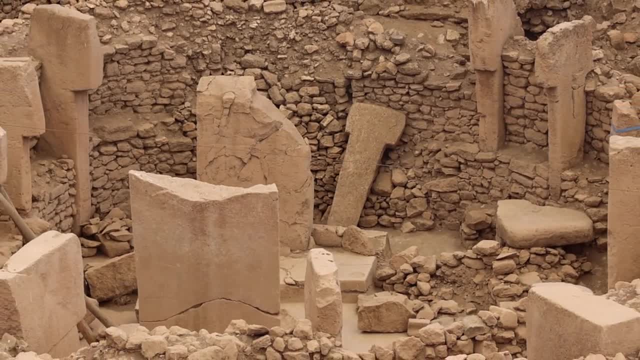 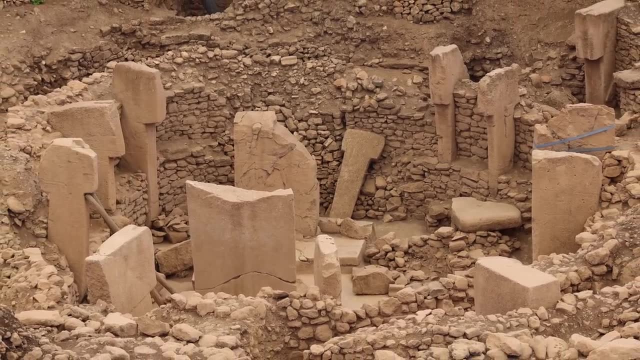 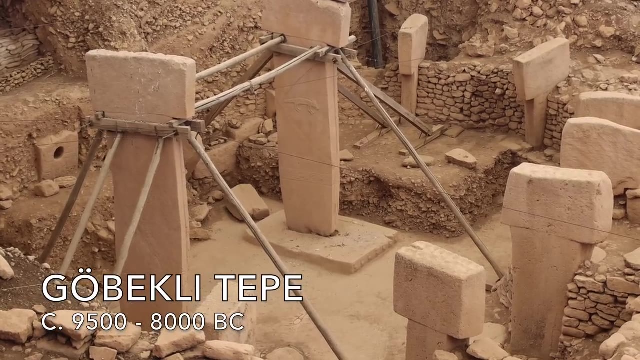 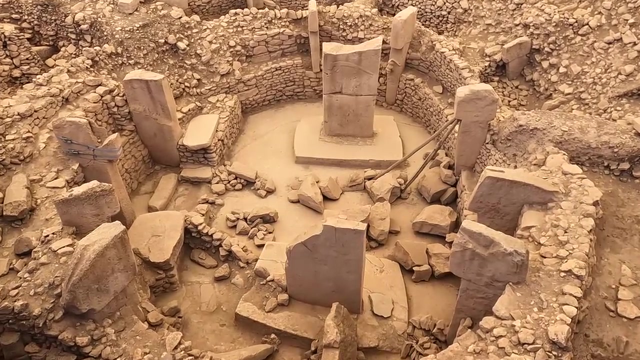 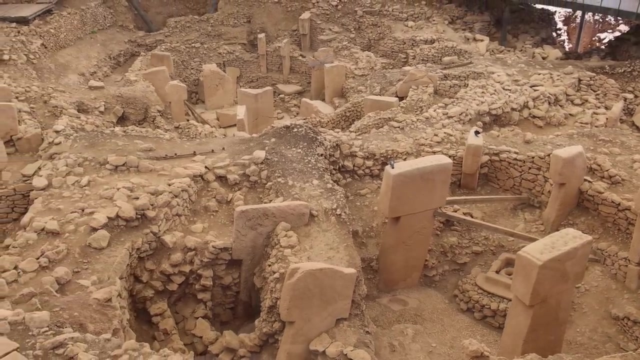 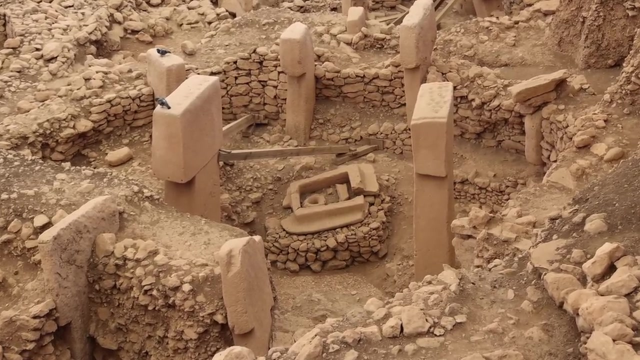 At Gobekli Tepe. gods and mortals once walked the earth, So the old stories must surely once have told Of the rituals, festivals and sacrifices of those ancient days. we can say little now, for certain Its people are gone. 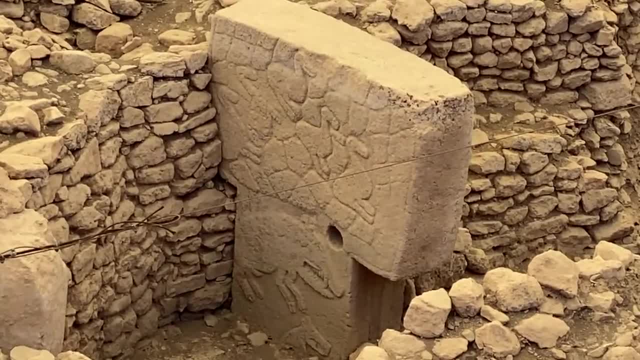 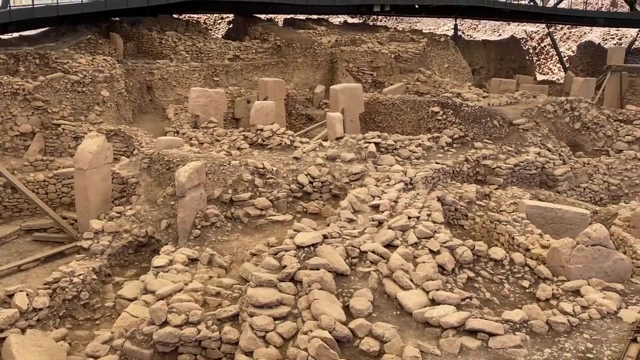 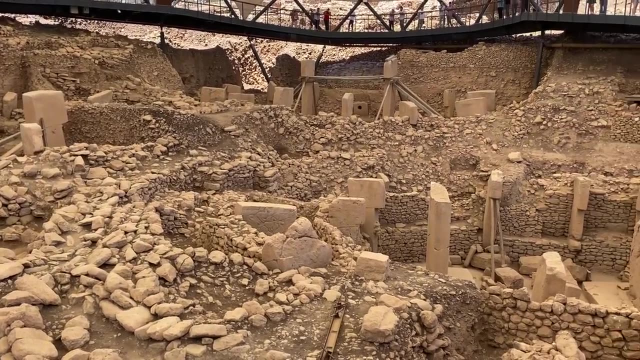 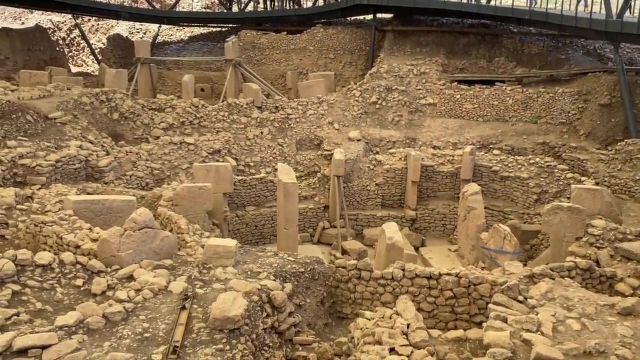 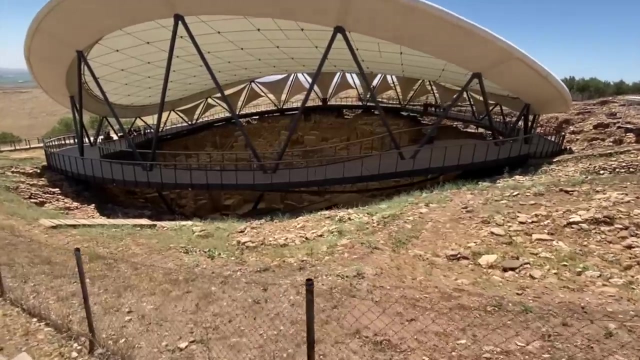 Deities cast into the void. What truly happened there, we will likely never know, And yet, since its rediscovery by the wider world in the 1990s, archaeologists, anthropologists and historians have done their best to weave together a flimsy shell of a story. 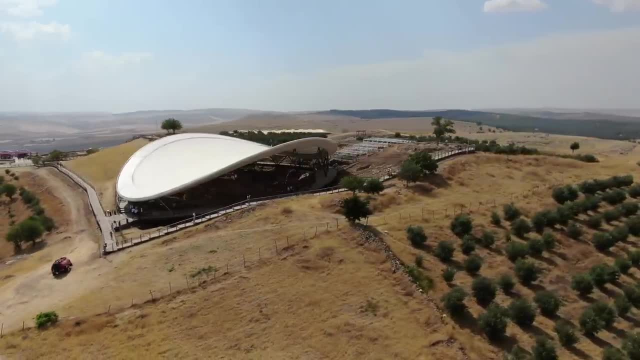 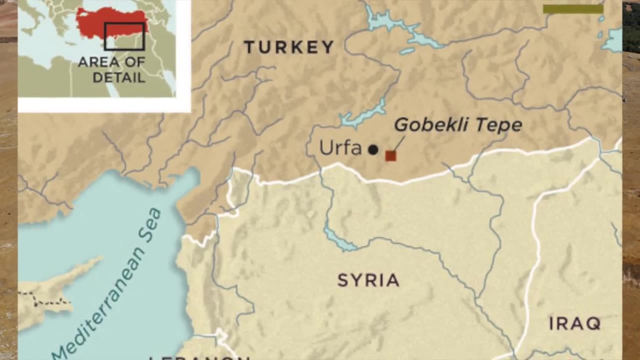 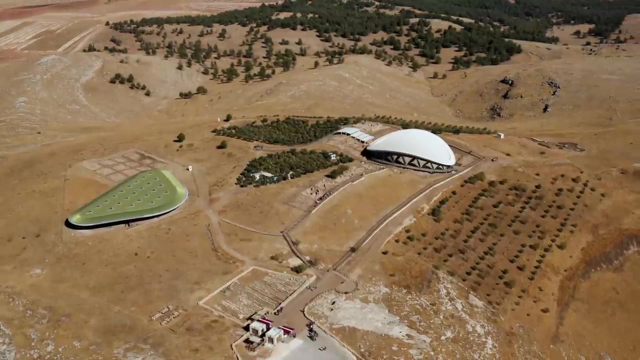 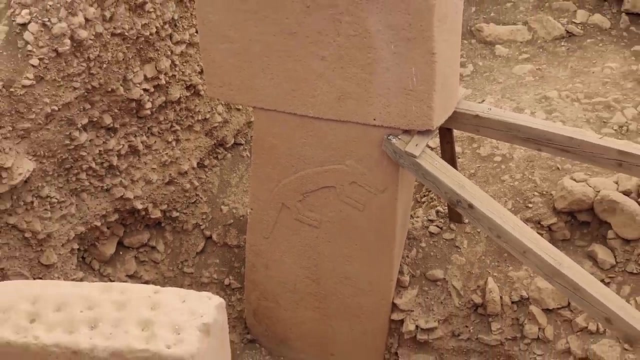 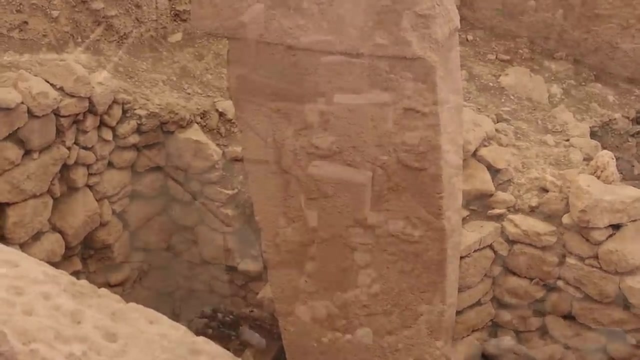 to do justice to that low-rising mound in the plains outside of Urfa, Utilising a vast array of data and techniques to mesh together a very basic idea of what the place was and who its builders had been. More outlandish commenters go further, embellishing the flimsy archaeological dataset. 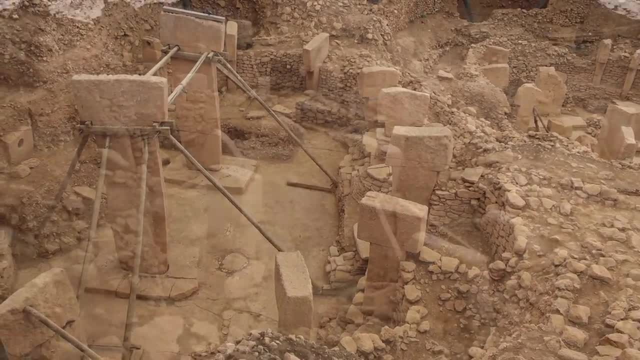 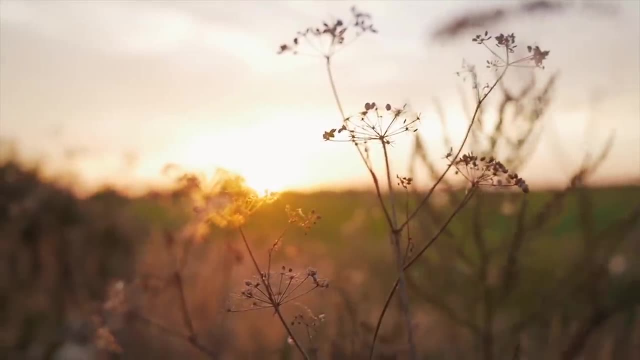 with their own New Age religious leanings and preconceived ideas. And yet this is not the end of the story. It is the beginning of a new chapter in the history of archaeology. It is the beginning of a new chapter in the history of archaeology. 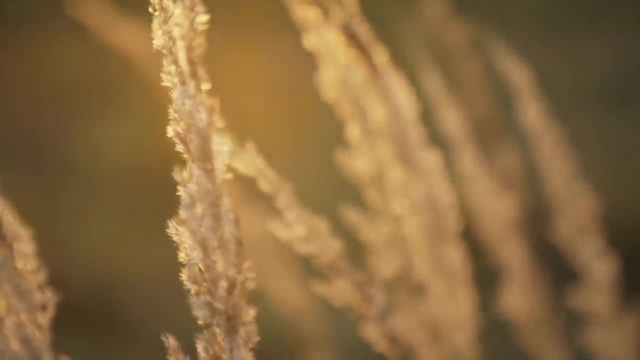 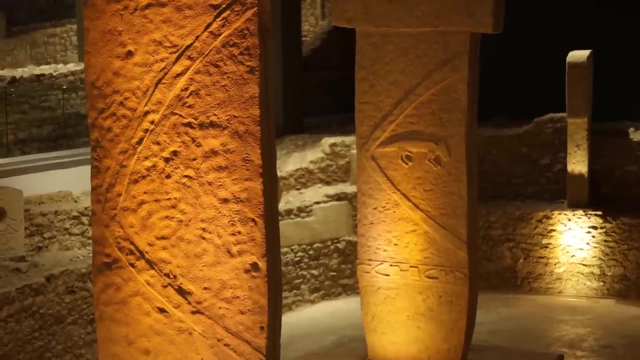 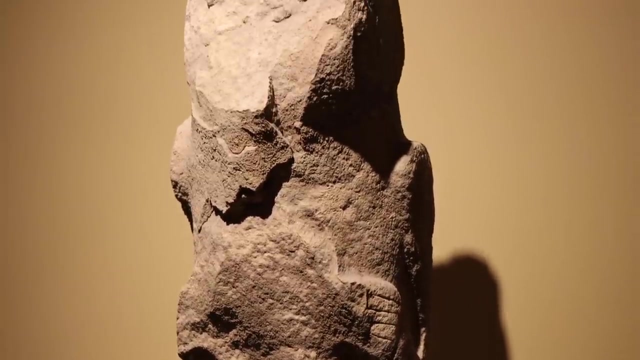 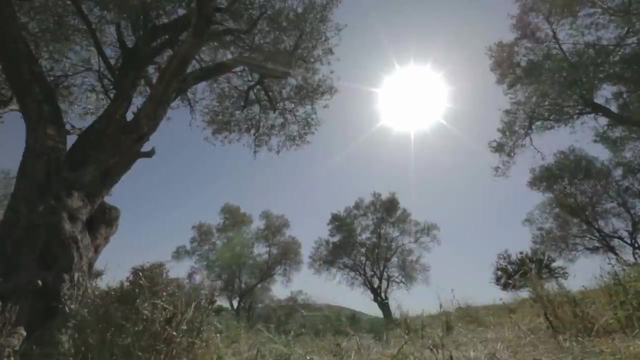 Turning concrete evidence of wild grasses, wild grains and as yet still undomesticated prey animals into landing grounds for aliens or the Biblical Garden of Eden. Wonderfully complex, genuine hunter-gatherer ancestors into ancient stories To the very high level of civilization. 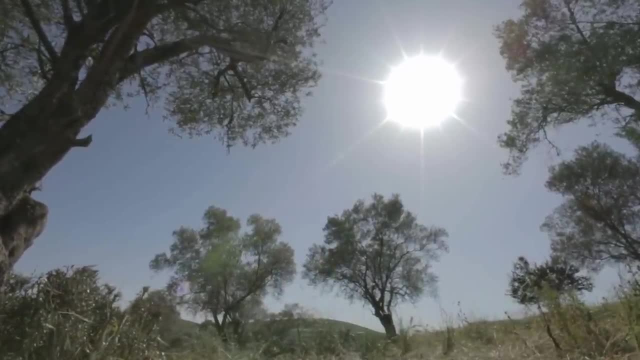 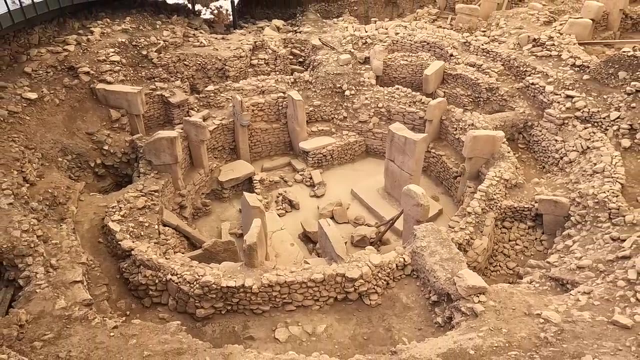 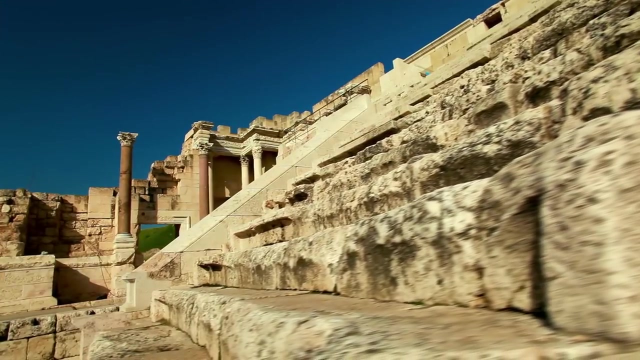 To the very high level of civilization. To the very high level of civilization. In reality, still, for the most part, Gobekli Tepe's secrets remain hidden, Unlike the other most famous discoveries in archaeological history, like Tutankhamun's tomb or the royal burial grounds of Ur. 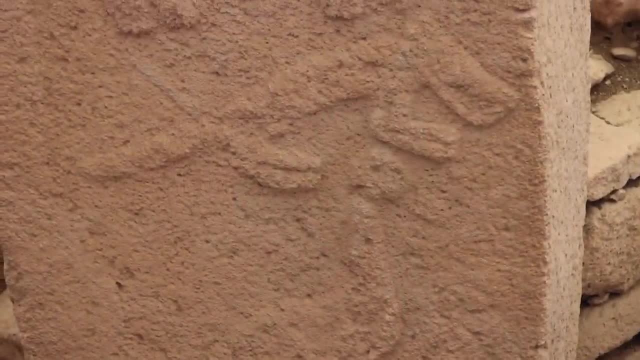 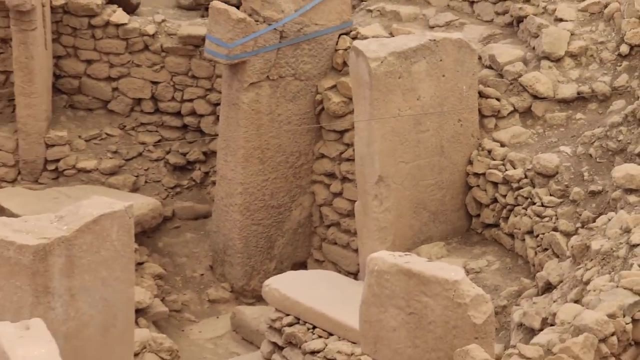 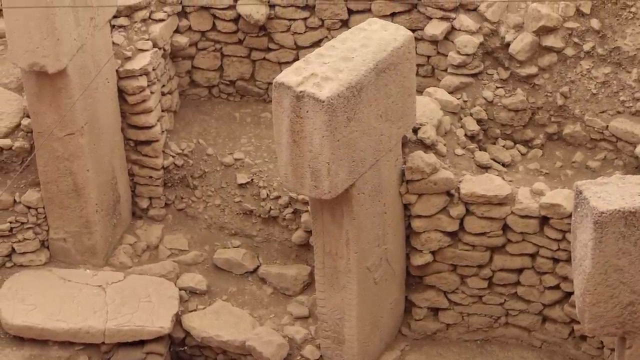 like Tutankhamun's tomb or the royal burial grounds of Ur. Here there is very little to go on, Little contemporary evidence to corroborate what happened, To explain those 200 or so monoliths arrayed into 20 megalithic enclosures. 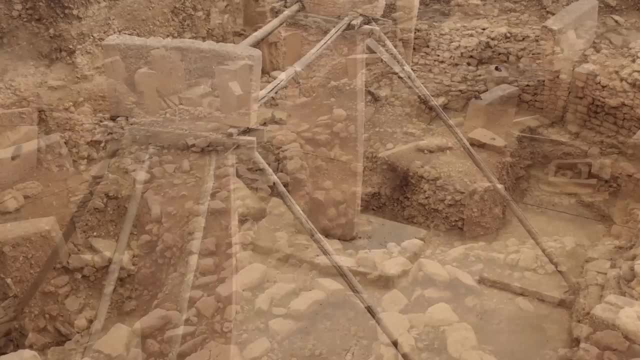 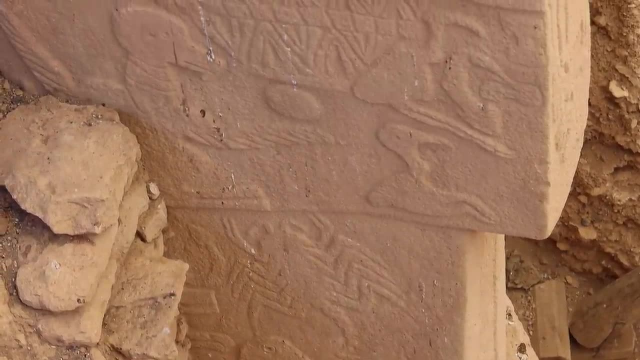 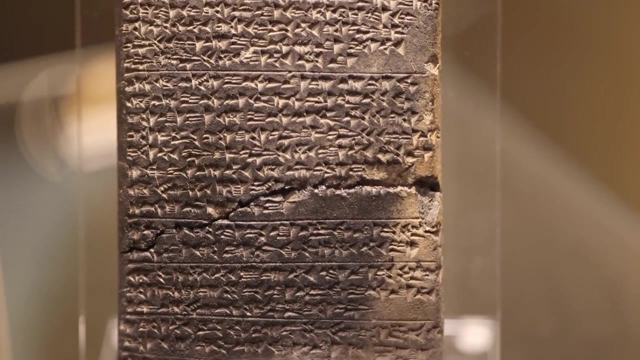 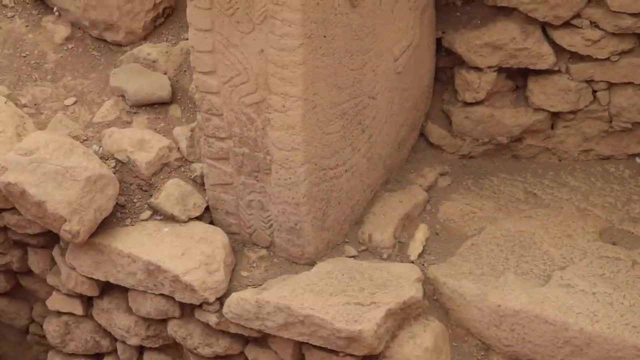 Some standing well over five meters high, their surfaces coated in bizarre, even nightmarish, creatures. Written accounts wouldn't exist for more than 5,000 years to come. In recent years, the discoveries of these monoliths have become more and more commonplace. 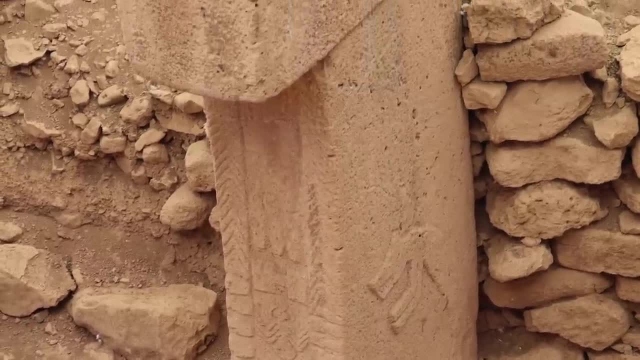 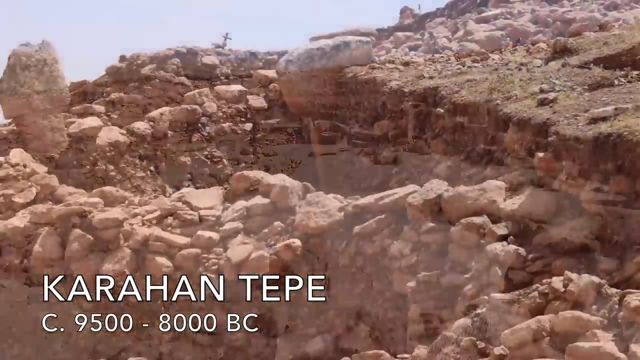 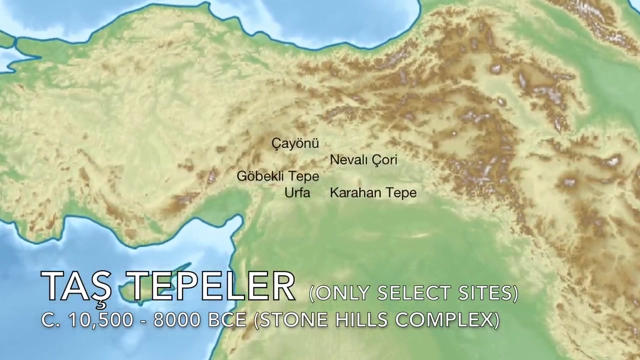 The remains of neighbouring sites with enclosures similar in scale, like Karahan Tepe, add to the already swelling ranks of a so-called Stone Hills complex in the foothills of the southern Taurus mountains, Sites like Nvali, Chori and Chianu. 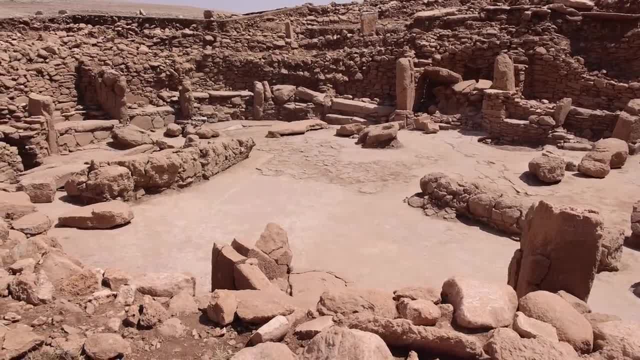 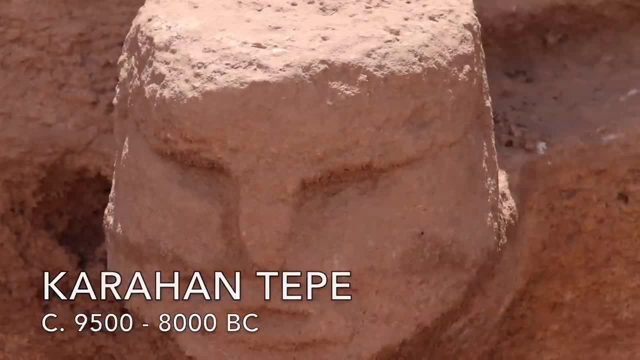 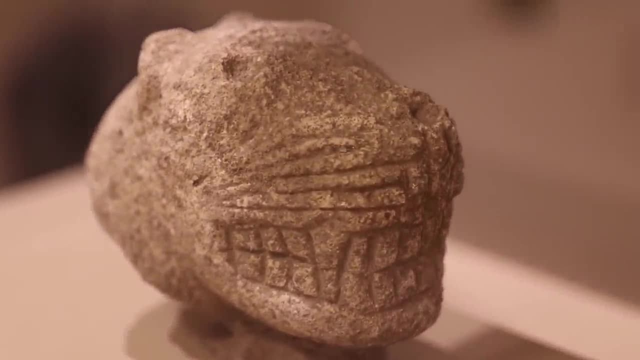 The sheer fact that Gobekli Tepe is a monolith is not, in fact unique, but one piece in a much larger picture makes it all the more enigmatic and captivating, Thus opening up seemingly endless new lines of inquiry. Thus opening up seemingly endless new lines of inquiry. 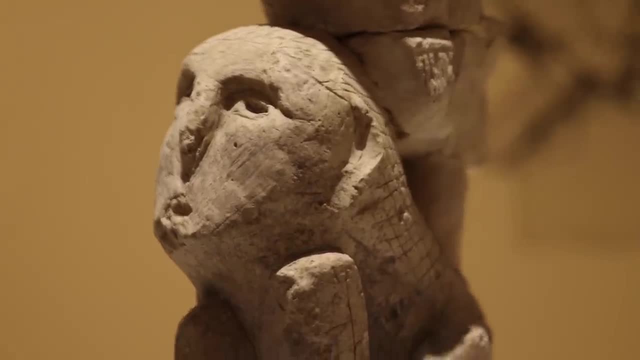 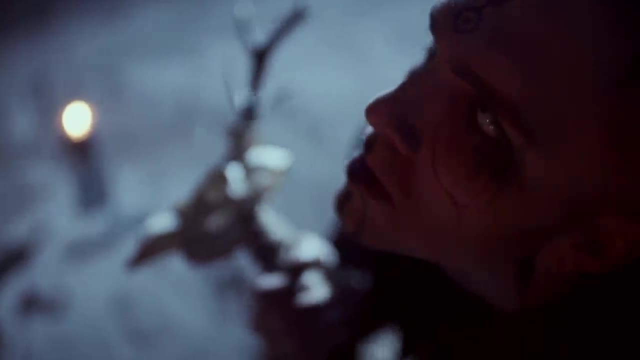 With its origins lying well over 10,000 years in the past. With its origins lying well over 10,000 years in the past, Perhaps its antecedents even longer, Perhaps its antecedents even longer: The sheer age of this incredibly sophisticated Stone Age culture. 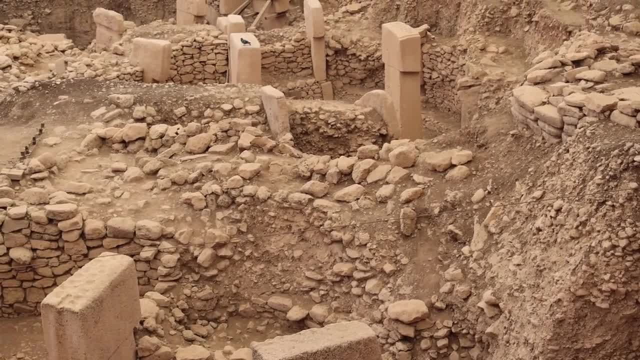 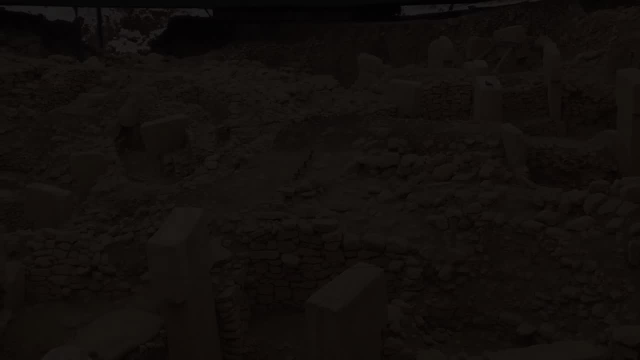 The sheer age of this incredibly sophisticated Stone Age culture has been enough to solidify its place, has been enough to solidify its place at the very forefront of prehistoric archaeology, at the very forefront of prehistoric archaeology, Even making inroads to the world of popular culture. 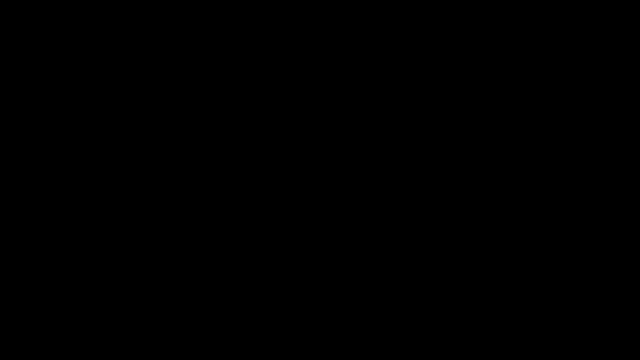 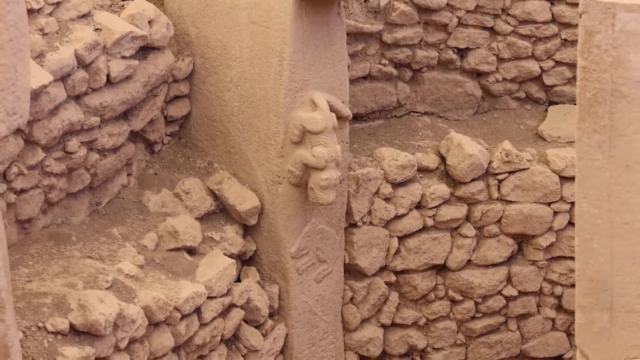 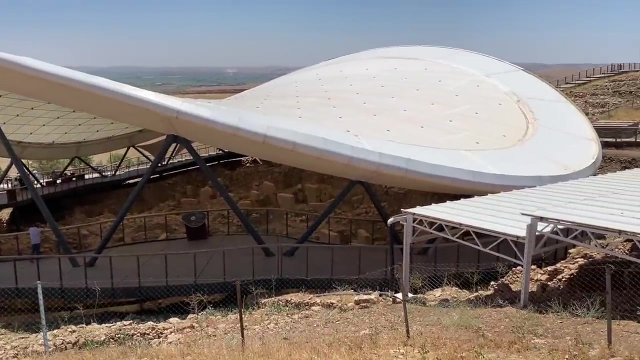 Even making inroads to the world of popular culture, Even making inroads to the world of popular culture. It's one of the big ones, One of the most significant archaeological discoveries, One of the most significant archaeological discoveries and one of the best excavations of all time. 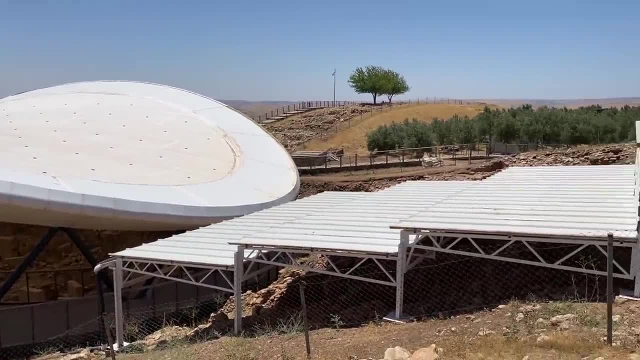 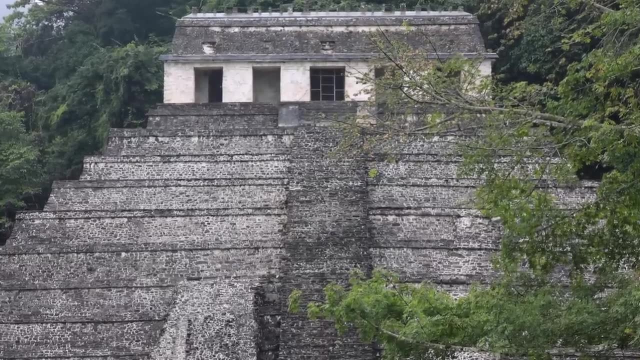 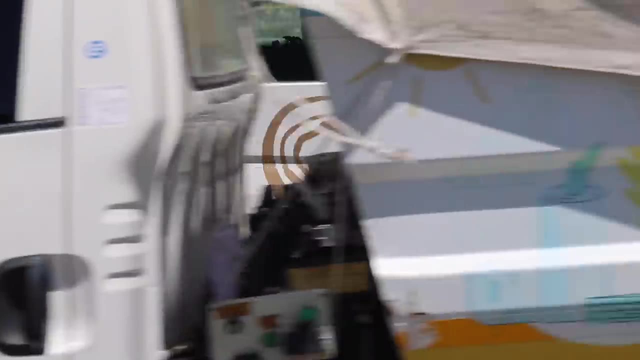 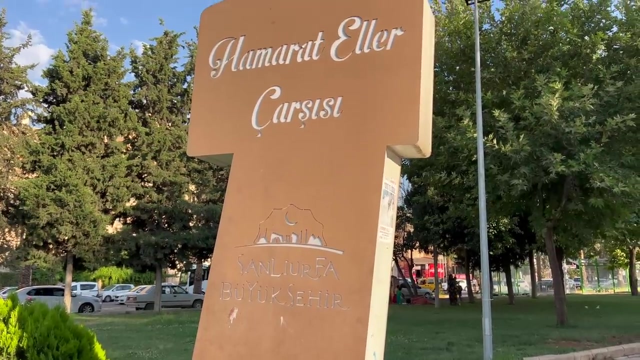 and one of the best excavations of all time, On par with Jericho Uruk, On par with Jericho Uruk and the tomb of Pakal, Though found much sooner. Though found much sooner only in the 1990s. Gobekli Tepe's impact on the cultural zeitgeist. 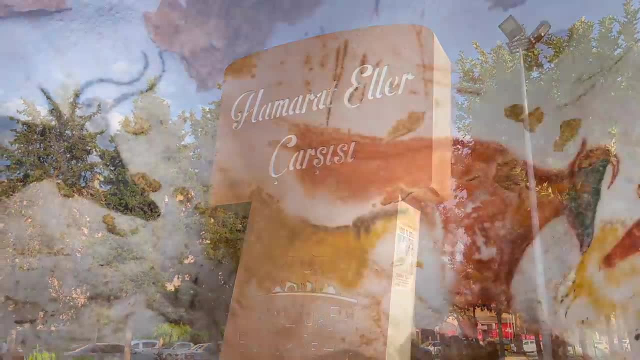 Gobekli Tepe's impact on the cultural zeitgeist is as great as that of the Lascaux cave art, is as great as that of the Lascaux cave art in the 1800s, in the 1800s. 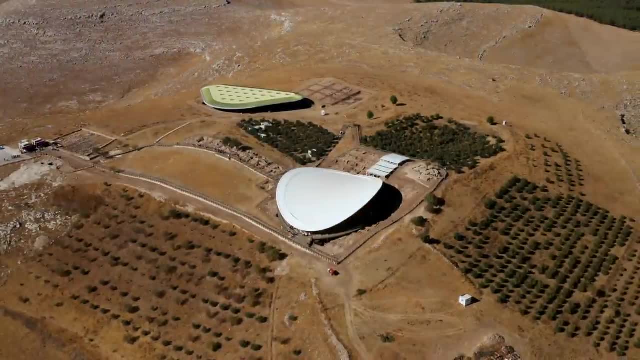 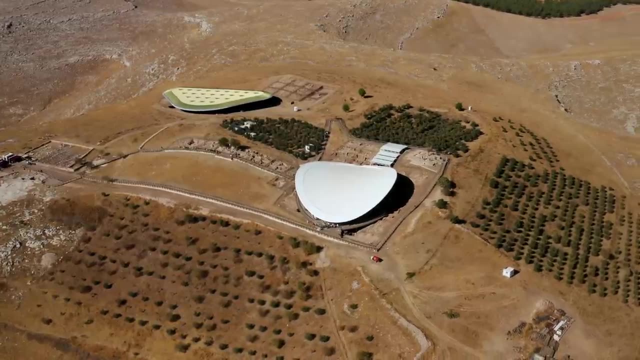 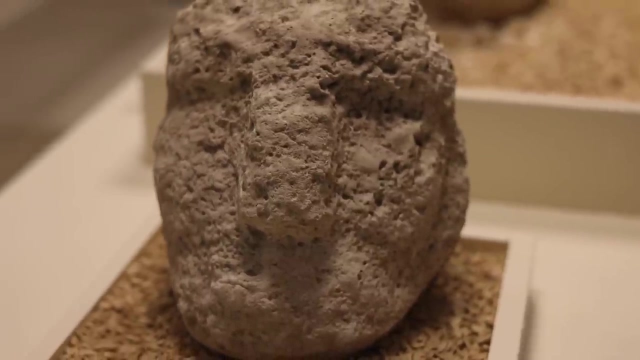 Only time will tell. Only time will tell what future discoveries will be made, what future discoveries will be made And in which ways the evidence And in which ways the evidence and research will point. And yet, still, And yet still, even after spending. 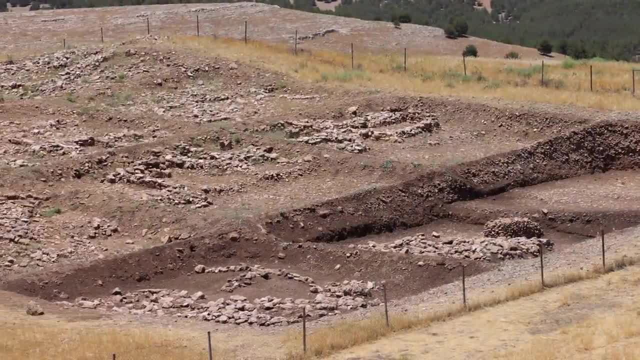 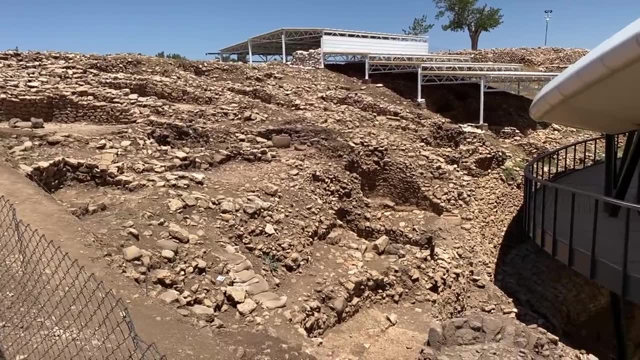 and yet still, even after spending time and effort in excavation, we are still, for the most part, we are still, for the most part, left answerless, Adrift to ponder and contemplate, Adrift to ponder and contemplate the outrageously complicated carvings. 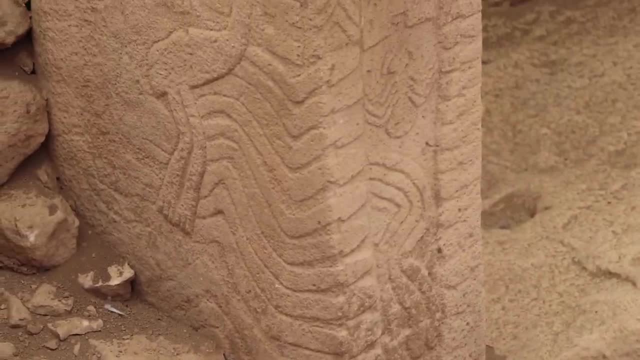 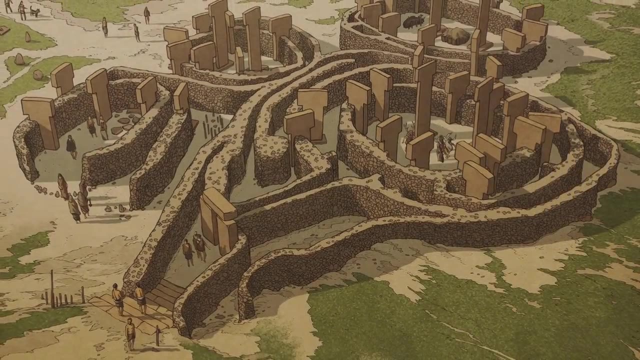 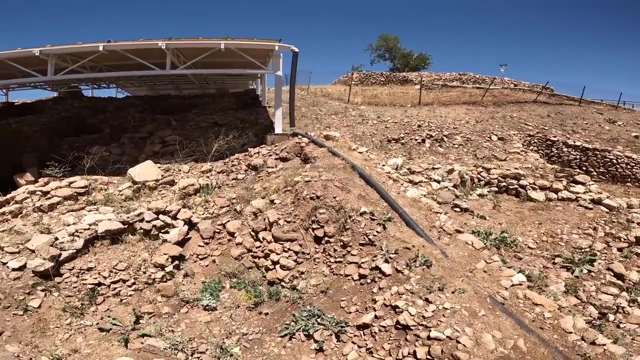 the outrageously complicated carvings and temples left behind by those people who lived so impossibly long ago. who lived so impossibly long ago? who lived so impossibly long ago. It will take many more decades. It will take many more decades, centuries even. 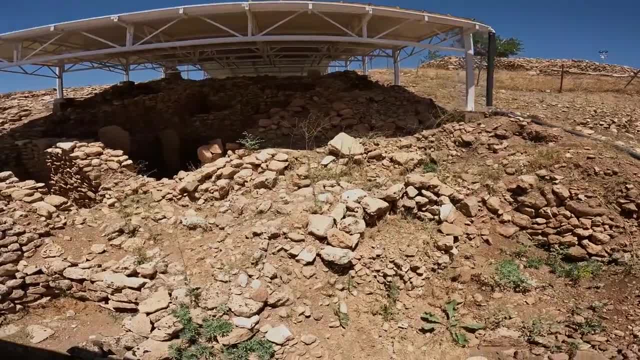 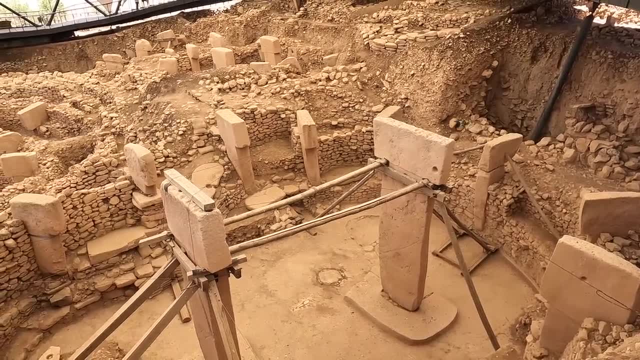 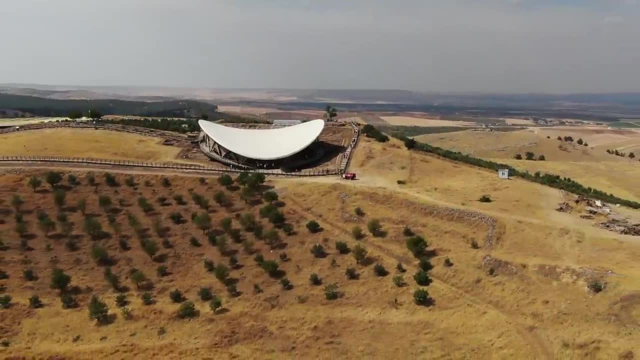 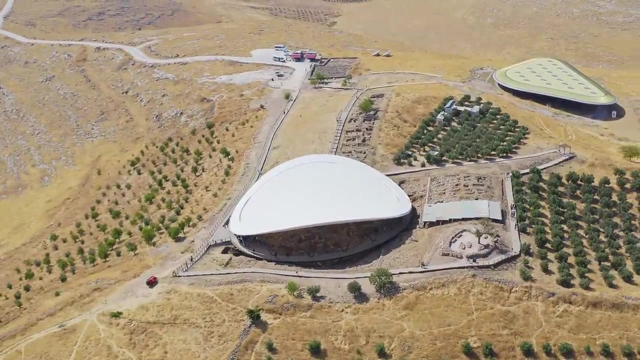 until the sheer amount of evidence piles up, high enough that the mysteries of those ancient days can truly be unlocked- can truly be unlocked and retold As of 2021,. As of 2021,, less than 5% of the site has been excavated. 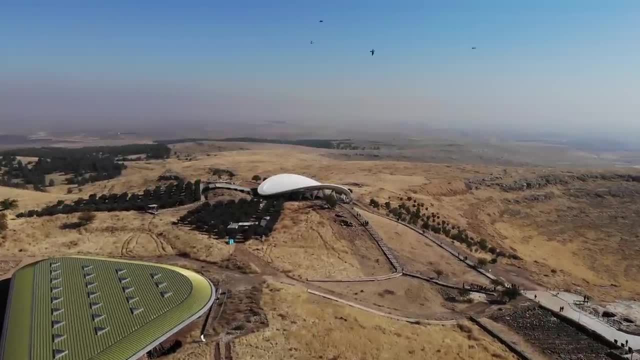 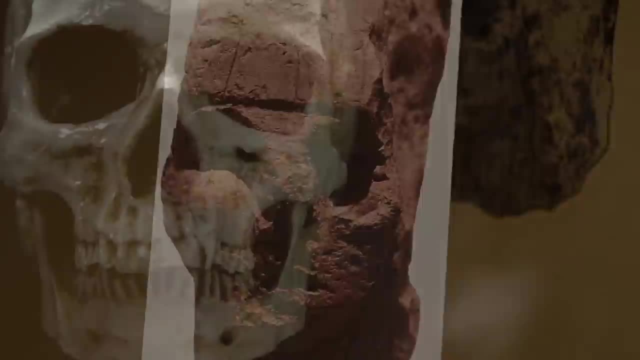 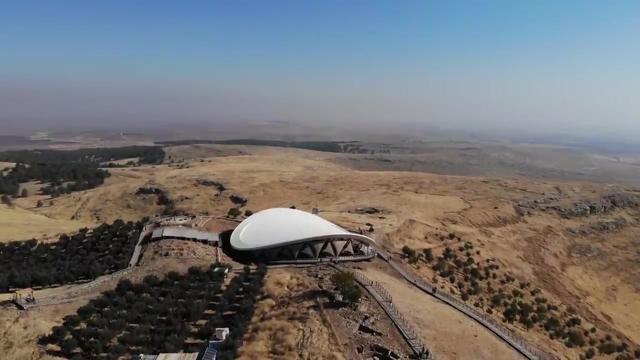 And yet, utilising the very latest archaeological data, historical stories and mythological and anthropological theories and anthropological theories, this is the entire history of not just Gobekli Tepe, of not just Gobekli Tepe. 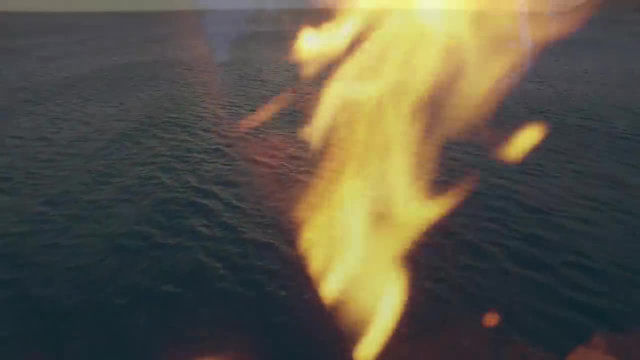 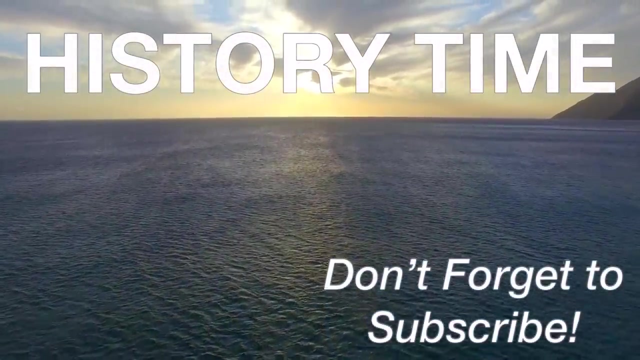 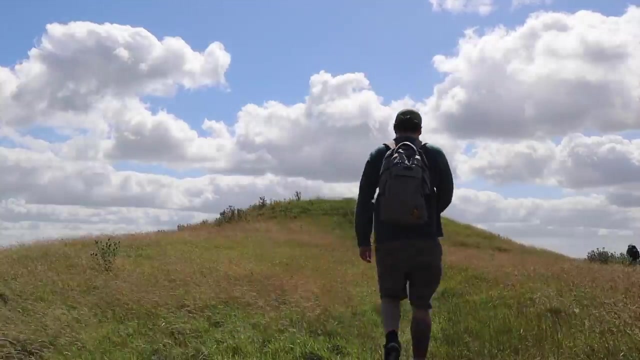 but the world it inhabited. but the world it inhabited. You're watching History Time. As always, I'm your host, Pete Kelly, The one-man team behind the channel, If you want to help me out as I continue to make these gargantuan monsters. 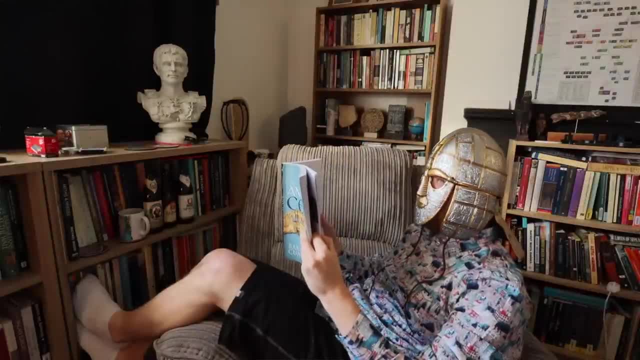 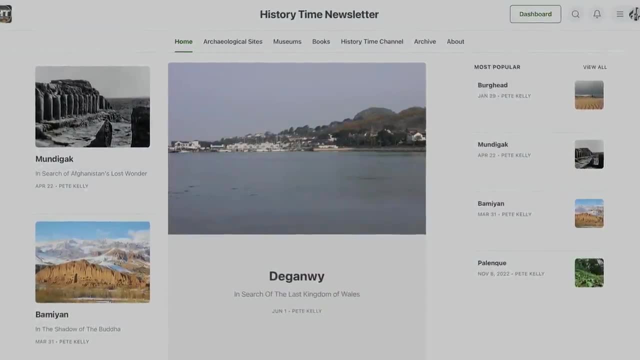 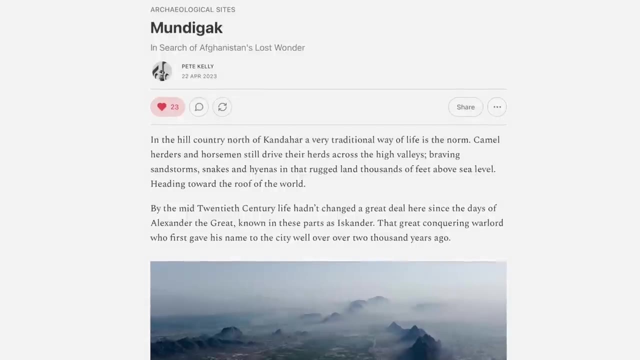 then don't forget to like and subscribe, Leave a comment letting me know what you think And sign up to my free newsletter where I travel to distant lands visiting the greatest archaeological sites humanity has ever known. Shortly, we'll get back to one of those rare 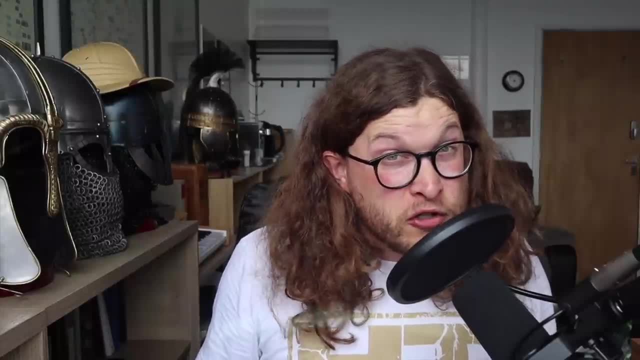 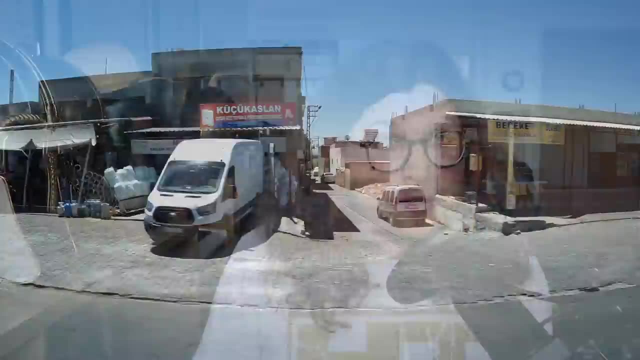 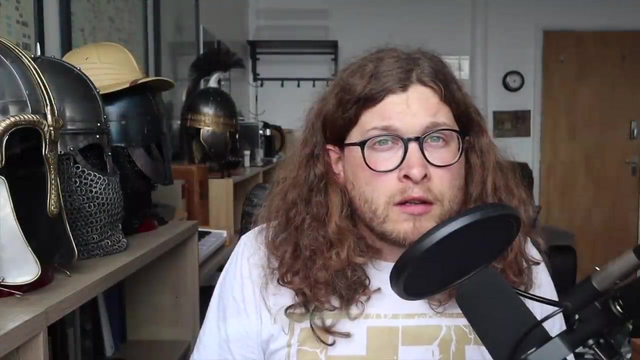 greatest of all time sites, One of the most mysterious of all. It's taken me well over a year to make and it's nearly three hours long. But first a quick word from our sponsor. Thanks to War Thunder for making this ridiculously time-consuming. 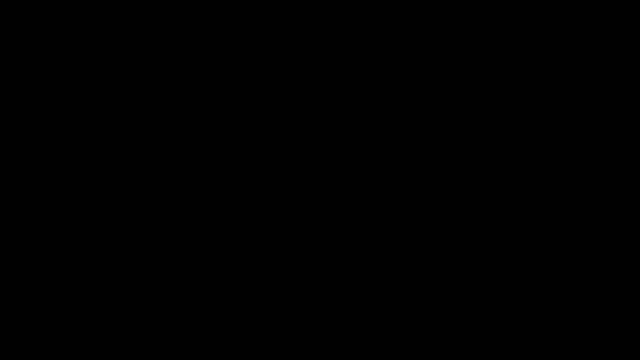 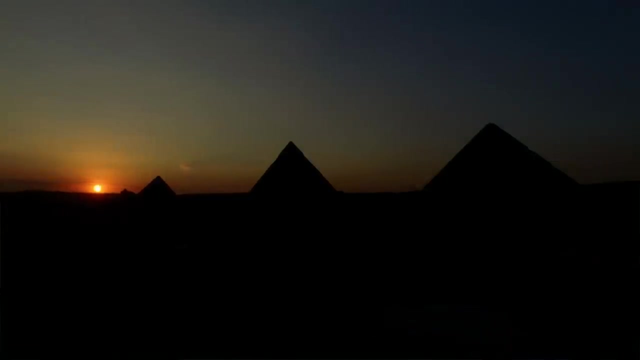 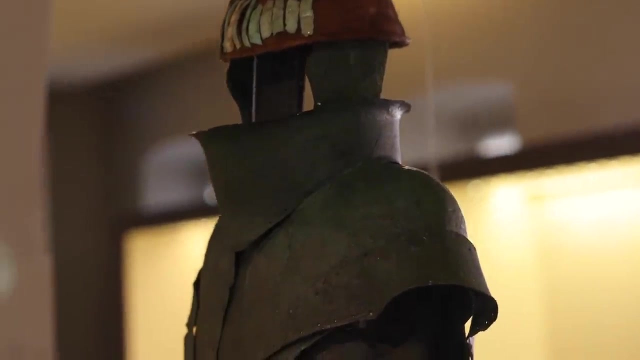 long-form project possible In the millennia following Gobekli Tepe. In the millennia following Gobekli Tepe, armored Bronze Age warriors have created battlefields Like this one found at Dendra in Greece By the medieval era. 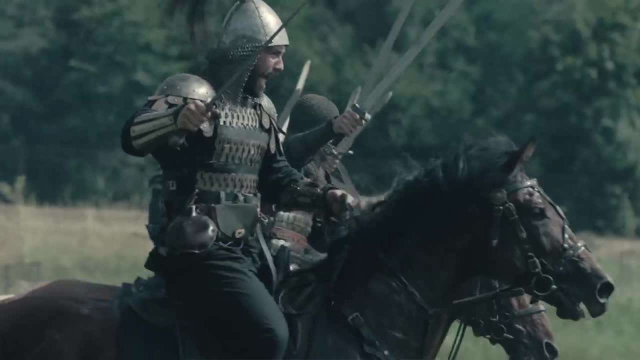 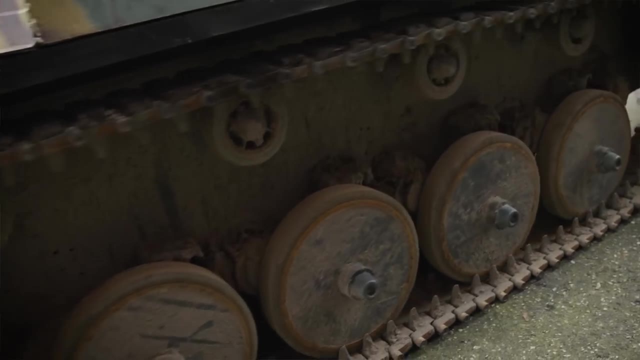 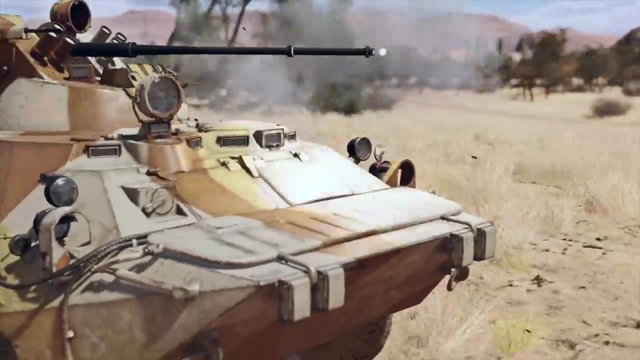 now mounted on horseback. similarly kitted out soldiers did the same. It wasn't until the 1910s and 20s that real tanks would be constructed, Completely changing warfare forevermore. War Thunder is the most comprehensive vehicle combat game ever made. 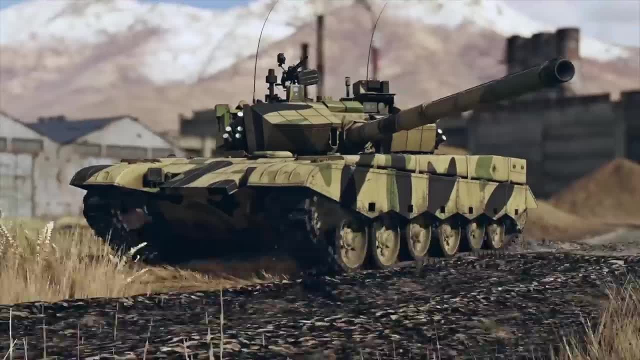 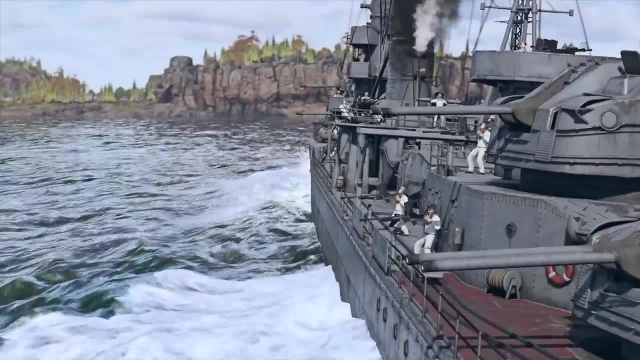 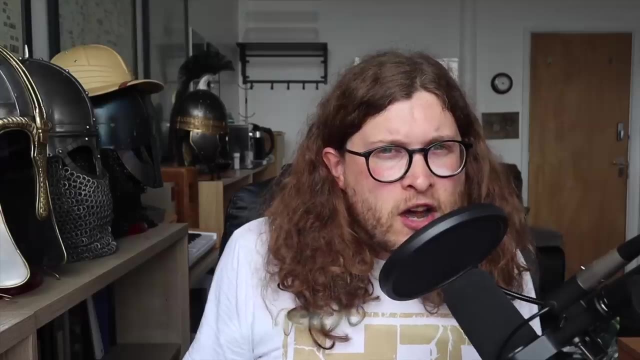 With its incredible graphics and details in 4K resolution, authentic sound effects and beautiful music. you can immerse yourself in the atmosphere as you choose from more than 2,000 tanks, planes, helicopters and ships to engage in dynamic combined arms PvP battles. 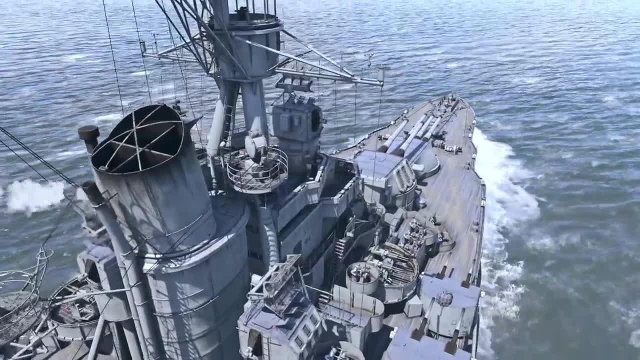 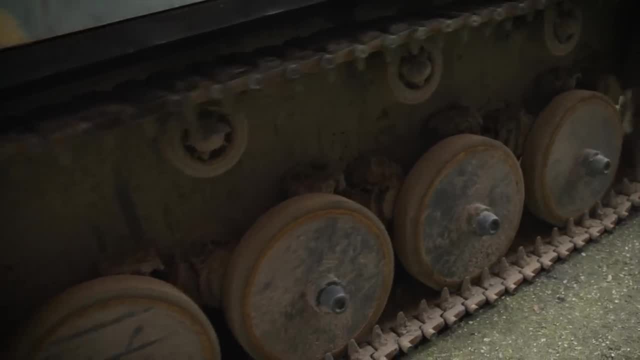 Of course, one aspect of the game that I like in particular is its historical accuracy and the chance to play as some of the very first clunky monstrosities ever to be built in the years following World War 1.. The collection of vehicles found. 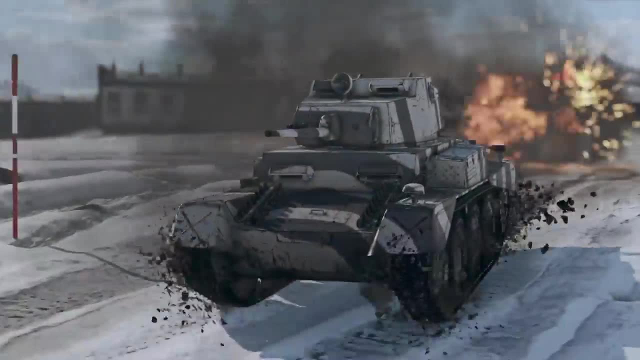 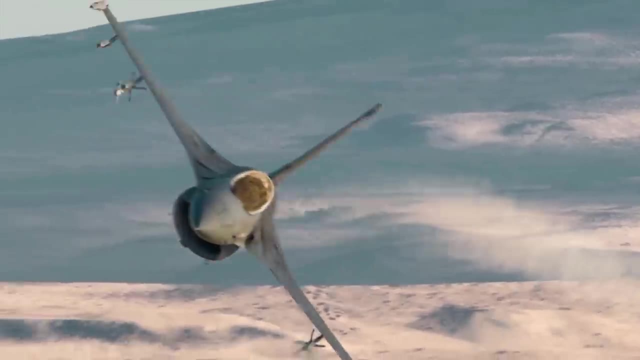 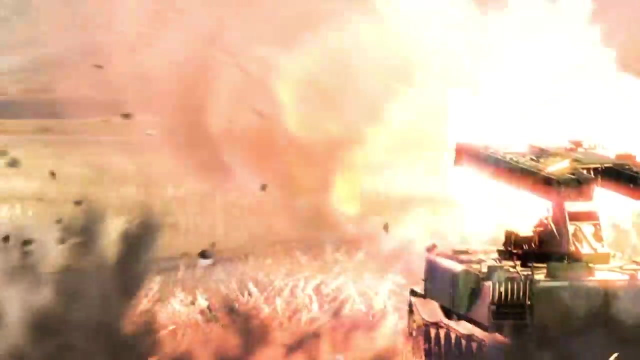 in War Thunder spans over a hundred years of fascinating history, in fact, from the 1920s to today, Every vehicle being incredibly detailed and modelled down to their individual components, offering a highly immersive combat experience. Use my link in the description below to play now. 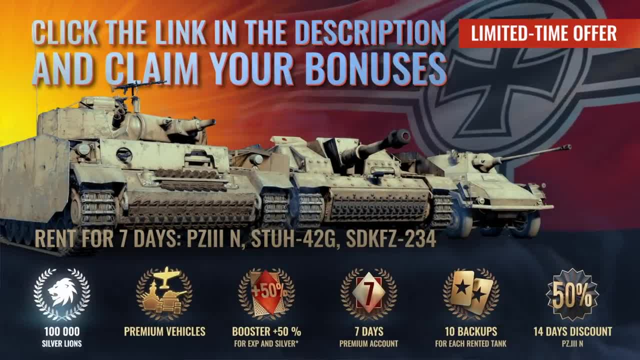 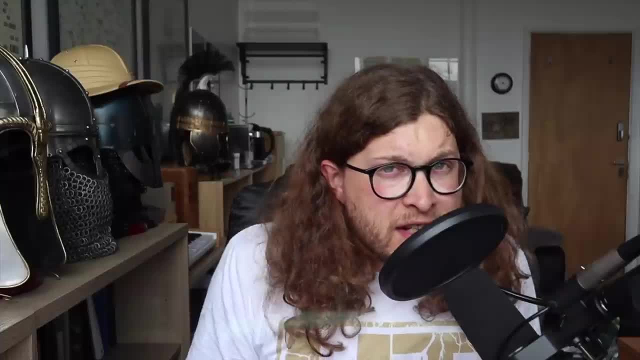 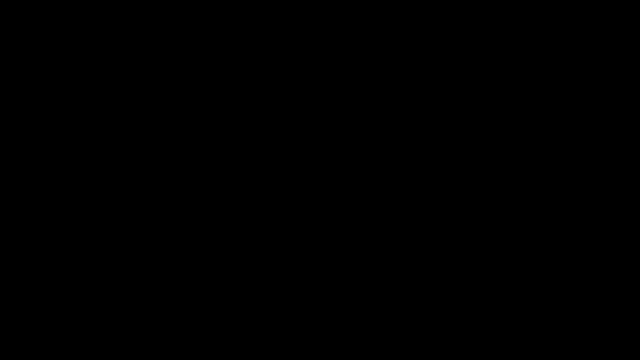 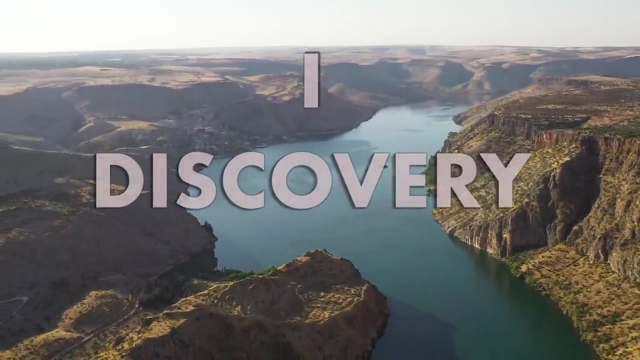 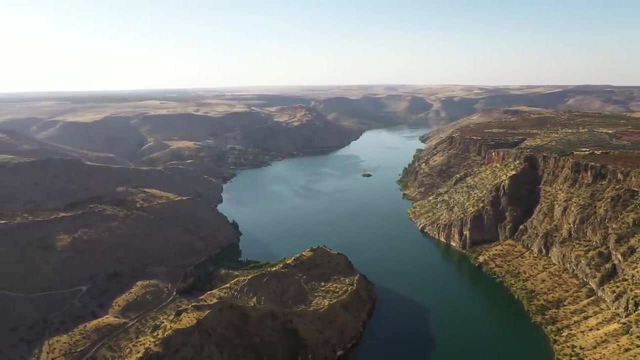 for free on PC, Xbox and PlayStation 5. or, for you old school people out there, you can even play on a previous generation console. Thanks again to War Thunder for sponsoring this video. and now back to the ancient past, When the final blocks of cement went into place. 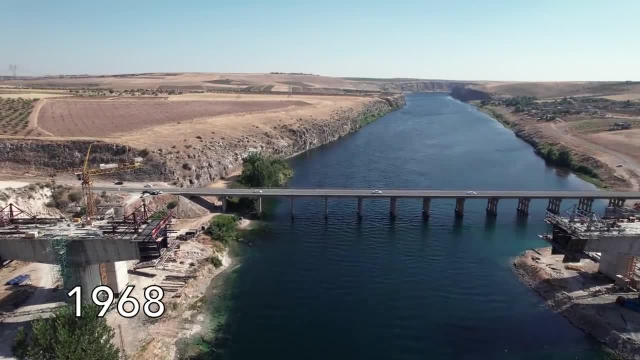 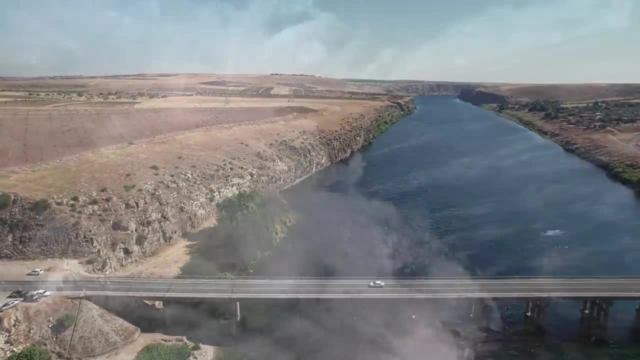 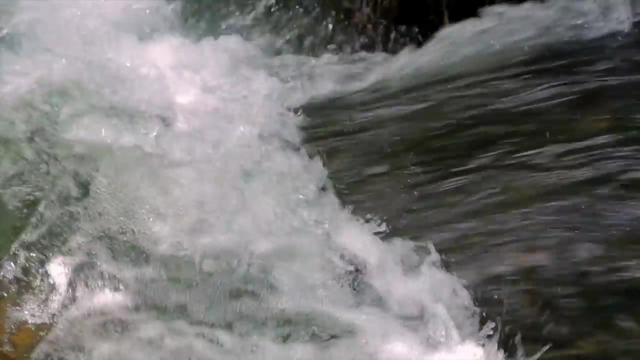 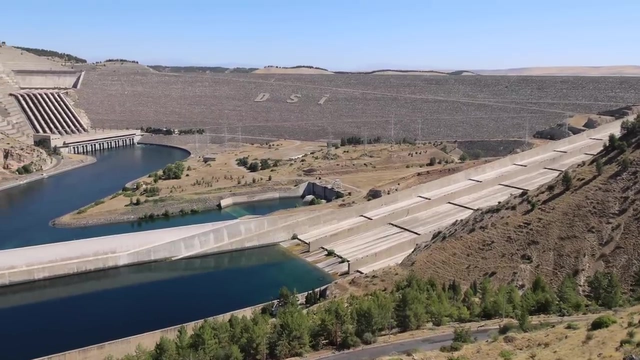 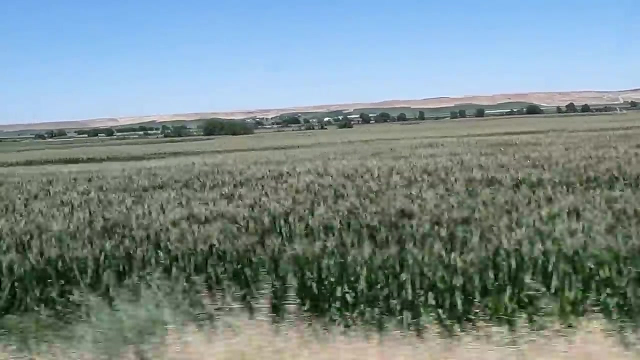 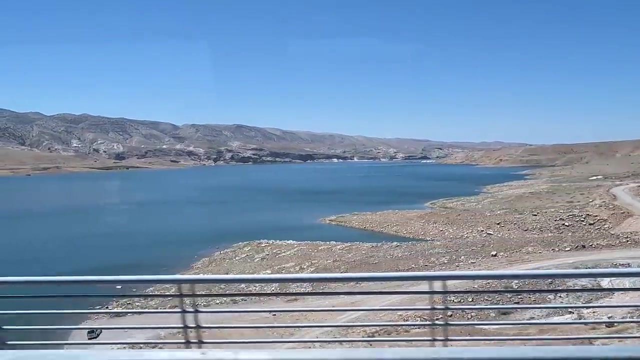 on Turkey's Kaban Dam in 1968. millions of litres of water quickly shifted into a torrent, inundating one of the richest archaeological landscapes in the world, Countless irreplaceable settlements and monuments disappearing under the flood. The first of many similar investments by the 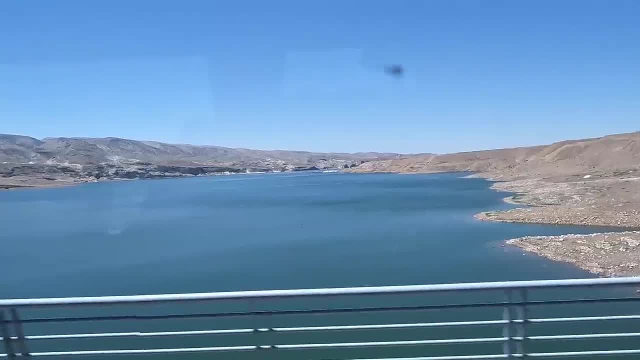 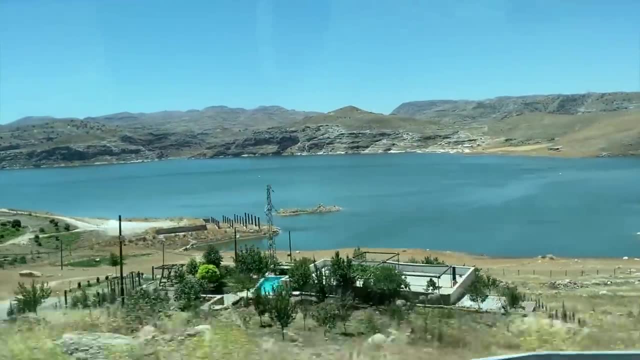 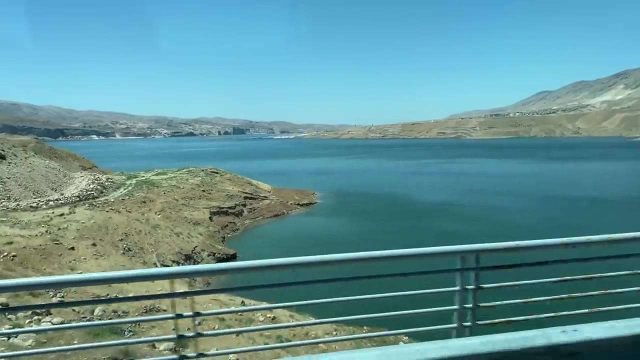 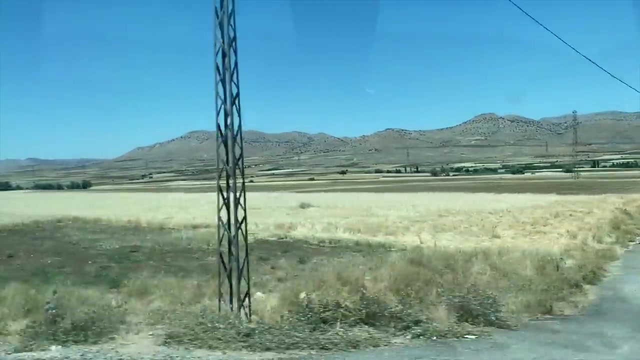 Turkish government in order to feed and water the tens of millions of people living in the dry southeast of the country. Though widely condemned internationally, largely by nations with plenty of drinking water themselves, Turkey's government was, then, far from a corrupt dictatorship, as in many places in the Middle East. 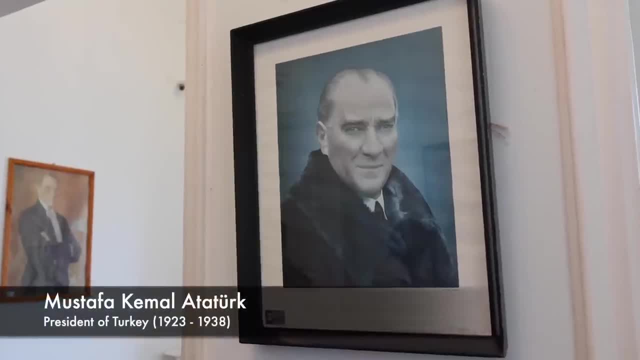 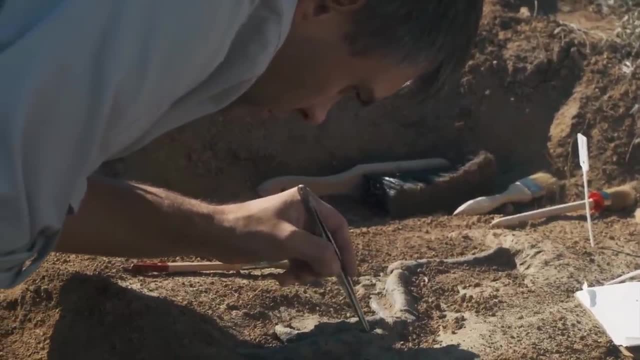 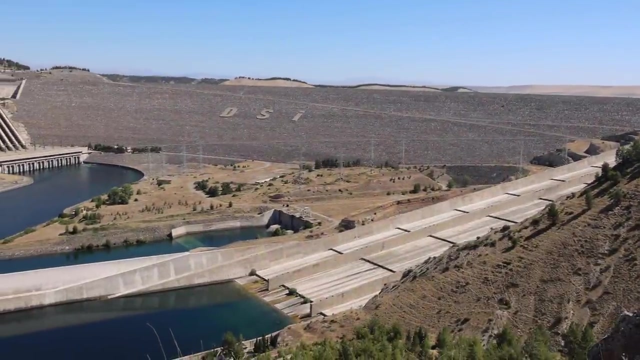 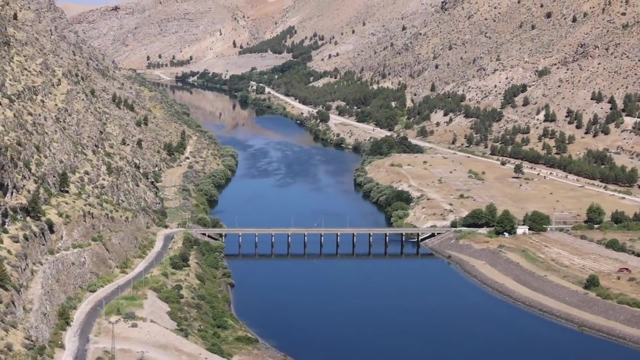 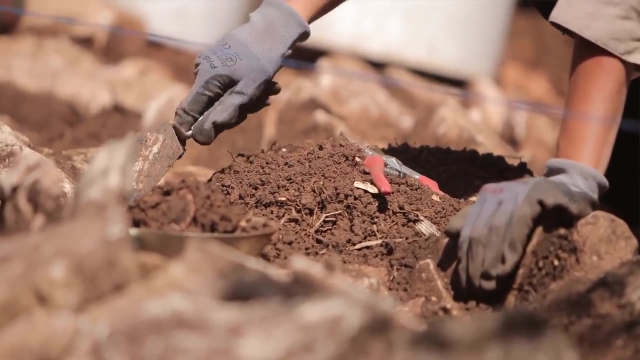 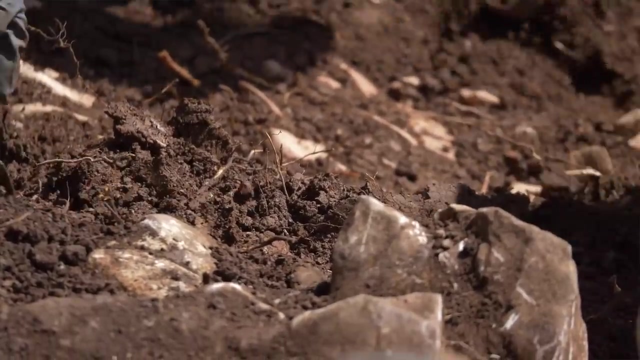 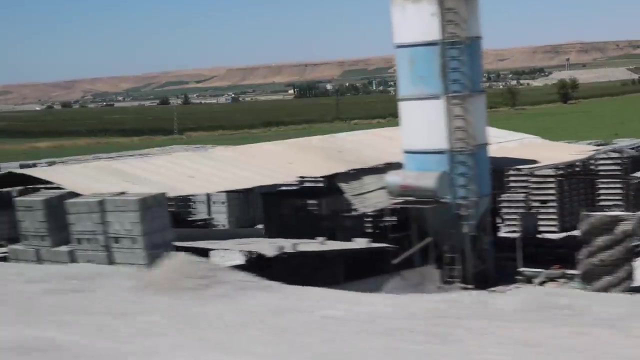 As a result of the reforms of Ataturk some decades earlier, a genuine homegrown desire to pursue archaeological investigation had been followed. The and an invasion of well-funded researchers from all over the world Invited in to help with this unique opportunity to rescue an entire region's 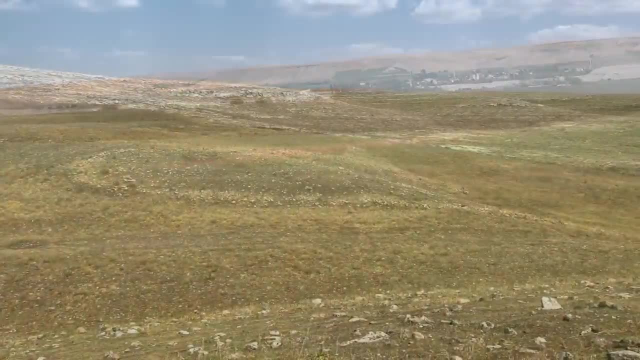 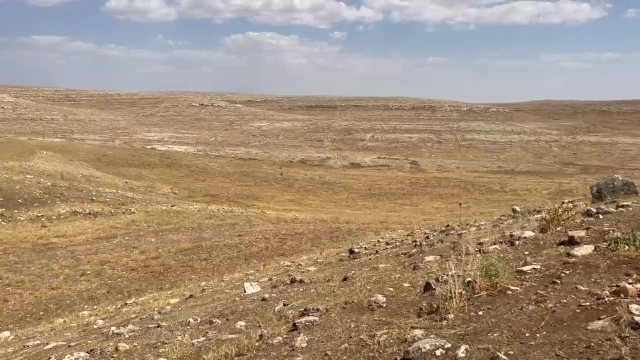 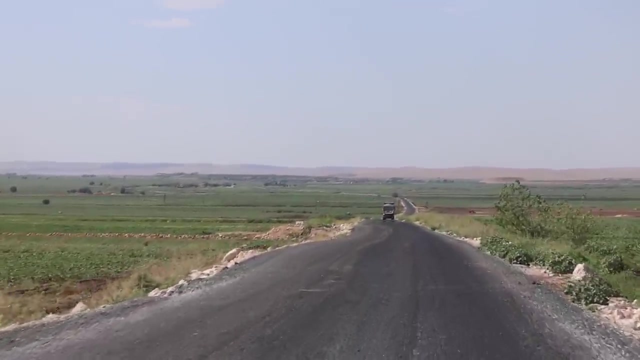 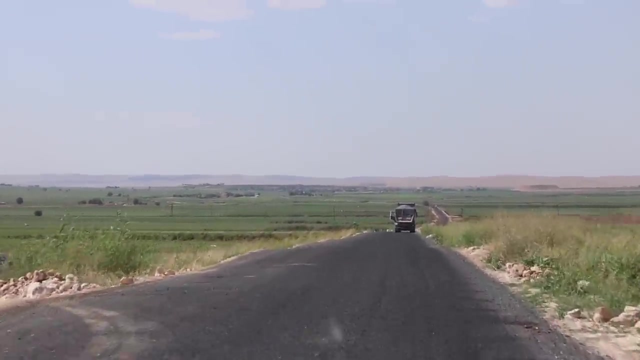 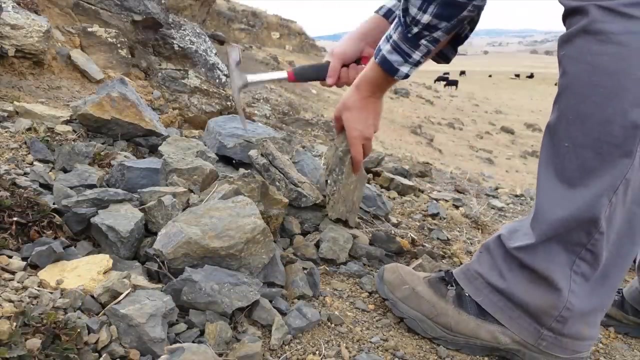 ancient past. It wasn't long before astounding discoveries began to be made. Four years earlier, in 1964, an American team working at the Neolithic site of Chianu had already pushed the clock back in the region by thousands of years, Under the supervision of Robert. 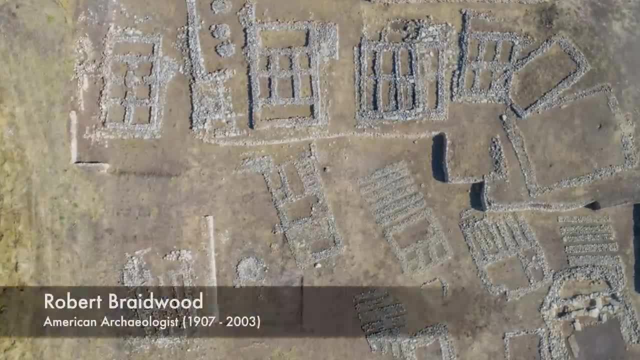 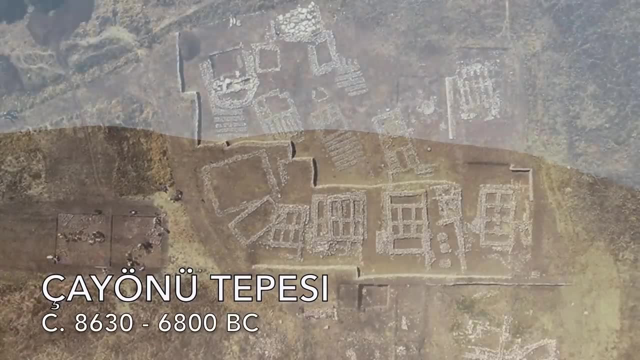 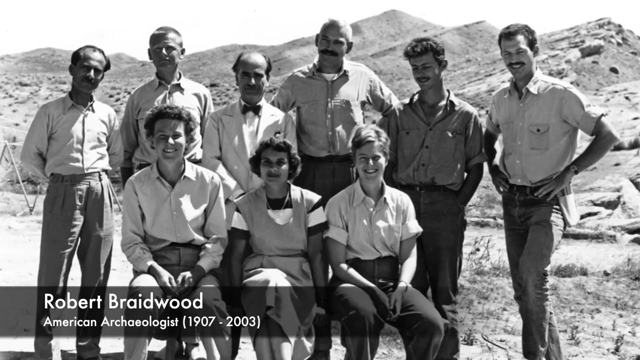 Braidwood the settlement had been found to date, to well over 10,000 years ago. Braidwood would continue to work at Chianu for another 14 seasons, But it was at Nvali Chori where headlines around the world would. 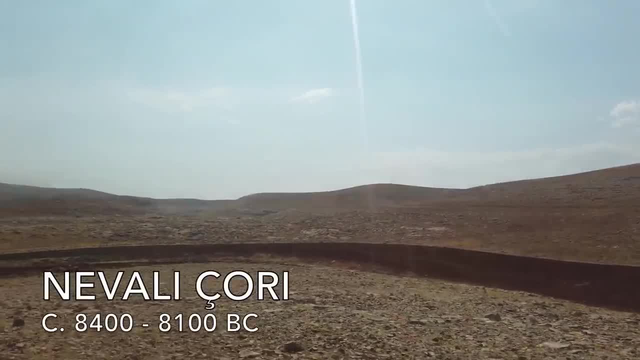 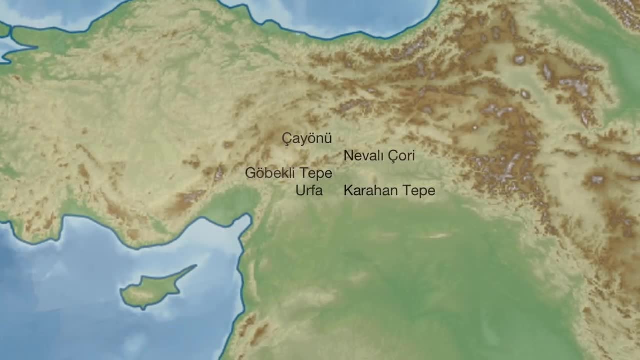 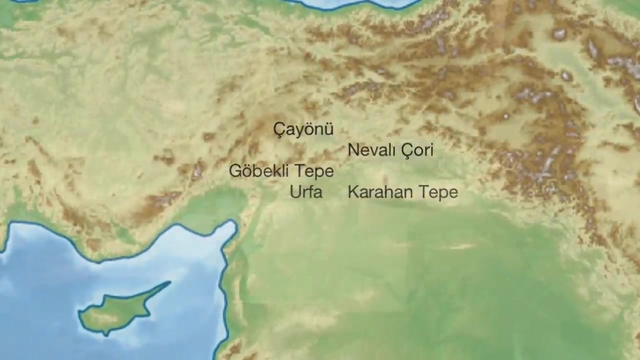 truly be made Hidden in a small side valley of the Euphrates, in a region already earmarked for submersion under another lake that was planned to be formed. In a region already earmarked for submersion under another lake that was planned to be formed. 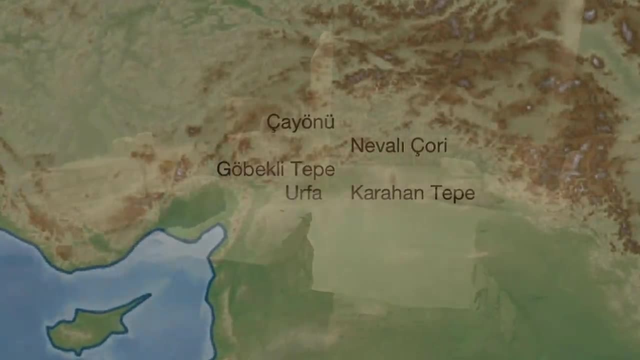 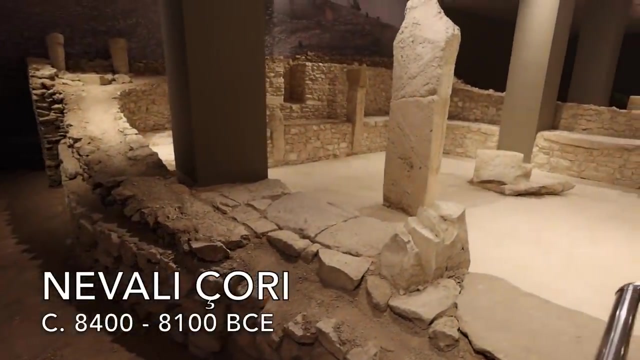 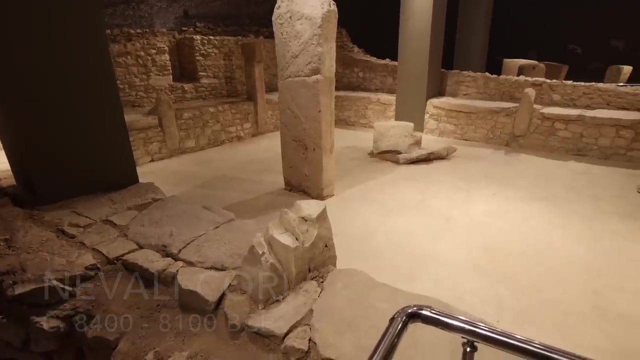 In a region already earmarked for submersion under another lake that was planned to be formed, Nvali Chori, translating rather ominously as the Valley of the Plague was initially investigated in 1979. At first thought to be early Bronze Age in origin. 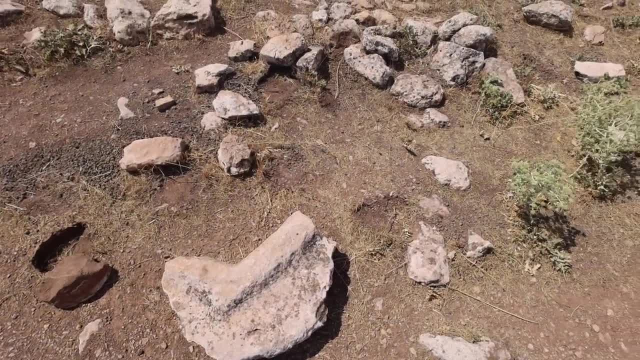 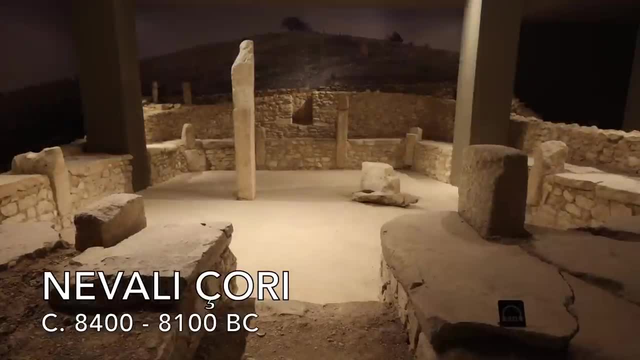 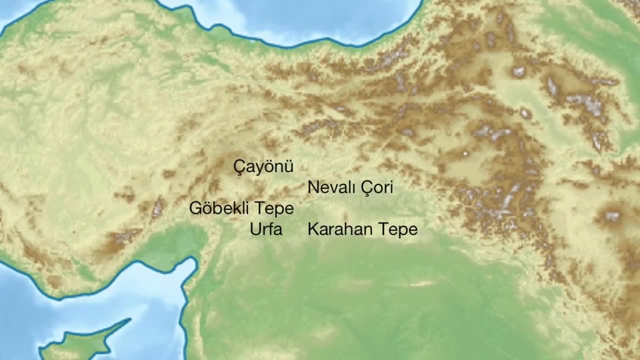 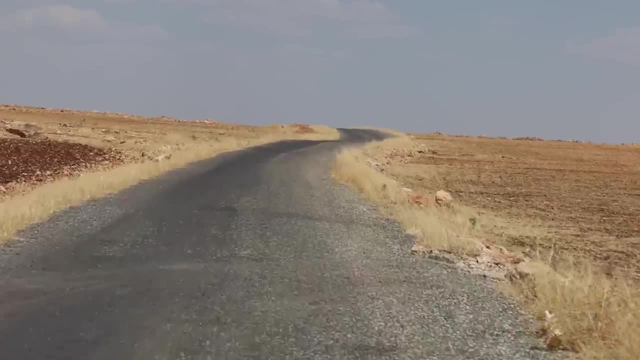 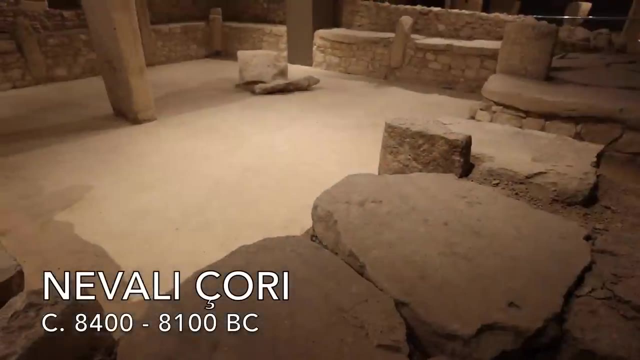 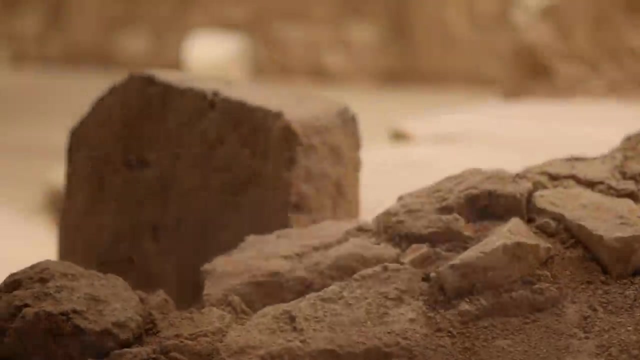 When excavations began at the early Neolithic site in 1983, it wasn't long before an unusually complex series of massive free-standing stone buildings began to be unearthed. began to be unearthed Initially known as the Roman Burial from 1987 onwards. 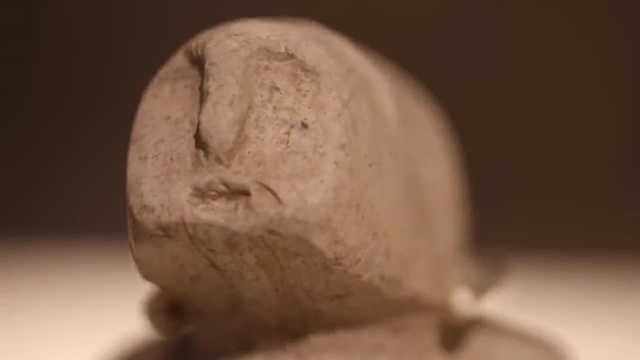 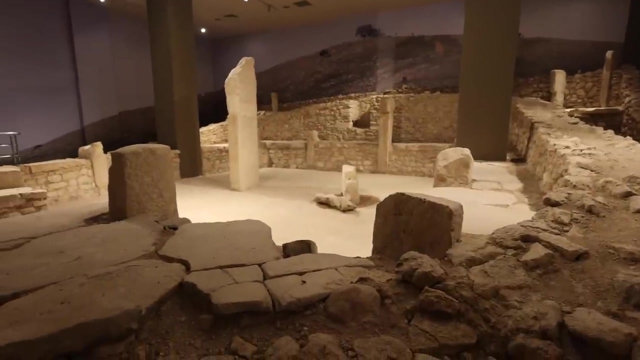 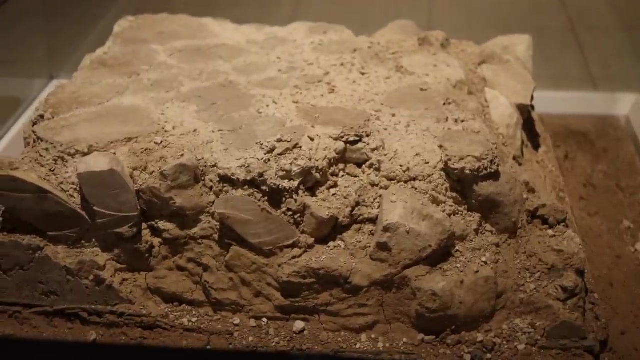 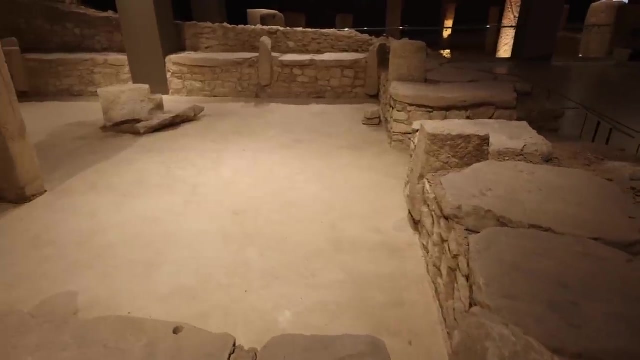 the plagues brought forth things never before seen by modern eyes. A terrazzo-floored building or enclosure began to be unearthed, Elaborately constructed with layers of burned lime, And then, as they dug ever downwards, one of the pillars turned out to be an. 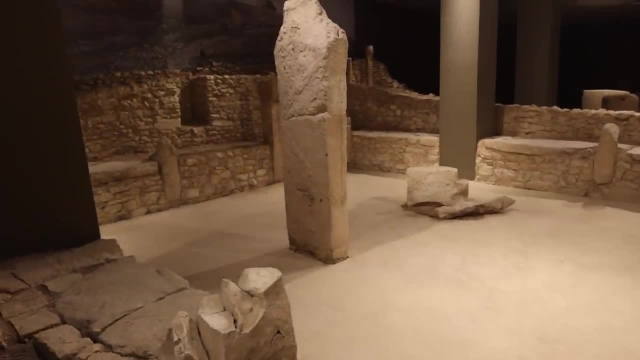 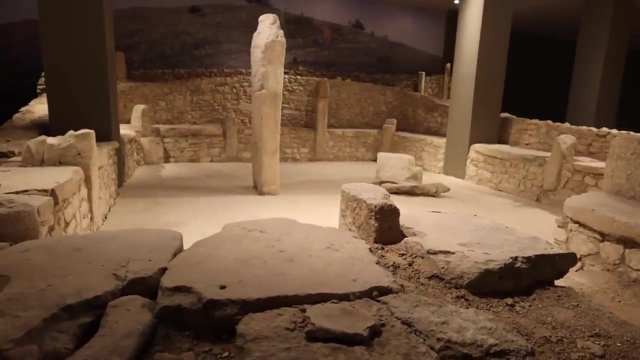 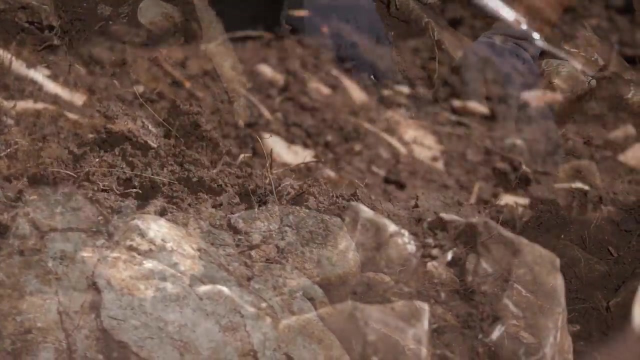 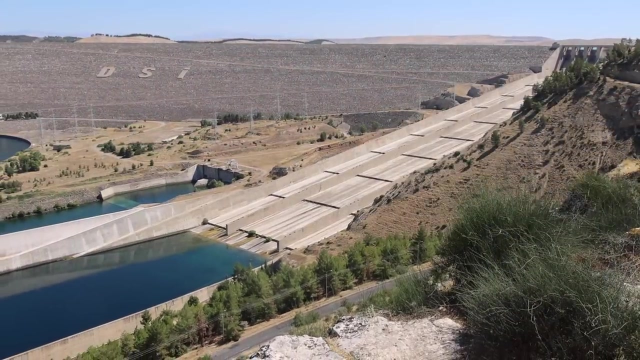 anthropomorphic being from an even earlier time, from an even earlier time. Unfortunately, its head was missing. its head was missing. The archaeologists were simply astonished, were simply astonished. And as the place disappeared under the waters of the Ataturk, 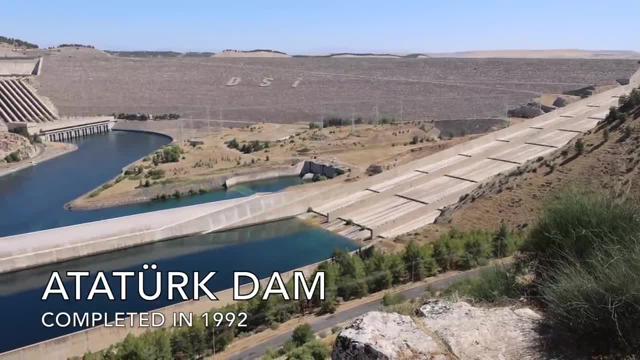 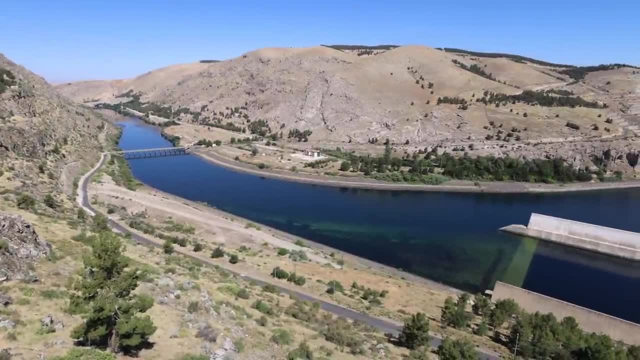 Dam in the winter of early 1992, Dam in the winter of early 1992, left to ponder the ancestors, gods or demons that had once called the place home. called the ancestors, gods or demons that had once called the place home. 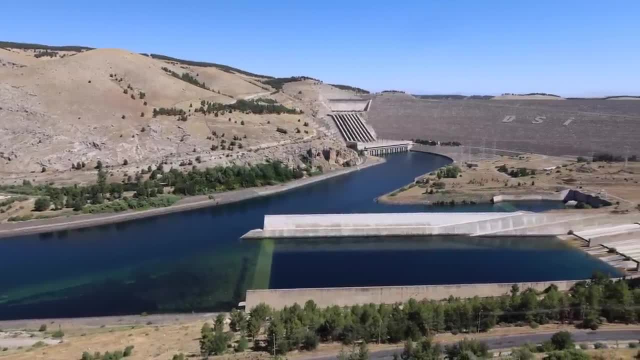 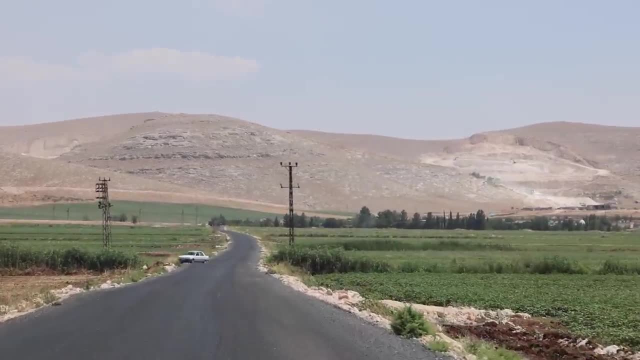 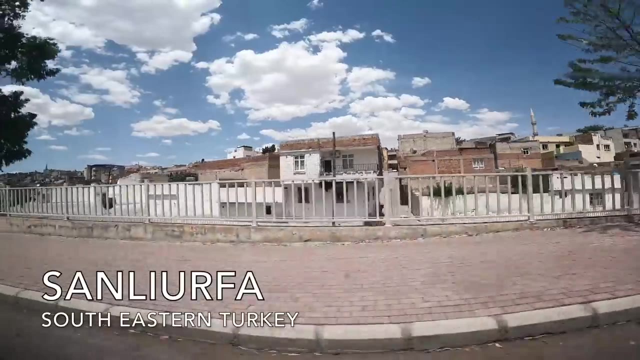 called the ancestors, gods or demons that had once called the place home. At around the same time, one of the German archaeologists working at Navali Chori working at Navali Chori would often make trips to the museum in Sanliurfa. 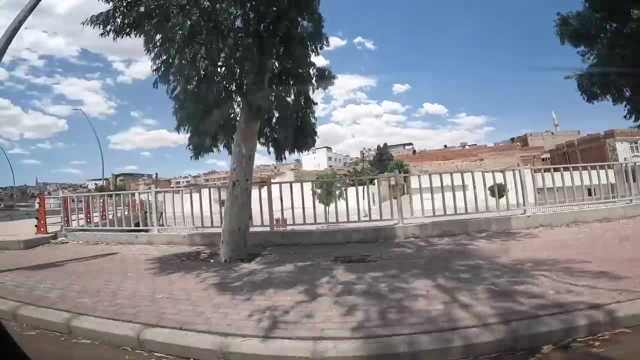 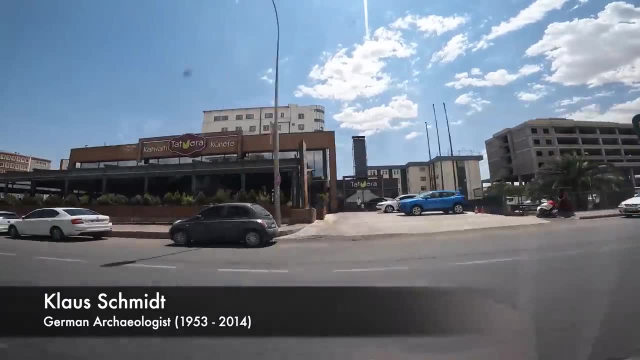 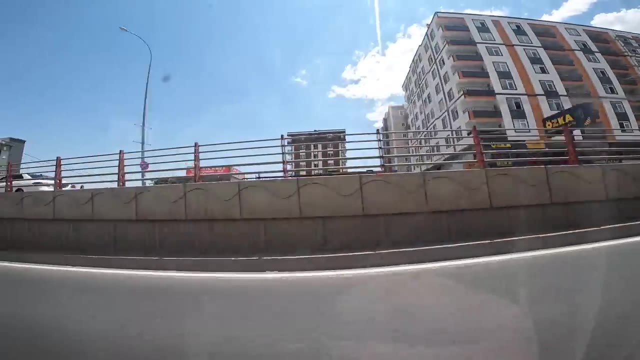 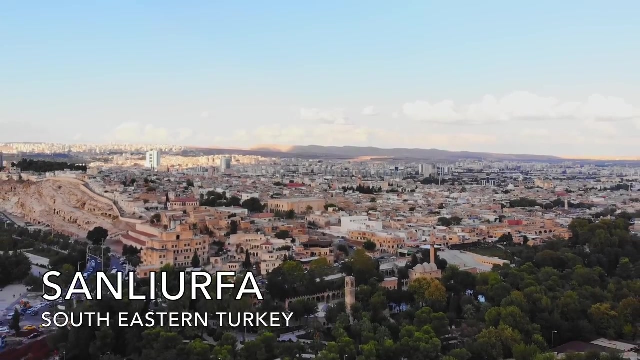 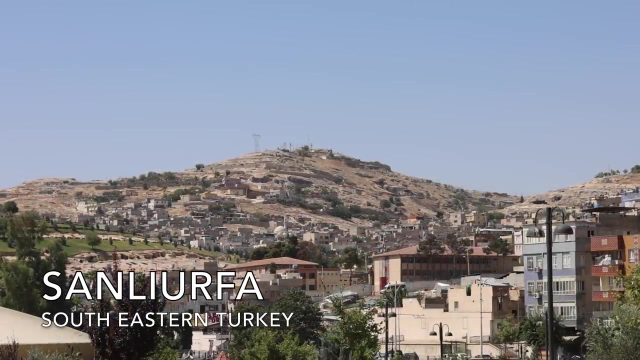 His name. His name was Klaus Schmidt, was Klaus Schmidt, And we will be hearing much more from him soon. much more from him soon. With a population of well over a million, one of the great cities in world history, Urfa, was given its 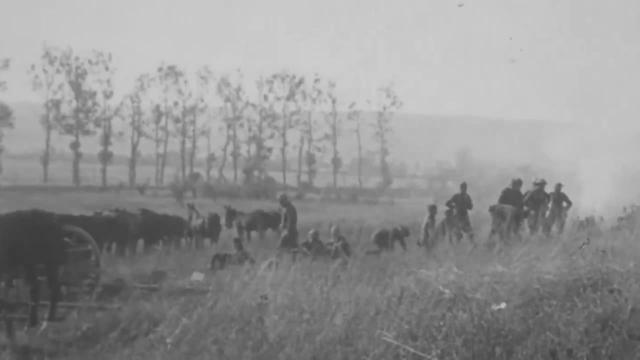 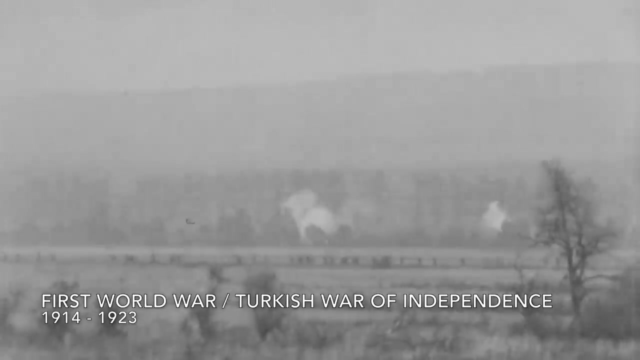 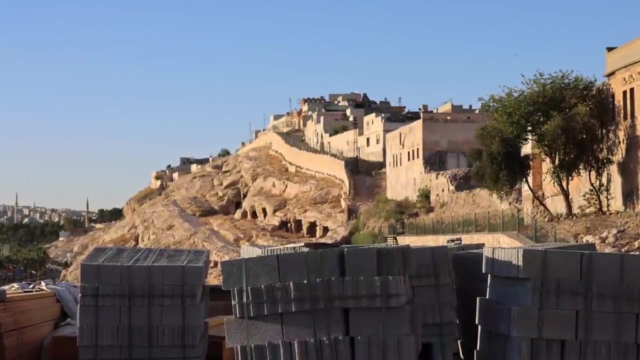 honorific title of Sanli, meaning honoured at the dawn of the 20th century after stalwart defences against the Russians in the turmoil of that age. turmoil of that age, But long before that it had a different name. 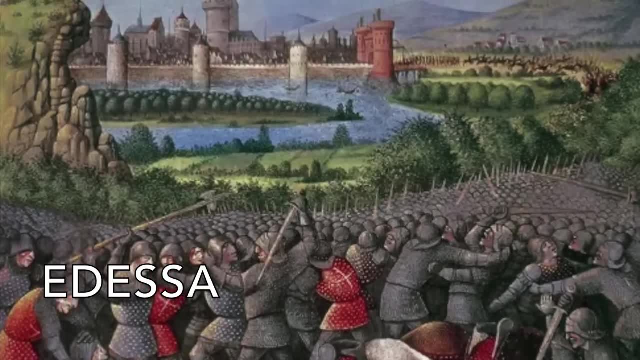 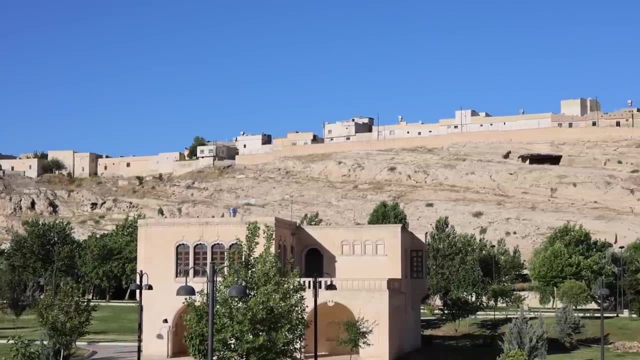 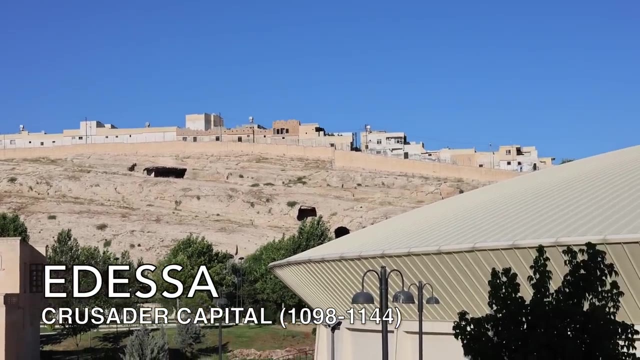 Odessa, Odessa. From this medieval powerhouse, the Oran Crusader lords had carved out a kingdom in the similarly chaotic 12th century. in the similarly chaotic 12th century, The city's fall had been the main catalyst for the Second Crusade. 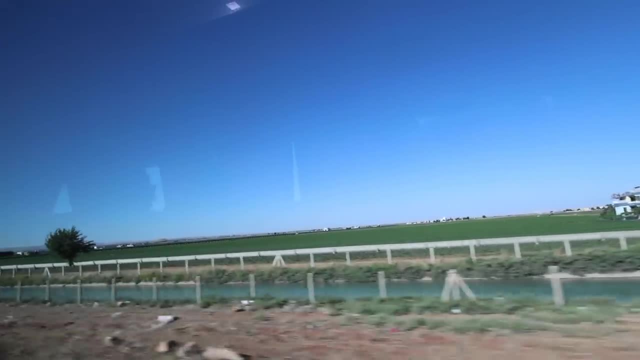 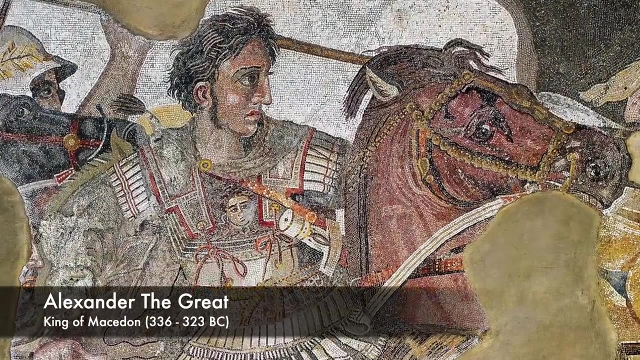 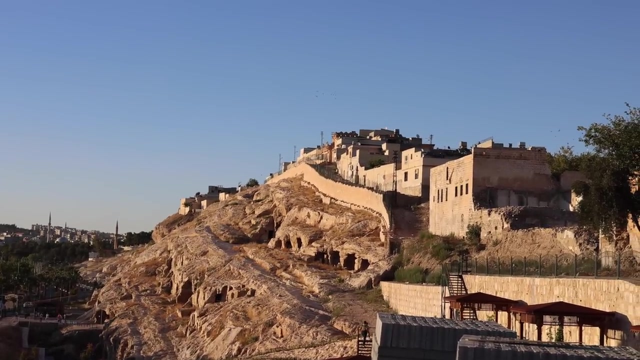 The name itself was brought by Alexander the Great during his incessant march to the ends of the earth, during his march to the ends of the earth, Given by his soldiers to remind them of the Odessa in their homeland of Macedon. But even in those days, 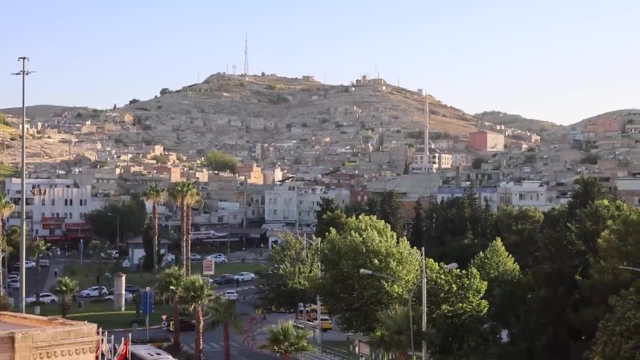 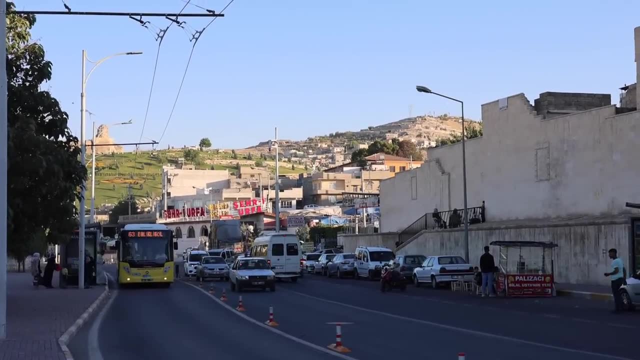 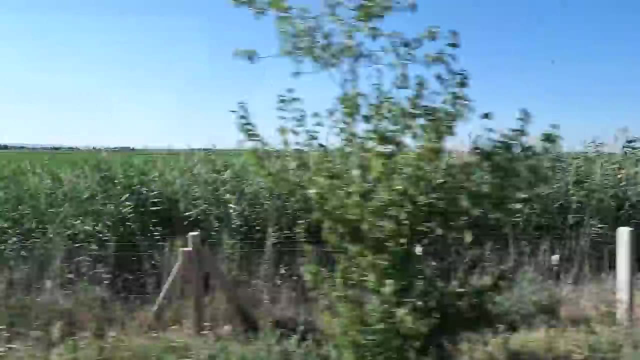 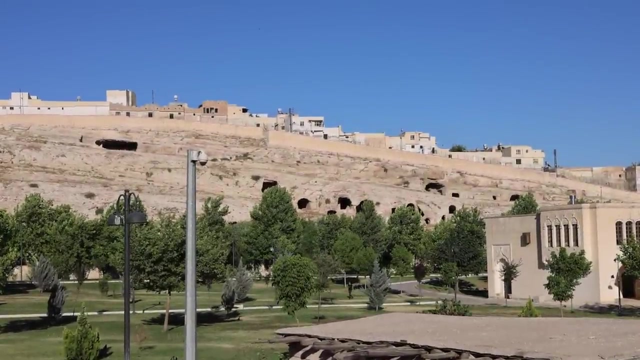 the place was already old. Situated around a number of karstic springs, rich irrigated farmland stretches out in all directions. stretches out in all directions, Just as it has for millennia, Just as it has for millennia The great rain providing chain. 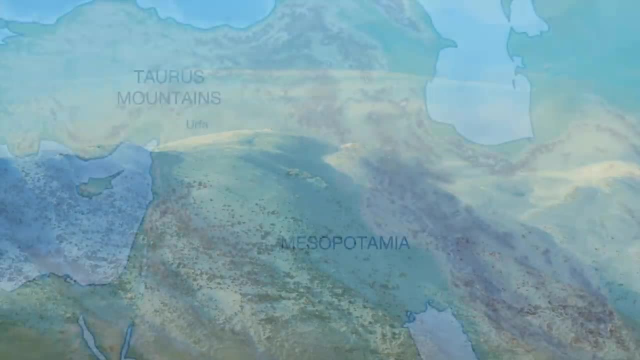 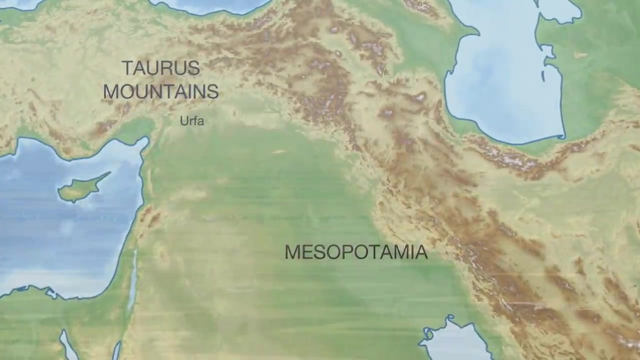 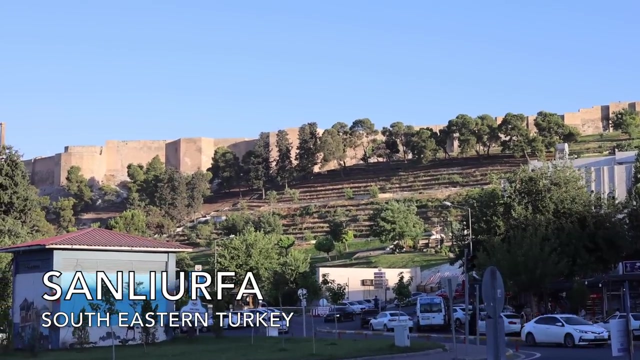 of the Taurus Mountains and the Anatolian plateau beyond, rising to the north At this gateway to the rolling plains of Mesopotamia. rolling plains of Mesopotamia. rolling plains of Mesopotamia. The myths and legends associated with, 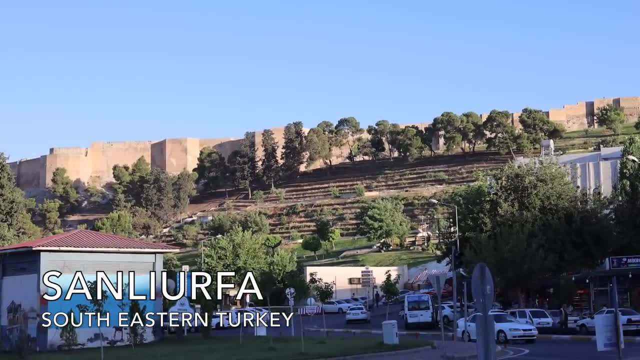 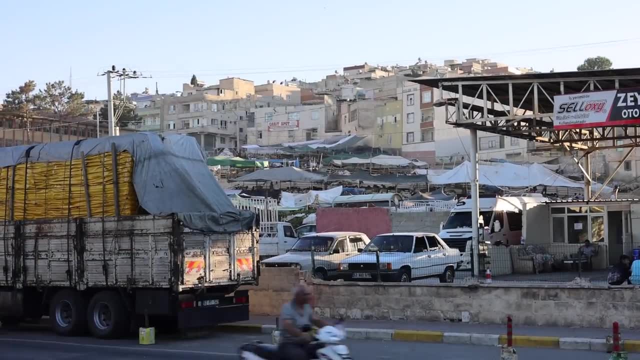 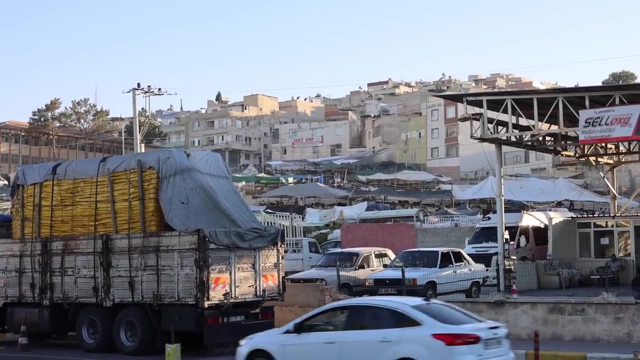 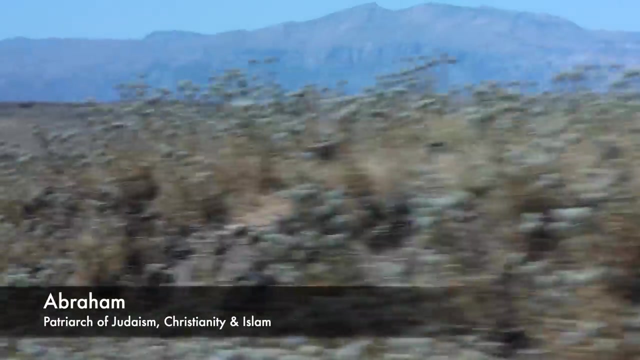 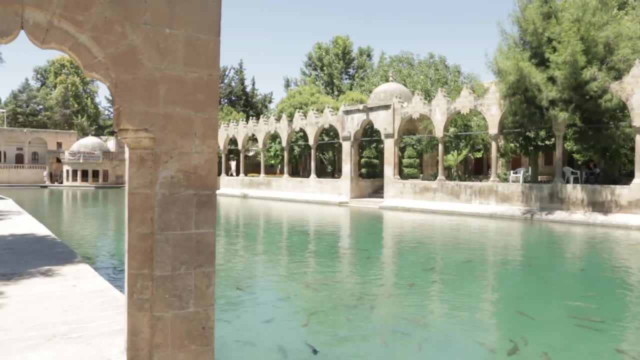 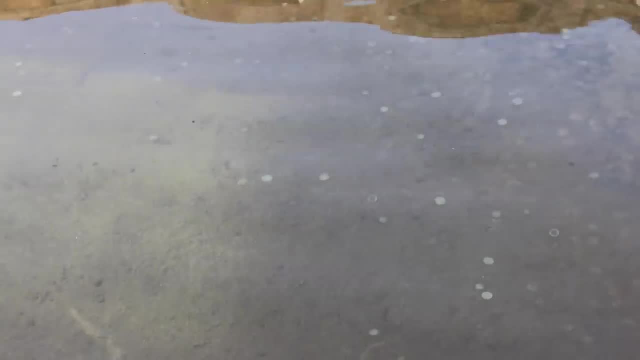 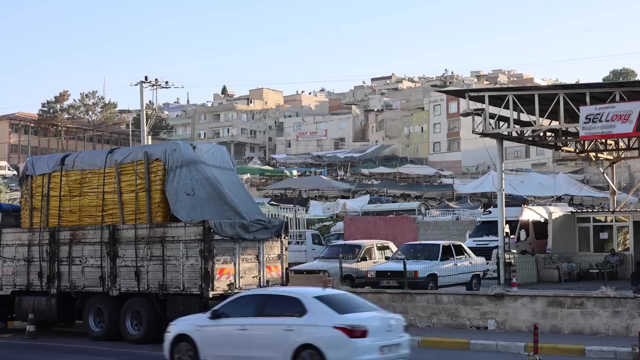 the holy springs here. the holy springs here. Just how long people had lived around those pools at the centre of town At the time, no one could say. But one thing is always abundantly clear. But one thing is always abundantly clear. 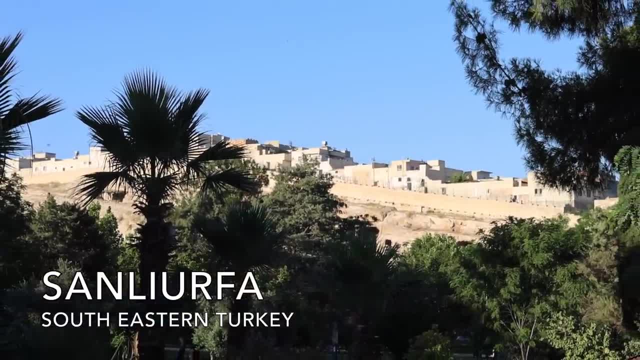 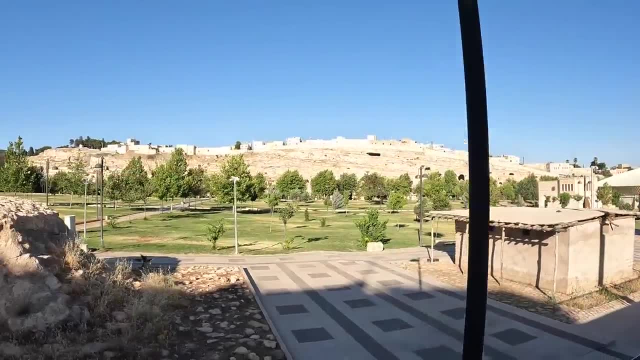 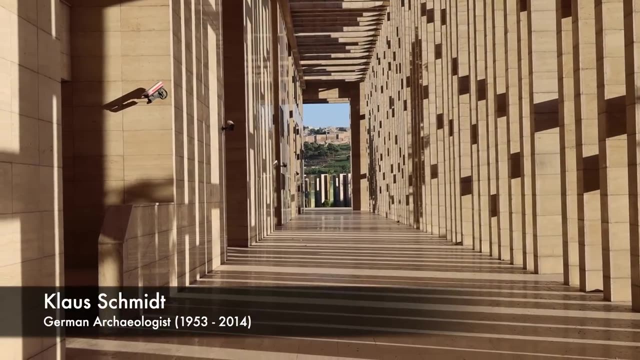 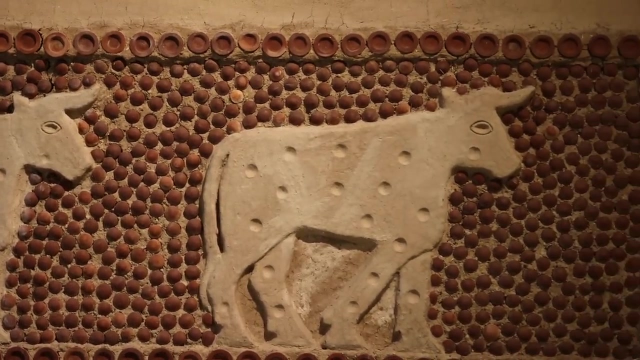 Urfa has lived many lives, many lives, many lives. On one fateful visit to the museum in 1994, to the museum in 1994,, as usual, Klaus Schmidt perused the storerooms of the influential institution, of the influential institution. 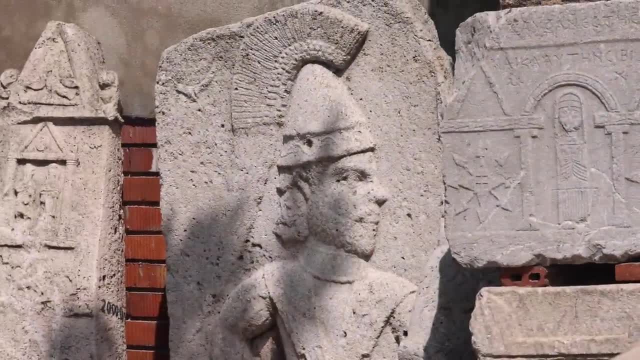 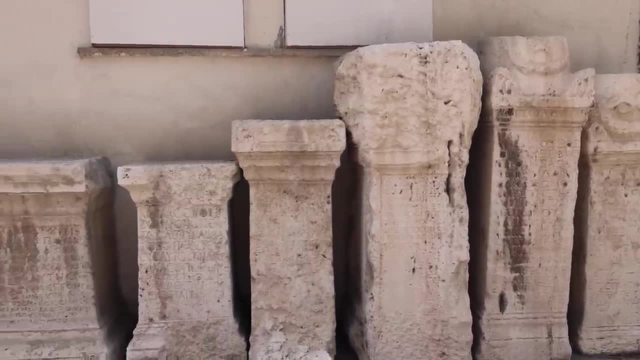 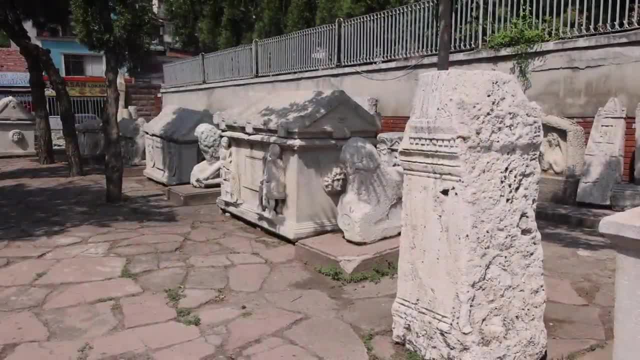 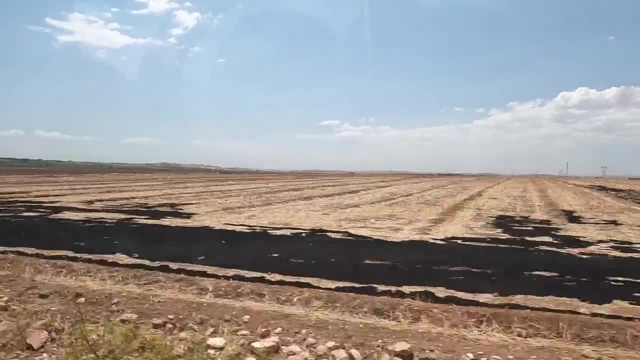 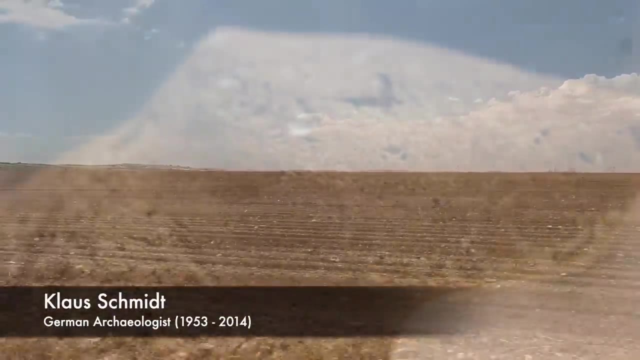 everything in his life was about to change, was about to change. Now armed. Now, armed with the newly gained knowledge of, he saw something in the Urfa museum that shouldn't have been there. that shouldn't have been there: Two naturalistic statues. 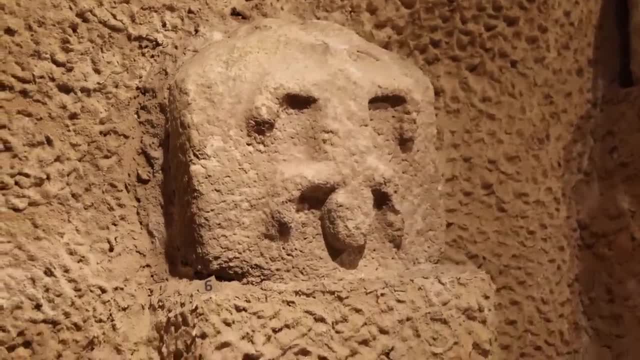 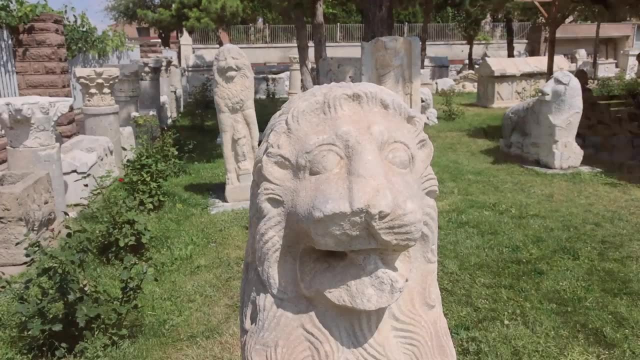 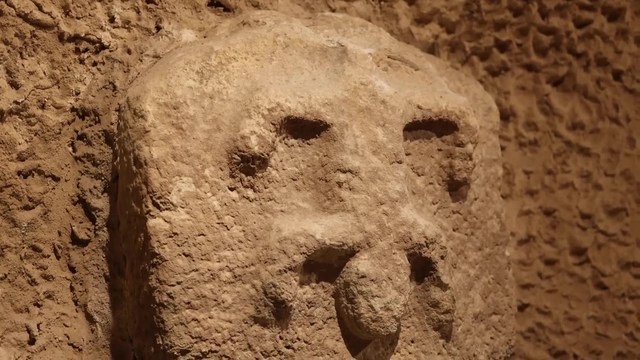 Two naturalistic statues: Reptilian in form. Reptilian in form Erroneously categorised as Byzantine. Erroneously categorised as Byzantine. Schmidt immediately knew better. Schmidt immediately knew better, Recognising similarities with vastly more ancient sites. 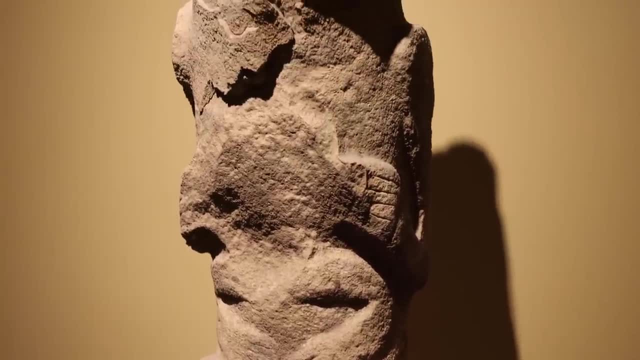 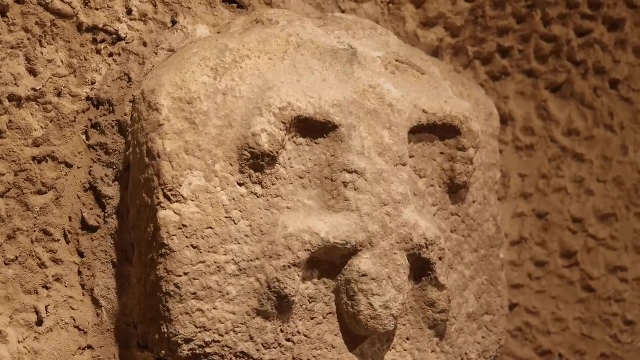 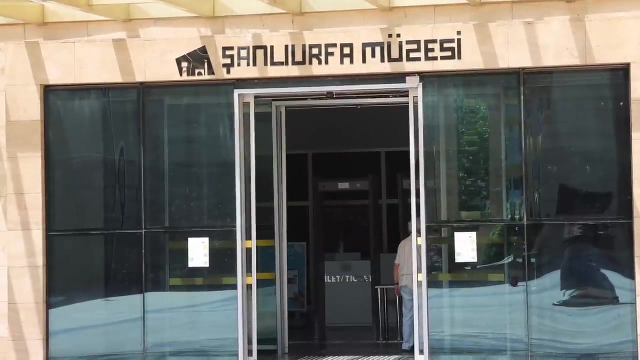 he'd been working on, with vastly more ancient sites he'd been working on, But how had they got to the museum And where had they come from to the museum? Thankfully, someone at the museum knew exactly, And just a few hours later, 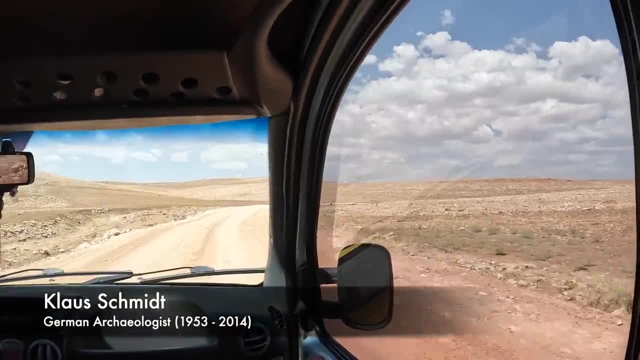 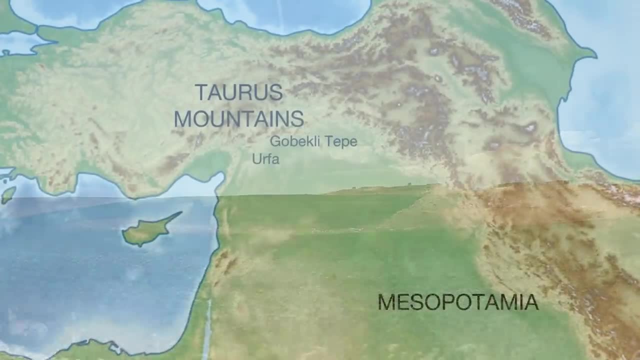 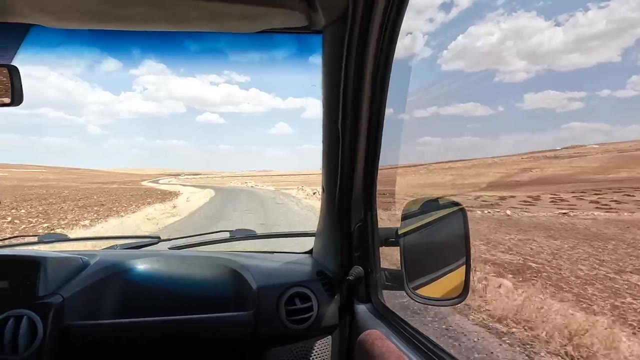 Schmidt, along with two colleagues, were in a taxi, were in a taxi Heading along dirt roads, Heading along dirt roads to the hill country northeast of the city, To an obscure plot of land on a desolate rock known as Potbelly Hill. known as Potbelly Hill. 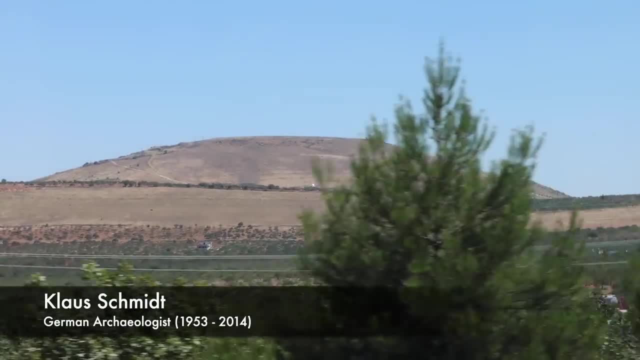 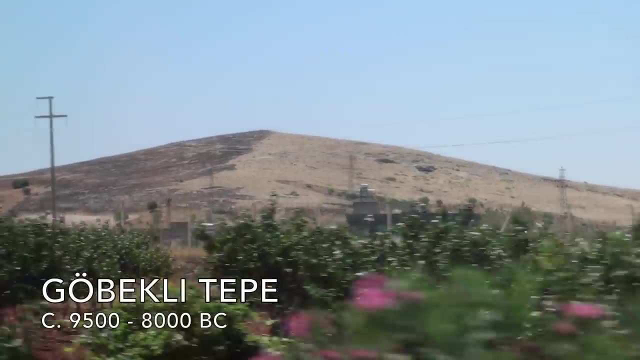 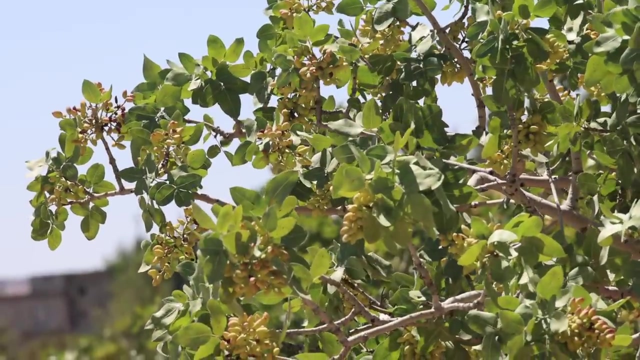 And, as Schmidt would soon find out, its Turkish name, Gobekli Tepe, was already known to archaeology, was already known to archaeology. Seven or eight years earlier, local landowner Ibrahim Yildiz and his son Mahmut had been clearing scrubland. 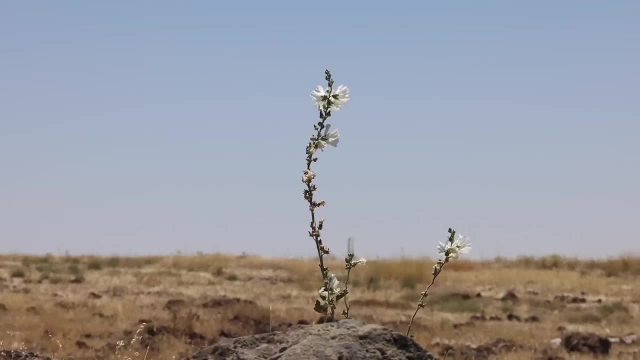 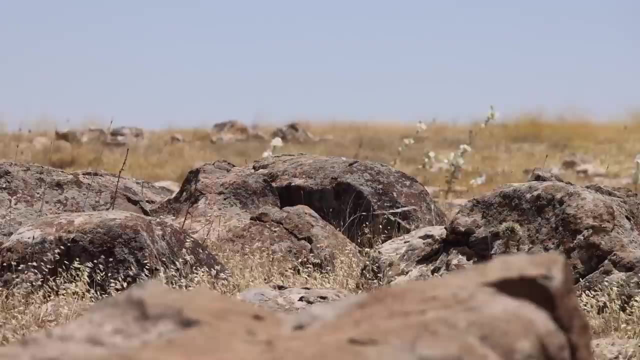 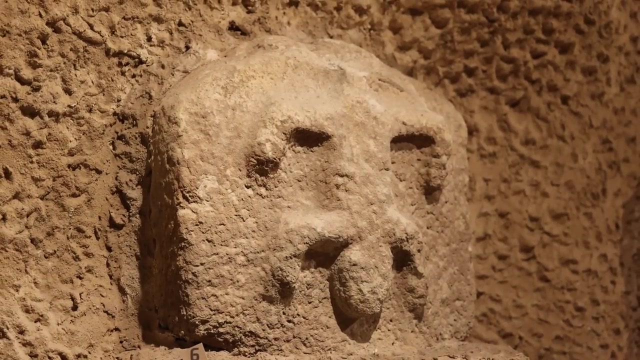 up on the hill overlooking their property when one of their spades hit something solid. hit something solid: Strange statues. Strange statues were then pulled up out of the ground, But there was a problem In the confused days that followed, as one of the statues- 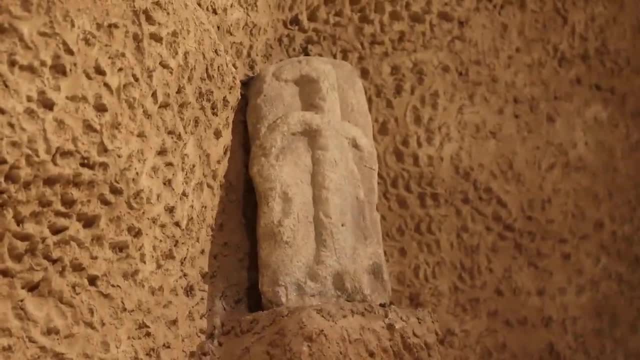 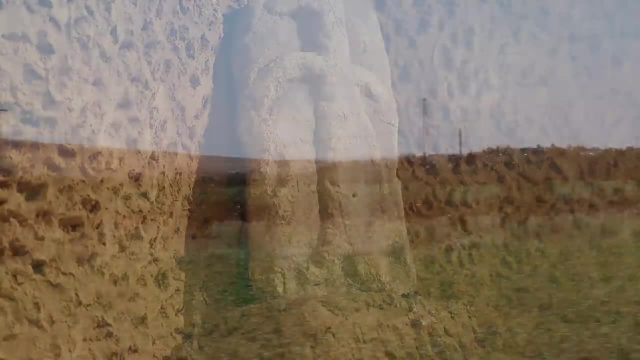 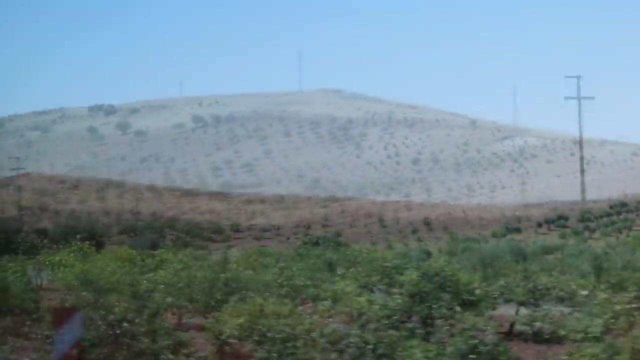 clearly had a large penis showing the two men kept them hidden as a steady stream of villagers came by to see the discovery, Not wanting to be perceived as idolatrous and bring shame upon their family. eventually, the local Imam came to see the finds. came to see the finds. 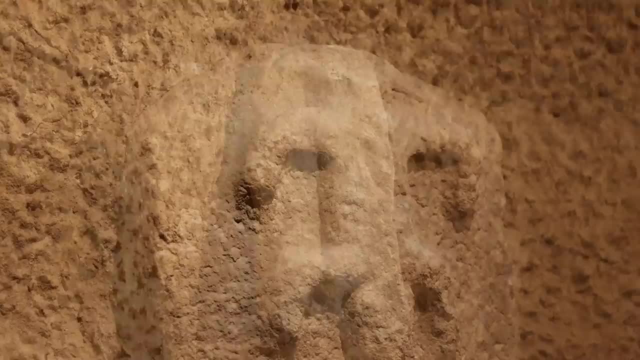 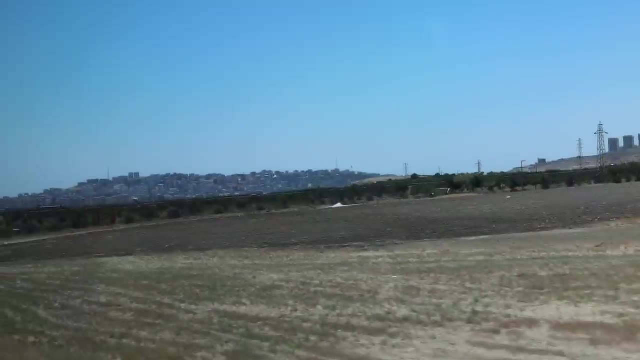 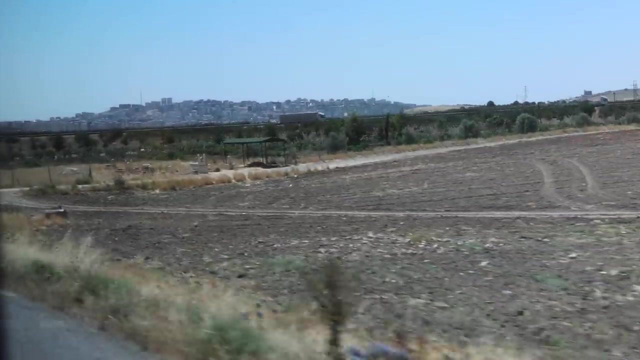 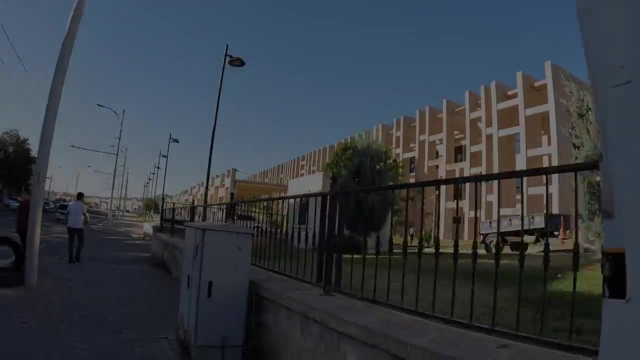 Far from chastising the men, recognising the potential significance of the finds, he encouraged the two farmers to take them to the Urfa Museum, Heading by horse cart along the old road to the west. once the two men arrived, the museum manager politely informed them. 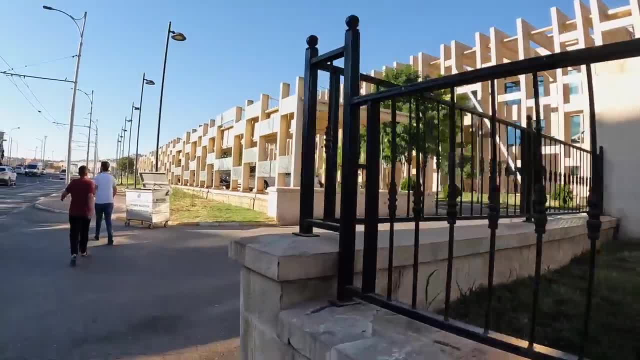 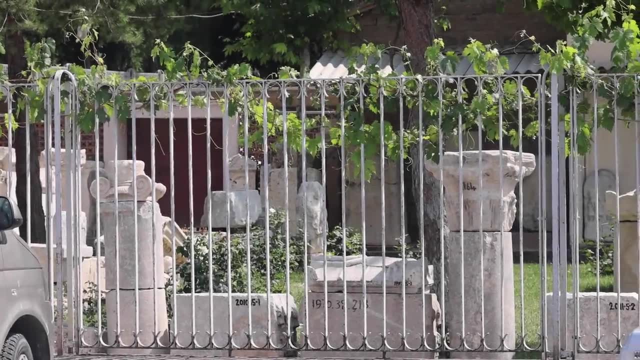 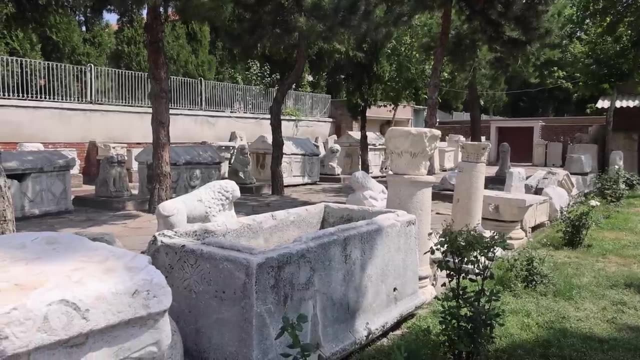 the pieces were, regrettably, not very old or particularly significant. not very old or particularly significant. Demoralised thinking: the journey had been for nothing. in order to not have to pay for another cart ride home, they left the pieces in the museum garden. 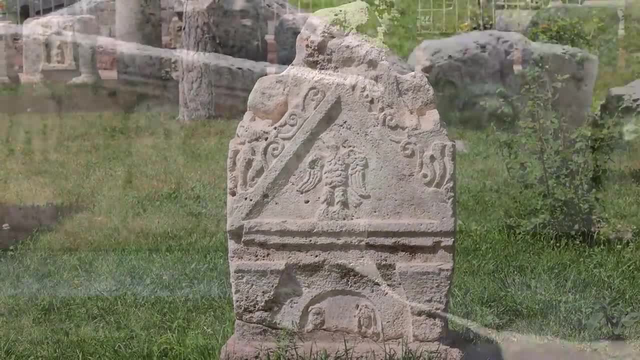 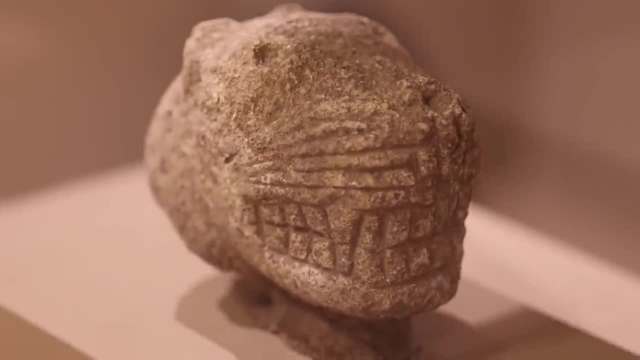 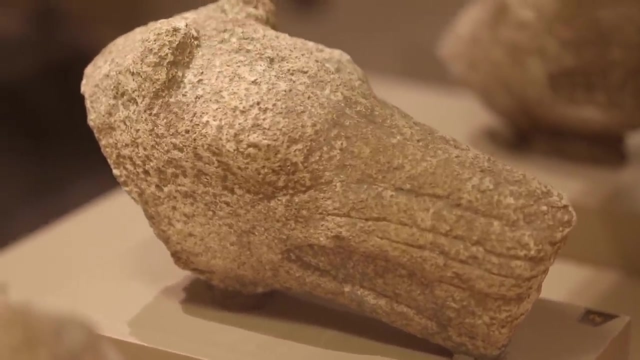 in the museum garden. No blame should be placed on the museum staff, however, nor the farmers, for at the time nothing of the sort had ever been found before. nothing of the sort had ever been found before, And this wasn't the first time. the significance of Gobekli Tepe. 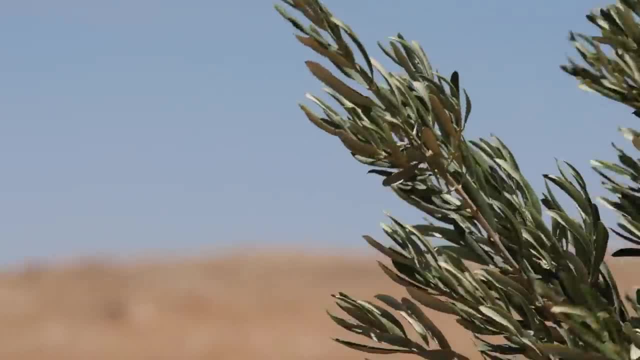 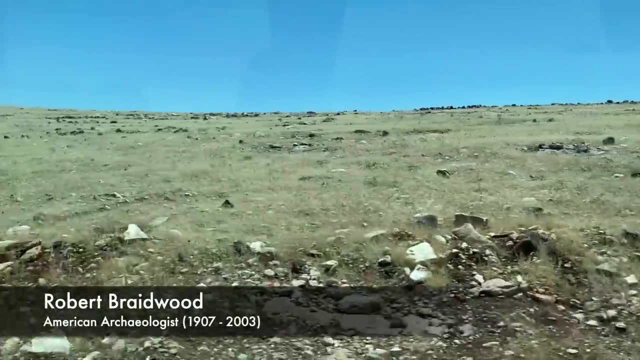 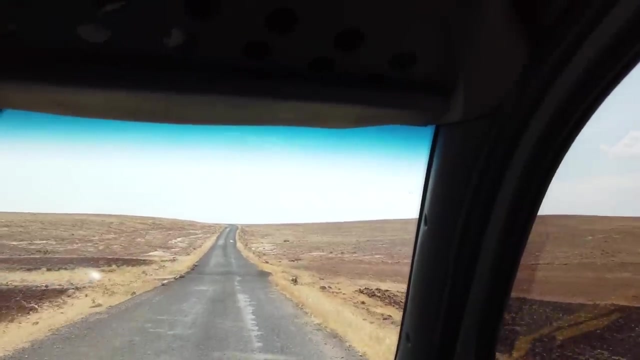 had been missed, had been missed Close to 30 years earlier in the 1960s. close to 30 years earlier in the 1960s, during Robert Braidwood's initial work at Cheanu- another American archaeologist, another American archaeologist. 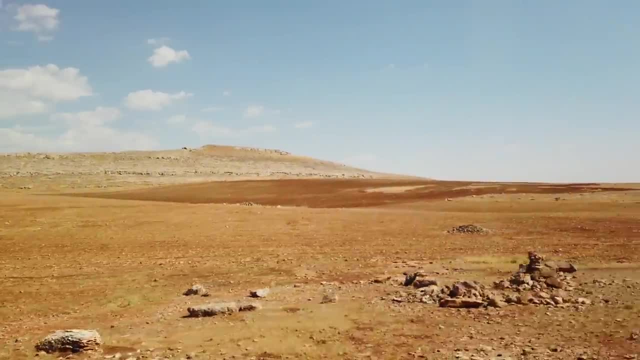 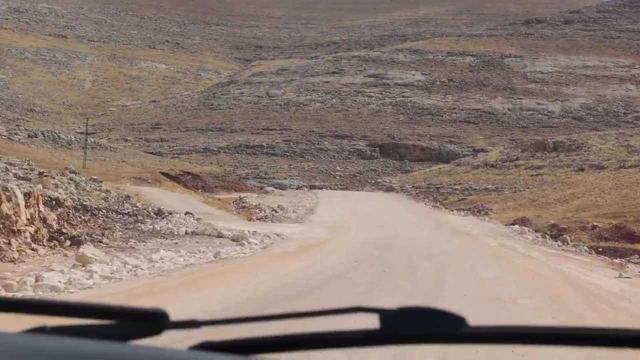 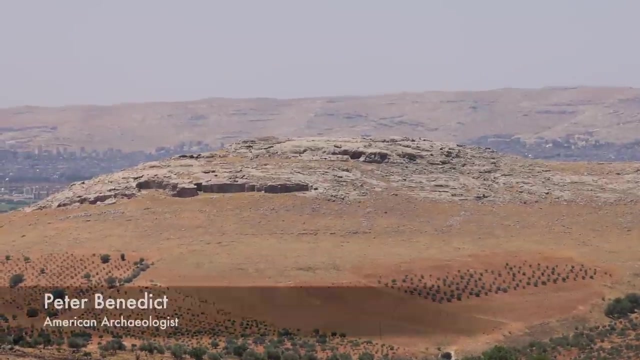 had scoured the region for similar sites, for similar sites, And though his ensuing report, dating from 1963 until 1972, ultimately missed the true significance of the place, Peter Benedict had spent quite some time at Gobekli Tepe, quite some time at Gobekli Tepe. 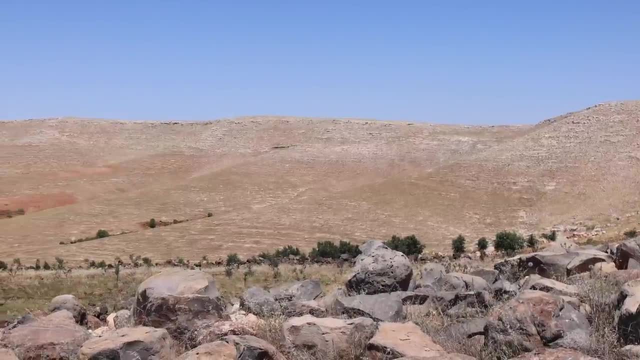 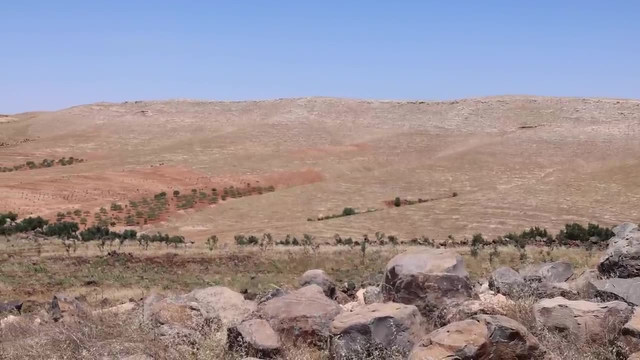 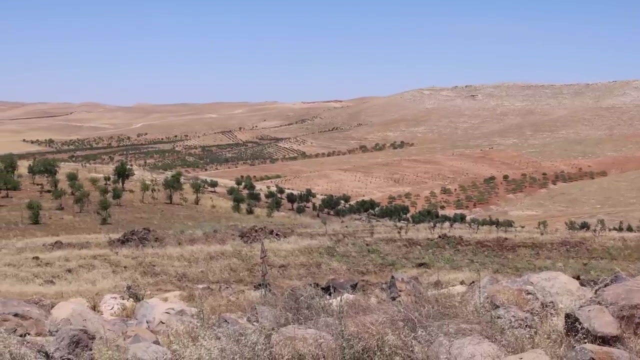 amidst a vast carpet, amidst a vast carpet of thousands of flintstones gleaming under the scorching sun, he'd found broken pottery pieces, flint blades and stone artefacts, many of which had been piled up by farmers over the span of decades, if not centuries. 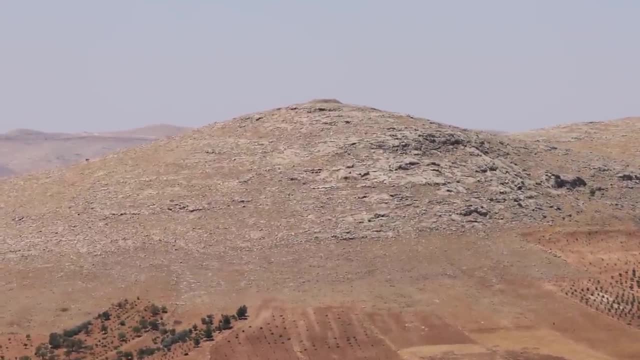 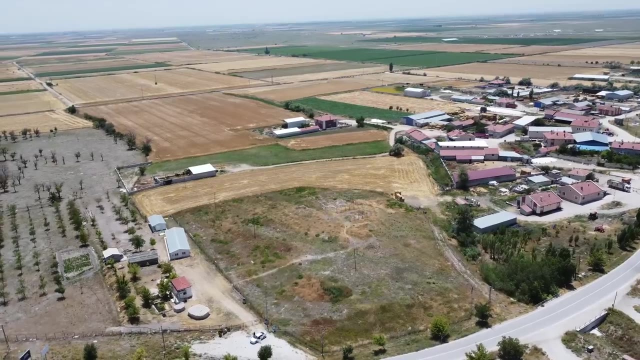 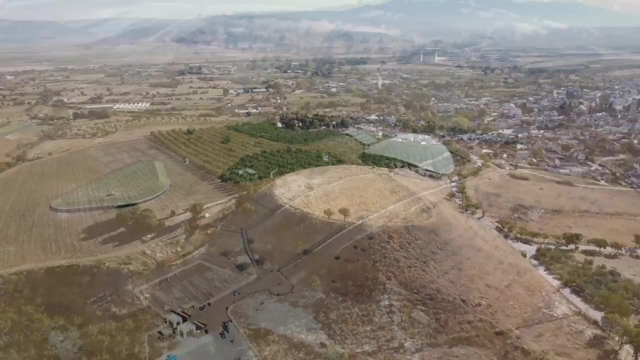 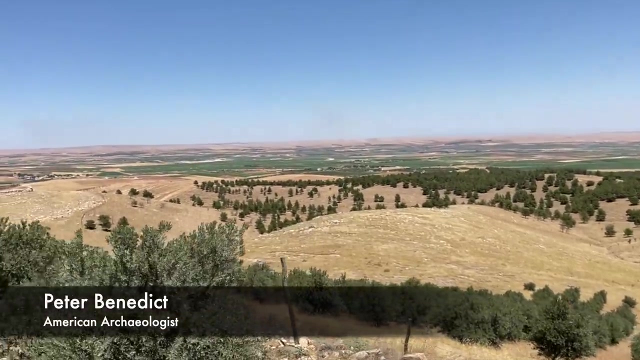 if not centuries. And yet Gobekli Tepe was just one tell amongst thousands, Curiously in the shadow of a great mulberry tree rising from the crest of the hill. Benedict wrote of locating a cemetery site, one which has never been found. 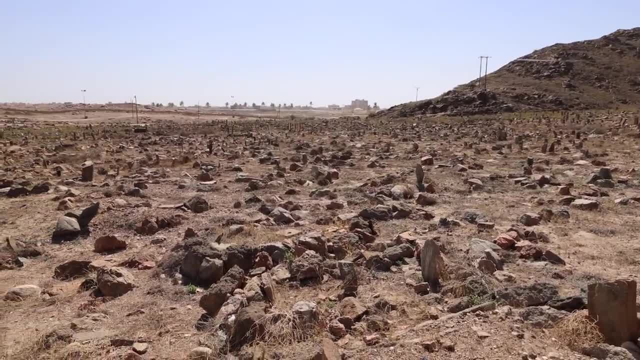 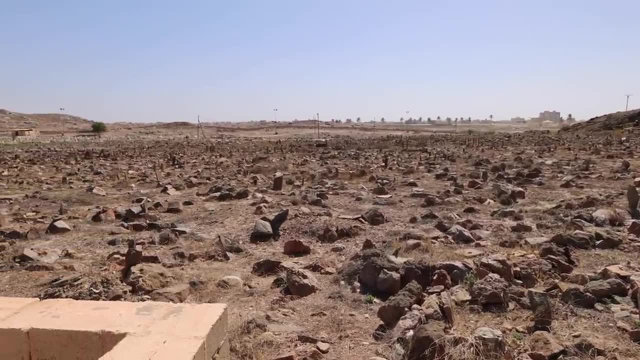 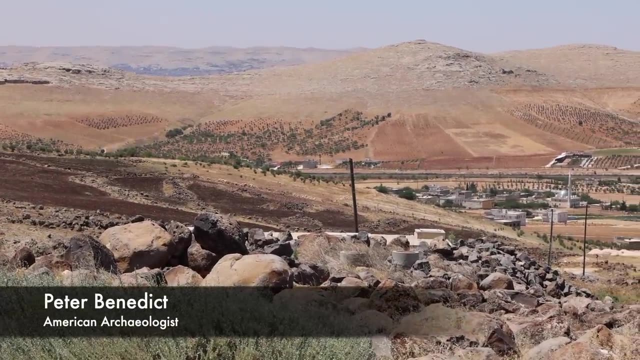 Islamic burial grounds are, of course, taboo for archaeologists, which could be the cause of him writing the place off for further investigation. It simply didn't cross Benedict's wildest imagination that practically the entire hill could be a great man-made tell dating from the pre-pottery. 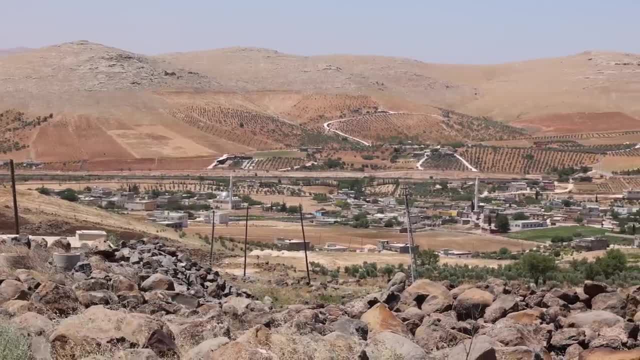 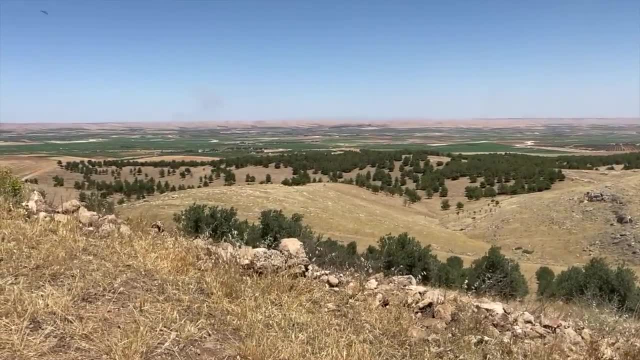 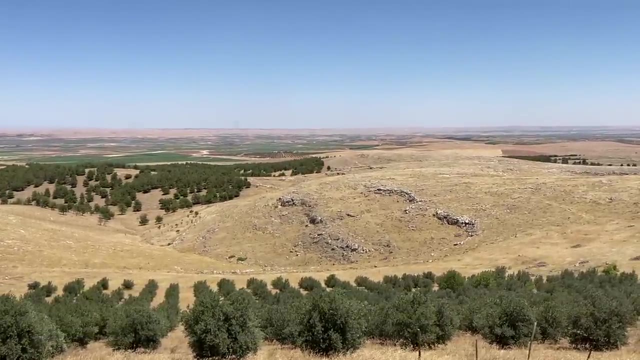 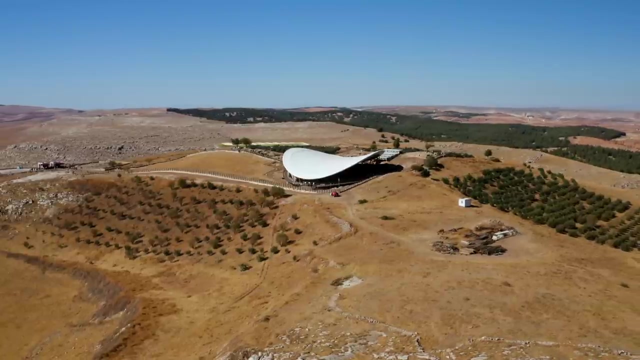 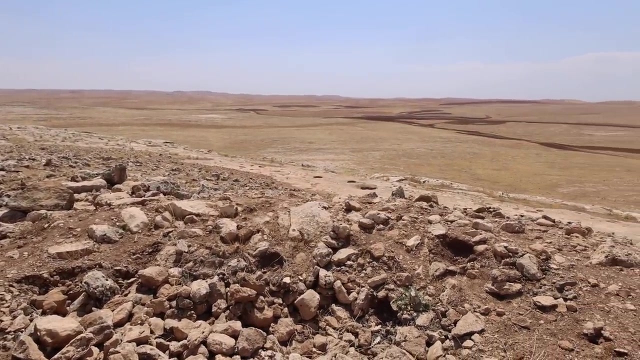 Neolithic Built up from the refuse of thousands of years of occupation. But when Schmidt arrived in 1994, it wasn't long before he made that exact conclusion. Far from a cemetery site, the half buried stones on the top of the hill in the process of being gradually. 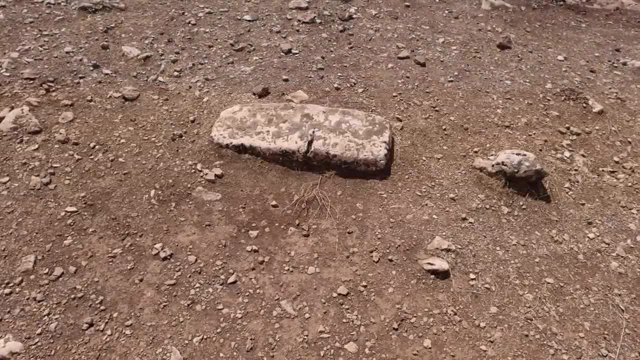 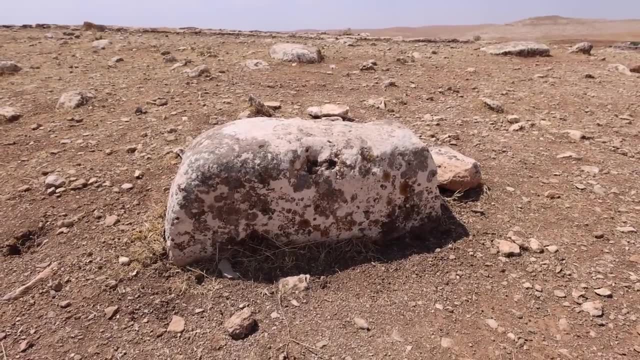 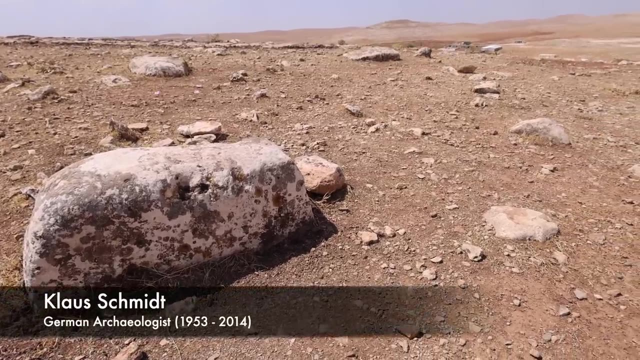 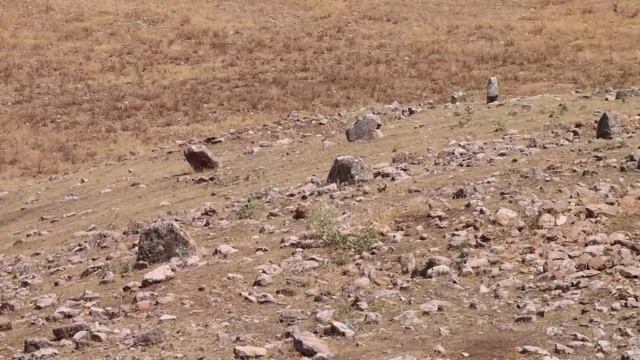 dug out by local farm workers were the very same style of T-shaped pillars previously found at Nvali Chori, But here they were everywhere he looked. With just a little trial digging, artifacts too could be pulled out easily from the ground, Just like the ones. 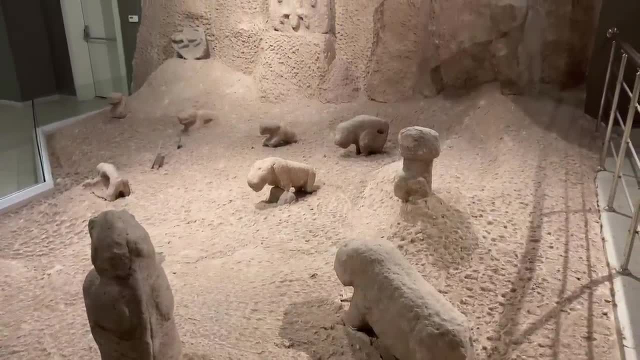 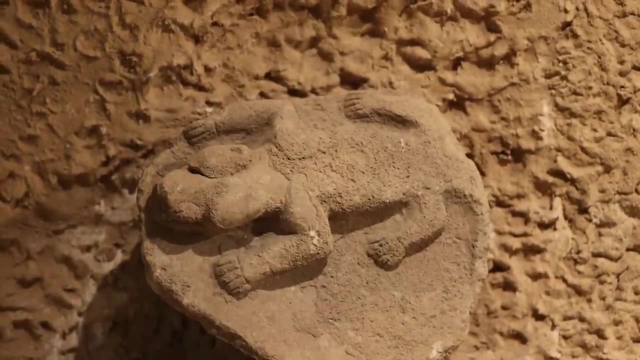 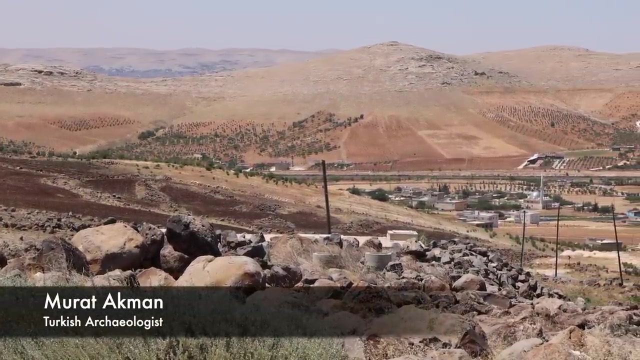 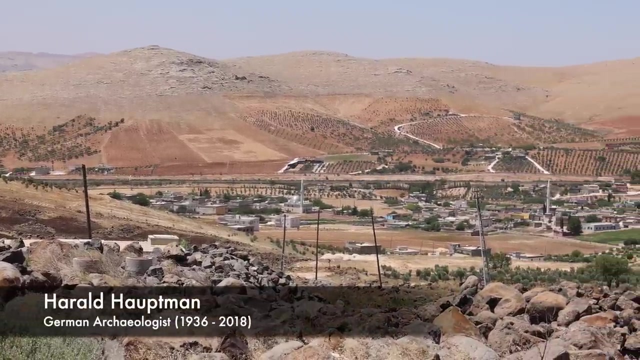 from the Urfa Museum, without which the site might not have been found When Turkish archaeologist Murat Akman arrived at the hill, whose previous digging experience took place at Chionu and Nvali Chori under Schmidt's mentor, Harold Houtman. 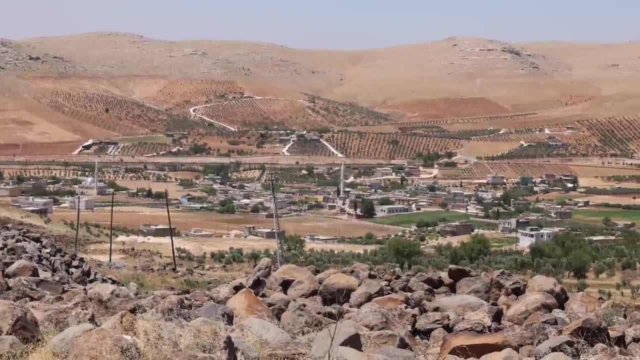 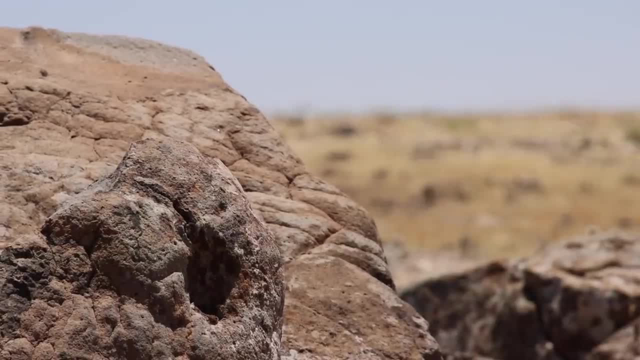 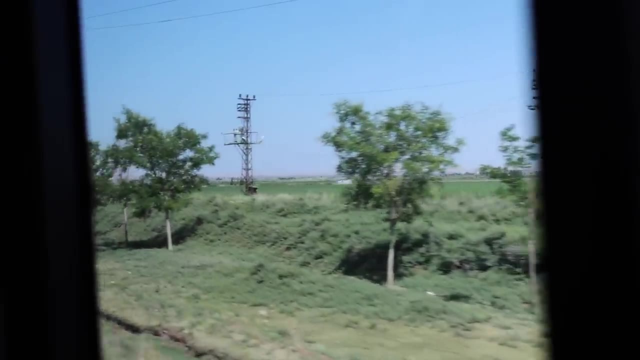 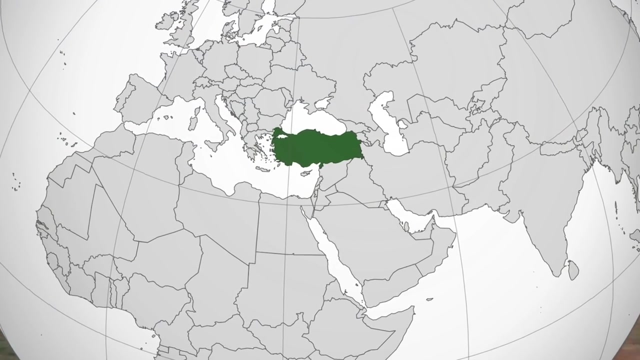 Schmidt didn't have to say anything at all. With little more than a look, both men knew intuitively everything in their field was about to change. Southeastern Turkey could be a dangerous place at that time, Shaken by Kurdish separatist groups, And when the local villagers 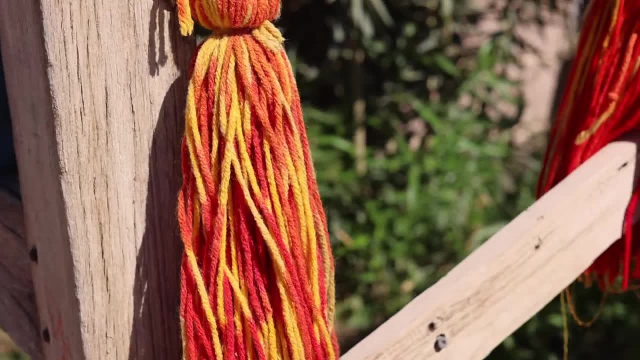 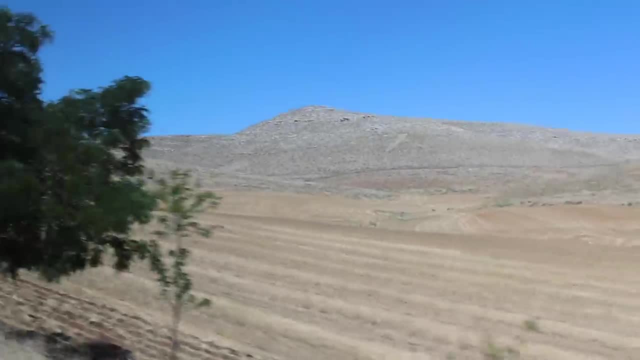 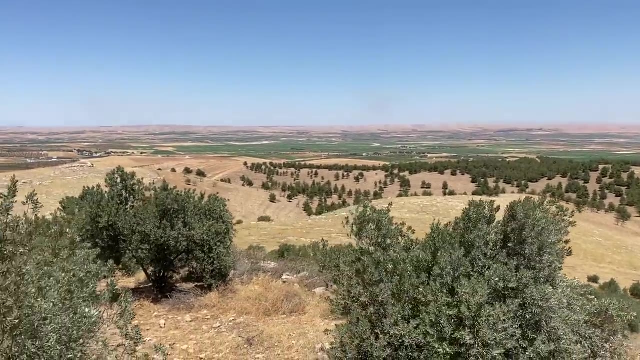 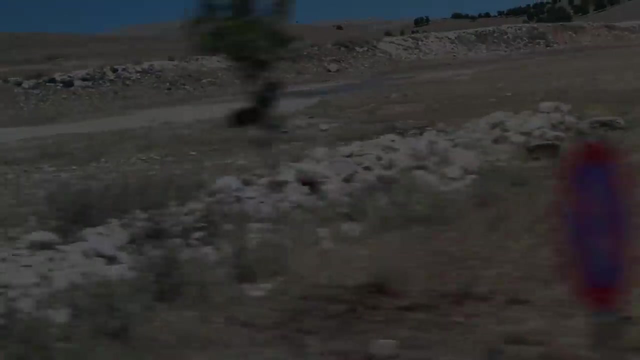 saw a group of strangers wandering around their fields that day, they turned up armed and ready to defend themselves. Eventually, through the diplomatic skills of a Kurdish taxi driver, the situation became disarmed and the AK-47 wielding village guardians backed down On that day. 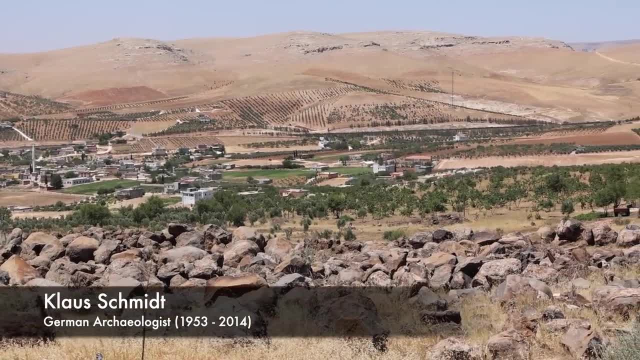 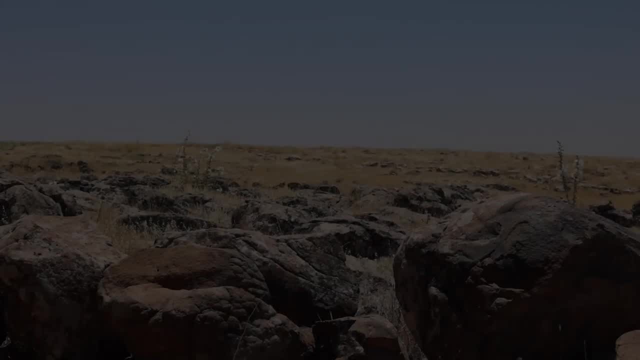 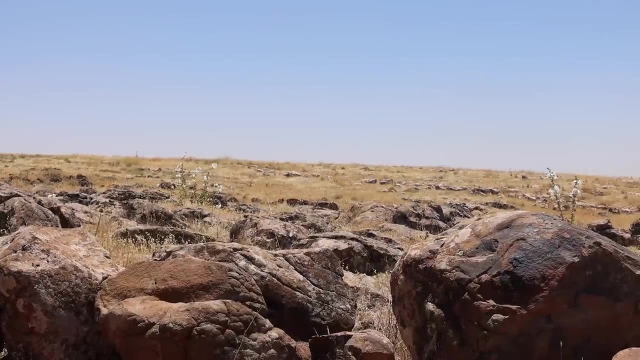 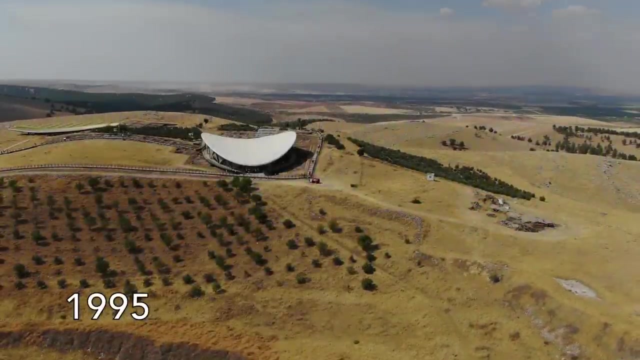 Klaus Schmidt realised, for better or for worse, his previous research plans had become utterly irrelevant. He had no choice but to dedicate the rest of his life to the place. Just one year later, a massive team arrived and one of the great digs in world history began. 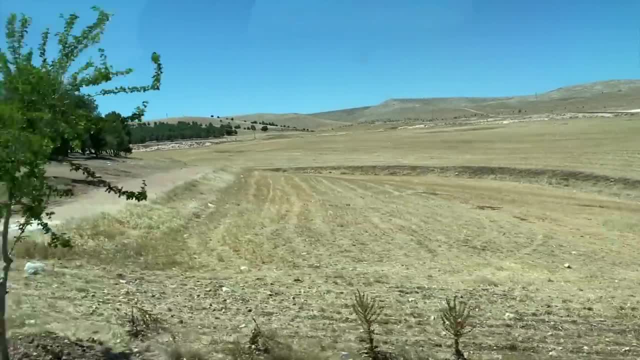 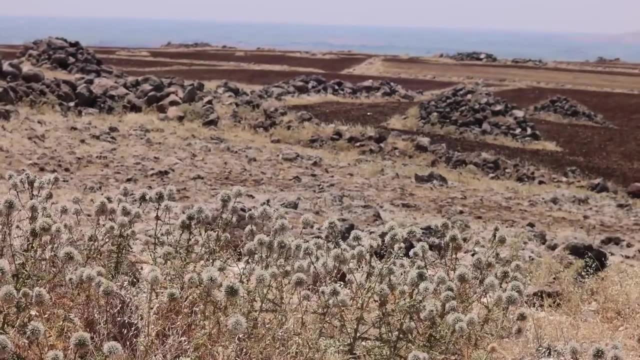 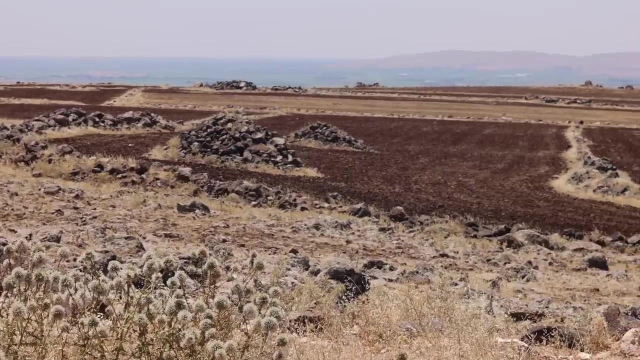 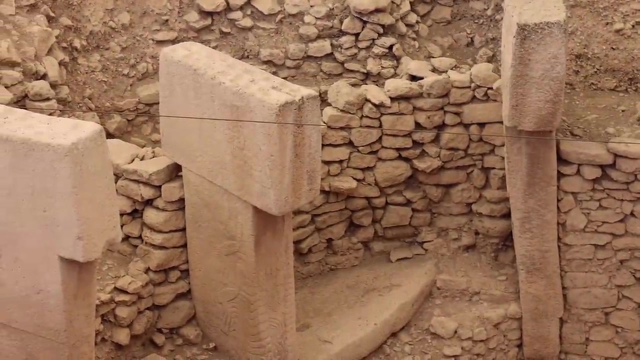 The farmers already inadvertently in the process of excavating were paid compensation for their land. And even though the damage wrought by spade and plough over the decades and centuries was great, the sheer scale and preservation of the site was astounding to behold. The dig was slow. 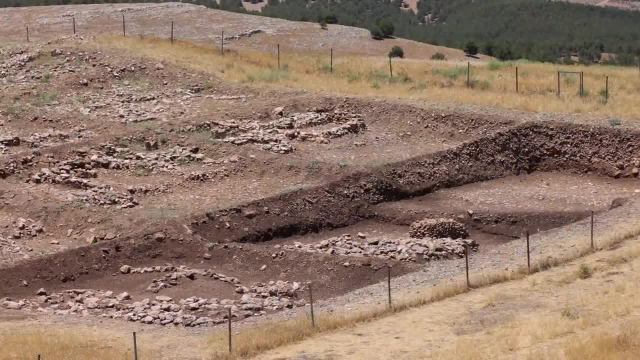 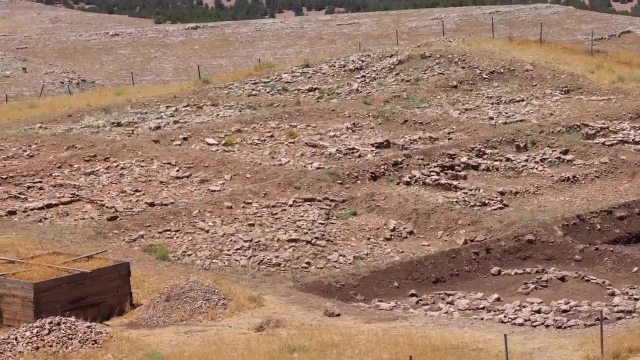 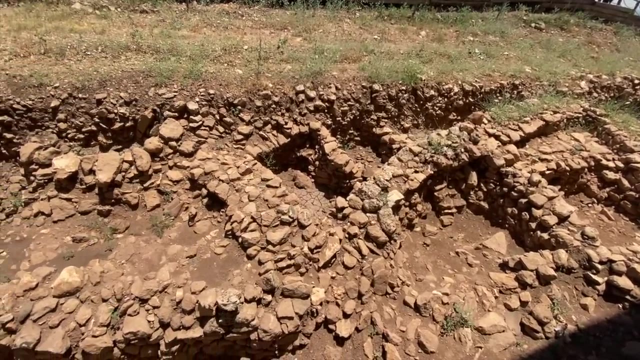 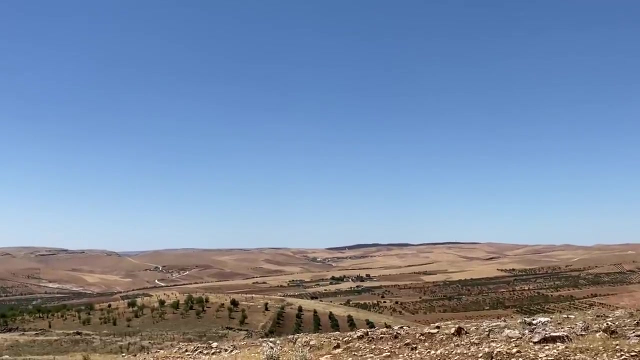 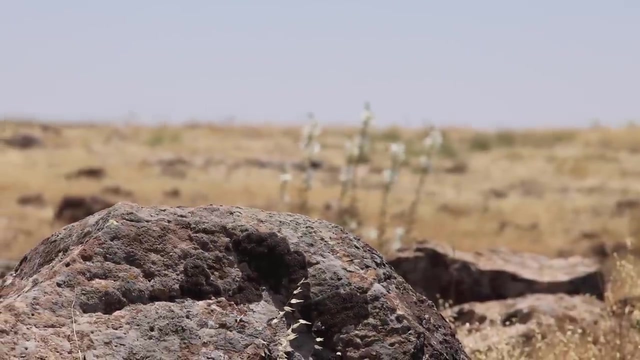 and methodical, utilising the very latest in cutting edge scientific techniques. But almost immediately a number of realisations were made, Not just one area of the site, but many other areas of the site that were covered in megalithic architecture All sides. 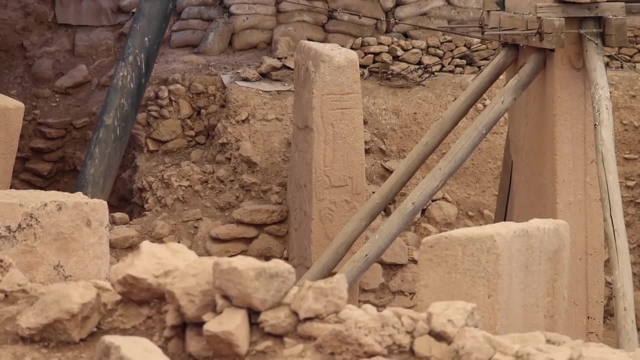 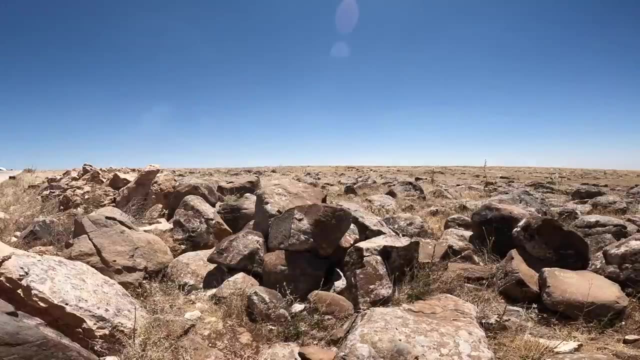 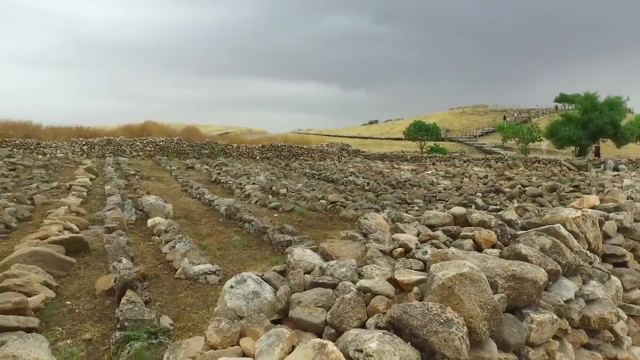 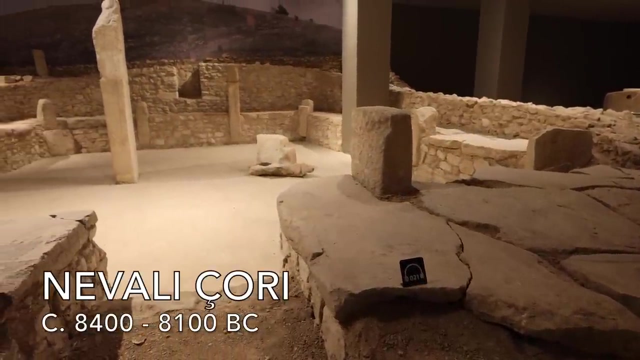 worked carefully by hand. Not only that, but broken pieces were everywhere, too Many. now housed in the so called Garden of Stones on one side of the hill, The earliest semi-subterranean enclosures of this story, meticulously documented in the 1980s. did indeed have similar features to those found at Gobekli Tepe. They dated from the same time when carbon dated Some 12,000 years ago, Not long after the end of the last ice age. But these were the most famous. 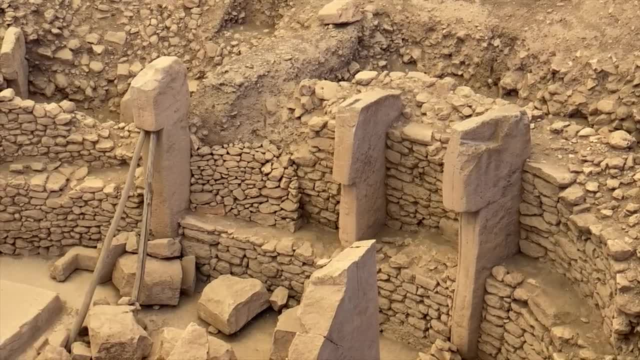 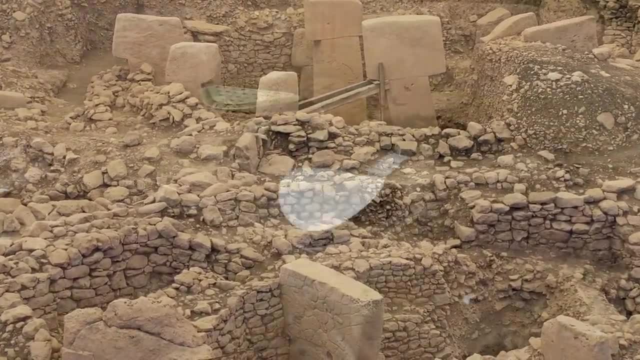 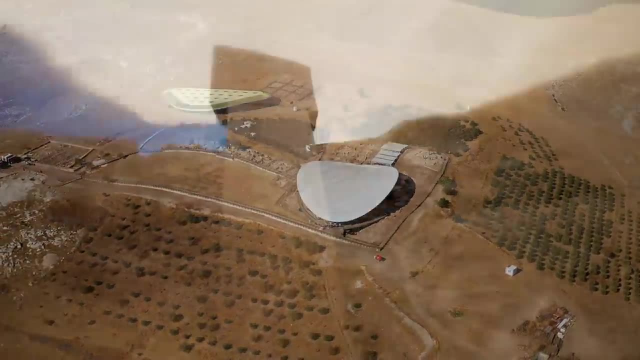 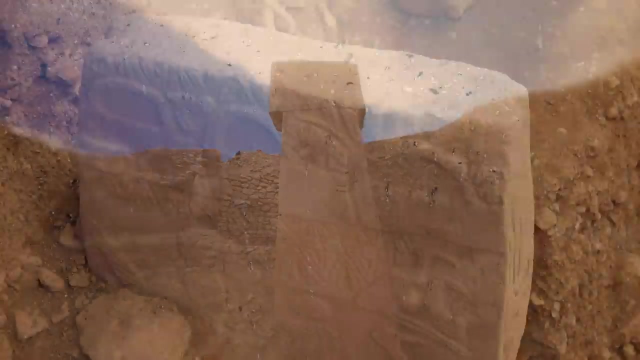 archaeological sites in the world. A couple of seasons later, and Gobekli Tepe was the most famous archaeological site in the world, Stretching for some 25 acres, at least 20 stone circles were unearthed, Each containing pillars as much as 9 feet tall. 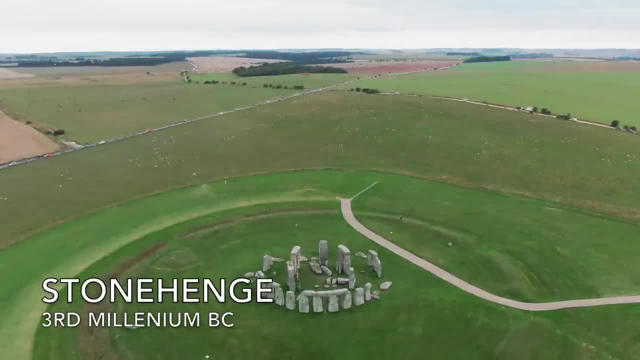 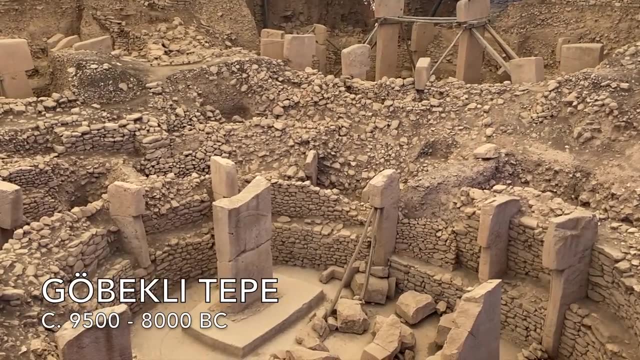 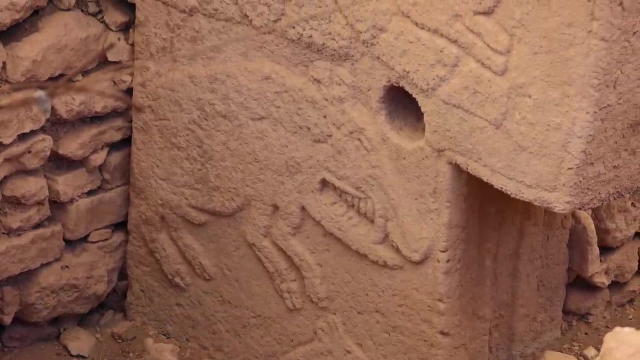 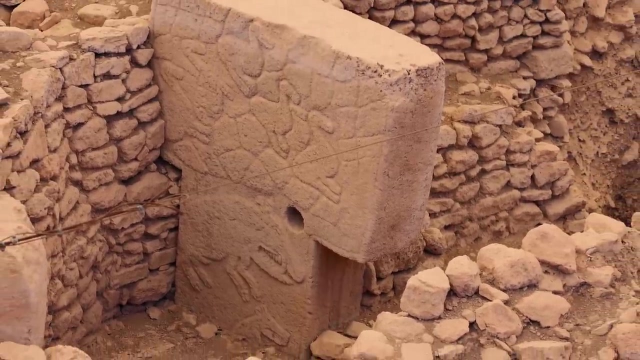 Predating Stonehenge and the Pyramids of Egypt by some 7,000 years. The evidence clearly showed the makers of this extraordinary set of monuments to be a people without the technology to create pottery And, even more astonishingly, just like the earliest. 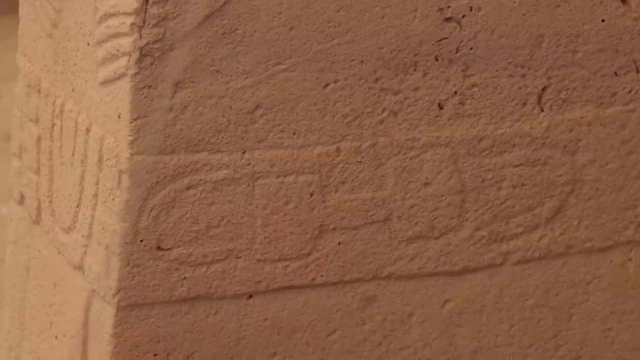 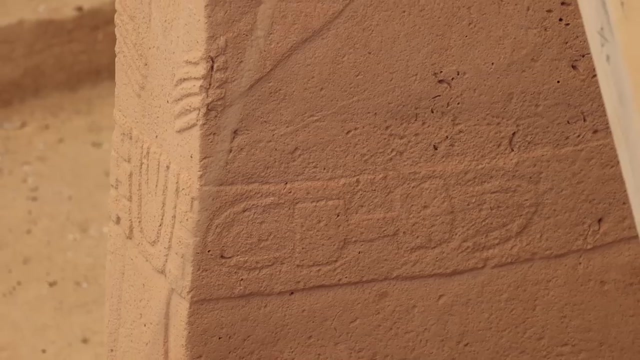 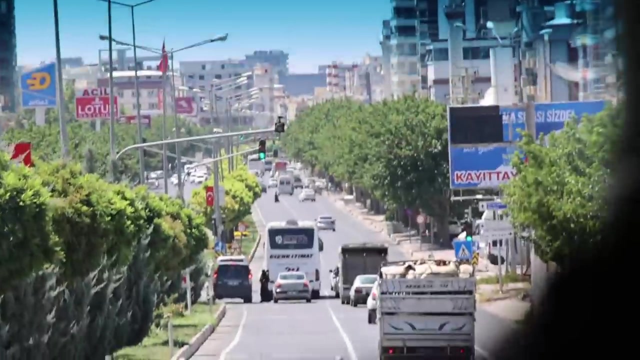 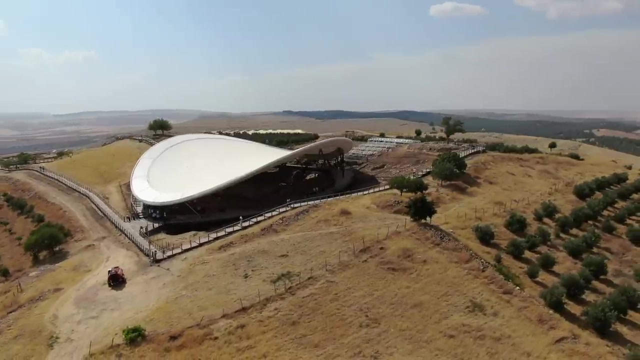 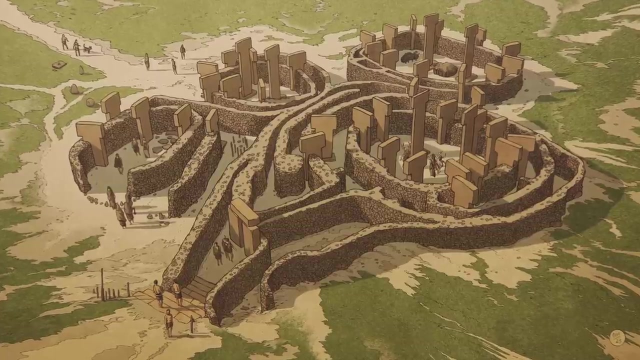 levels of agriculture, Only the remains of wild animals and wild plants being found Within eyesight of Urfa, Somehow having avoided discovery for all those millennia, Gobekli Tepe had once been a place of immense significance, And, as the seasons 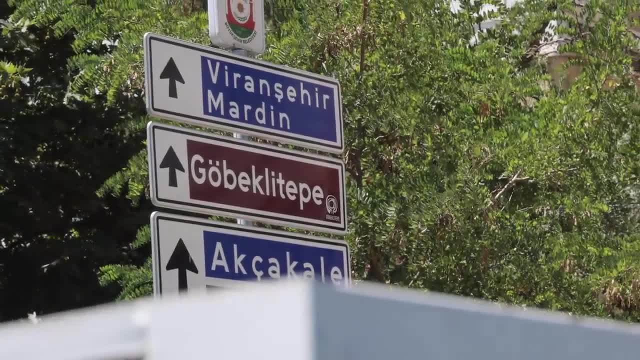 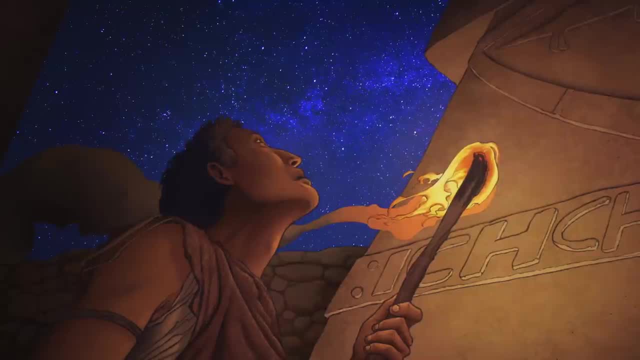 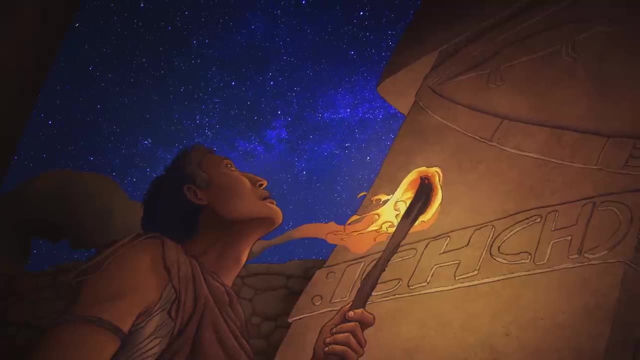 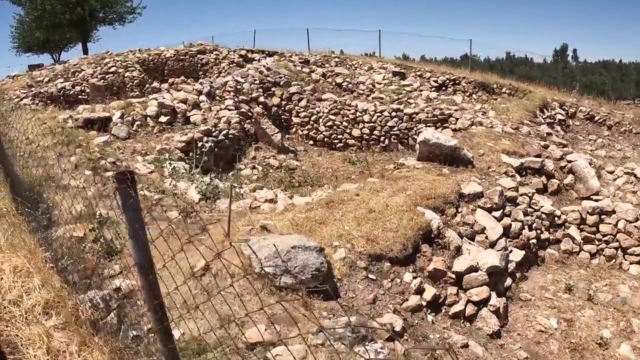 went on and the evidence continued to mount up, Klaus Schmidt began to form his opinions of the place As a spiritual centre for an affluent, nomadic people in a changing world, beginning to settle down and farm, But here not yet, Clearly possessing a complex and well developed. 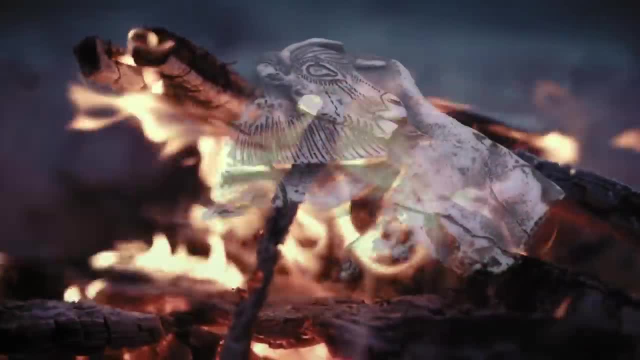 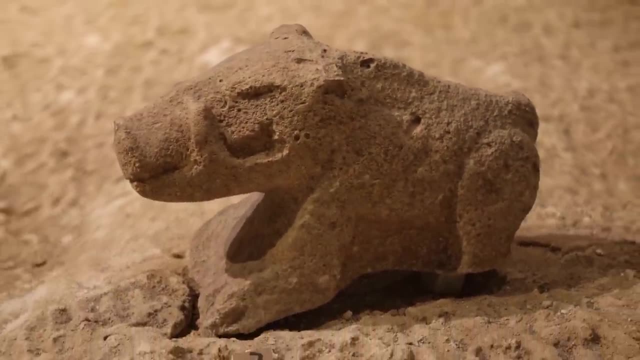 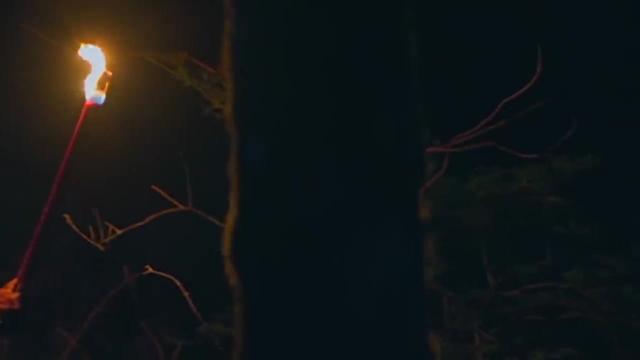 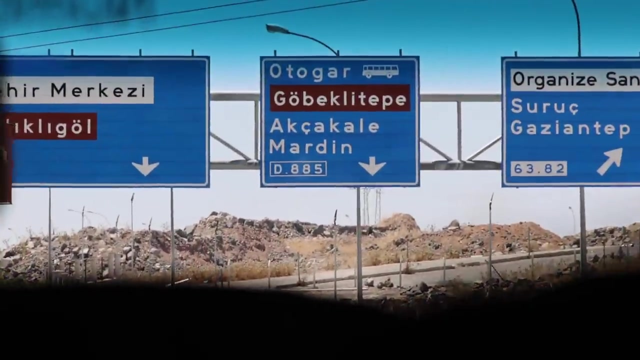 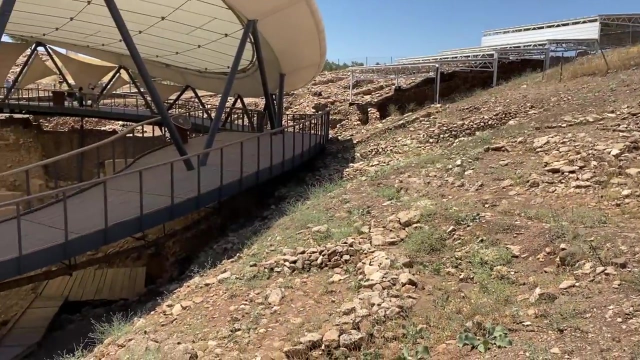 culture and mythology reminiscent of our Paleolithic ancestors. This was a sanctuary of profound importance On the border between hunter-gatherers and our settled world. to come Now, some 20 years later, digs continue and the site, which will always get funding, only becomes more. 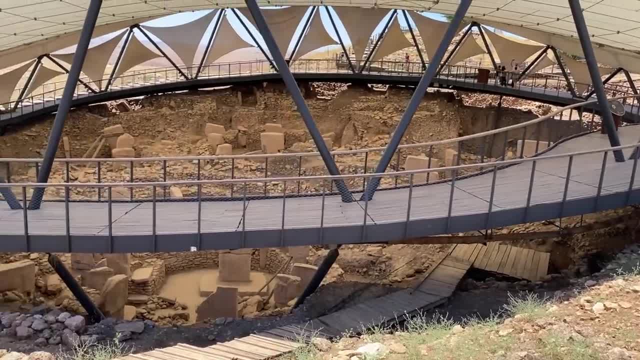 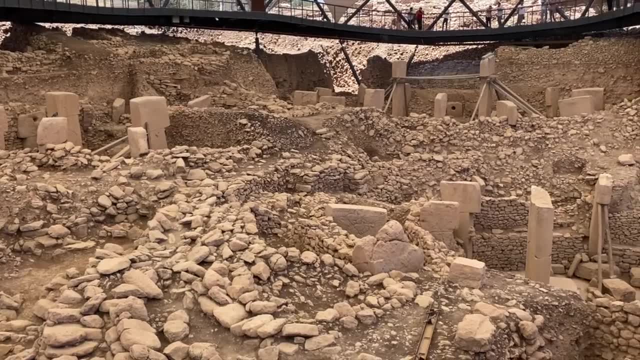 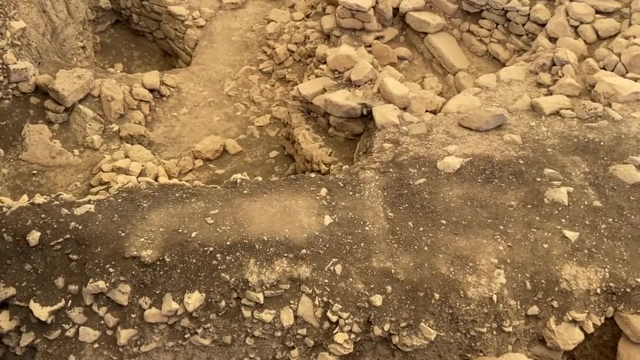 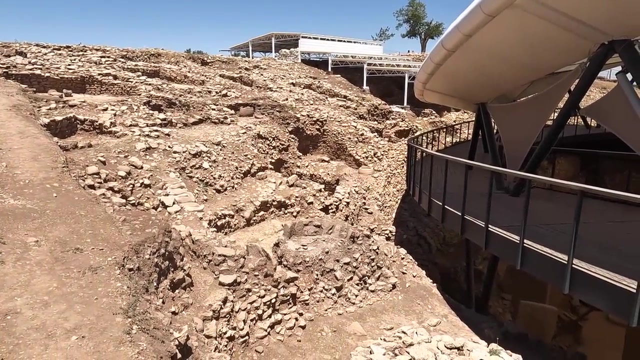 and more interesting. Geophysical surveys continue to show vast numbers of other structures still buried under the earth, Only 5% of the site having been excavated Today, Gobekli Tepe remains one of the key sites for understanding the transition from hunters to farming. 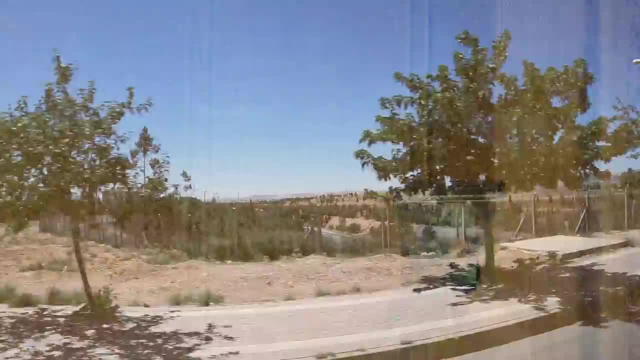 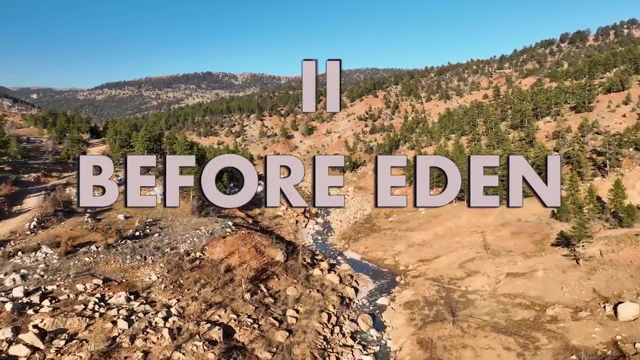 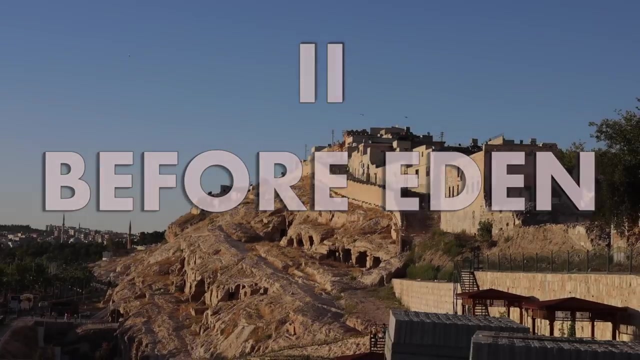 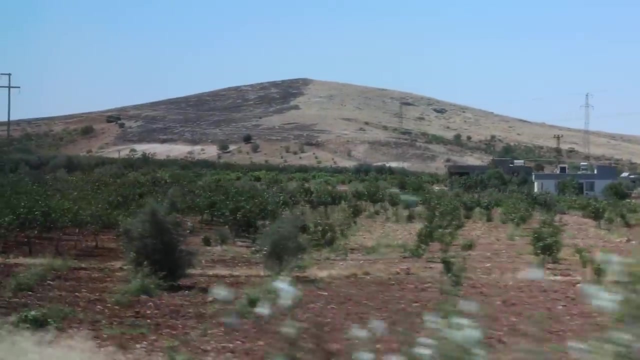 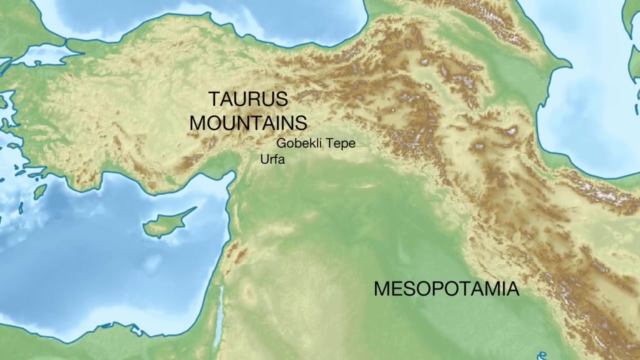 And the birth of civilization as we know it. When viewed from the old castle in Urfa, Gobekli Tepe can clearly be seen on the western horizon. Its pot-bellied silhouette is the highest point on the windswept Urfa plain. 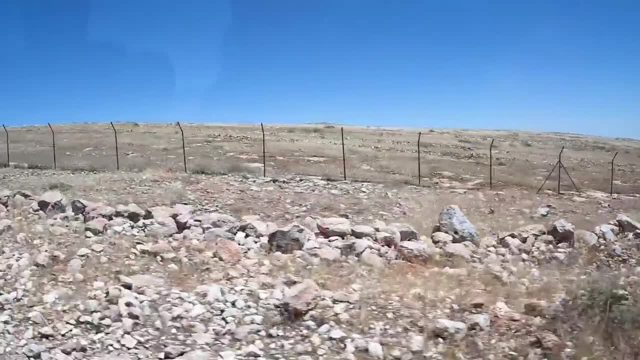 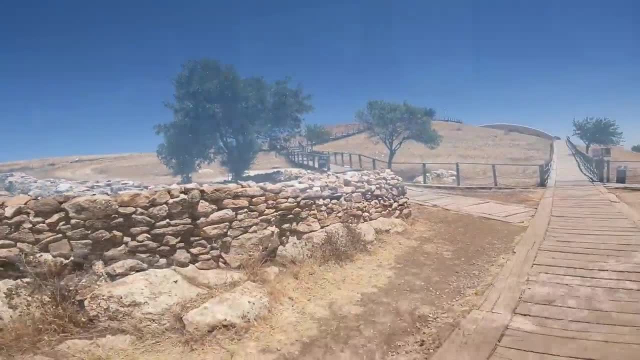 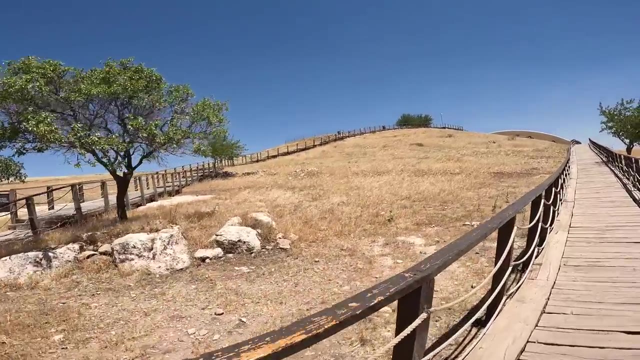 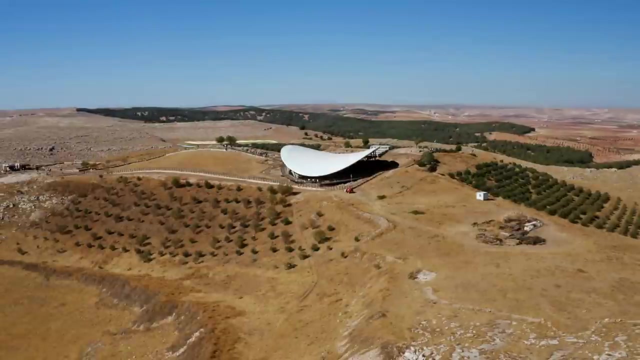 On first glance, particularly in the height of summer, it seems an unforgiving place, Trapped in the gaze of the boiling sun, Without any obvious source of water. And yet the probable remains of the Roman watchtower stand on the hillside: Clear evidence of ancient 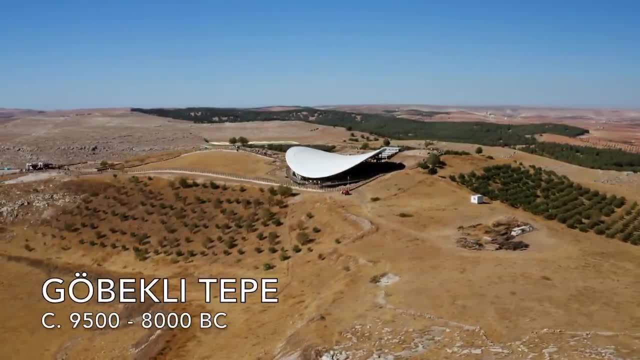 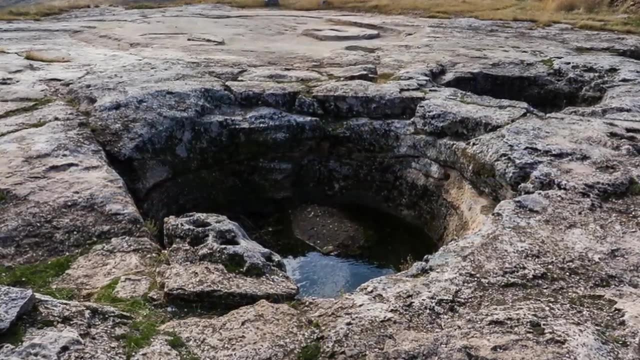 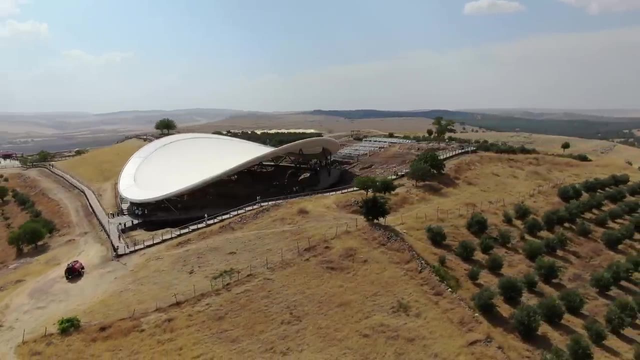 quarrying all around. On closer inspection, at more than half a meter in diameter, it's possible that the large stone rings all over the site could have served as cisterns for rainwater, And from the top of the hill you can see springs. 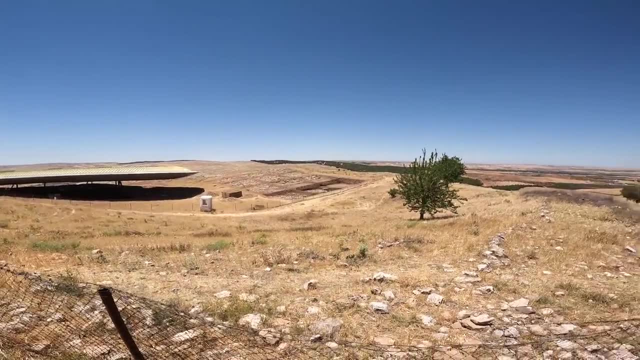 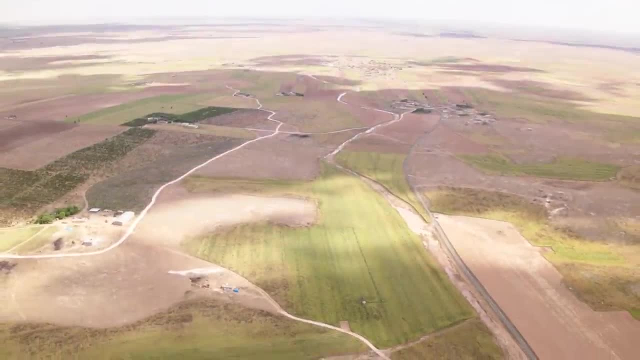 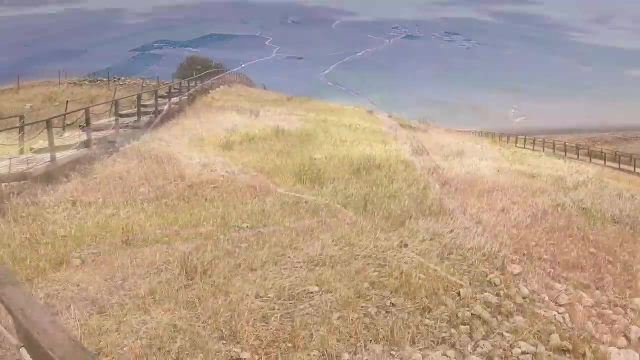 that have dried around, Such as those at nearby Balik And perhaps more, existed in antiquity Long since having dried away. What is obvious from walking the ridge line on the pot-bellied hill is that it very much possesses a commanding view. of a landscape all around The Taurus mountains to the north And the mountains of Haran to the south, When arriving from the south, in particular the next city of Mardin, Another vaunted settlement famous from Crusader times, Gobekli Tepe. 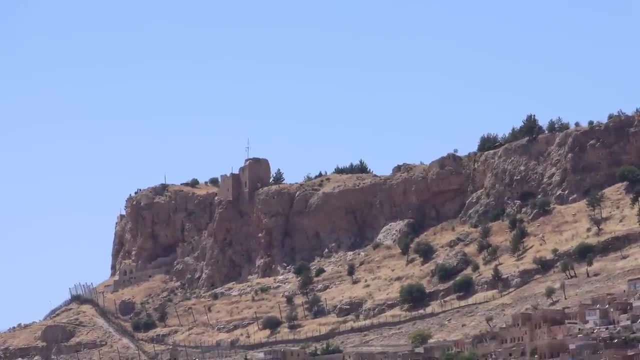 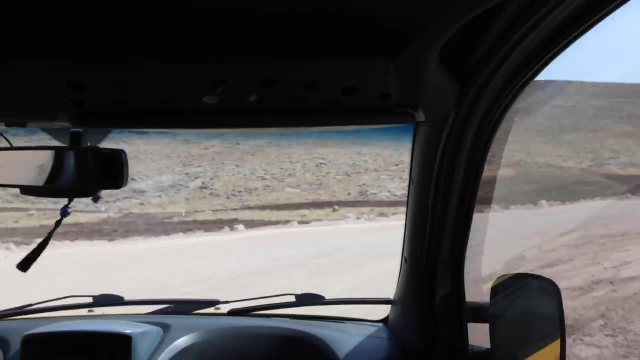 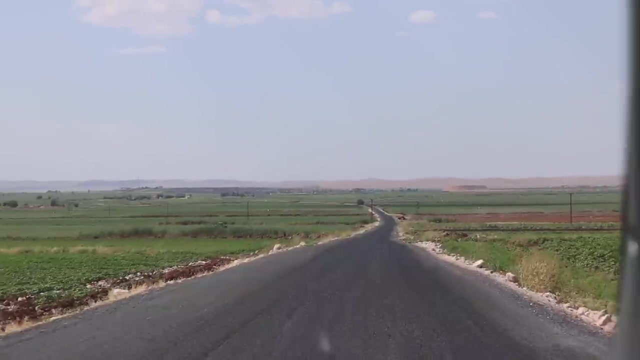 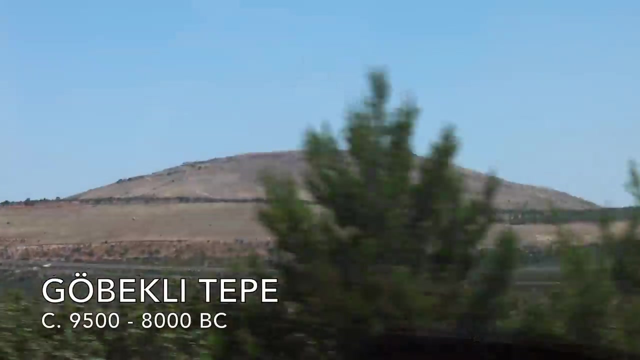 can clearly be picked out from a distance of some 20 km or more. With the benefit of hindsight, it is difficult to understand how such a place was missed, The landscape itself seeming to hint at a certain level of significance, Once you know where you're looking. 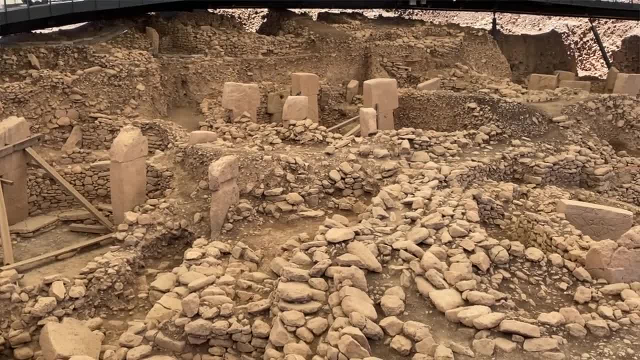 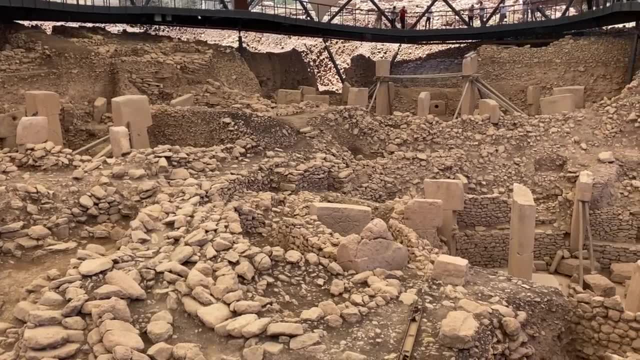 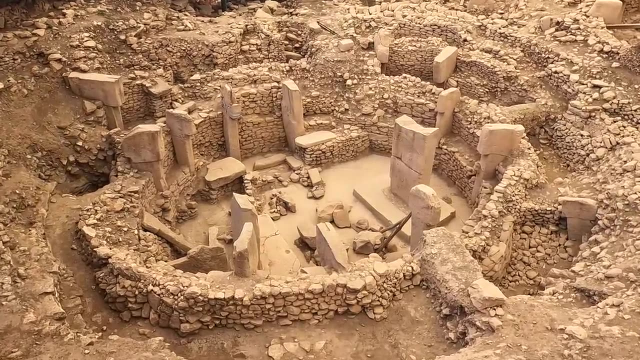 And when the buildings finally began to be stabilized and excavated in the mid 1990s, Sunken chambers dug deep into the hillside, opening up for the first time in well over 10,000 years. The place only became more and more unusual. 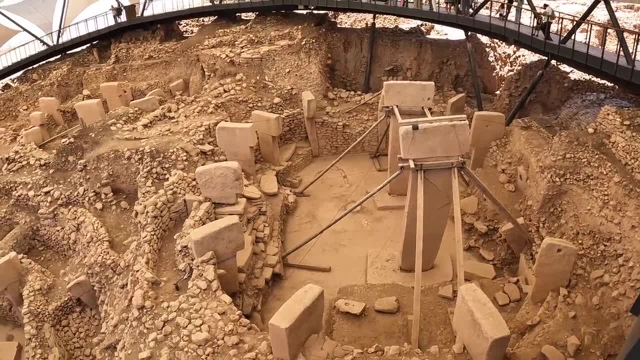 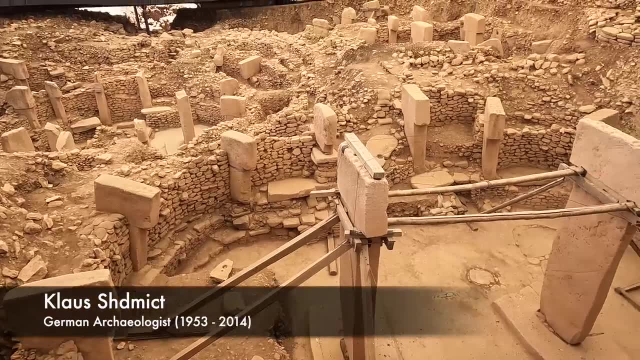 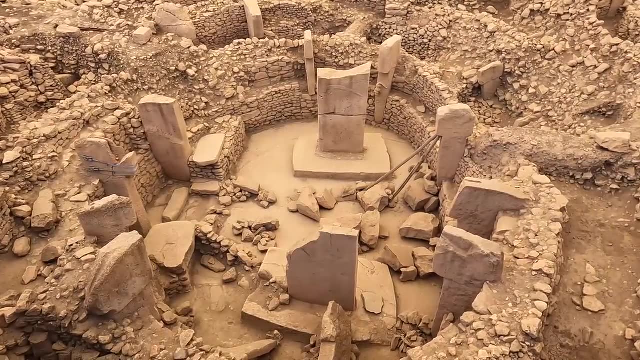 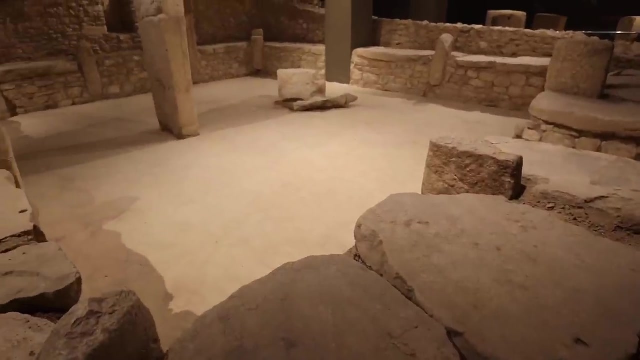 No obvious fireplaces were found, No ovens, No trace of domestic life of any sort, wrote Klaus Schmidt in an early report. Concluding: the structures not only be unroofed but ultimately unsuitable for human habitation, In stark contrast to Navali Chori. 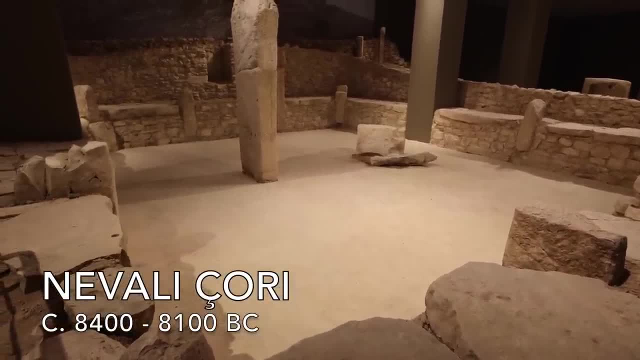 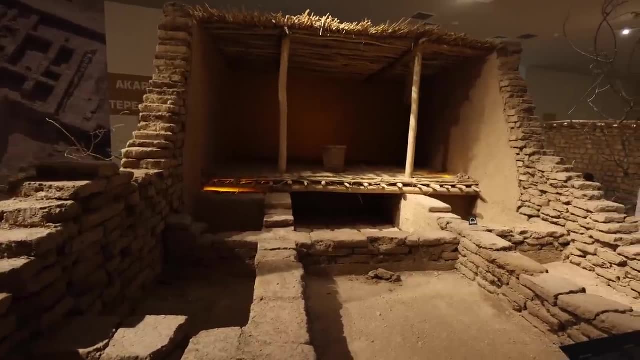 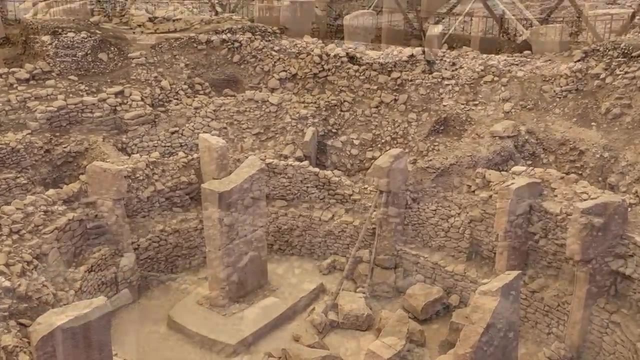 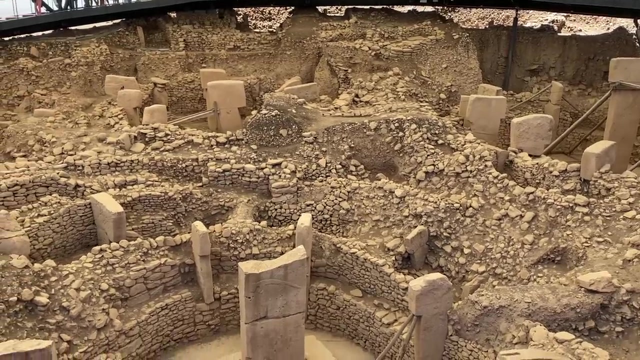 which, in its later phases at least, was settled by very early sedentary farmers living in permanent houses. Gobekli Tepe, with no evidence of settled agriculture whatsoever, seemed to be purely ceremonial in character For Schmidt, all of the excavated buildings from the second and third levels. 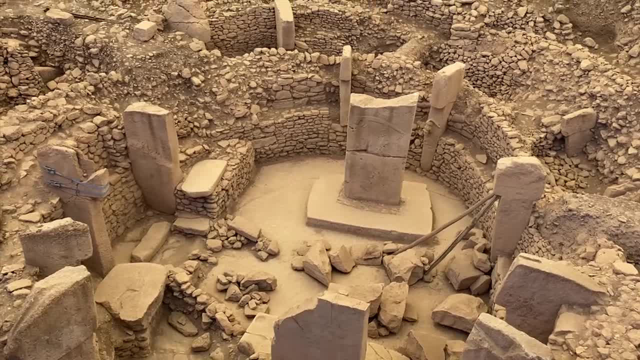 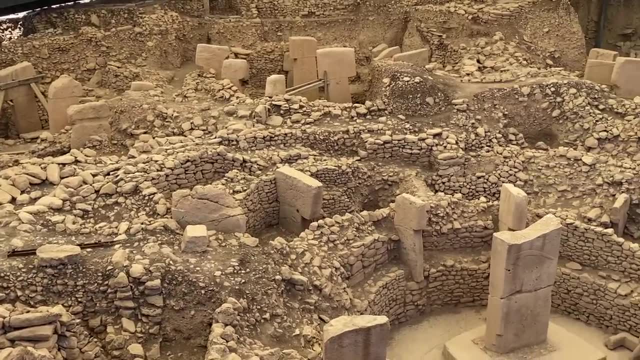 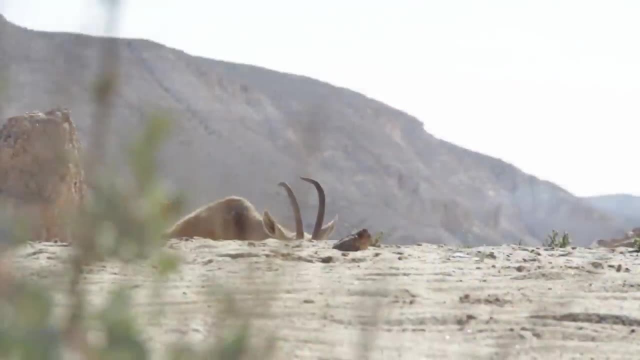 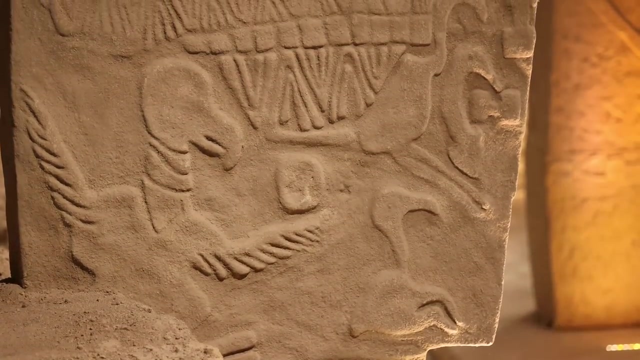 at Gobekli Tepe had been houses, but of the divine, At least in the lower levels, built not by early Neolithic farmers but by hunter-gatherers still living from the foraged bounty of the earth, Just maybe like Greek Delphi. 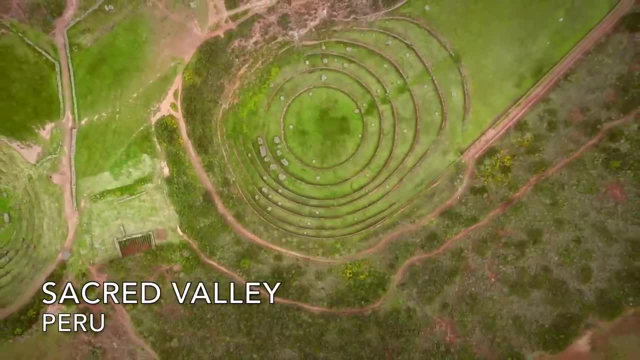 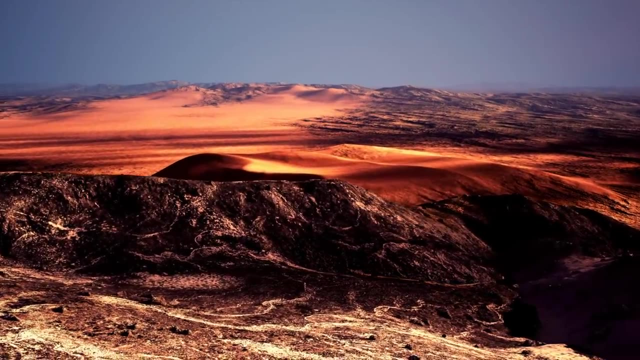 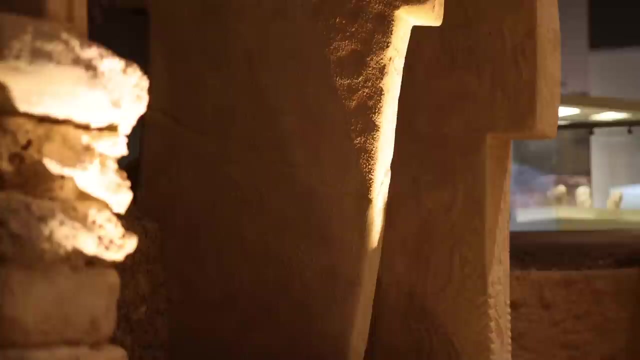 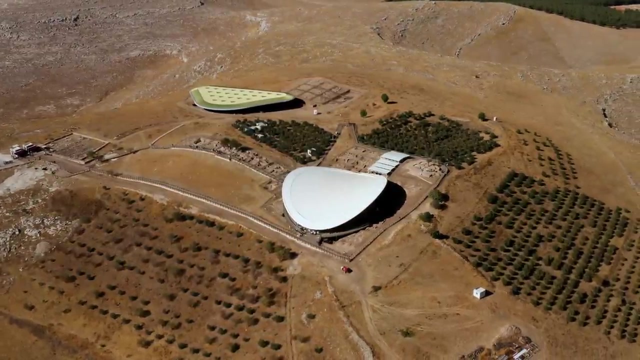 or Cusco in Peru, sacred navels of the earth, where pilgrims would travel from afar for sporadic festival activities, including the raising of vast monuments to ancient gods, ancestors, but not living at the site all year round. Gobekli Tepe could have been. 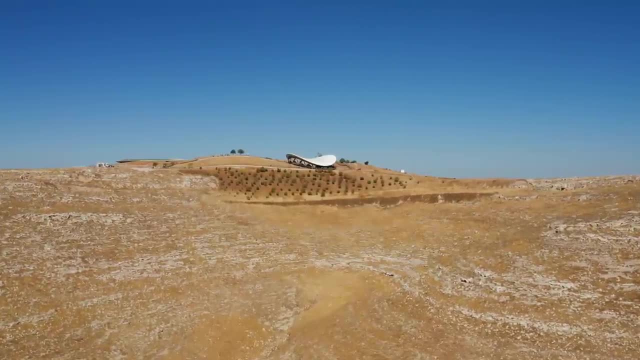 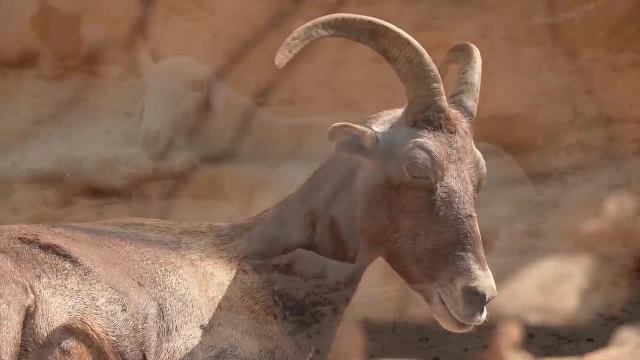 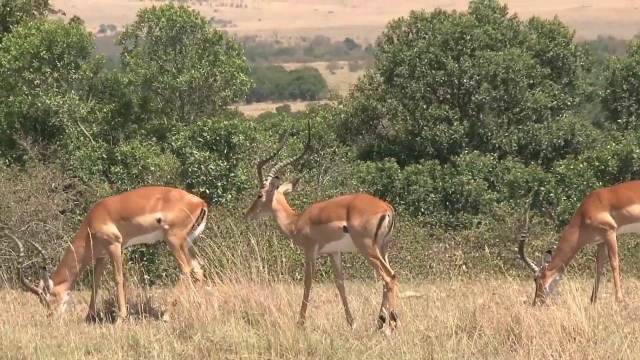 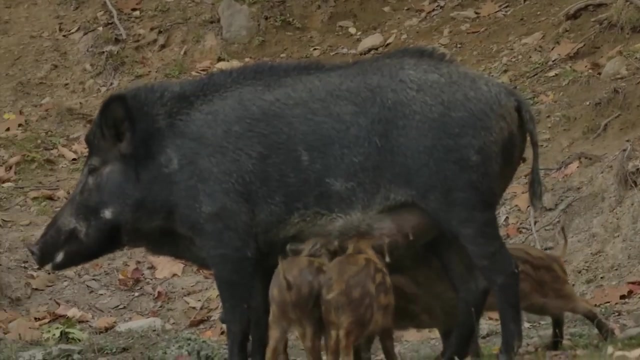 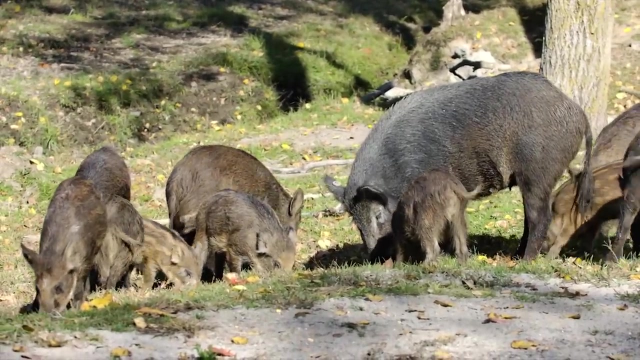 a cultic site. A vast collection of animal remains have been uncovered at Gobekli Tepe, including cattle, pigs, goats and sheep. After intense study by some of the leading experts in the world, all of the animals were found to have been wild. 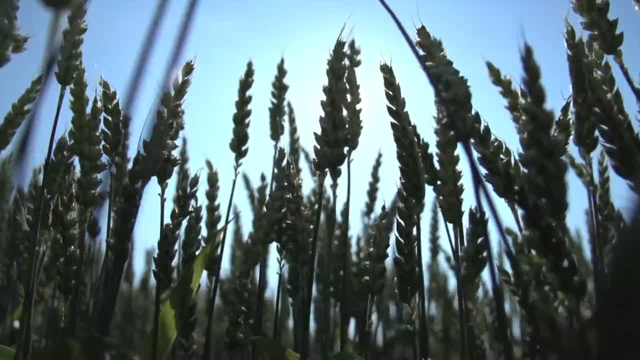 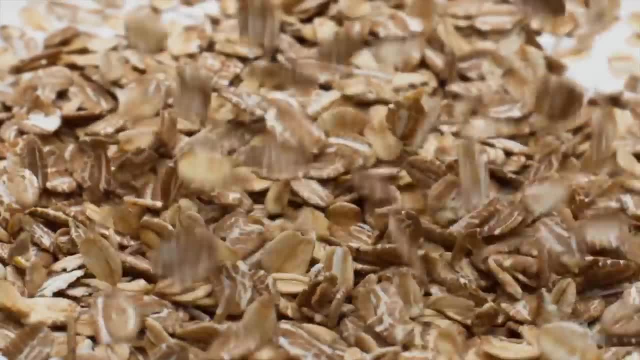 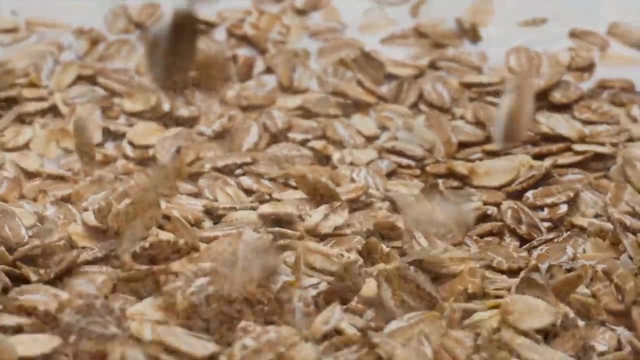 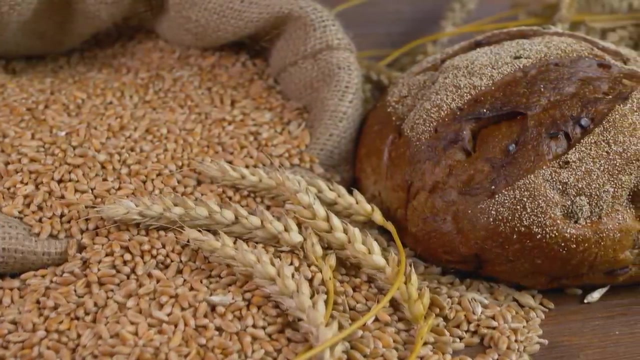 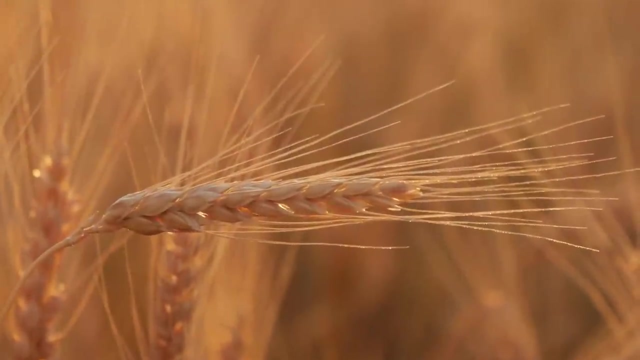 and not domesticated variants, which have different bone structures. Same as the plant remains wild almond, pistachio and grains being found in abundance, wild variants of which can be found on the site, One early idea that made its way into the popular zeitgeist in the late 90s. 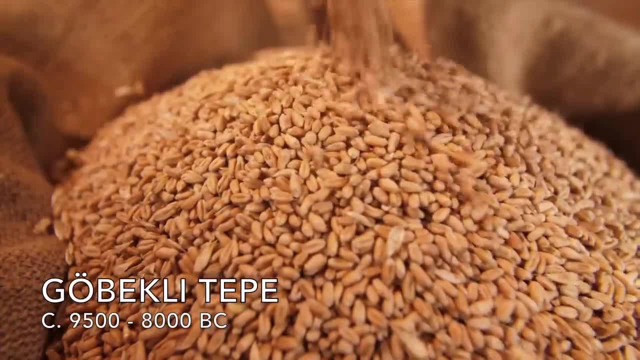 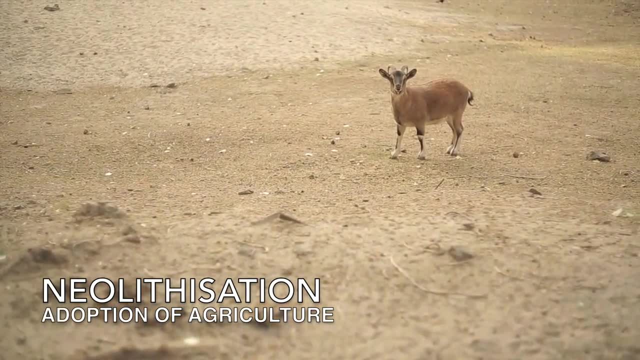 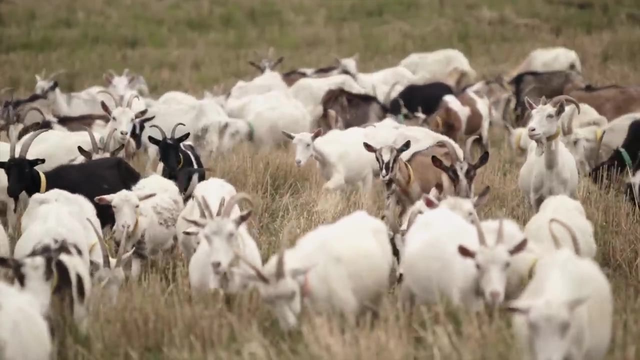 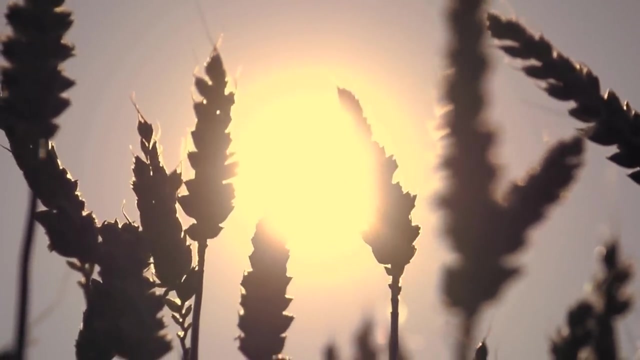 posited, in part due to the glossed sickle blades and early forms of wild wheat found at the site, was the suggestion of Gobekli Tepe, in other words, where hunter-gatherers first began experimenting with farming, After all, when agriculture did begin. 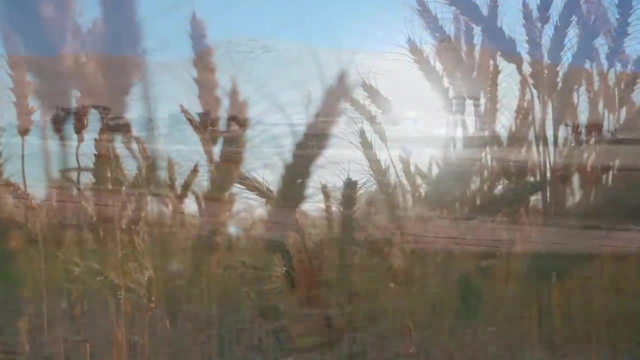 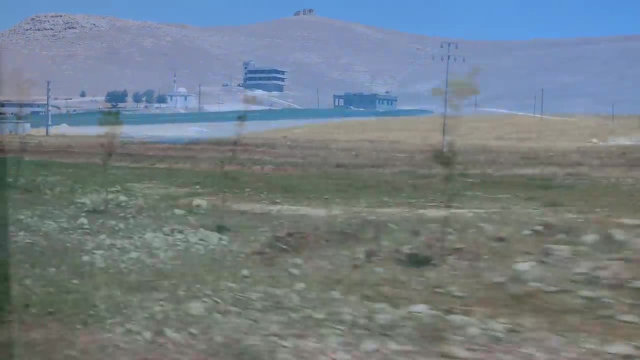 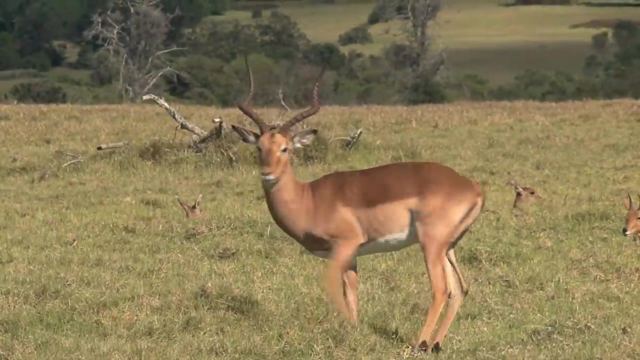 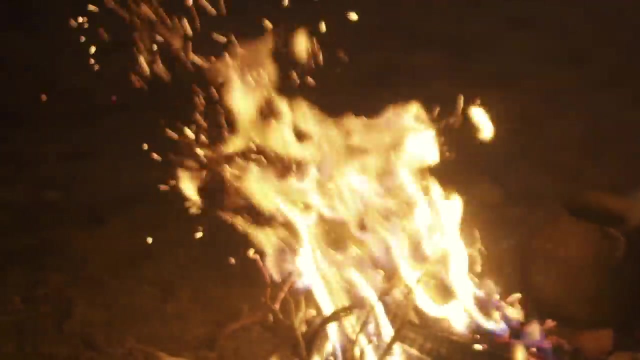 to take hold. analysis of ancient grains does seem to place one of its origin points on the Urfa Plain. One early idea suggests the controlled use of wild wheat and other foodstuff to have resulted from over-exploitation of local resources as a result of increasingly large 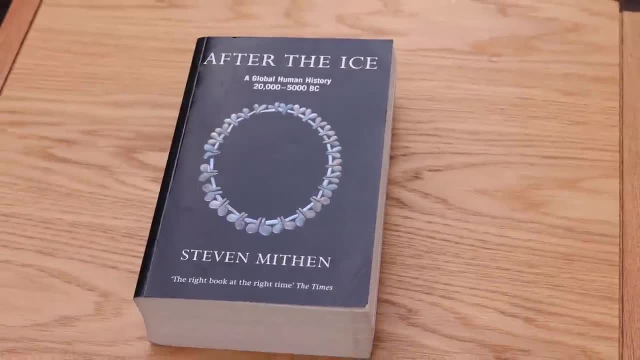 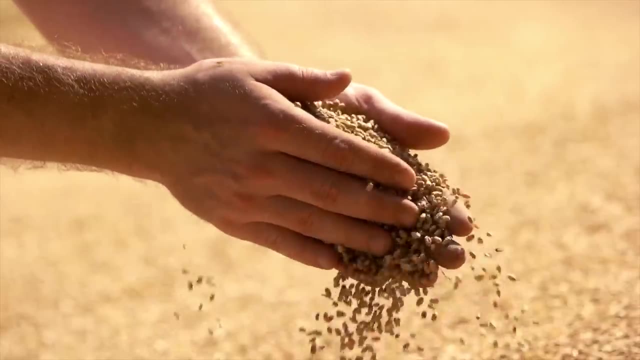 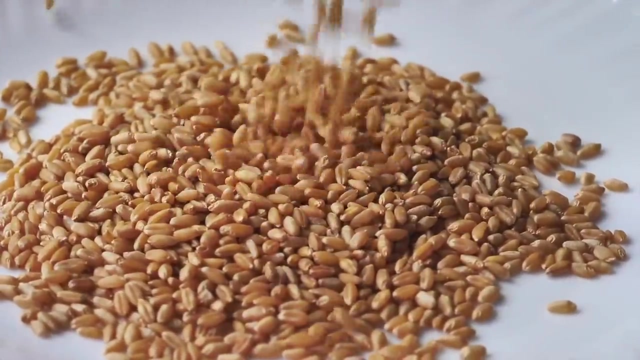 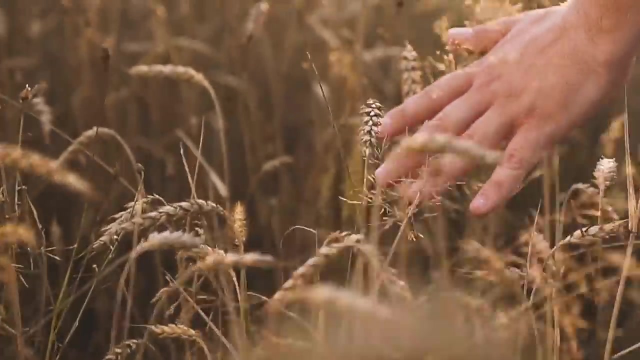 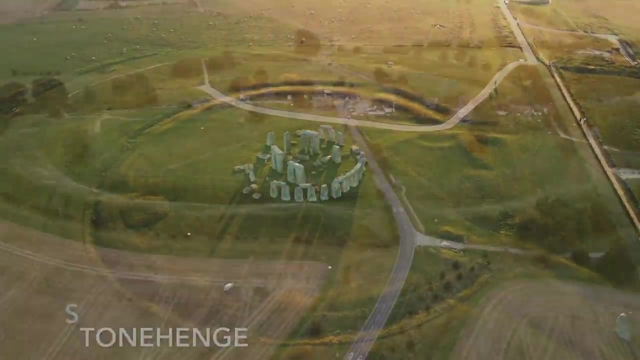 groups of people congregating over an extended period of time. In his 2004 masterpiece After the Ice, Stephen Mithen published a number of articles about how wild wheat can be used as a source of food, and as a source of food. and as a source. 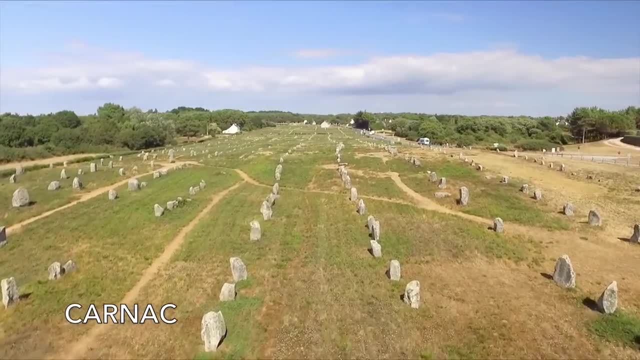 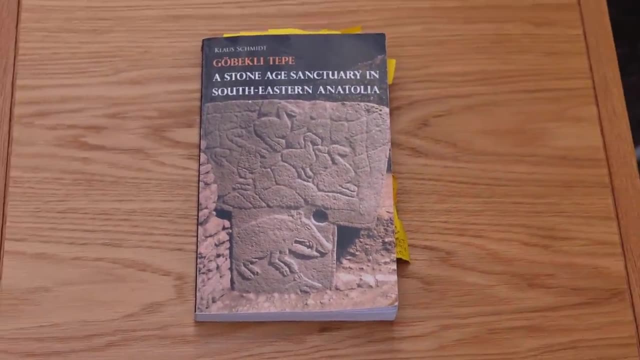 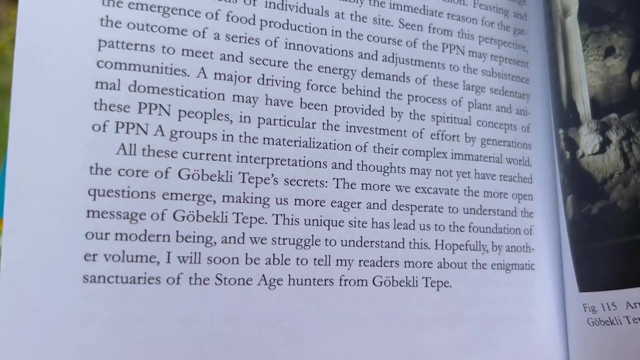 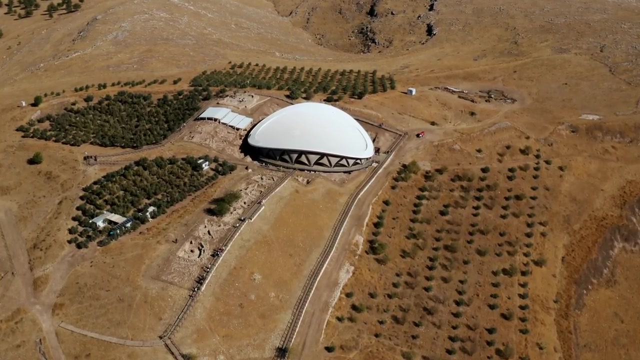 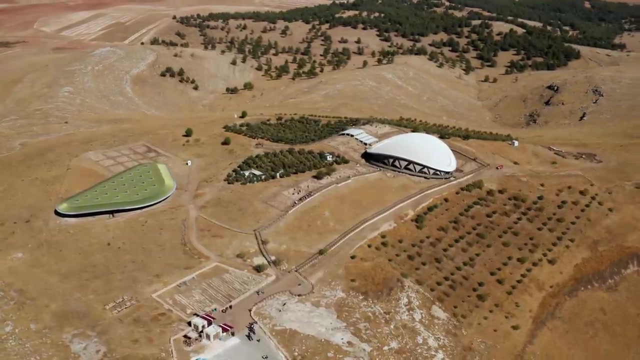 of food and as a source of food. as a source of food, has been published a number of articles and a detailed book on the initial finds at Gobekli Tepe, and another was on the way. Still only three or four percent of the site. 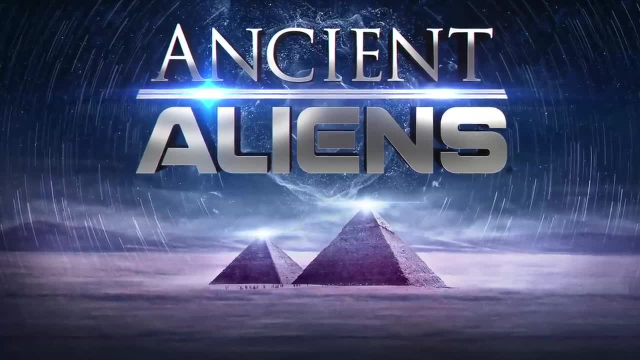 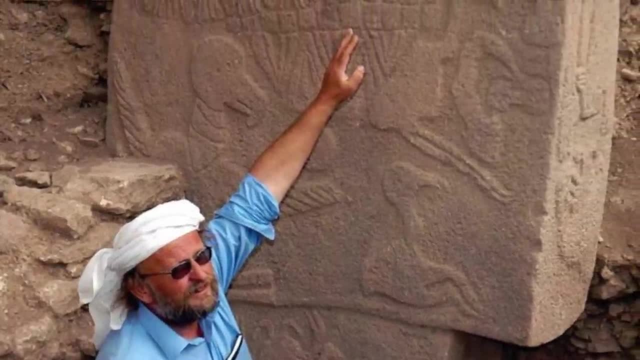 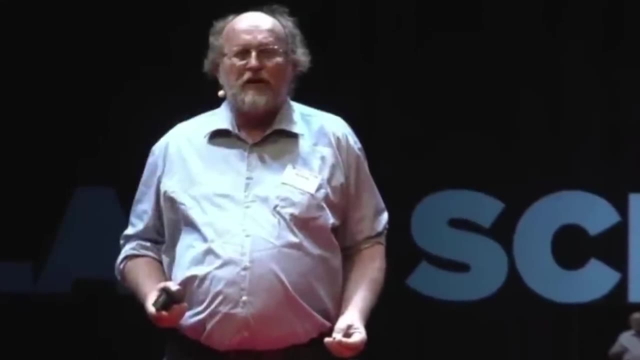 in the process. For 20 years, ever modest and patient, Klaus Schmidt had been a willing servant to the site, devoting all of his energy to speaking tours and tourism, to fighting misinformation and spreading awareness of archaeology to the general public. 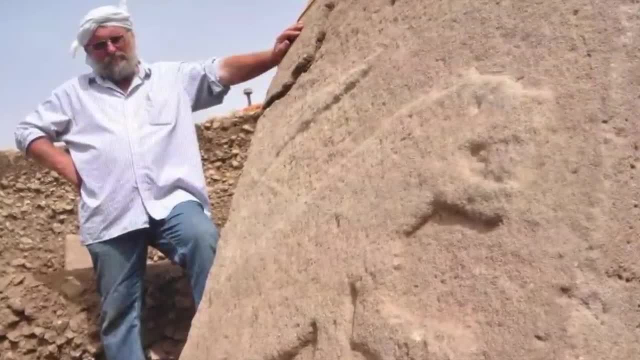 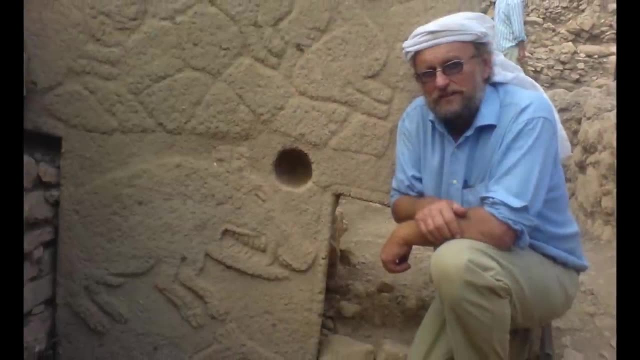 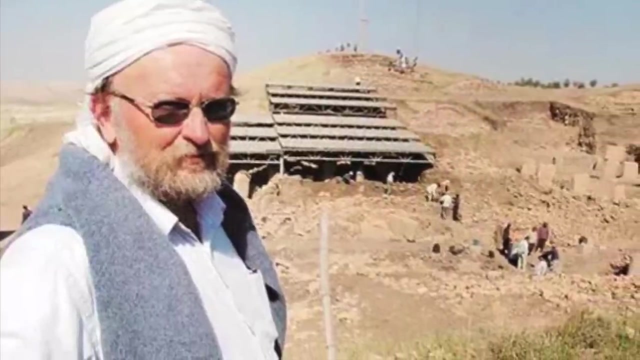 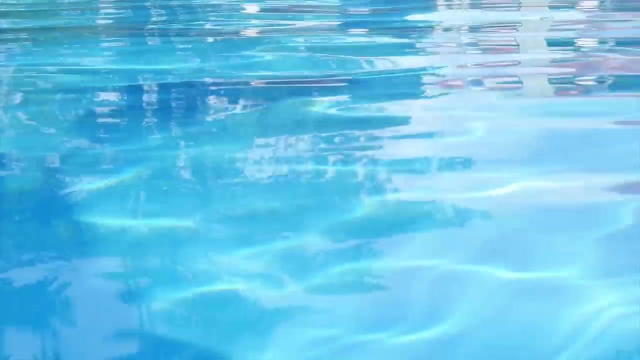 Always making himself available, even when publicly attacked by fringe theorists and dogmatic ageing archaeologists alike. Finally, by 2014,, it all came to an end. One Sunday afternoon in a swimming pool back in his native Germany, Klaus Schmidt's heart gave out. 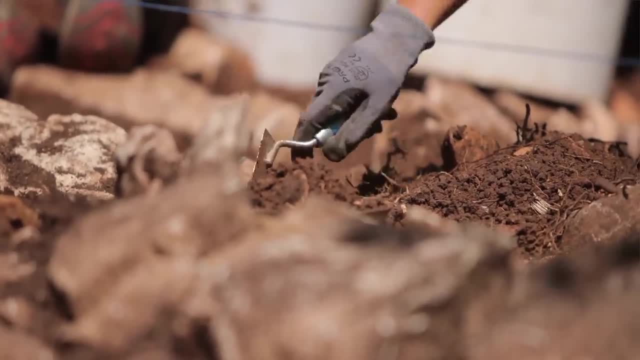 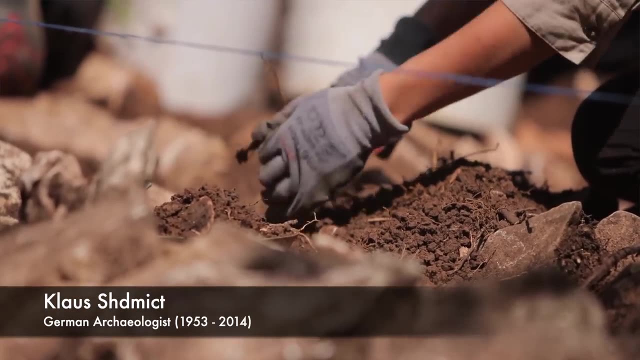 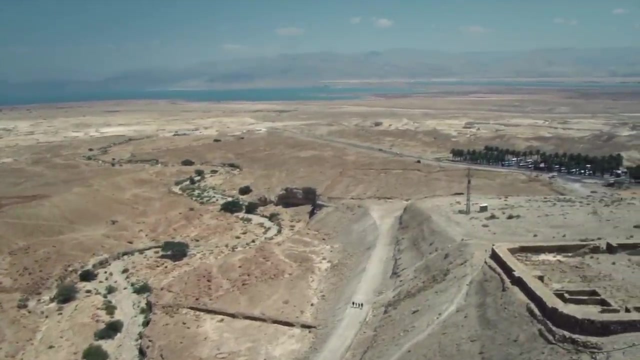 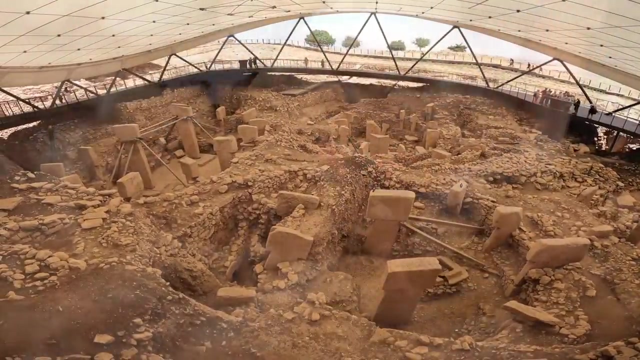 By the time of his death in 2014,, Klaus Schmidt had already cemented his place in the annals of archaeology. His dig will go down as one of the most famous in all of history, completely altering our understanding of the origins of civilisation as we know it. 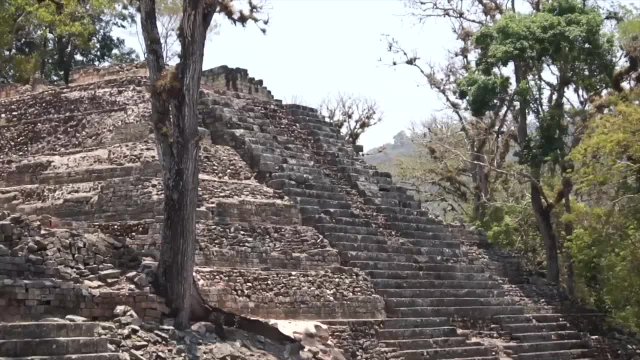 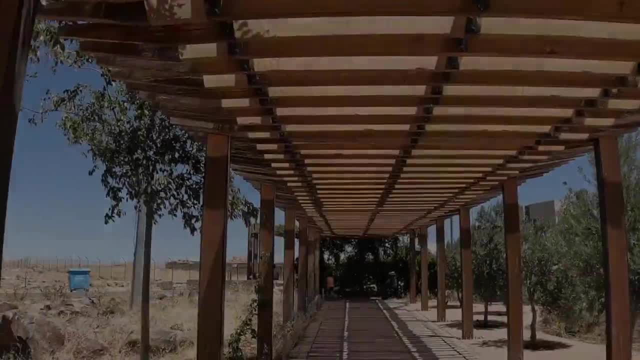 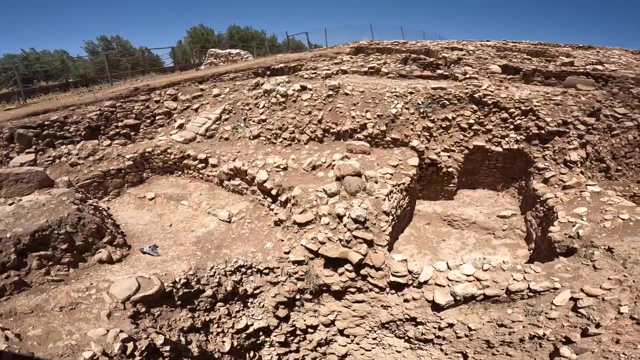 Like Troy, Olympia and the great Marlborough, the ancient ruins of Copan digs will likely go on for another century or more. The place will never struggle to get funding And, most amazing of all, by that time and in the years since, 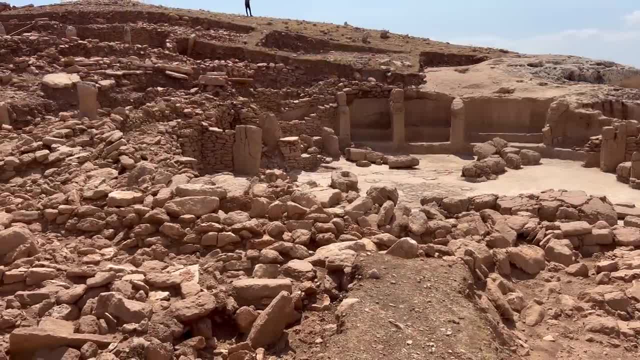 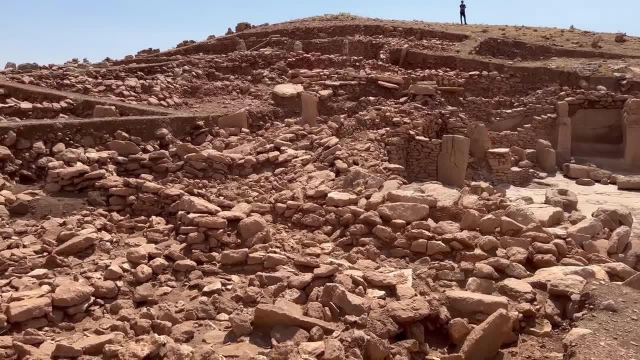 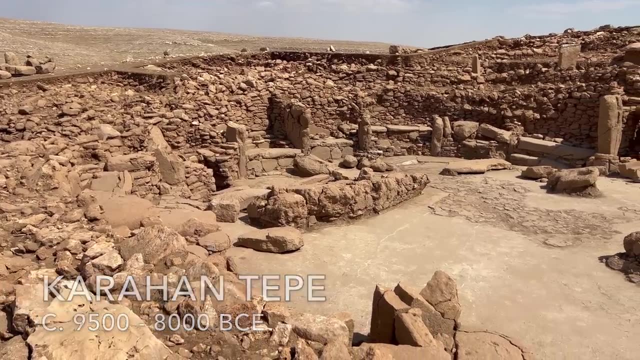 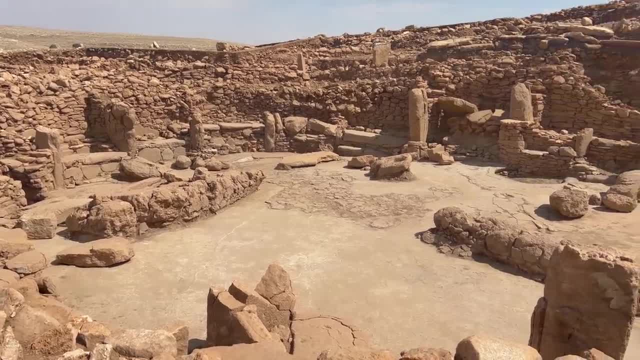 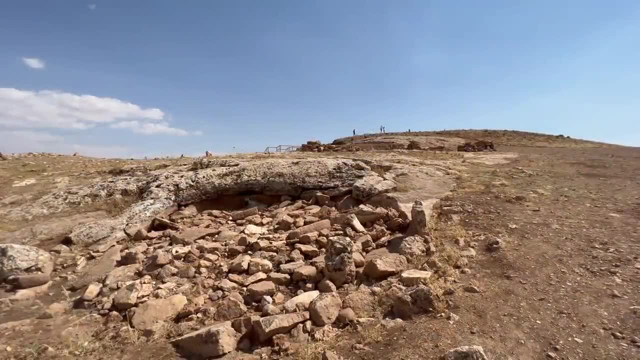 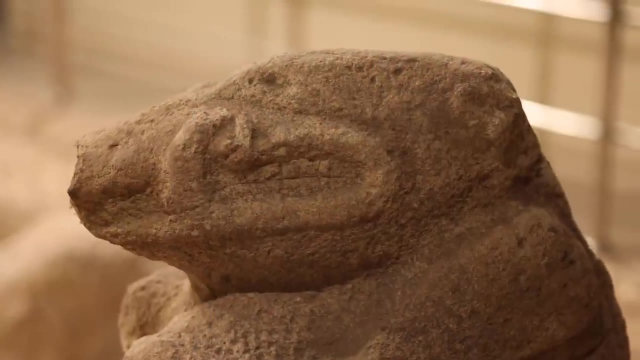 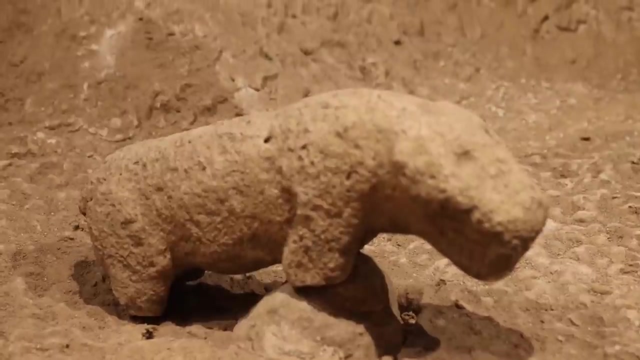 of eager Turkish archaeologists inspired by the likes of Klaus Schmidt. The results are astonishing. Far from an isolated phenomenon, Göbekli Tepe was part of an entire culture, similarly built by hunter-gatherers, many of whom, like at Chianu and Navali Chori, turned ultimately to incipient. 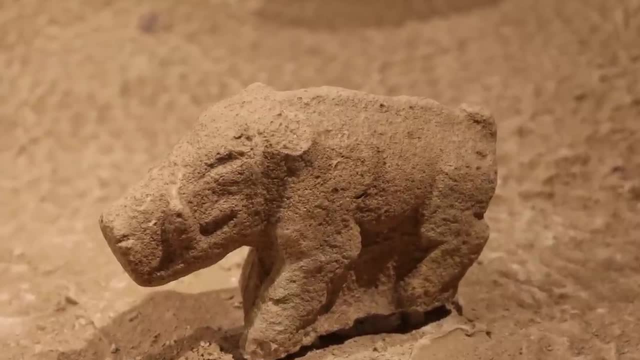 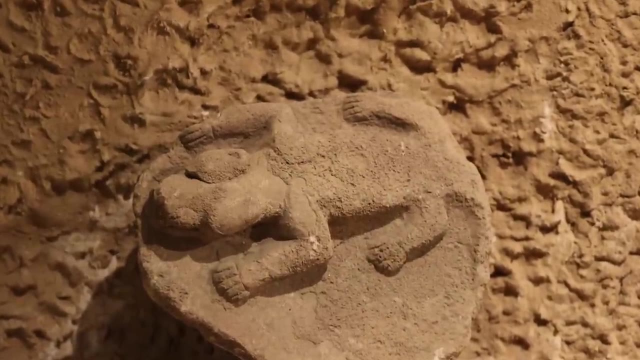 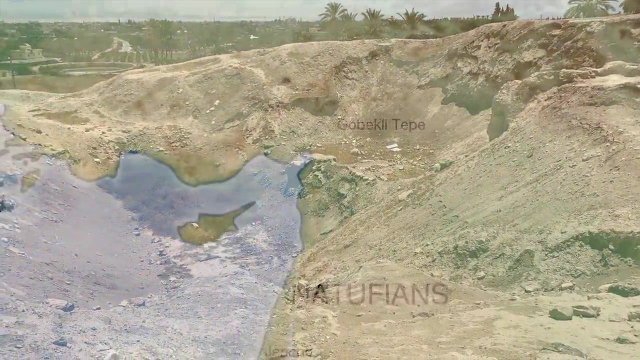 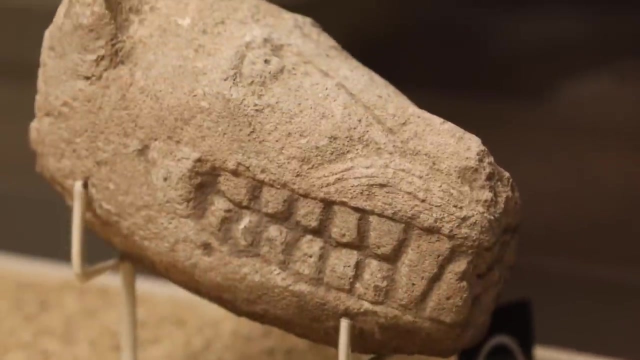 agriculture by the end of the lifespans of their settlements. When compared to the common model of previously discovered early farming communities in the Near East generally located further along the Levantine shore to the south, Gobekli Tepe and its sister sites offer a very different point of view. 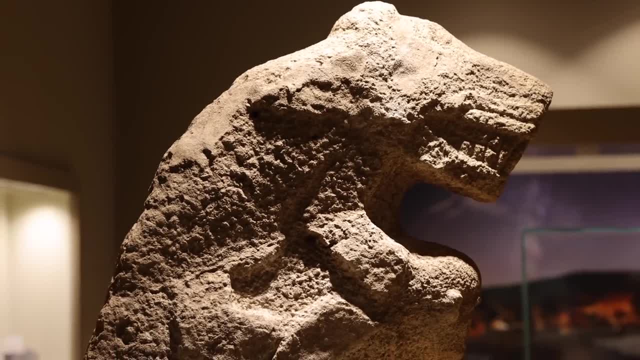 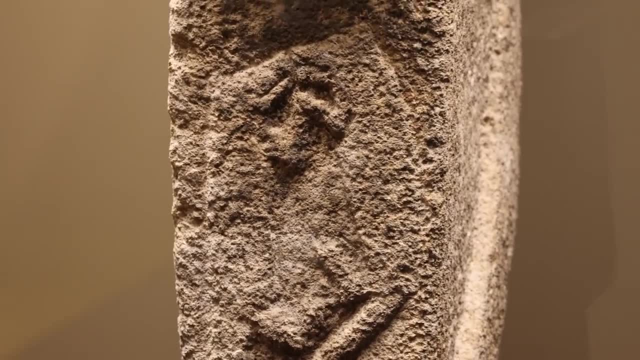 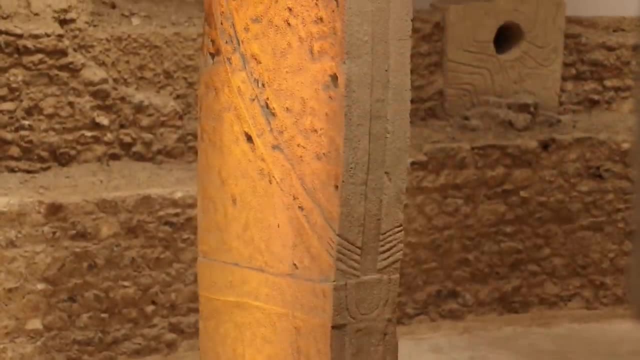 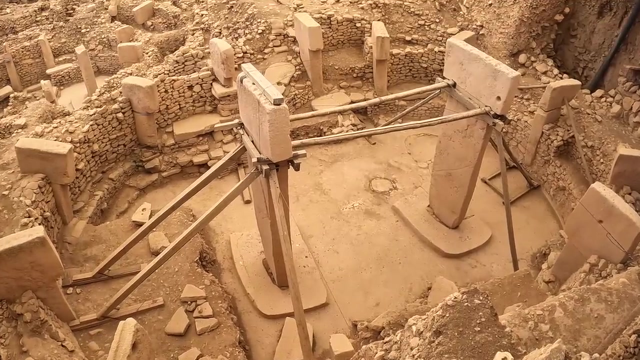 Here, rather than domestic dwellings, the utmost effort seems to have been placed in creating monuments of a non-utilitarian nature: Peace. Vast amounts of time and energy going into creating more than 200 T-shaped pillars, the largest of which stand three or four times taller than the height of a person. 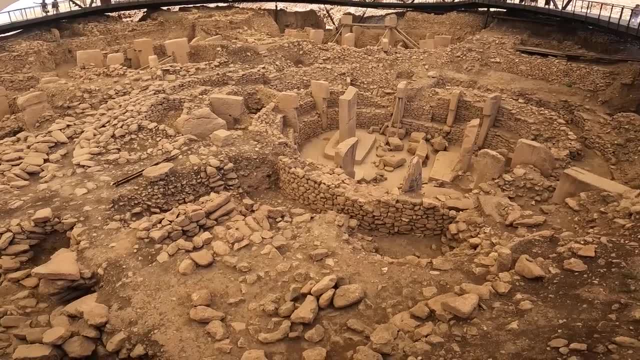 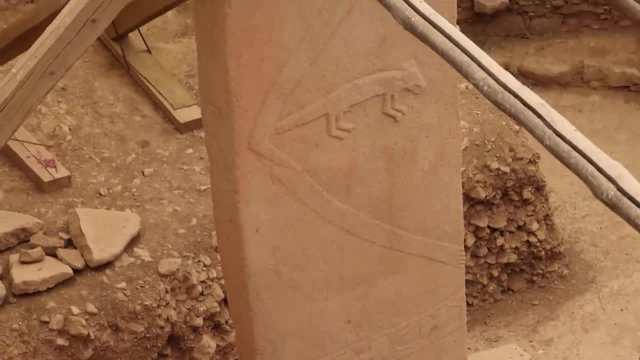 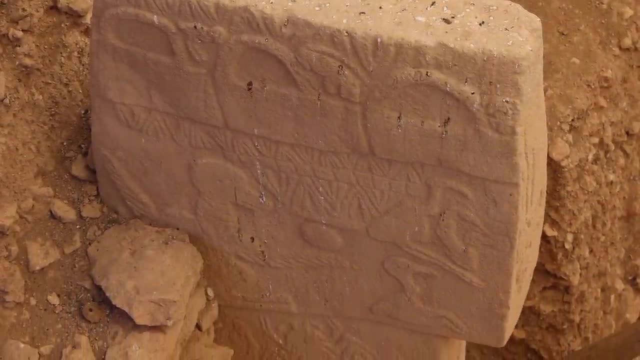 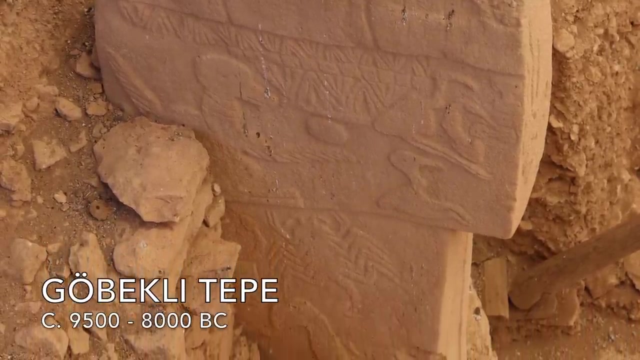 Intricately arrayed into at least 20 stone circles coated in carvings Stretching for some 25 acres. the place was clearly of the utmost importance to all who took part, Only to be intentionally filled around 8000 BC, consigned to oblivion at the end of its life. 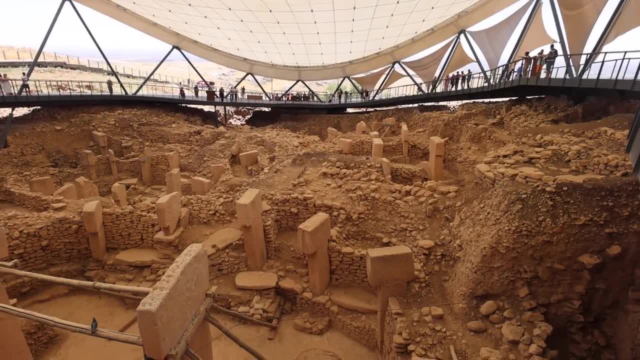 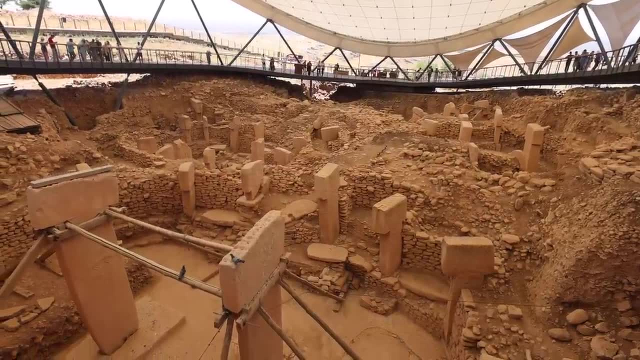 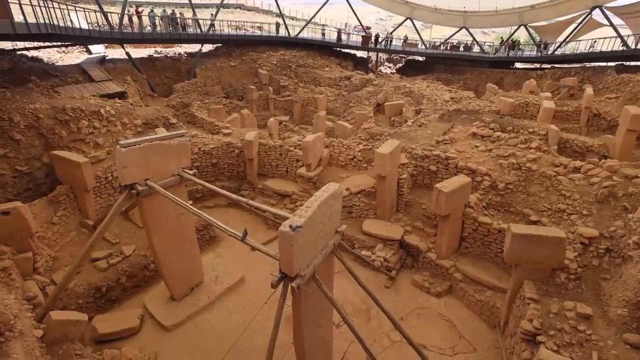 Even more paradigm-breaking was the fact that it was the earliest levels that yielded some of the most important buildings in the world: One of the largest and most impressive pillars and animal carvings. In complete defiance of conventional logic, the monoliths seemed to get smaller and more modest over time. 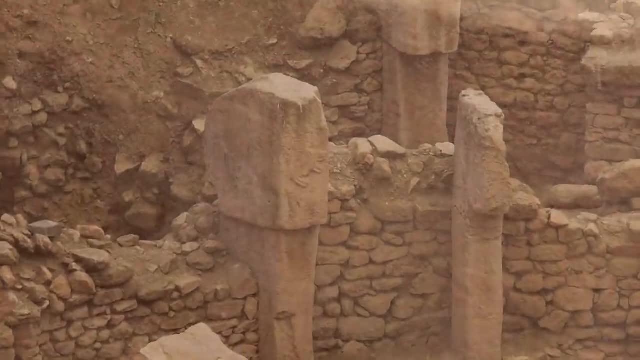 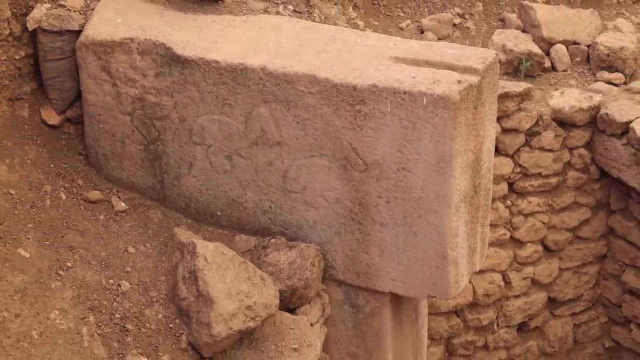 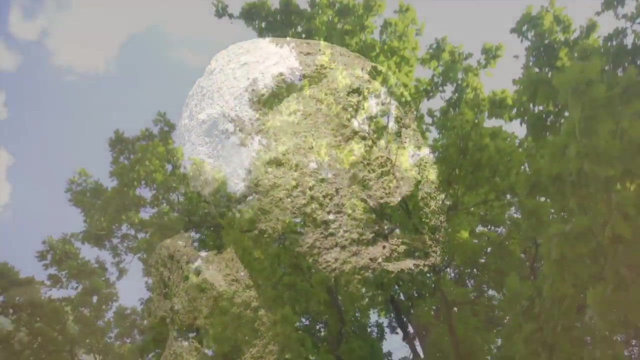 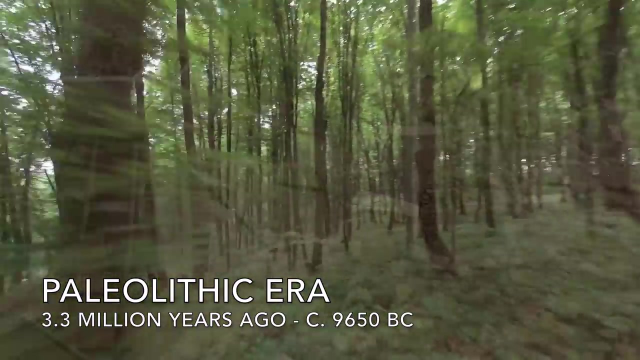 Far from a hypothesized beginning of all things, Gobekli Tepe seems curiously like an end Hinting of a great mythological tradition stretching far back into the perennial mists of the ice age. It's even possible that long-lost wooden circles preceded it. 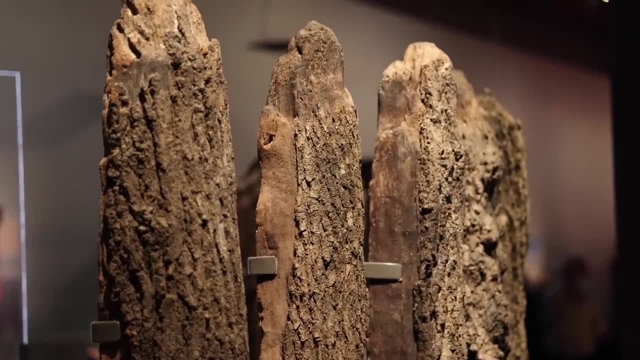 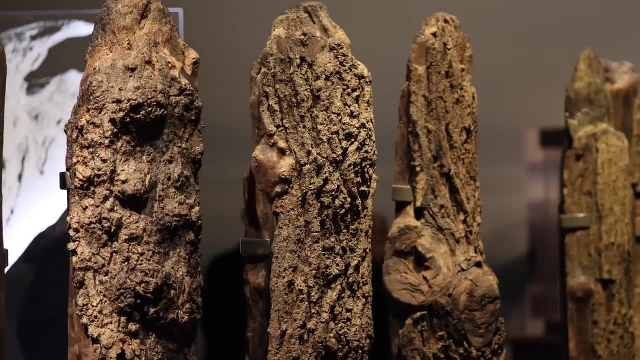 Similarly once vaunted monuments that rotted away to oblivion so many thousands of years in the past. That gave glory to the great rév, defiancement and contentment of the island's antiqued heritage, which in turn reACHED the cutting edge of medieval antiquity. 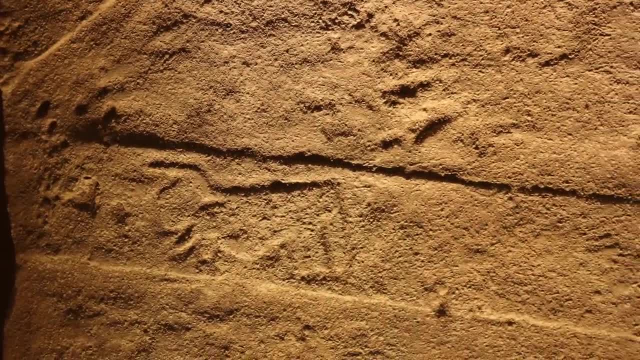 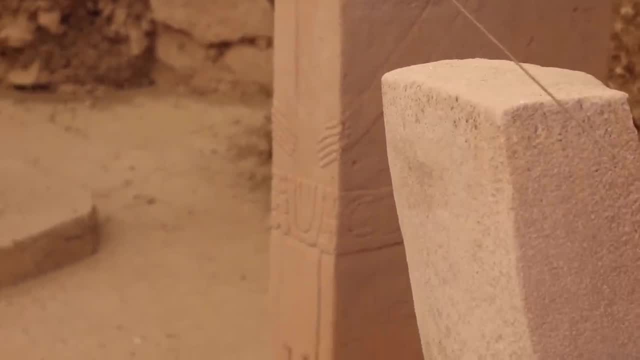 For Klaus Schmidt, ever living in hope of finding a foundational cemetery site under one of the enclosures, And partly in light of arms and hands having been found adorning some of the pillars, They perhaps once, having Nós, represented individuals. The process of discovering and entertaining can be inconvenient at times. 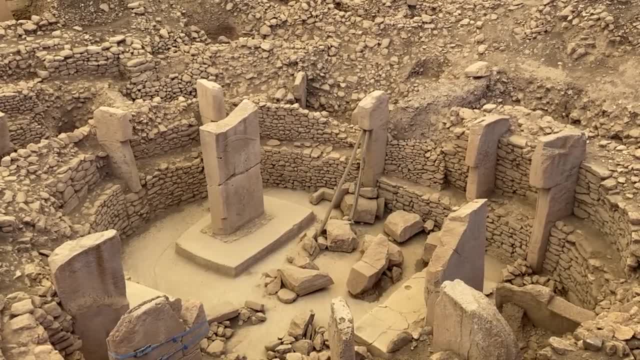 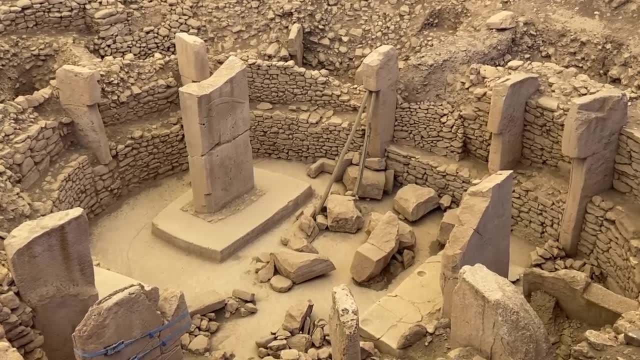 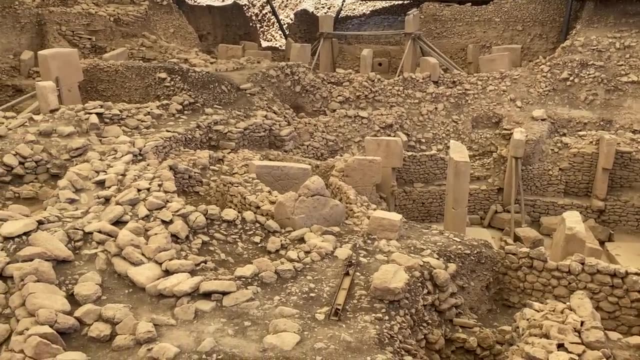 10, The site may have been a monument to 19ital enthusiasm to Влад毘 ancestors. Clearly, whatever its purpose, this was a place built with great skill and care. The seven metre long threaded pillar still lying in its quarry on the 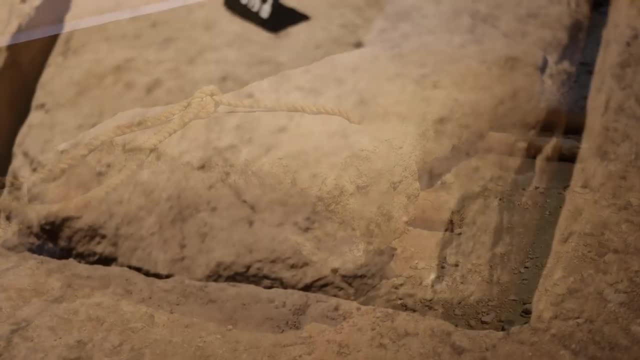 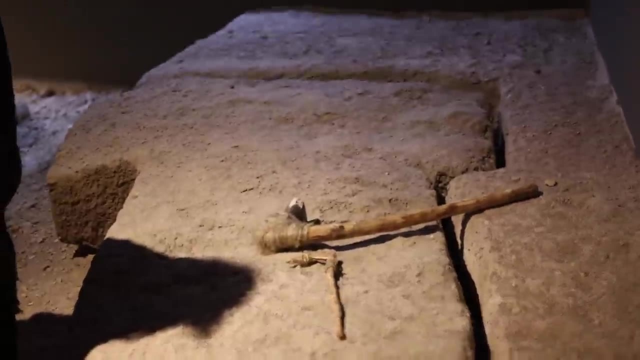 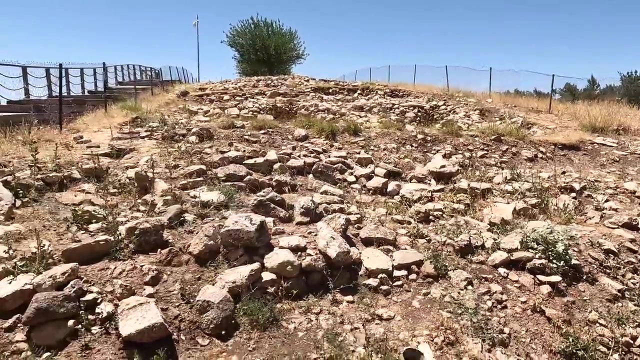 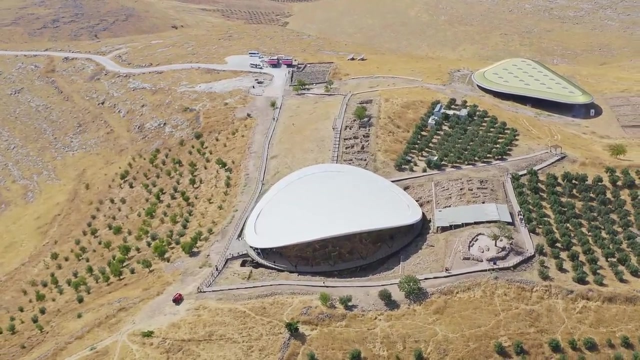 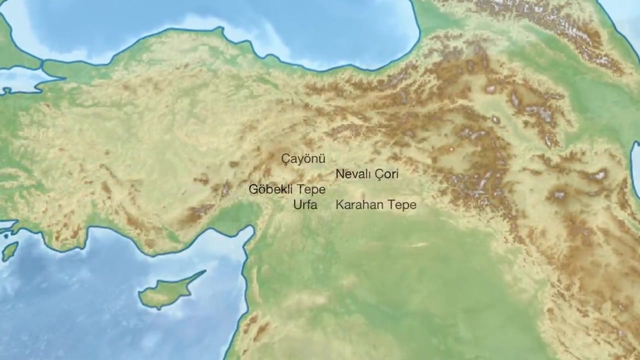 northern plateau tells us that much- with other quarry sites found around the hill, Though it wasn't only construction technologies that were in use here, but logistical support networks just as well developed as the mythology and ritual lives of this most ancient of prehistoric societies, Far from 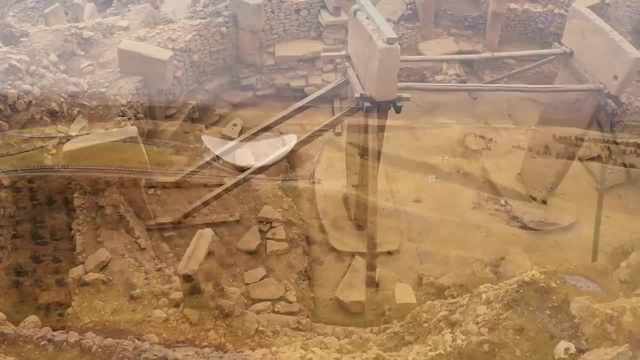 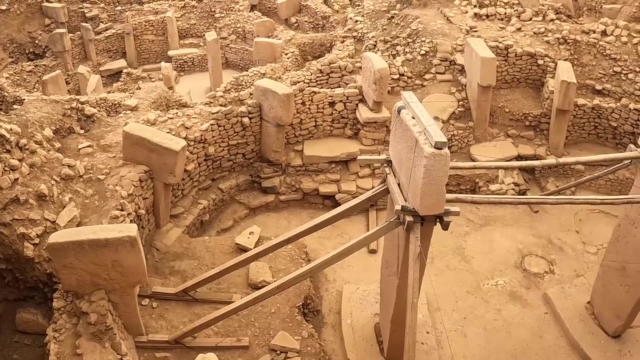 long-standing construction projects put together over lengthy periods of time. the archaeology suggests each enclosed structure was built in a way that was really getting work done. Both the material and the material would be actually cut up to make the structure. There was also a department of the 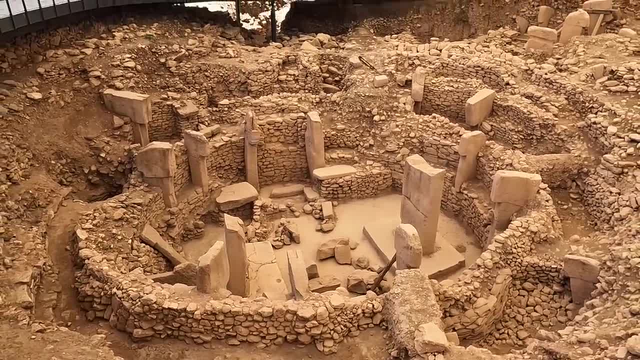 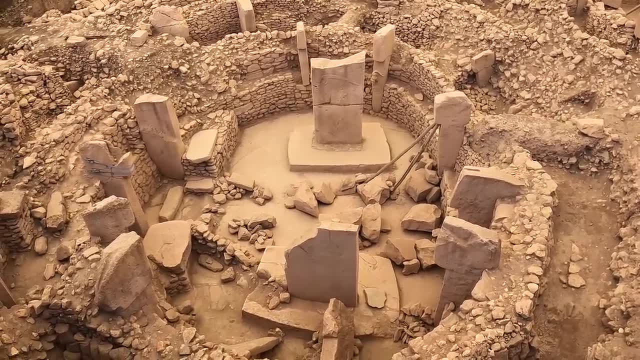 actual structure and a particularly Ratio of that structure might indeed have been particularly used, due to the natural situation of the location, Without the Şuhrer's land, in areas that were abandoned or gigantic and almost completely unorganized. Schmitt hypothesised that around 500 people would 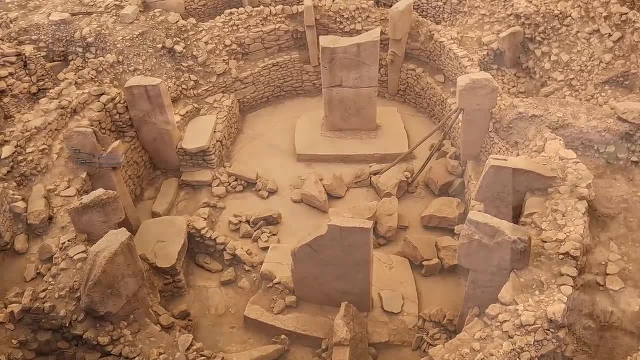 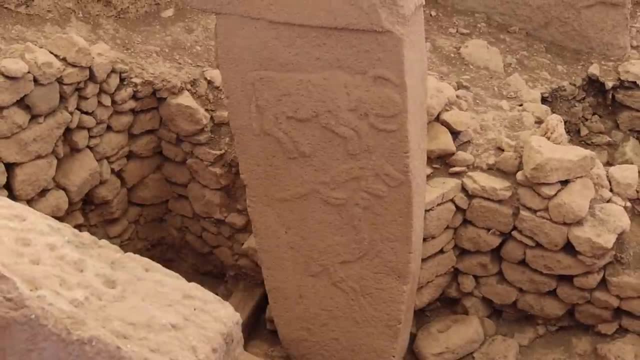 be required as labour. Further speculating on the existence of some kind of priestly class to plan, organize and contextualize the work, Schmitt revealed the idea that the structure was a space that could be used to store or store personal objects or 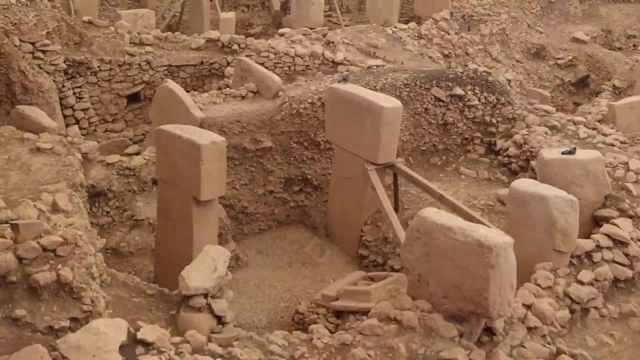 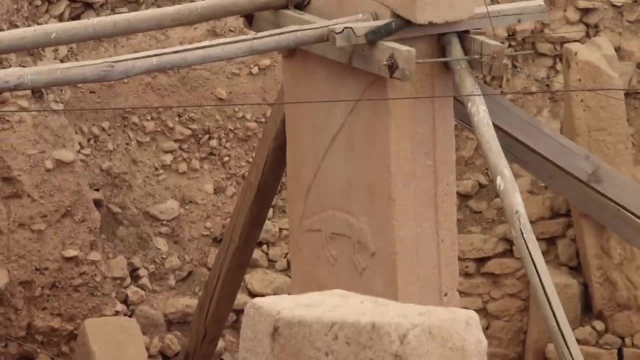 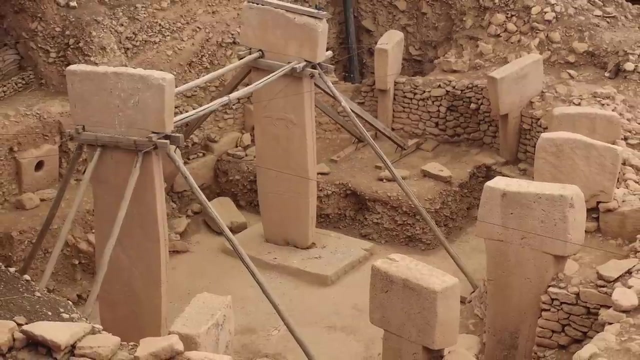 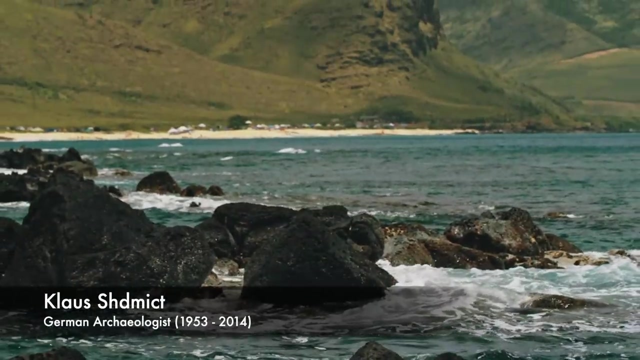 other objects of any kind. Perhaps either intentionally or inadvertently united in a singular purpose, it had the effect of binding the group together, a form of communal worship operating as the social glue. Since Klaus Schmidt's death, an increasingly wide range of alternate hypotheses have been. 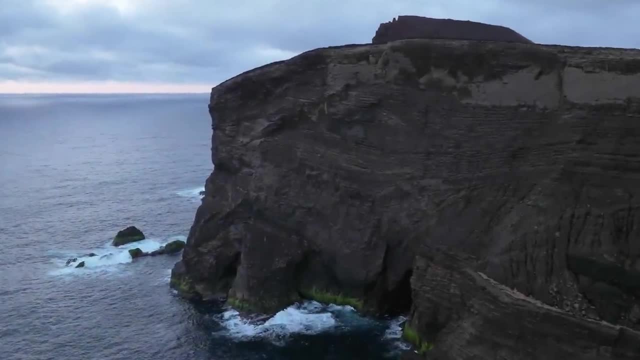 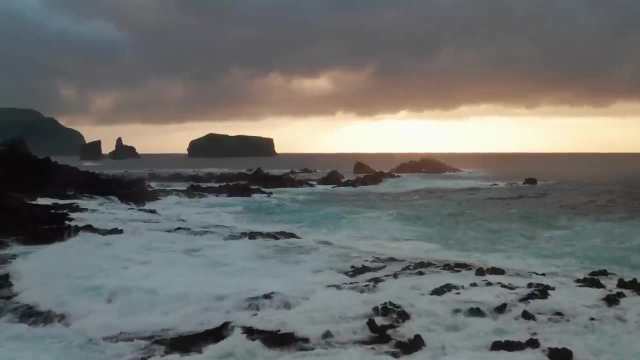 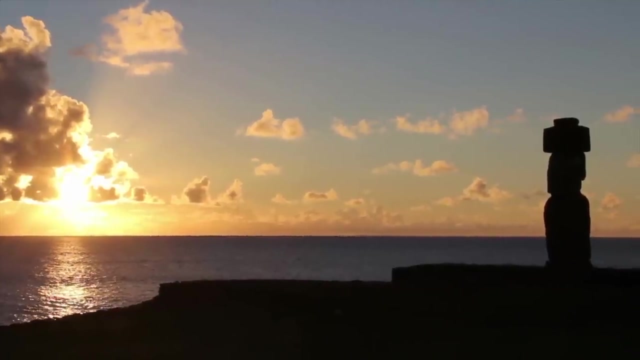 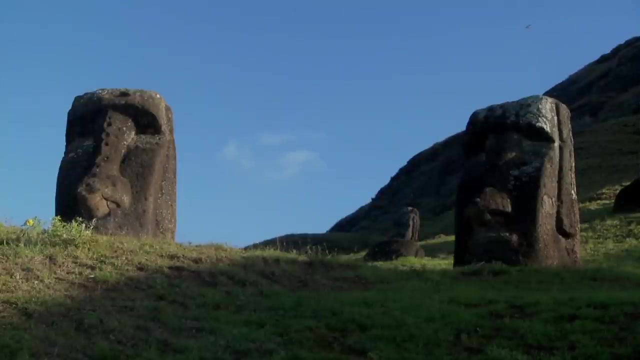 discussed too Far away in the midst of the distant Pacific Ocean. experiments with the megaliths of Easter Island have shown that the Moai there could in fact have been crafted and erected by significantly smaller groups of people than Schmidt's hundreds. In one experiment, just twelve men were able to find the Moai. 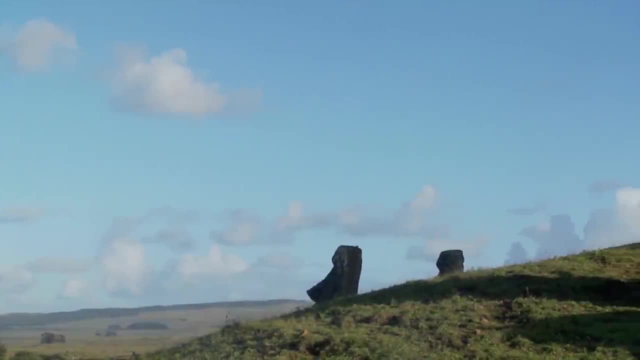 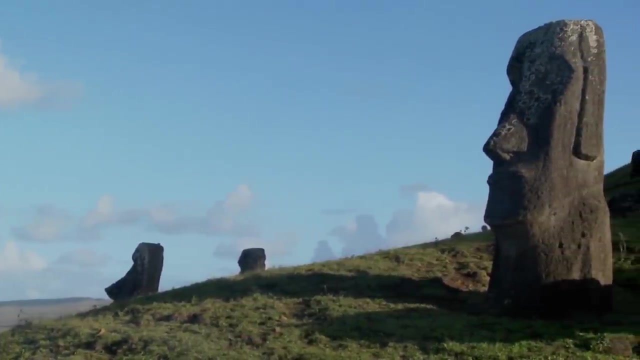 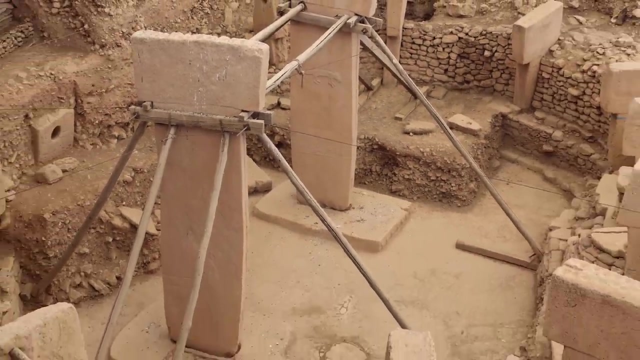 They were able to raise a 20-ton statue in just under three weeks. It is plausible, though by no means definitive, that Schmidt overstated the amount of labour needed at Gobekli Tepe, with just a few dozen individuals potentially having quarried and. 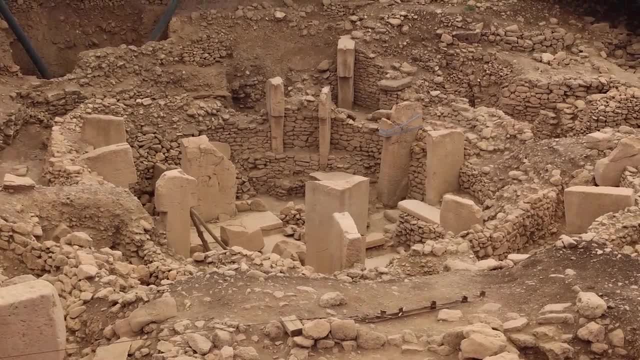 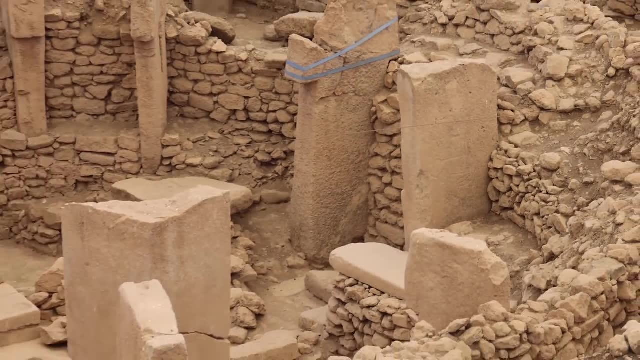 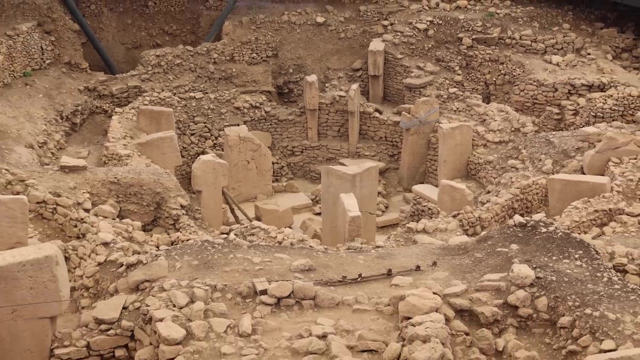 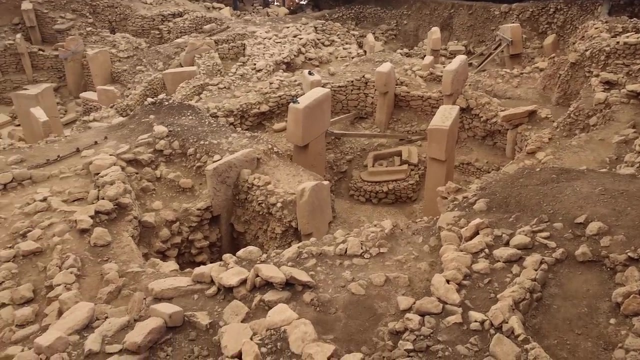 erected the monoliths there. Given the sunken nature of the enclosures and the particularly impressive floors within, it is also possible that the megaliths did indeed once support roofs, an artificial cave rather than a temple to the star-studded sky. 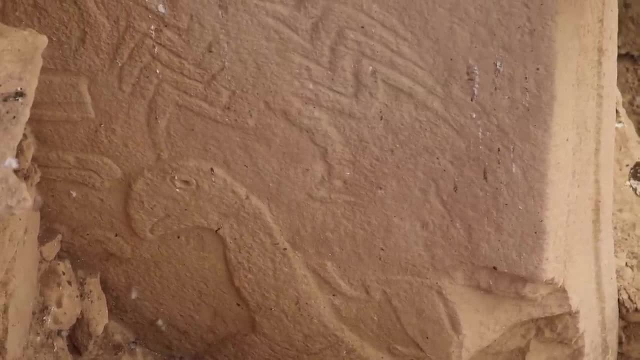 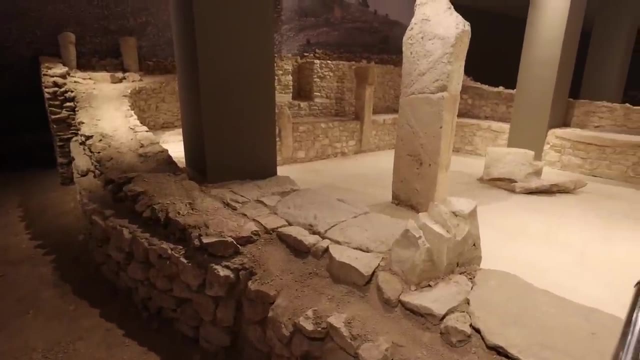 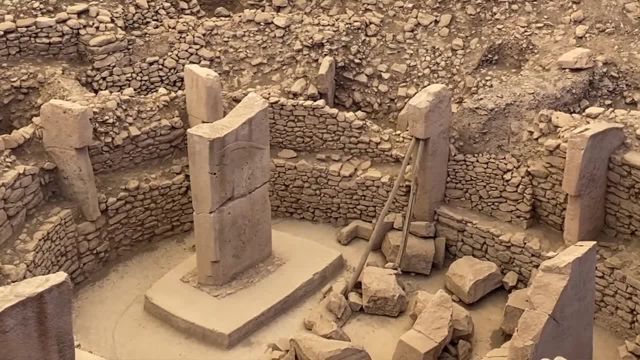 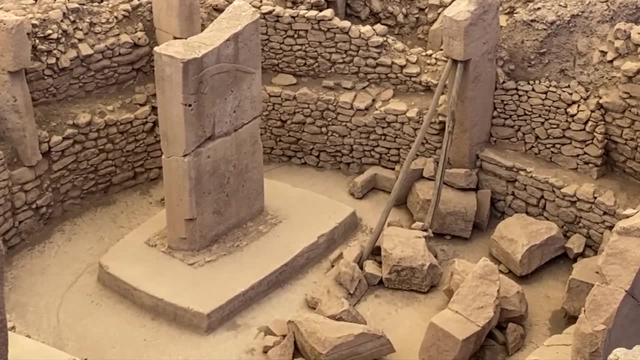 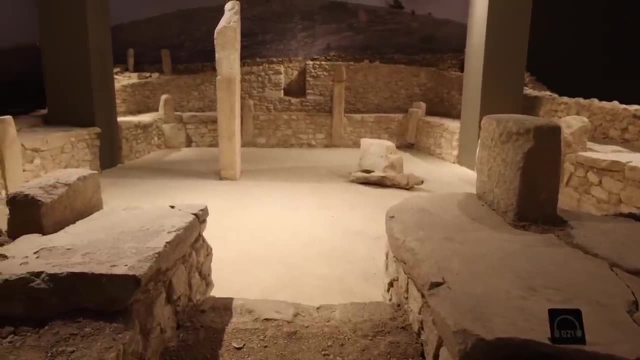 Tepe was made in a style known as Tarazzo — the earliest such examples found anywhere in the world — laboriously created by layering burned lime and clay over and over again to create a smooth, luxurious surface. At Na´valichuri and Chianu, though, 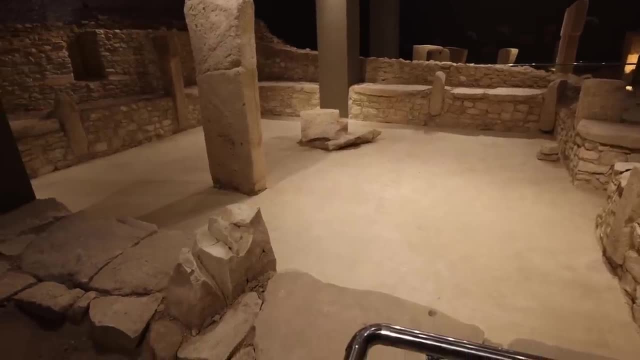 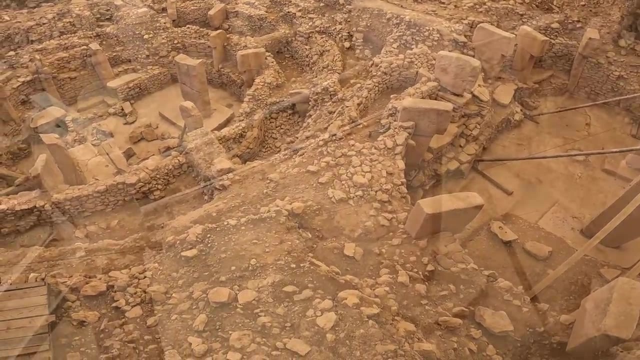 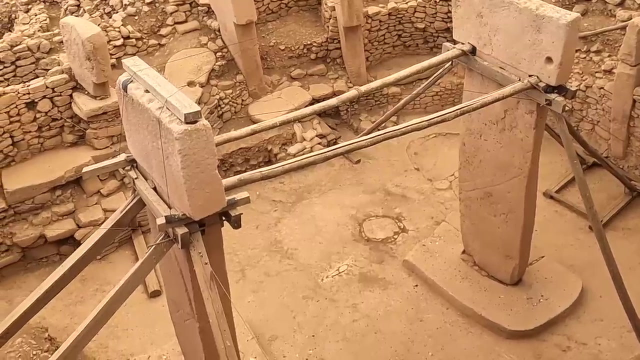 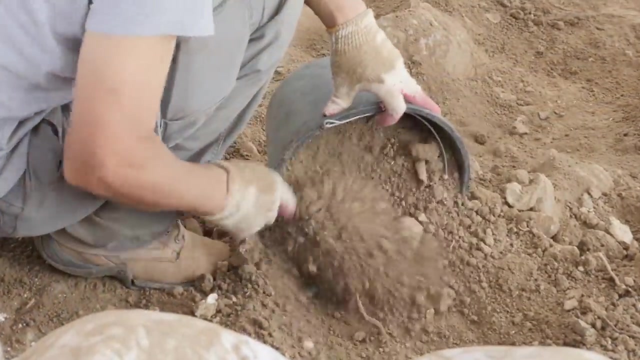 Only one example has been found At Gobekli Tepe. they appear over and over again, In one case four terrazzo floors having been built directly on top of one another down the long generations, For all the work of an army of scientists and scholars. 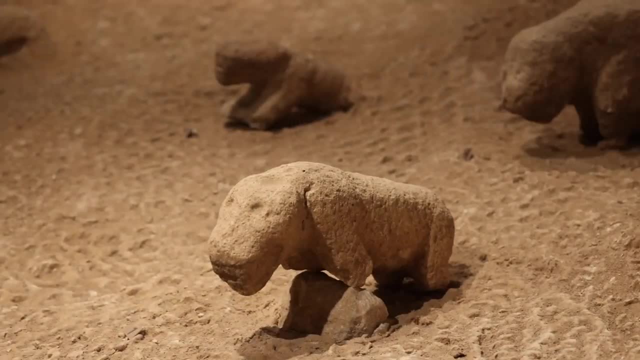 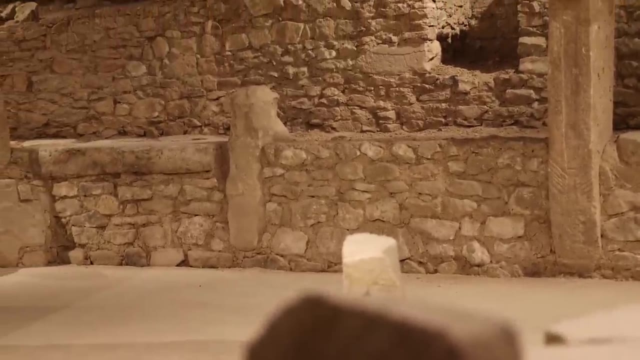 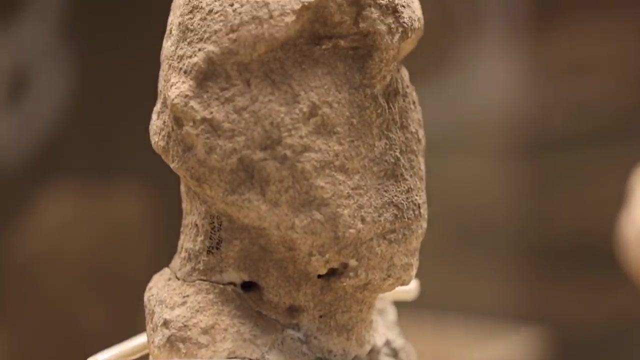 it of course remains impossible to fully reconstruct the interactions of that long-gone culture today, Of how the people at Gobekli interacted with Chianu, Nvali, Chori, Karahan and the others, Whether they borrowed elements from each other into their own way of life. 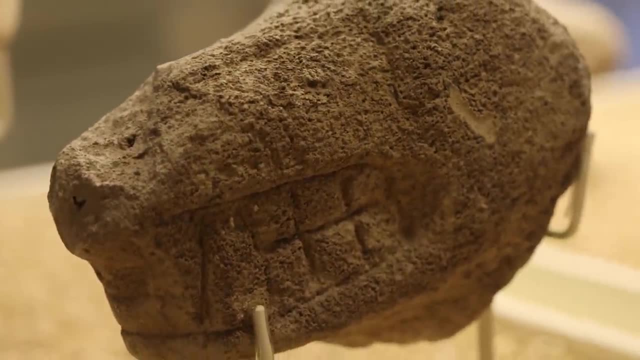 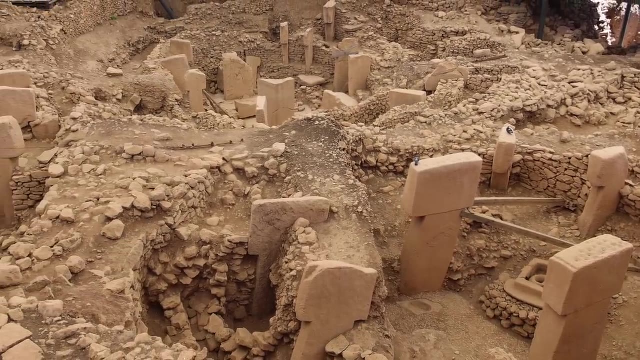 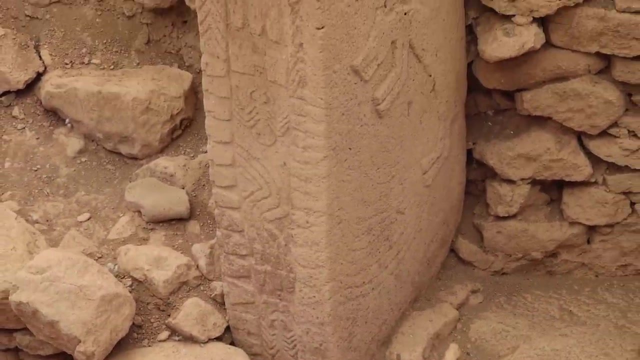 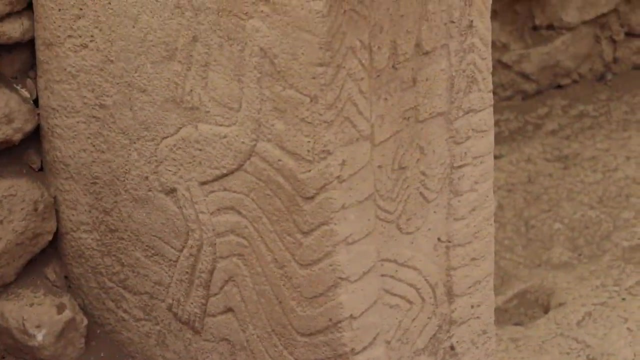 Whether they already shared the same culture and stories. However, the same themes do crop up again and again, Most obviously in the myriad carvings and bas-reliefs that march, crawl and fly over every visible surface. Almost all of the depictions are of animals. 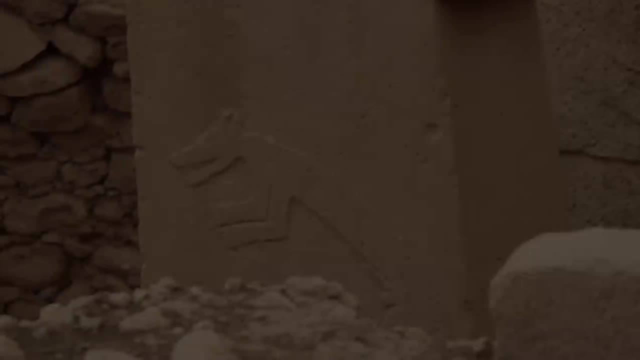 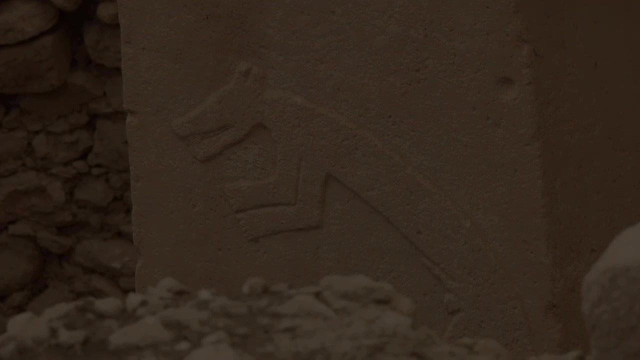 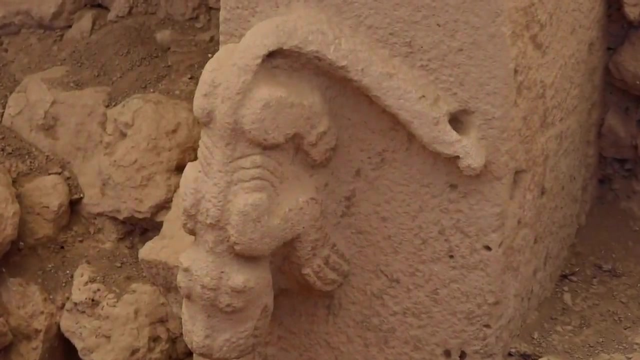 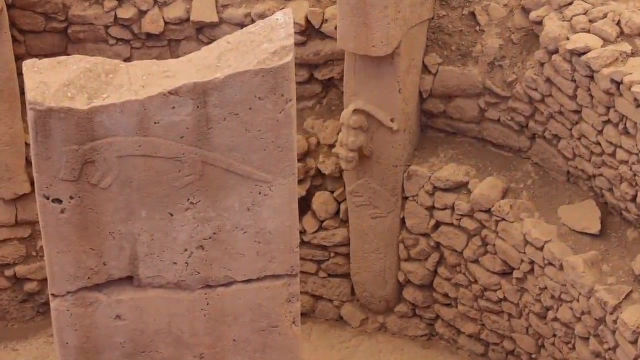 Appearing so fully formed and so near unfathomably old to be difficult to comprehend. It is these exceptionally artistic carvings that give us the best chance of bringing back from extinction just a little of that clearly well-developed ancient culture, Giving us some insights into just why this place came into being. 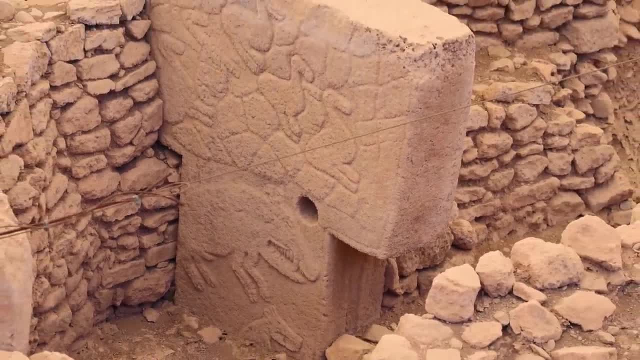 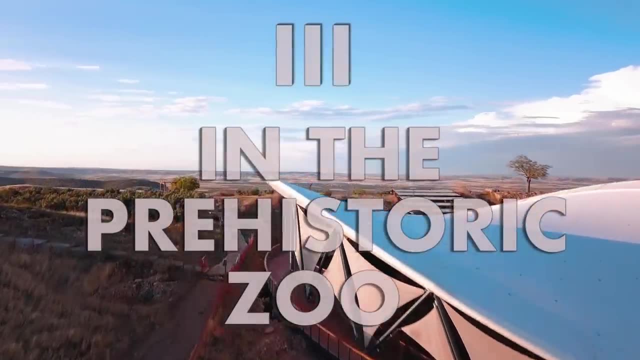 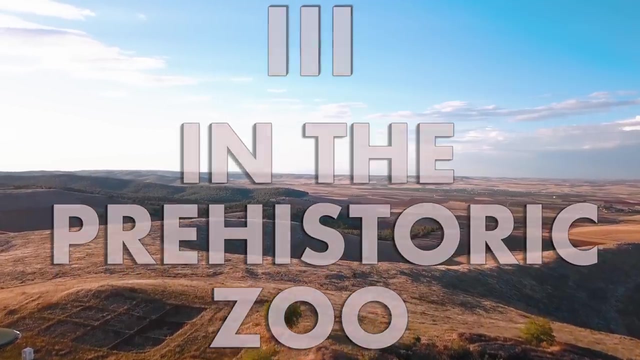 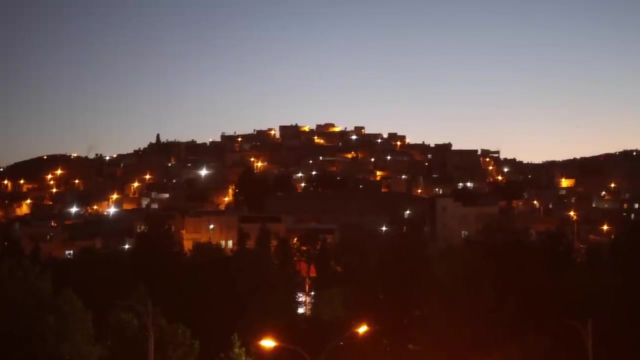 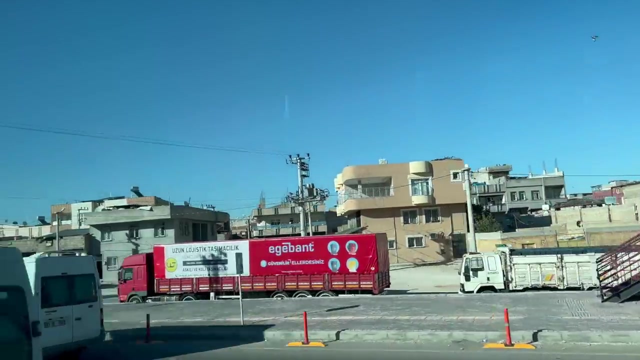 And some inkling into the long road to our world Which may have been forged in the process. In 1993, just before the discoveries at Gobekli Tepe, construction workers digging around the Balacagal area of the Urfa city centre came across something they weren't expecting. 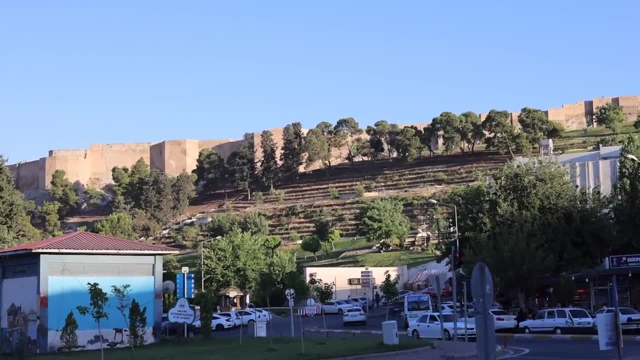 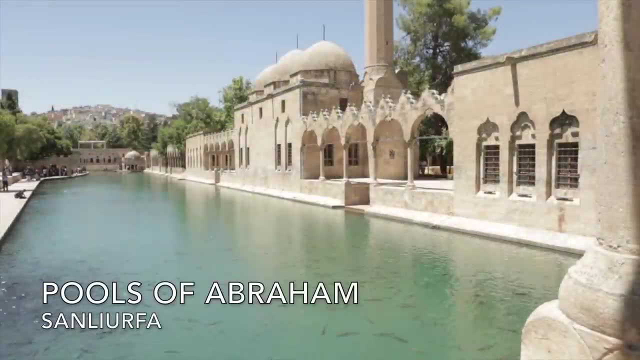 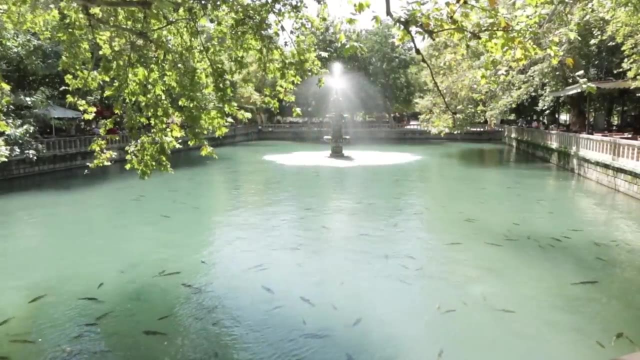 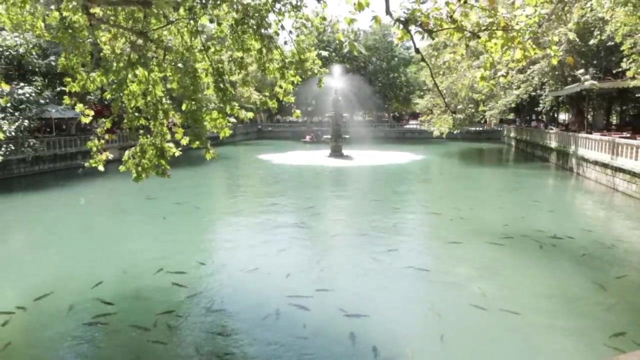 And it was the work of a famous sculptor, The ancient and most important piece of art from the early 19th century, The ancient deepwater springs known today as the pools of Abraham Blank. lifeless eyes stared back from the foundation rubble Prominently displayed today in the cutting-edge new museum at the heart of the city. 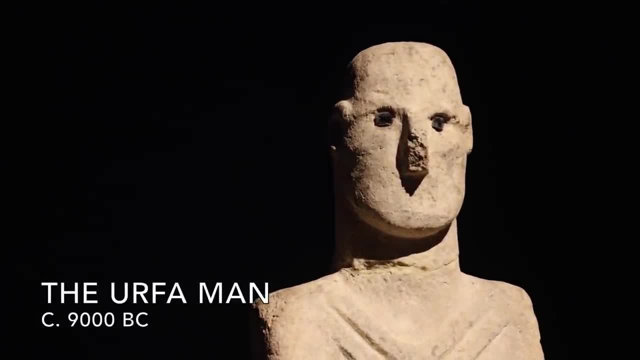 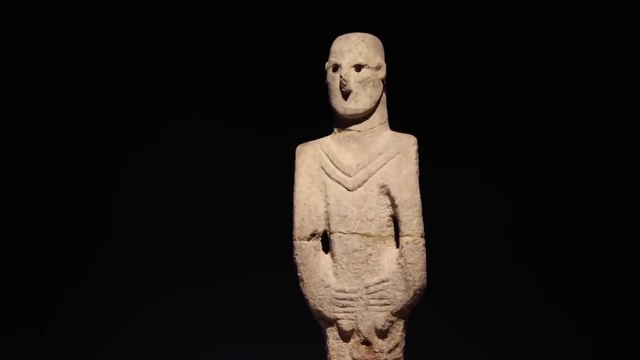 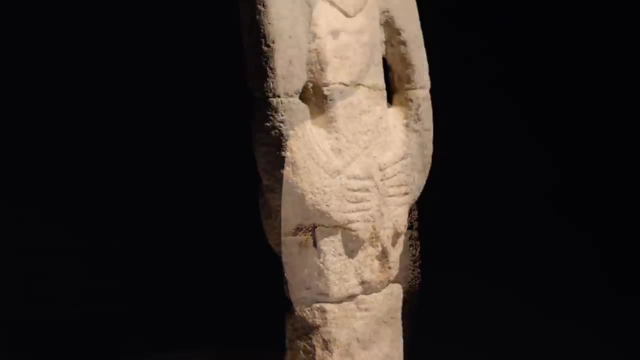 Prominently displayed today in the cutting-edge new museum at the heart of the city. The Urfa Man stands at 1.8 metres tall At around 11,000 years old. it is the oldest life-sized naturalistic sculpture of a human ever discovered in the world. And though very heavily damaged by construction work down the long millennia since its creation, when briefly investigated in 1997, before construction work was finished, the earth around the statue turned out to be a pre-pottery Neolithic settlement with similarities to Gobekli Tepe. 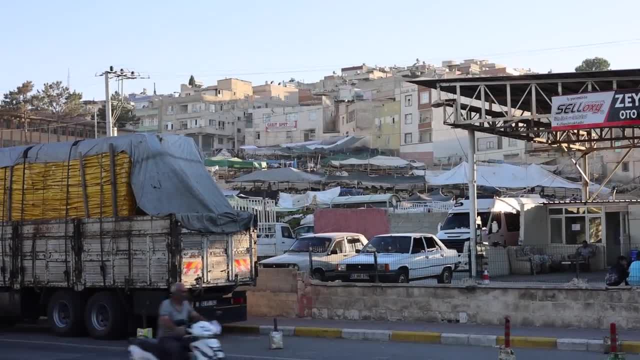 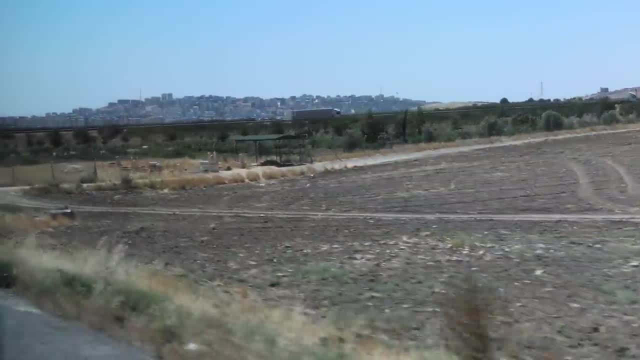 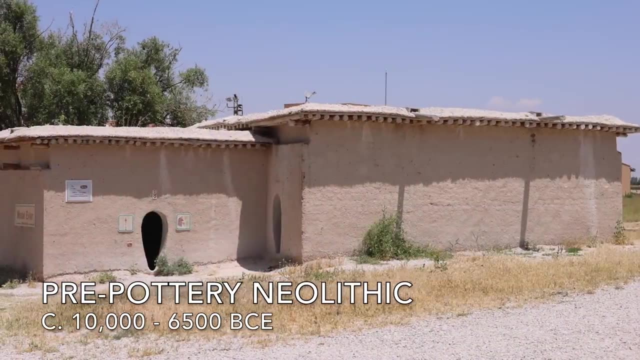 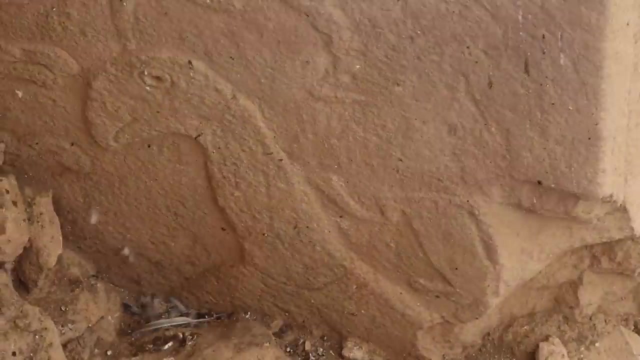 Concrete evidence of the deep antiquity of the city. And yet the sculptures at Gobekli Tepe are quite different from even the pre-pottery Neolithic world. at the very beginning of agriculture, Theirs was a symbolic landscape populated almost entirely by the wild. 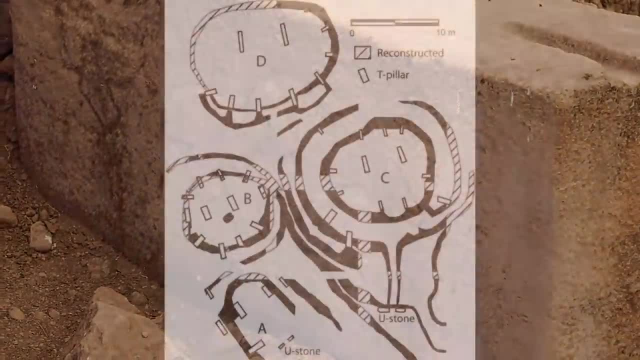 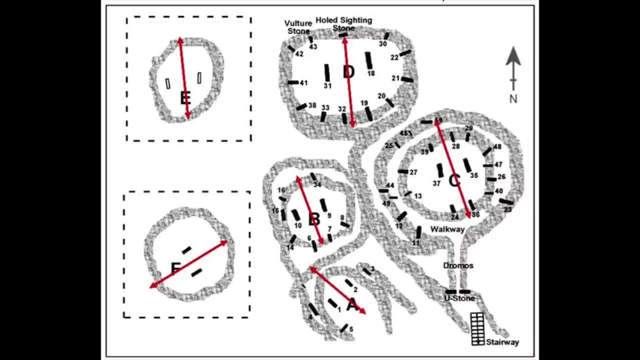 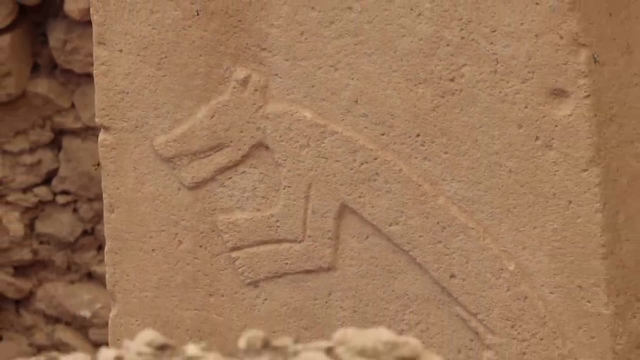 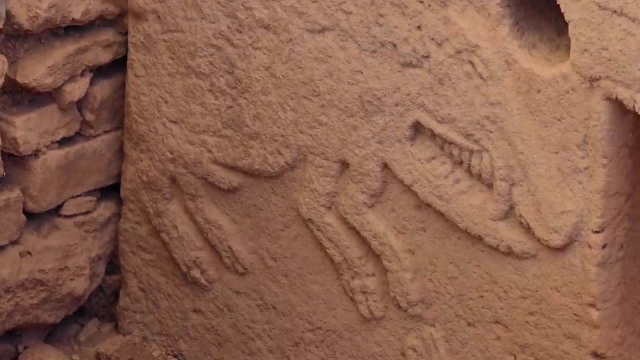 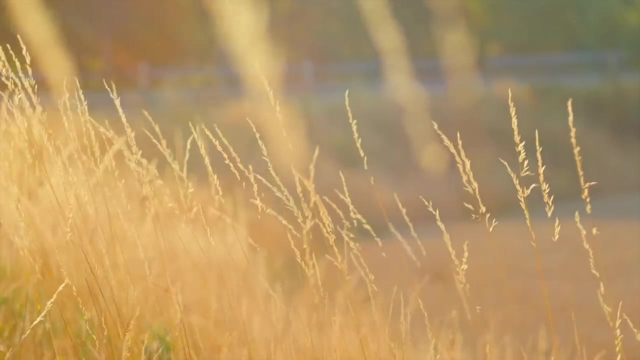 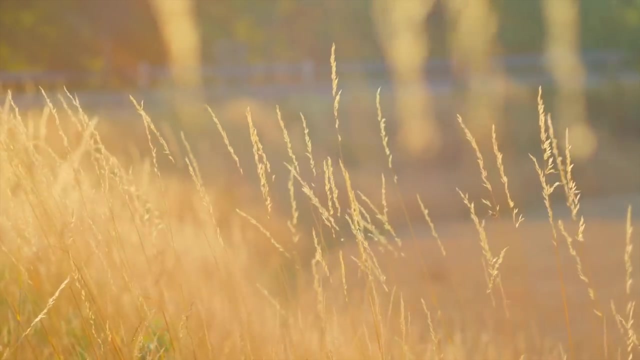 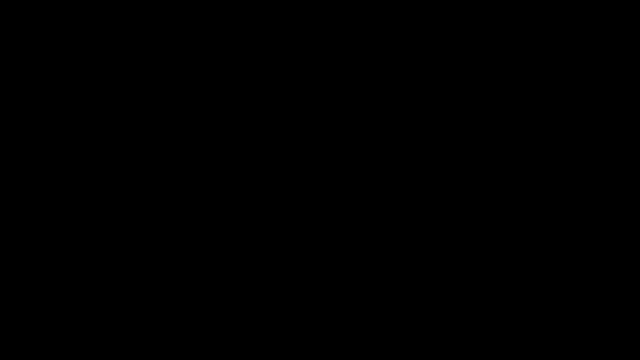 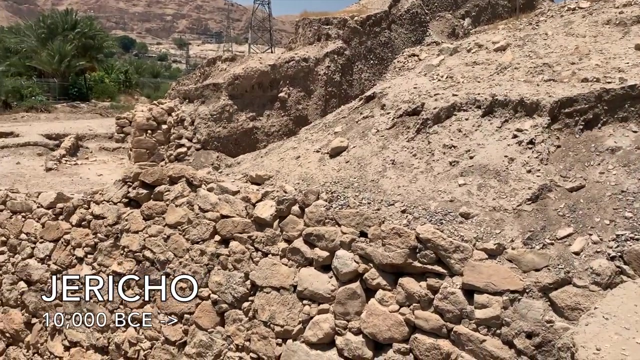 powerful animal forms are displayed, often depicted with prominent penises. For some reason, unlike in early near-contemporary farming societies, the female form is almost never depicted. No clay so-called Earth Mother figurines are to be found Here, in a quite different culture to that of the South, at places like Jericho, the 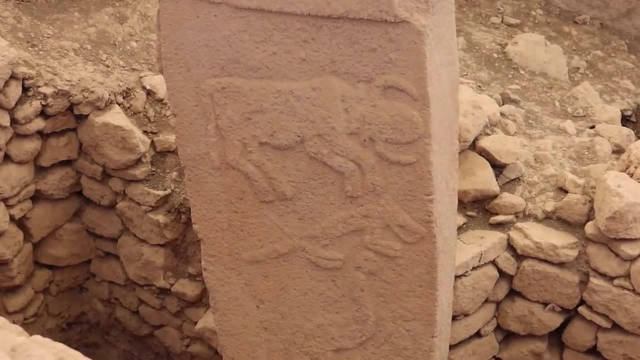 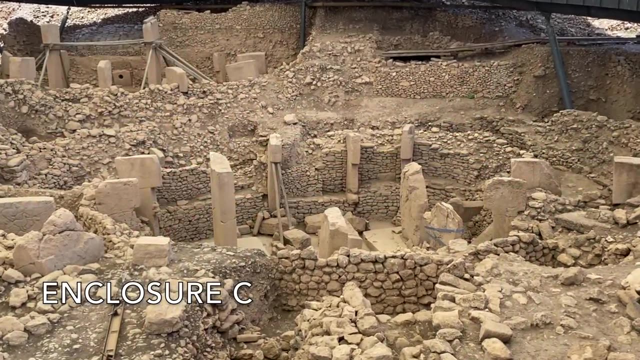 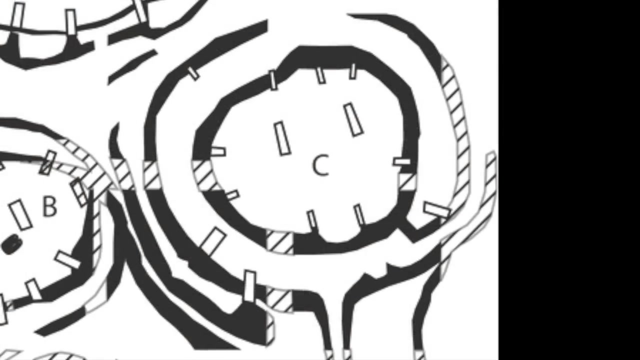 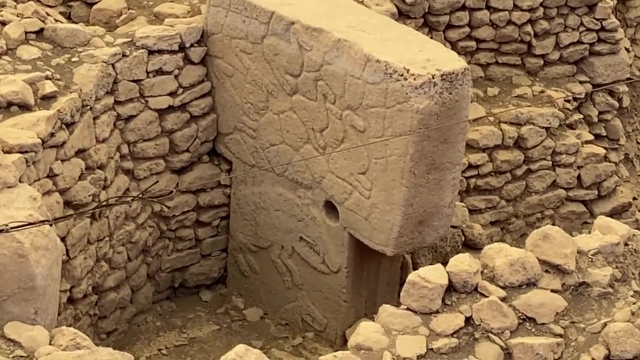 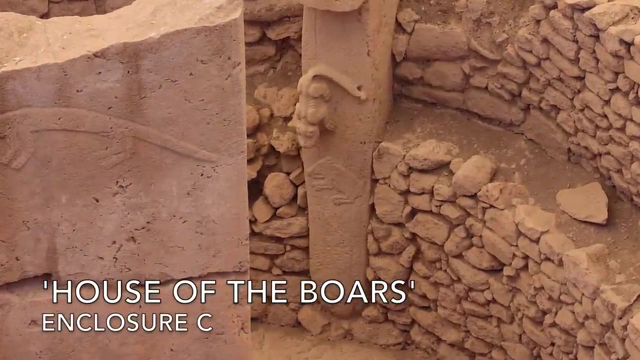 ferocious world of the Hunters took precedent In Enclosure C, where three concentric rings of walls were successively built up one after the other over the years, gradually receding the size of the interior. feral pigs dominate In this so-called House of the Boars. wild pigs bare their teeth menacingly. 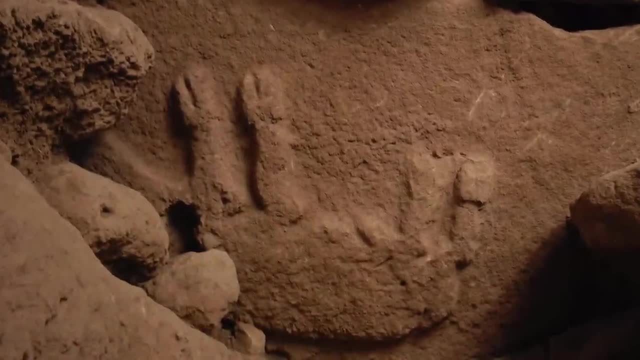 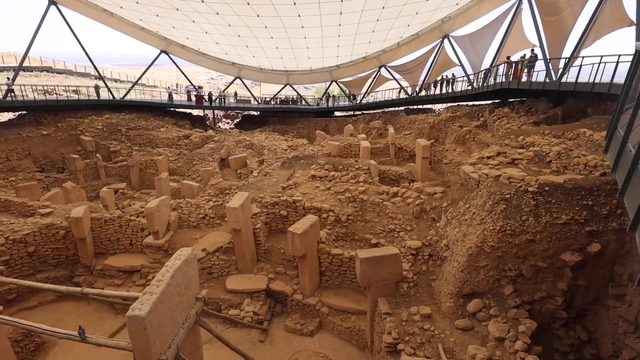 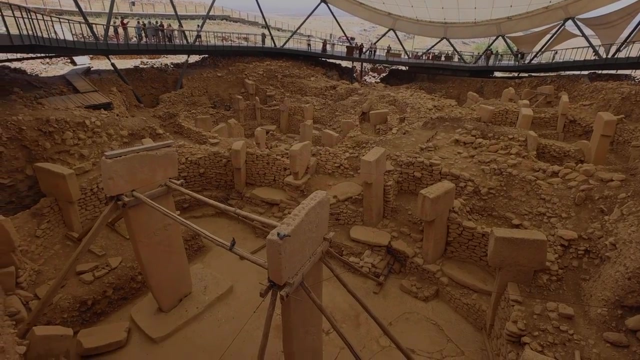 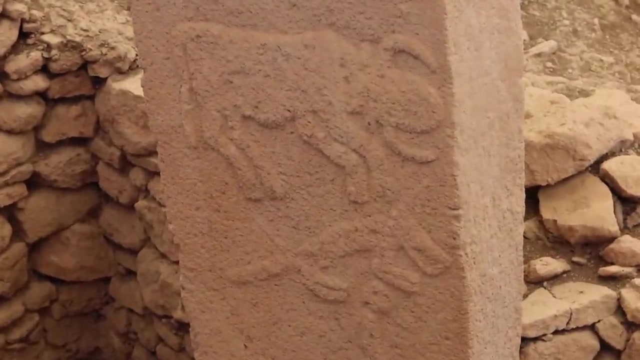 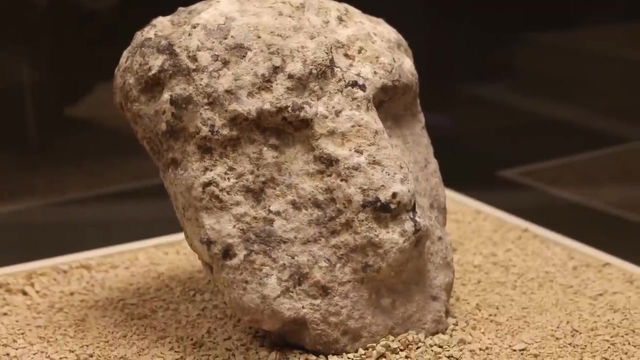 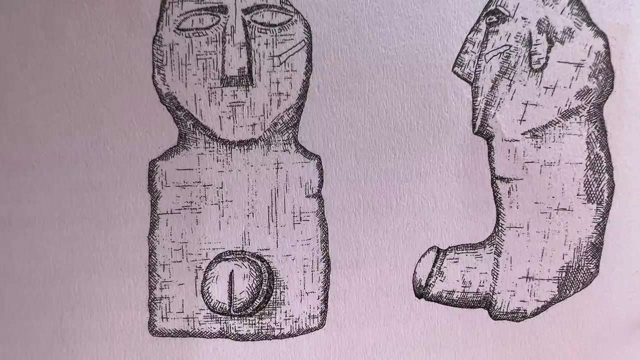 Another lies on the ground. Another lies on its back, deceased. perhaps Almost all of the animals are male. Several depictions of human skulls are found, too, ranging from the small to larger than life, Some also displaying prominent and erect penises. 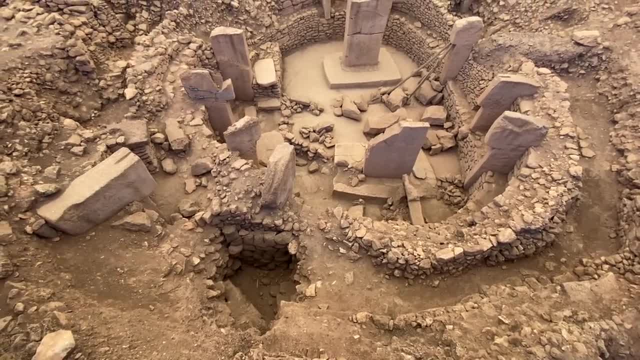 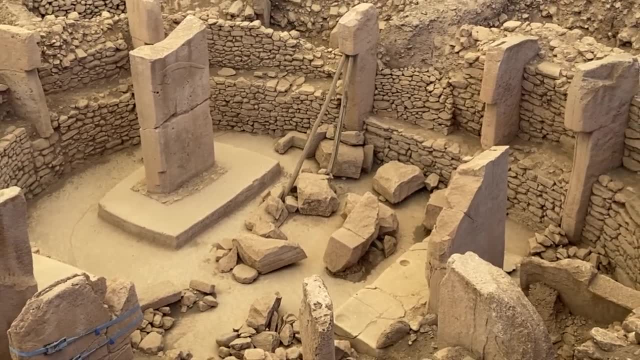 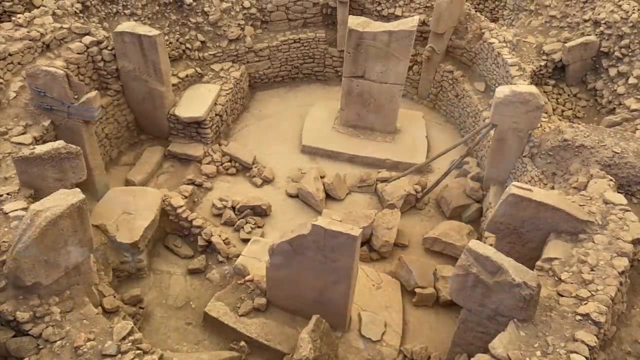 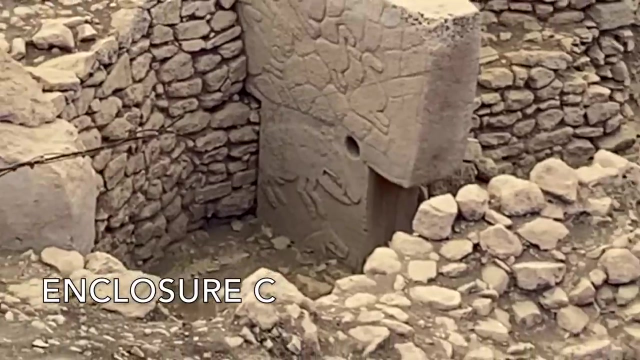 Unexplained holes. stepping stones and small cups are found too, with suggestions being made of stands for small fires to light the enclosure during the night. Interpretations of the enclosure Range from the cultic house of a clan utilising the boar as a heraldic totem to a nightmarish. 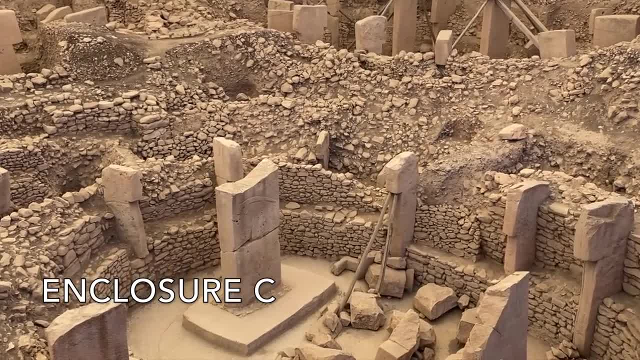 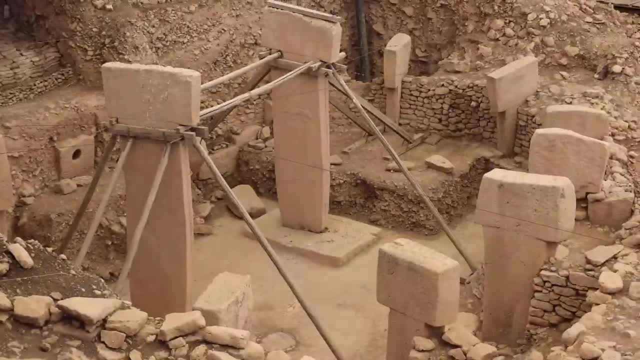 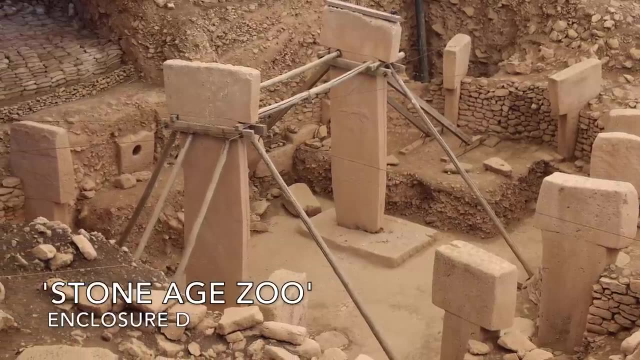 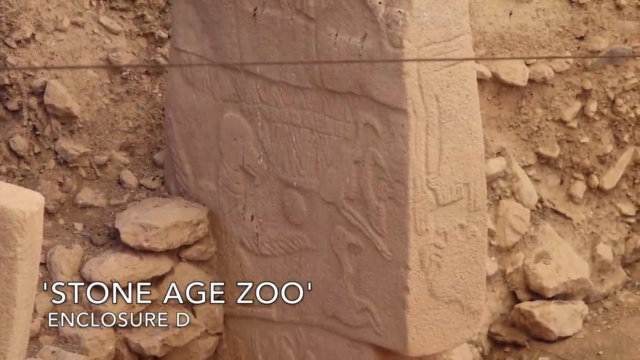 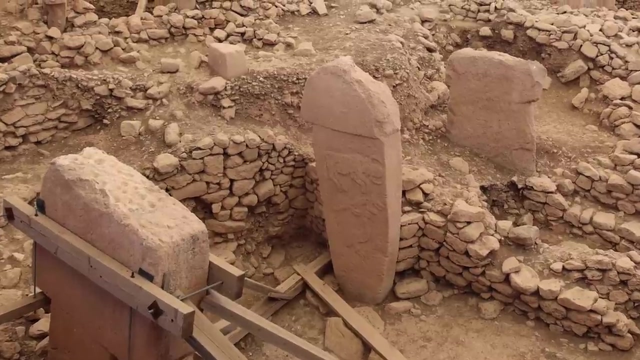 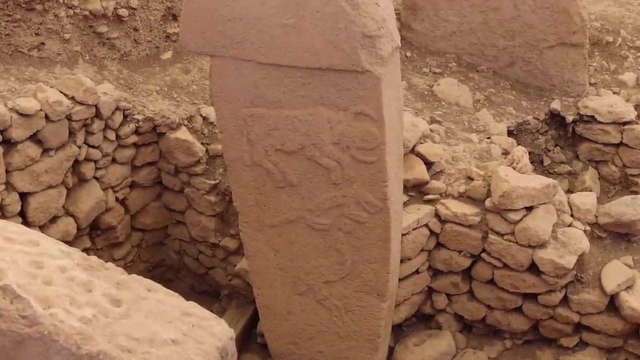 depiction of beasts guarding the entrance to the underworld. Inclosure D, which Klaus Schmidt fondly referred to as the Stone Age Zoo, is a much more varied affair: A veritable smorgasbord of fauna on display. Like enclosure C, a fox can be seen darting around the other creatures. 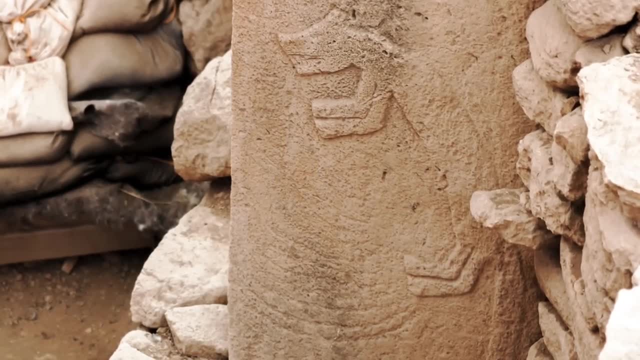 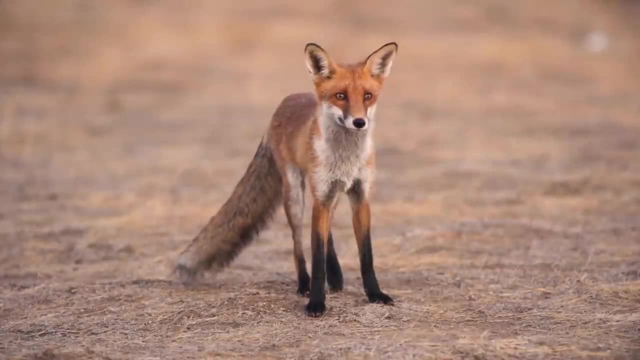 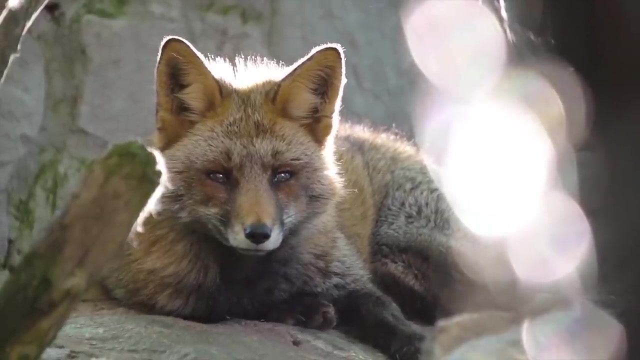 Though this one has snakes coming out where his penis should be. Inclosure C: The fox, The old fox, long seen as particularly wise animals in later Mesopotamian myth and beyond, and with links to potentially even earlier shamanic beliefs. 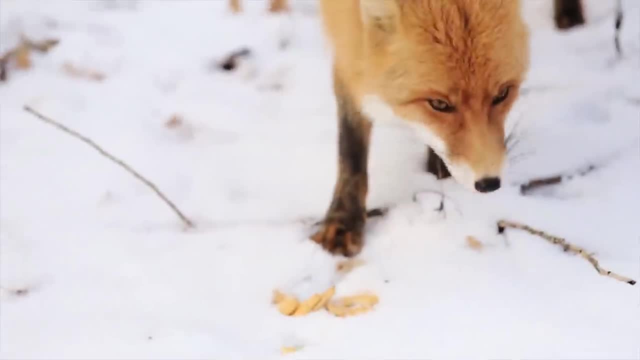 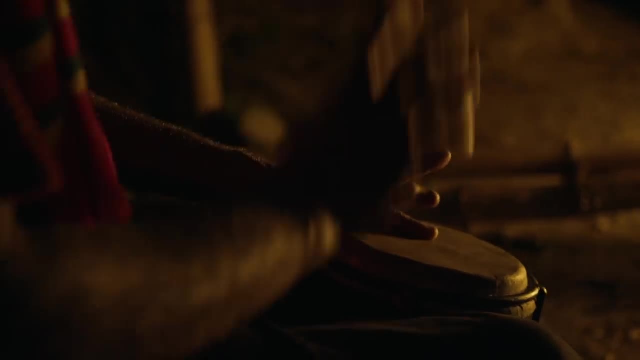 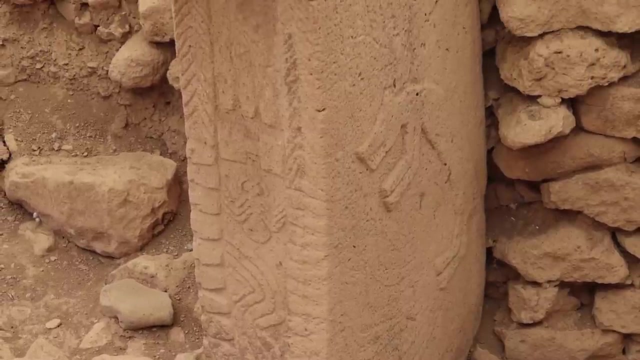 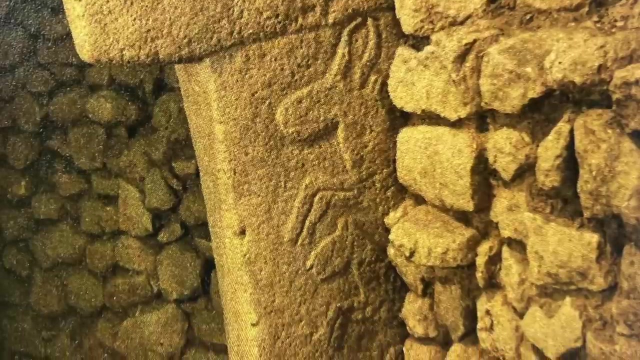 From all over the world. suggestions are often made of allusions to shape-shifting rituals and trances, with the fox representing the figure of the shaman Elsewhere gazelle gallop across the stones, Judging by their frequency on the pillars in many of the enclosures. 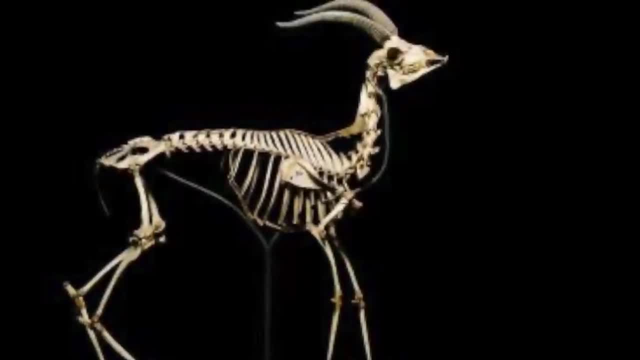 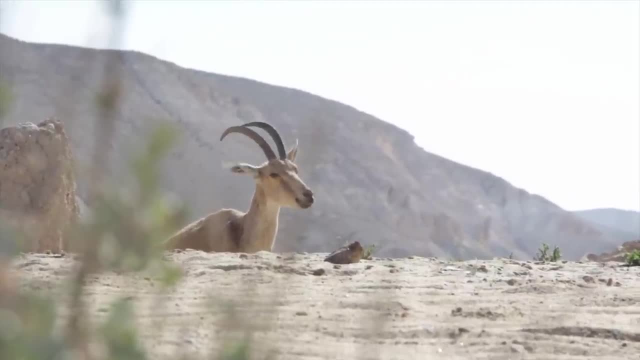 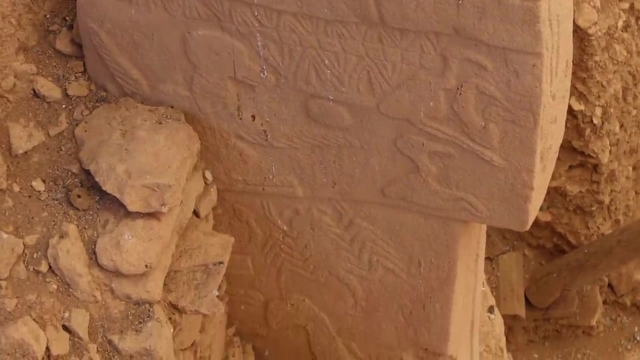 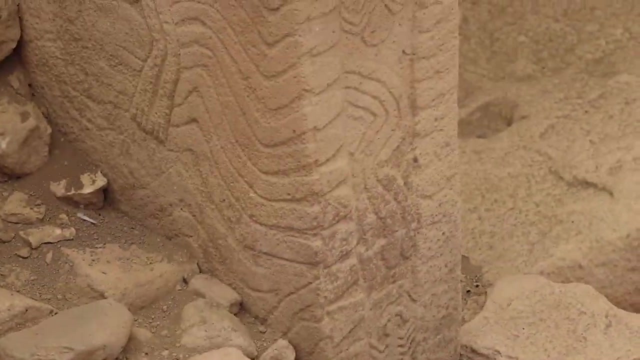 and in the skeletal remains they seem to be of particular importance. Vultures are seen too, creatures long associated with the realm of the dead. But other birds proliferate too. Cranes, a type of migratory waterbird, are common, perhaps suggesting some appreciation for the 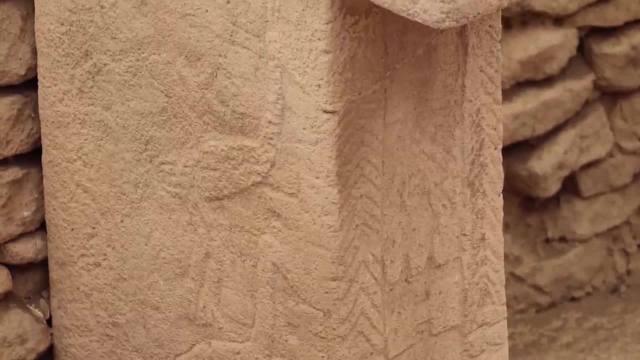 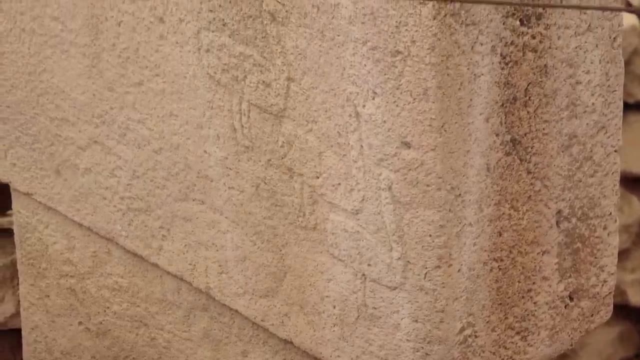 particularly striking dance of the dead. Cranes, a type of migratory waterbird, are seen too, creatures long associated with the realm of the dead. But other birds proliferate too- creatures long associated with the realm of the dead. Cranes, a type of migratory waterbird. 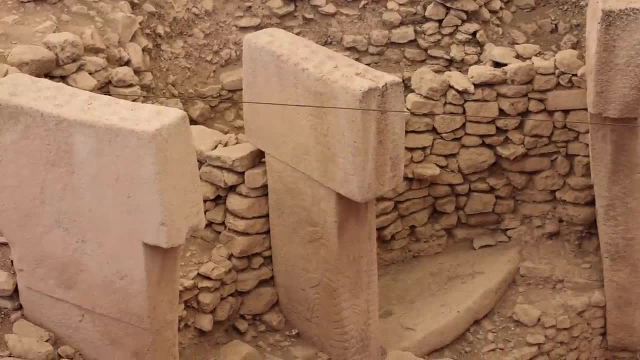 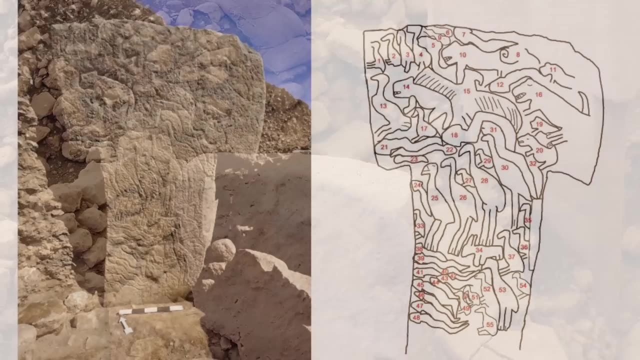 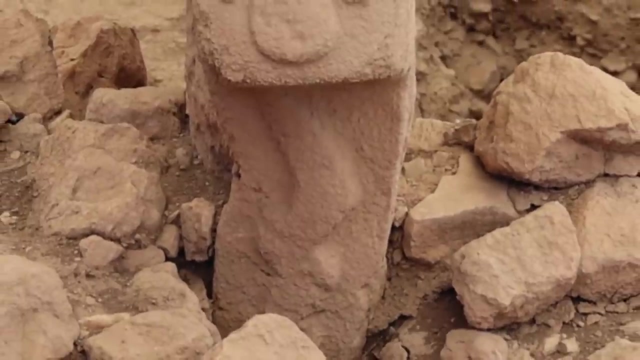 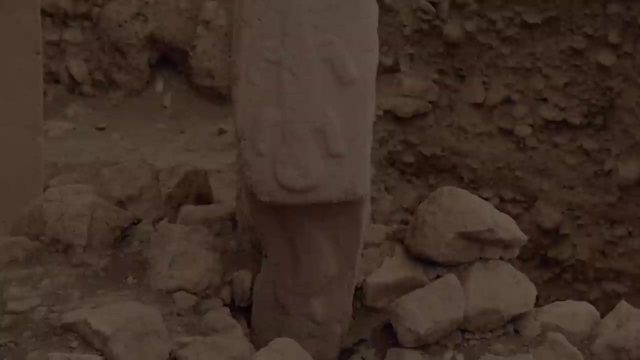 are seen too, creatures long associated with the realm of the dead. Among the more frequent motifs depicted at Gobekli Tepe is the snake In cultures all over the world, often associated with the underworld. In the late 1980s, one of the most striking finds made at Nvali Chori 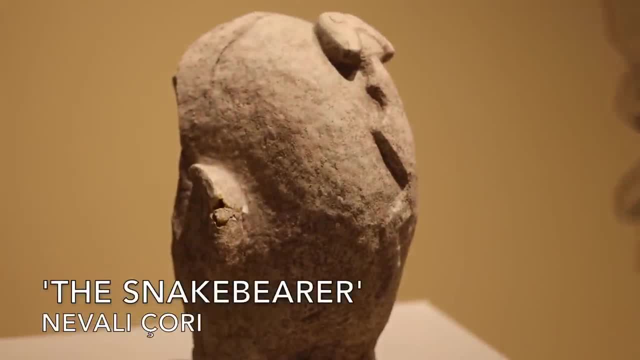 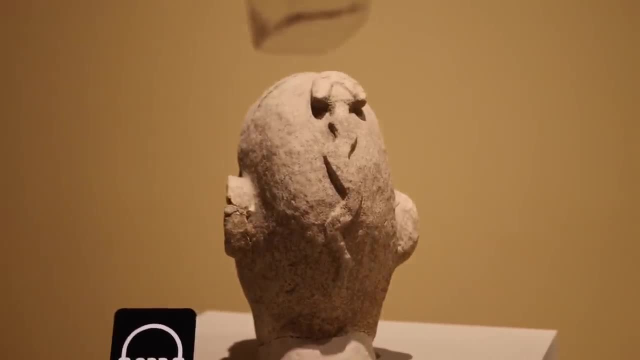 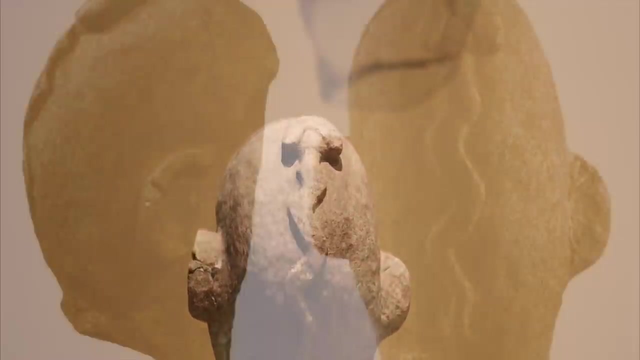 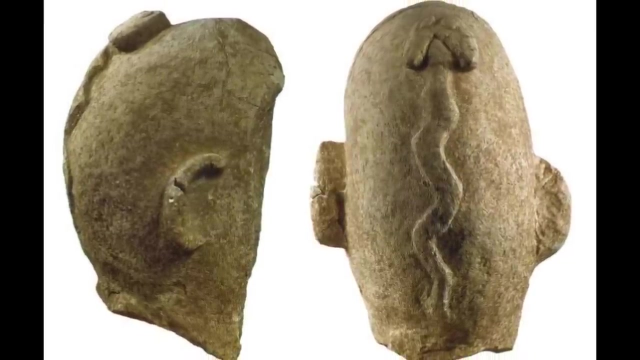 was the so-called Snake Bearer, A larger than life statue with a poisonous viper bursting forth from the back of his bald head, Though the face had unfortunately been broken off long ago. At nearby Kautik Tepe, many such serpentine images are found too. 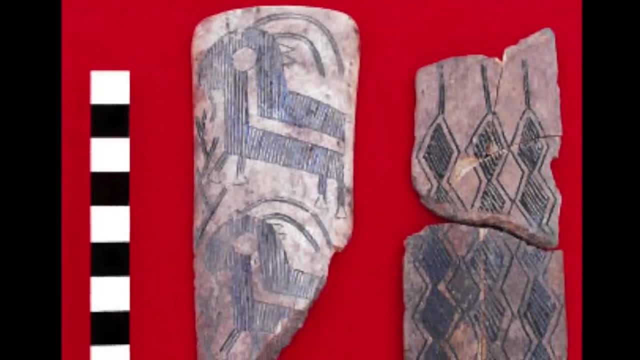 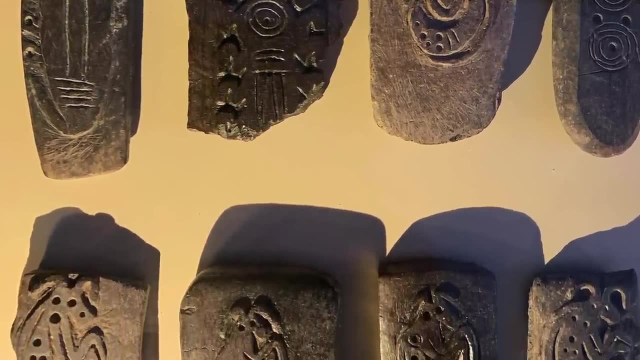 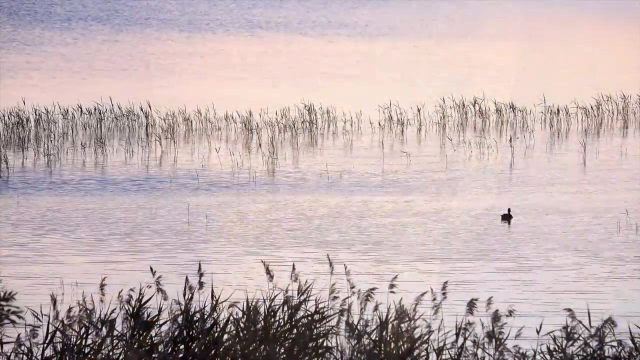 Scratched on stone vessels, as well as scorpions, another animal associated with the realm of the dead found also at Gobekli Tepe. Similarly, on the middle Euphrates, at the important site of Jurf el-Aqsa. 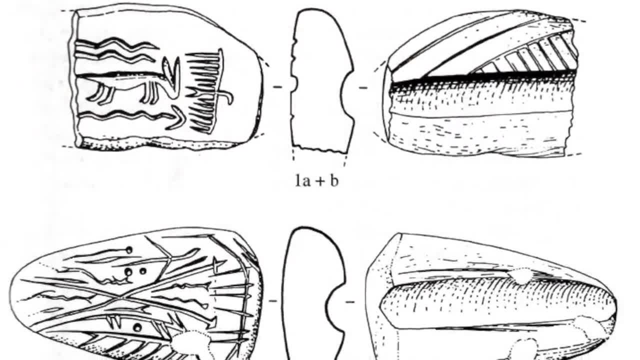 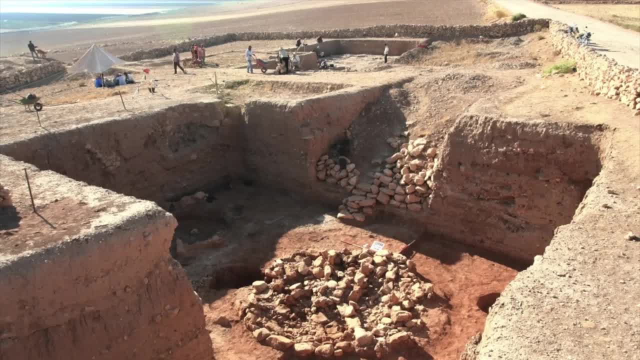 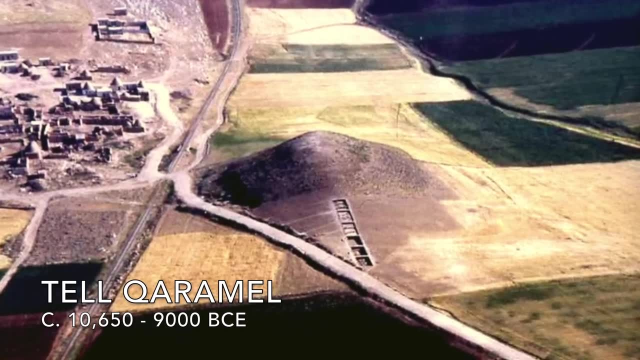 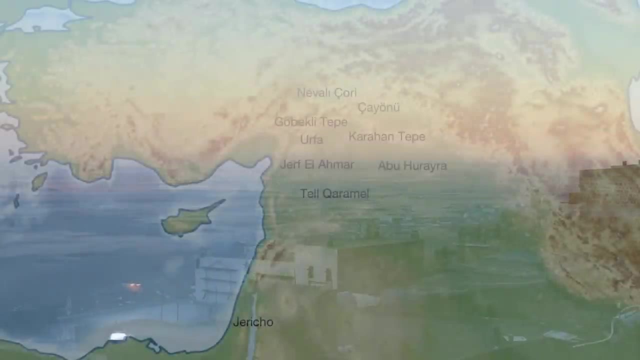 pictograms are also seen. They are also found even as far away as Tell Karamel, to the south, in Mesopotamia proper, where mighty prehistoric towers like those of Jericho are found too. The lands between Gobekli Tepe and the plains to the south seem to have been a borderland of 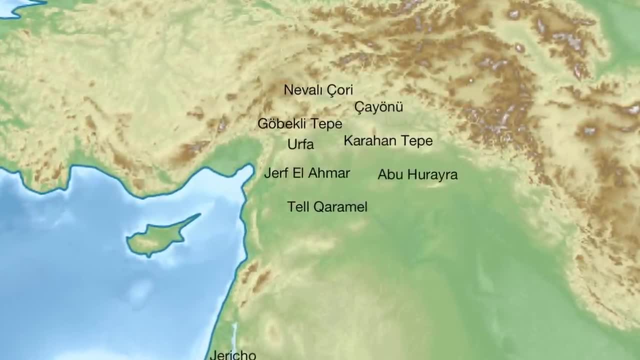 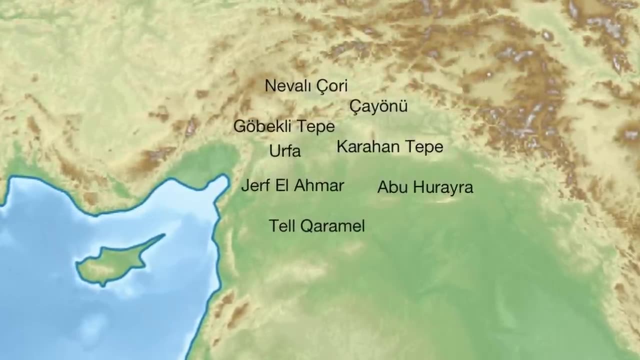 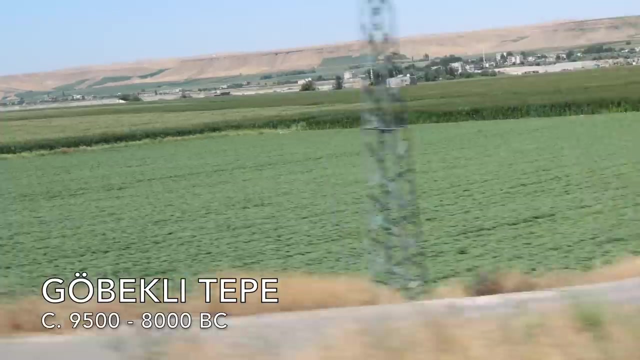 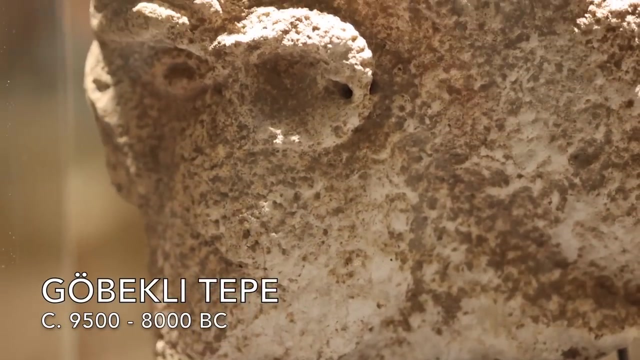 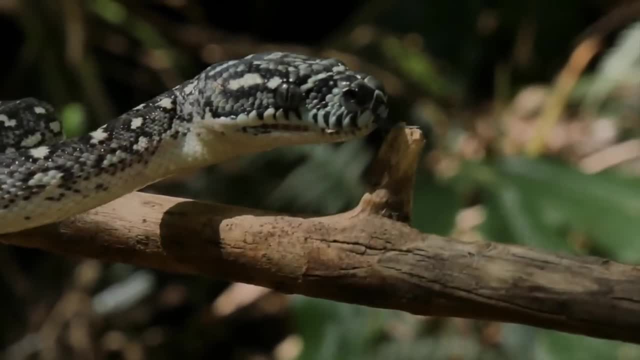 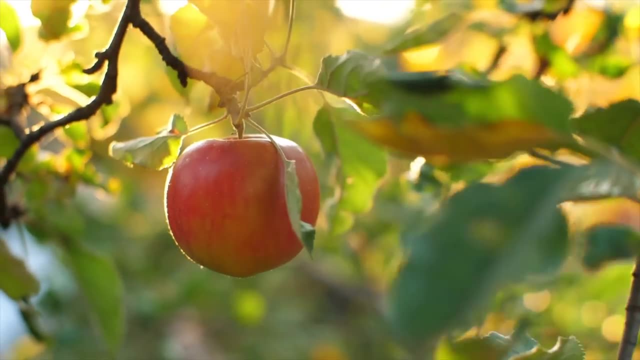 The story of Gobekli Tepe is a long story, but it is not the end of the story. However tempting it may be to speak of the serpent tempting Adam and Eve in the Garden of Eden, any such allusions to far later stories may well be entirely illusory. 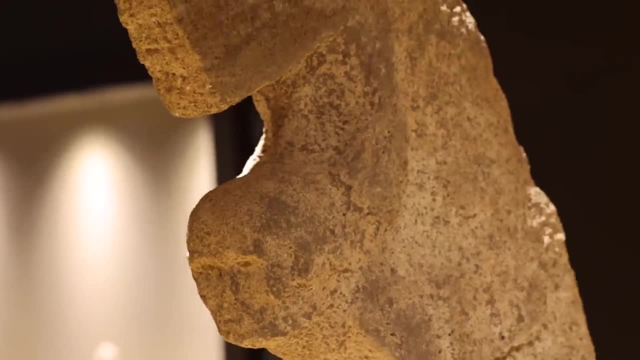 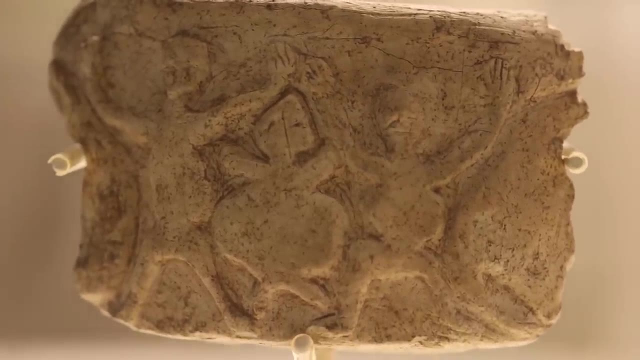 Quite simply, though, many would beg to differ with elaborate intellectual journeys of shamanic rituals and totemic creatures. quite simply though, many would beg to differ with elaborate intellectual journeys of shamanic rituals and totemic creatures. the images at Gobekli Tepe have lost their meaning. 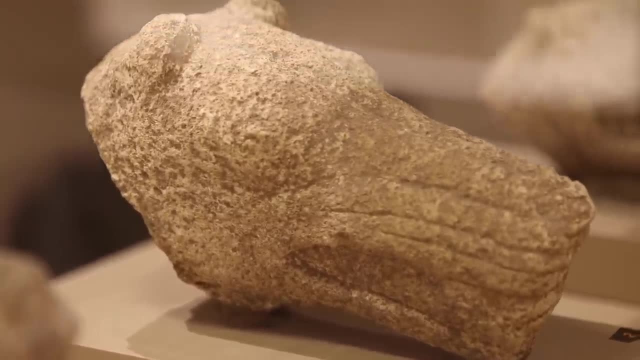 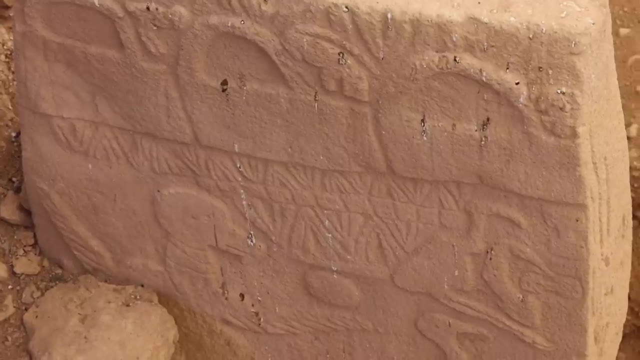 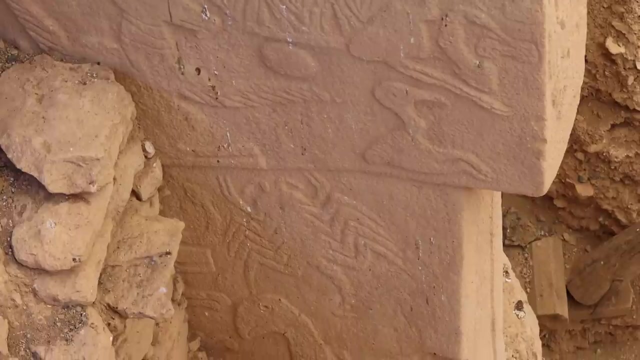 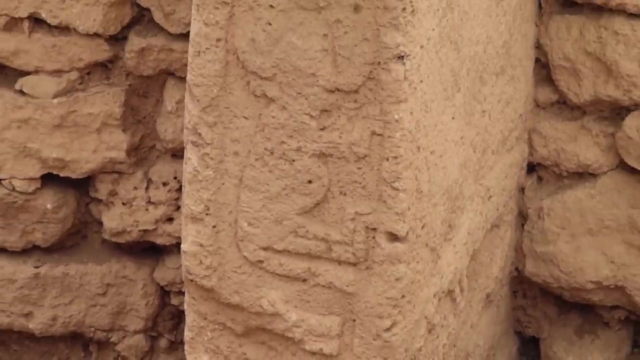 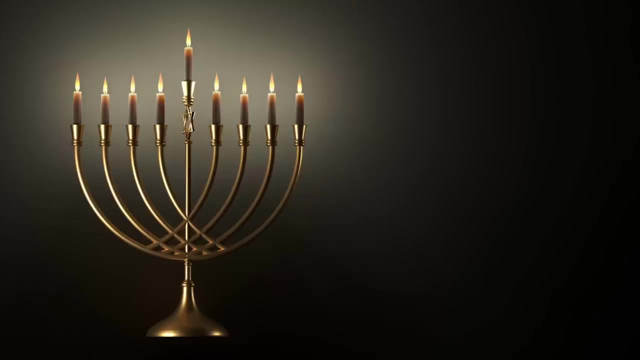 the images at Gobekli Tepe have lost their meaning. The intricate, often crowded gatherings of creatures, be they guardians, culture heroes or symbolic representations to ensure hunting success, may well also be illustrated storytelling aids for fables once as famous as those we all know today, long before Adam and Eve. 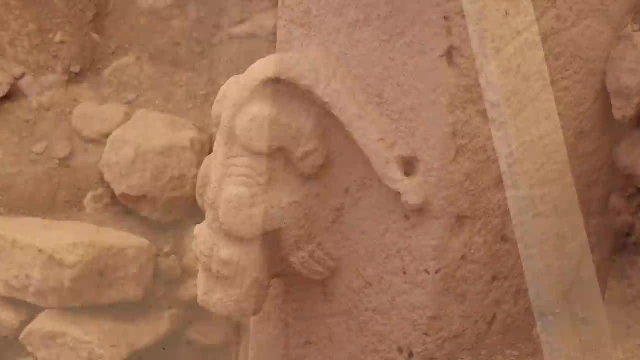 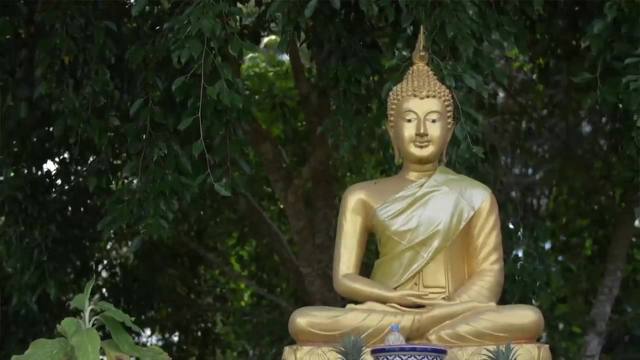 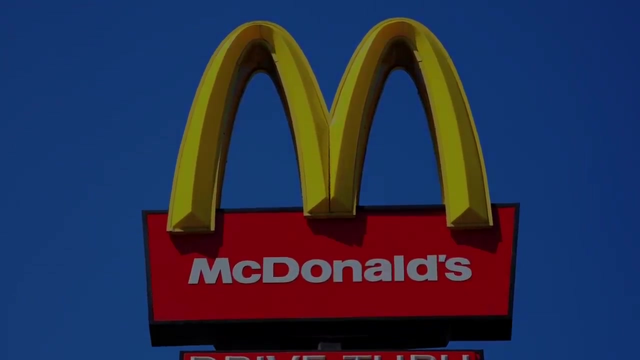 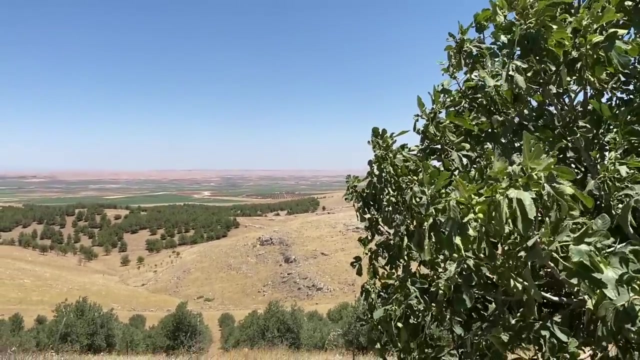 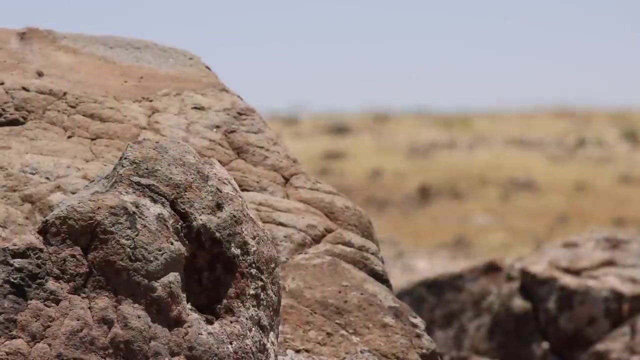 Who's to say that to the ancestors? they wouldn't have made total sense. No explanation needed. Like the Buddha, Jesus or McDonald's today. Today, visitors to the site still tie strips of cloth to a mulberry wishing tree, Perhaps a remainder of a custom from long ago when visitors arrived to pay their respects. 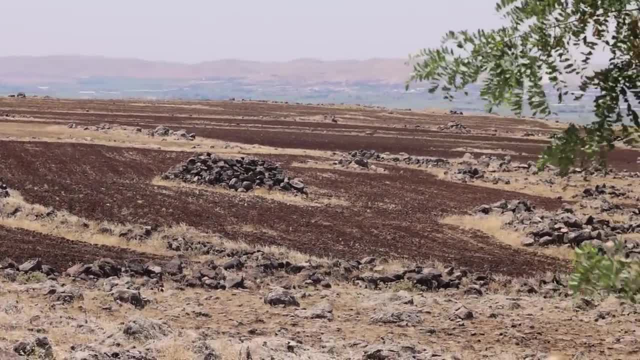 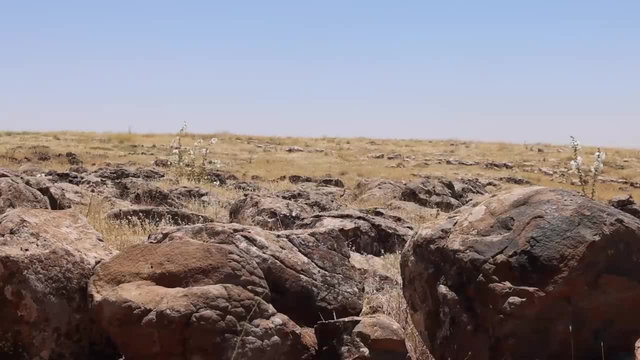 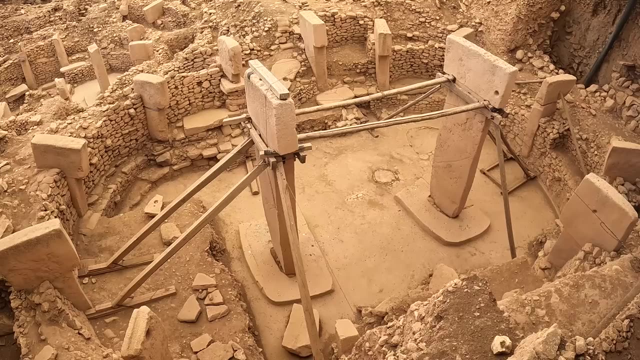 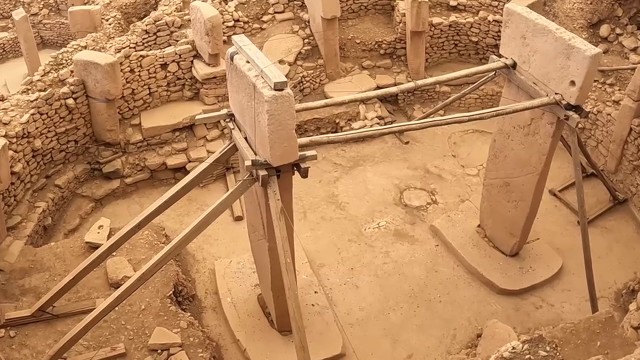 and beseech the divine. Though we can't say for certain what the purpose of the stone carvings was, they remain powerful representations of a clearly elaborate mythology. The most astonishing example, in fact, of a spectacularly profound creative explosion that took place here at the headwaters of the Balearic Islands. 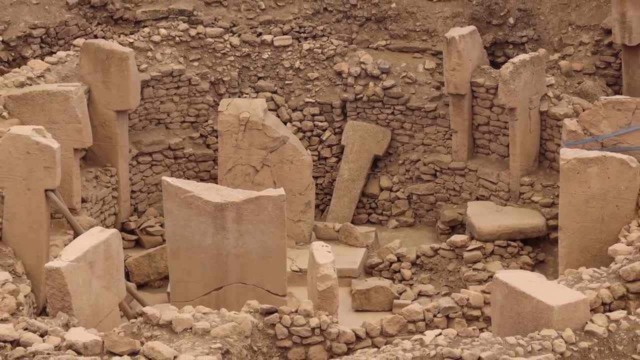 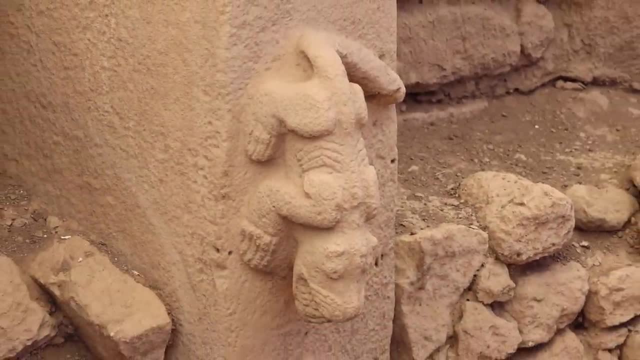 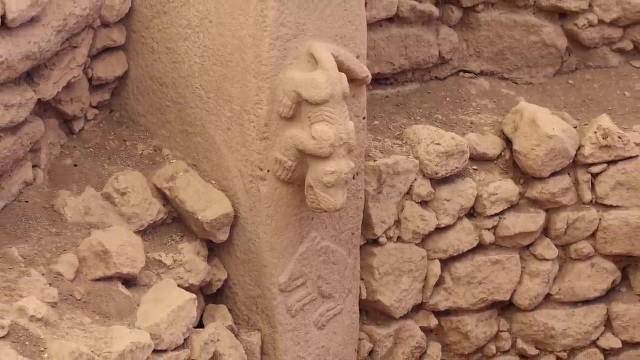 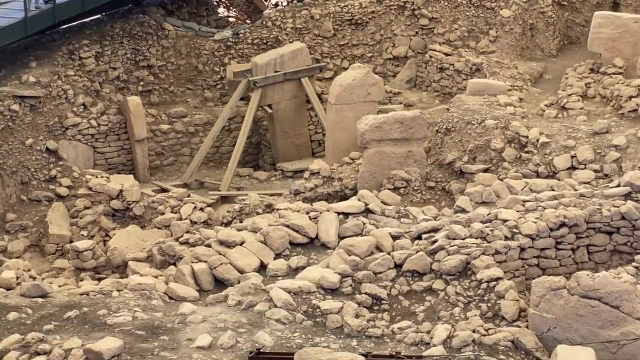 The most astonishing example, in fact, of a spectacularly profound creative explosion that took place here at the headwaters of the Balearic Islands. 1. throttle, Fallic Valley Some twelve thousand years ago. Fallic Valley Some twelve thousand years ago. 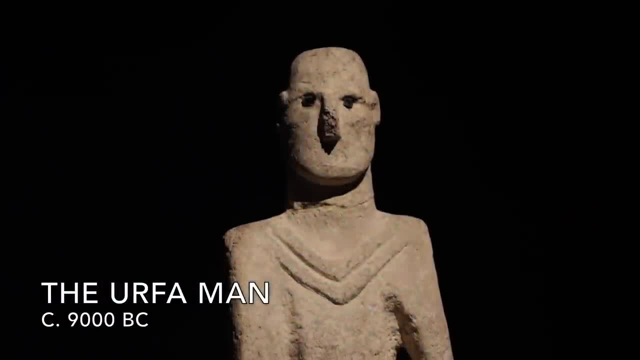 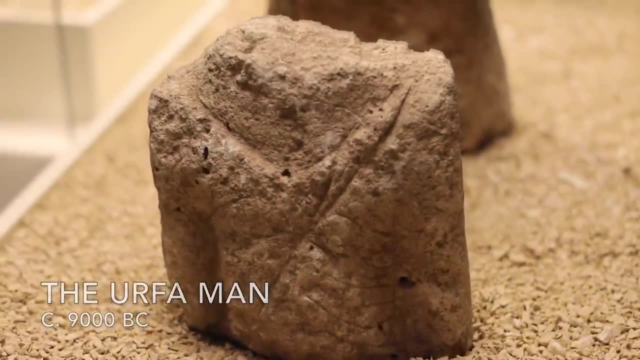 For Schmitt, one sculptured high-relief carving in particular totally outclassed the rest. The masterpiece of a Stone Age, Michelangelo, Celebrius P dynasty, Overland ninguna. there is free-standing sculpture too, Though much remains in a very poor state of preservation. 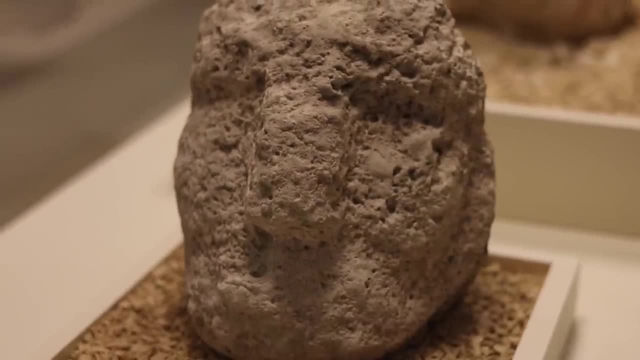 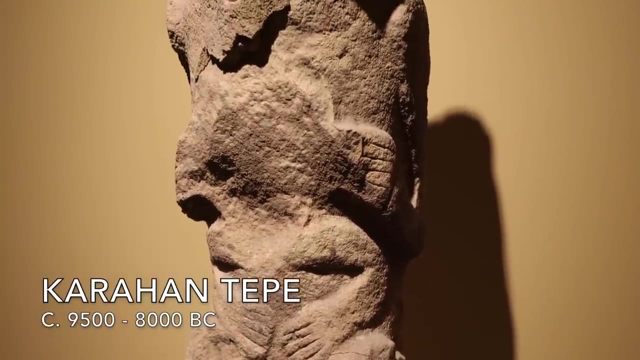 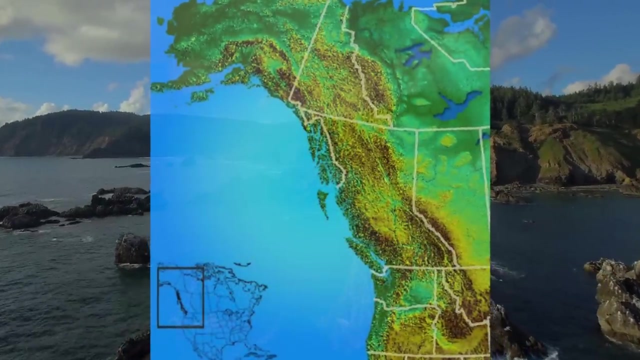 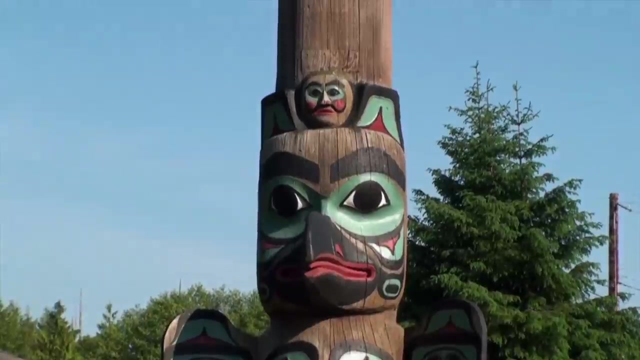 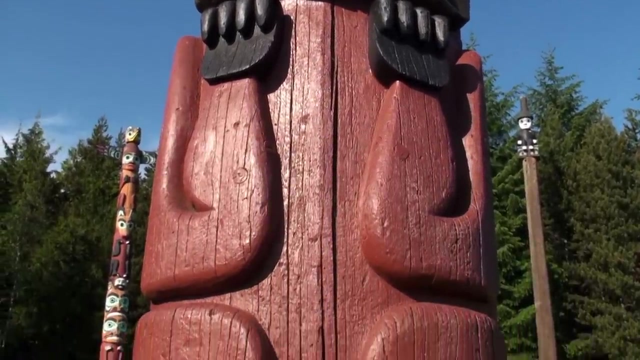 One colossal stone head may well have originally been part of a totem pole-like composite found also at Navalichori and Karahan Tepe, But of course most famously in the Pacific Northwest of the United States. But out there on the remote Pacific edge, such totemic creations 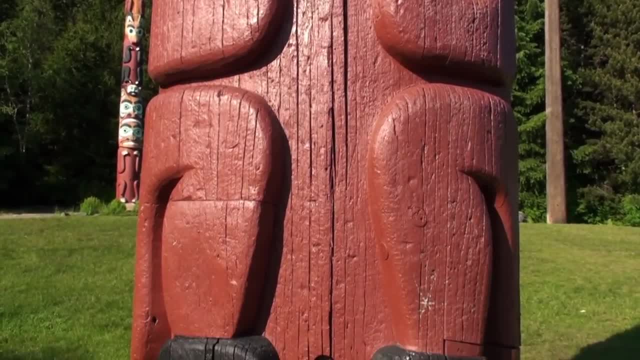 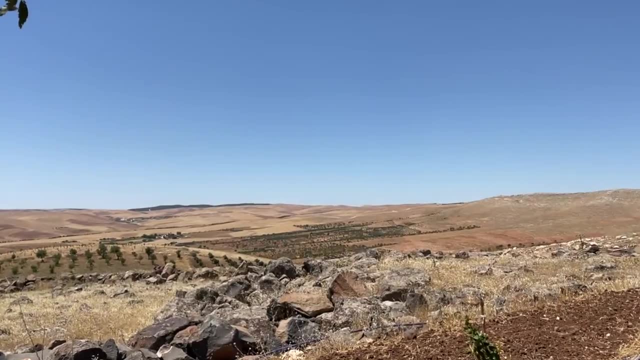 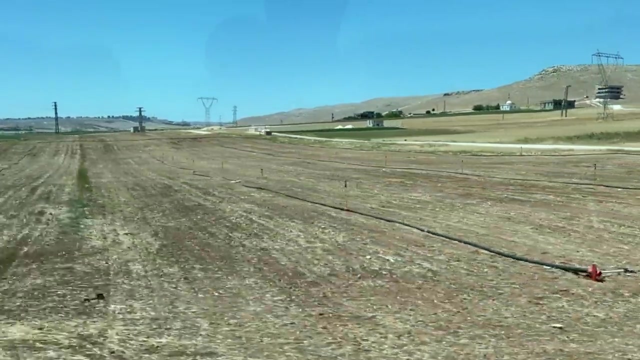 lined the thresholds of domestic homes as much as houses of the gods Since Klaus Schmidt's death in 2014,. another academic idea that has gained in prominence is the suggestion that the enclosures at Gobekli Tepe may not only have been roofed after all. 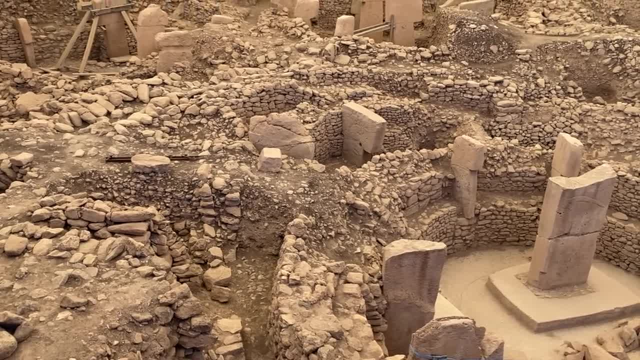 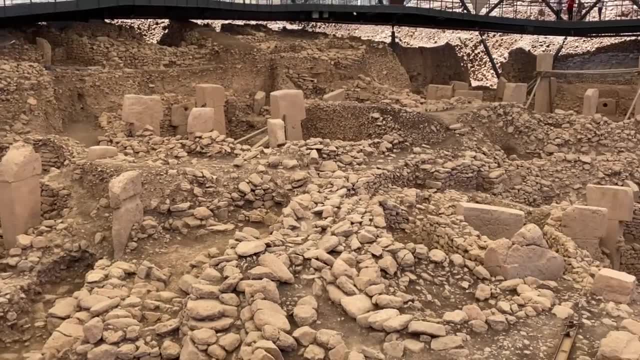 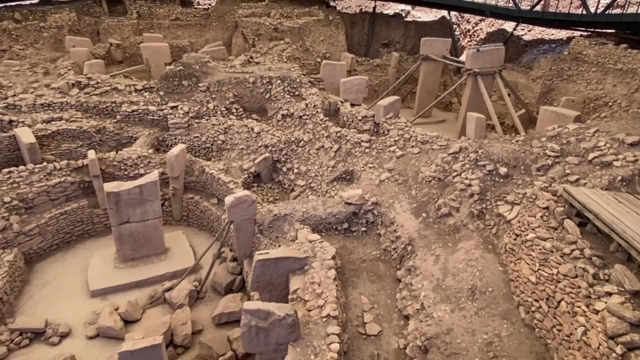 but could in fact have acted as sleeping quarters as much as temples. Whilst completely true that the structures at Gobekli Tepe look nothing like previously cemented houses from the pre-pottery Neolithic. it could be that they are simply a previously 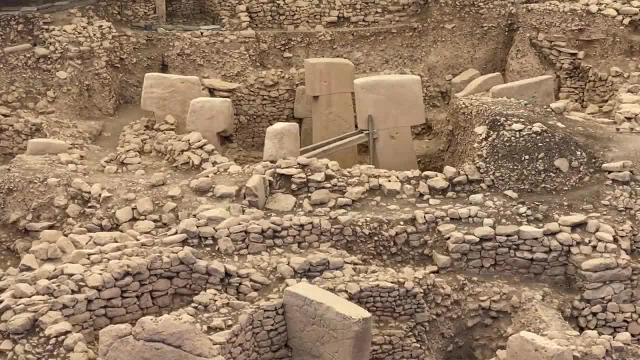 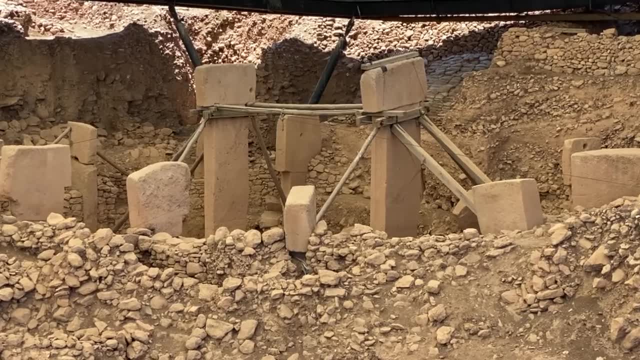 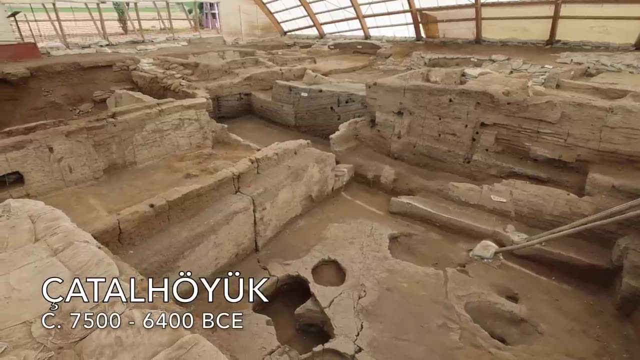 unknown example with no precedent discovered anywhere before. Pre-pottery Neolithic buildings were often built with the apparent intention for them to act as focal points for rituals, feasts, initiation ceremonies and the deaths and burials of members of the community. 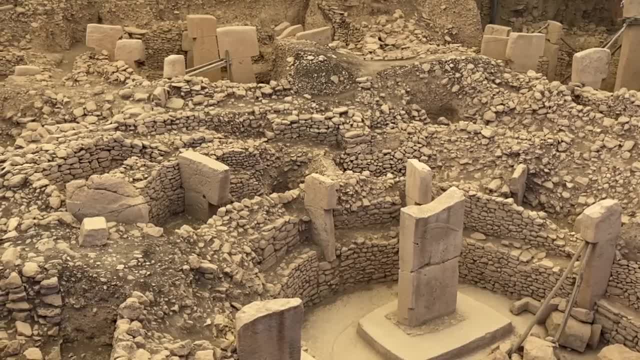 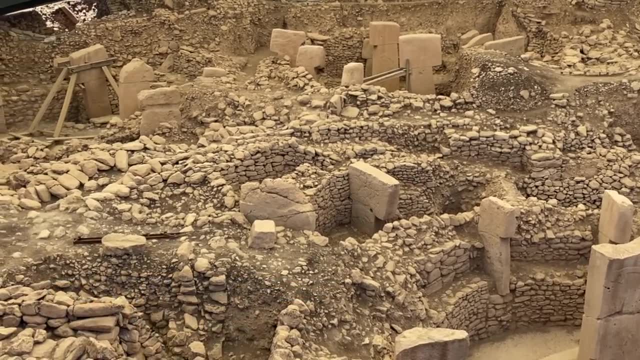 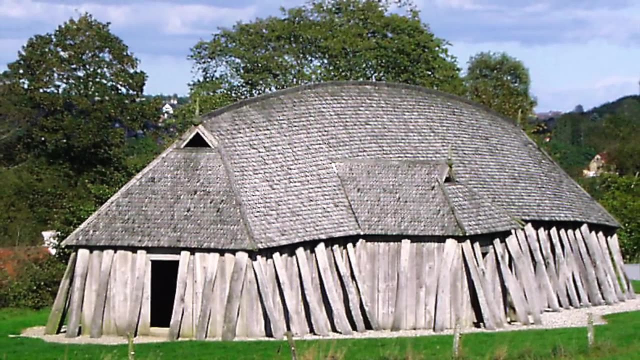 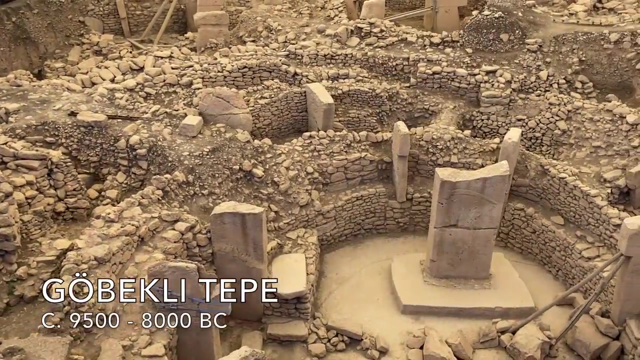 It's not impossible to suggest that they could have acted as houses in other times too, Or maybe at all times, Like Iroquois longhouses or the mead halls of an early medieval chief. But did the people of Gobekli Tepe? 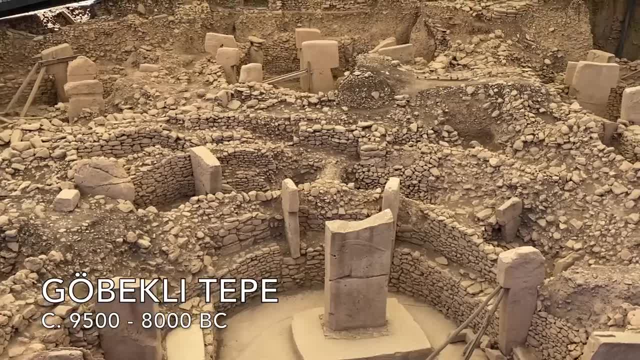 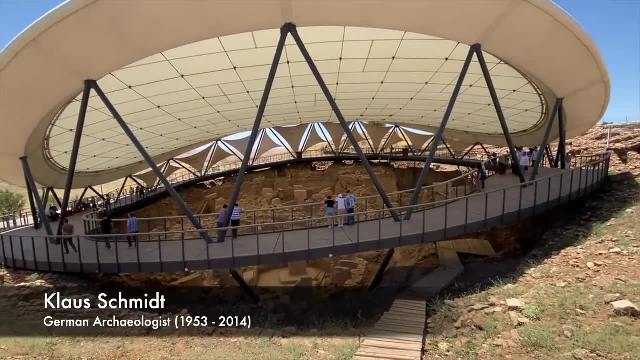 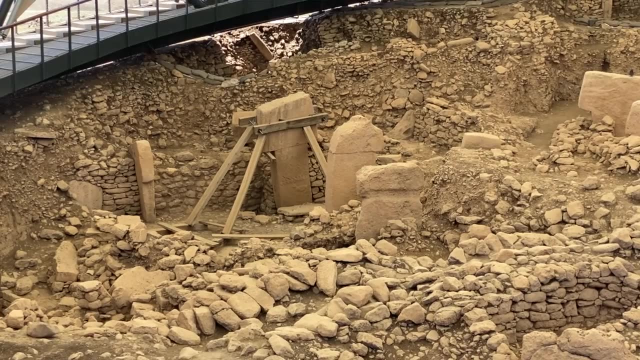 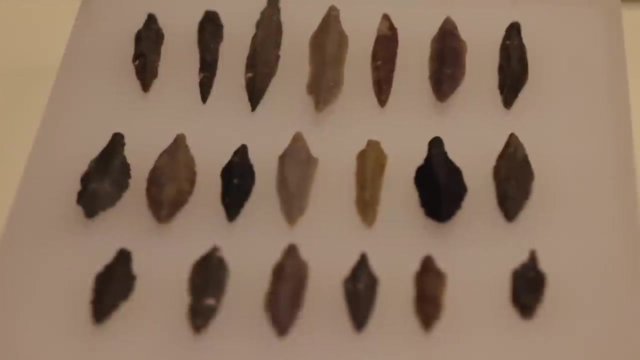 actually live there permanently. In recent years, Klaus Schmidt's assertions of no domestic activity at all being carried out at the site have been challenged. After all, there are significant amounts of tools related to domestic activity present at the site, as well as ostentatious animal remains. 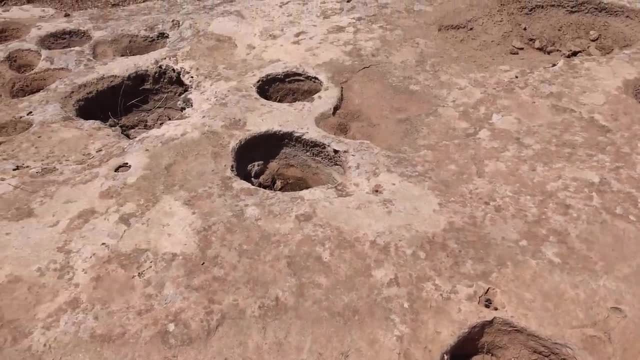 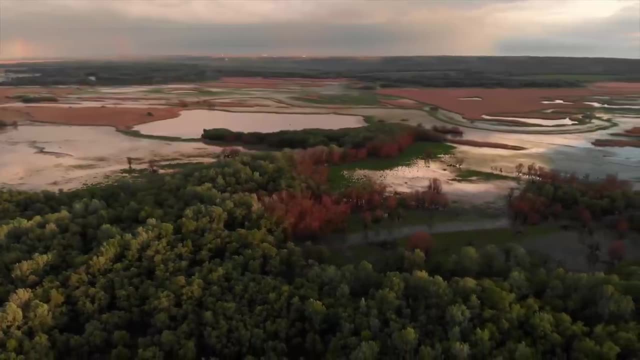 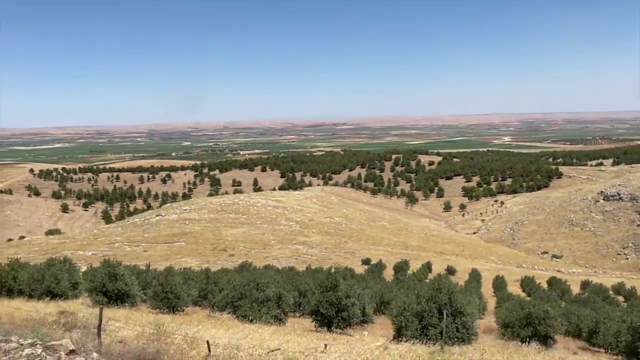 As for drinking water, Rock-cut cisterns and pools are found all over the hill, And in the more humid boreal period of some 12,000 years ago, the water table may well have been considerably higher, with the possibility of other water sources located nearby. 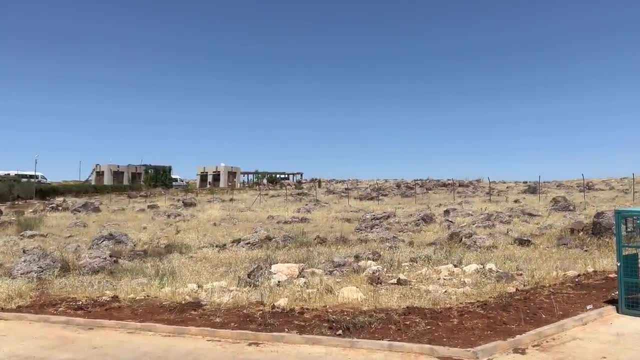 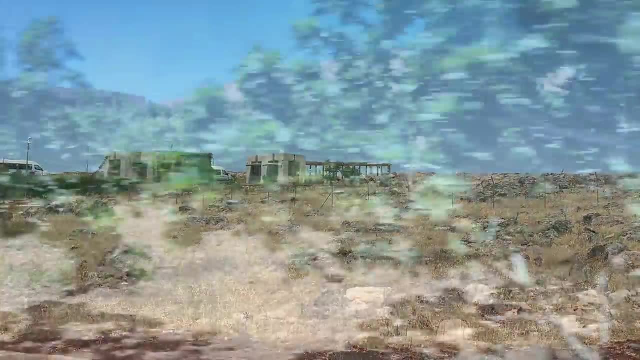 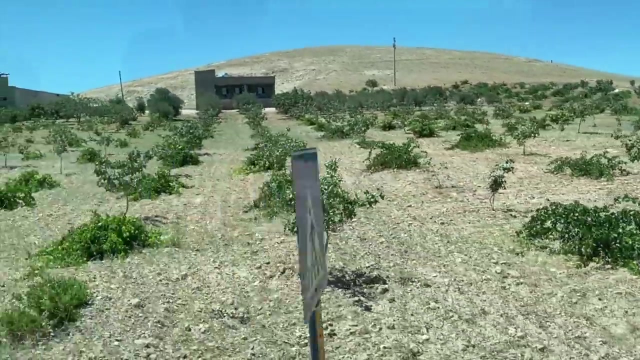 All in all, it's not completely outlandish to suggest that a small permanent staff could have lived on the site all year round, swelling to a much larger population at certain times of the year for festival activities, perhaps including the raising of monoliths. 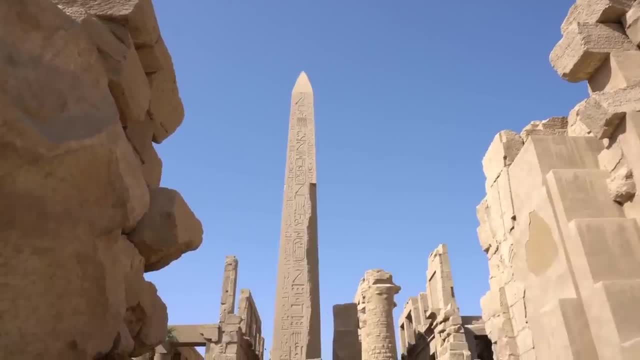 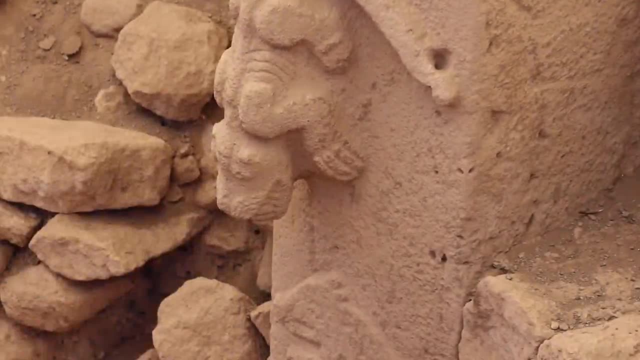 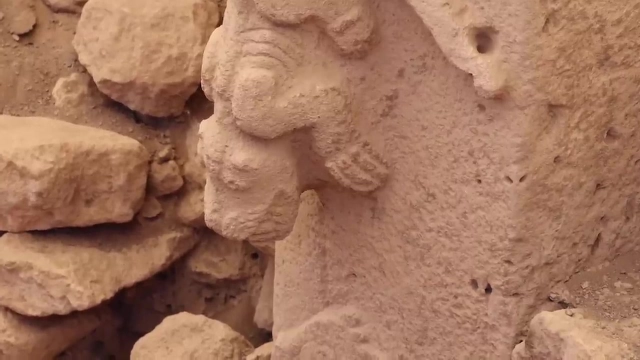 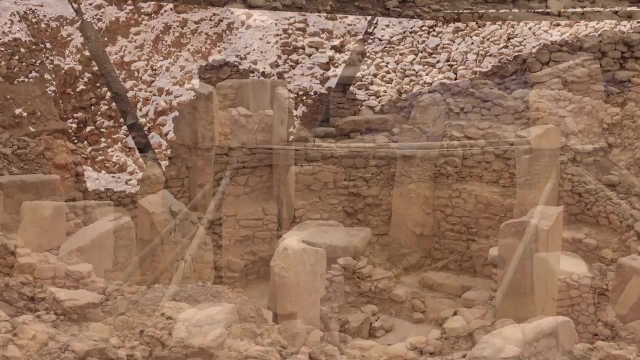 In ancient Egypt, for example, the very act itself being sacred. But what of those people who lived and worked at Gobekli Tepe? Human skeletal evidence remains extremely rare, Just a few hundred scraps of bones having been recovered, Two-thirds of which are skull fragments. 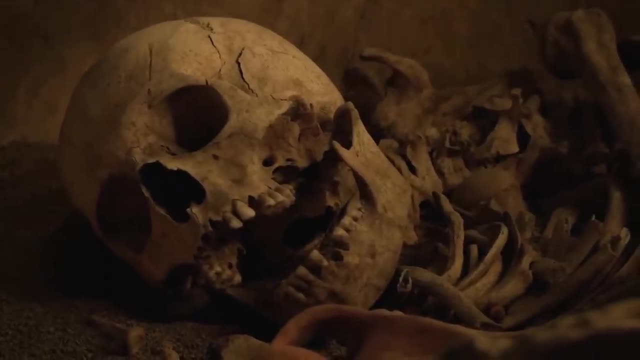 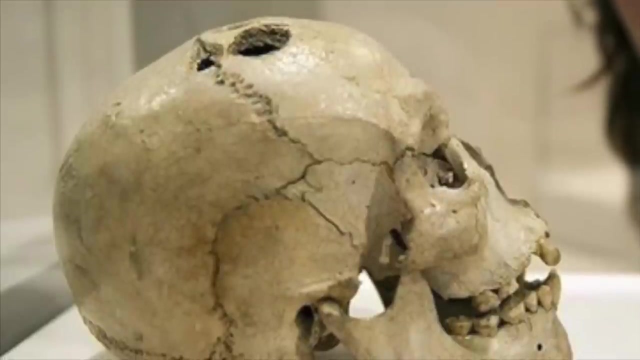 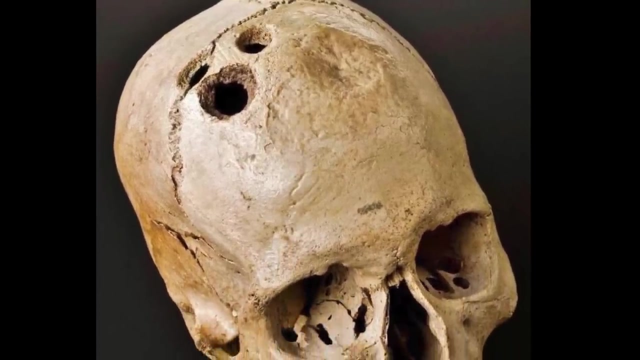 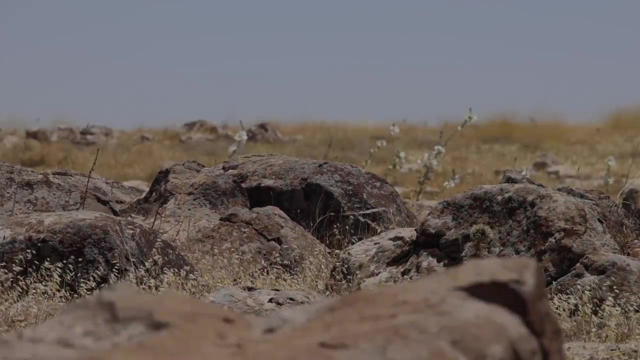 A few of them show evidence of decapitation and de-fleshing. Ominously, three have holes drilled into them, perhaps to be hung up or mounted on a pole. It's a tiny, potentially nightmarish window into those ancient days. 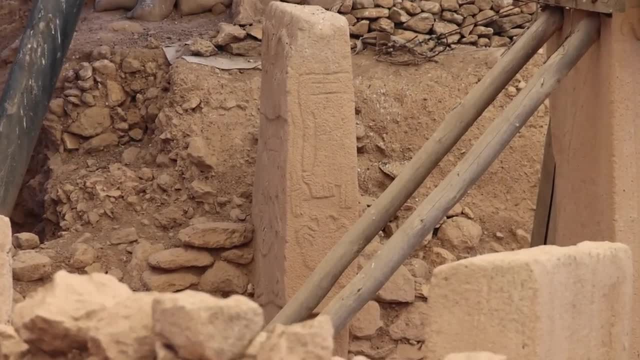 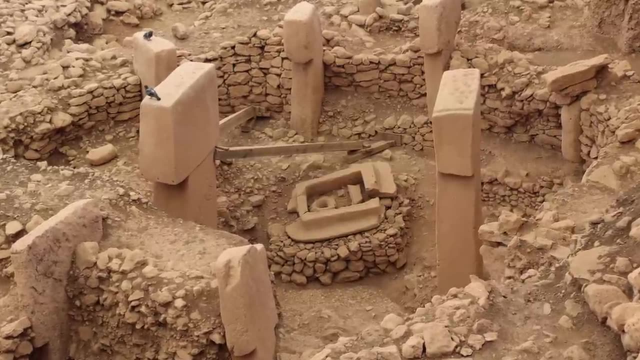 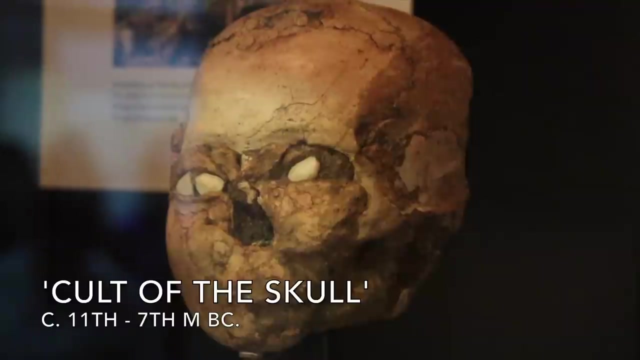 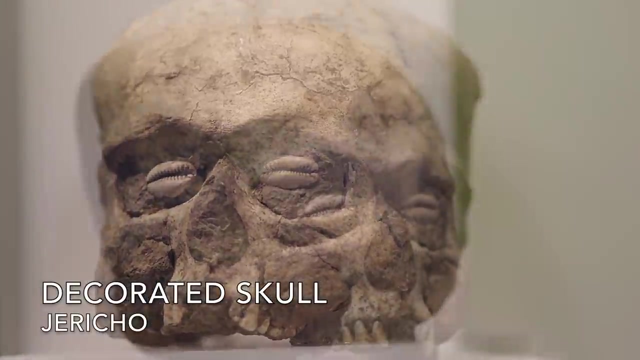 Though, equally, the finds may well represent the venerated remains of dearly loved ancestors, Perhaps relating to the so-called Cult of the Skull, which continued on in the Levant for thousands of years and even predates Gobekli Tepe at Natufian sites to the south. But possibly still maybe at the Natufian sites. we can use our own information to guess what happened. However, the only evidence that can help us make us think of what ought to be the time when this was discovered was the time when Gobekli Tepe was discovered by the Tamariki Hera. It has some quanto to say that it's worth noticing that these remains are of dearly loved ancestors, Perhaps relating to the so-called Cult of the Skull, which continued on in the Levant for thousands of years and even predates Gobekli Tepe at Natufian sites to the south. 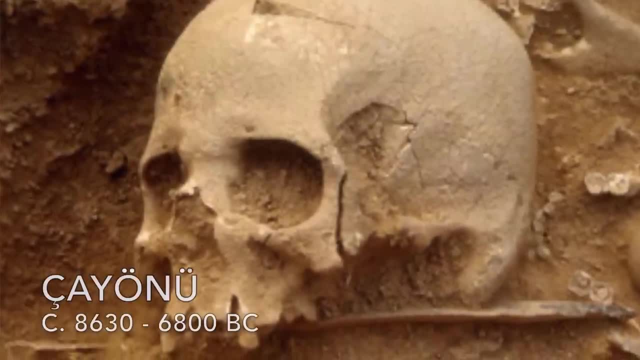 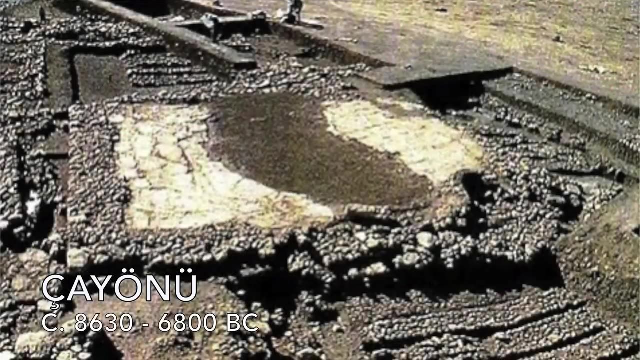 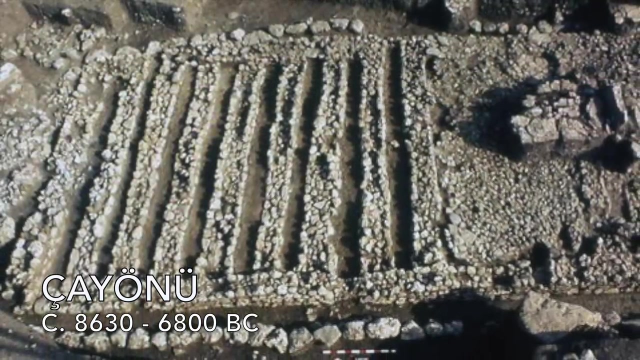 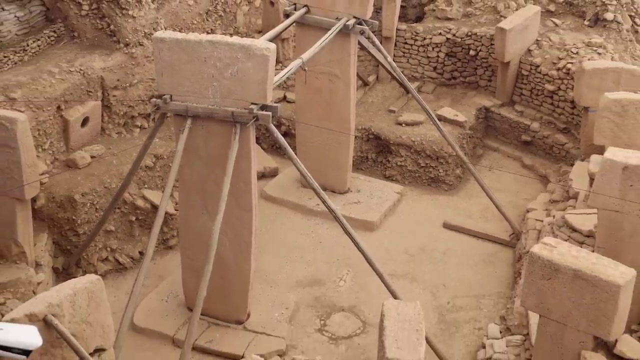 However, equally probable evidence at nearby Chiyonu cannot be overlooked. There, on a blood-encrusted altar, ritualistic human sacrifices may well have been carried out, perhaps shedding light on a darker side of the Gobekli Tepe phenomenon. 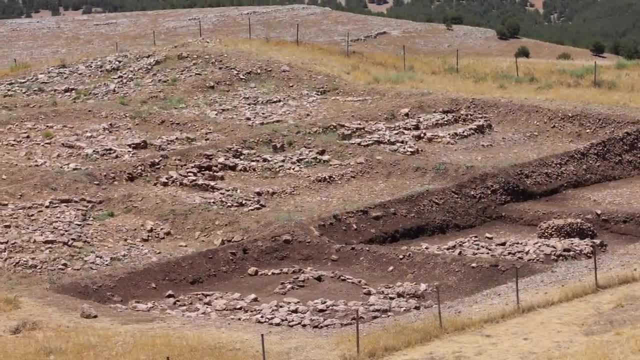 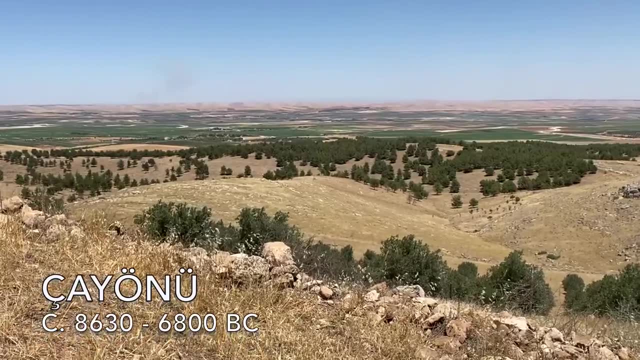 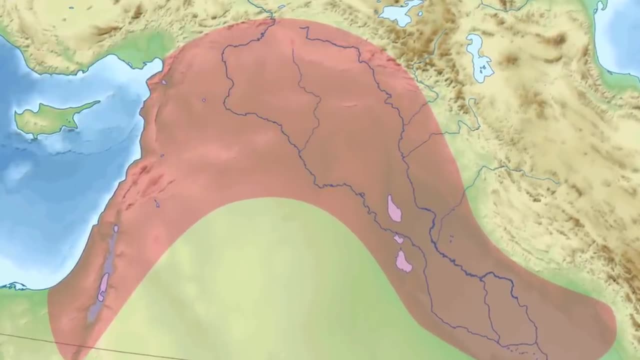 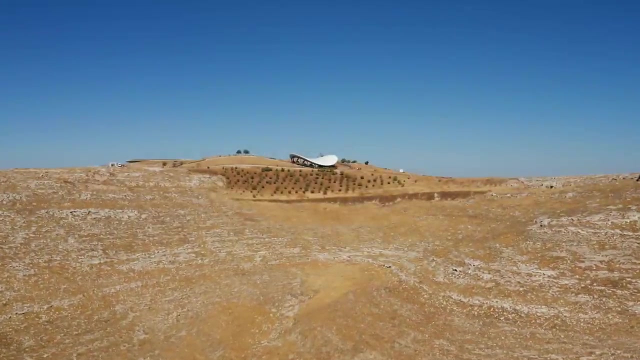 Although no direct, irrefutable evidence has yet come to light- and the Chiyonu finds are ever open to revised interpretation By around 8200 BC- whether a community of complex hunter-gatherers had indeed lived at Gobekli. 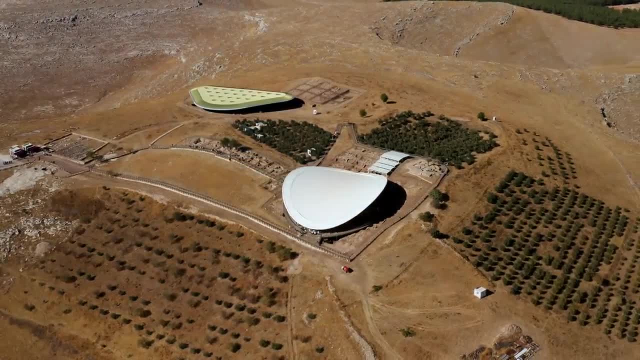 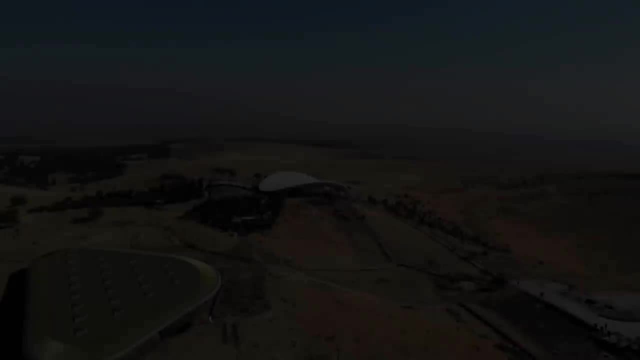 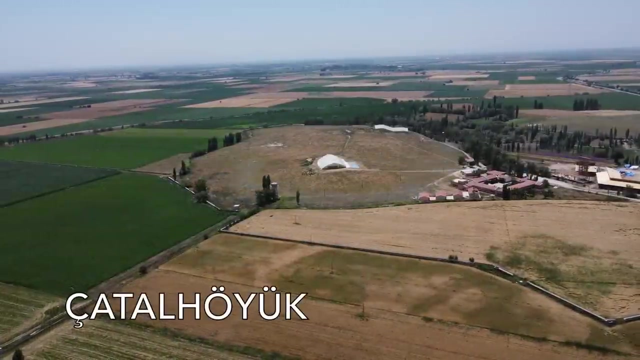 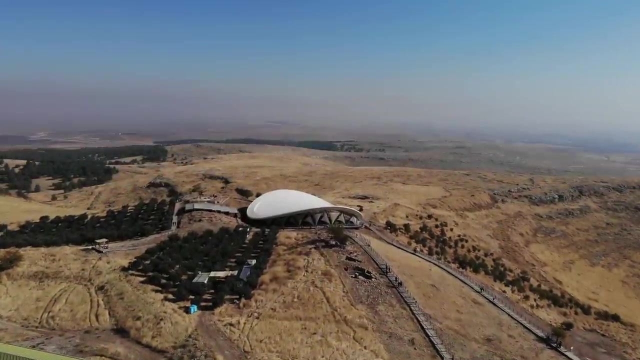 Tepe, permanently or not. life at the site came to an end In a scene reminiscent of the so-called house-closing rituals of later Neolithic sites like Çatalhöyük and admire cities alike. the very last stone circle made up of human-shaped pillars. much. 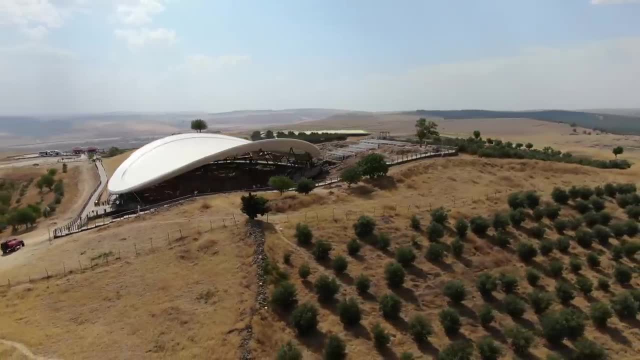 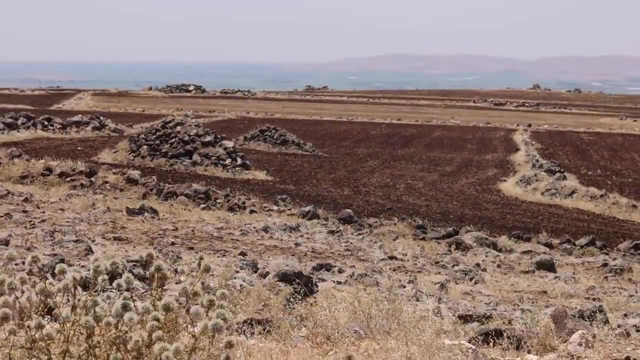 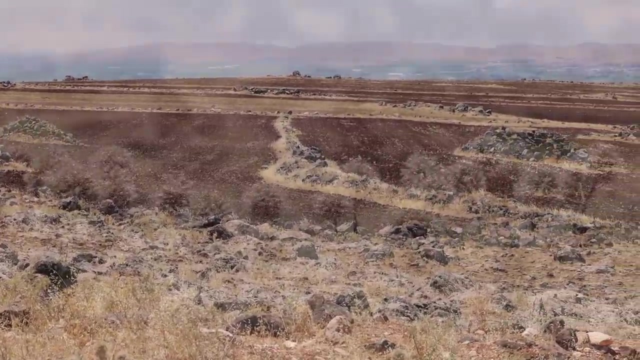 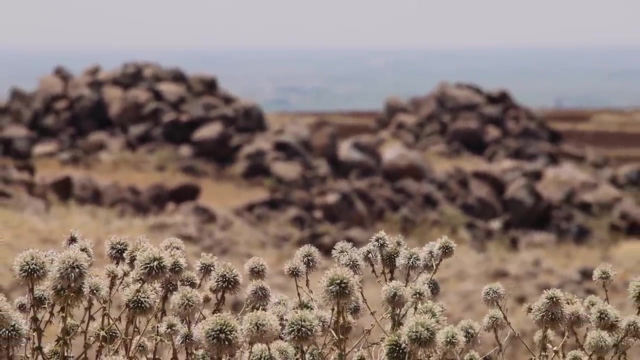 smaller than its predecessors was just like the previous circles had been Intentionally buried under up to three metres of earth. Though it's possible, people continued to come to the place in the years after very little could now be seen above ground. 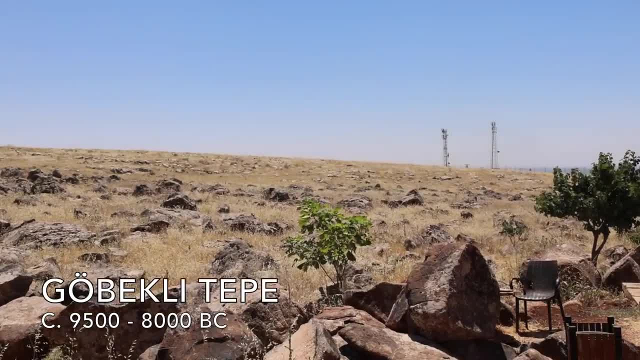 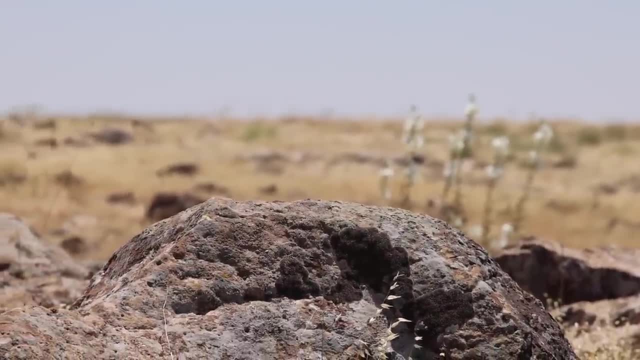 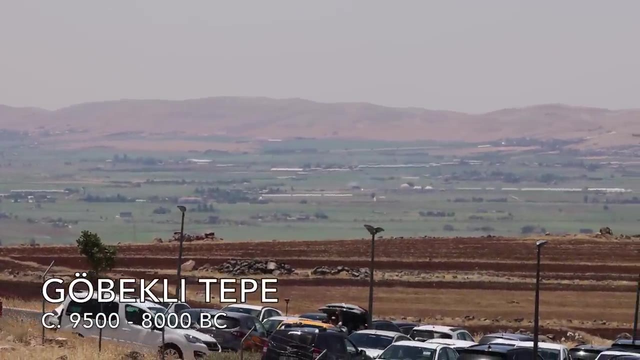 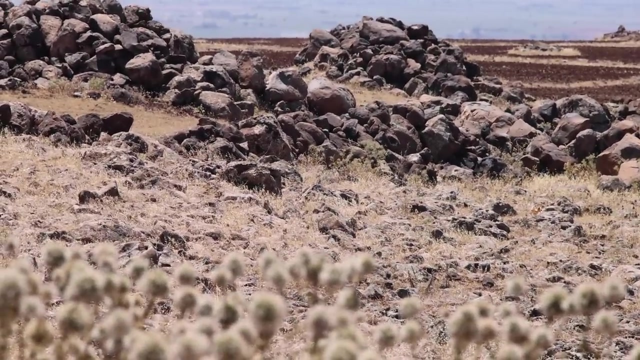 It's likely that, symbolically, the place was dead. Many conclusions have been drawn as to the end of Gobekli Tepe, ranging from violent conflict, drought, starvation and zoonotic disease to new conditions of sedentism making. 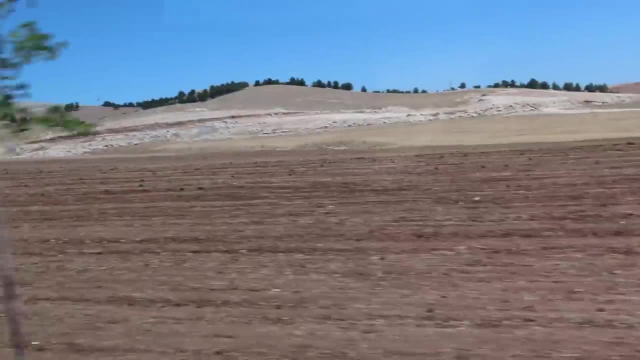 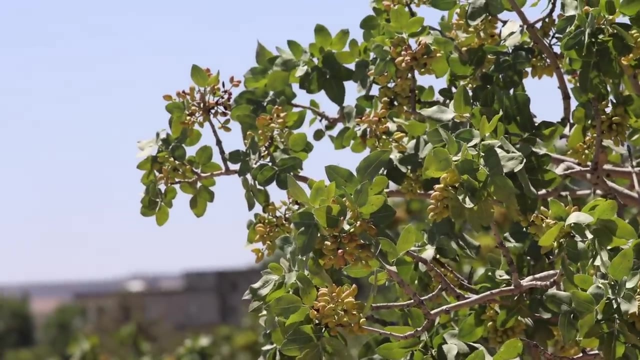 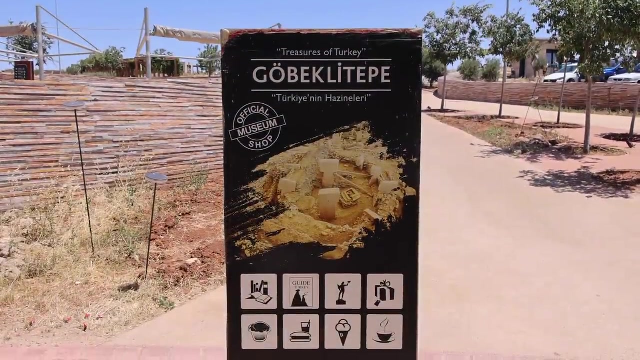 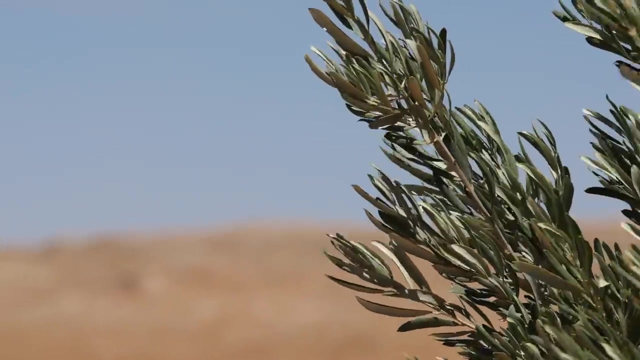 the old ritual places of the hunters irrelevant. The reality remains a total mystery, But in examining the context of the birth of the Neolithic and how Gobekli Tepe came into being in the first place, we can uncover yet more clues. 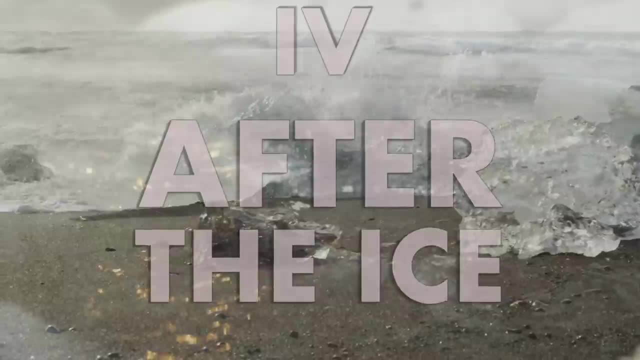 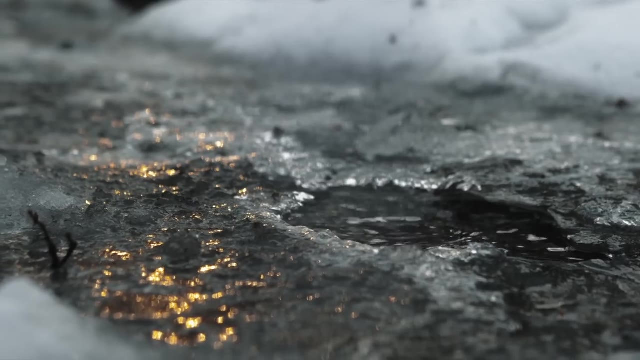 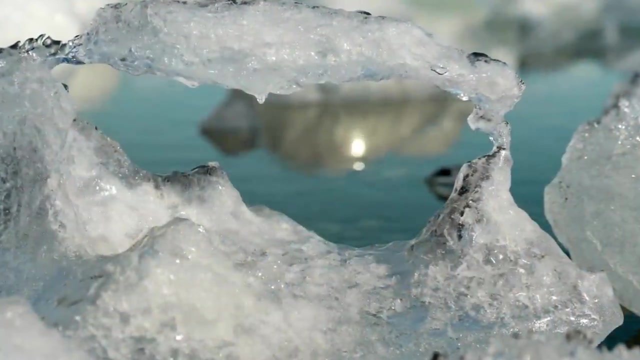 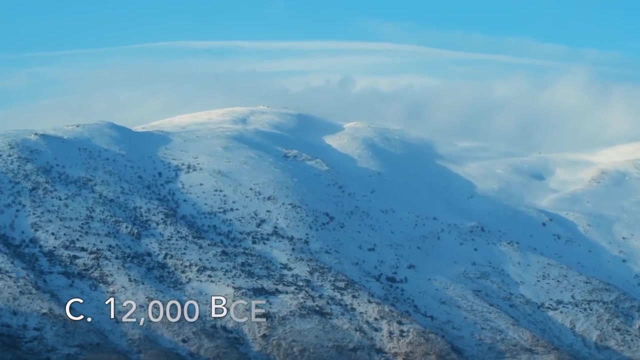 As the colossal ice sheets that had held Europe in thrall for tens of thousands of years finally began their long retreat back to the frigid Arctic wastes. by around 12,000 BC, the foothills of the southern Taurus Mountains were awash with green. 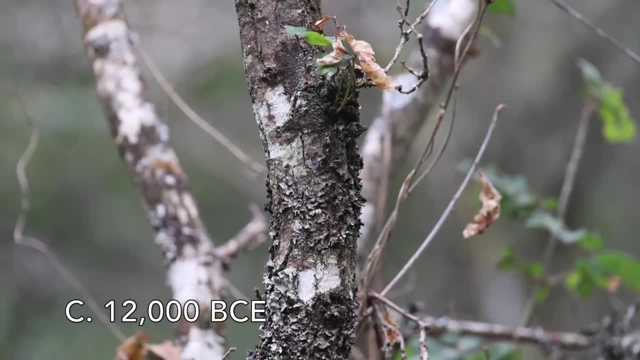 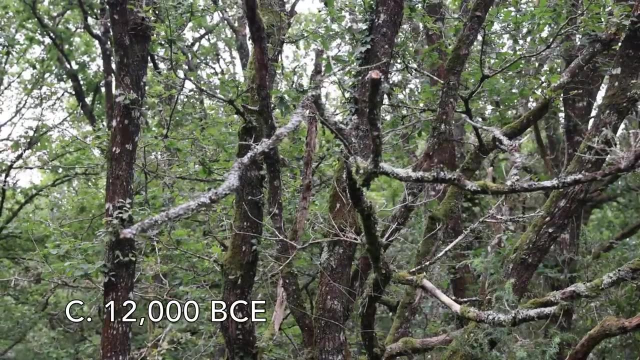 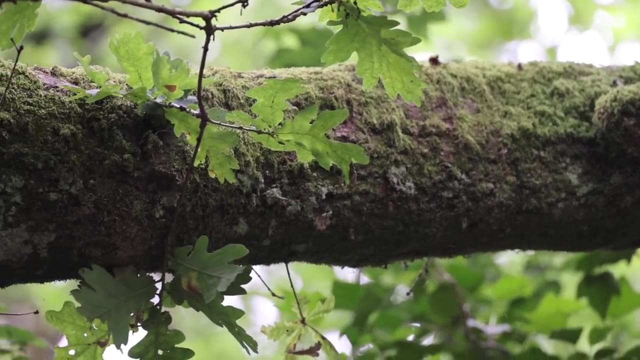 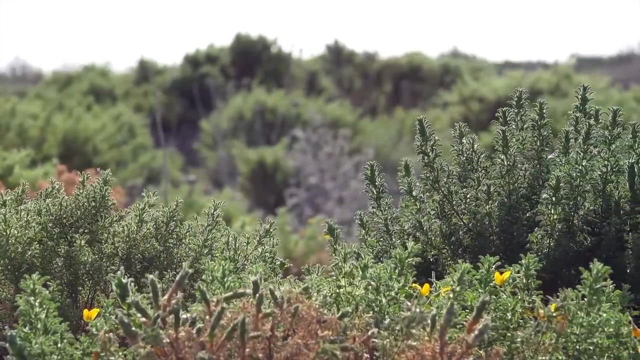 Lush river valleys, ran tracks past verdant prairies, Ever-expanding forests of pistachio and oak spreading along the open frontier to previously barren plateaus and patches of scrub-studded desert, And into this New Eden, And into this New Eden. 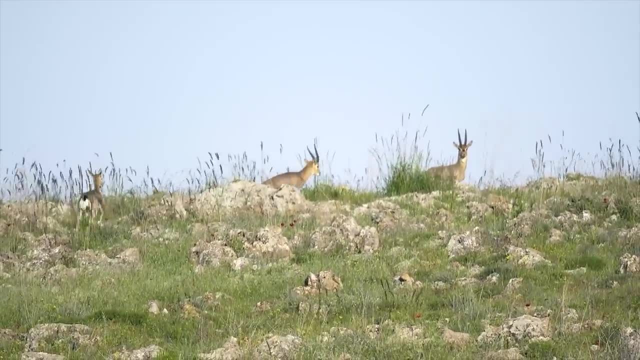 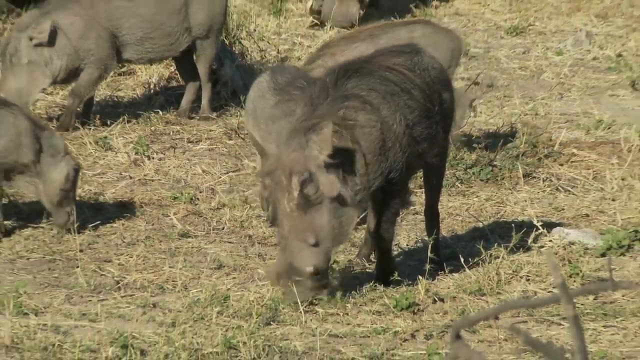 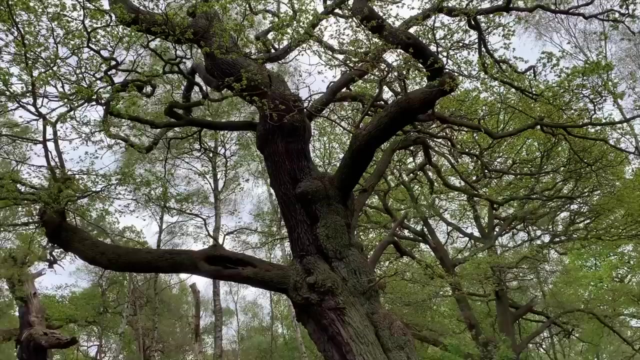 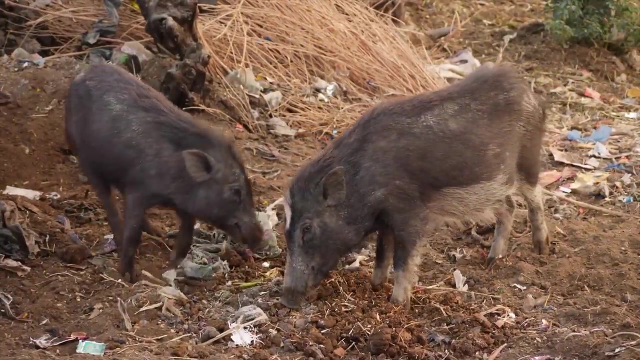 Came, vast herds of gazelle, along with wild boar making their homes in the woodland, All manner of goat, auroch and bird wandering the hills and riversides. It was a landscape teeming with life and, for the previously isolated communities of 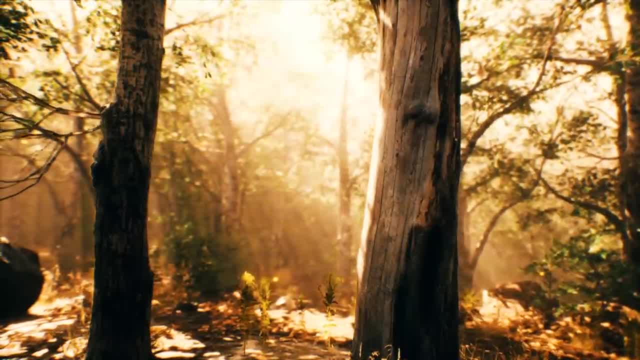 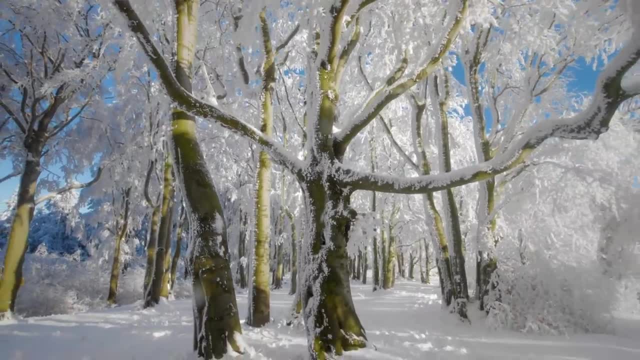 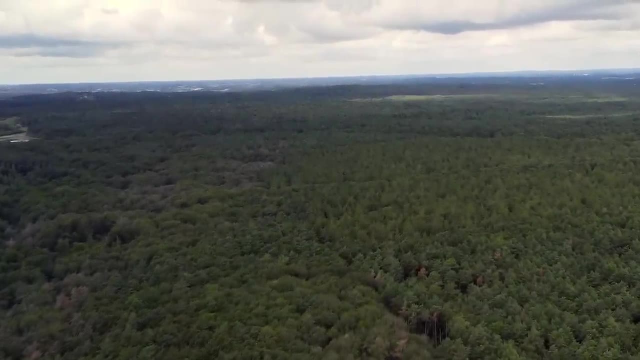 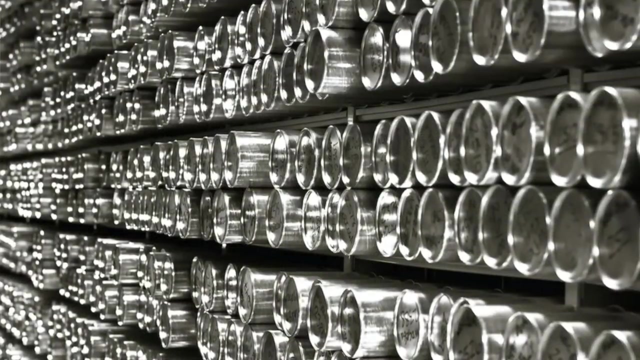 late Palaeolithic, humans often restricted to sheltered refuges in the wake of harsh climatic conditions. It must have seemed like paradise. Climate models built up from prehistoric ice cores over the last 80 years or so suggest a significant increase in climate change. 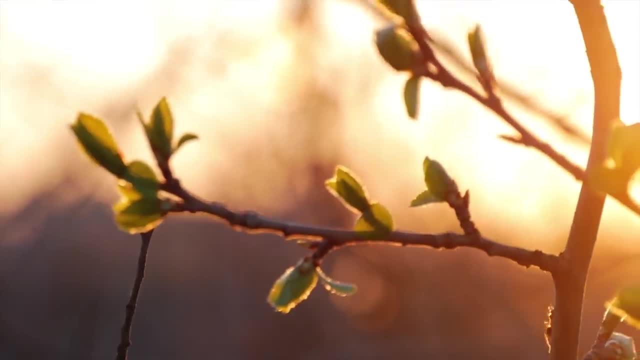 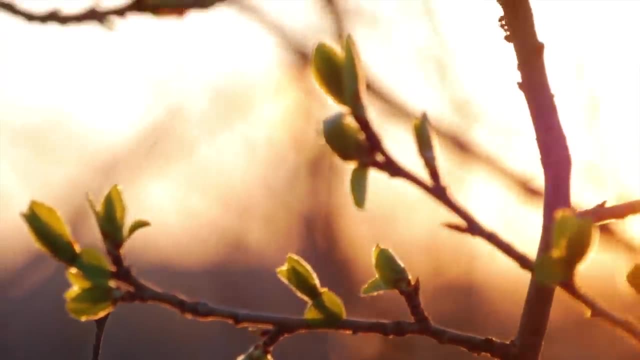 In the late 1800s and early 1900s, there was a rise in both rainfall and temperature following the last glacial maximum of around 13,000 BC, thus paving the way for the emergence of a new way of life. 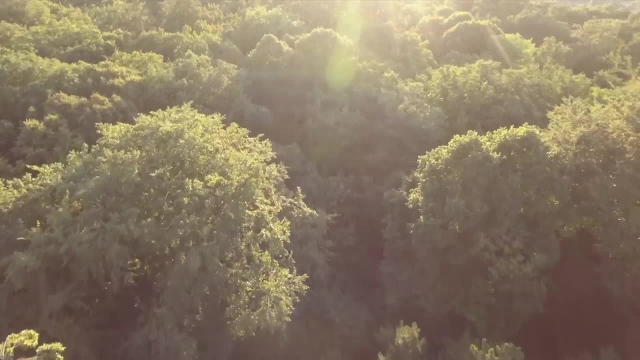 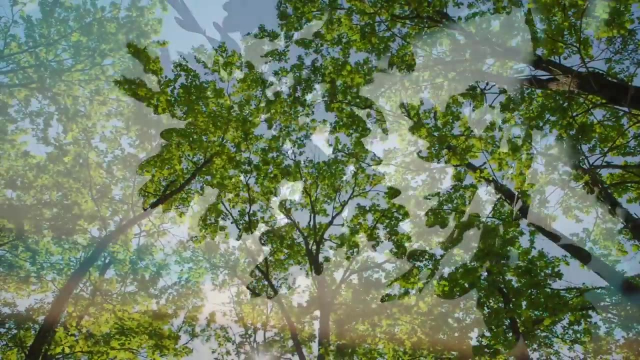 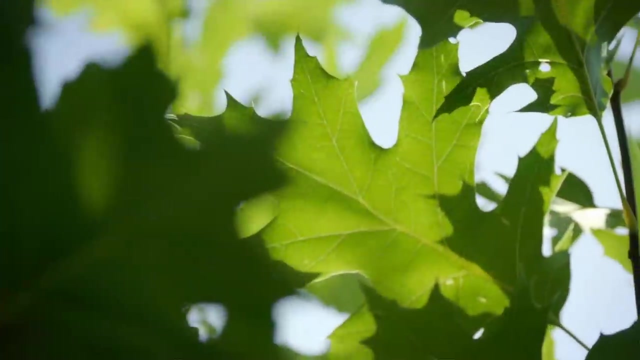 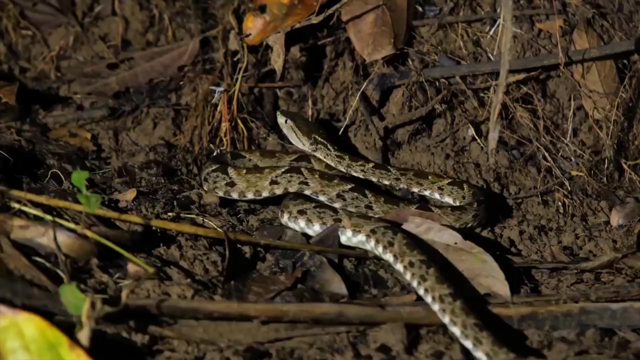 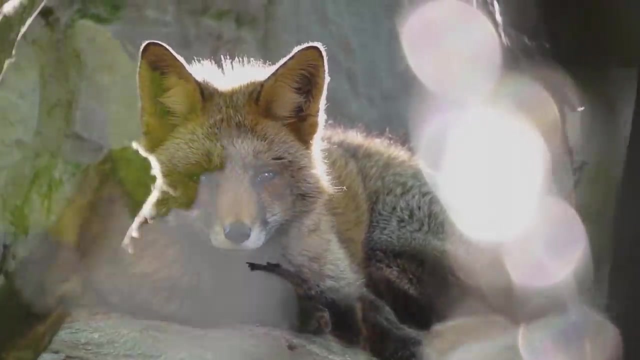 Though still wide-roaming, people were beginning to settle down into territories They knew extremely well, More so than ever before, Landscapes of dangerous carnivores and poisonous reptiles Of swift-running game waterfowl and furry scavengers. 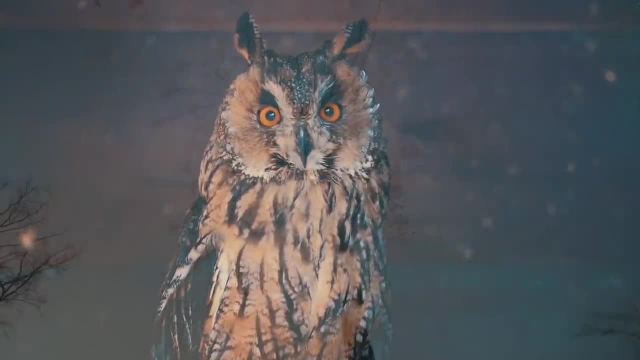 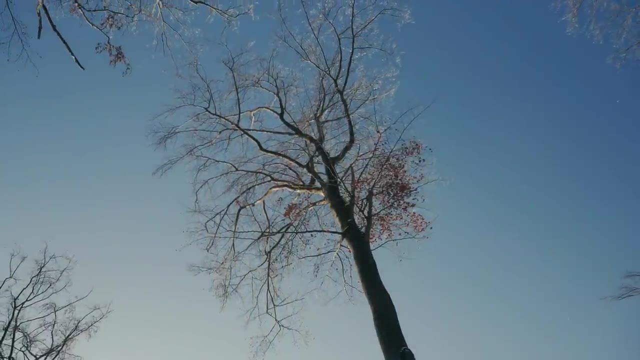 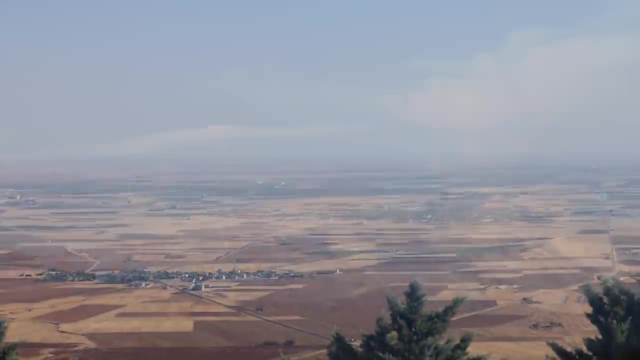 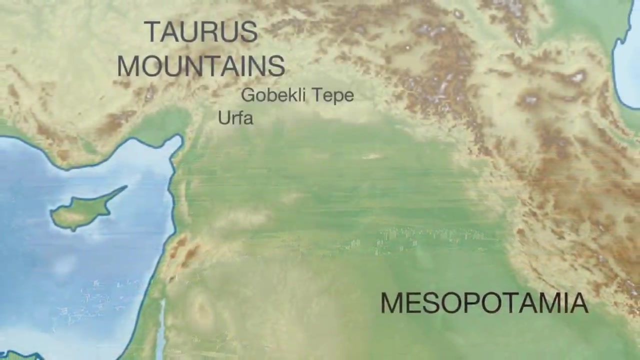 This was the world inhabited by the builders of Gobekli Tepe. To the west and north, The snow-capped peaks of the Taurus Range loom. To the south, The Haran Plain stretches all the way to what is now Syria and Iraq beyond. 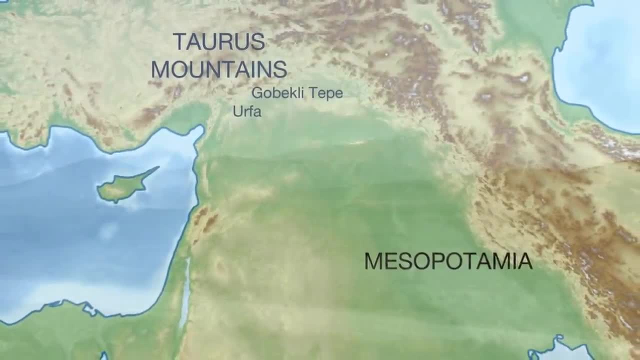 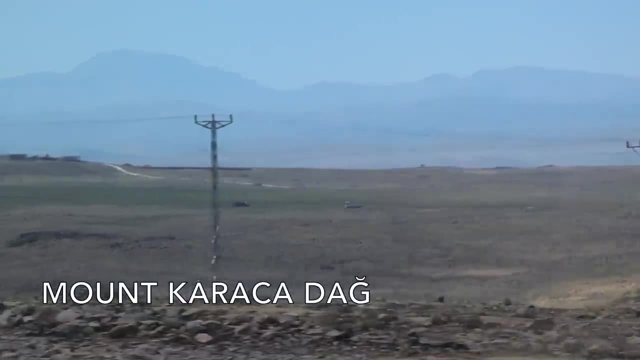 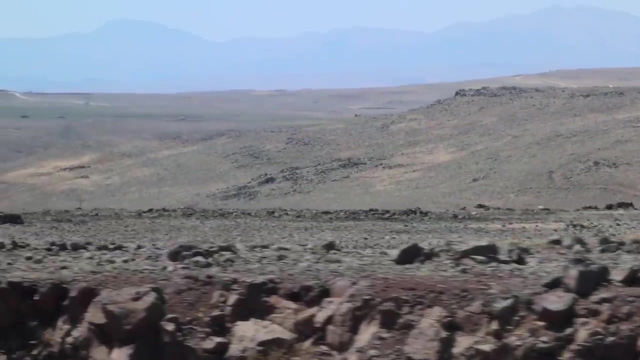 To the north-east, The great mountain of Karakadog sprawls Always prominent extinct volcano, from where some of the earliest evidence of cultivated einkorn wheat has been found. Perhaps it is no coincidence that in a great arc around Gobekli Tepe, some of the most 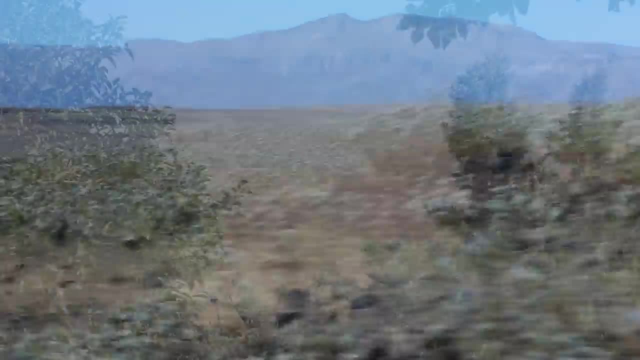 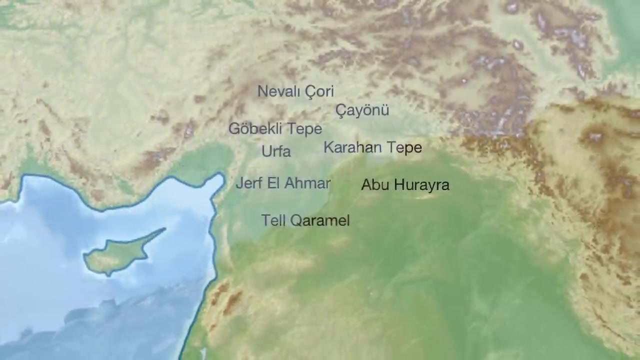 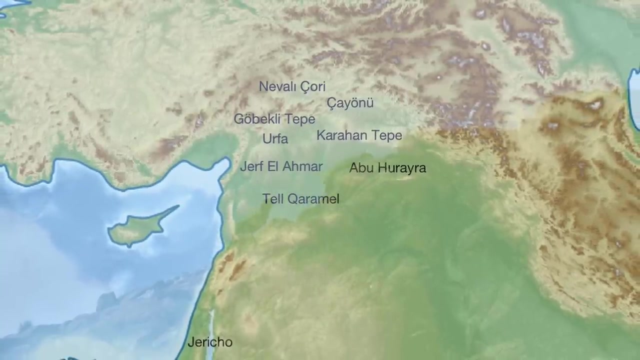 important early Neolithic sites found anywhere have been discovered At Tel Karamel, Djerf el-Akhmar and Chianu, to mention a few. The evidence speaks of a world on the verge of aggravation. To the east, To the west. 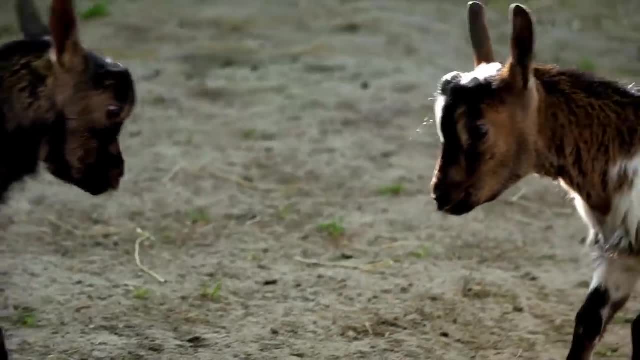 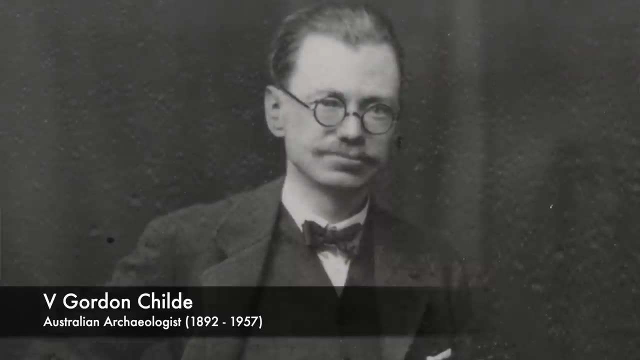 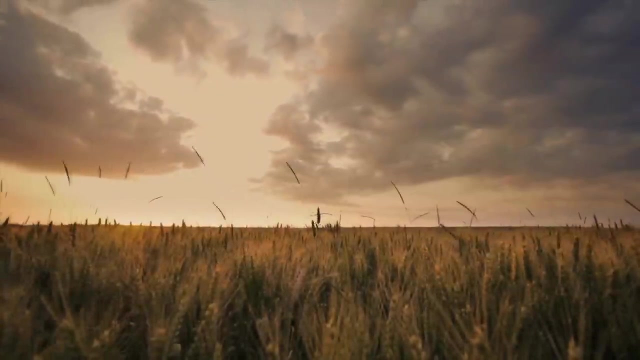 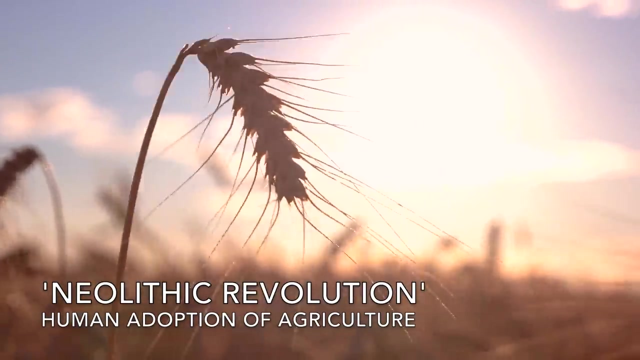 To the north, To the south, Still more to be discovered. In the 1930's, only a short estimate of Israel's Final Revival was left: ation, The Taurama was the only long-function Arab Castle To North In the 1930s. molt was brought to a humble wrist by one. and this next great, the rolling 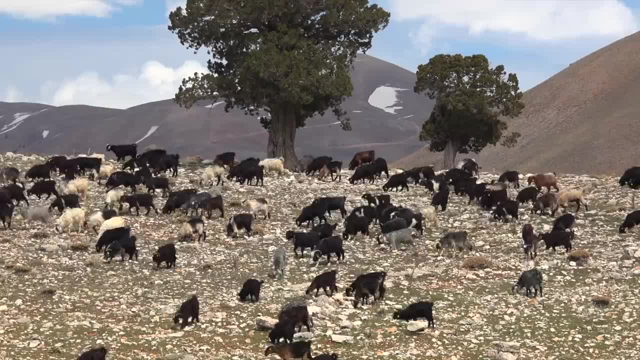 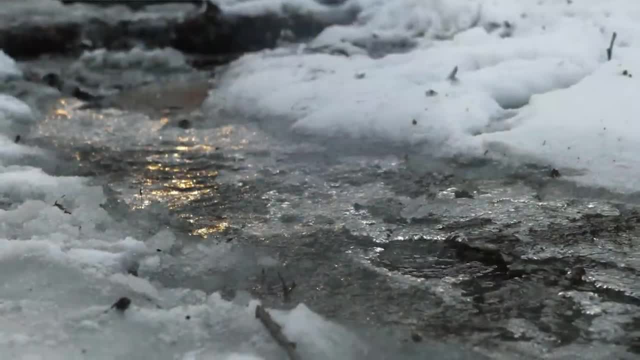 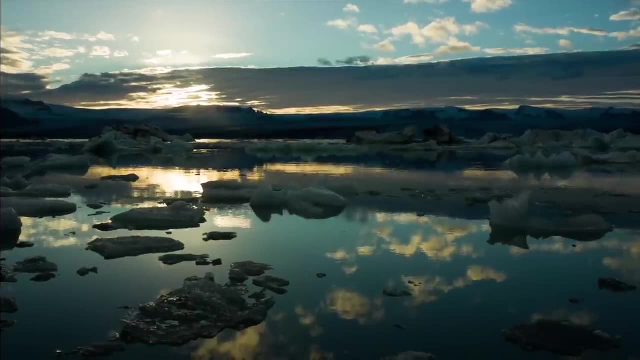 of heavy people brought продолж Wiedersehen to hurting the country, Only man securing this. such a fifth" Thanks to Lobko Sal Shar. as well as art. then, By around 10,800 BC, a relatively brief yet still centuries-long return to cold, dry conditions. 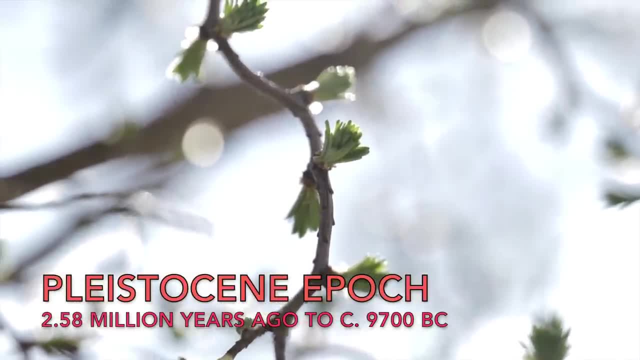 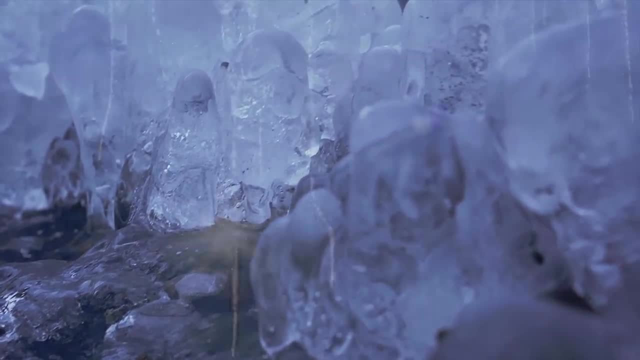 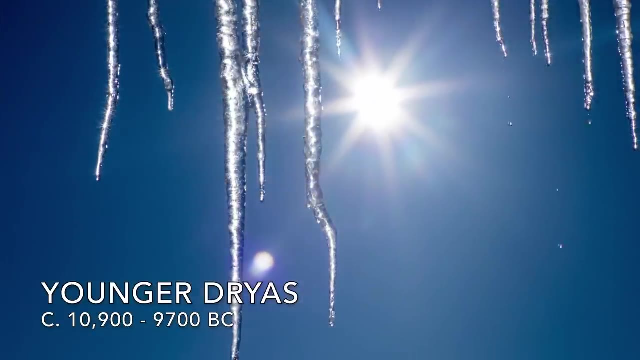 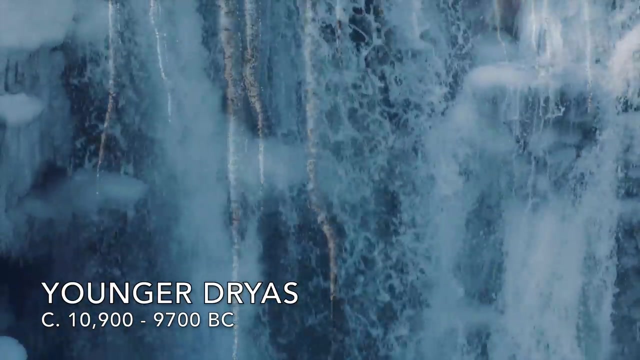 of the last Pleistocene was ushered in, potentially lasting for a thousand years. Since its initial discovery well over a century ago, the Younger Dryas period has loomed large in accounts of the origins of agriculture, with the suspicion that many newly swelled. 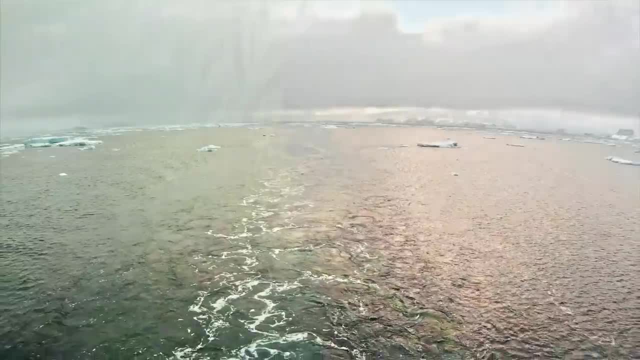 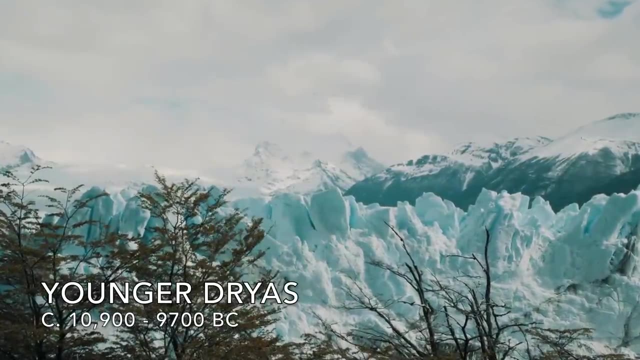 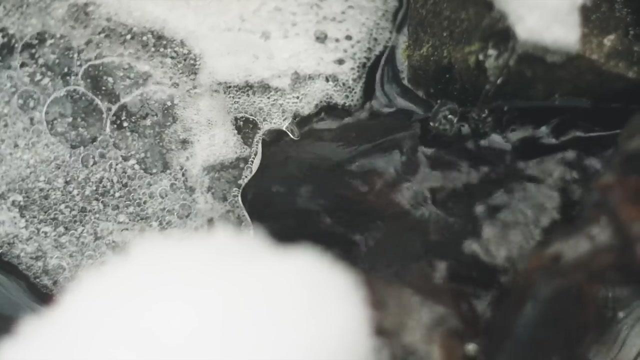 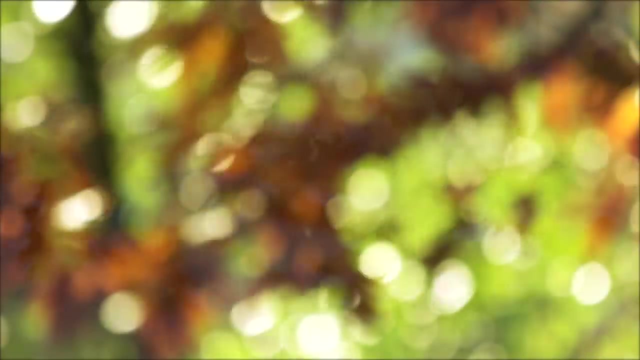 communities would have had to change their lifestyles yet again, congregating around water supplies And possibly intensifying their food production strategies, according to some theorists, beginning to experiment with sowing and tending crops and cereals, and eventually to trap and keep. 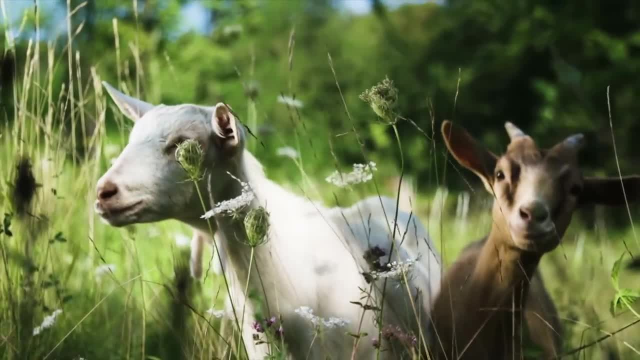 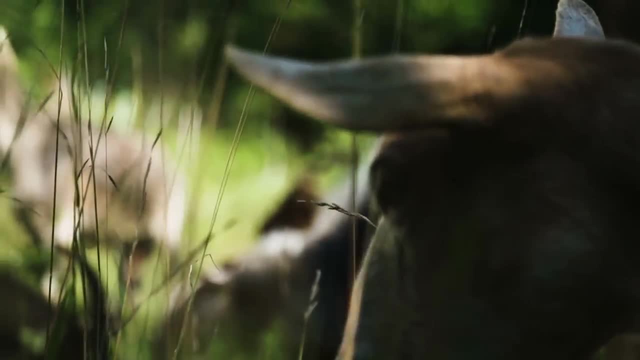 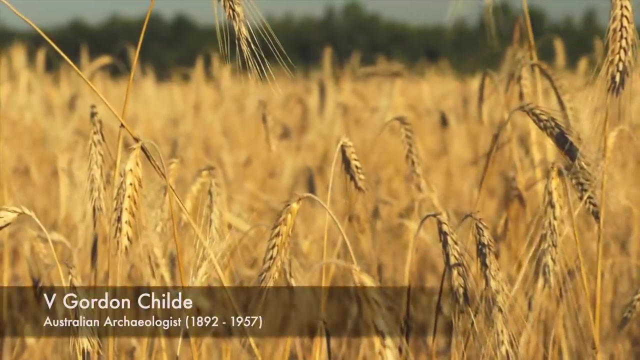 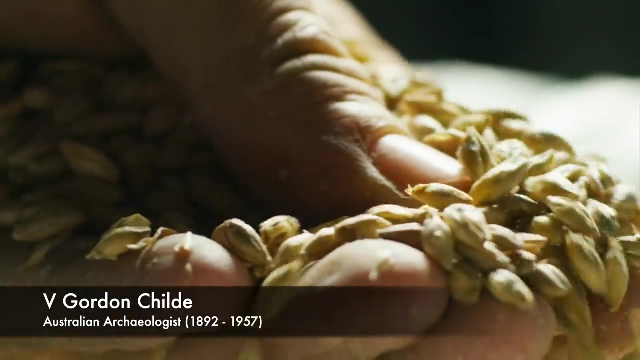 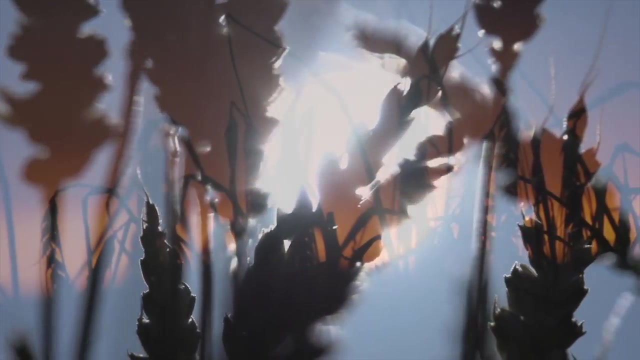 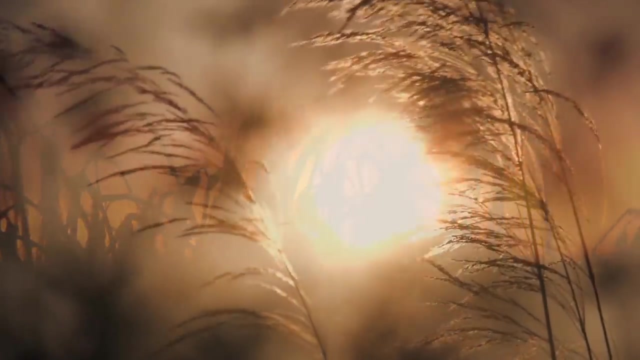 animals. In recent years, the picture has changed, With the recognition that early theorists like Childe succeeded in explaining the how, but not the why or, perhaps most importantly, the when. Just in the last decade, vast amounts of new empirical data has continued to stack up, creating 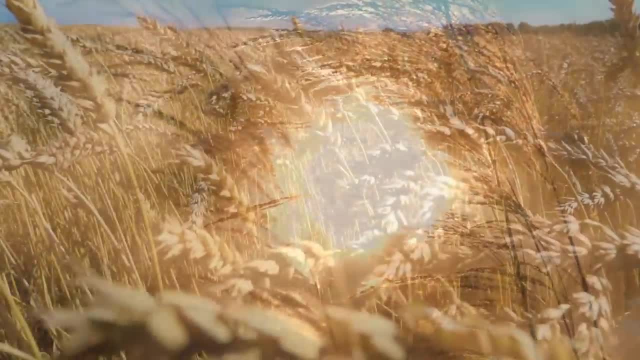 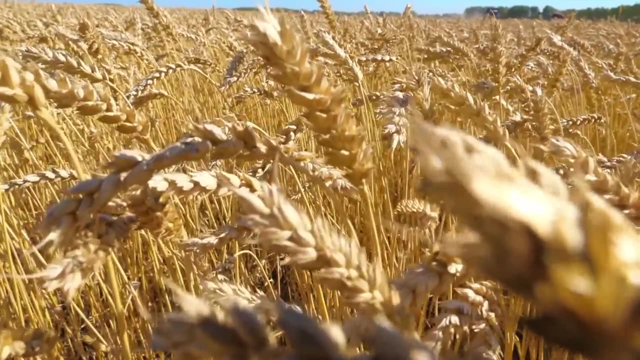 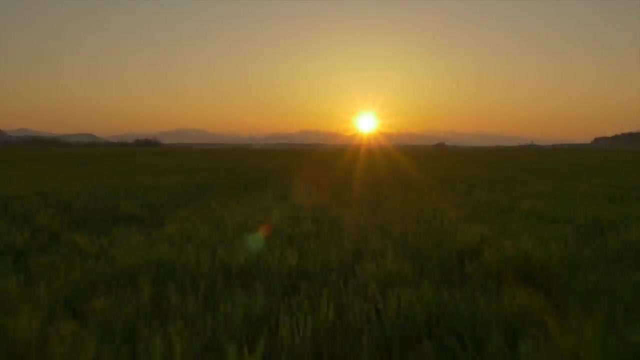 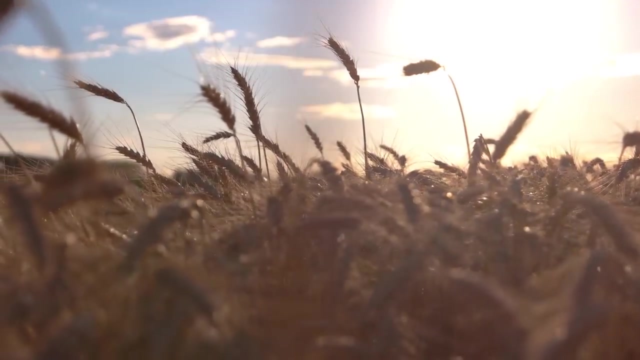 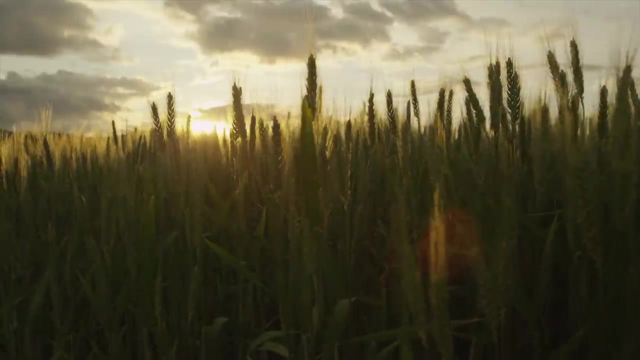 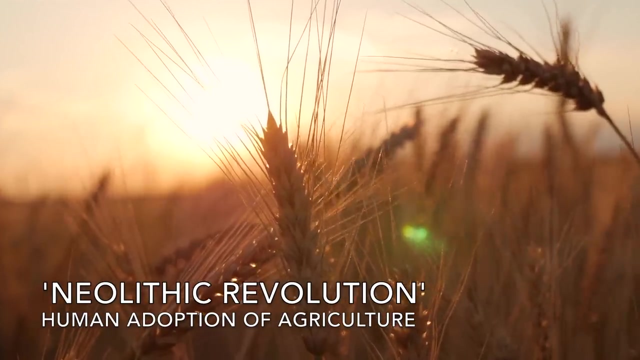 an increasingly fine-tuned account of the transition from foraging to farming, Overwhelmingly suggesting not one origin but many places and many times, Some ultimately unsuccessful attempts taking place long before Gobekli Tepe, Rather than a revolution per se, eliciting the idea of some kind of an overnight transformation. 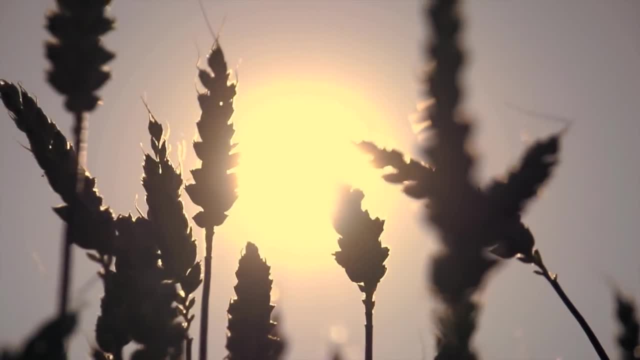 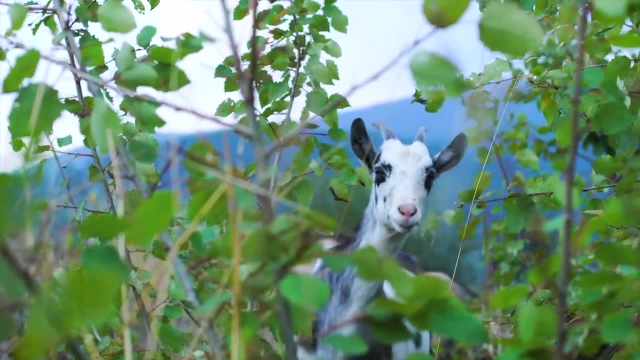 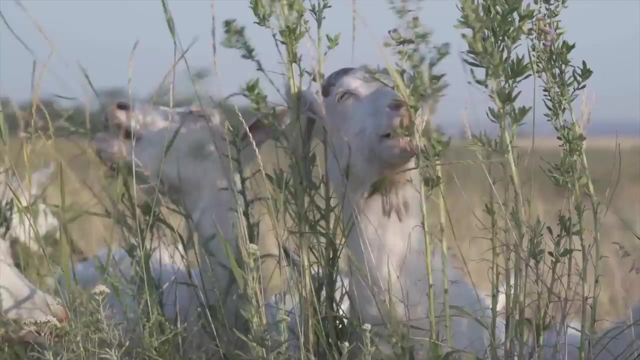 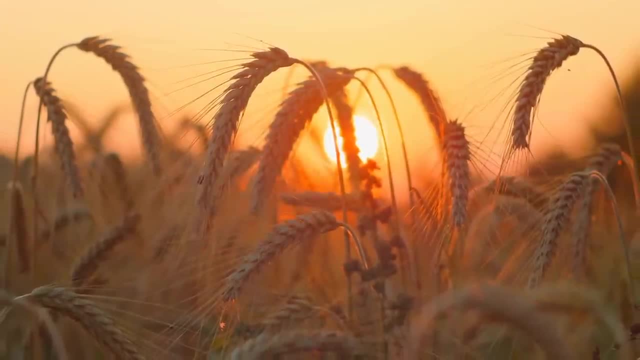 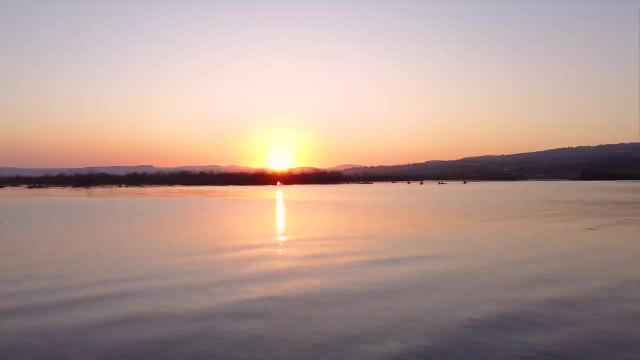 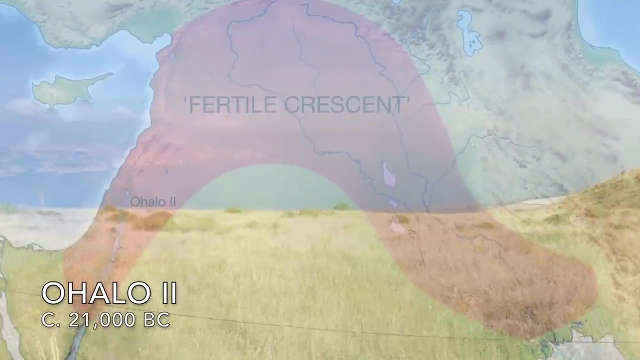 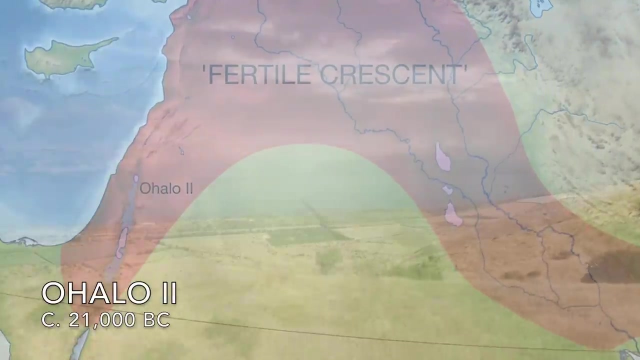 One particularly early example of attempted plant domestication was found on the shores of the Sea of Galilee At Ohalo II. the remarkable remains of a Paleolithic settlement yielded an impressive array of of seed grasses and legumes, along with the tools needed to thresh and cultivate them. 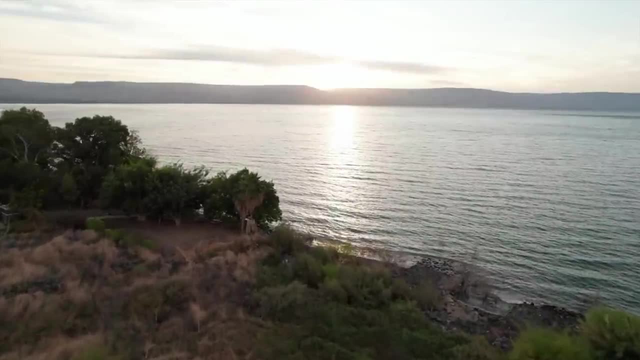 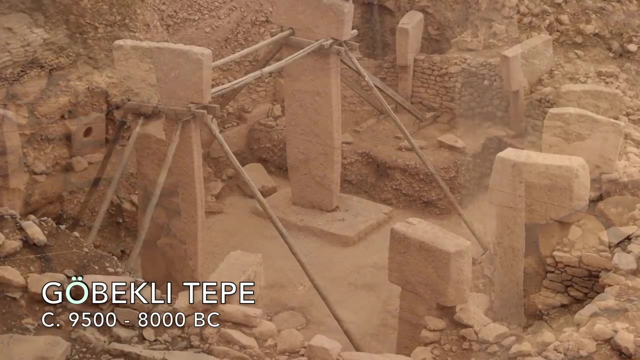 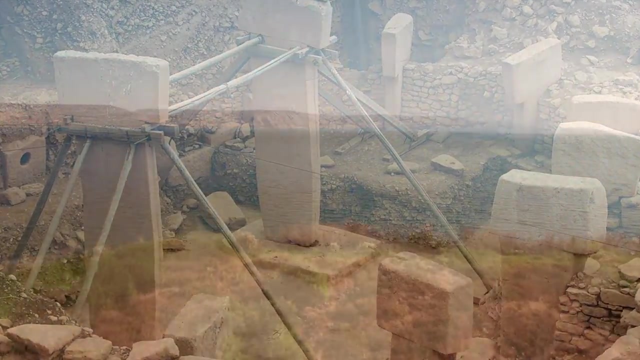 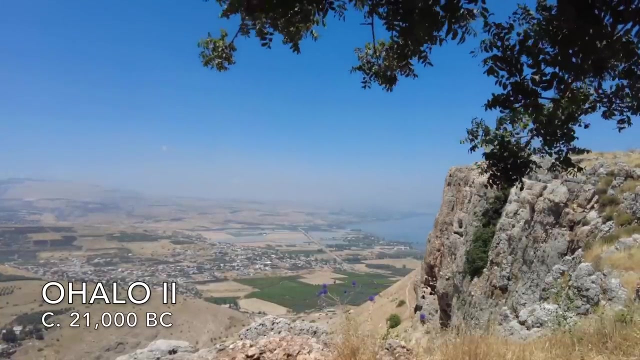 Thus, by the time the first monoliths were erected in the southern foothills of the Taurus Mountains, humans had already been experimenting with farming for over 10,000 years. The evidence from this one very small community continues to detract from the hypothesis of 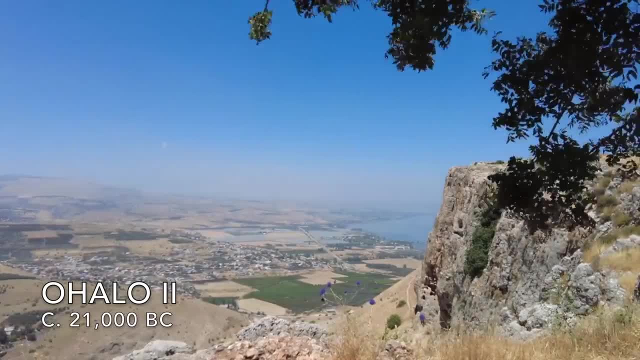 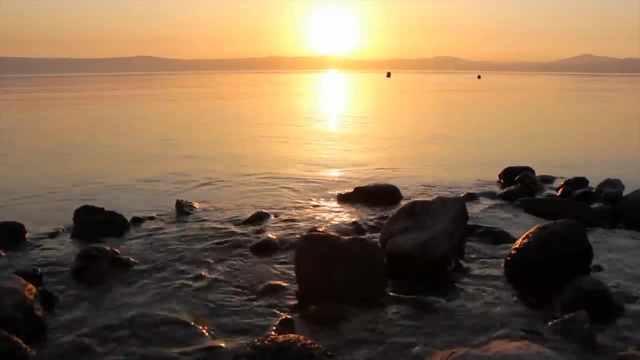 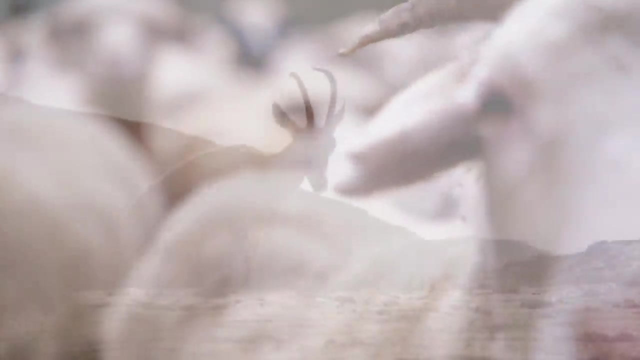 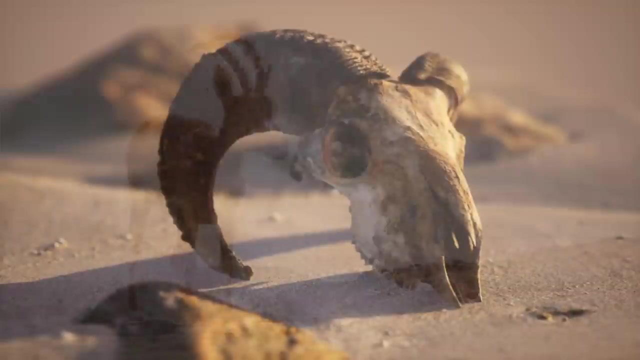 population pressure being the primary driver of sedentism and agriculture. Animal husbandry was different, As we have seen, no domesticated animals at all were allowed to live in. the wild have been found at Gobekli Tepe, and very few before that time anywhere else in the world. The process of domestication, which actually changes the physiology of the animal in question, is only even possible with a very small number of animals, And even then the shock and trauma of captivity very often creates infertile or deformed offspring. If procreation 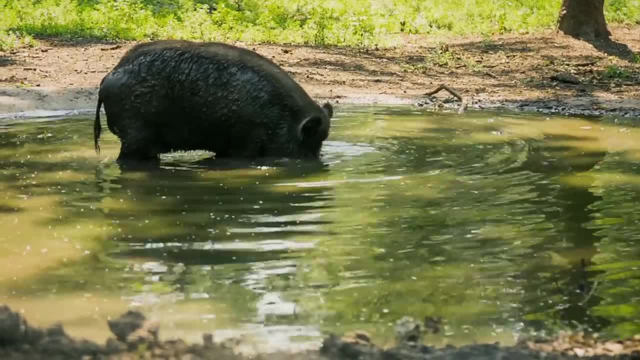 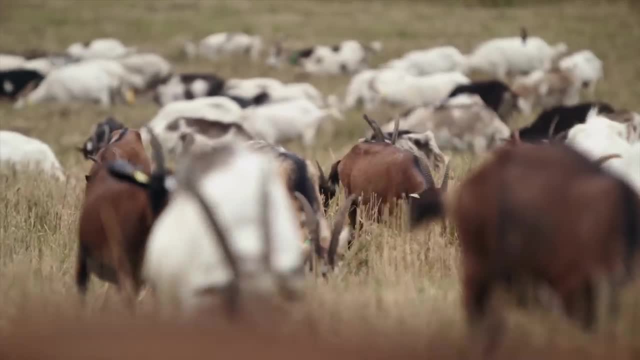 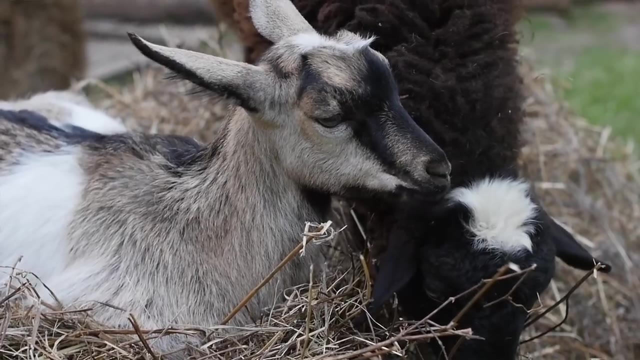 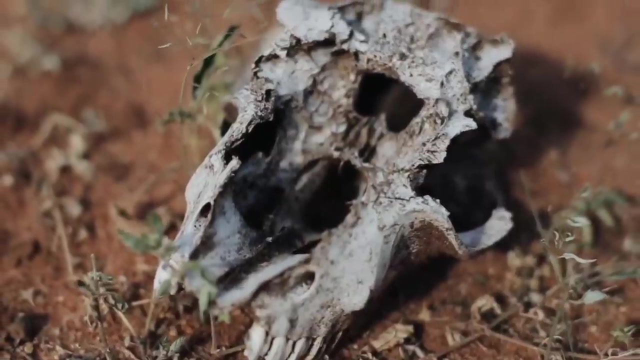 is even possible at all. In short, animal domestication requires a great deal of effort with very little return in the short term. There are some indications that Gobekli's neighbouring site of Chianu was somewhat successful with the domestication of animals, But there are also some indications that Gobekli's 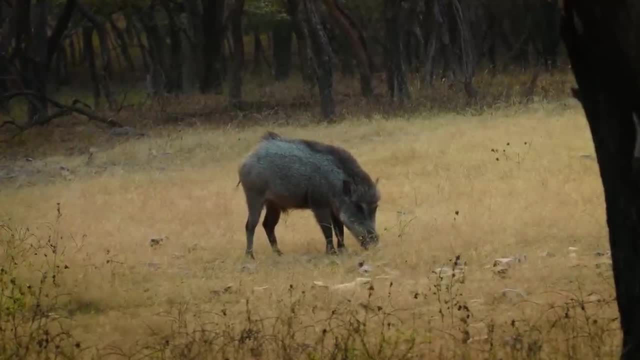 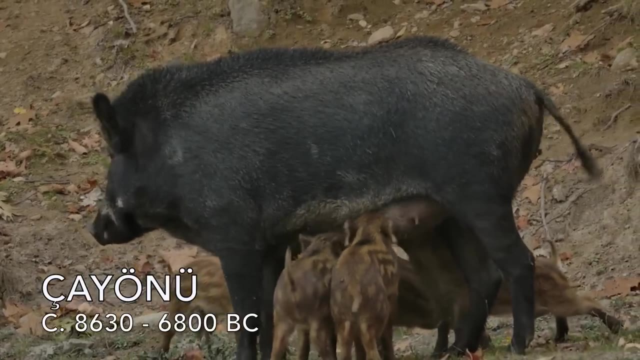 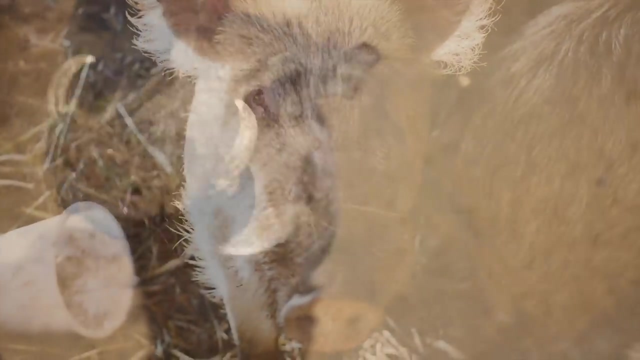 neighbouring site of Chianu was somewhat successful with the domestication of wild boar, With remains having multiple indicators of domesticity by around 8,000 or 9,000 BC, by which time the place had been a permanent settlement for quite some time. 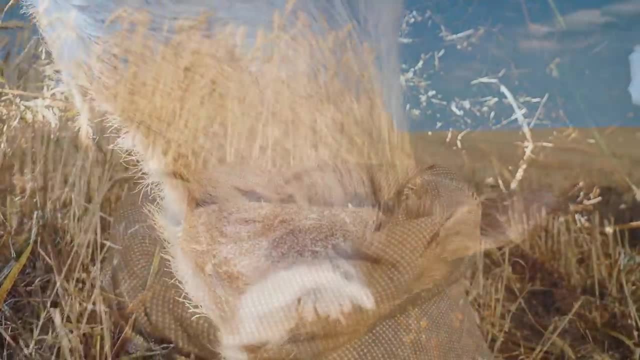 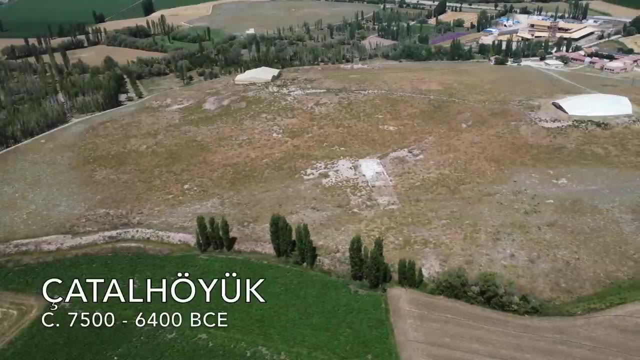 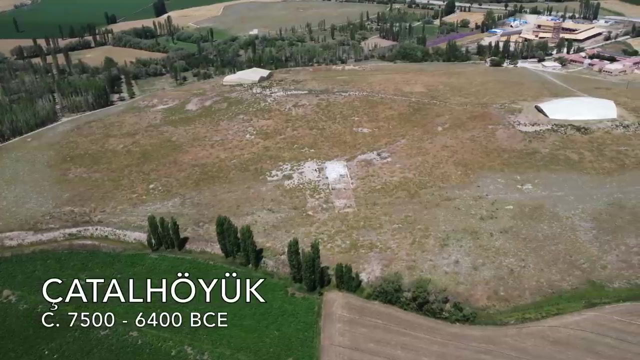 The evidence for farming being the main cause of sedentism keeps getting smaller and smaller, Even at Çatalhöyük, a vast Neolithic proto-city of at least 5,000 people that developed much later than Göbekli Tepe. 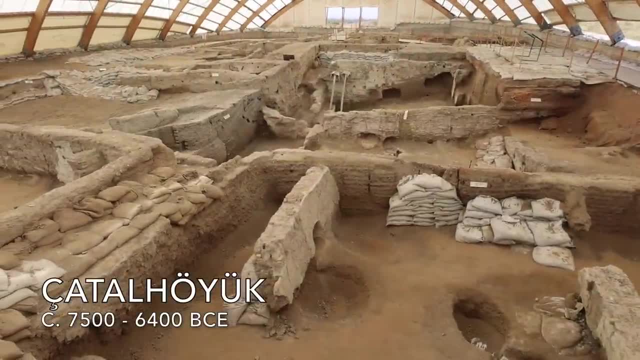 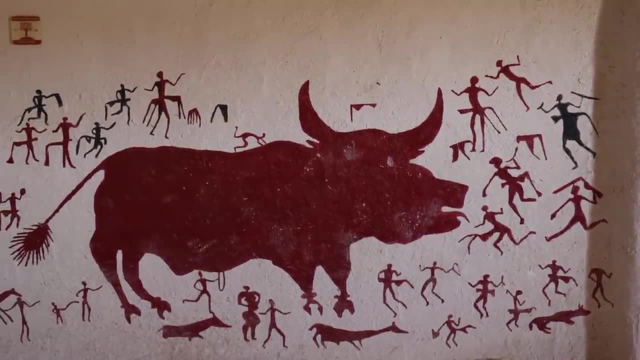 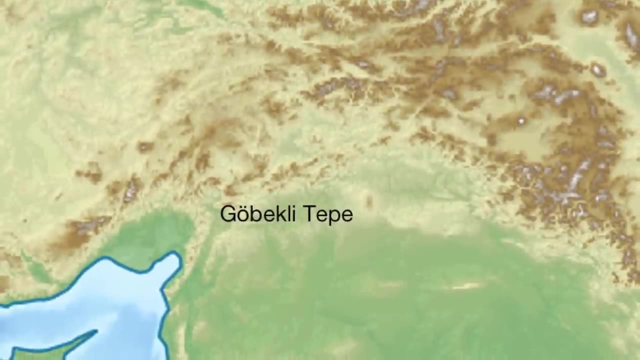 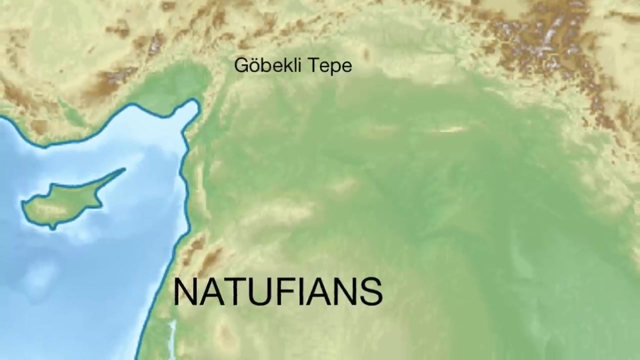 there is almost no evidence of domesticated animals hunting still playing a huge role in the ritual and domestic life of the community. To the south of Göbekli Tepe, along the Levantine shore, not far from Ohalo II, can be found some of the best evidence for the origins of so-called Neolithicisation. 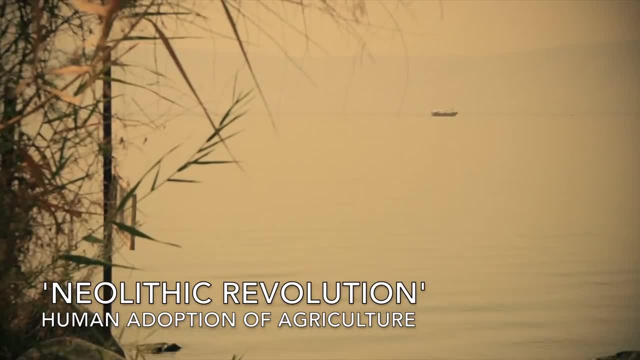 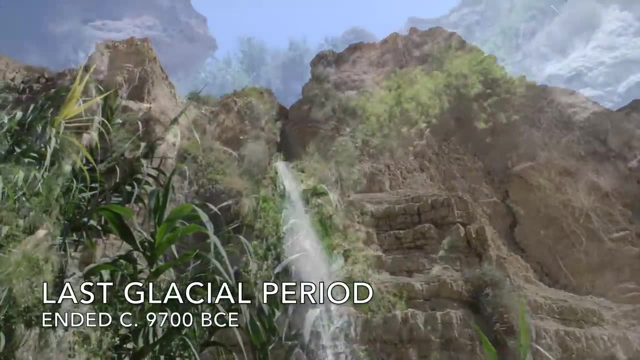 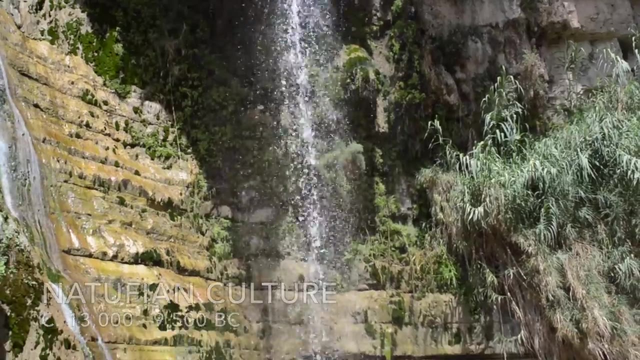 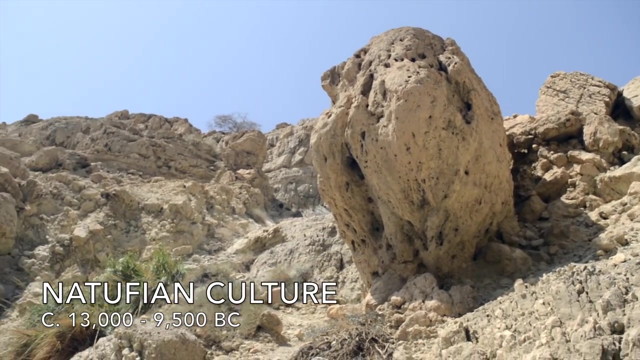 For here, in a surprisingly well-studied region, people seem to have begun to truly settle down towards the end of the last ice age. This was the time of the Natufians, And incredibly there is good evidence here for a revolution not in farming technologies, but in the mind. First discovered by pioneering archaeologist Dorothy Garrard in the early 20th century and discovered in the early 20th century and discovered in the early 20th century named after the typesite of Wadi al-Nutuf in what is now Palestine. 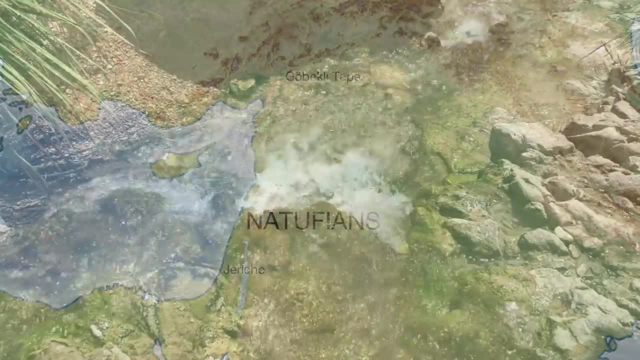 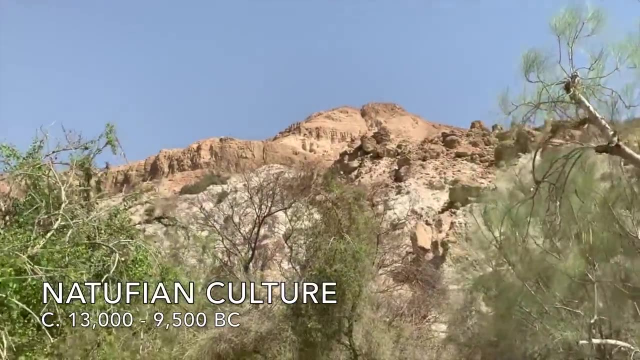 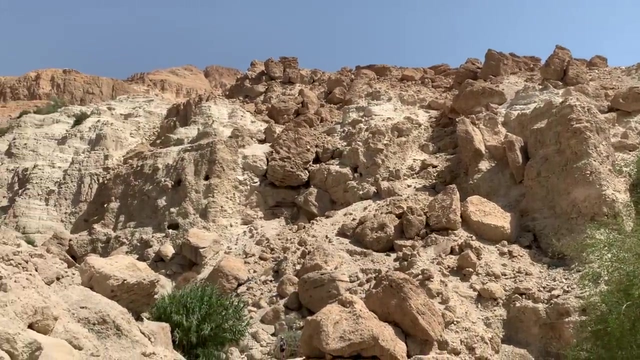 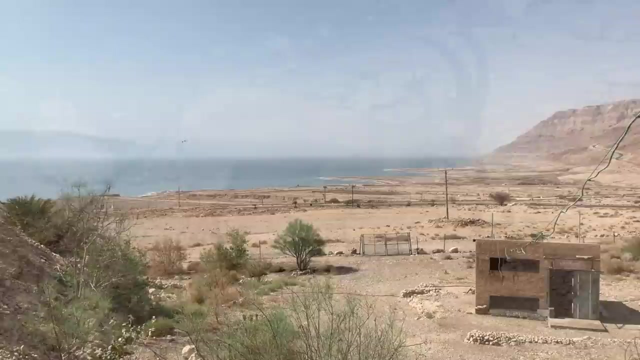 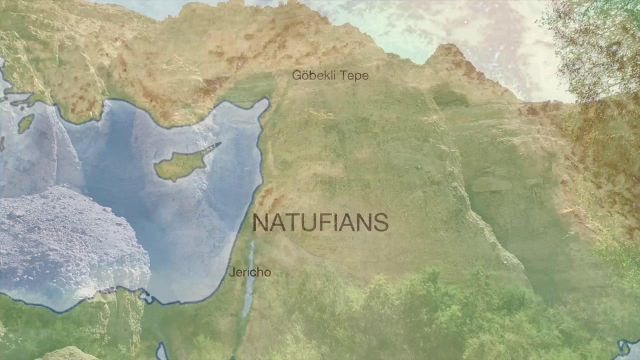 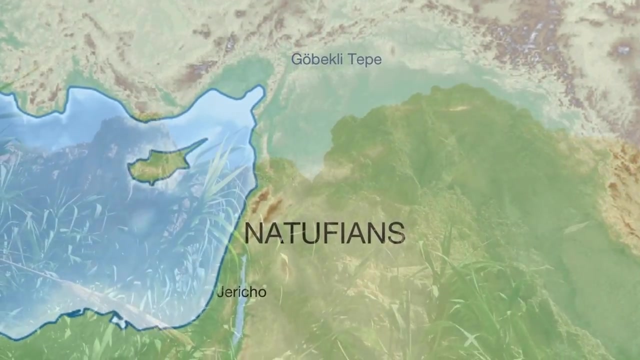 Like Göbekli Tepe, the astonishing culture of the Natufians made headlines all over the world. The Natufians still lived a largely hunter-gatherer existence, but seemed much more of a complex state than groups before. They lived in set areas, in settled villages, where they returned to bury their dead, engage in elaborate burial rituals and create impressive works of art. 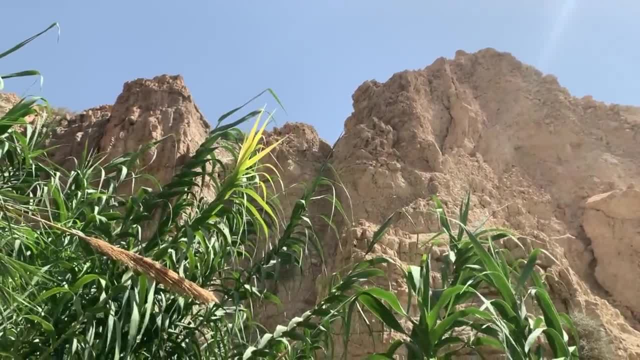 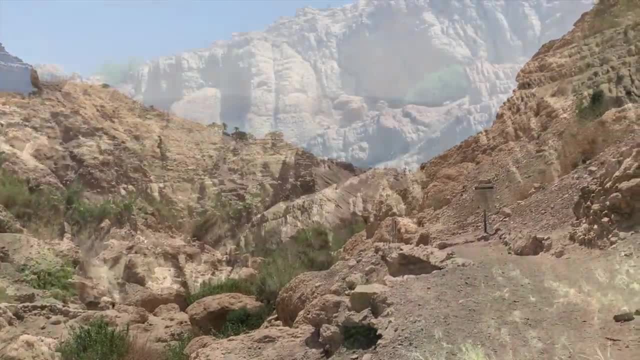 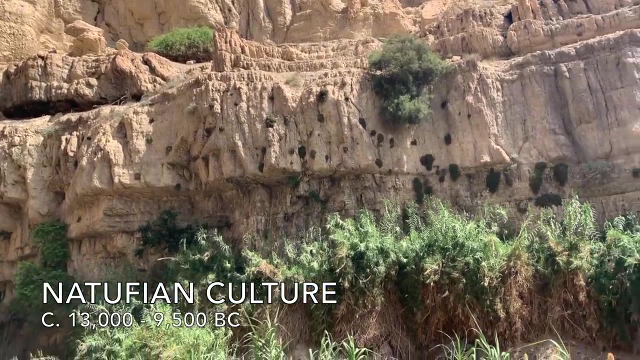 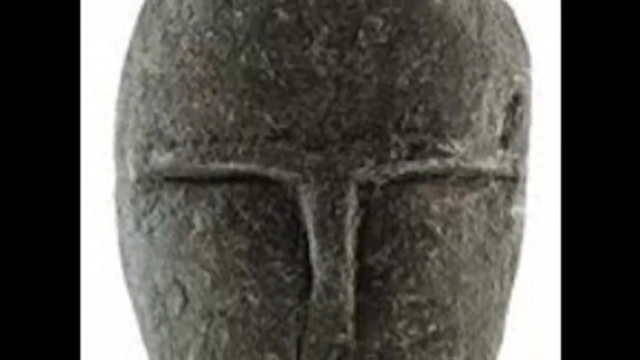 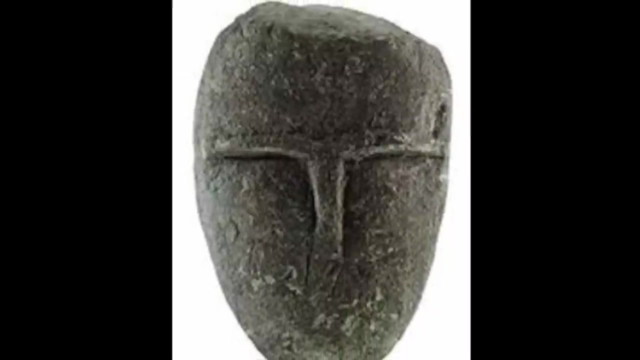 Traits which probably reinforced cultural identities and links to the land, Perhaps one of the first complex societies, Complex societies found anywhere. So then, was it culture, human creativity rather than economics, that spurred on the adoption of agriculture? And just how far back does the evidence go? 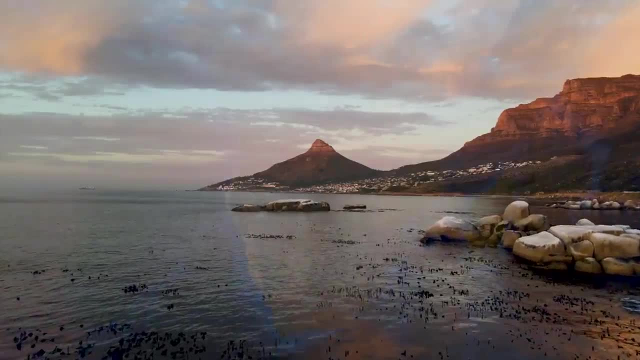 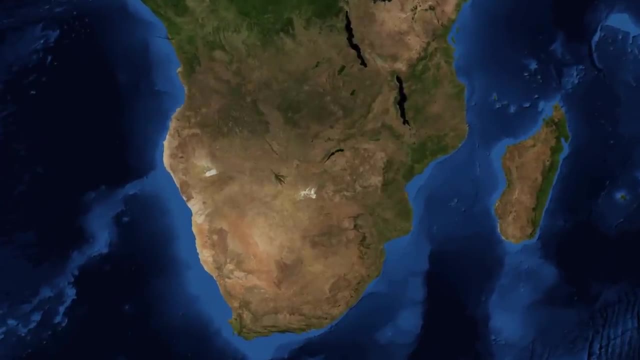 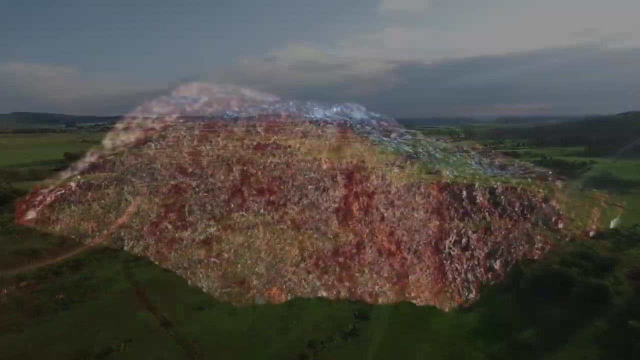 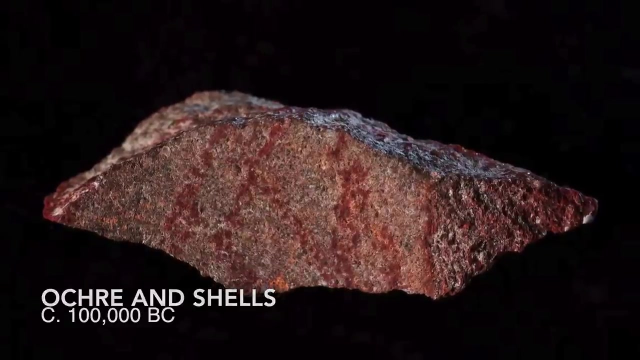 The first visible glimmerings of human creativity in the archaeological record appear on the southern tip of Africa as much as a hundred thousand years ago, in the form of ochre pigments and later in crafted shell decorations As much as a hundred thousand years after the first evidence of anatomics. 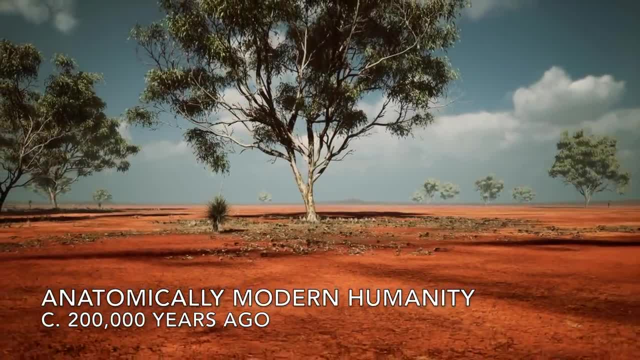 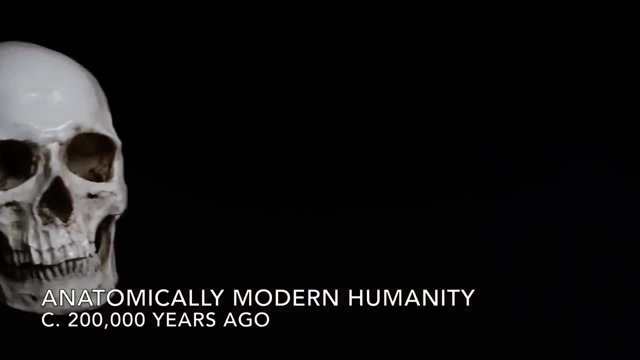 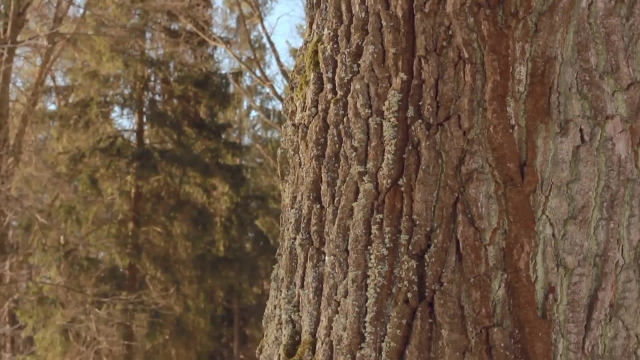 As much as a hundred thousand years after the first evidence of anatomics of anatomically modern humans identical to us today, capable of complex forms of communication for the first time. However, it is only after around 45,000 years ago that evidence for creative 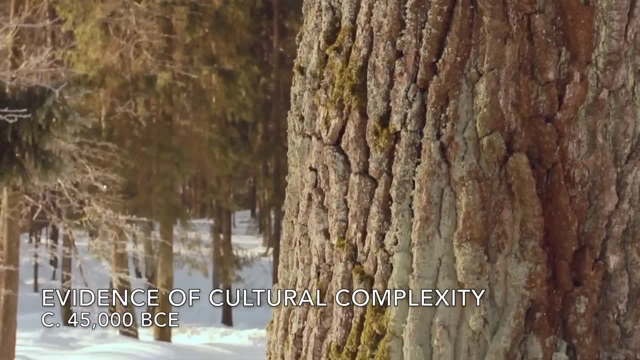 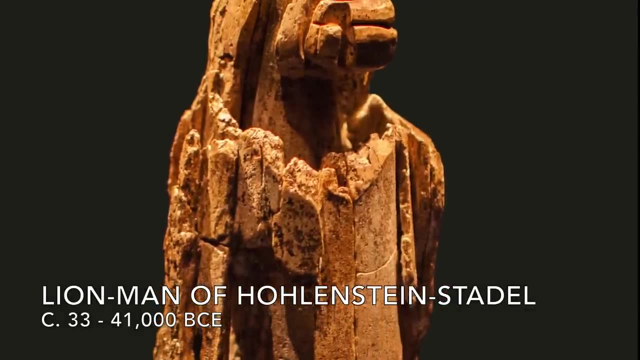 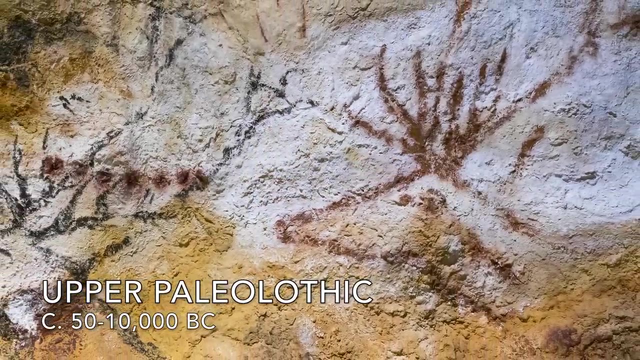 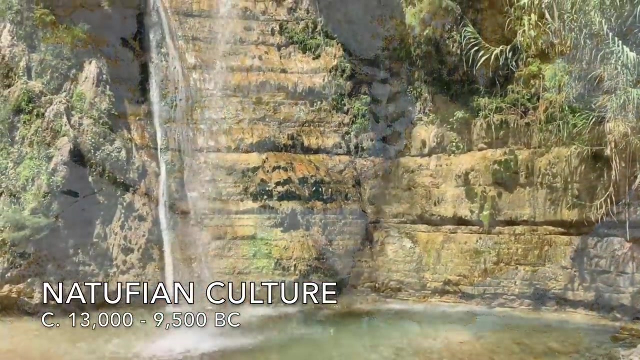 complexity really begins to be found In isolated pieces like the lion man of Holenstein, Stadel, scattered Venus figurines and ultimately, in the cave paintings of the Upper Paleolithic. Arguably it is only with the likes of the Natufian some 15,000 years ago and 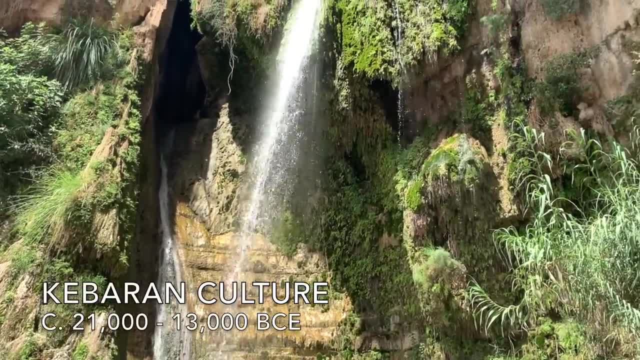 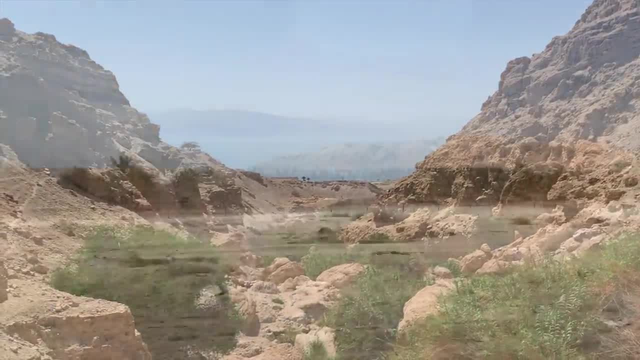 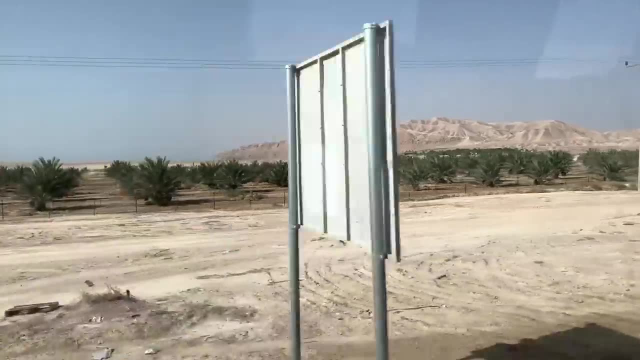 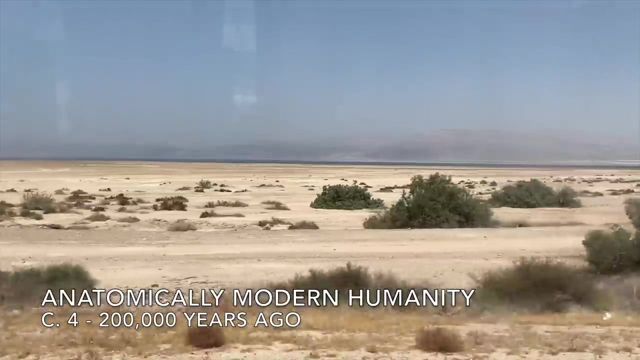 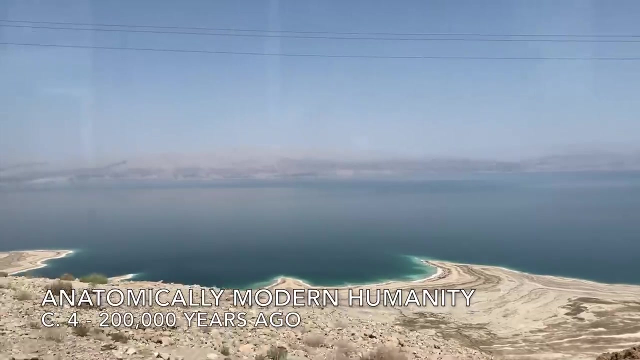 perhaps the Qabaran before it, that evidence of societal formation really begins. The question of why it took so long for anatomically modern humans to develop such artistic and cultural ideas and objects has been defined by British archaeologist Colin Renfrew as the Sapient Paradox. Anthropologists would say that the concept of a large group of 100 or more living permanently together in close proximity all year round. 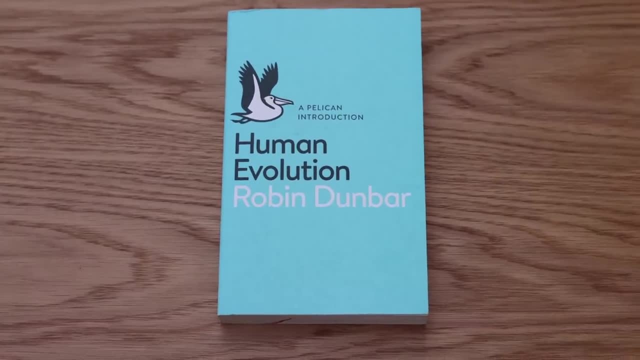 The question of why it took so long for anatomically modern humans to develop such artistic and cultural ideas and objects has been defined by British archaeologist Colin Renfrew as the Sapient Paradox: The question of why it took so long for anatomically modern humans to develop such artistry all year round. 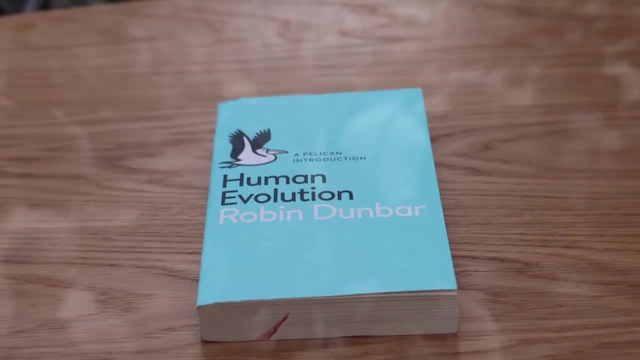 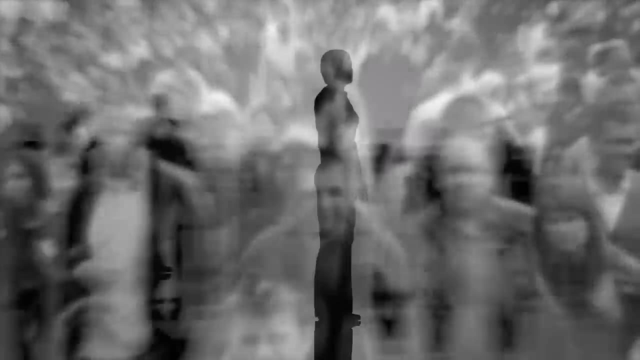 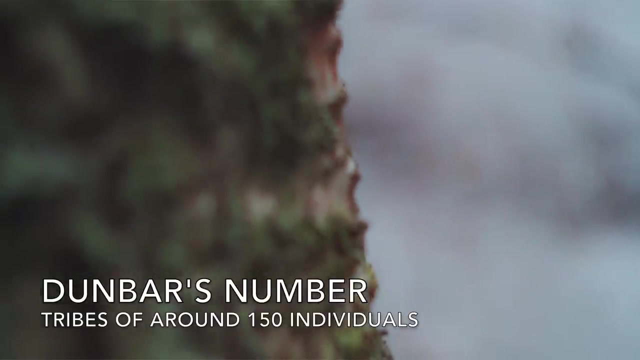 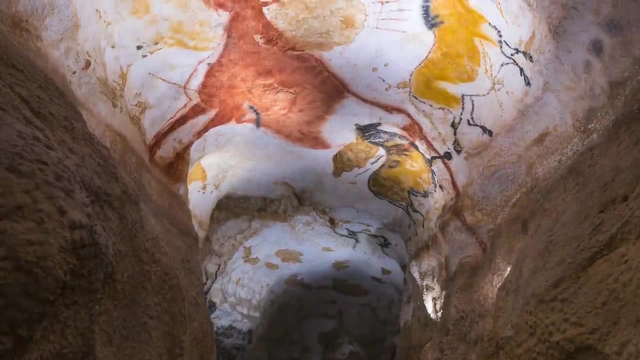 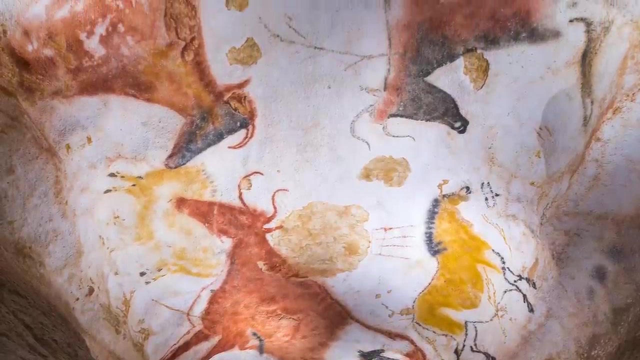 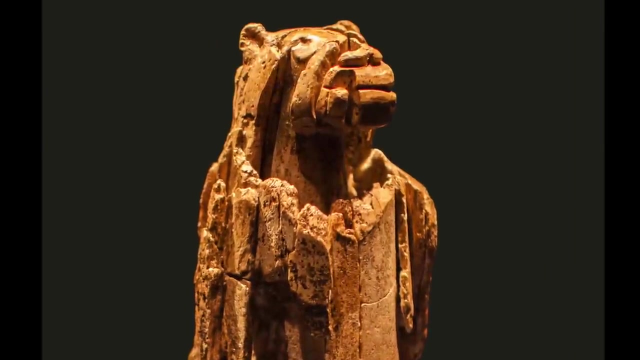 The question of why it took so long for anatomically modern humans to develop such artistry all year round. Some strategic reason for that was the hunter-gatherer groups. A shared story or collective idea spurred on not by biological evolution but by culture. A hypothetical revolution in shared symbolism which would 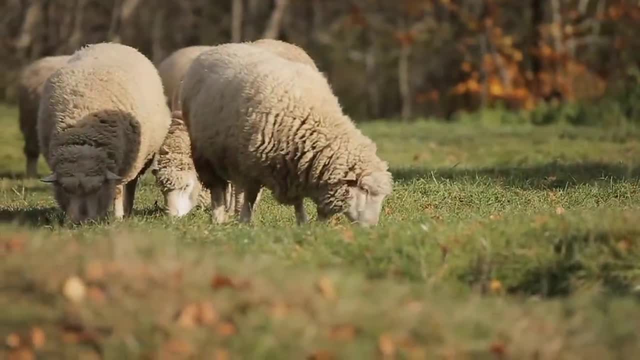 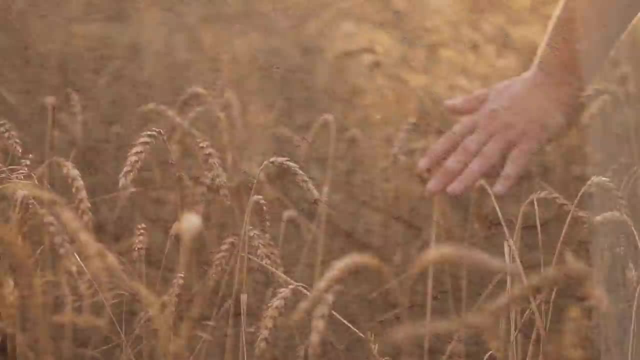 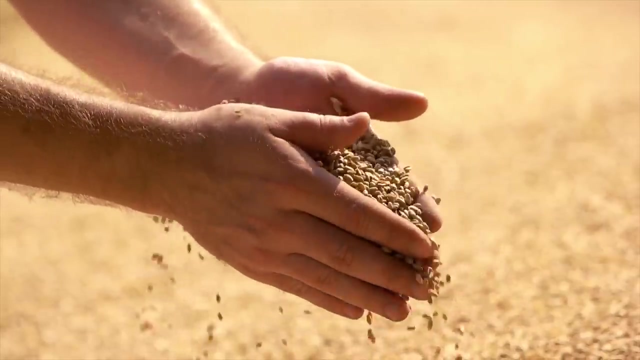 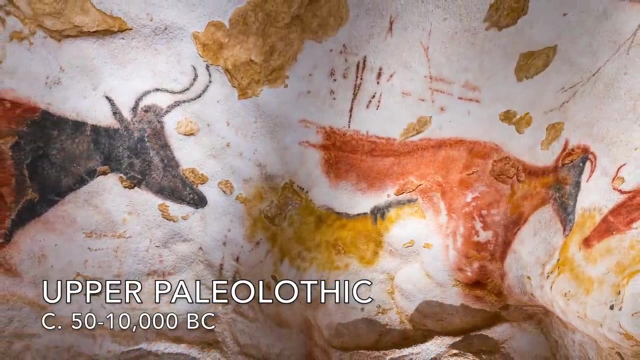 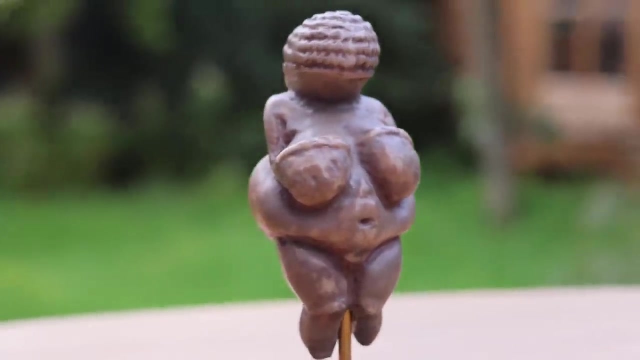 eventually spur on mastery over nature, division of labour, increasingly impressive artistic achievements and population growth. A revolution which began in the mind. The creative explosion of the Upper Paleolithic, most commonly represented by cave art and the famous Venus figurines, is well-known in popular culture. Less well-known are the 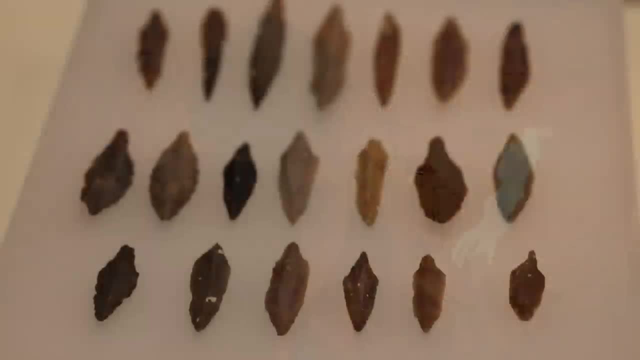 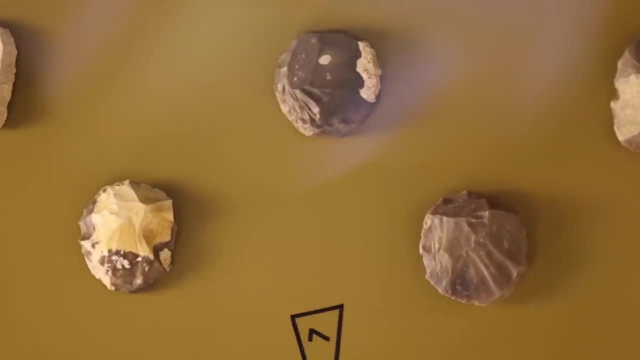 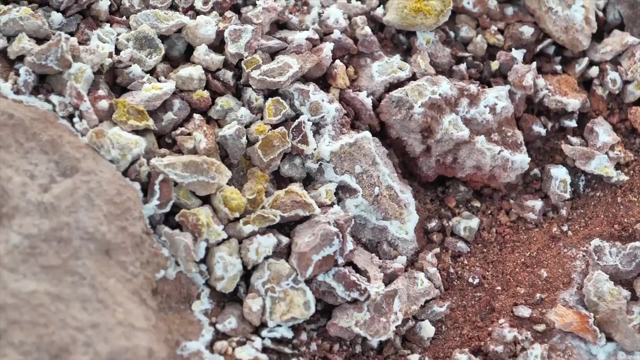 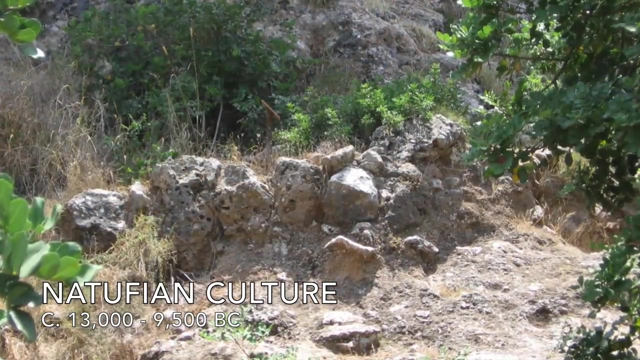 vast amounts of worked items that went alongside them, signalling the apparent new-found harnessing of a vast amount of raw materials such as bone, antler, ivory, shells and minerals, The latter being especially common in Natufian settlements, Still considered hunter-gatherers who invested significant. 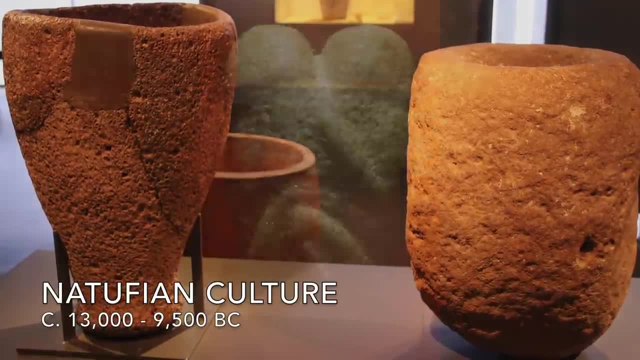 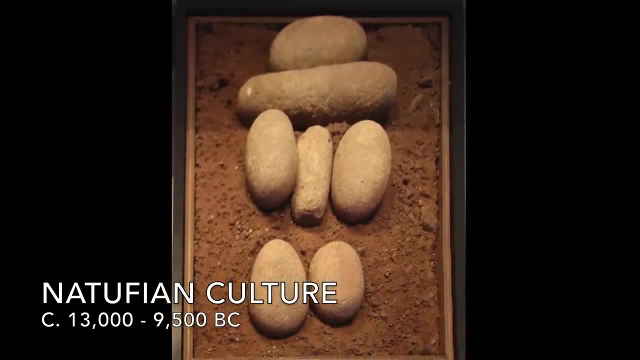 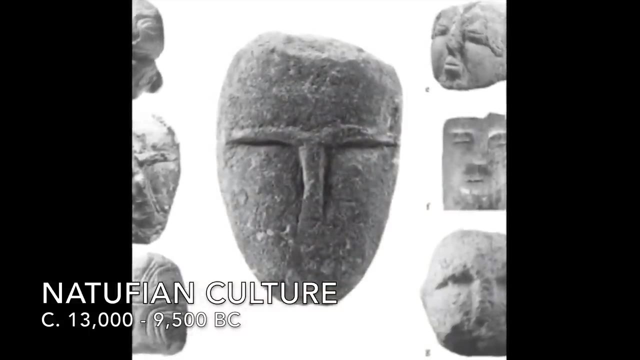 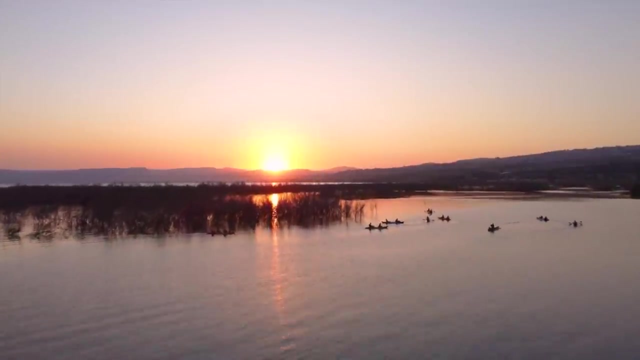 amounts of time into creating such artistic pieces. Given the sheer amount of time and effort invested, such pieces must have been immensely important. Just maybe early indicators of a shared culture to unite a people together, Such as that so clearly and strikingly depicted at Gobekli Tepe. 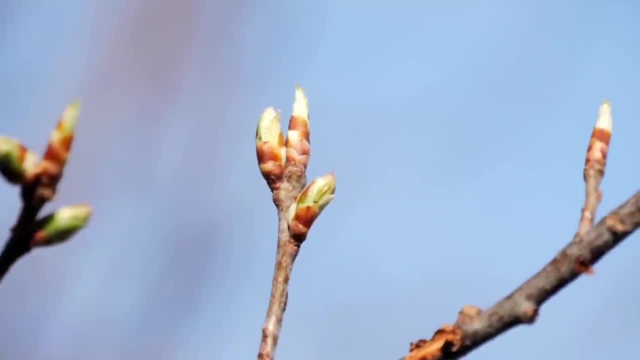 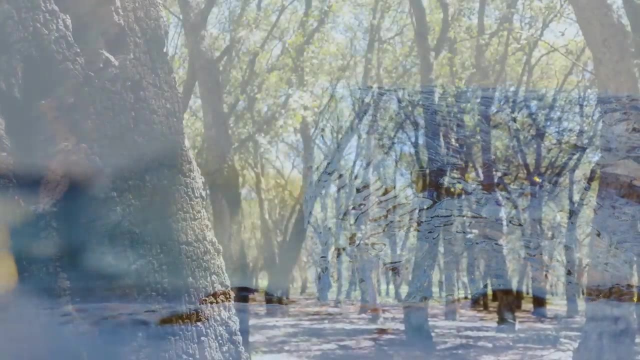 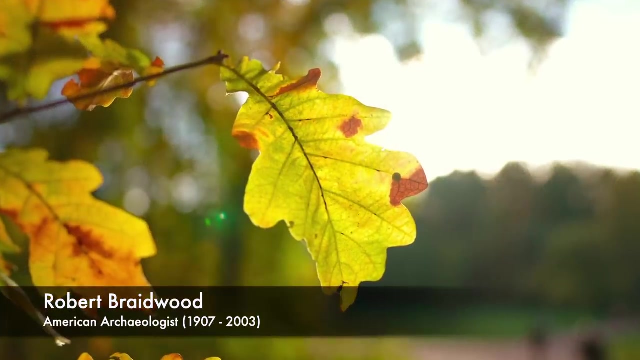 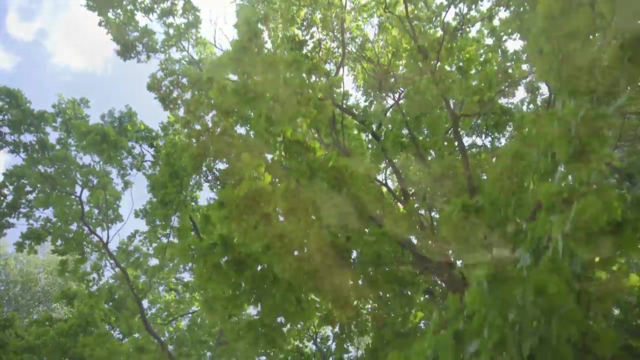 The organisational abilities required to deal with ever more seasonal and changing environments in the past has long been identified as a key factor in human advancement. The work of Robert Braidwood went further, seeing agricultural emergence as a manifestation of human ingenuity, Our ability to make life better through technology, Our ability to 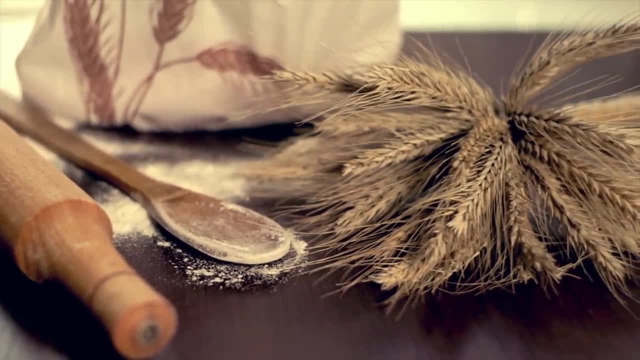 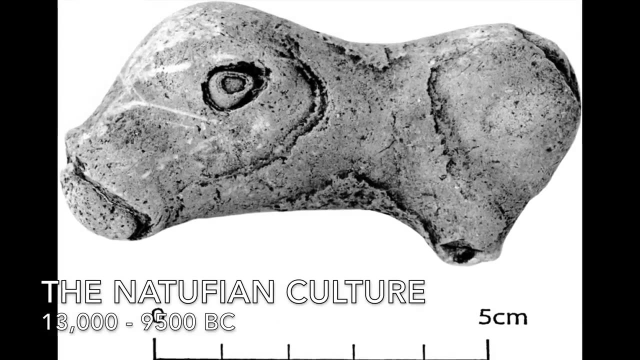 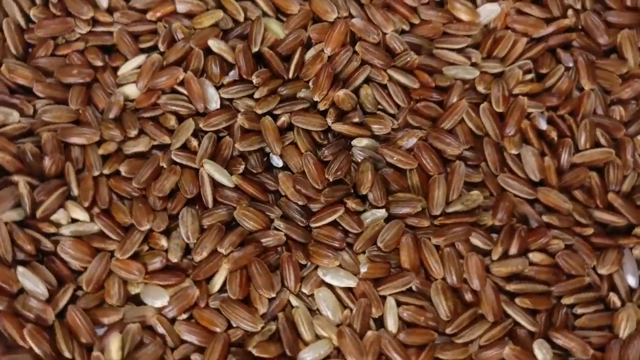 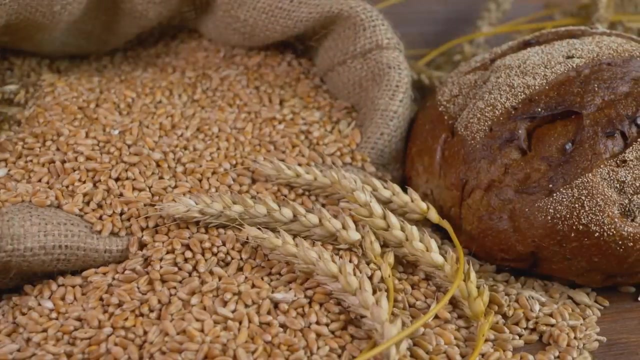 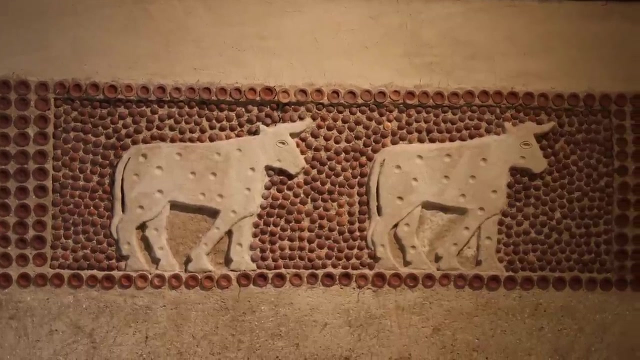 make life better through technology By creating a surplus, Such as can be seen with the Natufians and at Gobekli Tepe, Surpluses which could eventually be appropriated by people in positions of authority for individual rather than collective gain, Leading to the hierarchical societies usually favoured by. 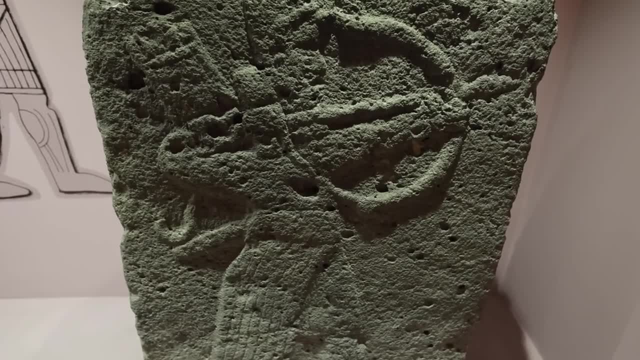 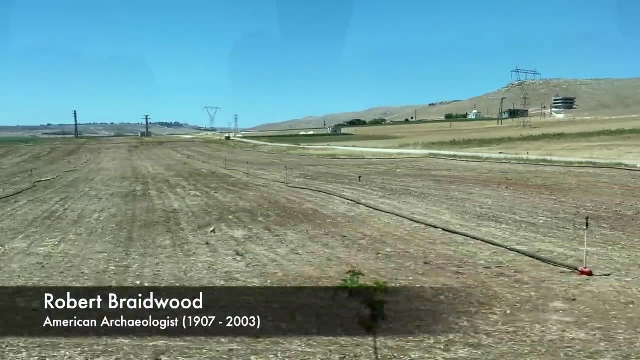 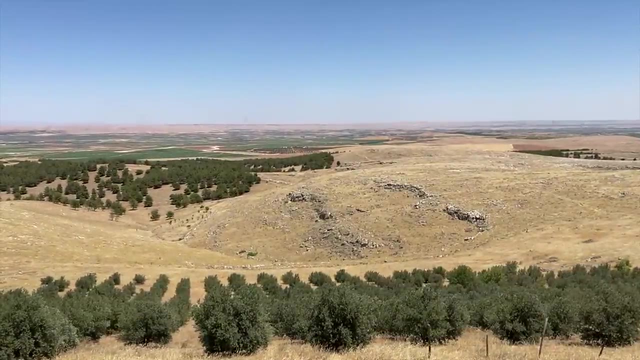 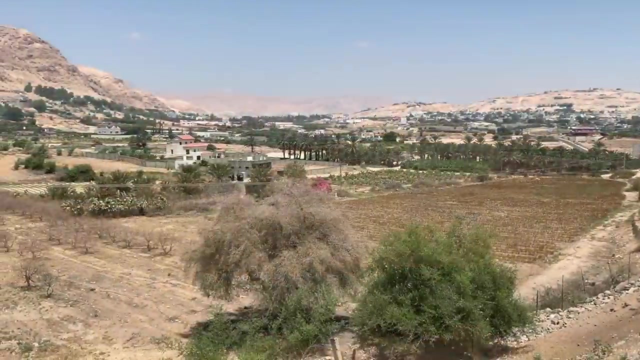 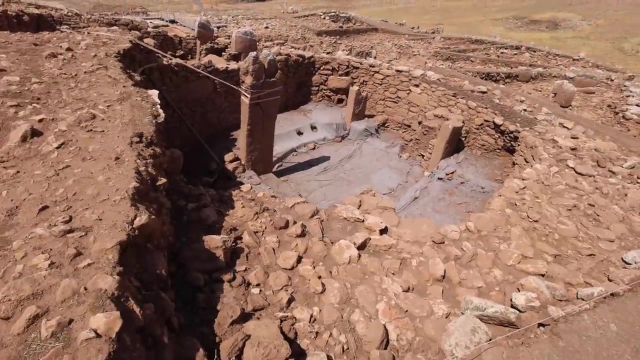 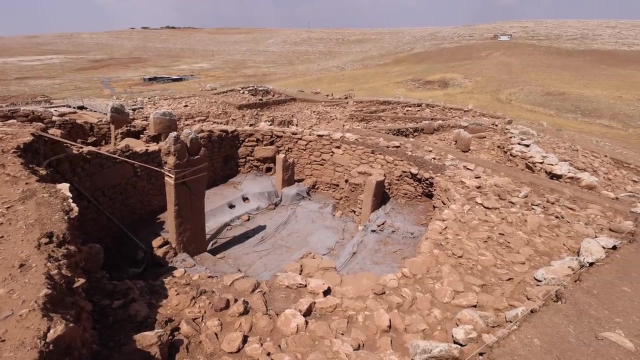 farmers. For Robert Braidwood, then, this settling in process allowed for a deeper understanding of the environment than ever before And the development of requisite technologies to manipulate it, Allowing humans to bring plants and animals under their control. And yet, despite the mounting evidence gathered over the last 200 years and more, 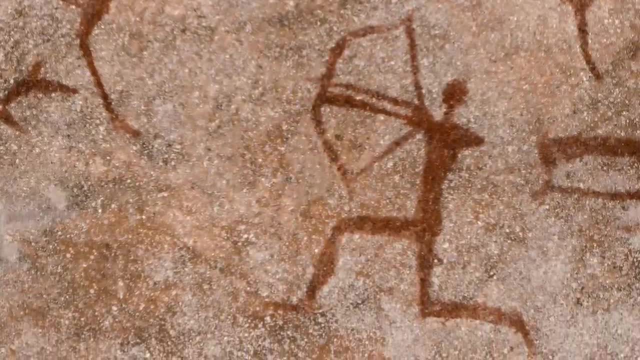 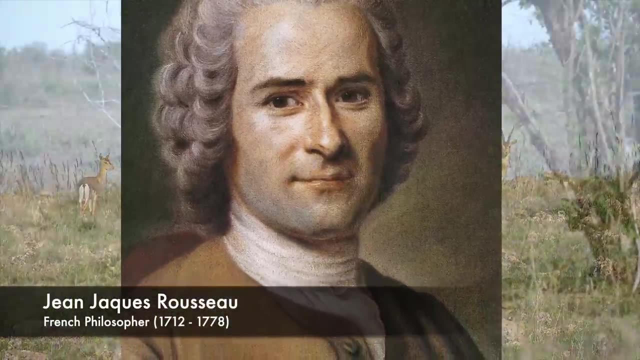 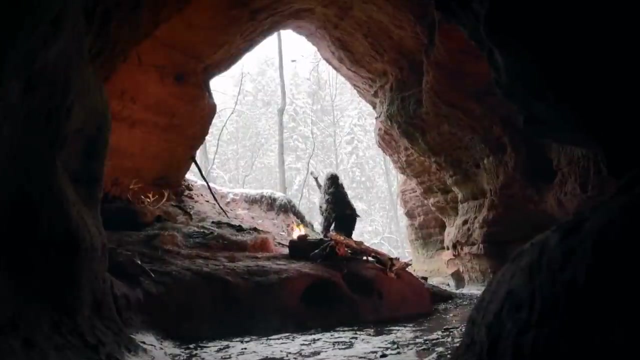 The enlightenment vision of the noble savage, first conjured up by French philosopher Jean-Jacques Rousseau, is still the prevailing view of hunter-gatherers societies in popular culture, Of simple people living simple lives with very little culture to speak of. 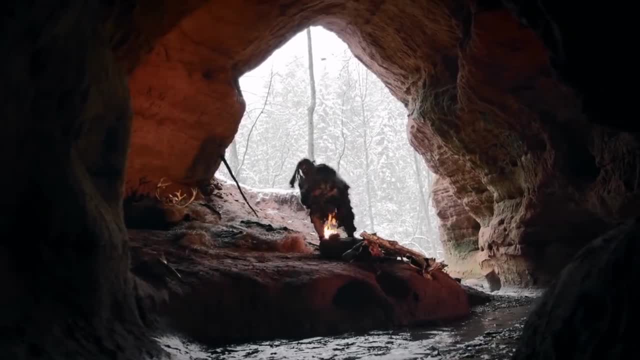 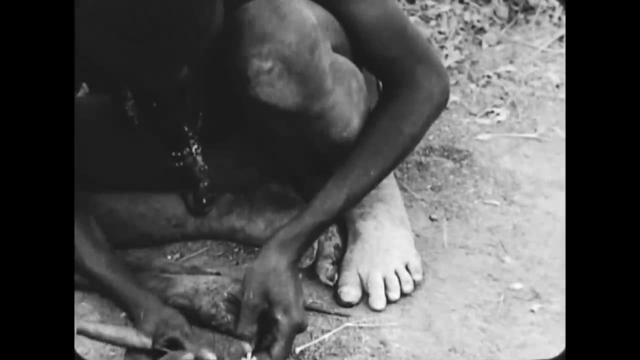 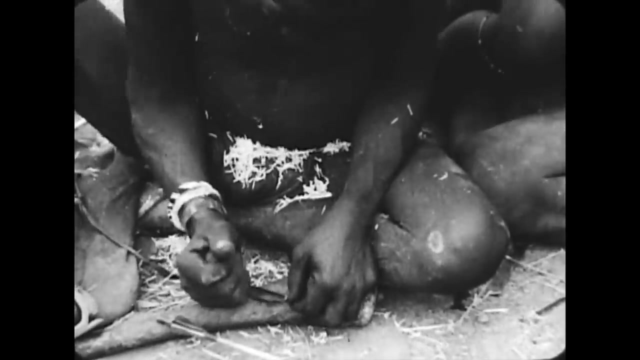 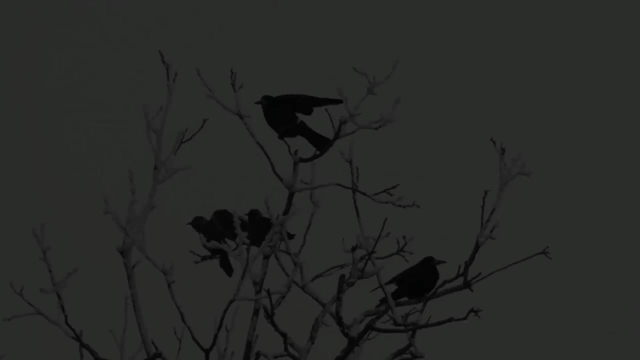 Ethnological studies of very unique groups such as the Kalahari and Mabuti Pygmies in the 1960s further complicated the picture as seeming to somehow represent all hunter-gatherer groups that have ever existed. The reality, as we have seen, is very different. 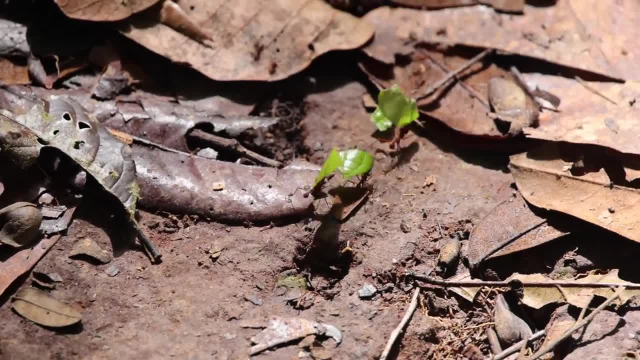 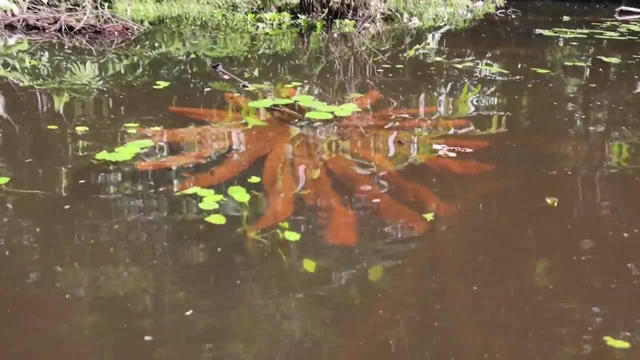 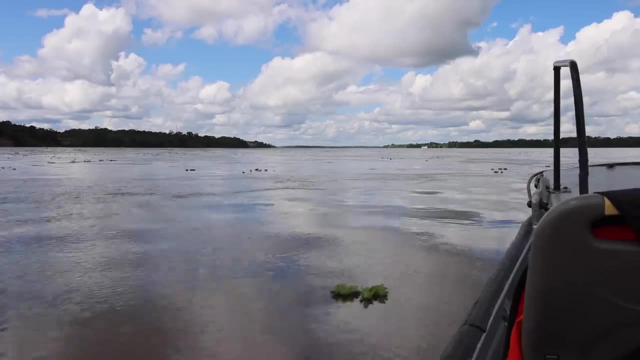 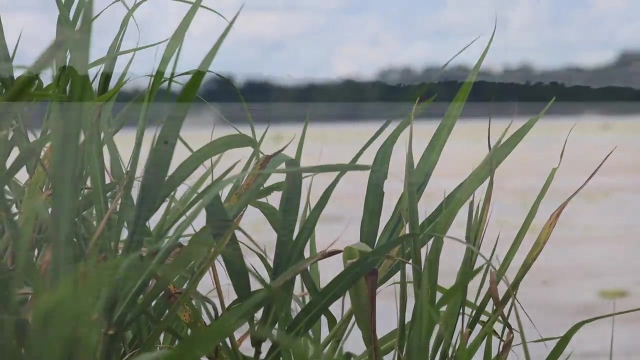 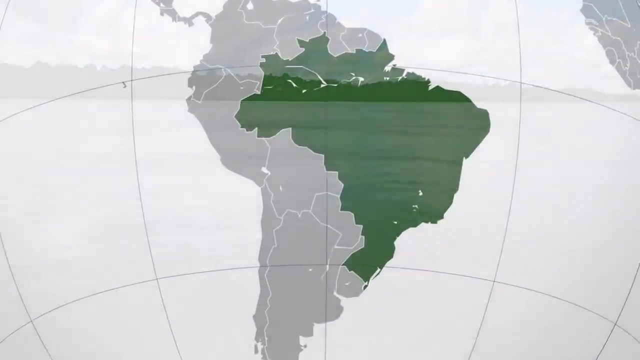 and much more varied and complex. Far away in the dense heart of the Amazon rainforest, anthropologists began studying another hunter-gatherer group to survive into the 20th century, Making their home deep in the Brazilian wilderness. The Nambicawara still regularly alternate. 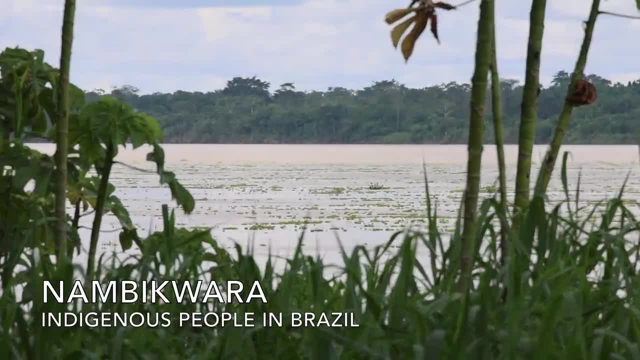 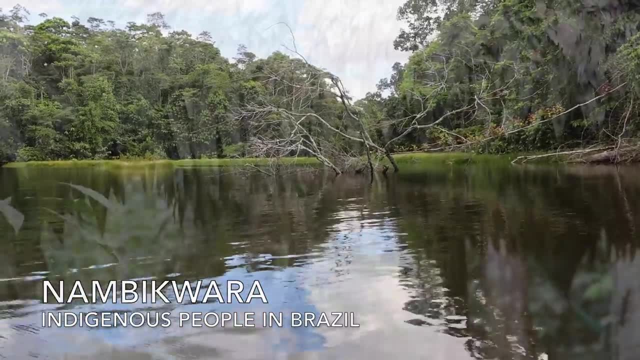 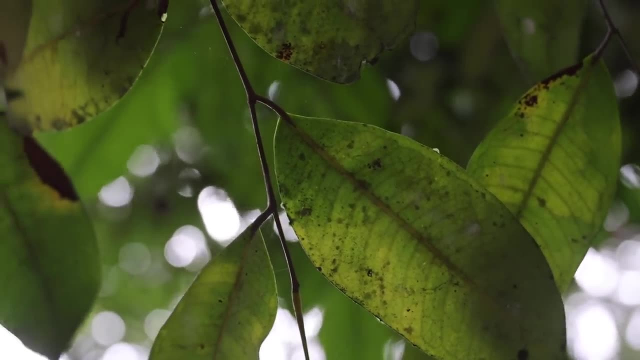 between densely settled villages in the wet season and wandering bands in the dry, Between strict hierarchies and loose egalitarianism, depending on which particular mode suits the current situation best. The reality, as we have seen, is that the Nambicawara are not only a group of hunters-gatherers. The reality, as we have seen, is that the Nambicawara are not only a group of hunters-gatherers. The reality, as we have seen, is that the Nambicawara are not only a group of hunters-gatherers. 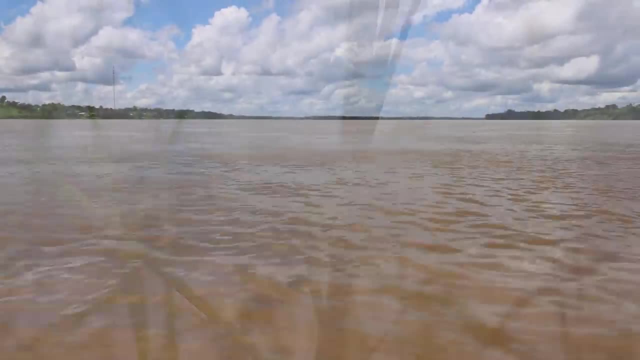 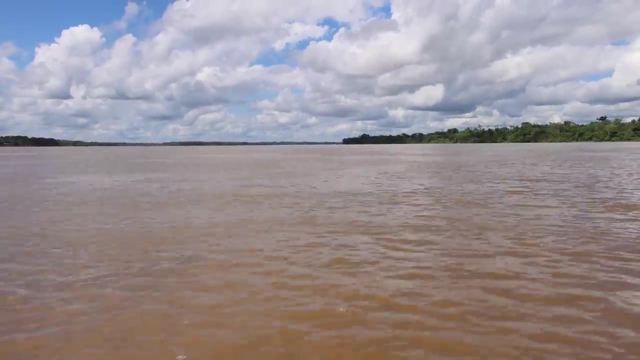 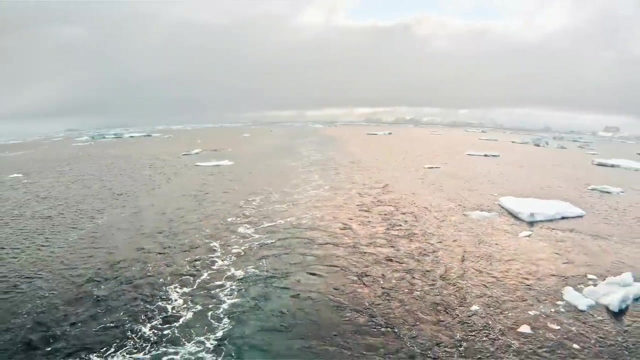 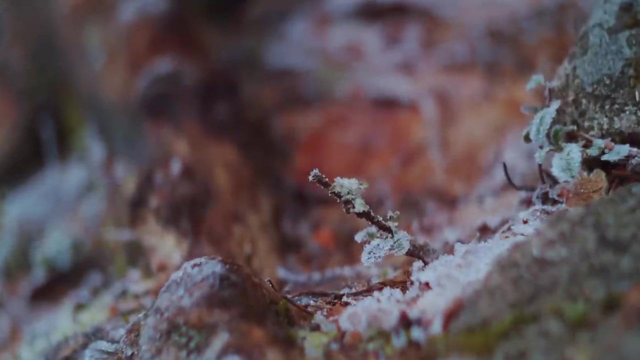 is that human culture is exceptionally malleable and human beings never simple. Let us now consider even earlier examples of organized communal sites and markers of complexity. For this we must go back even further Deep into the midst of the land of the last ice age. 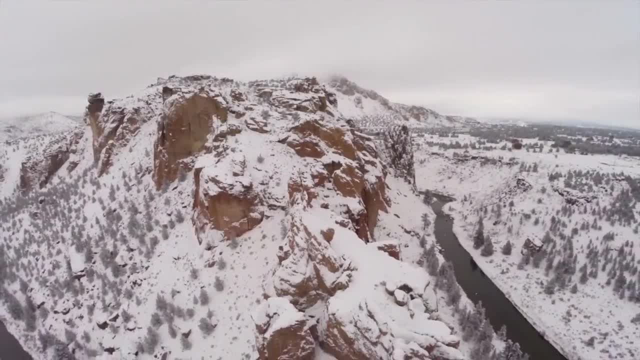 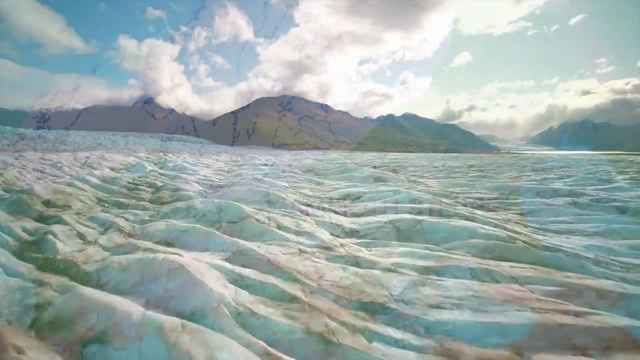 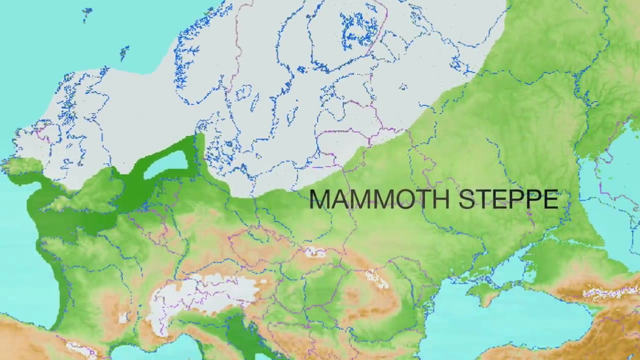 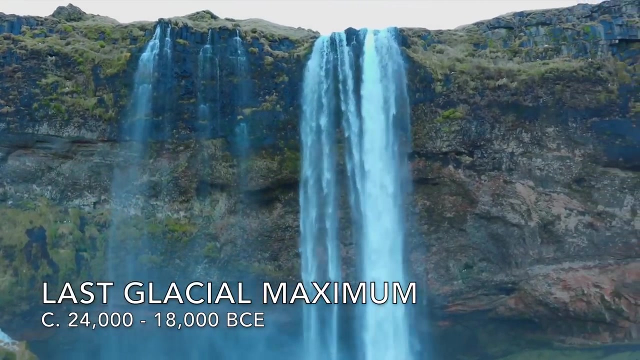 Around 25,000 years ago, in a wide arc from what is now Spain to the open steppe land of Siberia. an extraordinary flourishing of human culture took place In those millennia, just before the last glacial maximum, at the very height of the last cold period of the ice age. 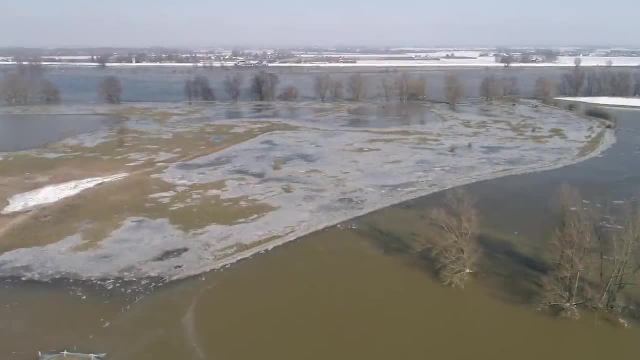 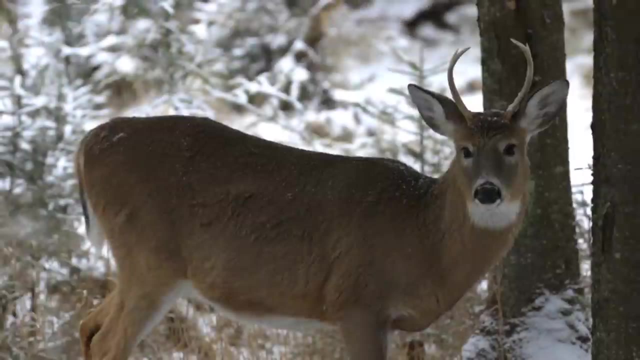 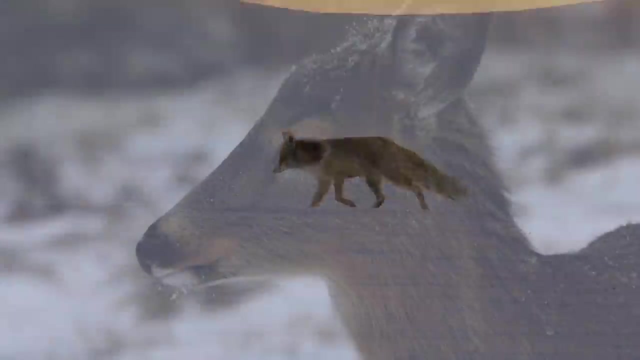 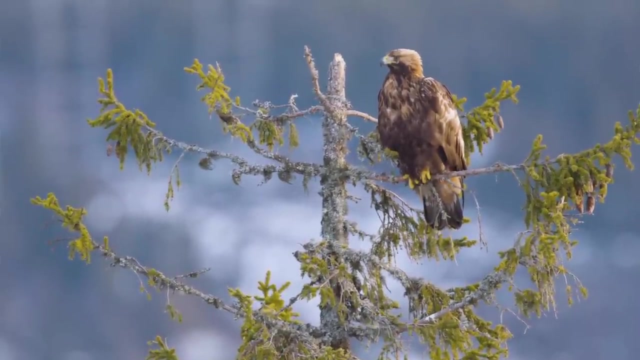 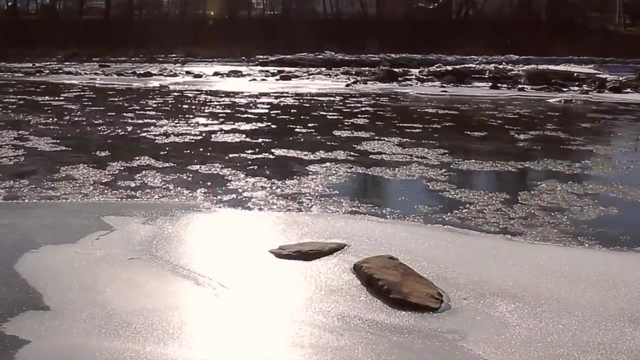 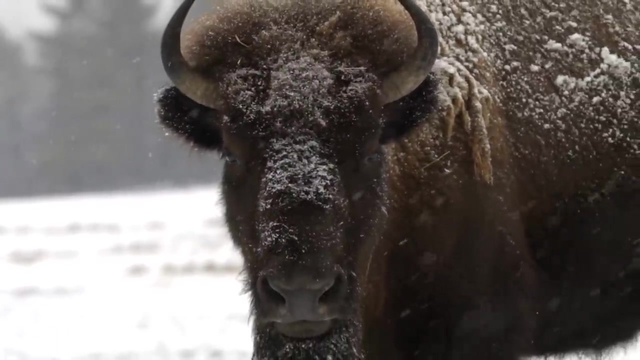 it was a world utterly unrecognizable to today, A world surprisingly full of life. In the summer months in particular, near never-ending seasonal parklands would open up along the river valleys and ahead of glaciers Populated by vast herds of migrating bison deer. 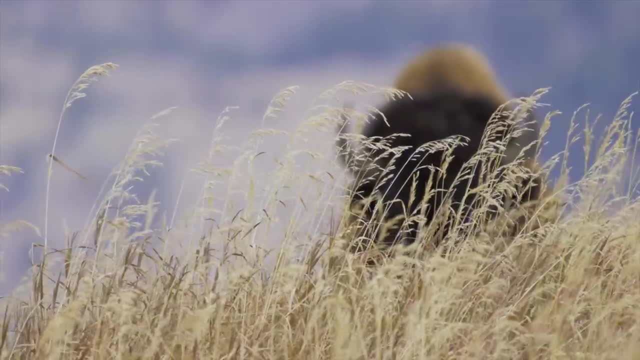 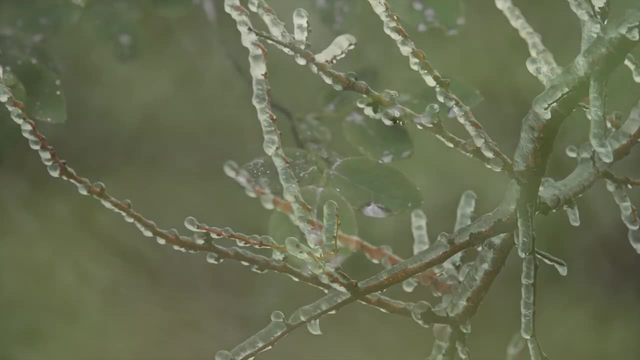 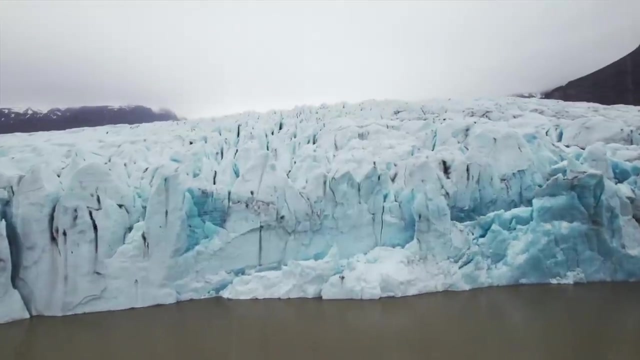 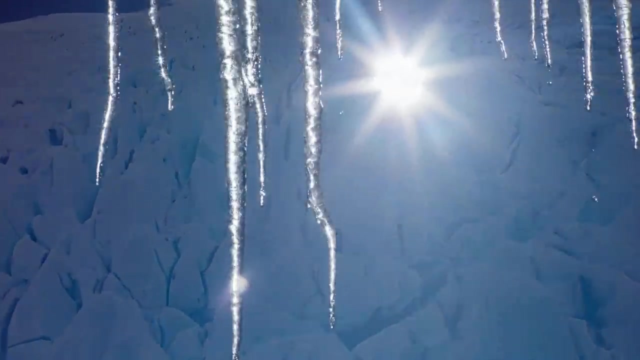 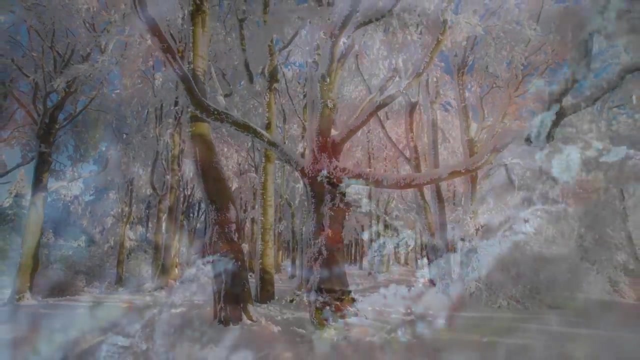 and a wide variety of megafauna, much of which is now extinct. Moments of calm amidst the brutal, unforgiving cold. Of course, one of those creatures is much more famous than the rest: The largest of all and absolutely vital to the survival of humanity. 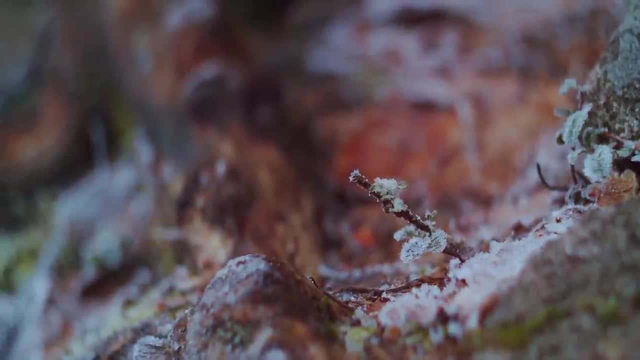 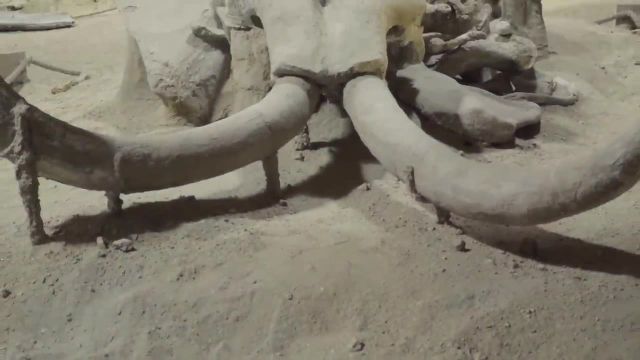 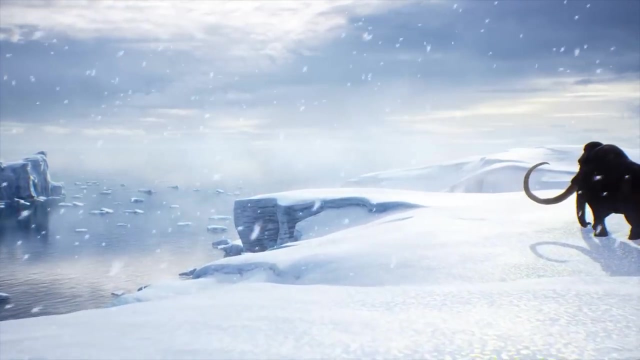 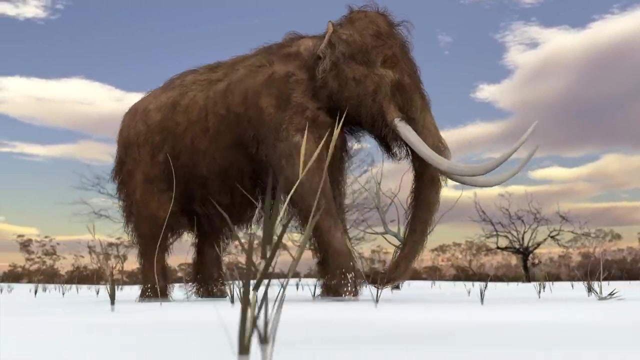 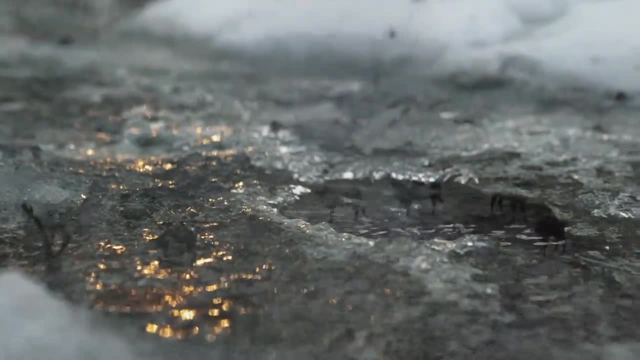 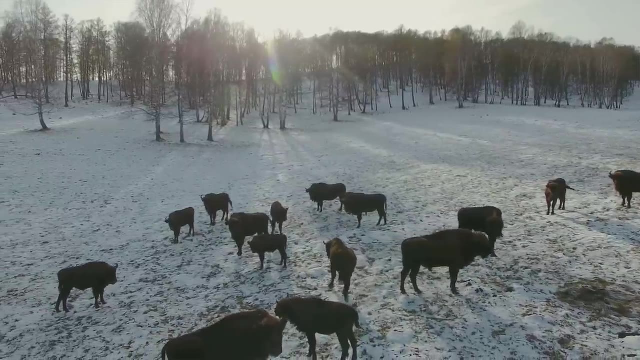 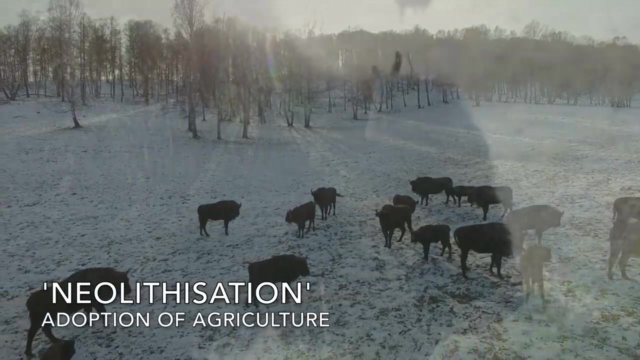 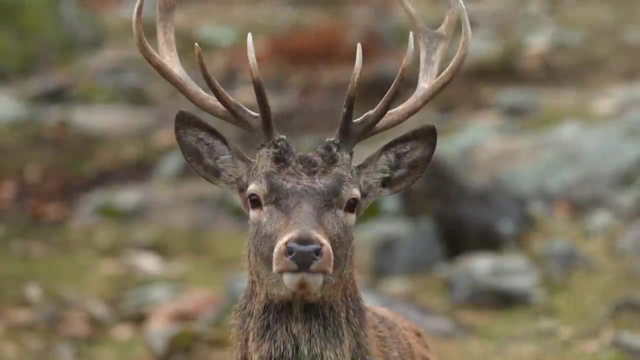 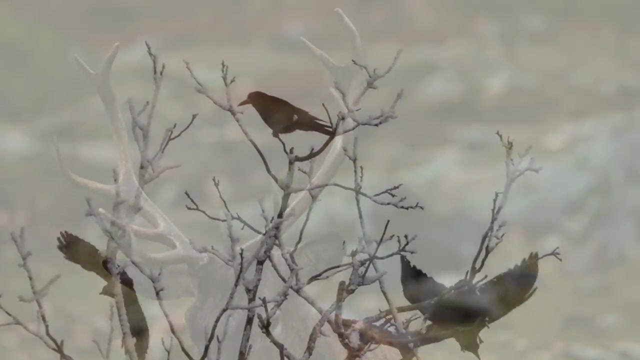 of vast river valleys and colossal herds. some of the earliest evidence of human sedentism and even very early tenets of so-called Neolithicisation have been found: Modest clans and tribes sheltered in the life-filled pockets, filled pockets between tundra and forest zones. 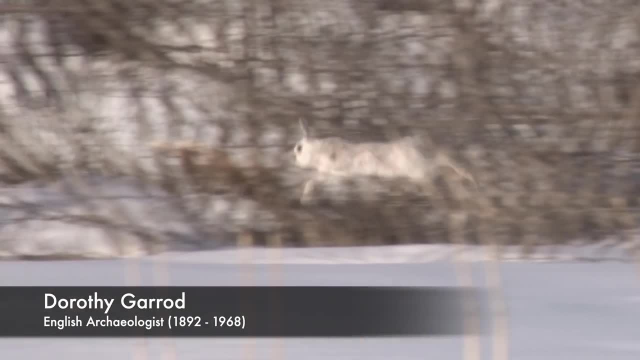 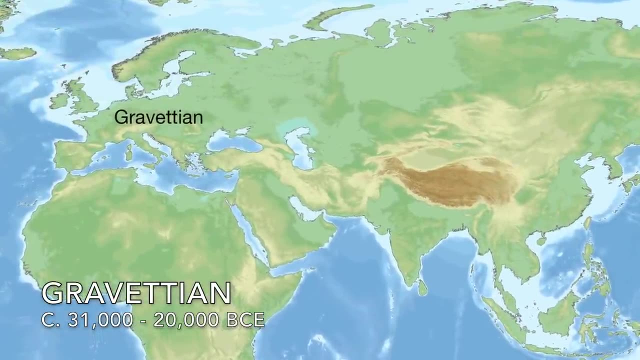 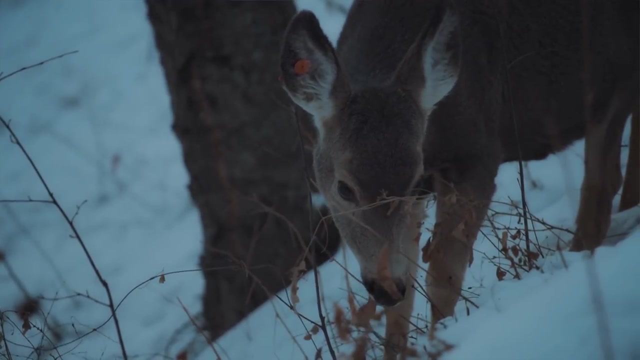 First defined by Dorothy Garrett in the 1930s. the archaeological culture we know today as Gravettian lasted for over 10,000 years in that bitterly harsh environment. Just as much time from Gobekli Tepe to today. 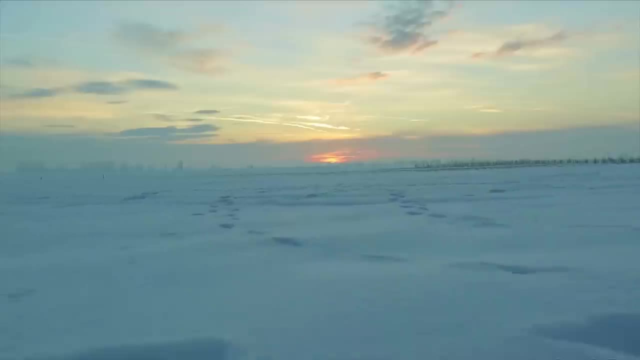 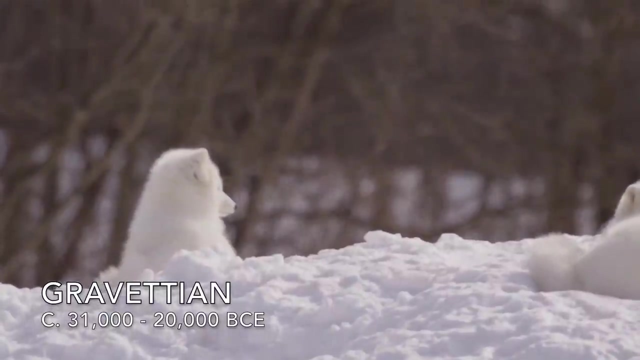 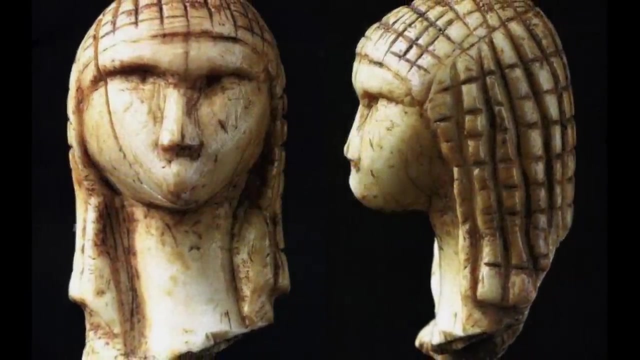 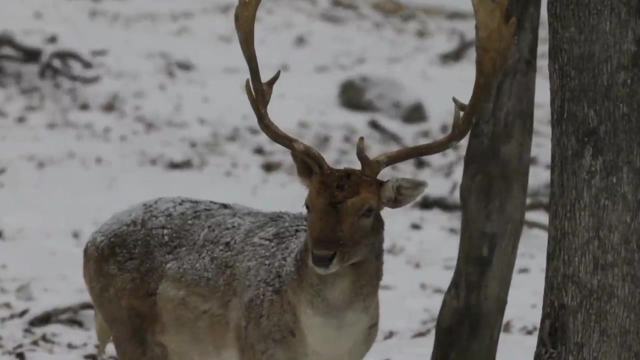 And yet, though, today, the image of a perennial struggle to survive for our Ice Age ancestors is fixed in the public imagination, this was clearly not always the case. The Gravettians spent significant amounts of energy in creating art, Almost all of which is lost. 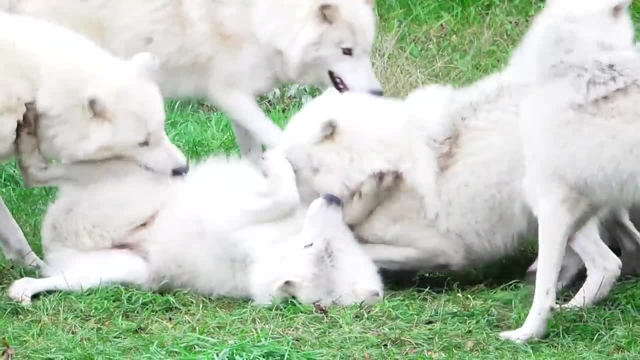 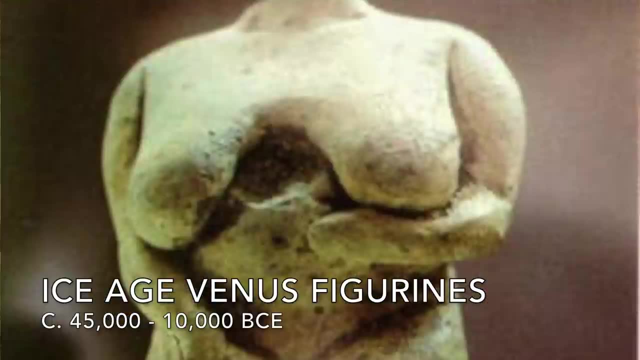 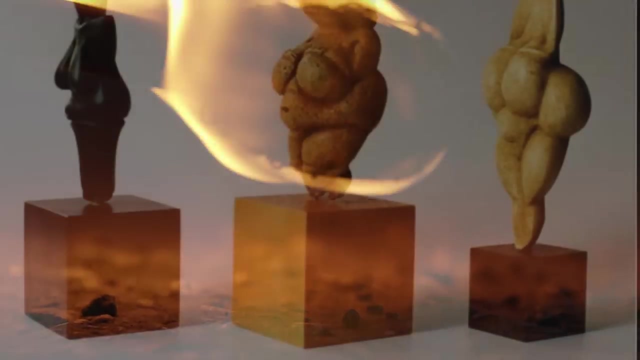 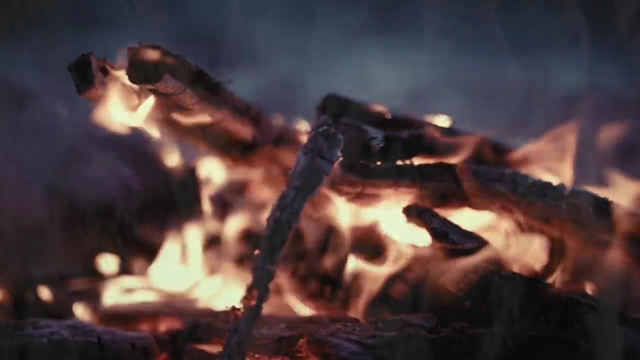 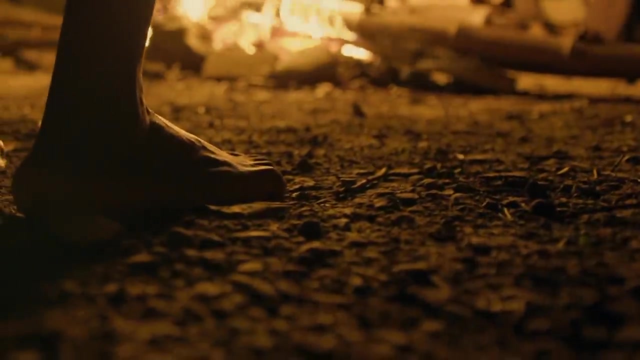 Though the famous Venus figurines, over a hundred of which are known, give some small hint of the lives of these people Arrival for the very first time, beginning to live in settled, long-lasting communities, The Eastern variant of the Gravetian, nestled in the Pavlovian hills of southern Moravia. 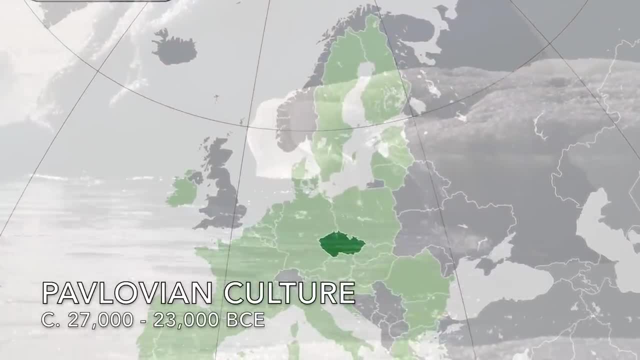 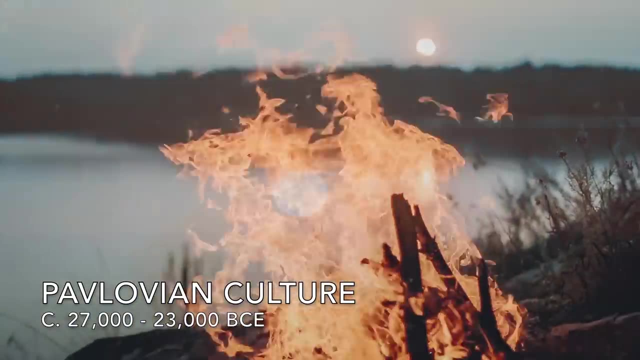 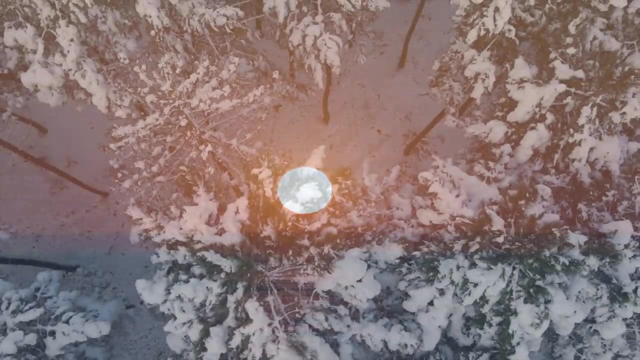 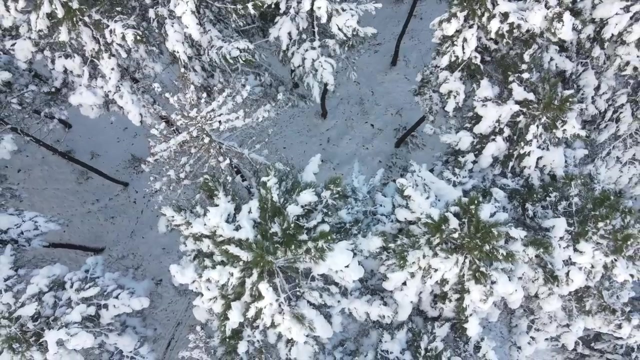 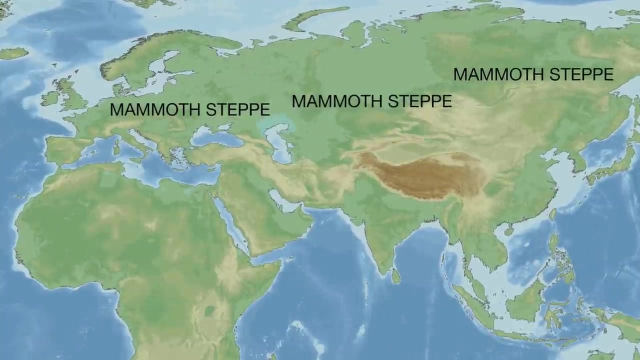 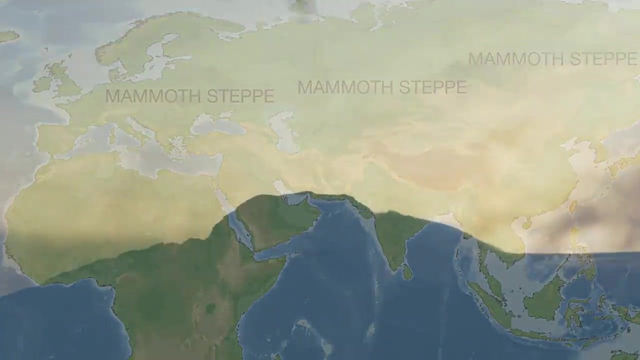 also lived settled lives, but here they did so in vast open-air settlements, the remains of which have survived to the present. Though multitudes exist in a rich archaeological landscape stretching far out into what is now the plains of the Brescia of Russia, One of the most famous and important is, in the modern day Czech Republic: Its name. 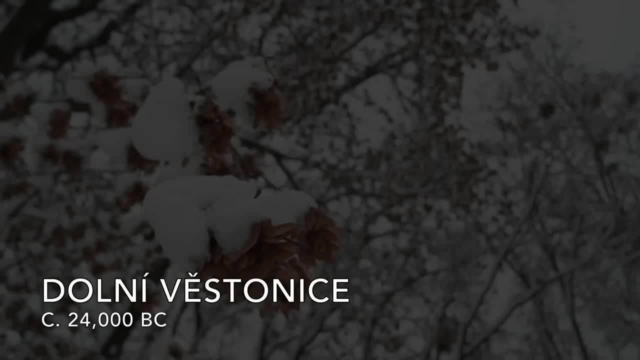 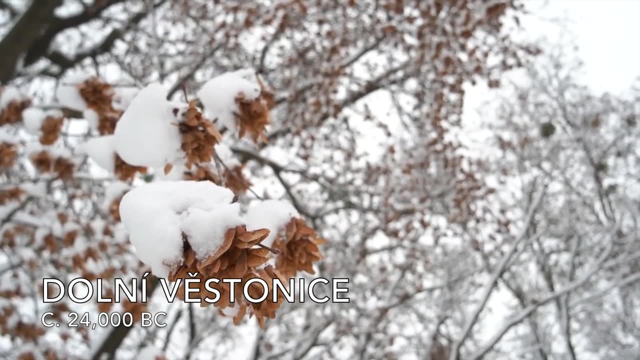 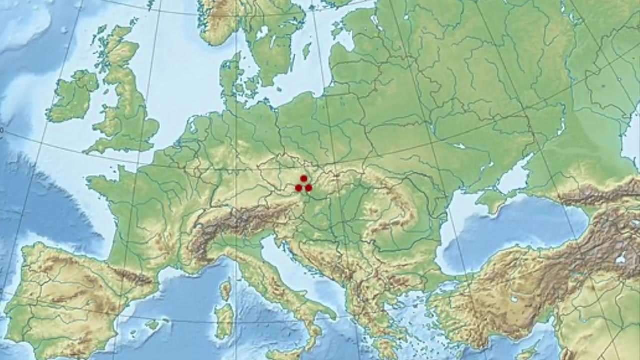 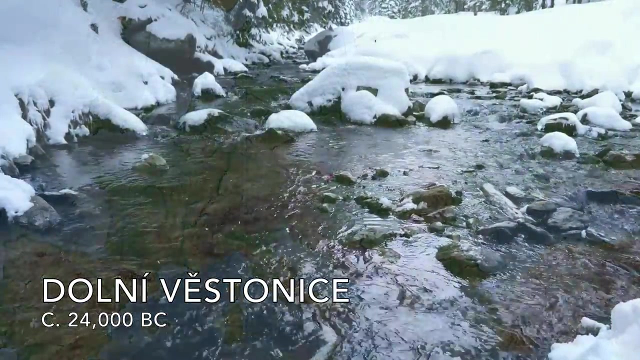 is Dolny Vesta Nietzsche, and it is in this region that we get not just some of the first evidence for large settlements in the world, but of burials too. Dolny Vesta Nietzsche is an impressive sight In the midst of a mighty perimeter fence of. 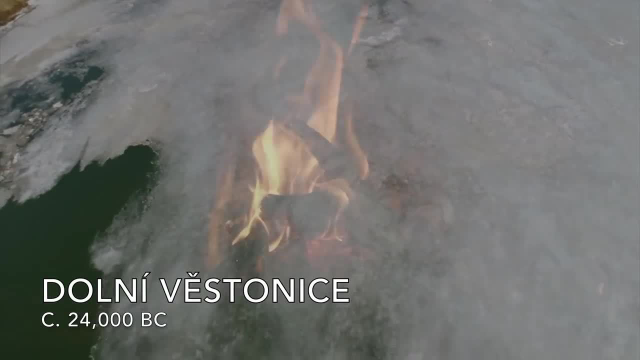 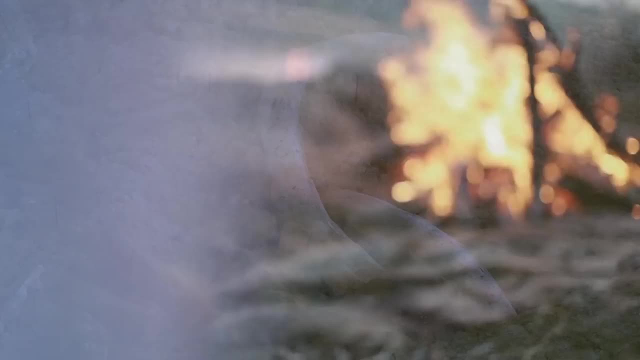 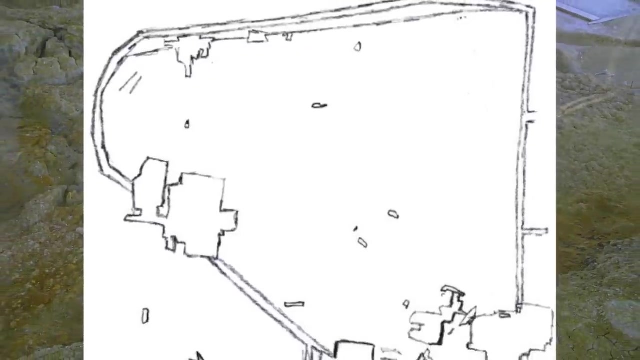 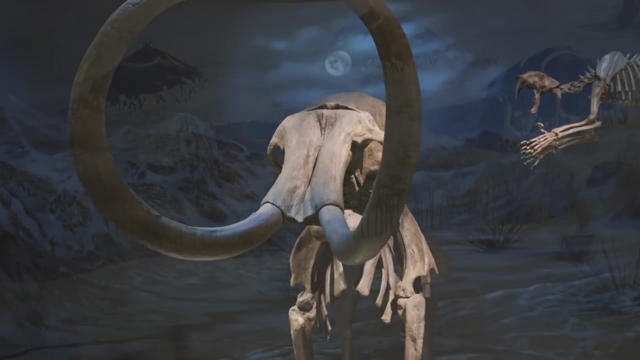 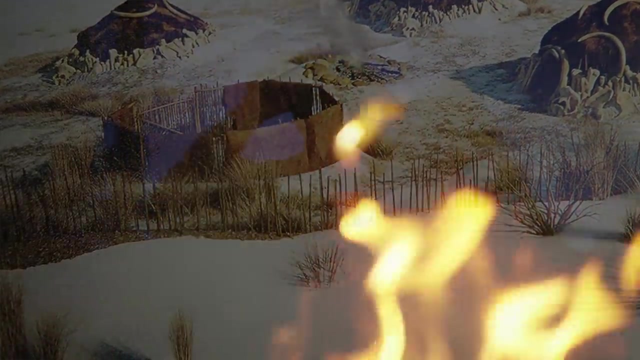 mammoth bone, a massive bonfire burned, Surrounded by elaborately built circular structures also made of mammoth bone, likely covered in skins and hide rendering. Within the perimeter fence, an abundance of artistic depictions of humans and animals have been found, alongside significant evidence of vegetal 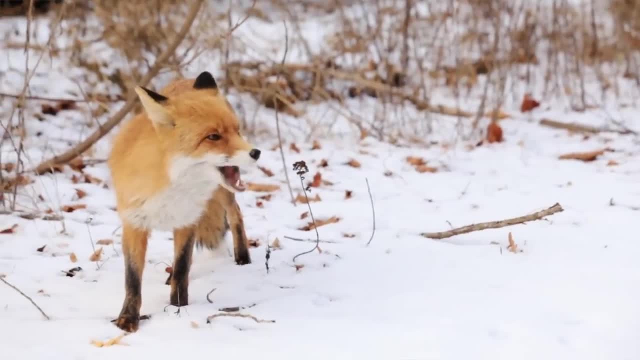 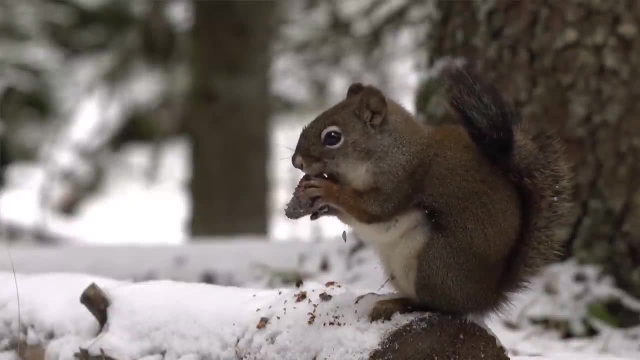 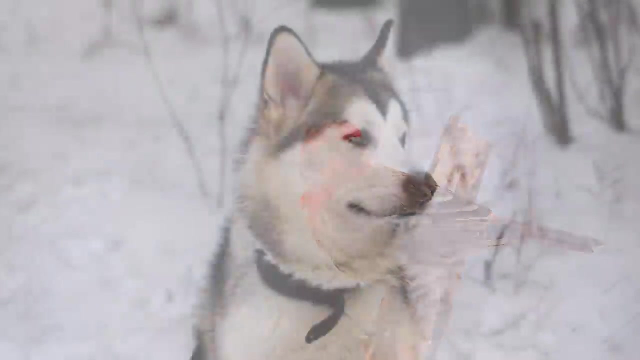 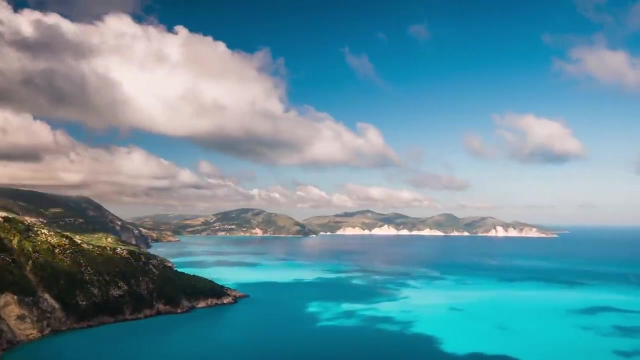 remains too, And all manner of smaller animals caught in nets. Also, inside the enclosure, alongside an abundance of art and symbolism, is found not only the earliest evidence of weaving found anywhere, but shells originating in the distant Mediterranean, Evidence of far reaching contacts. 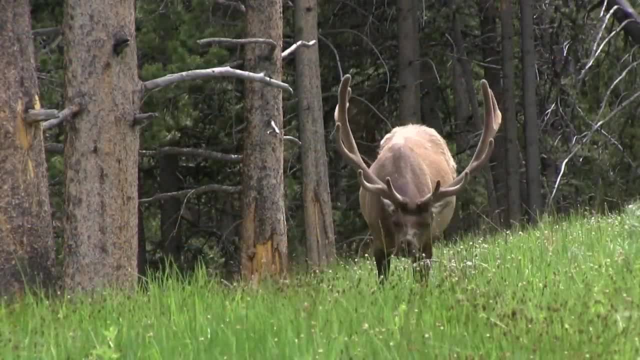 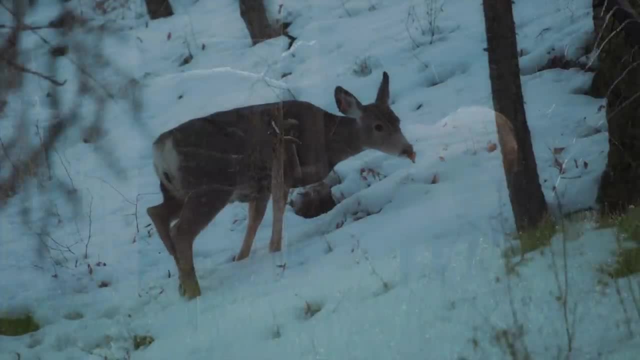 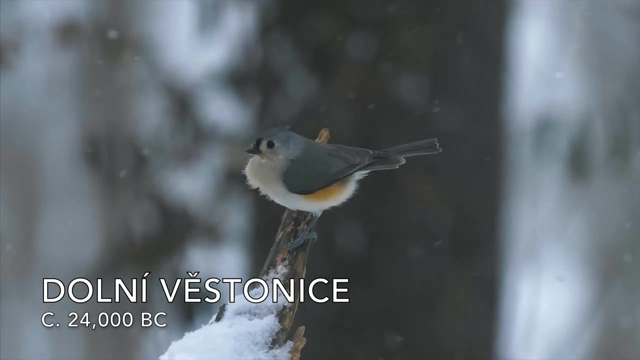 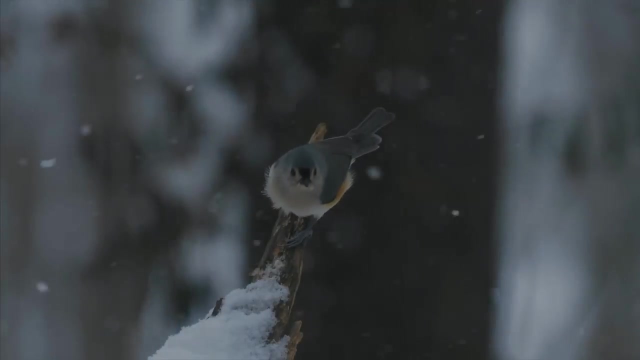 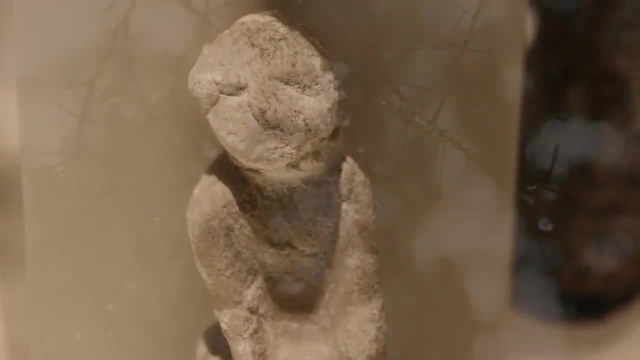 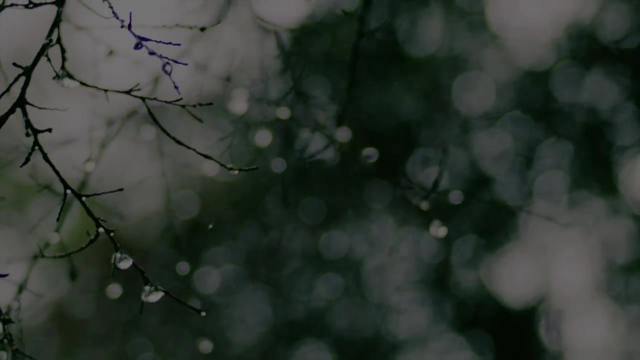 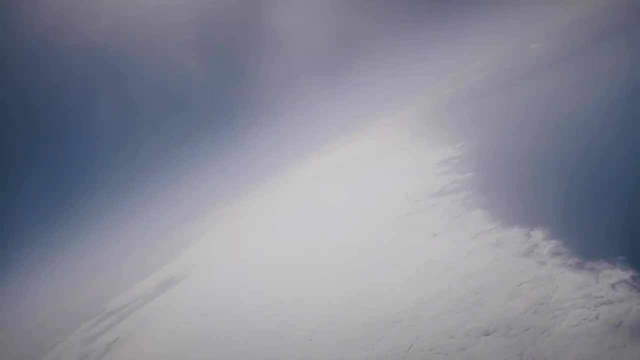 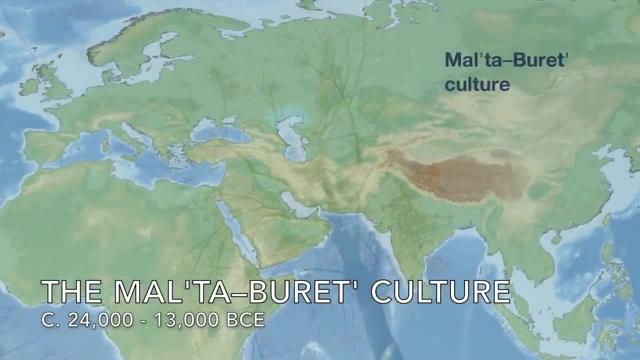 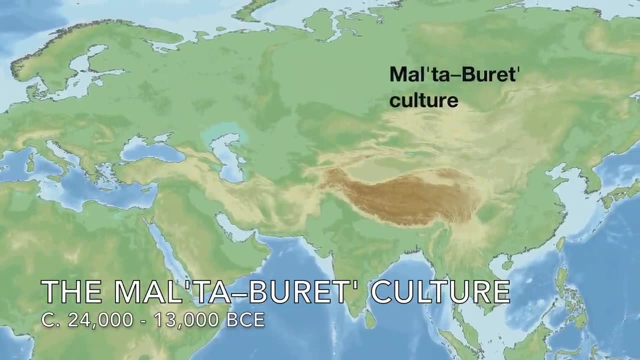 Also living in massive mammoth bones structures in the open air And also spending significant money angling the ashes of living animals. A combination of both in a single condition, with the very important design, significant energy in the creation of artistic works. it is at sites like this: 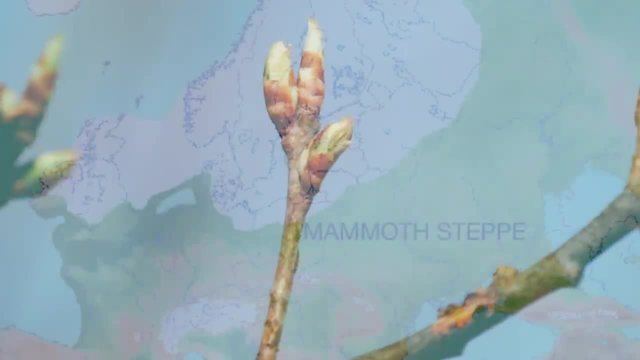 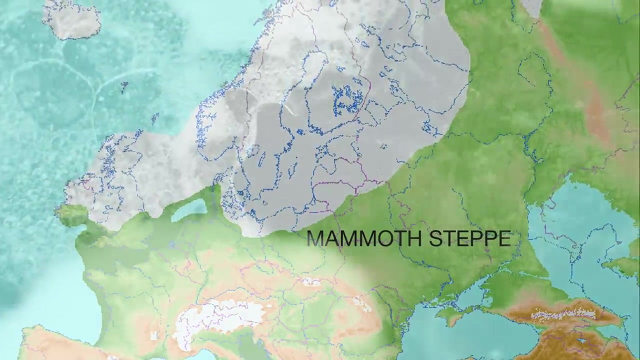 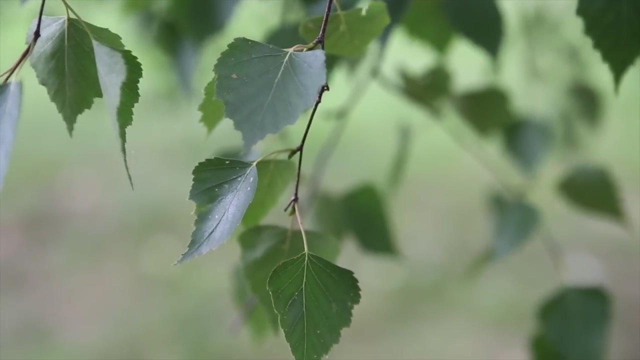 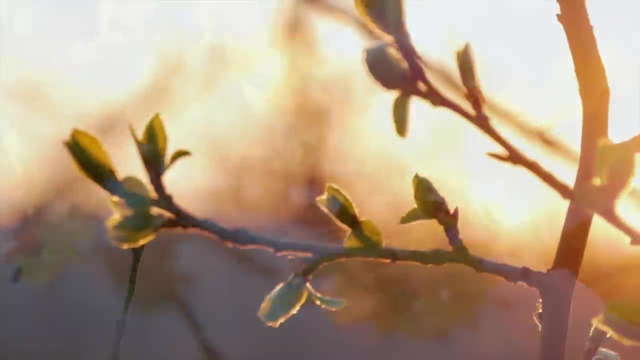 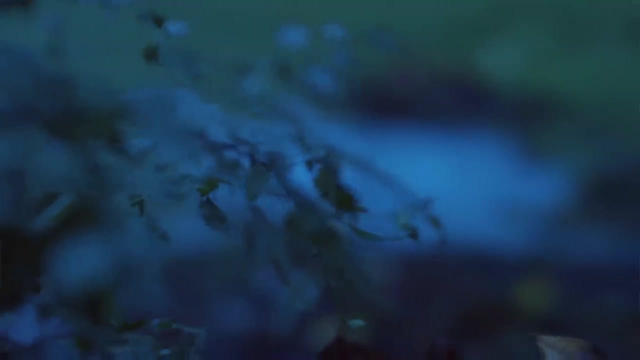 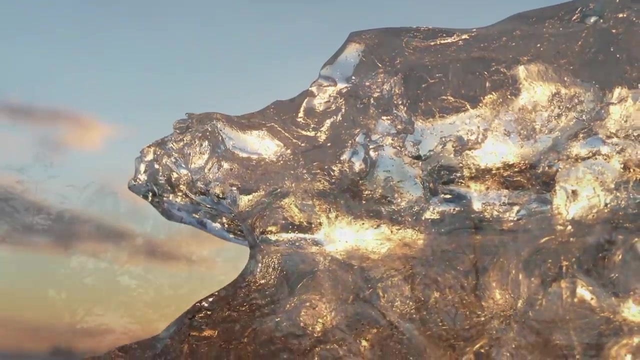 from as early as around 25,000 years ago. the several innovations appear to suggest burgeoning movements toward the harnessing of agriculture. the great human experiment in full force, though, as we know, now perched in an environment particularly susceptible to environmental change. the odds were stacked up against them, and those 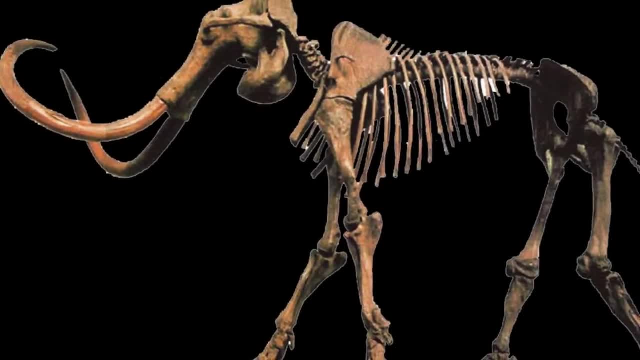 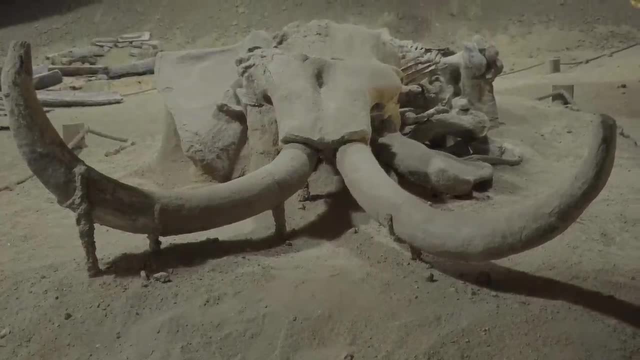 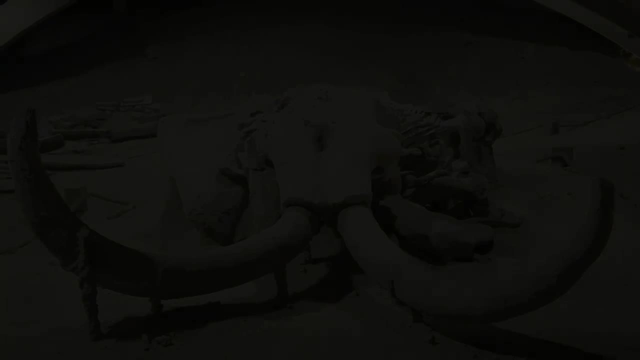 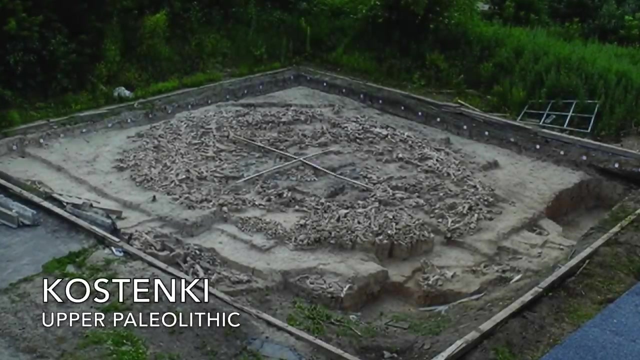 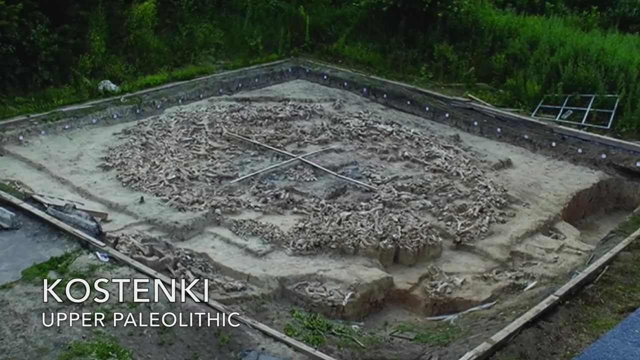 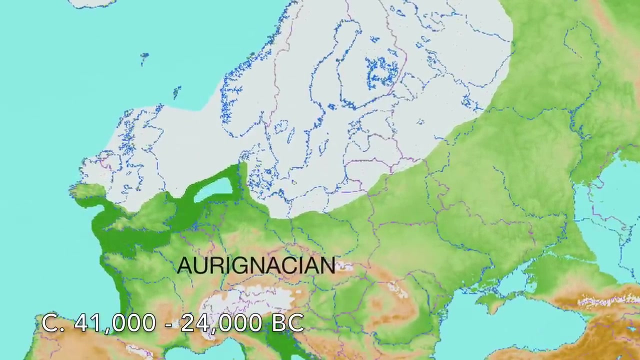 mammoth structures themselves, as we shall see, could often be much larger, sometimes being referred to as monumental. at Kaustenko in Russia, a recently discovered example of megalithic mammoth bone architecture has been uncovered, originating and the Aurignacian period of around 40,000 years ago. this site shows signs of an impressively 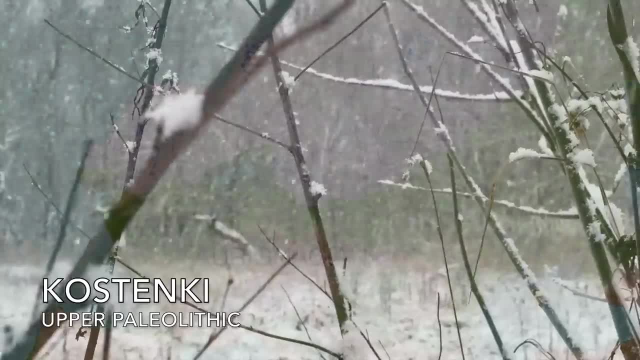 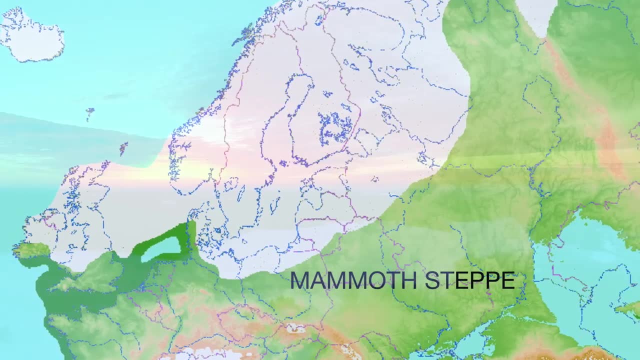 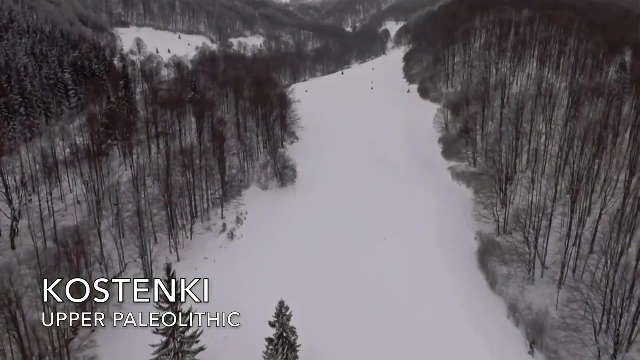 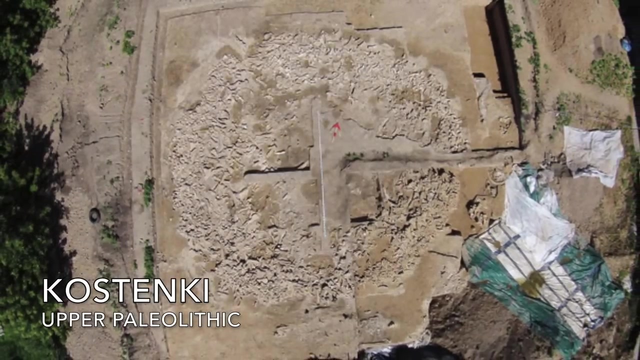 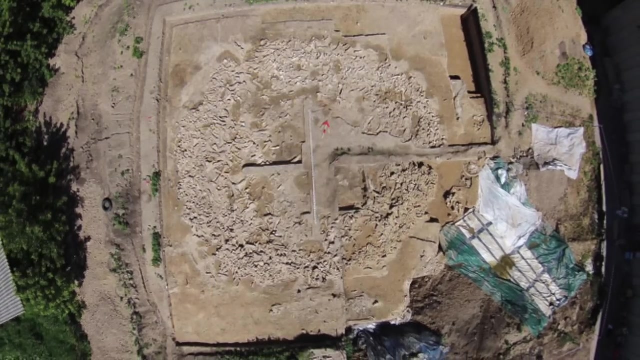 lengthy series of habitations from then onwards in just one find within an astonishing archaeological landscape In around 23,000 BC, the remains of at least 60 mammoths had been arrayed into a massive circular structure over 12 meters in diameter. It is quite simply one of the most impressive. 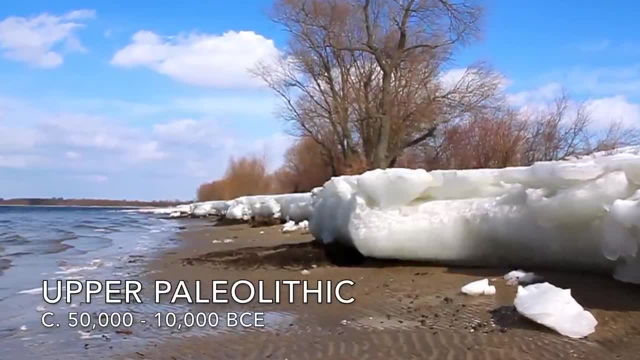 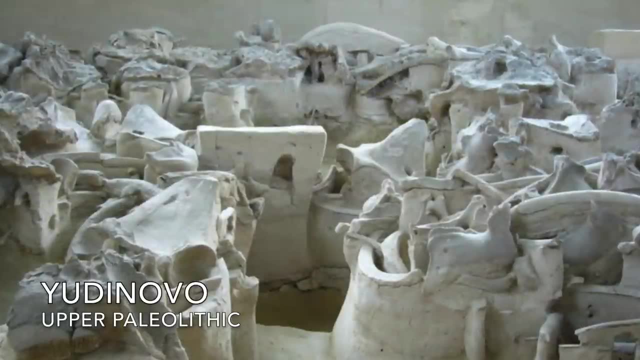 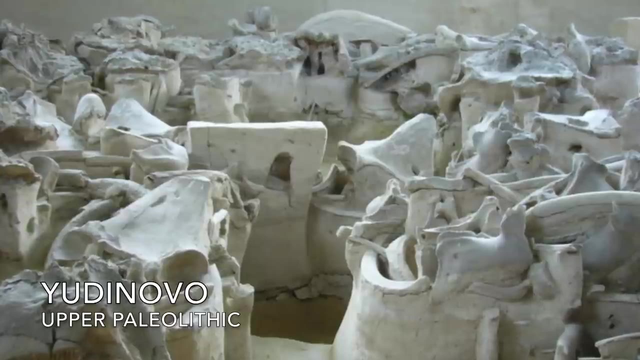 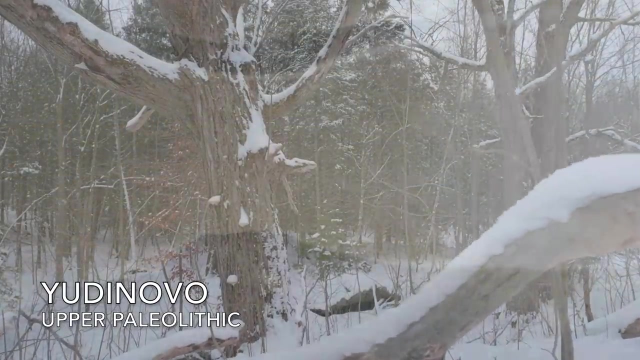 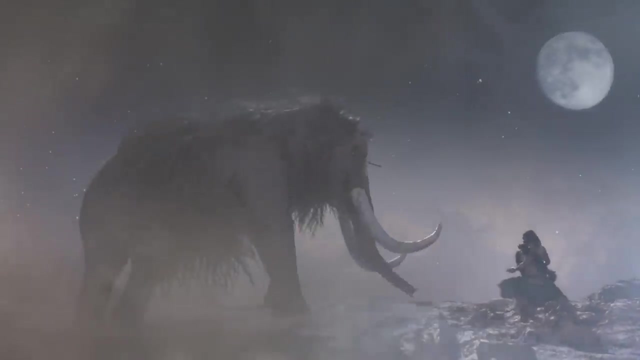 Paleolithic finds ever made. Research at another Russian site, Udenovo, suggests that these so-called mammoth houses may not in fact have been dwelling there, But carefully planned and built to commemorate a great mammoth hunt, the meat, hides and bones of which must have created a sizeable surplus for the community. 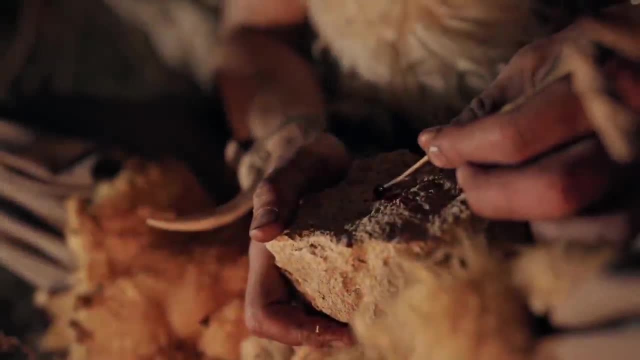 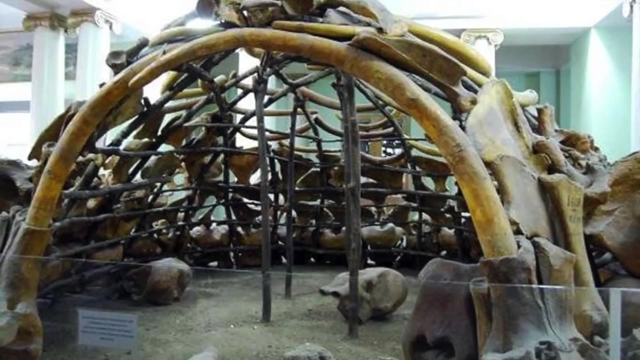 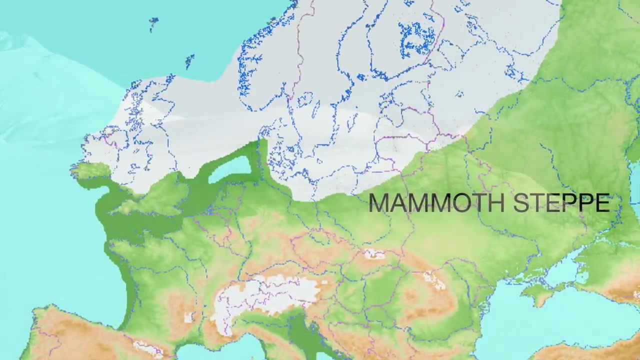 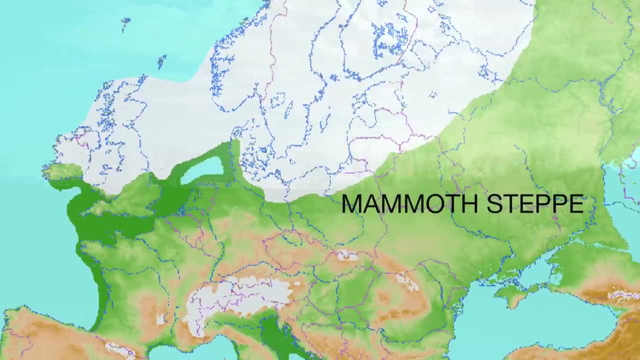 Which also undertook artistic endeavours and exchanged animal pelts, amber and seashells over great distances. It all begs the question: could sites like Dolni Vestanice, Kostenki and Udenovo have been seasonal congregation places where people came together annually to trade? 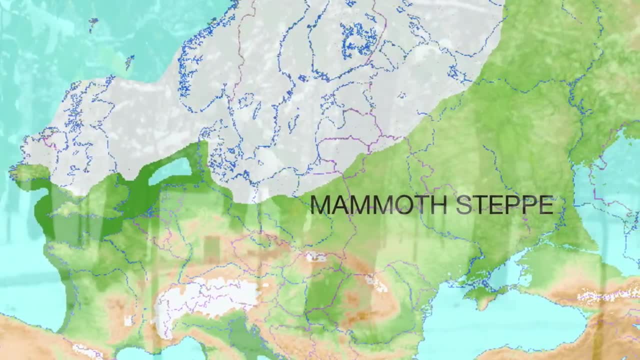 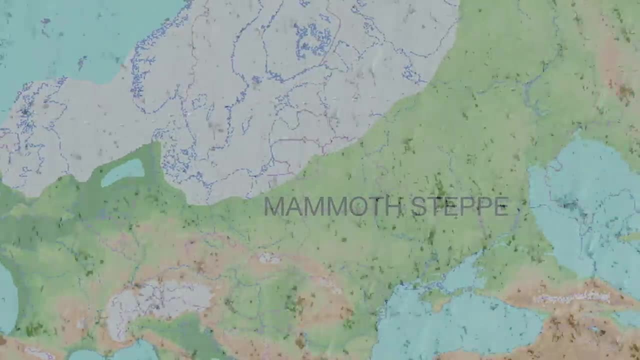 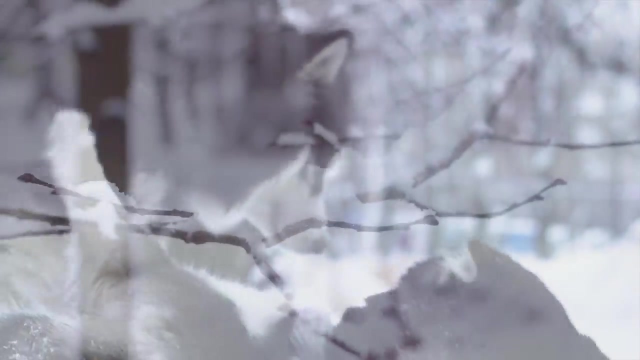 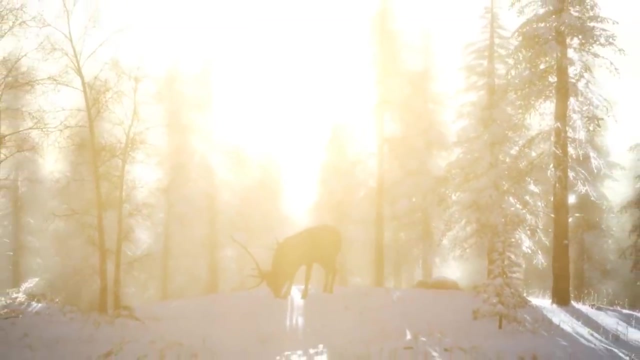 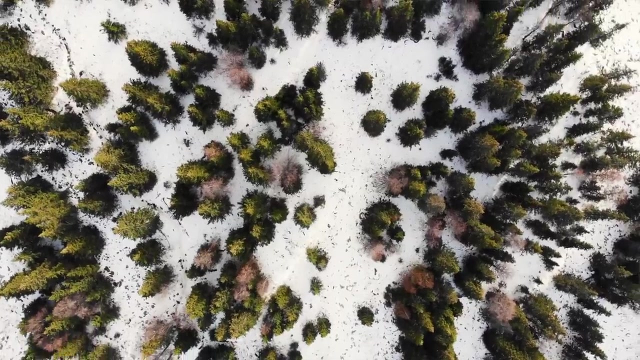 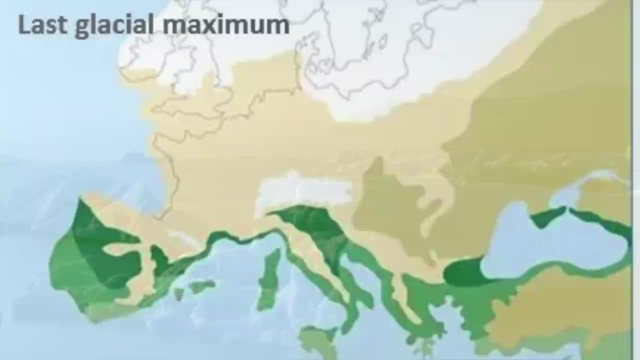 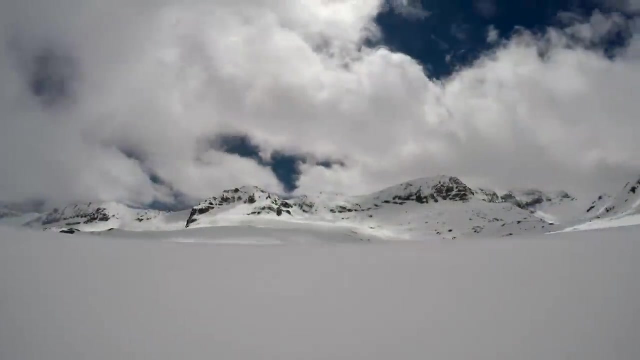 elaborate monuments and artistic works, Just maybe an early form of Gobekli Tepe. The only constant in those days was change, And before it could fully develop into fruition, the lifestyle of the mammoth hunters was extinguished In the wake of advancing ice sheets rolling down from the north. 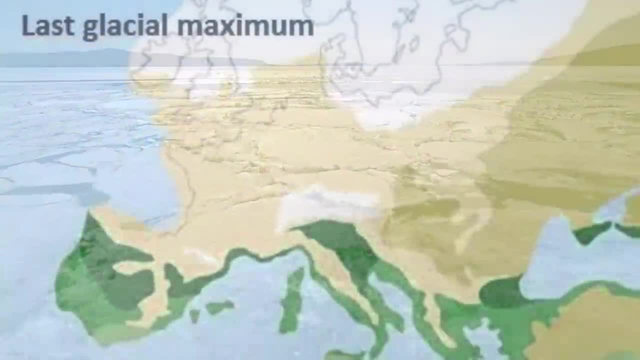 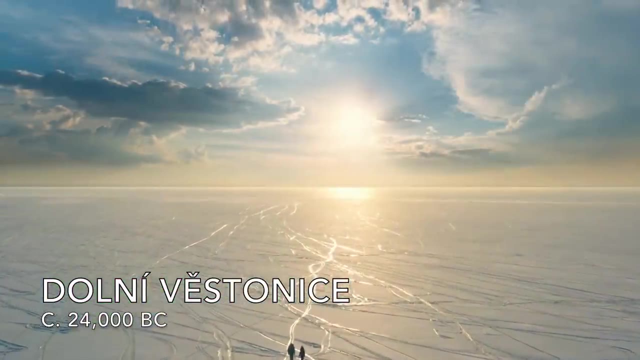 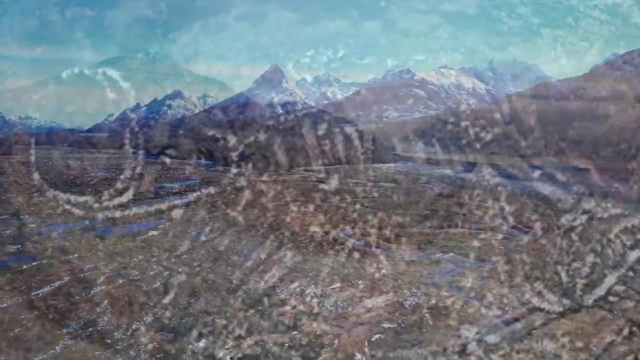 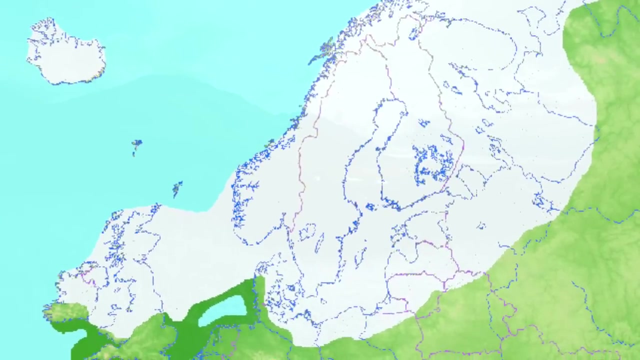 to the last glacial maximum of around 20,000 years ago. Dolni Vestanice and many other sites like it were abandoned, Their people forced to move ever southwards to escape the certain death of the permafrost By around 18,000 BC. however. 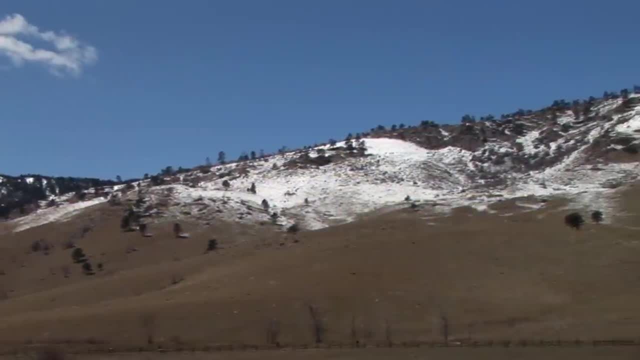 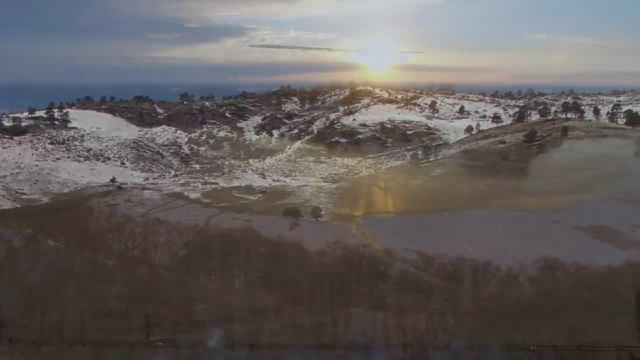 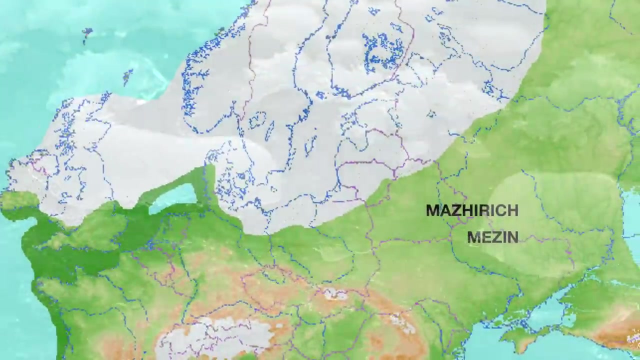 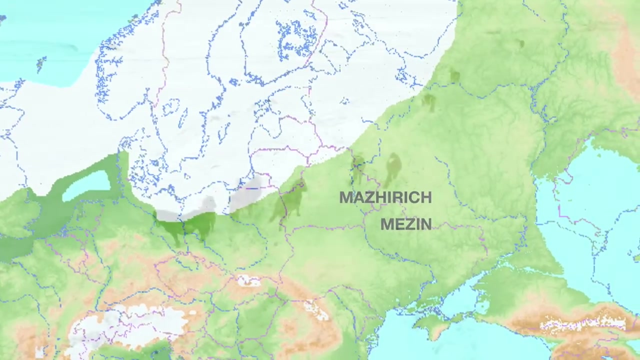 permanent settlements of considerable scale once again began to form in areas particularly abundant in life At the sites of Mezin and Mazarych in northern Ukraine, found on the banks of major river systems, where the annual north-south migrations of horses, reindeer, bison and mammoth could easily be hunted. 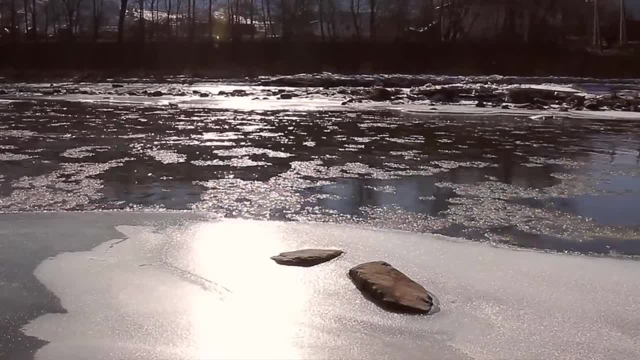 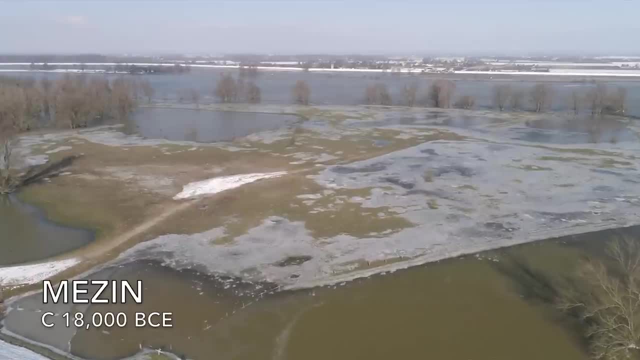 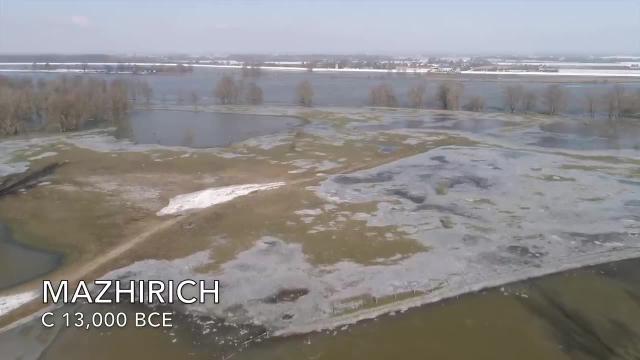 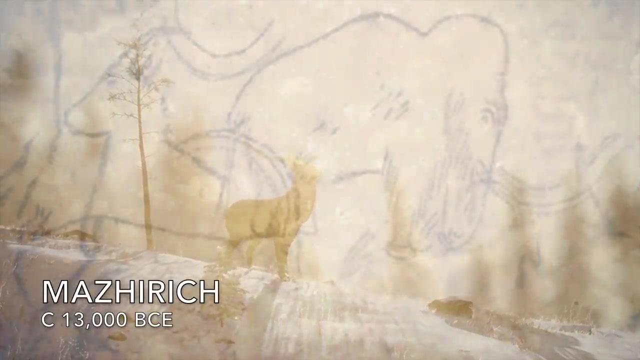 spectacular permanent mammoth bone structures again became the norm, Dating to around 18,000 and 13,000 BC respectively. this was the age of a second apogee for the settled complex hunter-gatherers of the mammoth steppe. 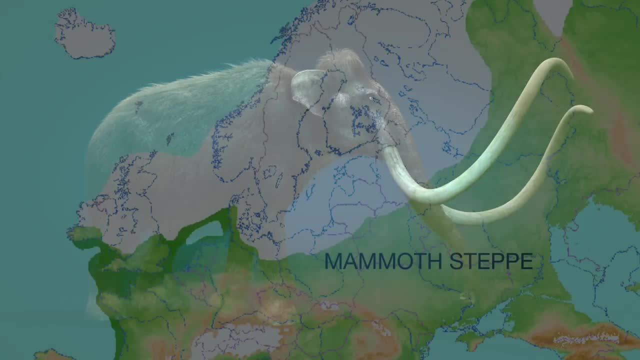 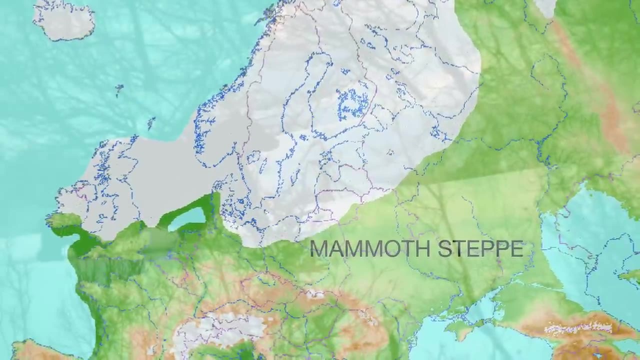 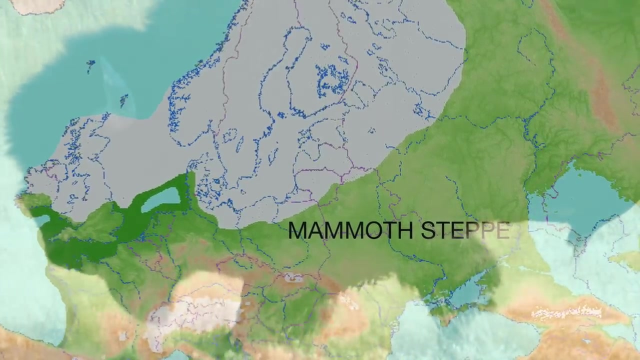 Especially in the regions in what is now the Russian Plain and in Eastern Europe. Again, heavy stone industry, artistic flourishes, the separation of domestic spaces from those considered to be ceremonial, carefully curated burials and the importance of vegetal food can be found. 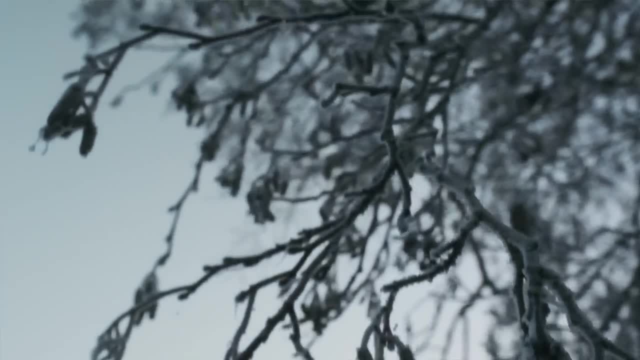 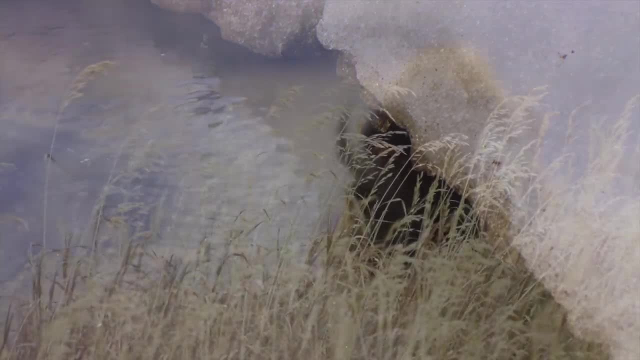 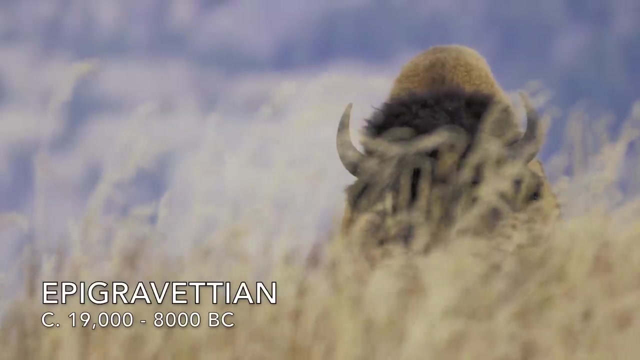 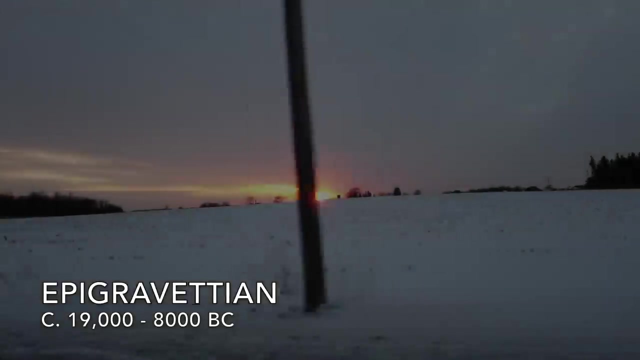 And, of course, most impressively solid and very large, elaborately made structures built of mammoth bones. Today we call this era the Epi-Gravettian, During those millennia from around 16,000 to 10,000 BC. 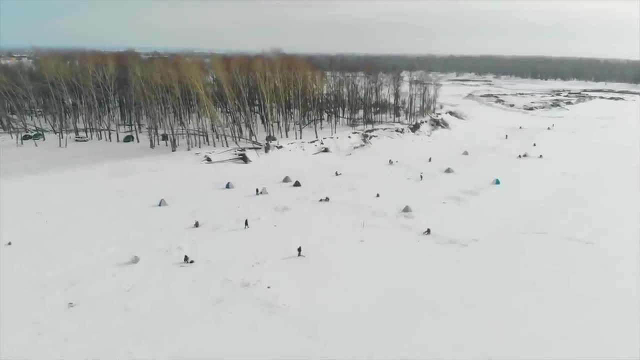 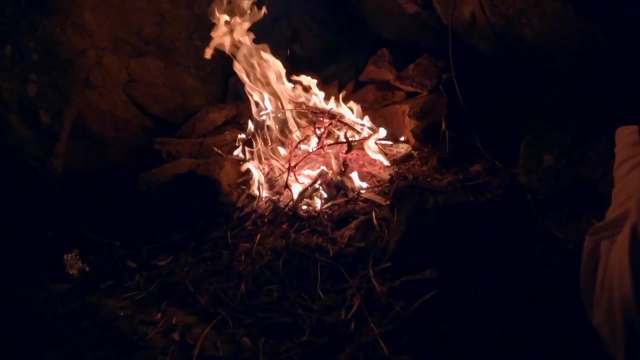 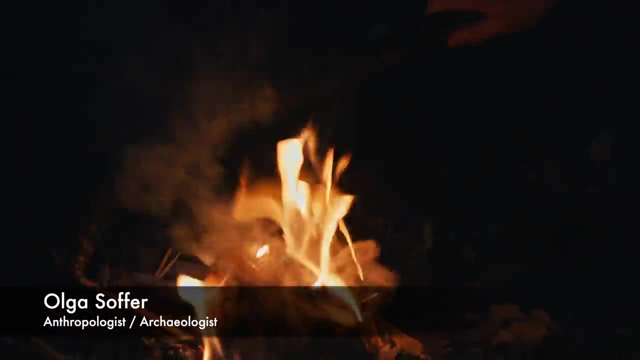 in a great arc from Krakow to Moscow. people again lived permanently in impressive circular houses of mammoth, tusk and bone, Described by anthropologist Olga Sofa as Pleistocene public works. many of them go far beyond the needs of domesticity. 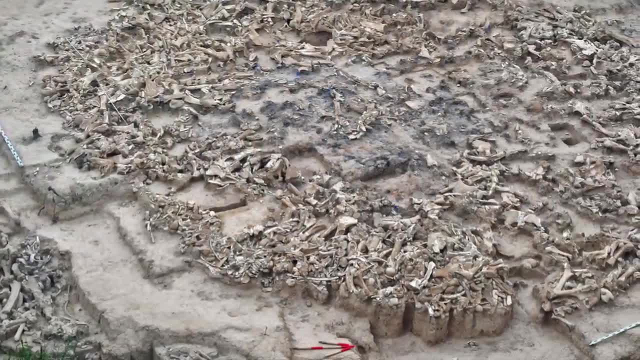 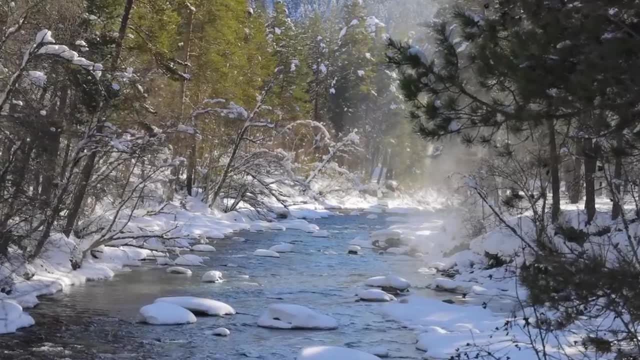 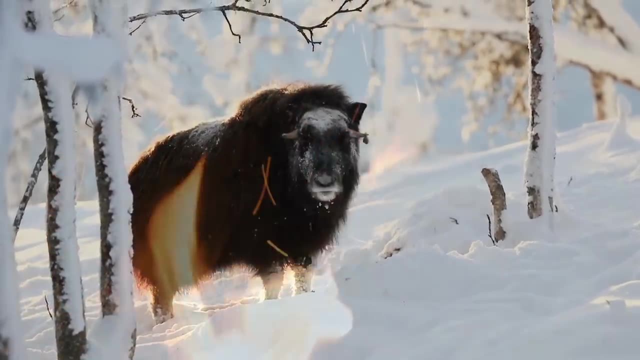 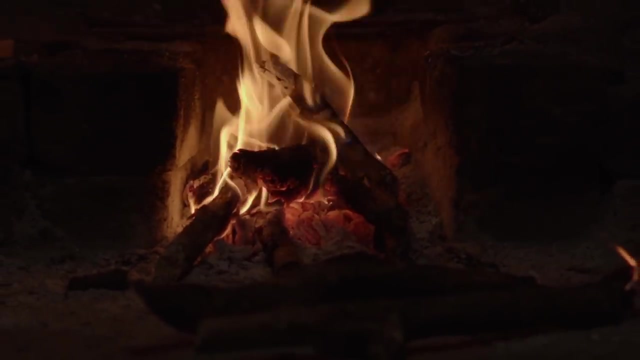 arrayed in rhythmic patterns that swirl artistically. What happened inside remains a mystery, but is often theorized to be, at least in part, of a ritual nature. Again, we must ask the question: are these the prototypes for the sunken temples of Gobekli Tepe? 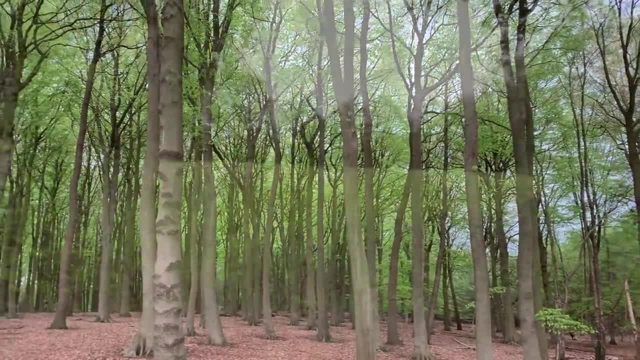 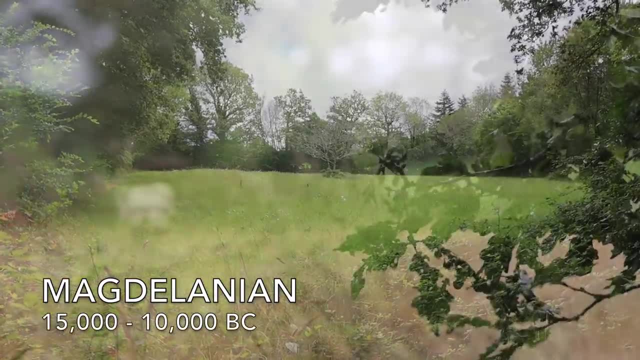 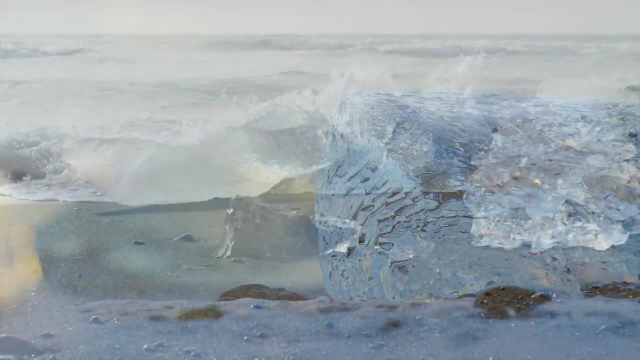 In Western Europe too, in the land of the cave painters, an archaeological culture we know today as the Magdalenian. the world was also changing By around 15,000 BC, as the ice finally withheld its hold on the continent for good. 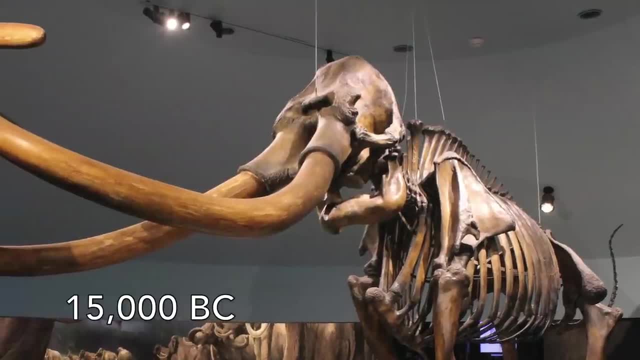 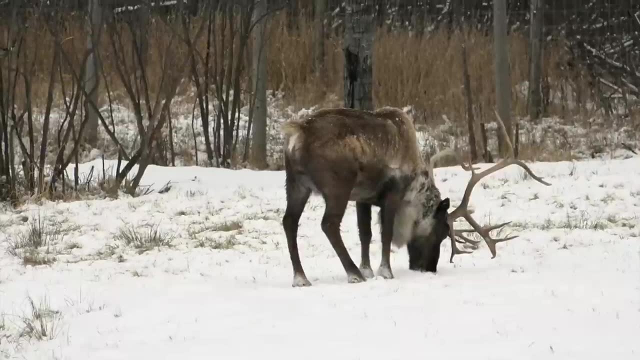 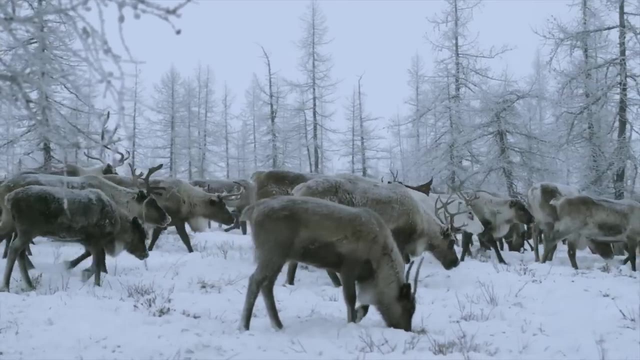 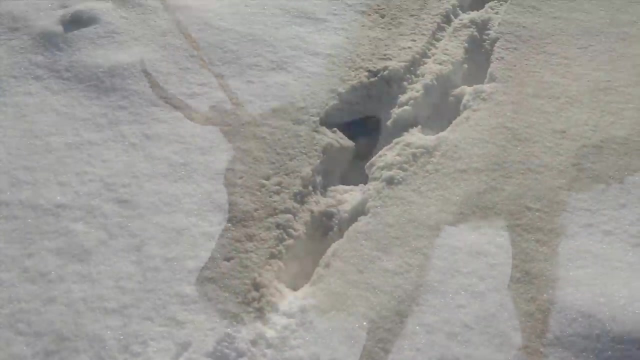 the days of the woolly mammoth were numbered. In its place came an abundance of reindeer. The epic, wide-roaming seasonal migrations of these sub-Arctic animals might not seem conducive to a semi-settled way of life for those following them. 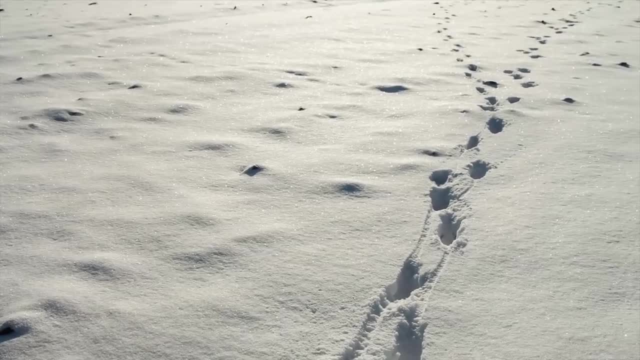 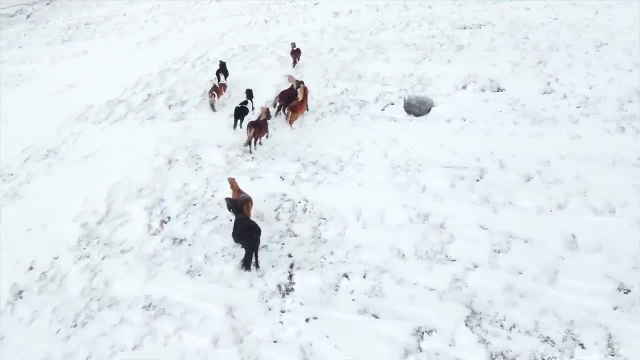 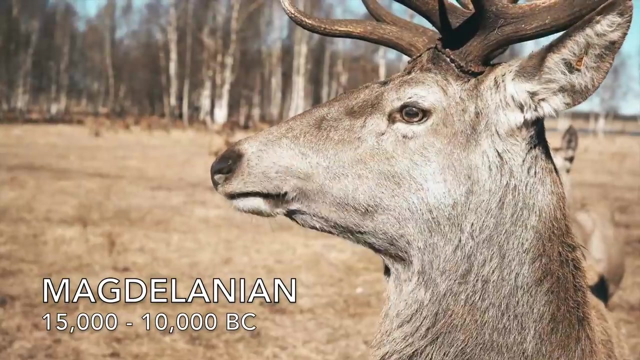 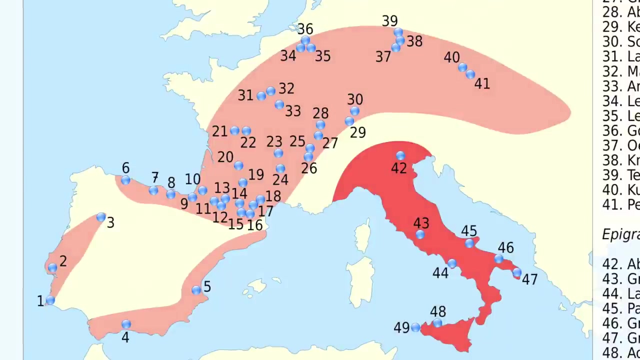 And yet there were places the hunters went back to year on year. Several so-called Magdalenian-era mega-sites have been found, Winter enclaves of the French Périgord and Spain's Cantabrian coast with deep records of human activity. 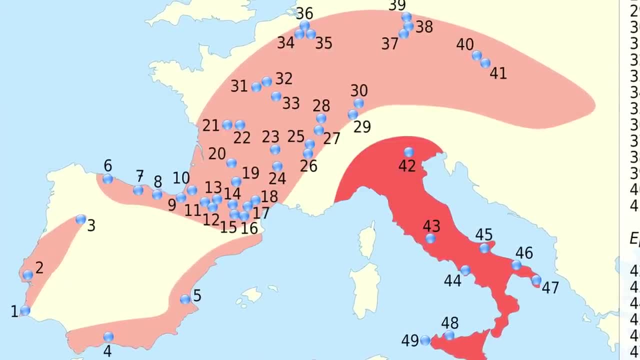 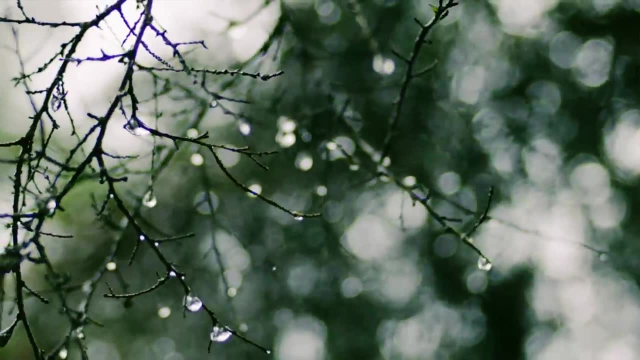 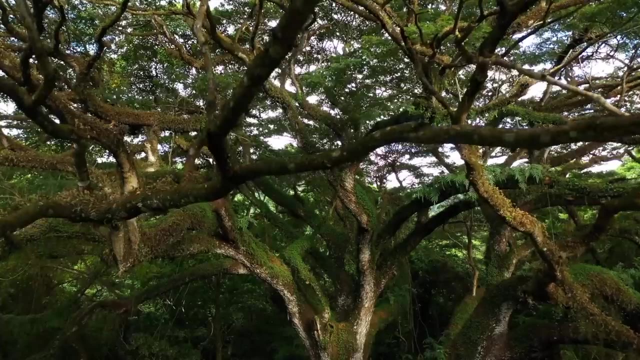 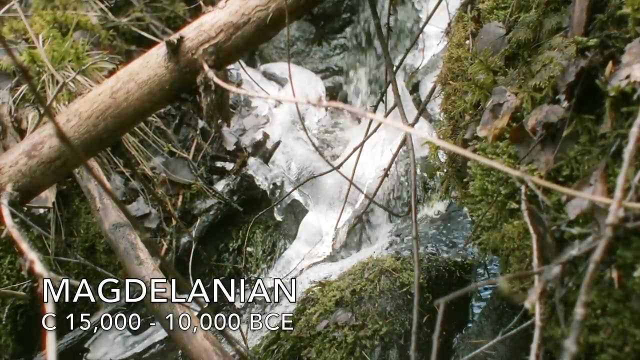 Where sizable groups of people may have annually congregated to take shelter during the early autumn before moving on in spring, During the time of the Magdalenian, as lush animals and plants flooded in to replace the barren tundra in the centuries following the last glacial maximum. 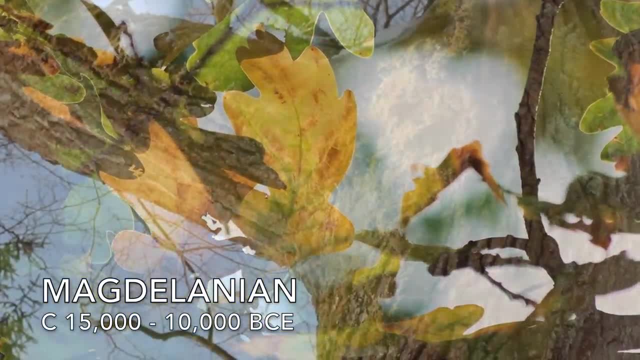 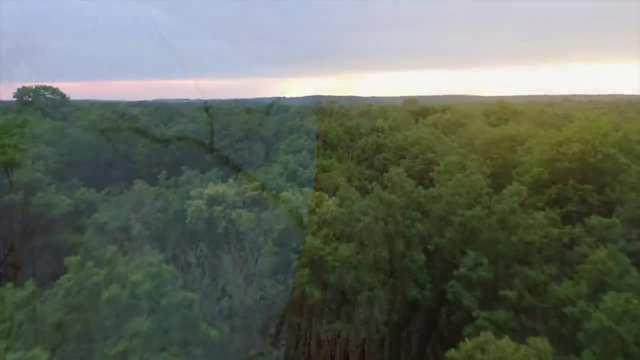 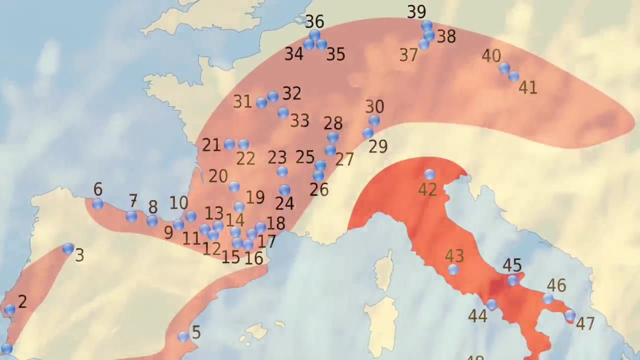 southwest France was to become one of the most heavily populated areas in Europe, Bolstered by the vast numbers of fauna available to hunt, between around 15,000 and 10,000 BC. these were people living complex lives with a wide variety of hunting strategies. 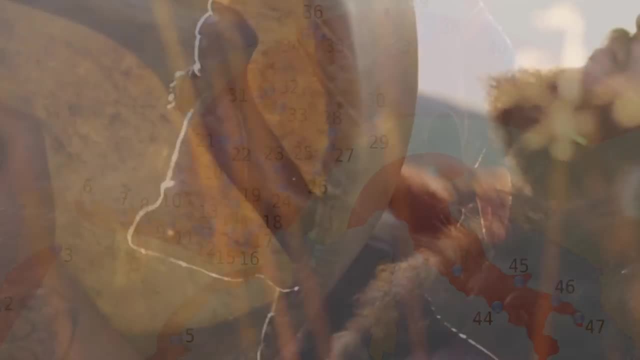 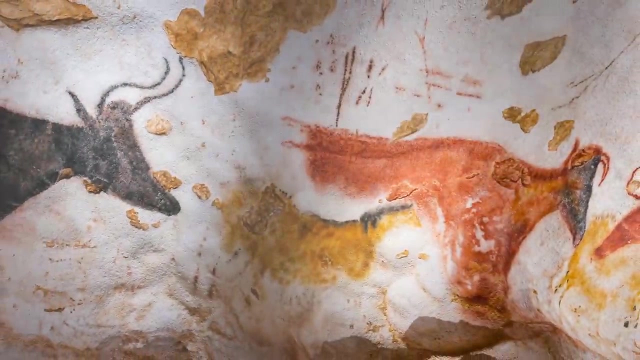 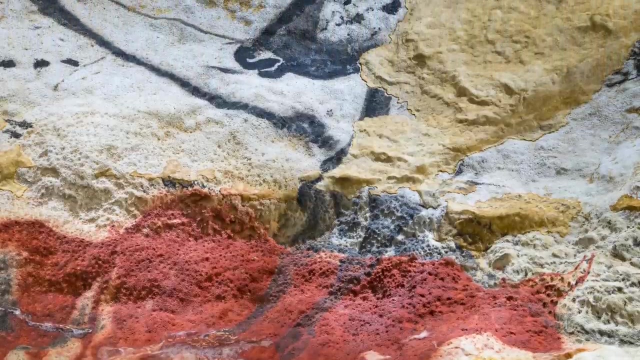 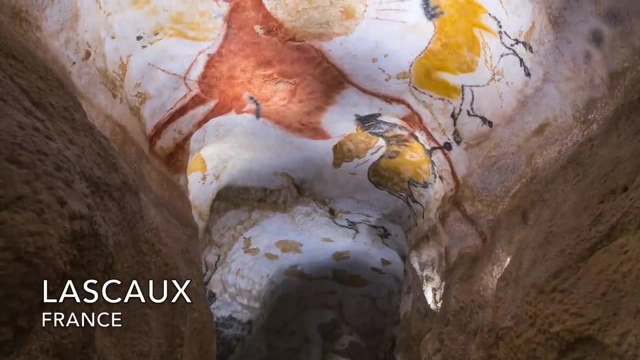 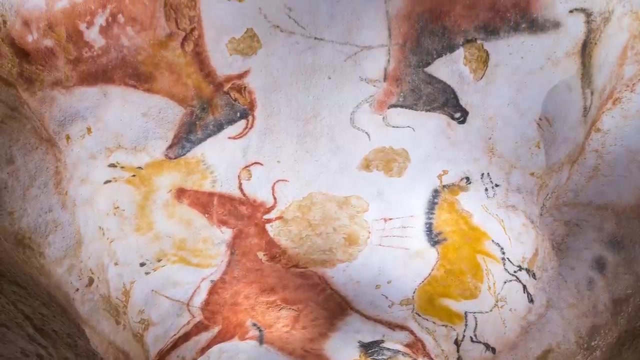 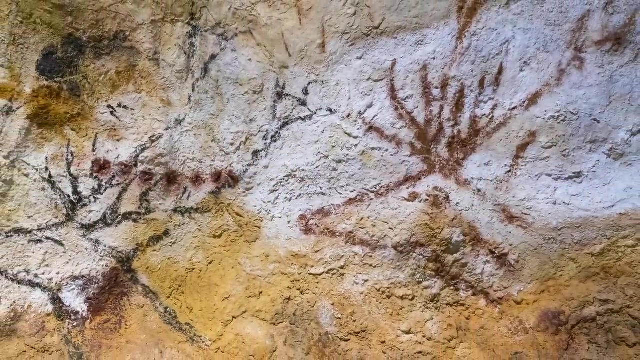 gathering techniques and artistic and cultural pursuits, Including, of course, cave art, Found in an abundance of locations but famous from sites like Altamira and Lascaux. Masterpieces of Paleolithic art At French sites like La Madeleine and Abbe Poteau. 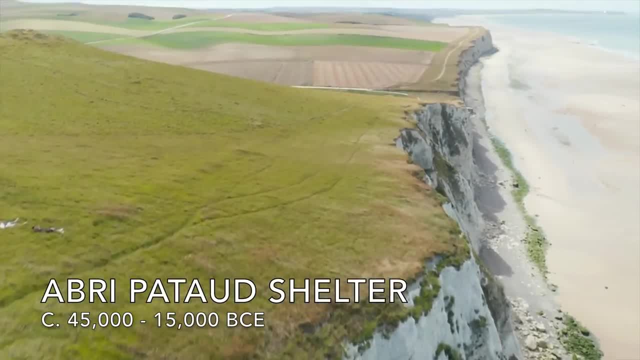 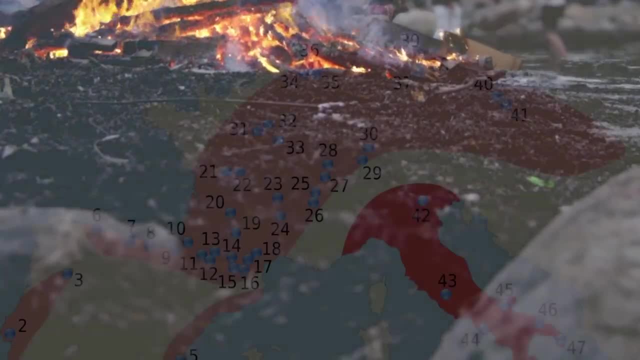 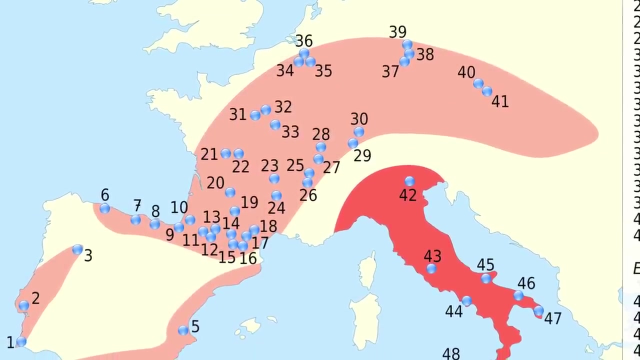 marine shells, animal pelts and significant quantities of amber speak of trade, or at least exchange networks spreading far and wide across the continent At such winter times. according to the work of archaeologist Randall White, who studied reindeer teeth and antlers, 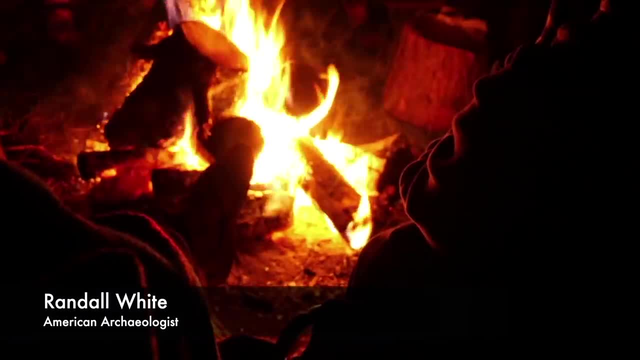 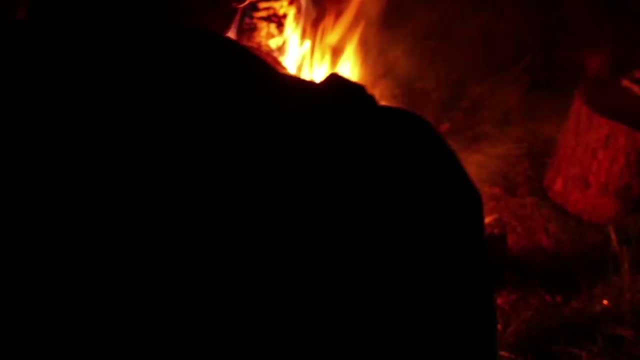 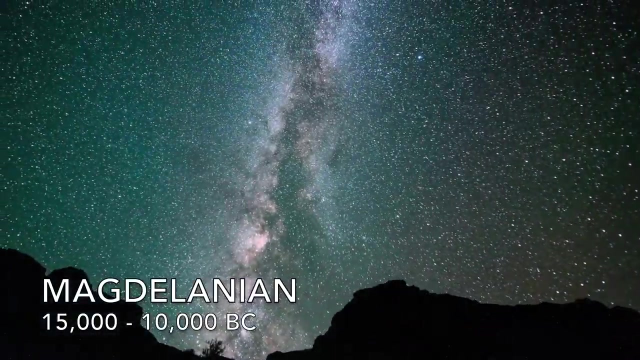 there is evidence of heightened cultural creativity in the form of cave art, carvings and ornaments, and, very possibly, social differentiation. It is at least possible that these winter communes gave rise to or facilitated already known rituals and religious rites. 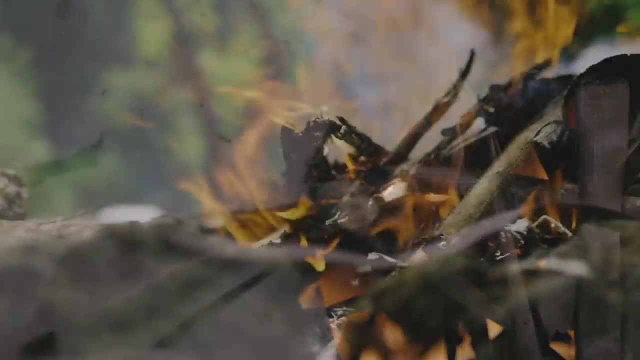 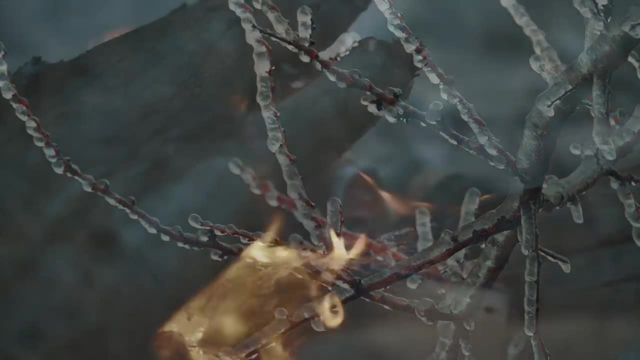 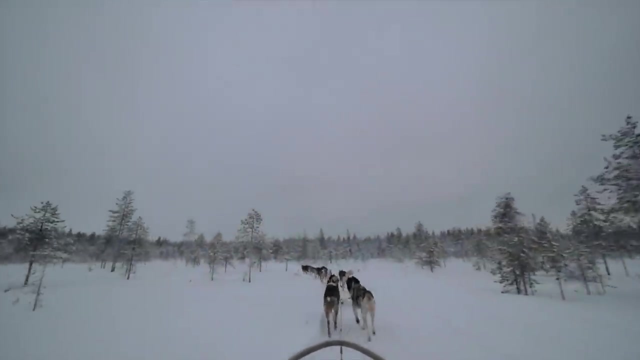 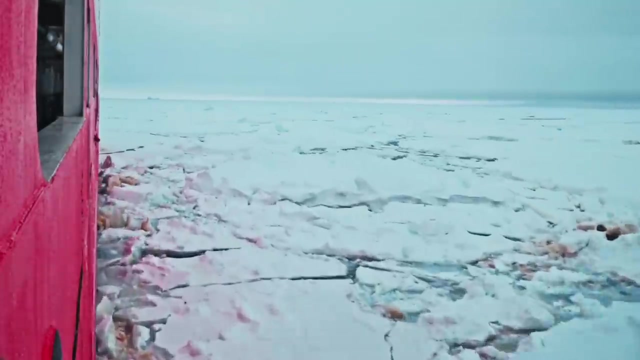 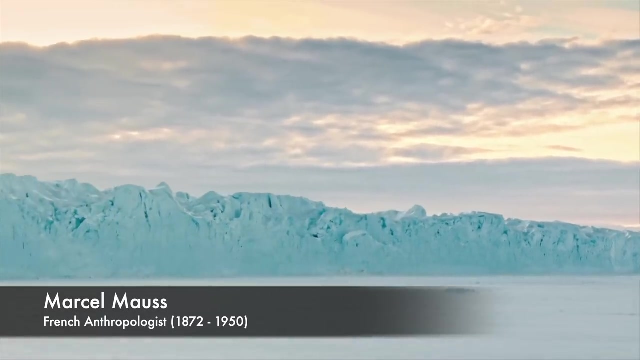 carried innately with the clans down the millennia A set of customs not vastly different to certain Inuit societies of the last 200 years. In the early 20th century, French anthropologist Marcel Mauss spent significant amounts of time studying the Inuit communities. 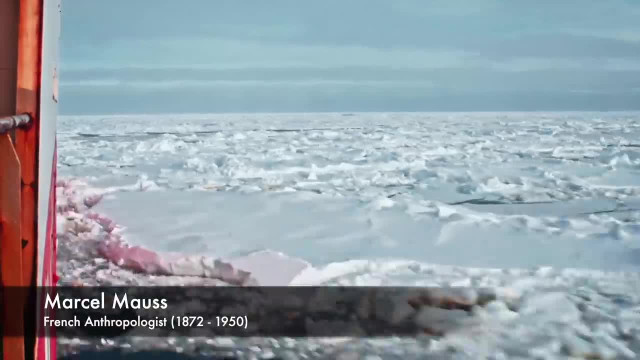 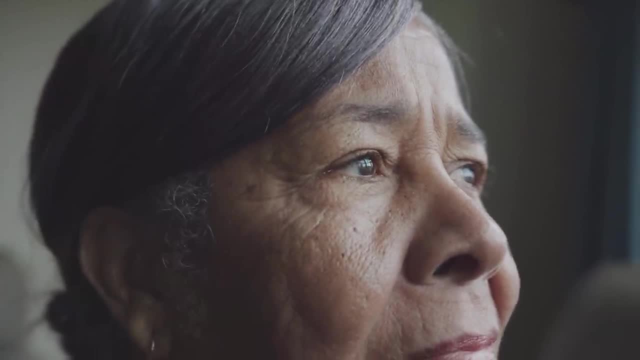 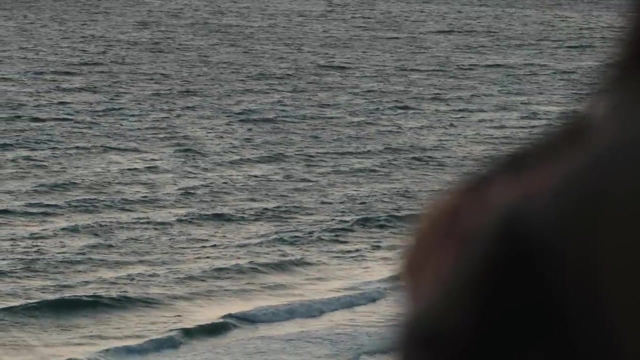 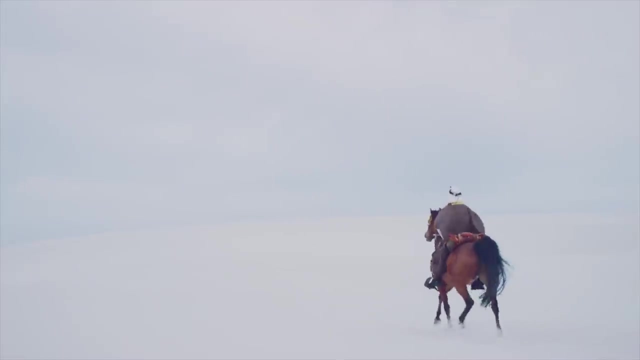 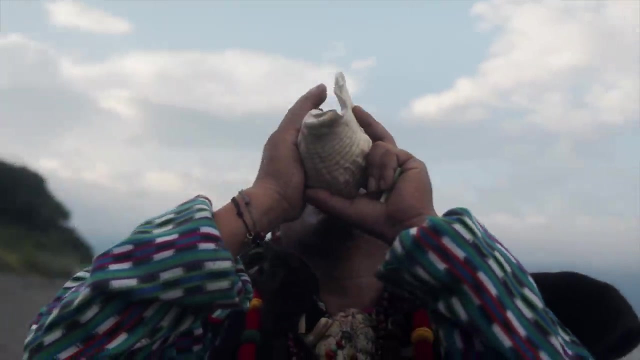 of the sub-Arctic Americas and Eurasia, Finding them to organise their societies in certain unique ways, Very different to the settled agricultural societies that cover most of the globe During the winter. a relatively authoritarian structure would form, Dictated to and governed by confraternities. 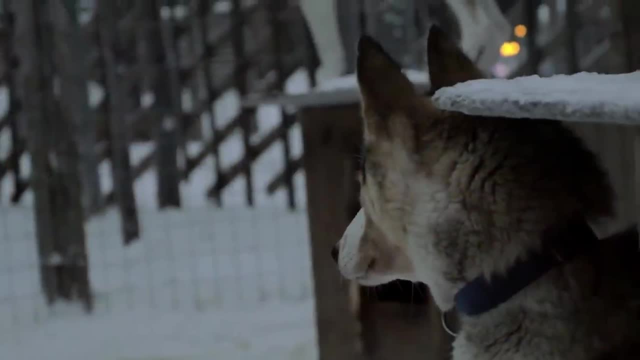 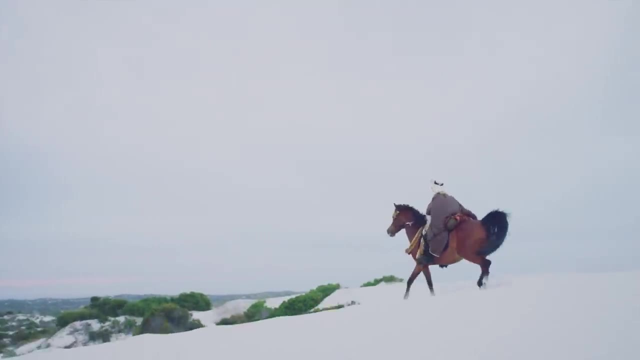 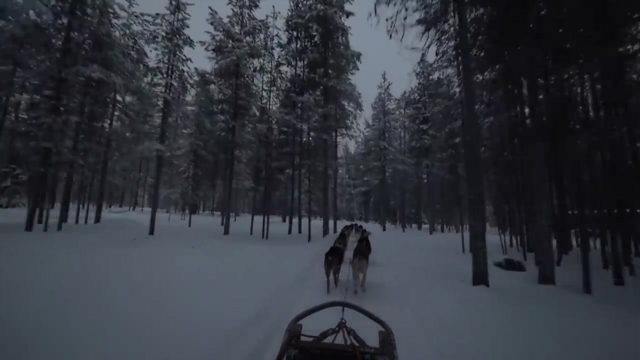 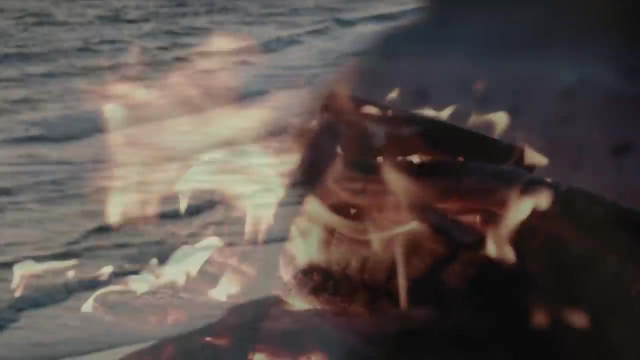 of priests, nobles and commoners. In the spring, individualistic egalitarianism would arise once more, As people spread out into the landscape again to forage and hunt, Before, eventually, the next autumn, perhaps, in a timeless scene that echoes down the ages. 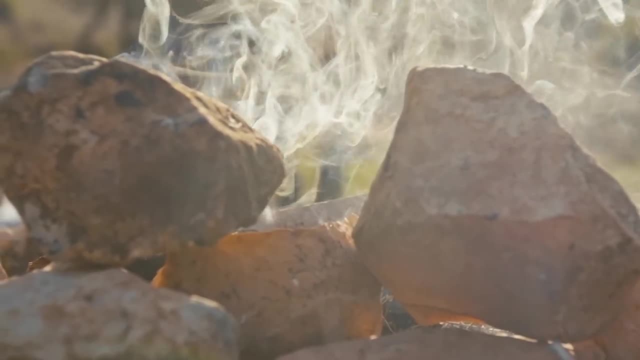 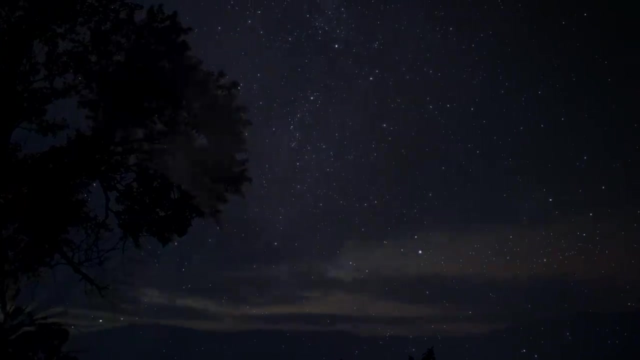 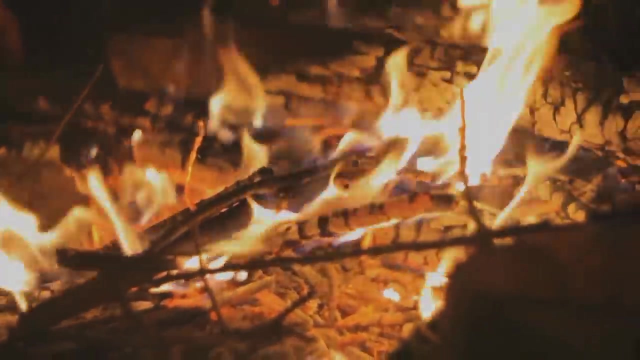 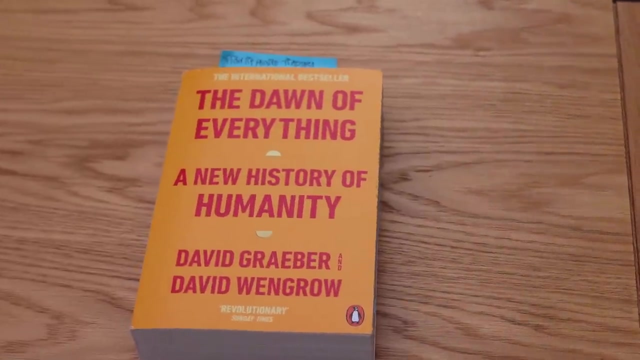 they would gather again for intense communal celebrations of cosmic order and the cycle of the world. In their recent book, The Dawn of Everything, anthropologist David Graeber and archaeologist David Wengro entertain the notion that similarly structured societies and customs may have actually been. 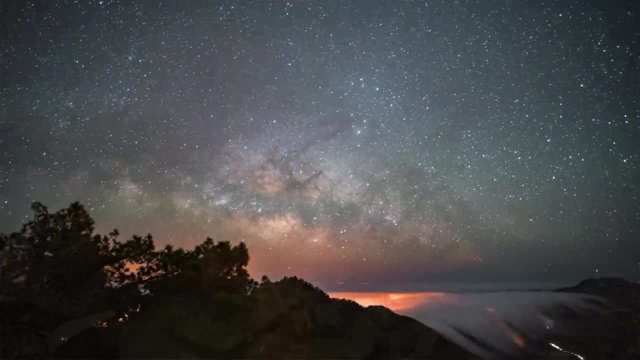 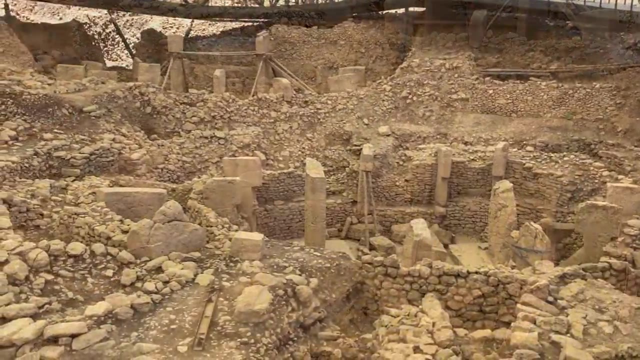 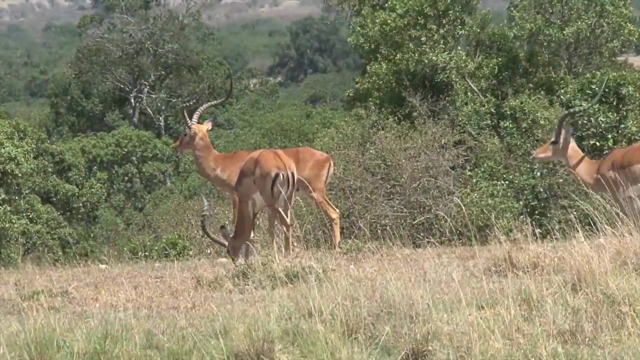 the driving force behind the creation of the Gobekli Tepe phenomenon, The construction of enclosures now even being linked by isotopic evidence to periods of annual superabundance, When vast herds of gazelle would descend on the Haram Plain. 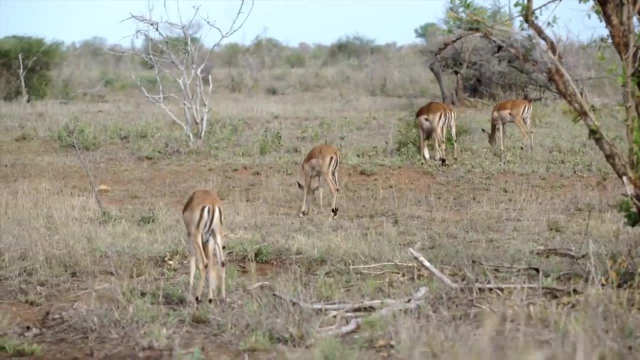 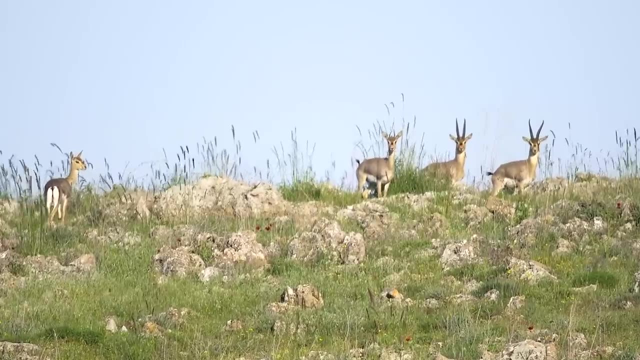 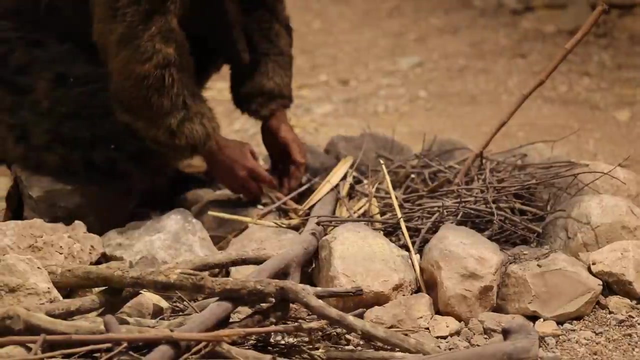 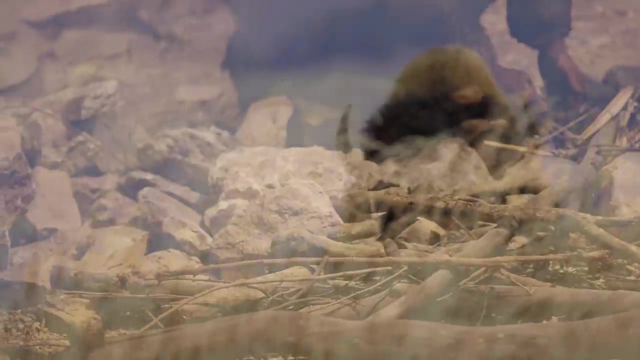 Creating an immense surplus of food for the hunters living nearby. As we have seen time and time again, our ancestors weren't just our equals in cognitive capacity, but in intellect, even philosophy, too, And so we turned back to the megalith builders. 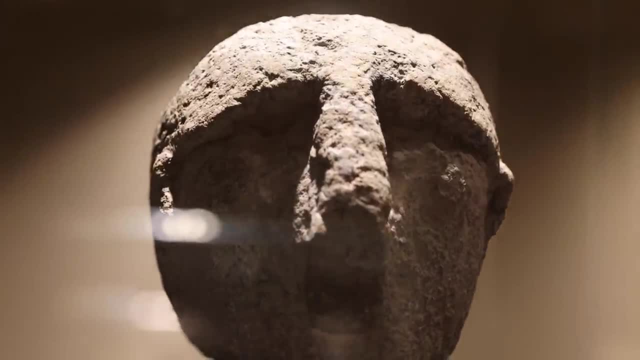 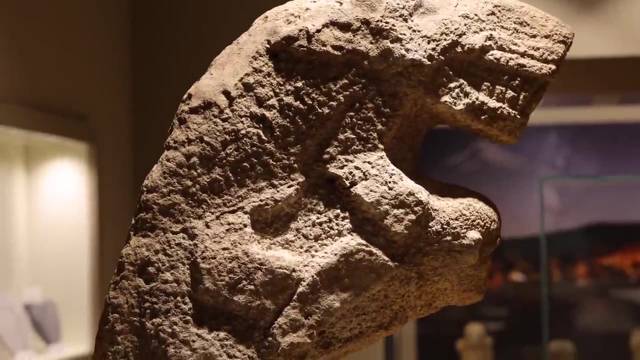 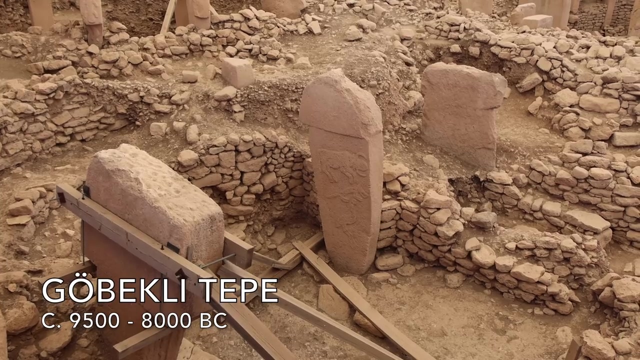 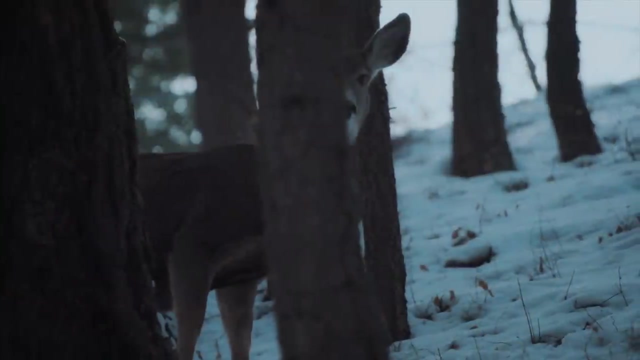 of the Urfa Plain. Despite their impressive size and the great skill of their construction, the enclosures at Gobekli Tepe seem only to have been used for a relatively short amount of time, Much less, for example, than some of the previously discussed. 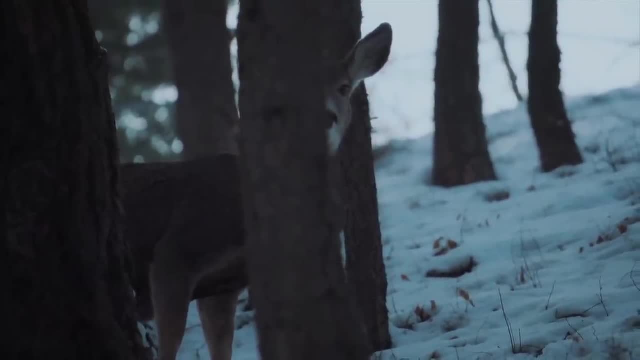 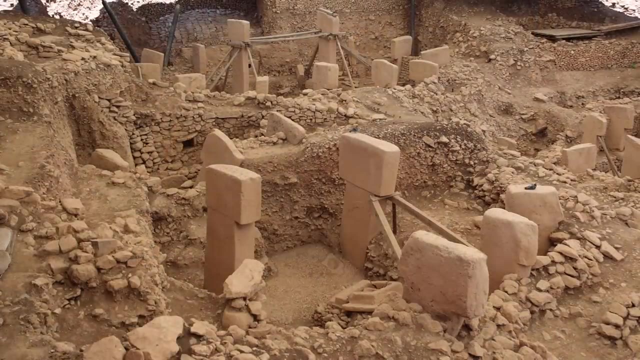 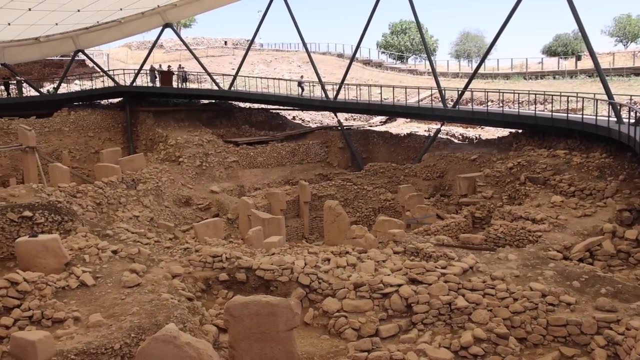 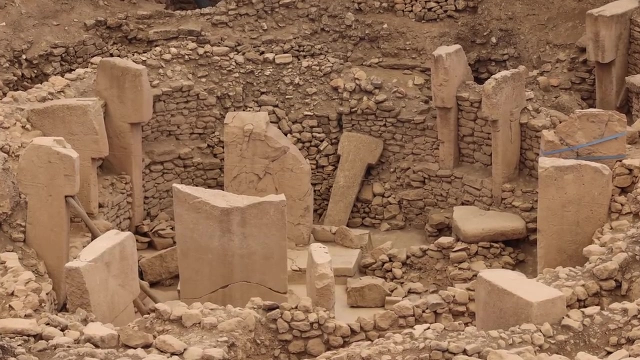 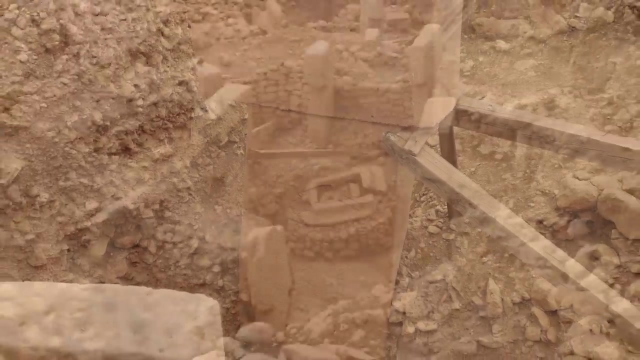 Ice Age sites, Their raising and, ultimately, ritual deaths and burials, often within just a few generations, may well have been the point: Hierarchies raised to the sky, only to be torn down again as part of some long lost ceremony. Just maybe. 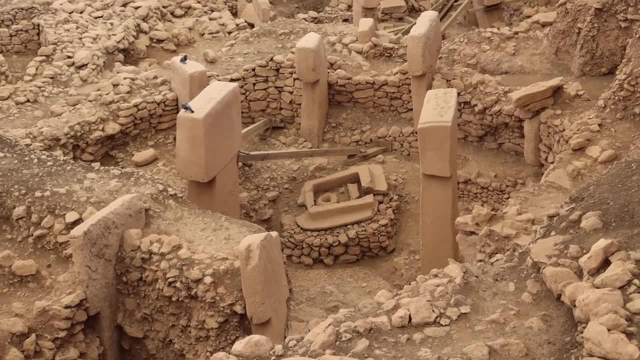 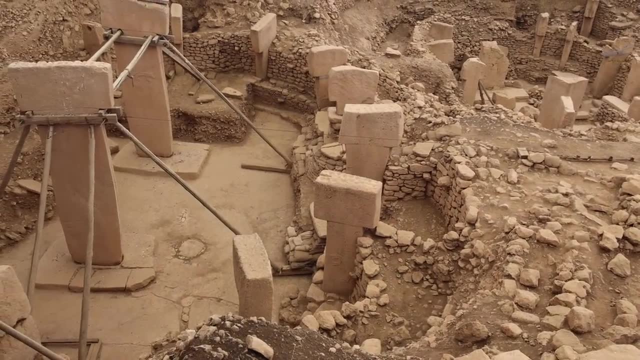 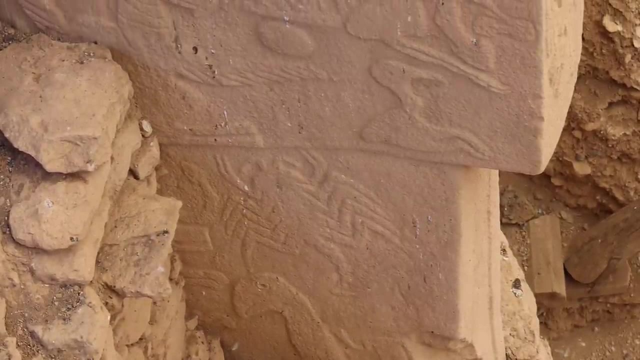 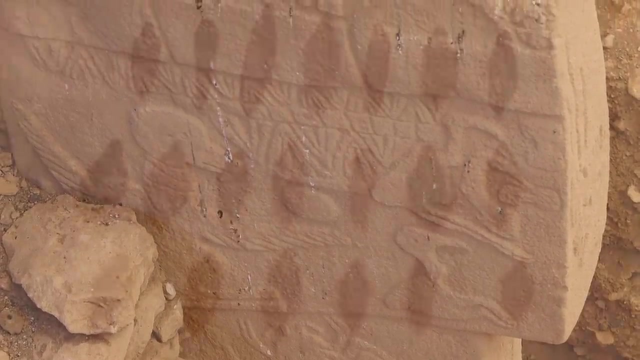 it is festival activities at sites like these that the very first beginnings of larger societies and nations first began to coalesce, United by stories and the links fostered during those communal times. Indeed, the abundance of flint shards found all over the surface of Gobekli Tepe. 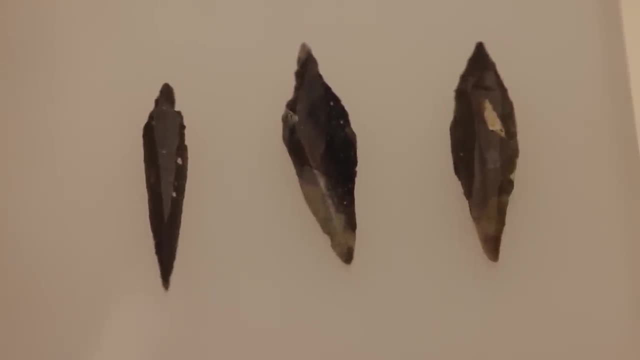 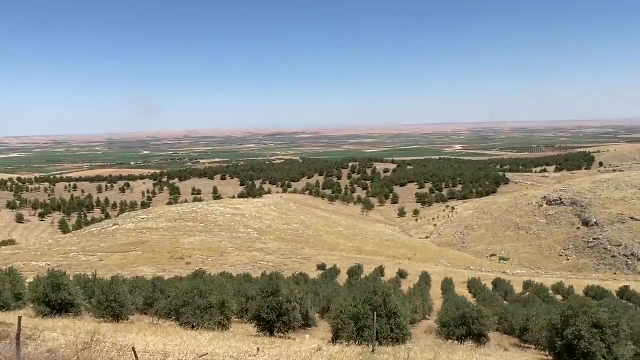 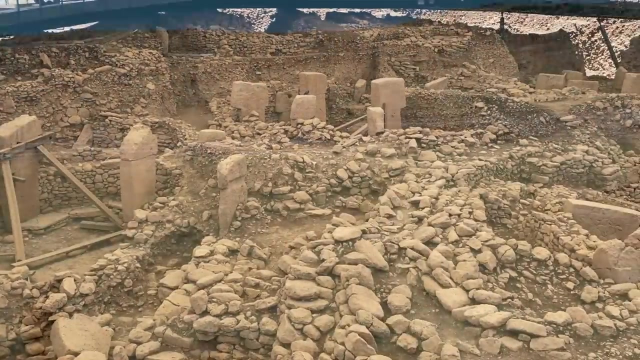 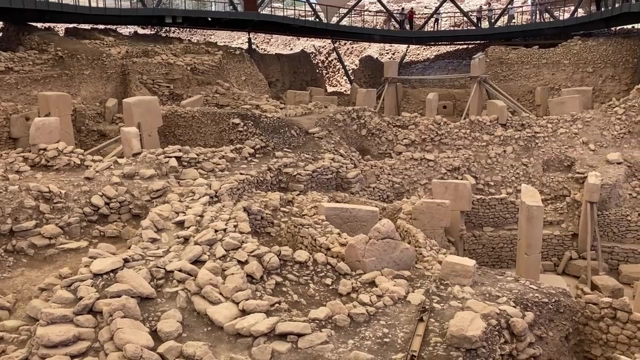 many of which were brought in from afar, suggests trading or exchange activities with distant groups, or even full blown seasonal migrations, Whether the stones themselves were taboo for most of the year. Access denied to anyone but a hypothesized temple elite, But given free access. 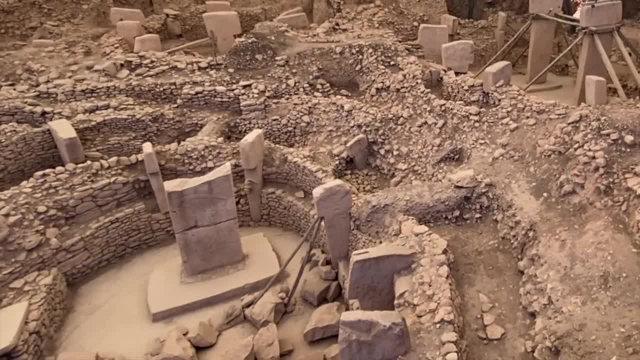 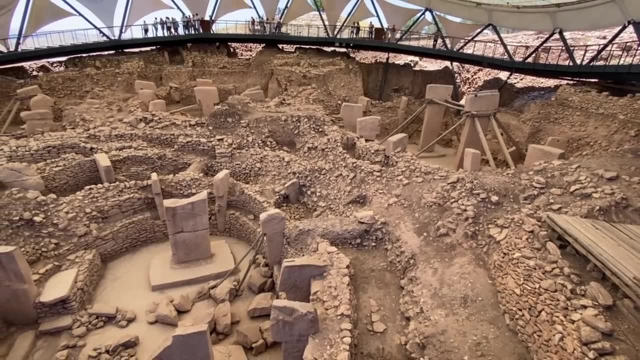 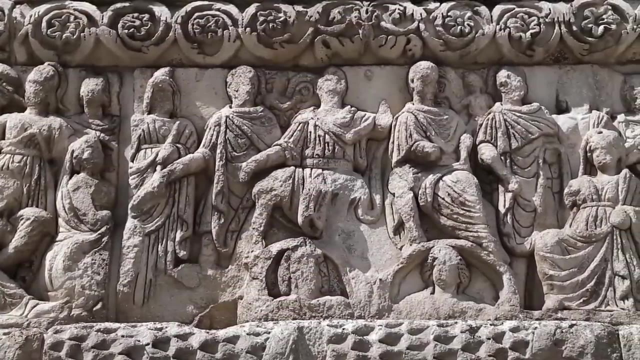 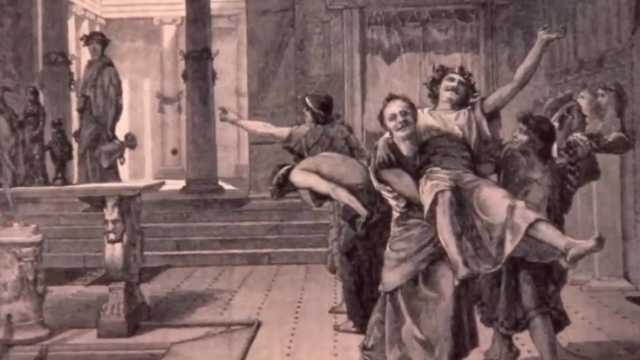 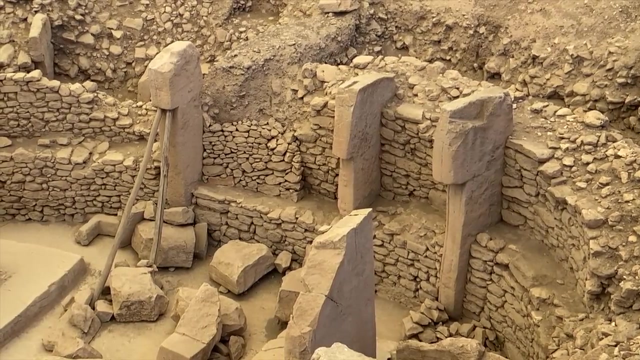 during festival times, we can't be sure- Left to conjure fleeting visions of a medieval carnival or Roman Saturnalia, Where societal roles were switched, The world turned upside down. There is, however, concrete evidence in the abundant remains of gazelle. 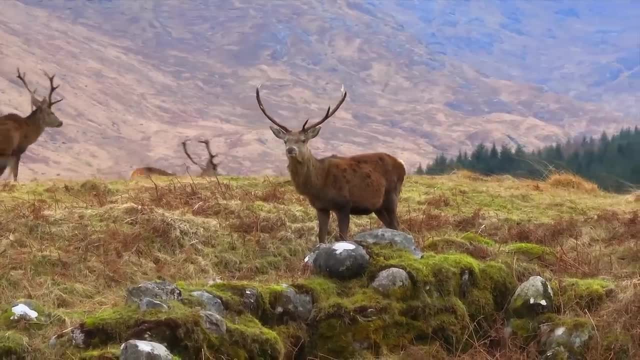 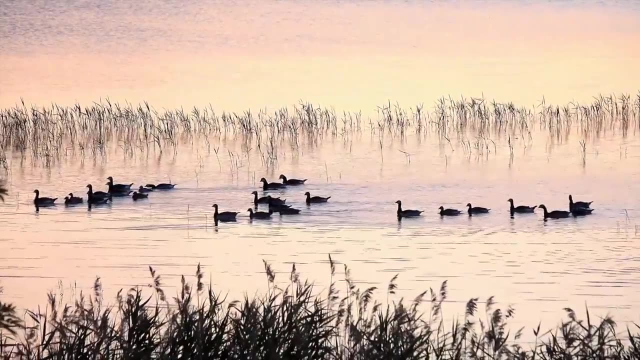 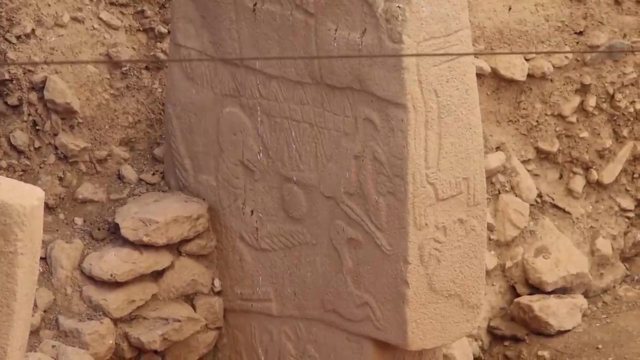 boar goat, red deer, sheep, oxen, vultures, ducks and an entire menagerie of birds- Most of the animals depicted on the monoliths That Gobekli Tepe was very likely a site. 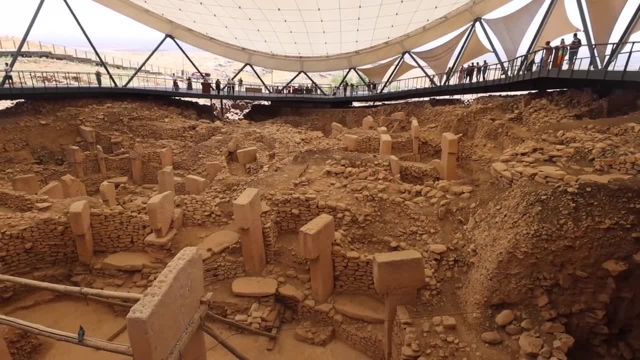 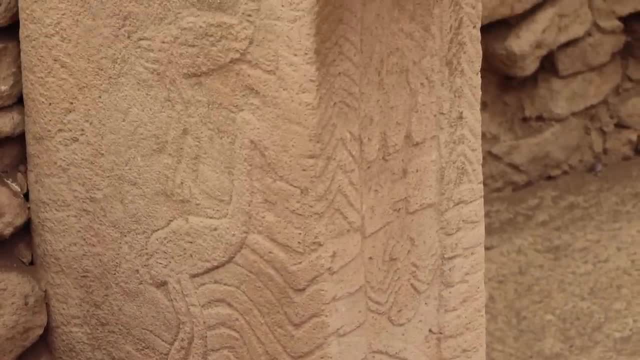 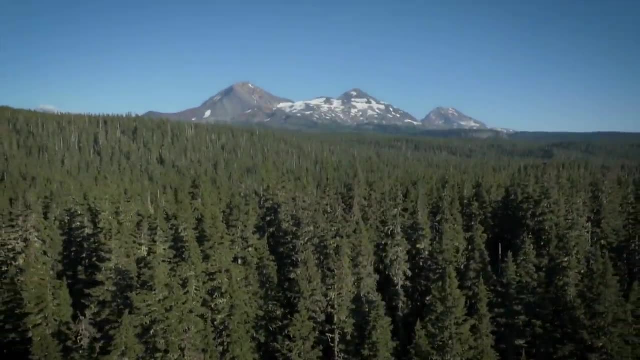 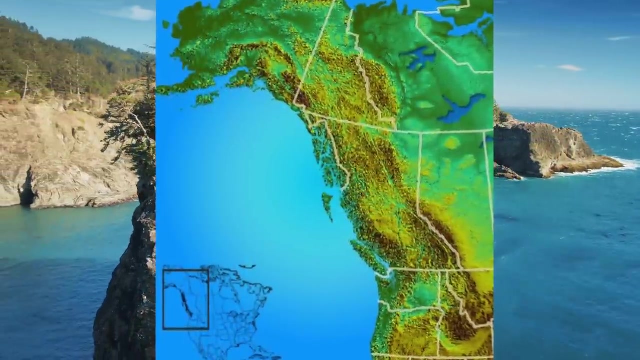 for feasting events. But what did those feasts actually look like? Turning to the far edge of the world, In the Pacific Northwest of the United States, Another land of totem poles Awash with memory and the customs of long venerated ancestors, 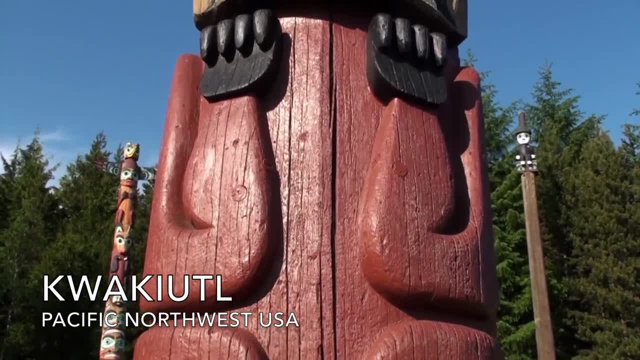 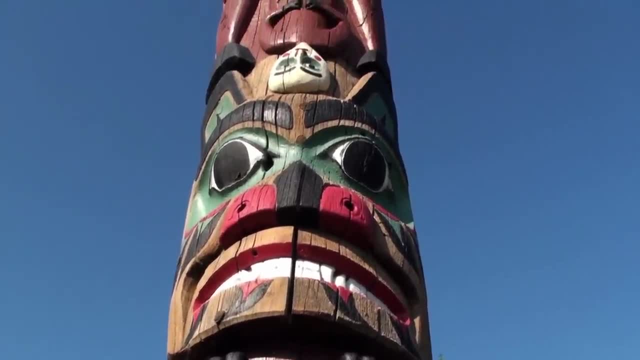 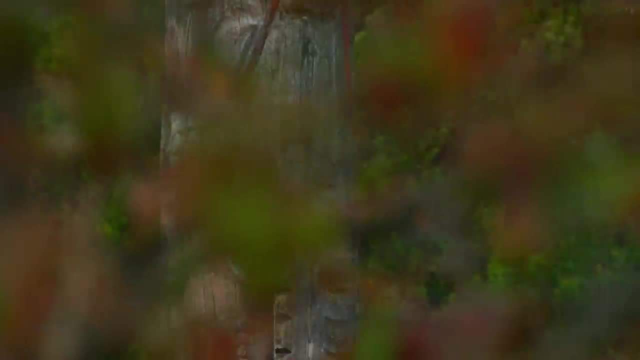 The Kwakatole people have exercised a mid-winter ceremony for as long as anyone can remember, When people came from afar to congregate and regroup Under the harsh grip of an icy black sky, A shifting ritual of so-called bear dancers. 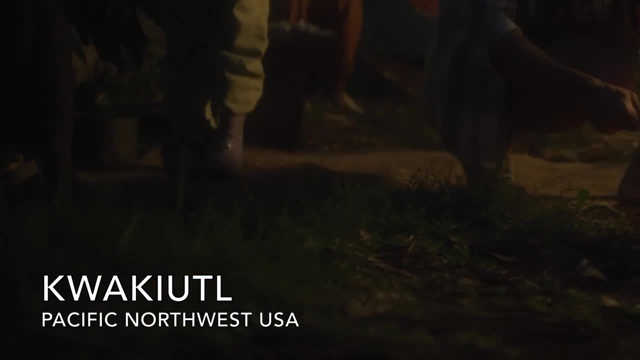 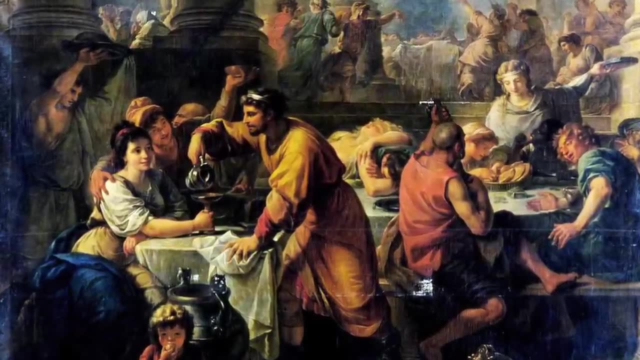 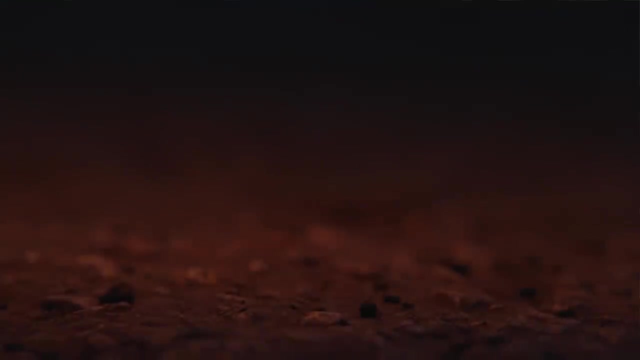 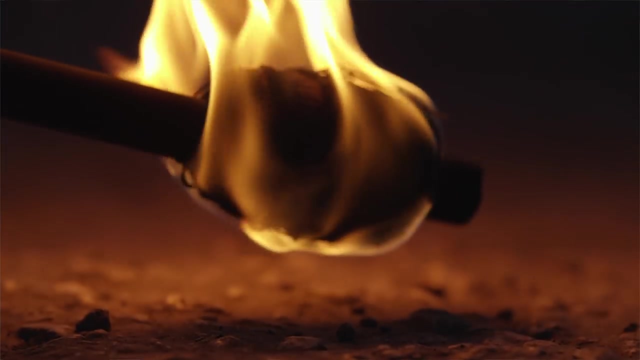 and fall dancers replaced the usual social hierarchy, In scenes reminiscent of Roman Saturnalia and the medieval carnival. The mid-winter is a time when the lowest of the low are elevated to the highest positions in society And vice versa, Though, of course, separated. 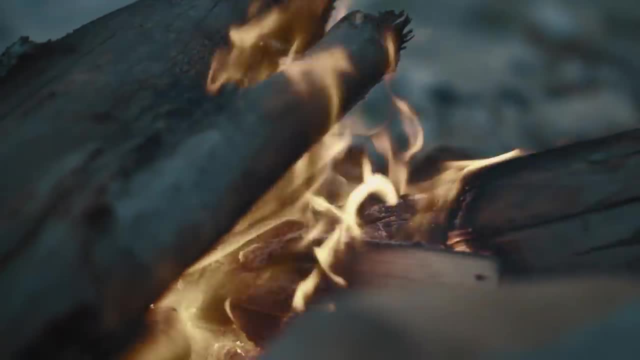 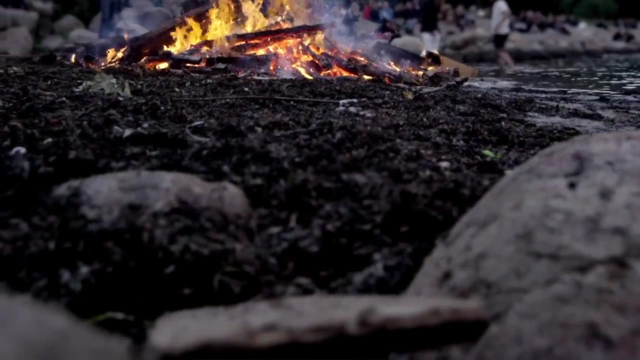 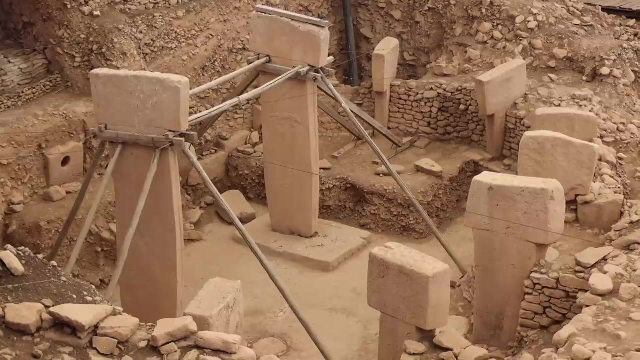 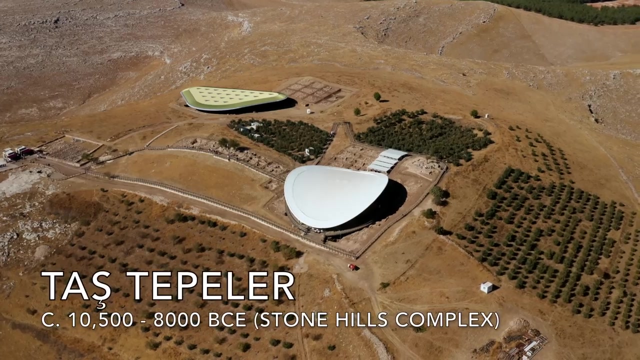 by vast gulfs of distance and time. Perhaps some small similarity may be found with those purported festivals on the southern edge of the Taurus Mountains so long ago. For evidence of the festivals themselves in that so-called Stone Hills culture, We can look to Quebecli Tepe's. 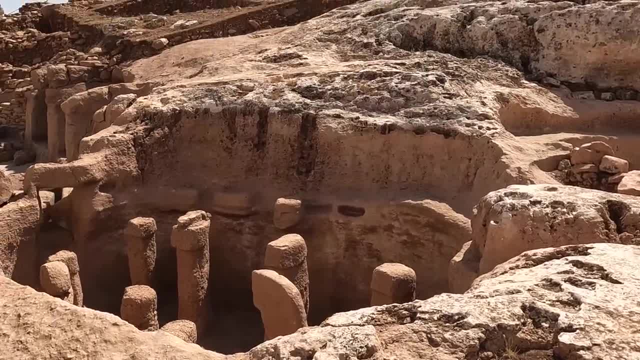 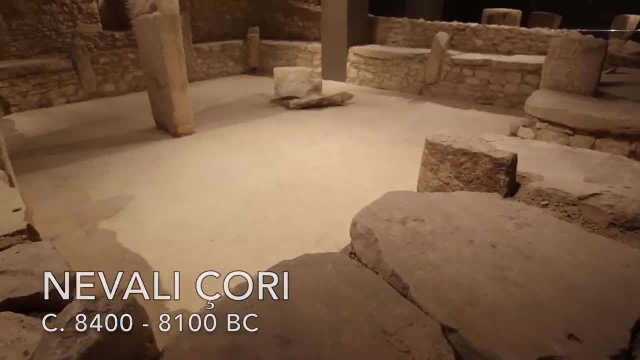 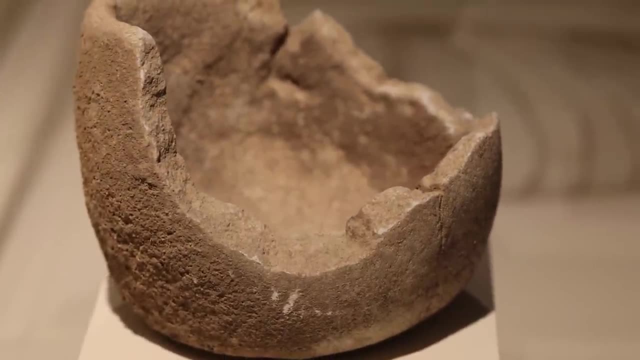 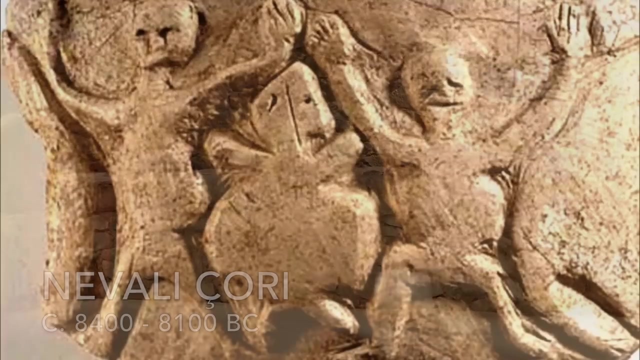 sister sites too. Nvali Chori, in particular, is a site which has yielded an unusually rich array of artefacts of many types. One rare engraved stone basin on the floor of one of the houses. There's even been suggested to be a sacrificial altar. 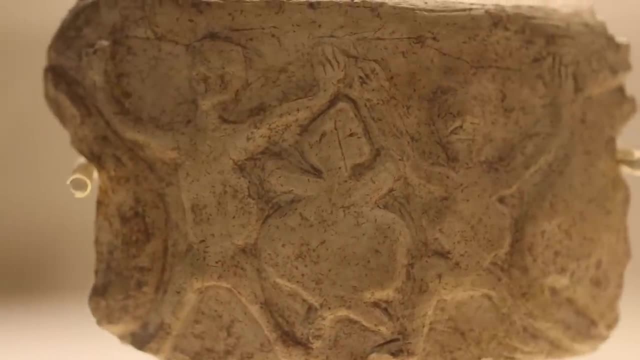 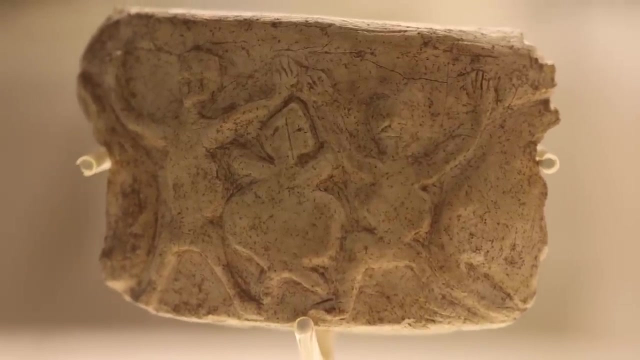 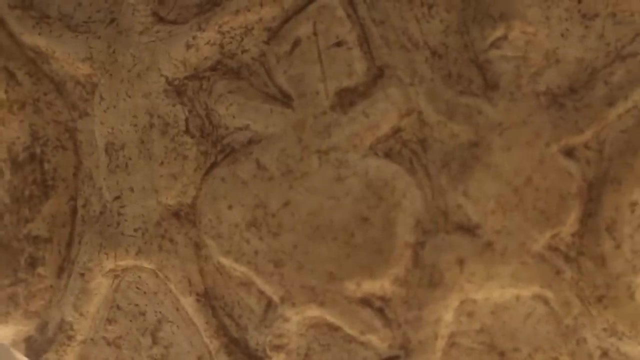 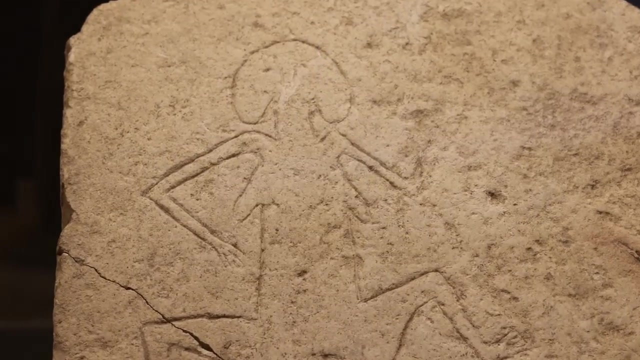 It was carved with an unusual central figure. Originally interpreted as a turtle, opinions have shifted since to interpret the scene as a woman in dance, Feet pointed down, her arms raised to the sky. If true, this would be one of the earliest dancing scenes in all of history. 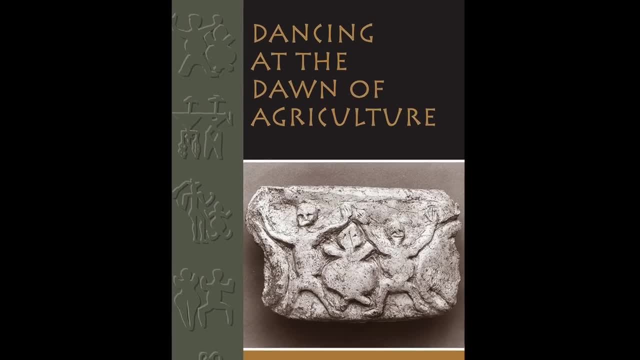 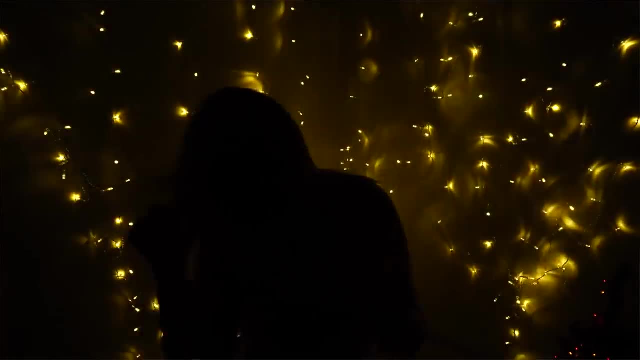 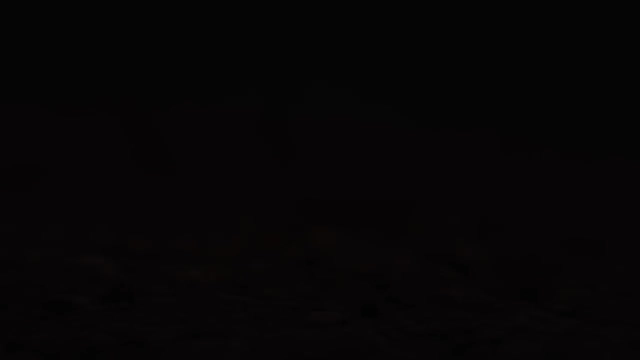 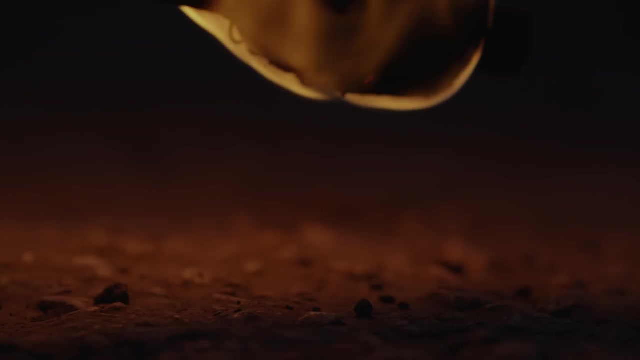 An activity very often tied up in festival and religious activities, Found in almost every society in history. We even have evidence of musical instruments, too, Stretching far back into the Paleolithic, In the form of bull, roarers, clappers, rattles and scrapers. 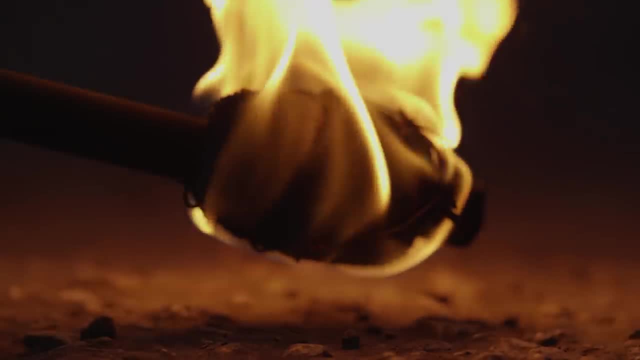 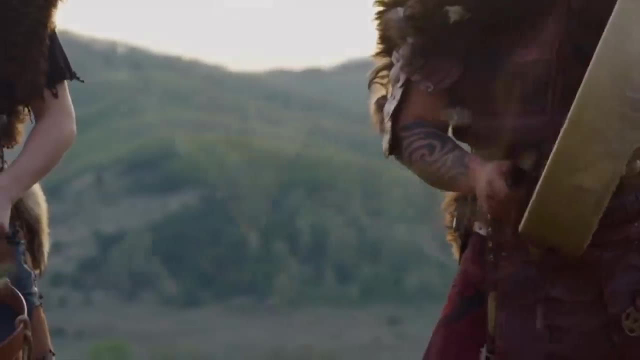 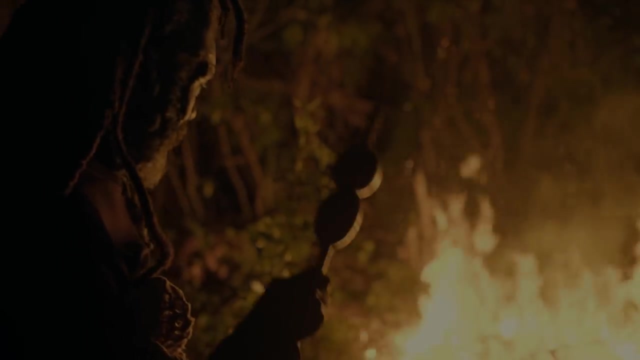 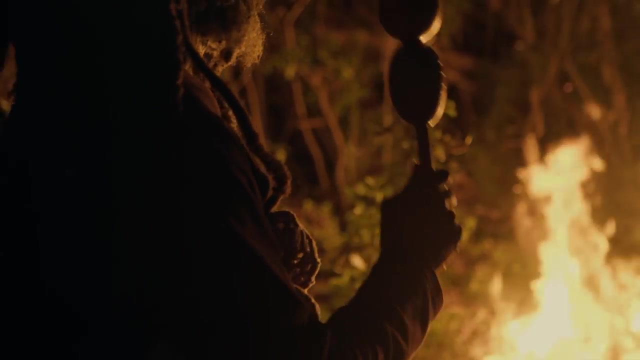 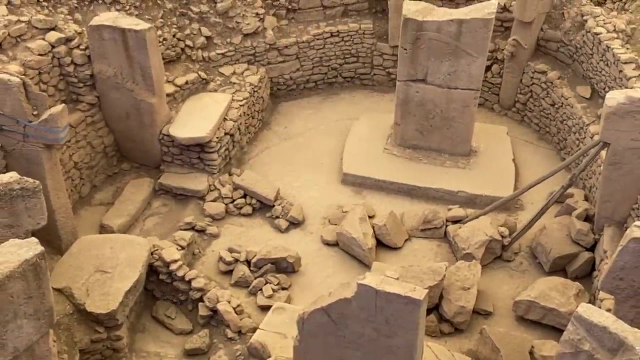 When reconstructed and played today, they recall primordial sounds of travellers dancing to the drum of the divine Pilgrims even come from nearby and distant lands to sacrifice, to feast and to celebrate in the shadow of the obelisks. We also know that Gobekli Tepe's 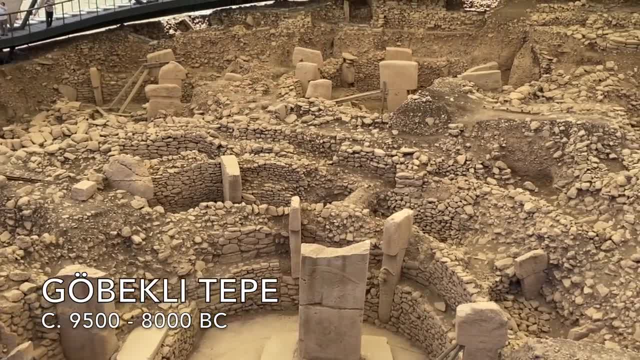 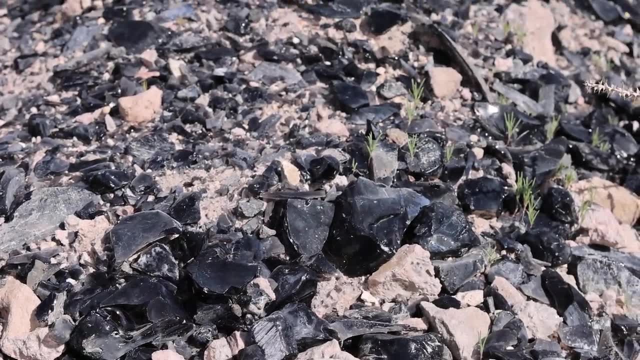 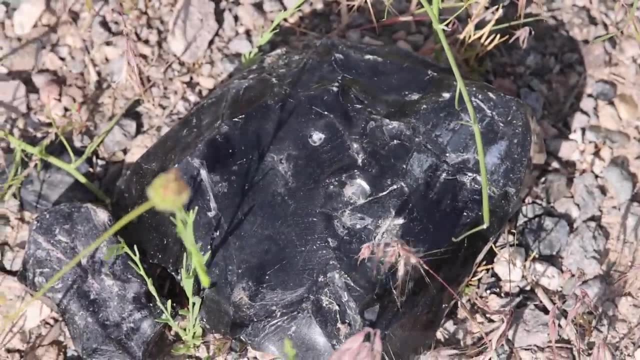 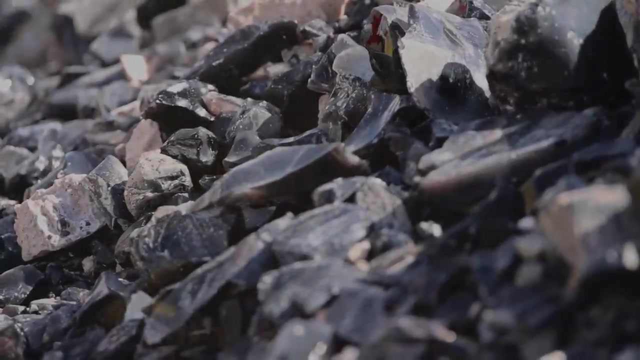 significance extended far beyond the Urfa Plain Obsidian deposits originating in Cappadocia to the northwest and beyond, perhaps brought by travelling specialists imbuing items and themselves with power and energy for the year to come. Other travellers at the dawn of settled 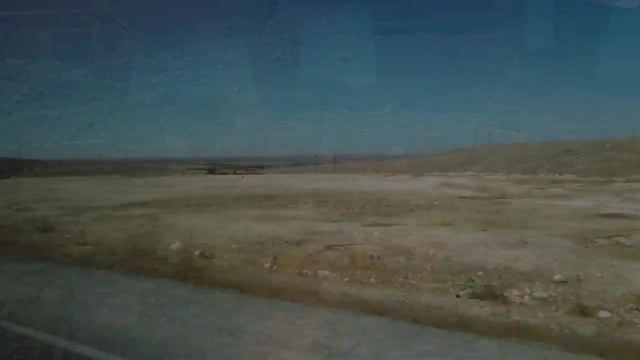 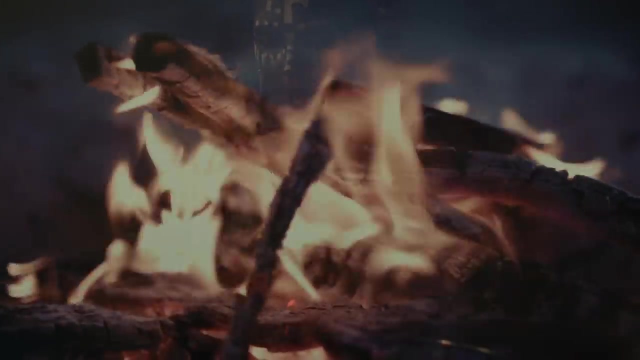 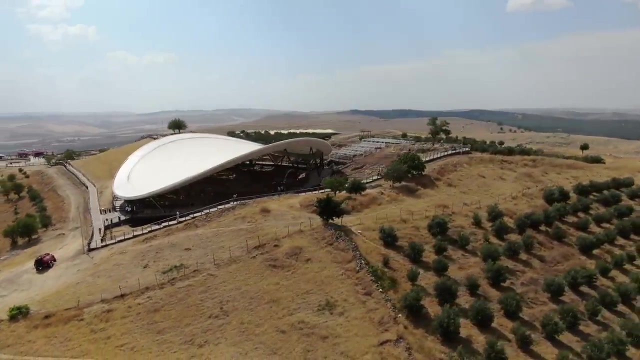 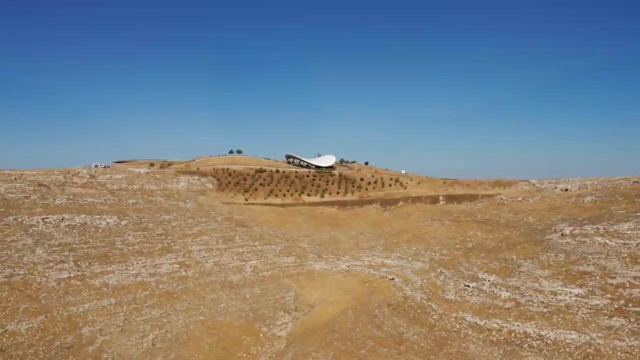 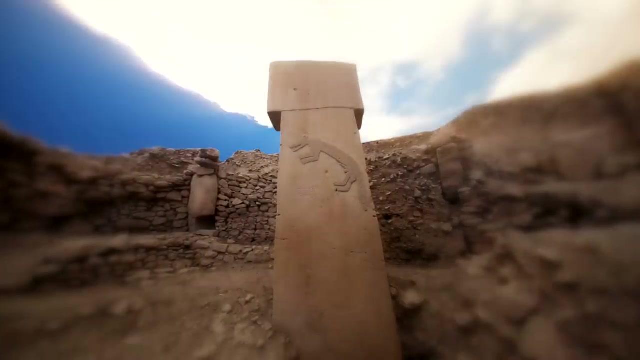 life- entertainers, healers, storytellers- cannot be proven Any evidence that might have once existed long ago, having disappeared into nothing. Though the history of Gobekli Tepe is a long history, We can speculate nonetheless Since the very earliest days of archaeology. 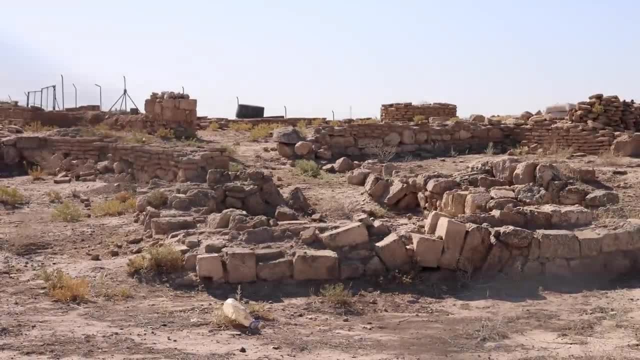 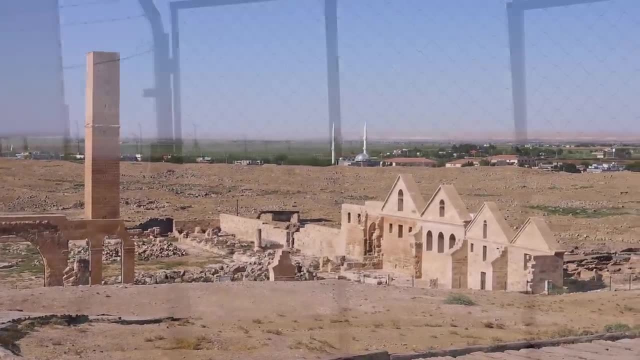 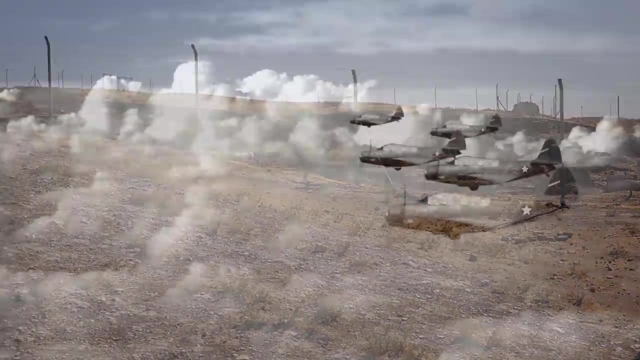 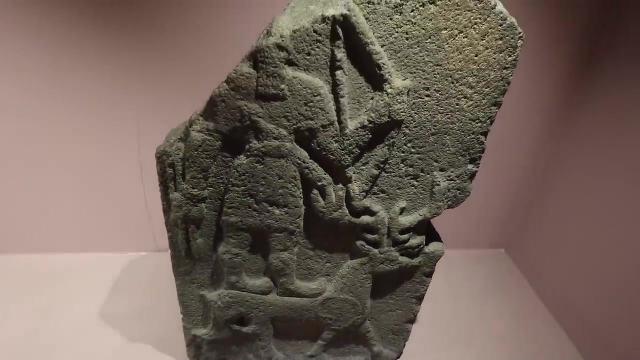 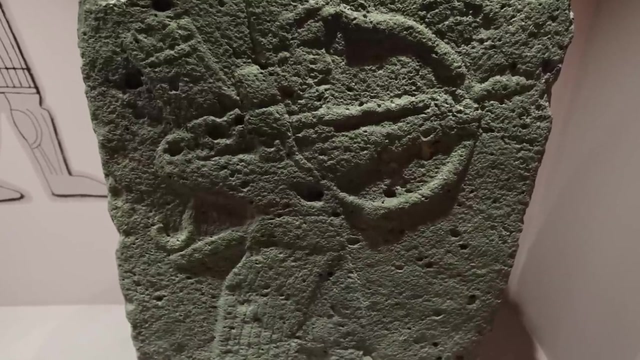 and anthropology scholars have sought an understanding of how our world came to be. One of the most enduring and popular ideas was an ominous one: That warfare lay at the heart of everything. Social complexity spurred on by fear and hatred above all. And yet in recent 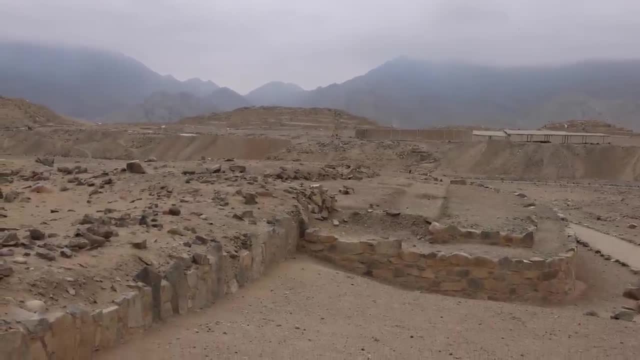 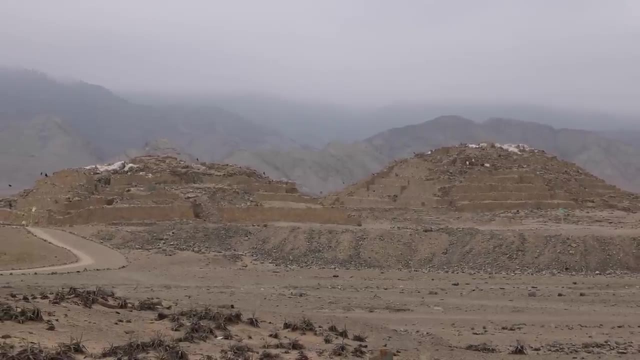 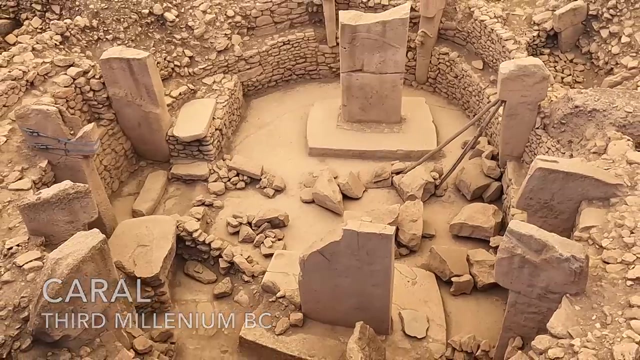 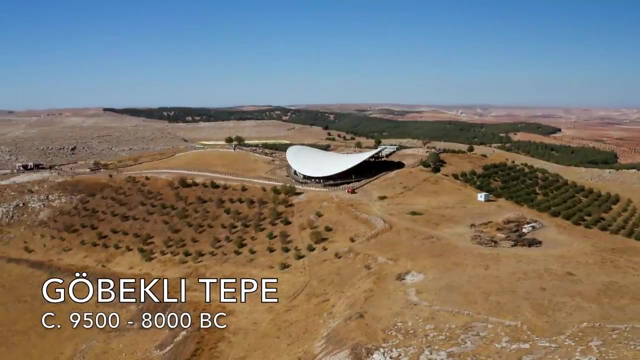 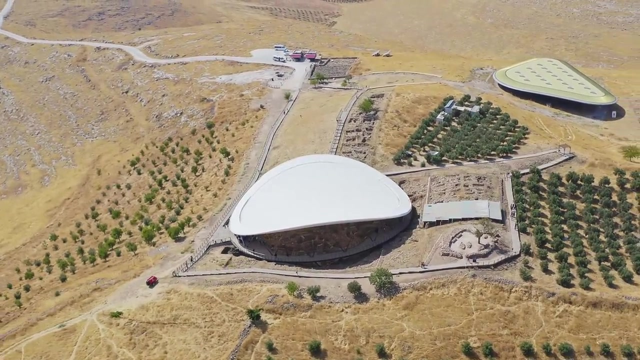 decades this concept has been undermined by a thousand cuts. Again and again, new discoveries are being discovered on sites like Corral in the Americas and now at Gobekli Tepe. lying at the very beginning of settled societies show no evidence of any kind of 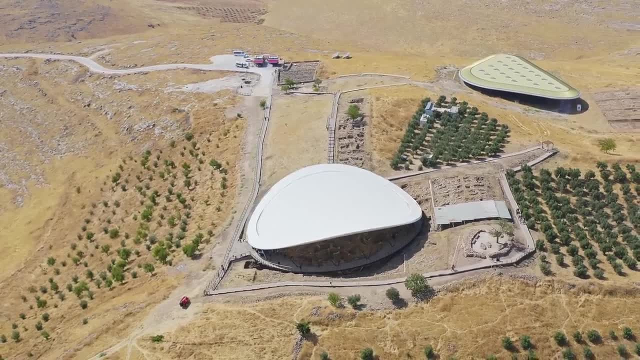 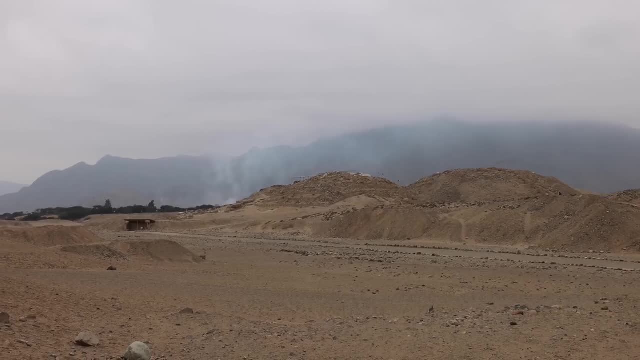 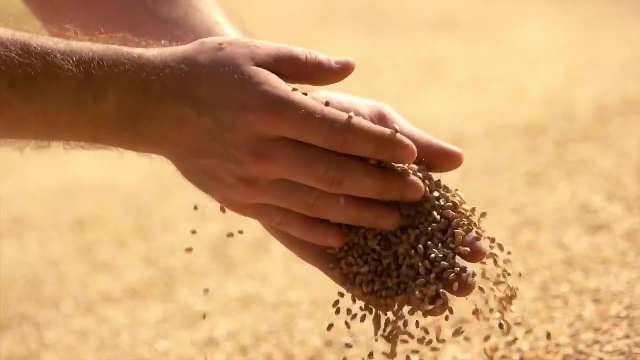 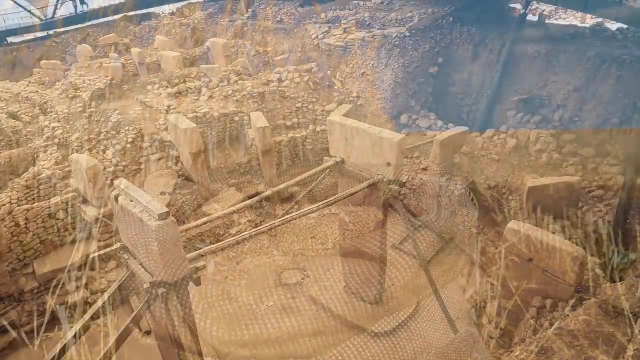 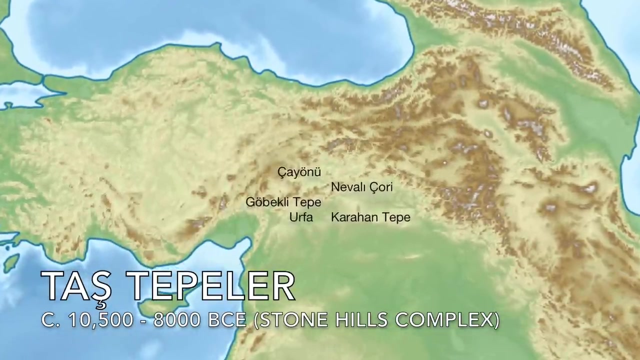 fighting. Instead, a new theory has increasingly risen in stature. The concept of the stone hills might actually be ritual. that led to the adoption of agriculture and stratification and its initial development. Though they weren't quite there yet, the affluent hunters of the stone hills 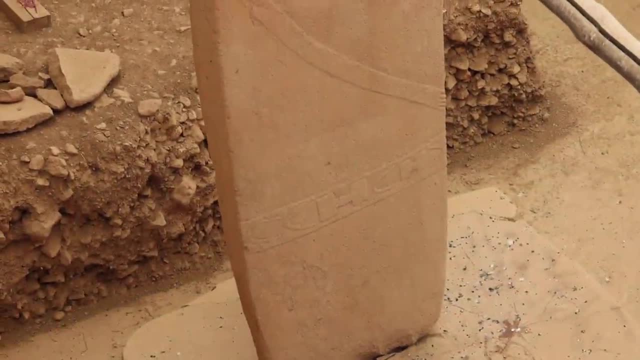 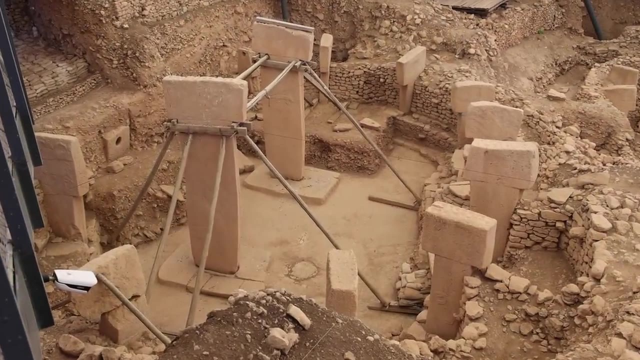 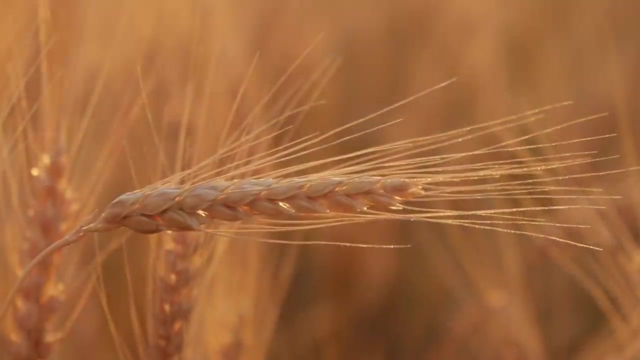 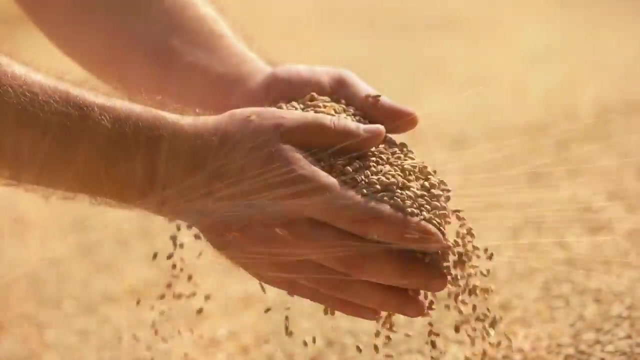 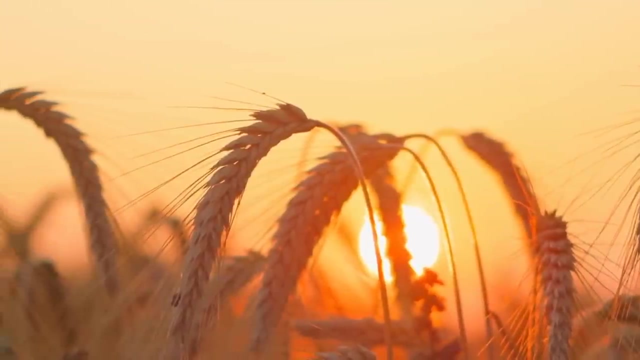 culture would be soon After all, ritual and a strictly followed set of ideas are necessary for a farmer society, Ideas which often give no instant gratification, like that of the hunters. Instead, immense amounts of work has to be invested in the work of the farmers. 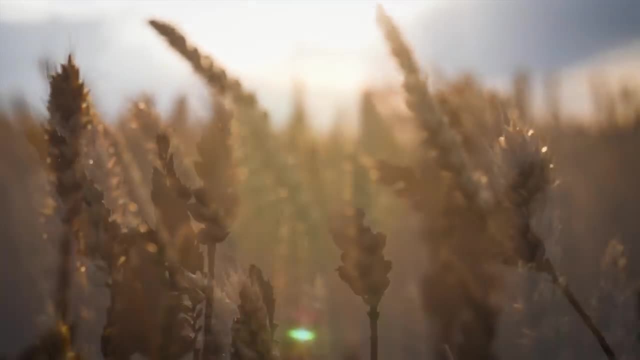 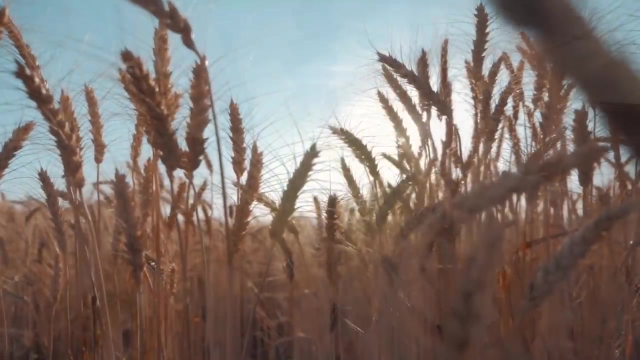 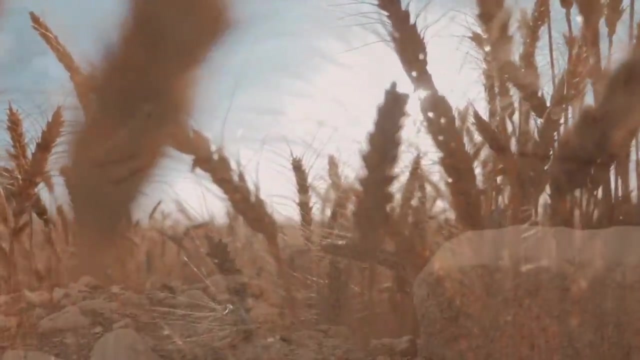 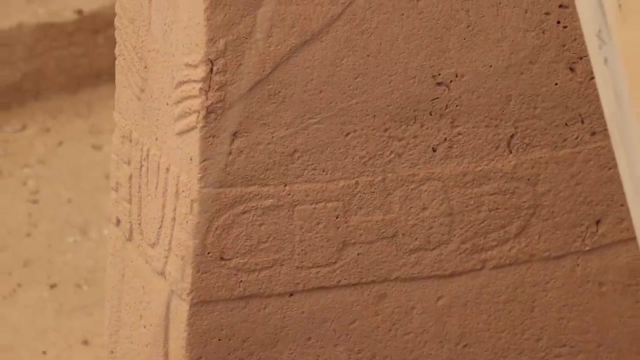 Early agrarian societies needed a high level of social cohesion and management simply in order to motivate their people to get past this first step. Could it be that such powerful bonds were fostered at sites like Gobekli, with feasting as the ultimate social 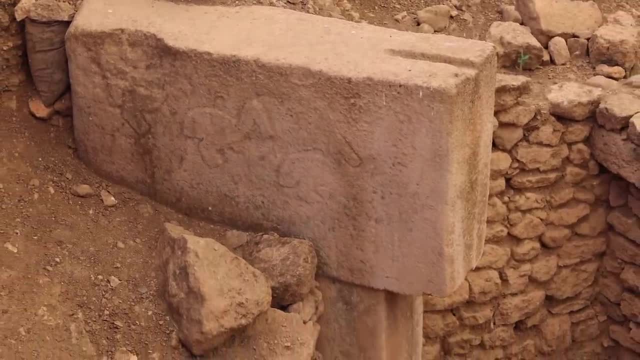 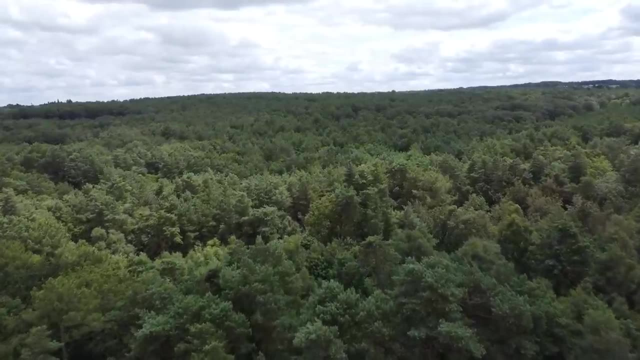 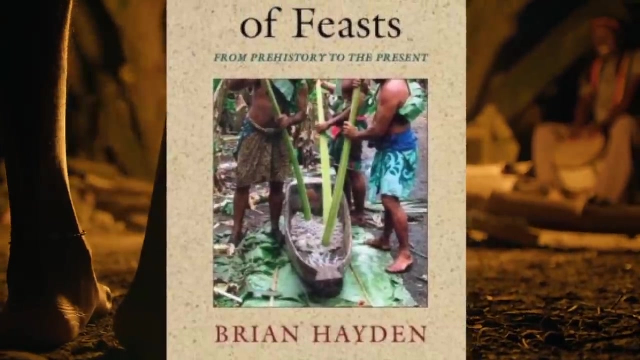 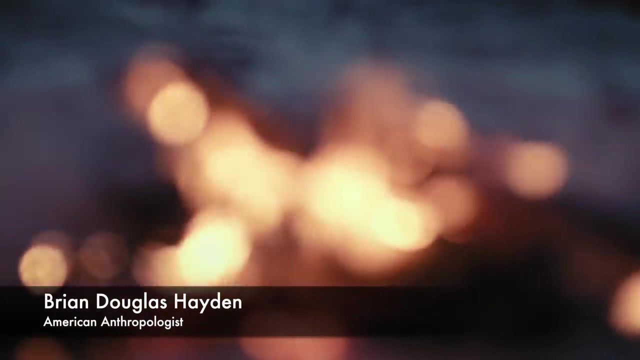 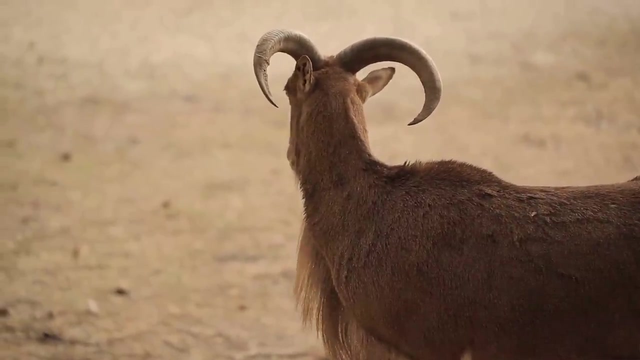 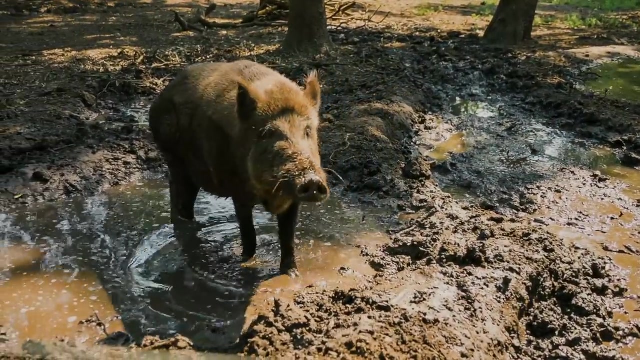 glue Towards the end of the 20th century, basing his ideas on a lifetime of research in the field. anthropologist Brian Hayden took this into consideration in the early 20th century. In the early 20th century there was an enormous demand. 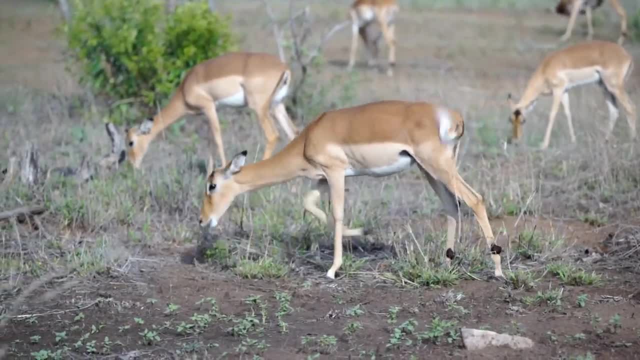 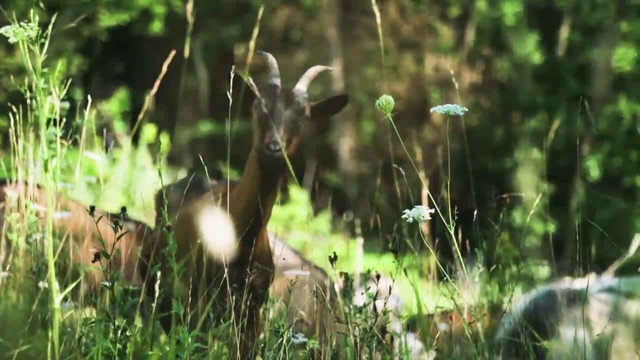 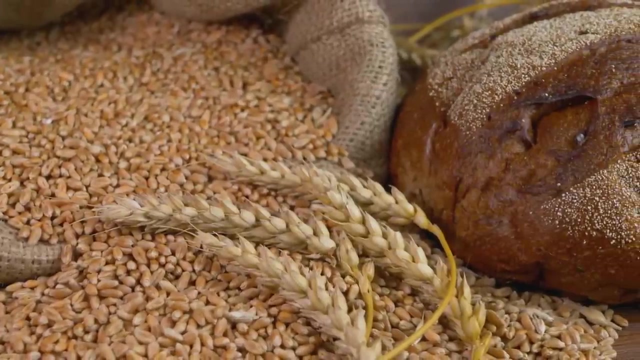 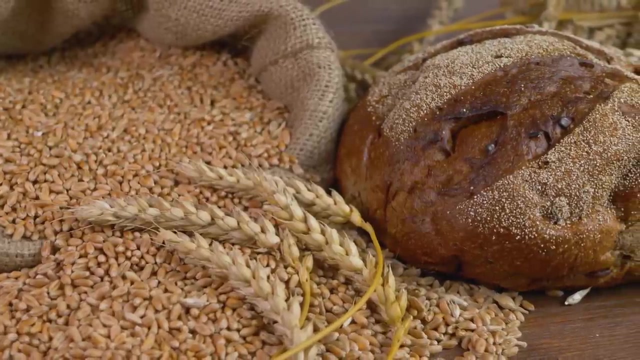 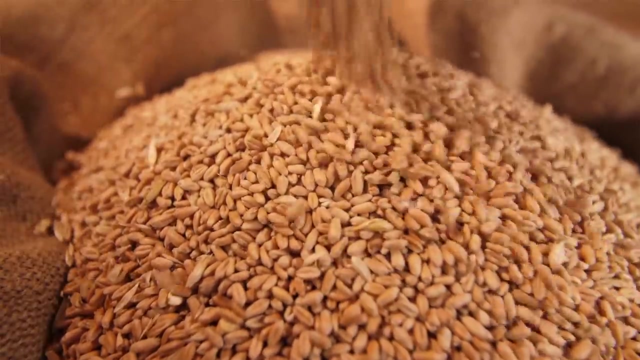 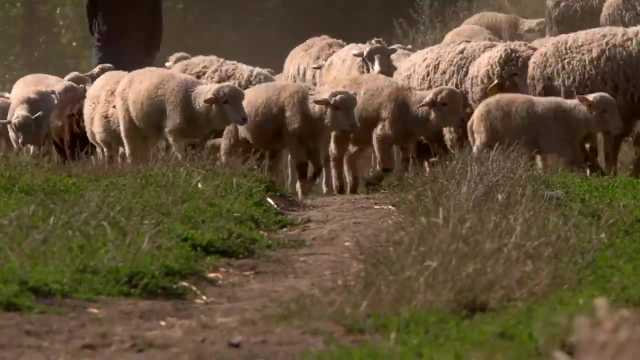 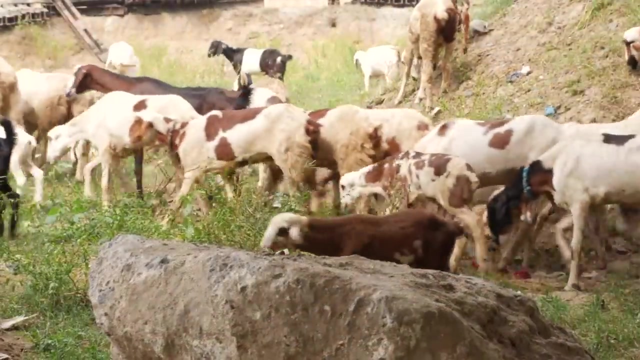 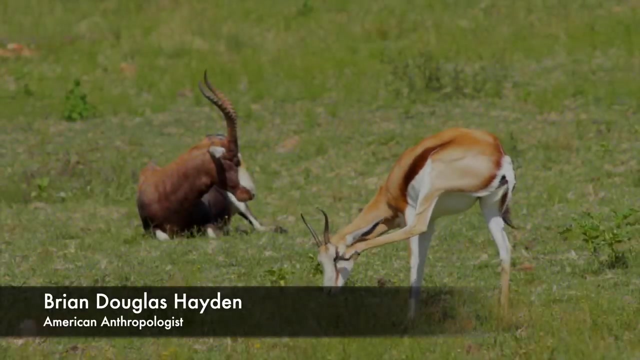 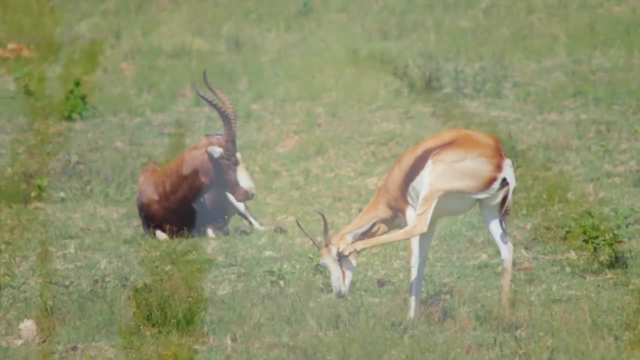 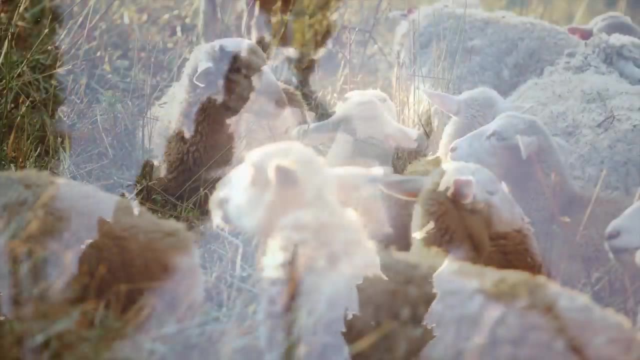 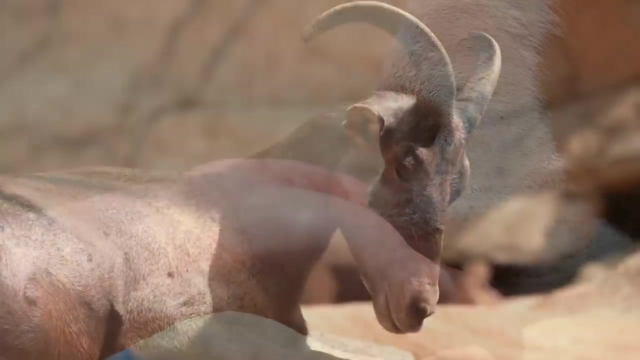 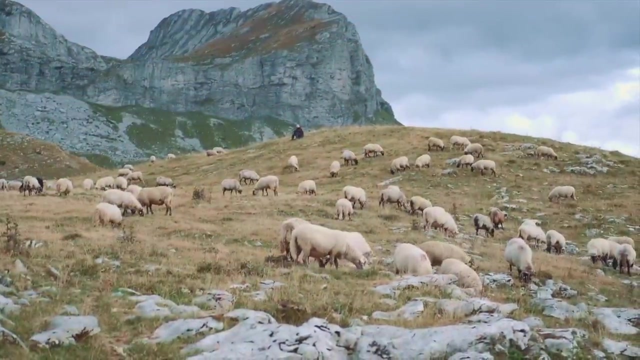 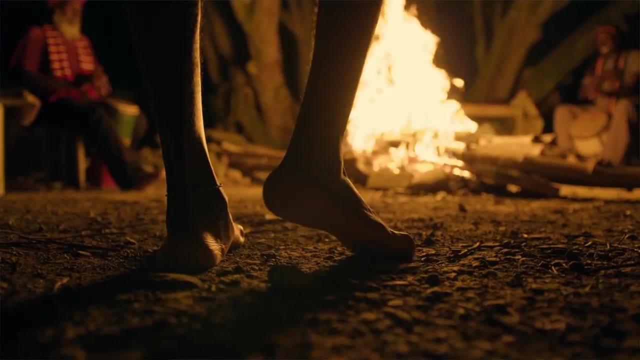 once competition for influence between rivals begins, experimentation in farming is driven forwards, as the potential to produce a much larger surplus is realised. Individuals can then pursue prestige and power through favours owed to them. And yet feasts are clearly not always competitive in nature. The norm 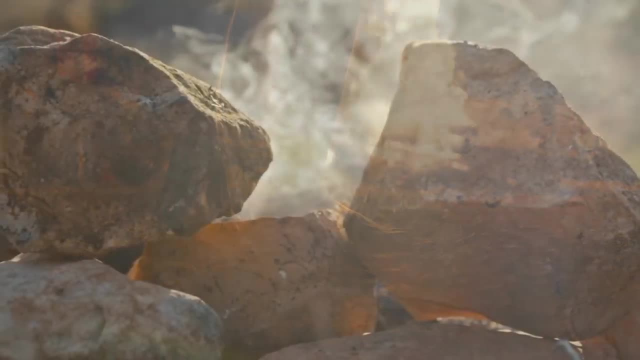 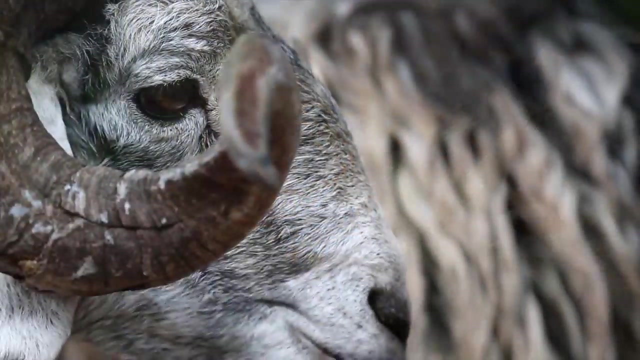 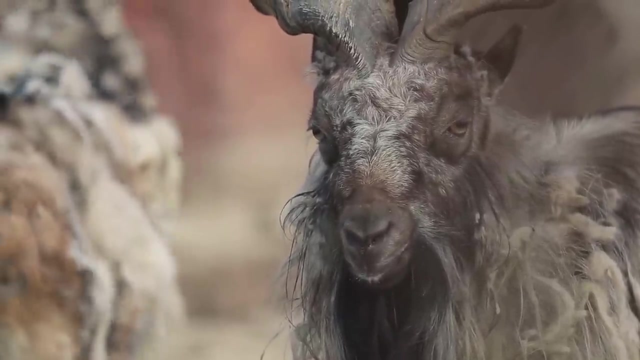 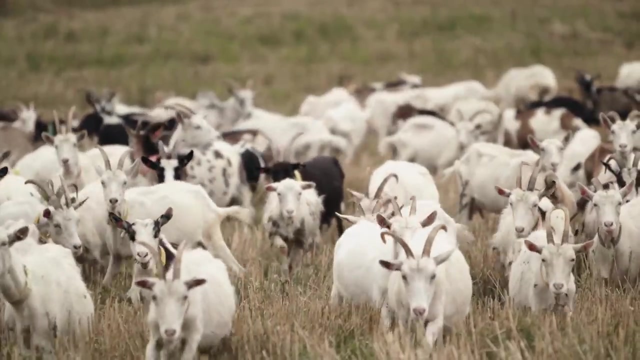 may even have been the complete opposite of Hayden's idea That feasting was egalitarian in nature, aimed at counteracting tendencies towards the formation of unequal hierarchies and promoting the obligatory sharing of food, Though it may well be that feasts had little to do with the harnessing of 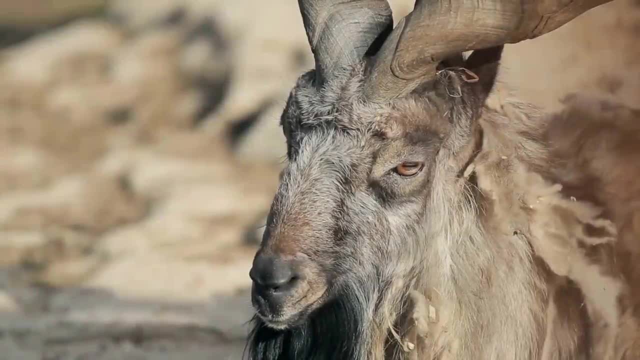 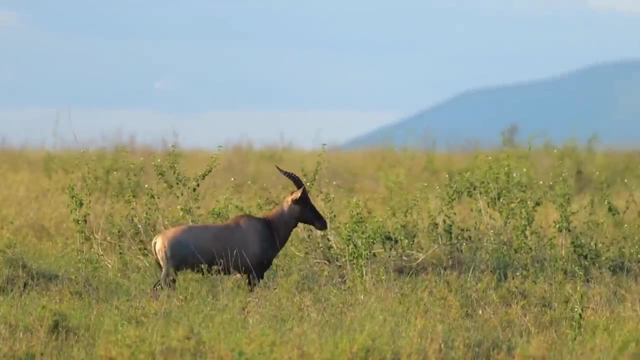 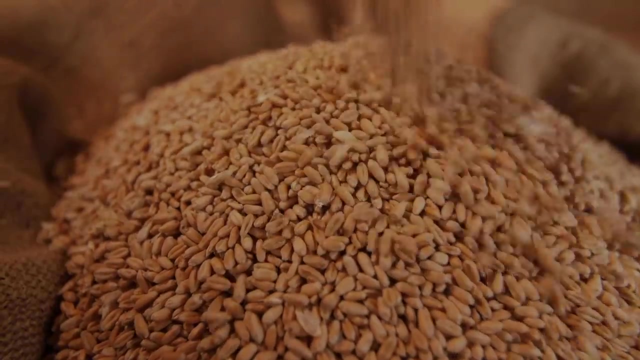 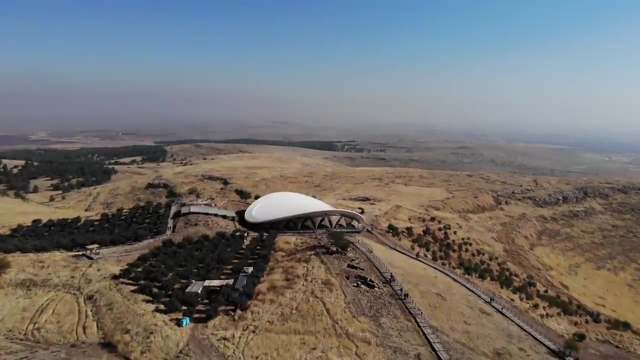 agriculture. After all, animals and grains were all wild at Gobekli Tepe. The origins of agriculture could well be entirely separated from that nearly twelve-thousand year old sanctuary of megaliths. Nevertheless, regardless of the origins of agriculture, it is clear that when 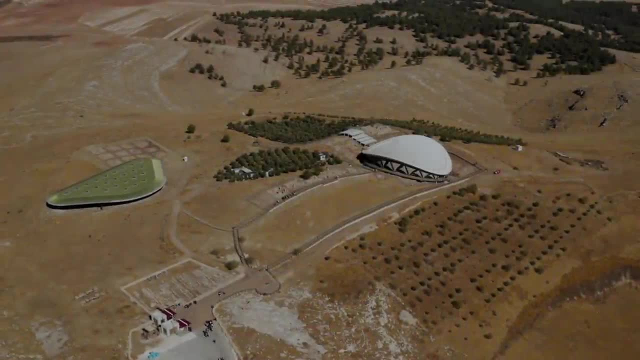 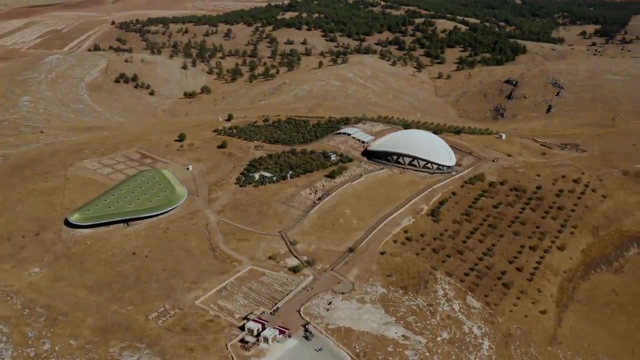 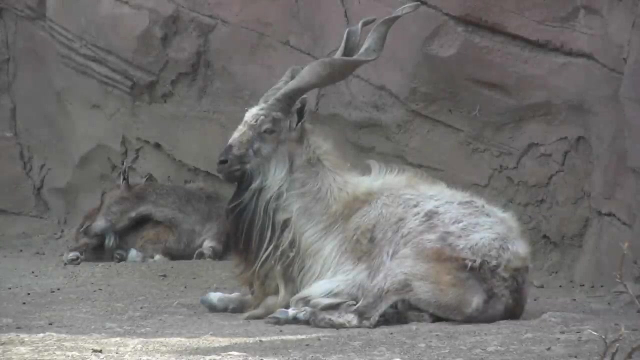 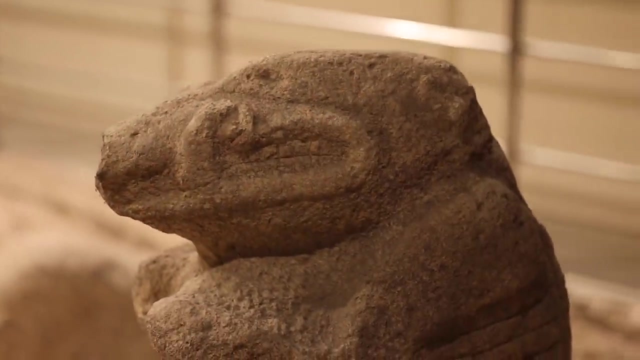 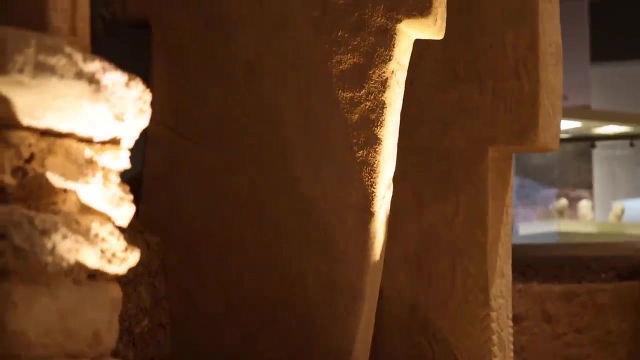 societies knew how to organise their members effectively, they gained the evolutionary advantage: Intentioning like thatø deal of energy going not into obviously productive work or even food producing, but in formulating a sense of unity and shared identity. The emergence of agriculture, then, could be tied to investment in ideology, A greater 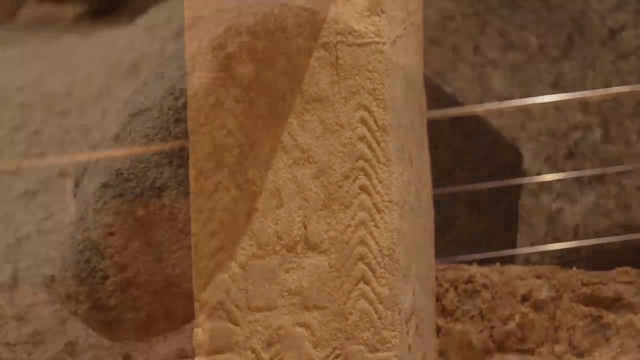 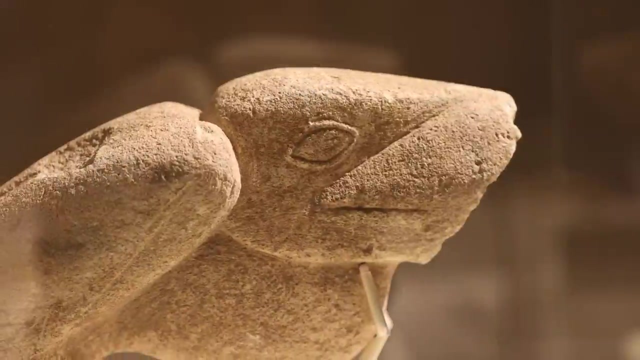 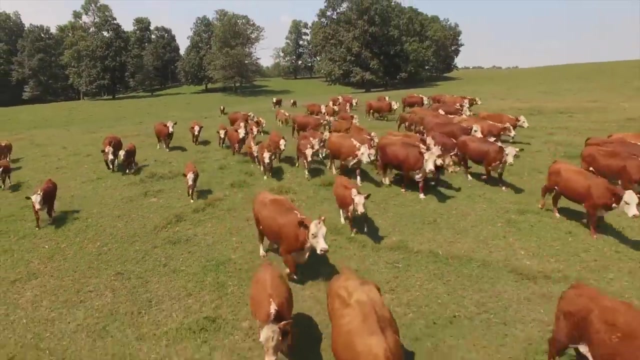 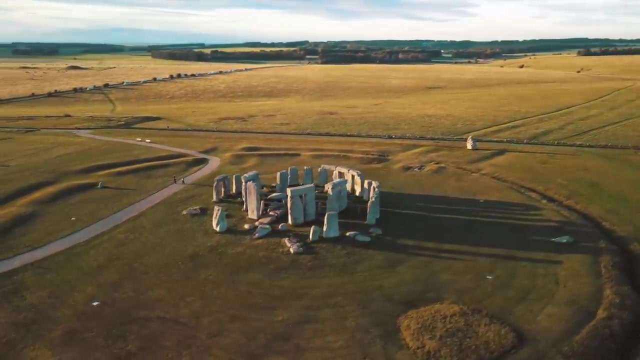 societal good that would allow willingly for the tolerance of inequalities and hierarchy to form The same sort of sentiment that, some 7,000 years later, would lead far-flung people to bring their cattle to Durrington Walls near Stonehenge, Even later at Delphi and 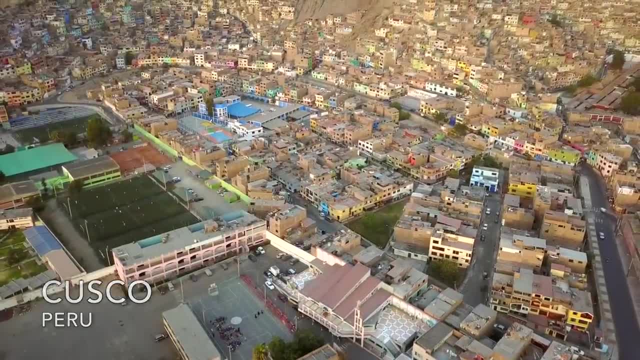 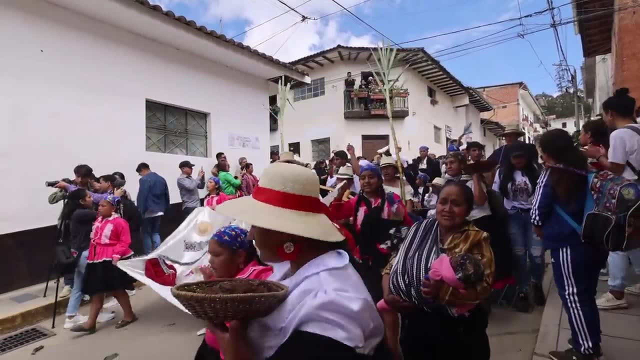 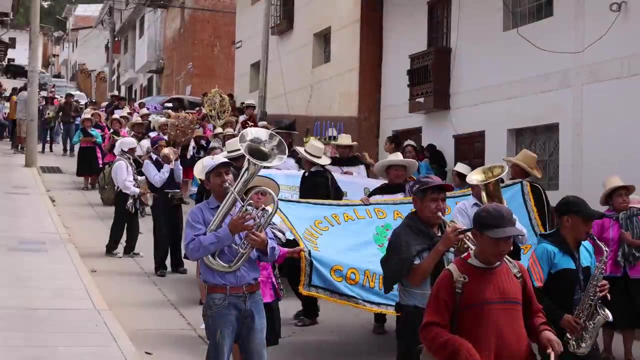 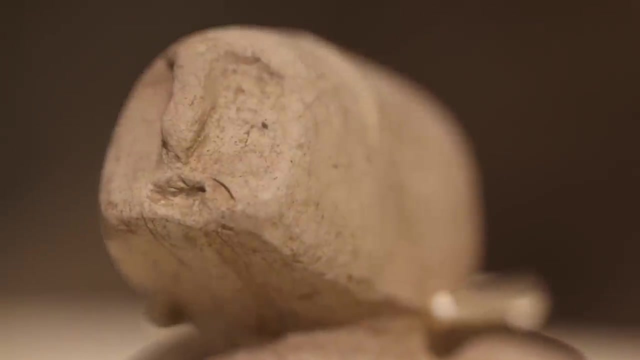 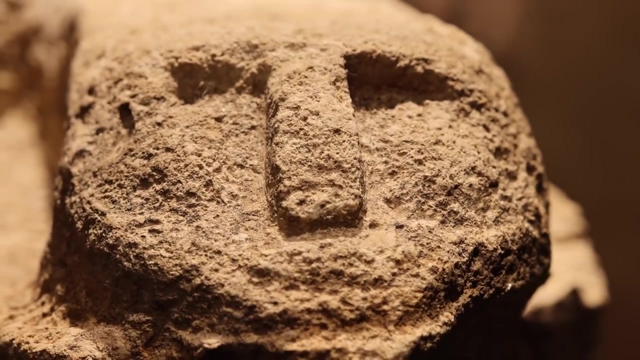 Cusco, And at modern festivals too, where people still go to hear news from neighbours, to meet husbands and wives and to inadvertently spread communal culture. But of course, there is often another aspect to it as well: A chance to burn. 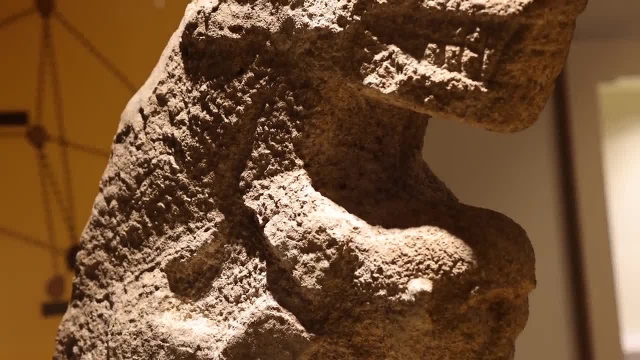 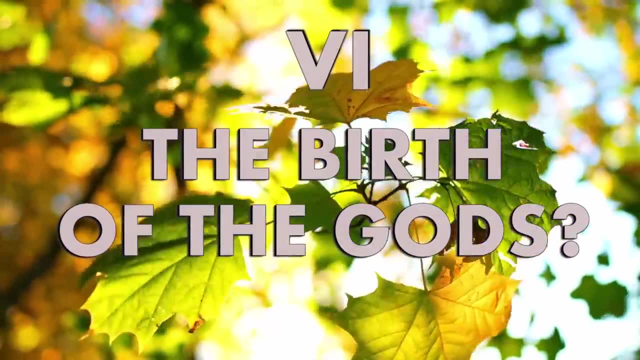 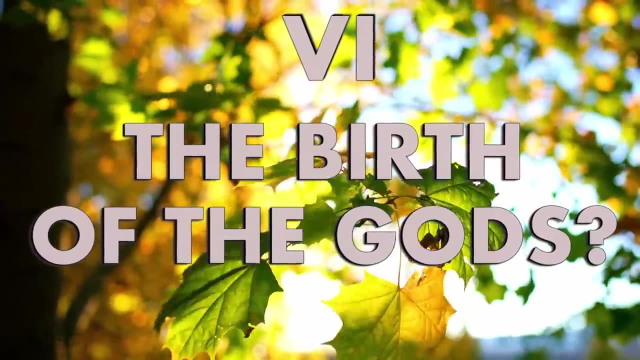 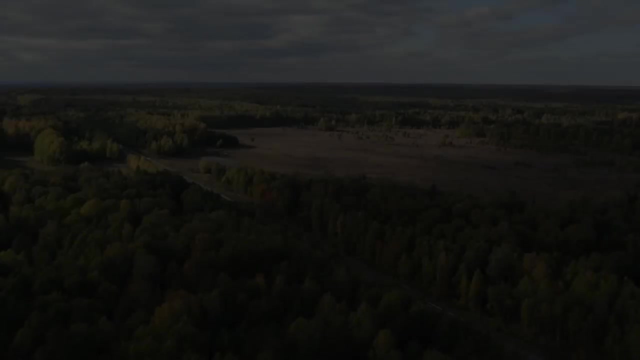 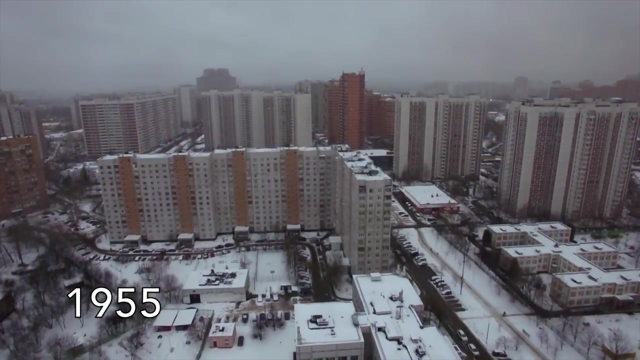 to reason with the other world and the divine. In 1955, Russian quarry workers digging pits some 200 kilometres east of Moscow came upon a man who had been a quarry worker for a long time. They came upon something they weren't expecting. 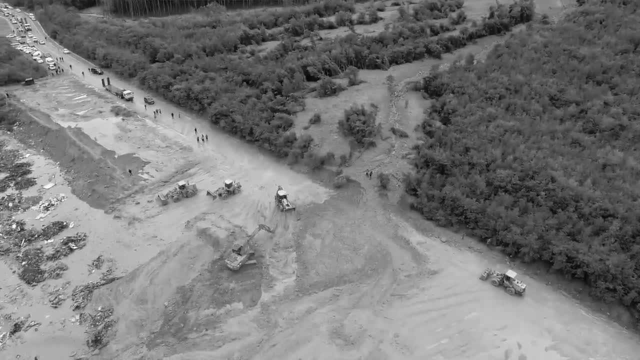 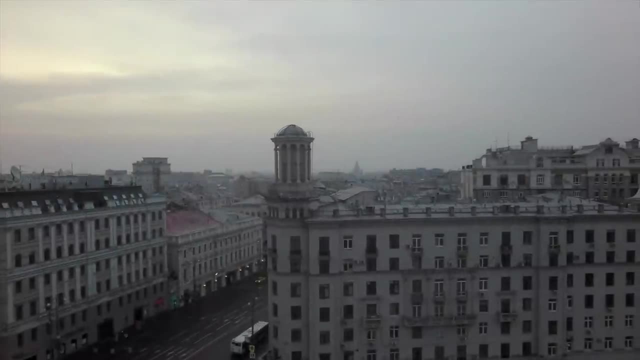 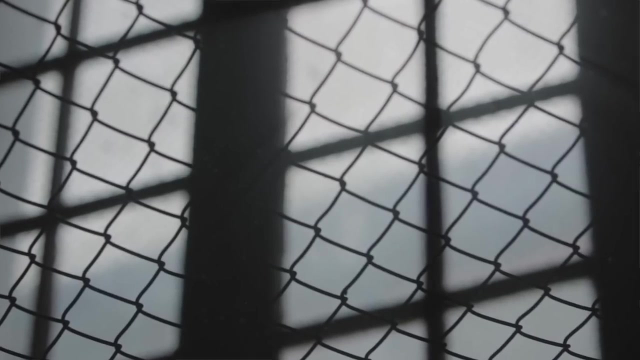 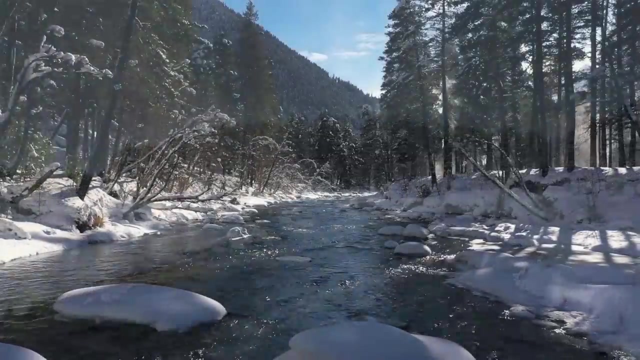 The ruins of an ancient settlement buried in the clay. When the radiocarbon dates came back, the group of experts called in from the Russian Academy of Science could scarcely believe the results. Scattered over five kilometres on the edge of a remote Russian riverbank, 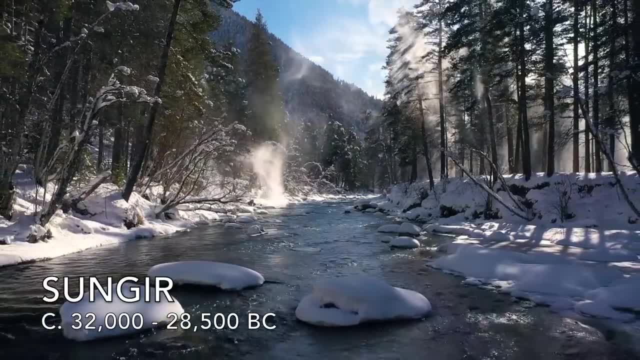 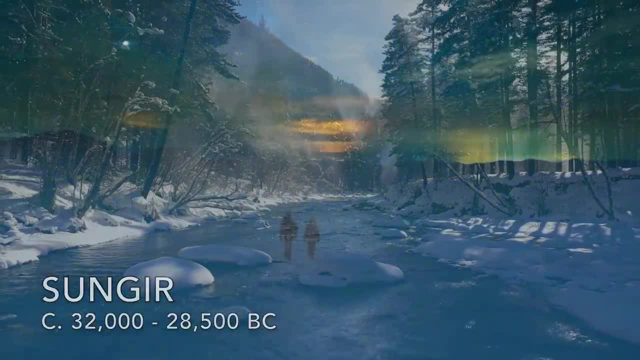 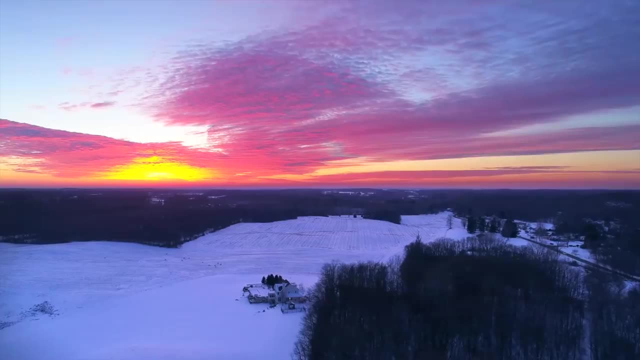 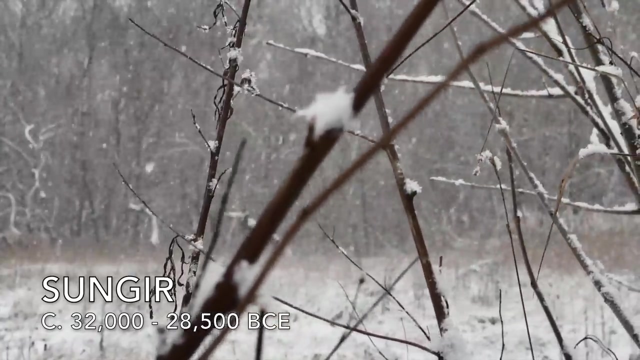 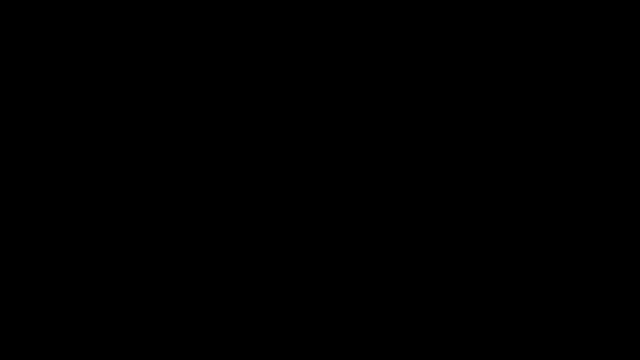 the prehistoric settlement of Sungir turned out to be one of the earliest recorded sites of anatomically modern humans found anywhere in Eurasia, Dating to somewhere between 32 and 28,000 BC, Though still largely unknown in popular culture, particularly in the West, due to the disconnect of the Cold War. 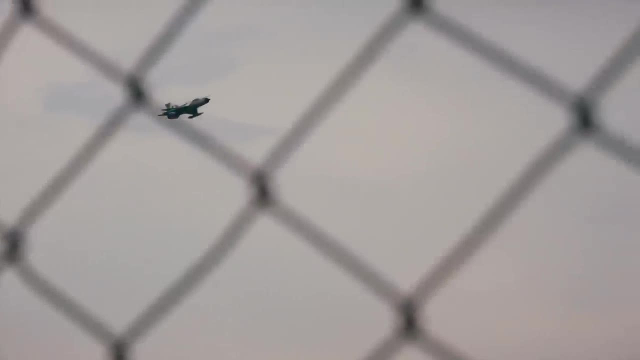 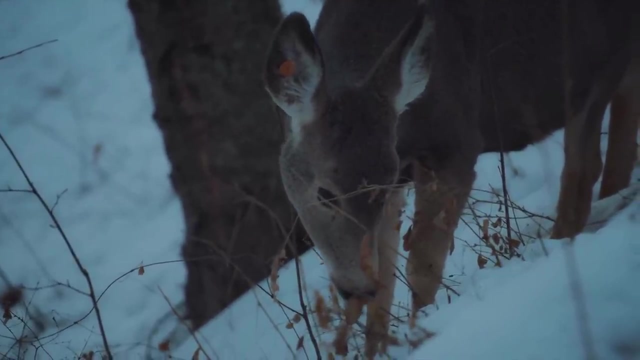 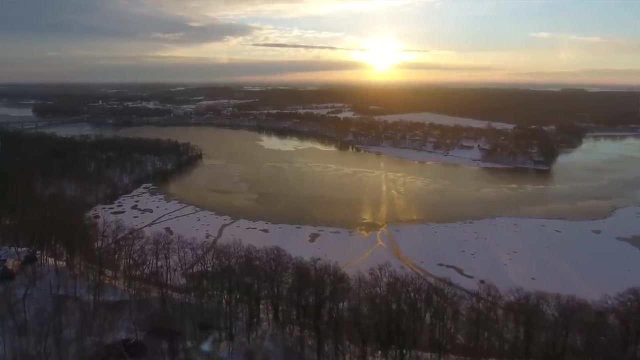 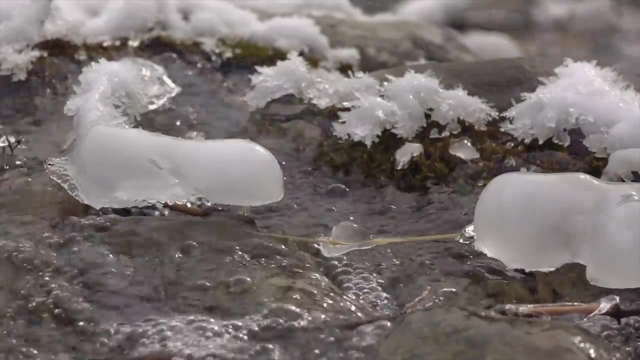 over the next 20 years of excavations, the wildly significant discoveries kept coming in, Perhaps most astonishing of all, both in terms of their state of preservation and their use in the world reservation. and their contents were the grave sites, also some of the earliest ever. 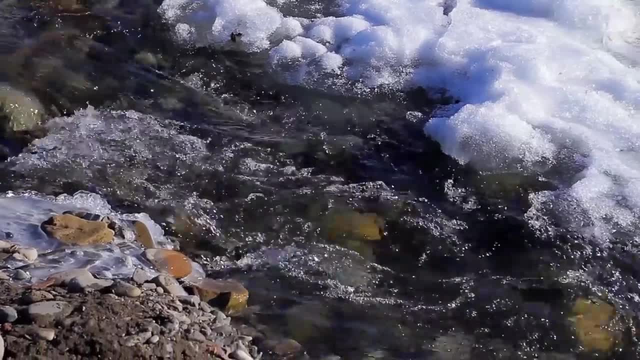 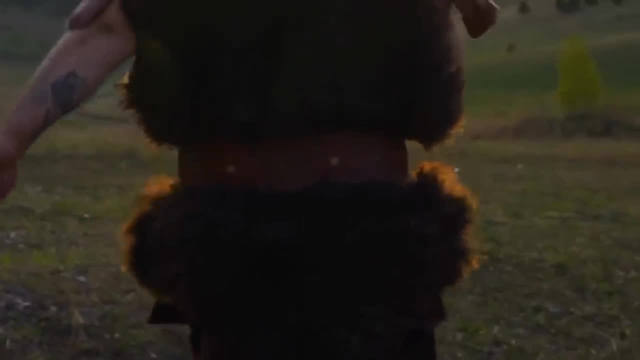 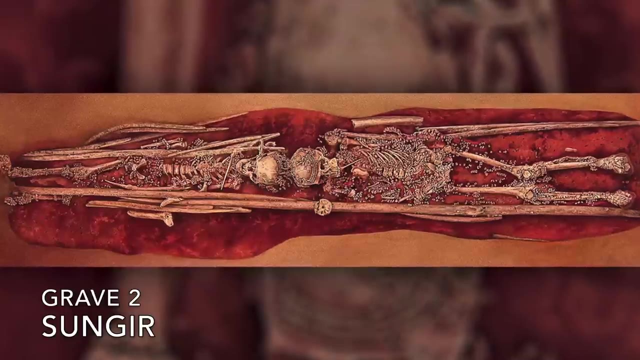 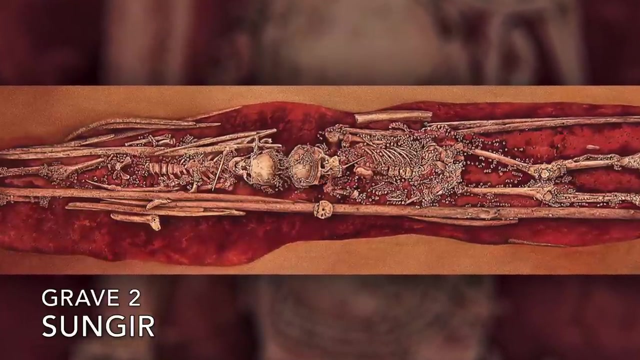 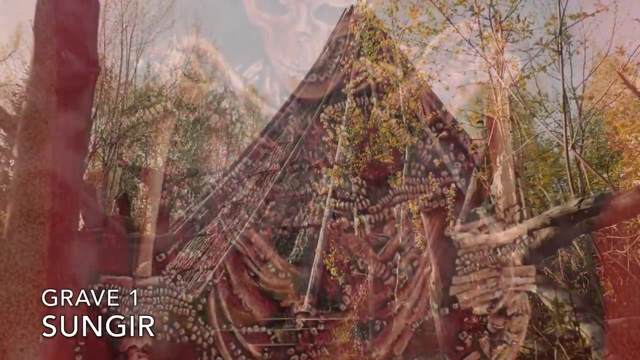 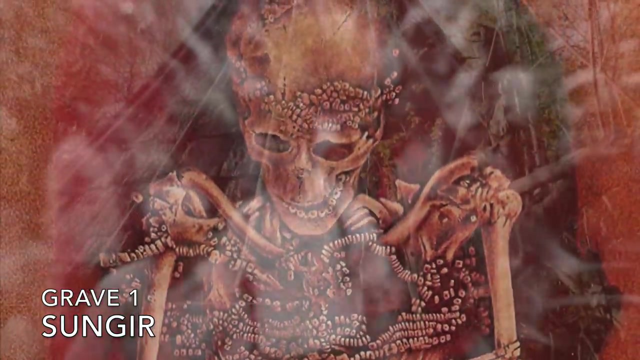 found in Eurasia and, as we shall see, among the most unusual. Grave 2 consisted of a pair of adolescent children laid down facing one another head to head, along with an adult leg bone filled with ochre. Grave 1 contained an adult male, similarly coated in red ochre, a substance associated. 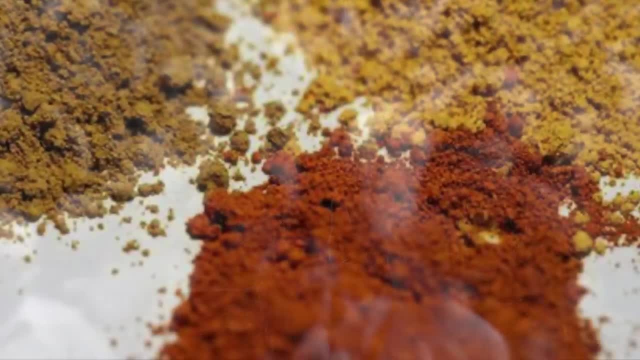 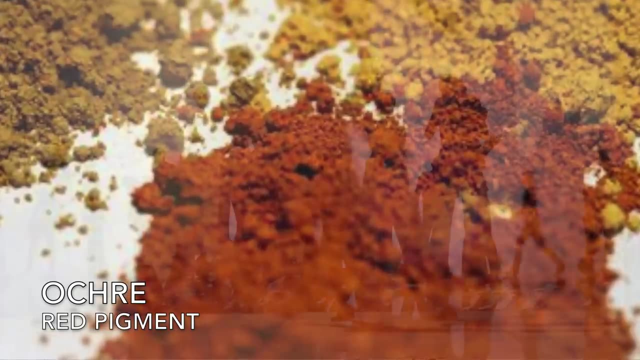 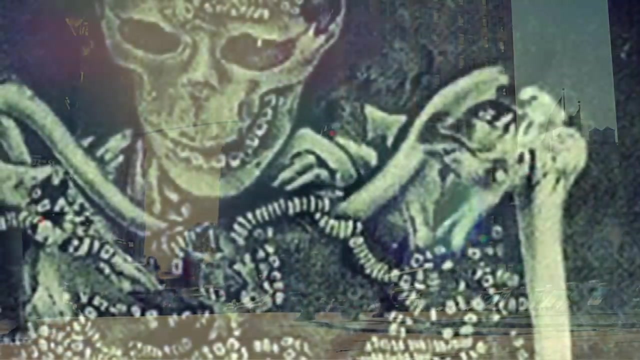 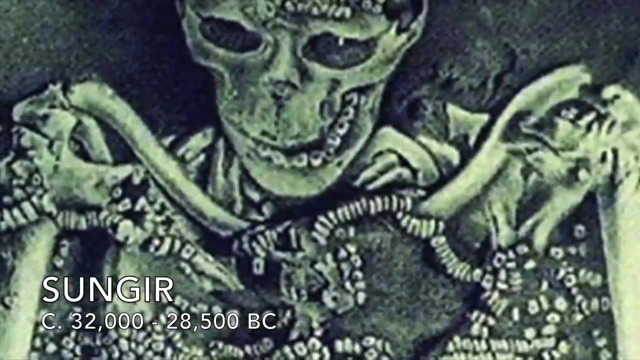 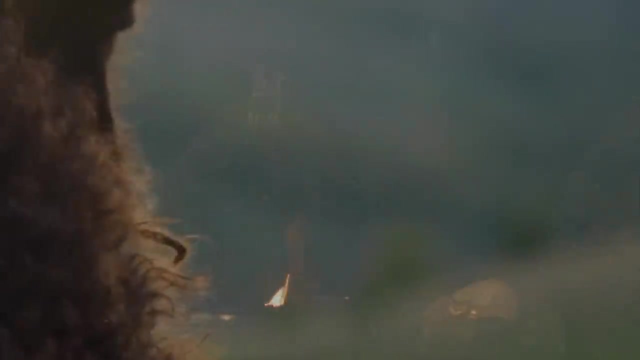 with religious rites, Massacres and death rituals took place and the bodies were resembled. But most amazing of all were the thousands upon thousands of intricately crafted pieces of jewelry, clothing and spears, among other items, Quite literally coating the bodies. 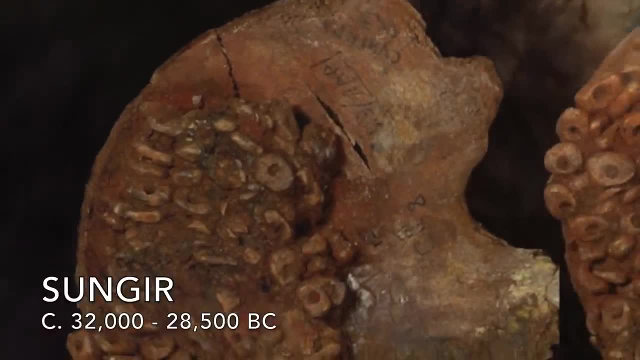 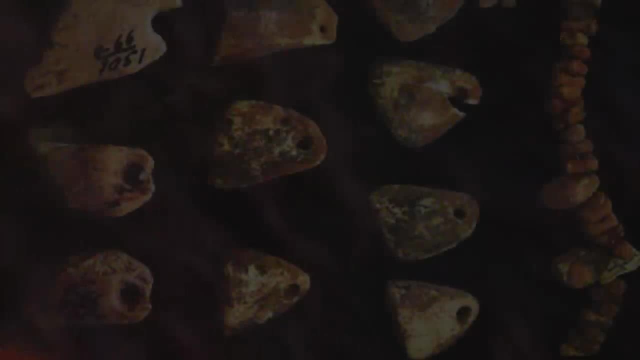 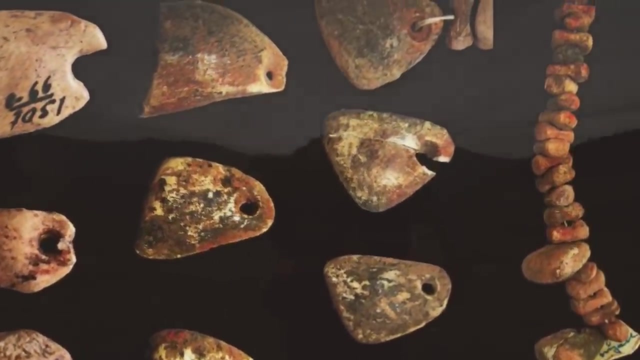 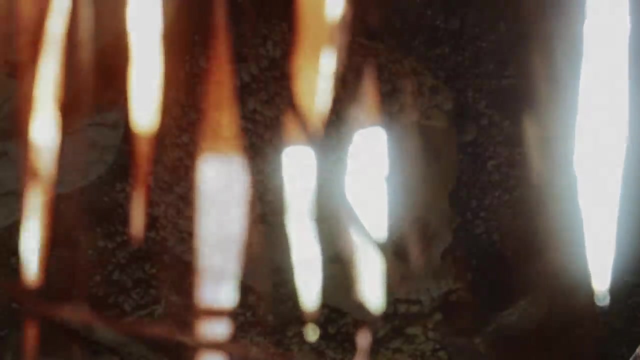 One single piece of clothing, Some 13,000 beads in all, having been uncovered, An artistic effort that would have taken an estimated 10,000 hours to produce A truly vast investment, As well as being taken as some of the earliest direct evidence. 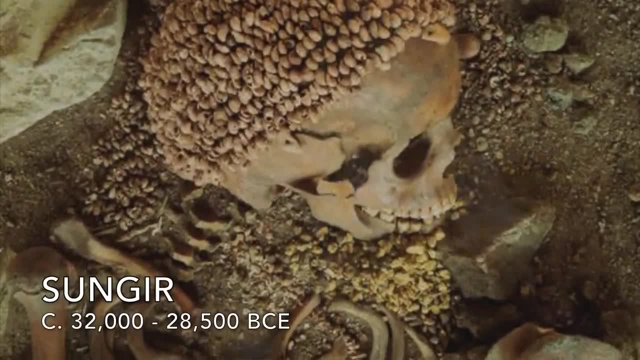 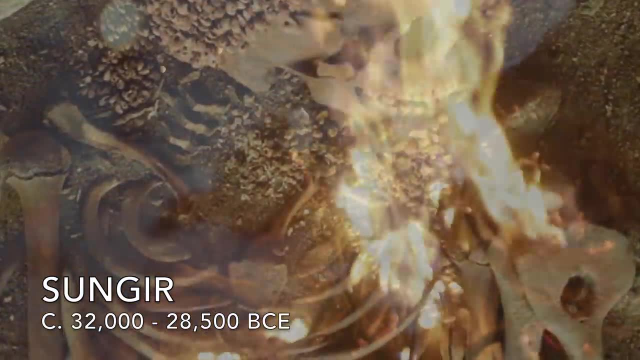 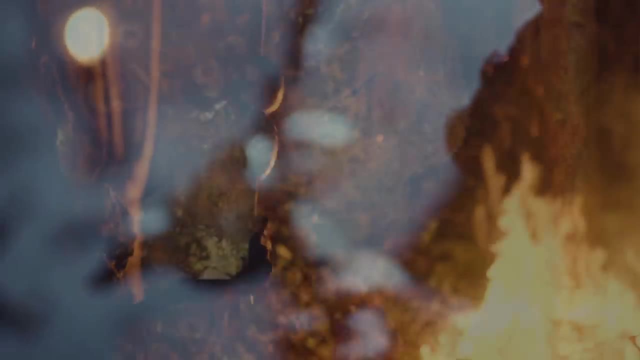 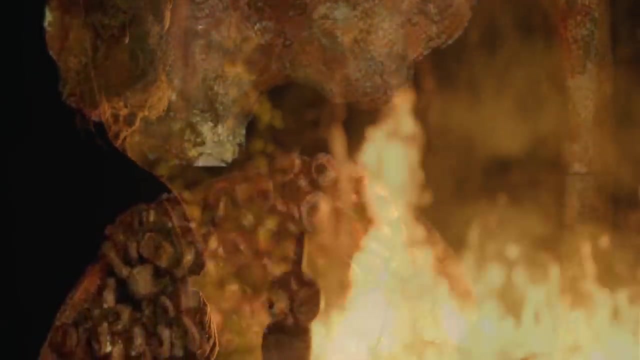 for religious practices in Eurasia. the Sungir burials are also often seen as a particularly early example of highly developed systems of rank existing deep in the Paleolithic past. It is a view further bolstered by a similarly ancient find in Italy known as El Principe. 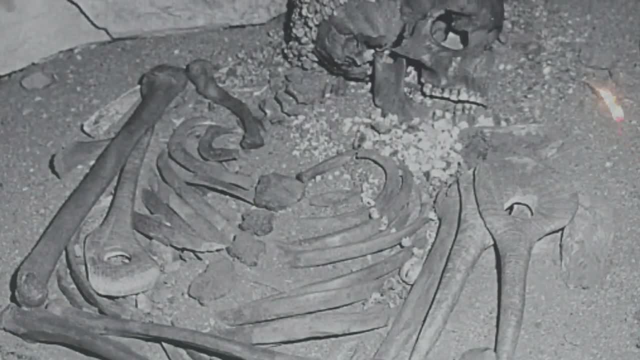 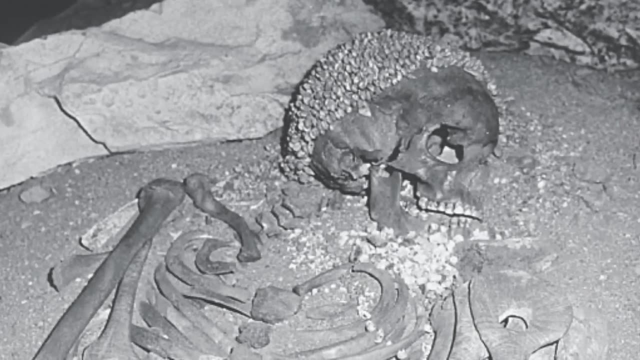 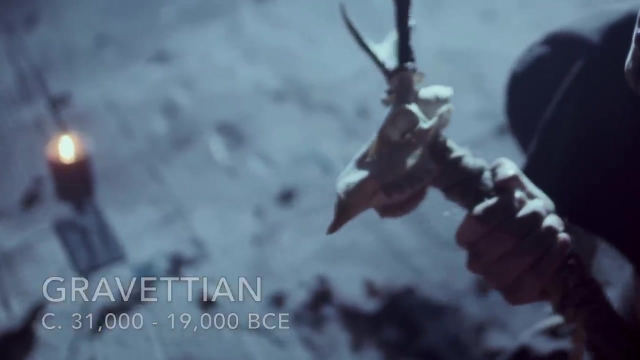 Adorned with a similarly incredible array of grave goods. And yet further investigations into Paleolithic burials, from the Aurignacian to the Gravettian to the Magdalenian, from Spain to Russia, to the Levant. 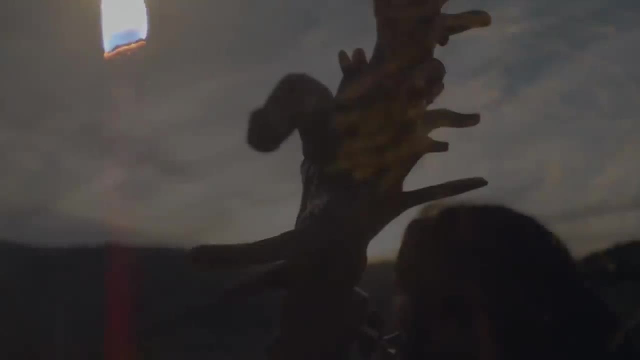 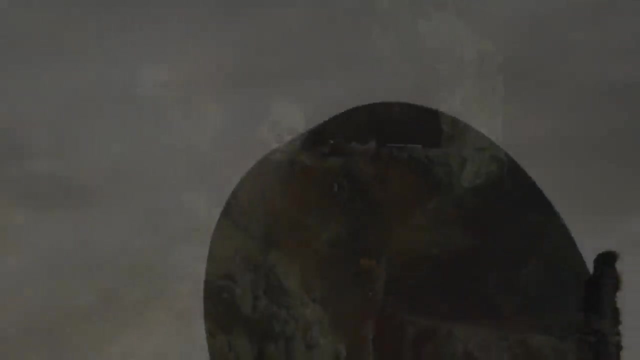 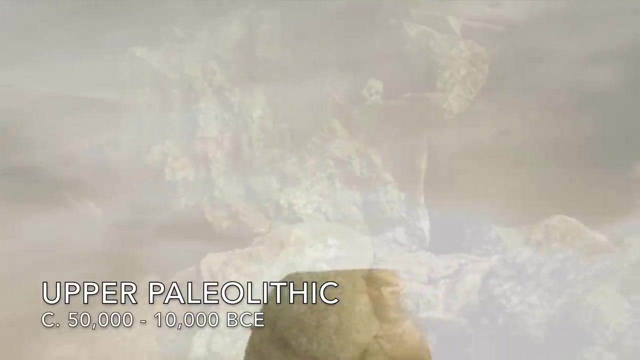 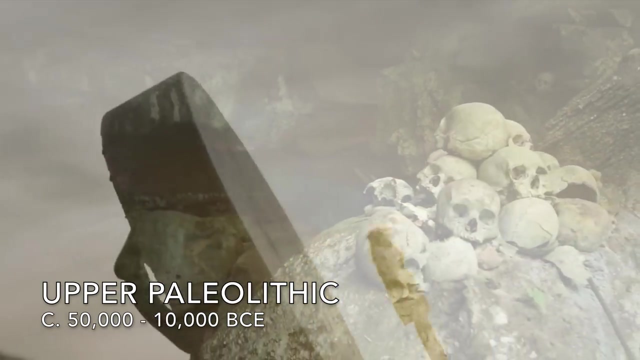 may hint at more unusual reasons for having such ornate burials. After all, no fortifications, storehouses, palaces or any other evidence of conventional chieftains have been found, Let alone anything resembling a state that we would recognise. 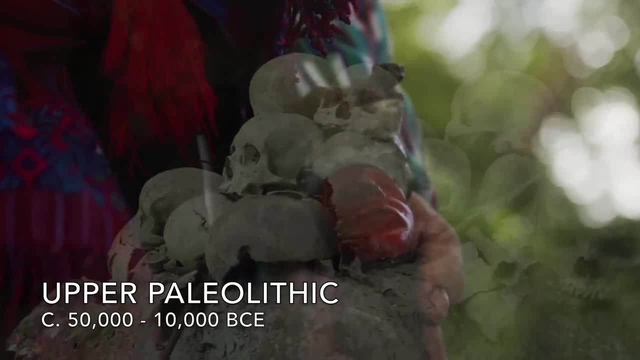 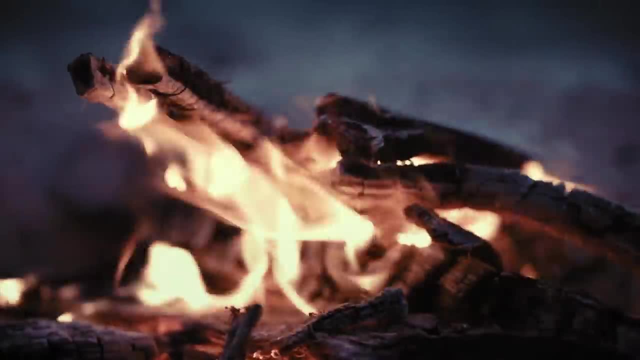 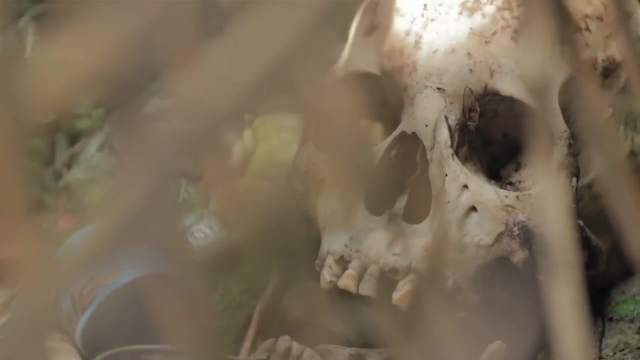 Elsewhere in Eurasia during the Paleolithic, a striking number of burials have been found. The burials contain individuals with unusual physical characteristics, Sometimes placed in striking and unusual poses, Spiralling outwards, crouched or laid out facing other deceased individuals. 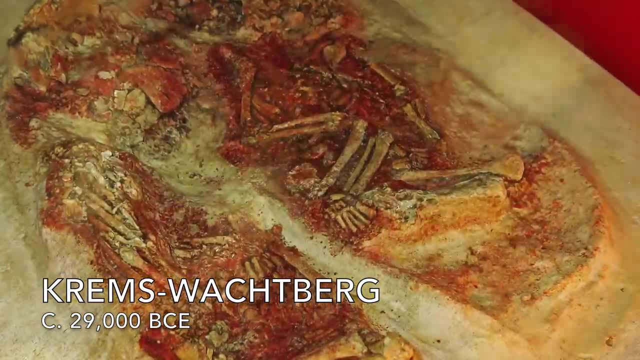 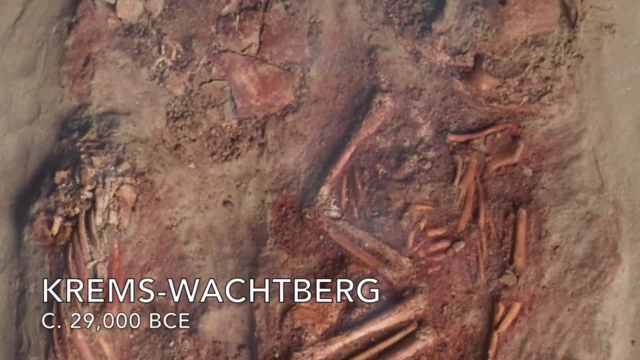 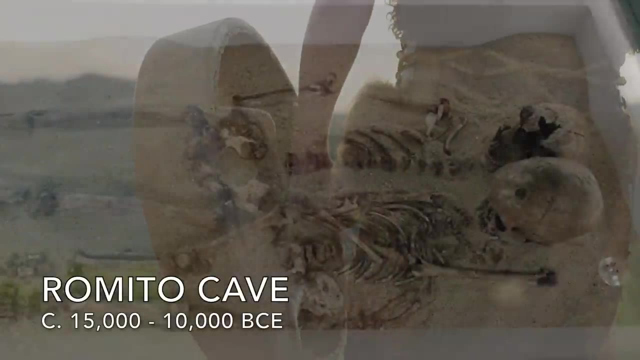 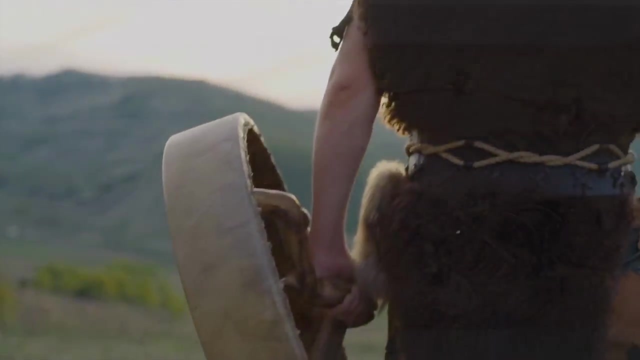 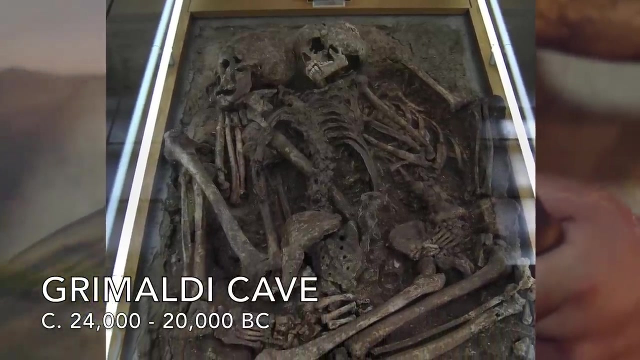 At Krems in Austria, identical twins were found, Their bodies flanked by great mammoth tusk lances And coated in beads and ochre. At Romoto in Calabria an individual with dwarfism was discovered, And at Grimaldi Cave an extremely tall individual with gigantism was given special care. 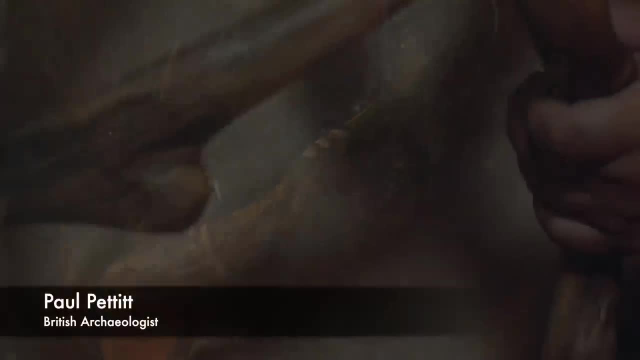 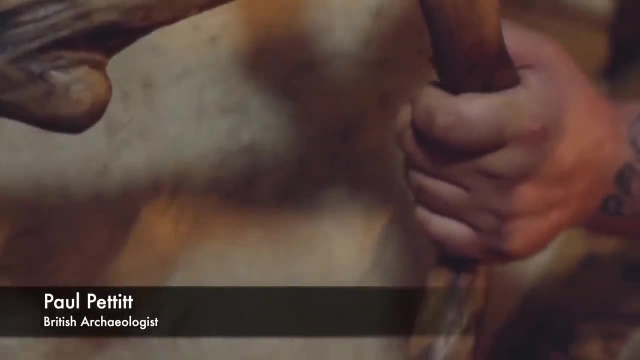 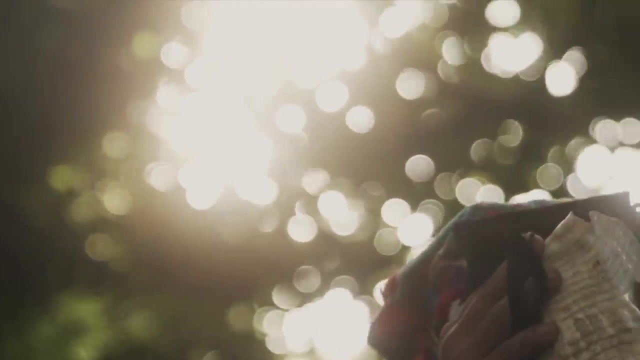 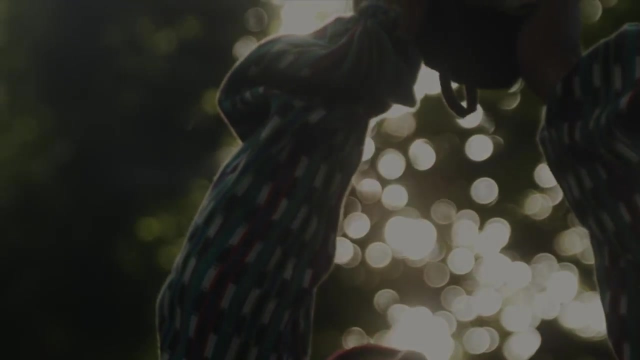 In recent decades, British archaeologist Paul Petit has argued for significant efforts being made by those interring the dead to pin certain deceased individuals down With mammoth bones, wooden planks, stones or vast amounts of decorated ornaments, Often tightly binding the bodies in place. 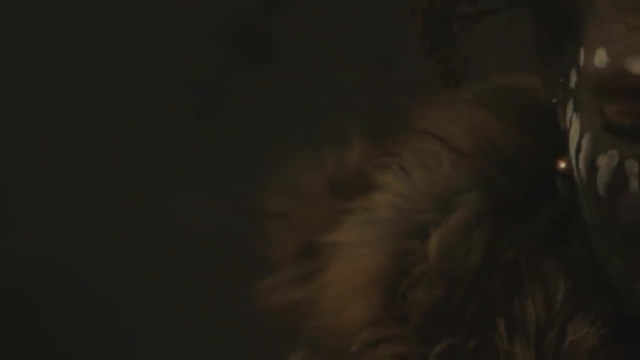 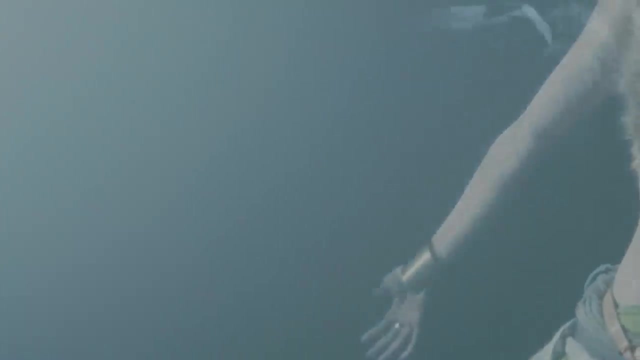 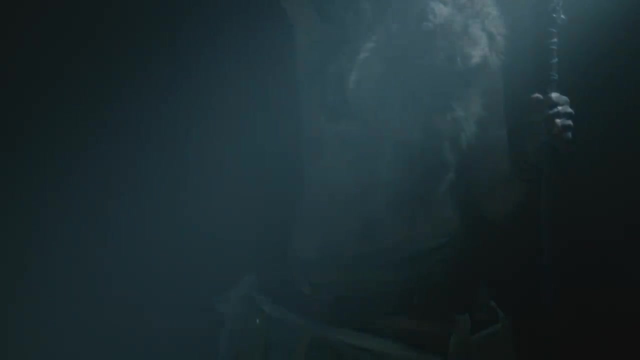 Rather than reverence, the evidence sometimes suggests more a culture of fear, Just like in societies throughout history, lasting well into the modern era, mourners perhaps beseeching the dead to stay in the afterlife, Even making certain precautions to stop them from coming back. 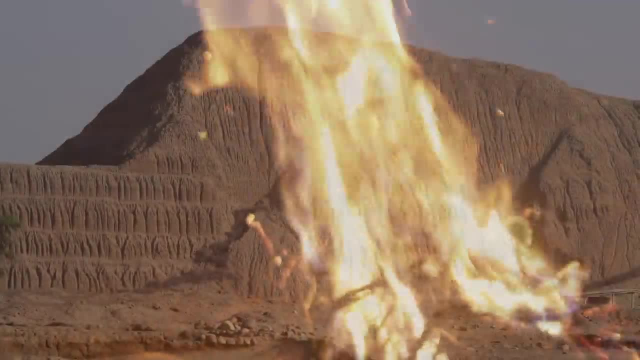 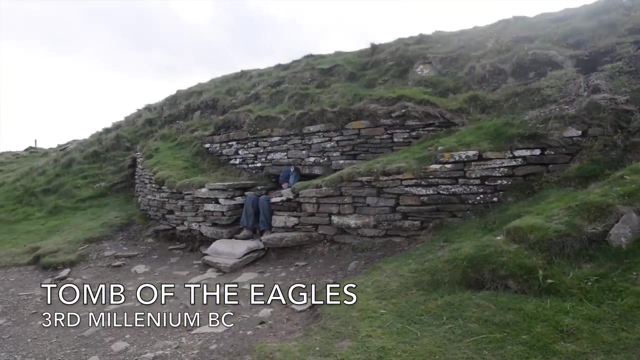 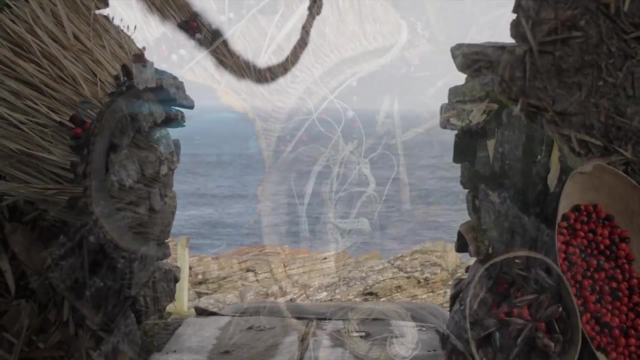 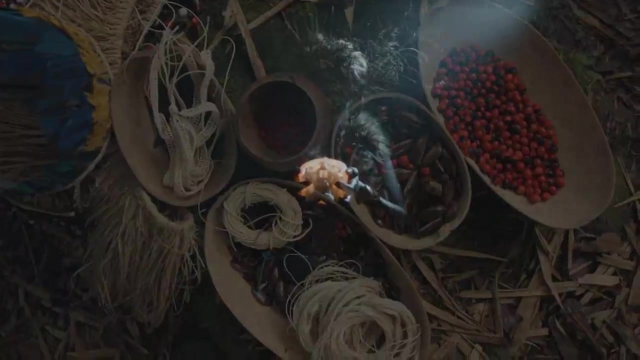 The history of the human race is a mystery, From the Moche pyramid builders of the Peruvian coast to the passage graves of Neolithic Orkney. Throughout history and all over the world, Particularly in ancient shamanistic societies, Individuals who are different in some way, either mentally or physically, have often been thought to possess unusual. 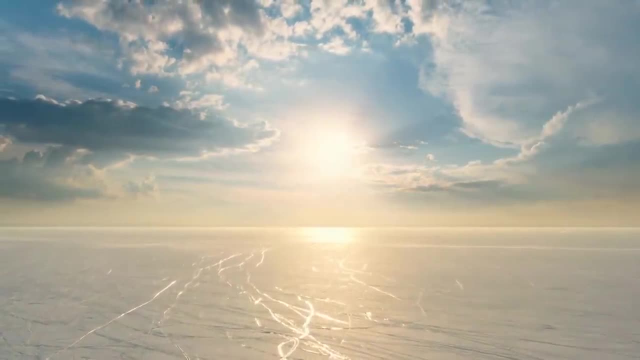 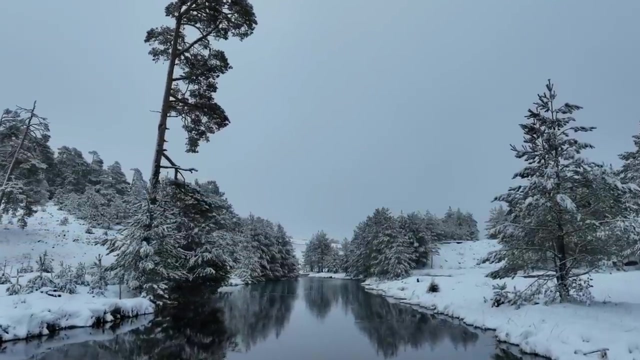 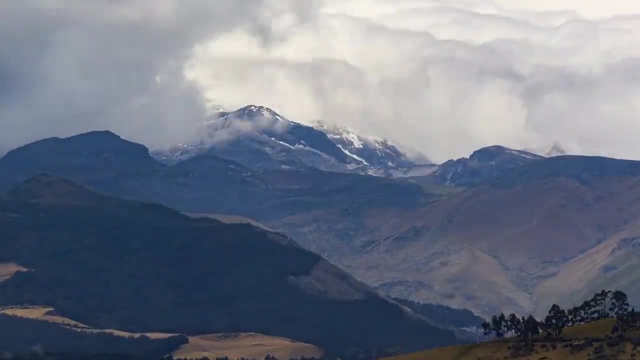 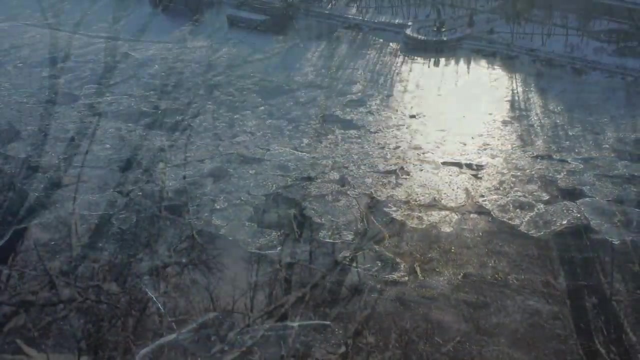 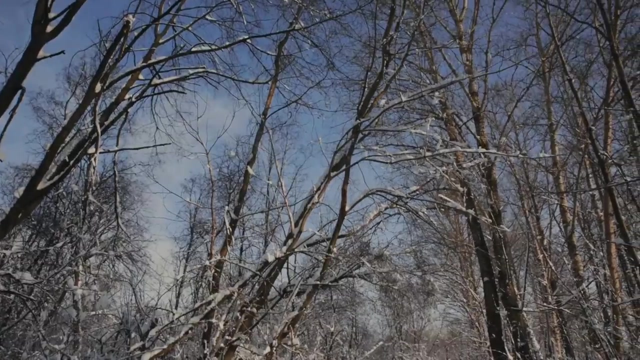 or screwing things up Unusual. Unusual, unusual supernatural powers deemed closer to the gods. Perhaps the so-called princely burials might have been different in some way too. Maybe they were albino, autistic or another genetic condition otherwise unseen in the archaeological. 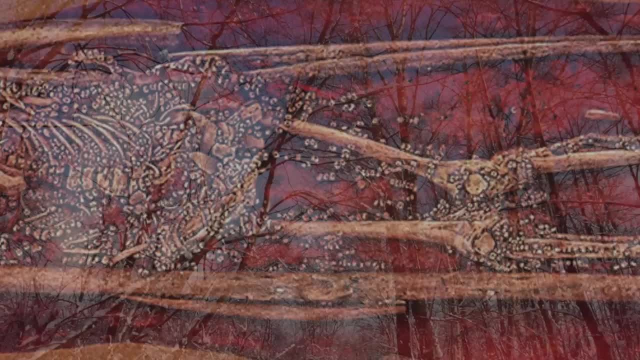 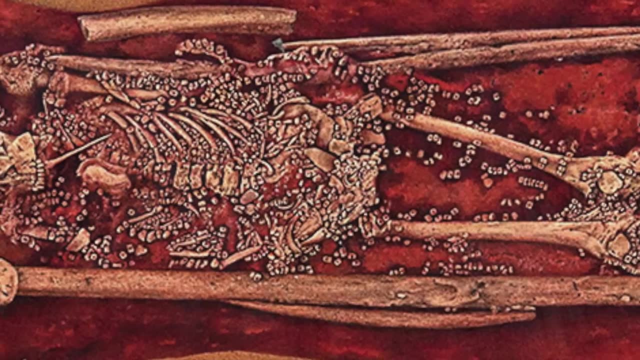 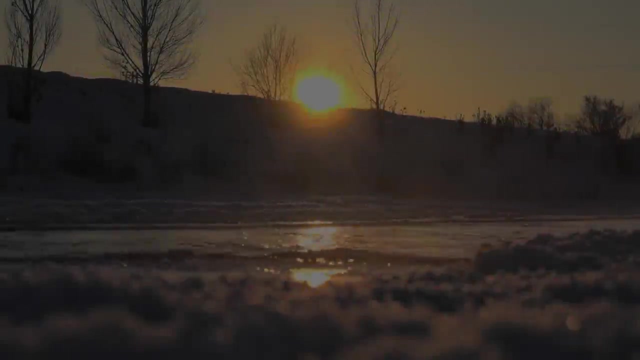 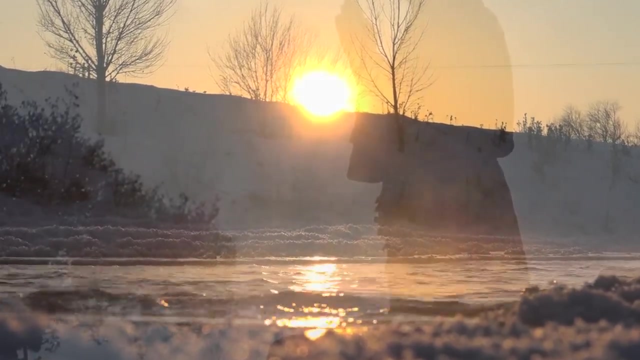 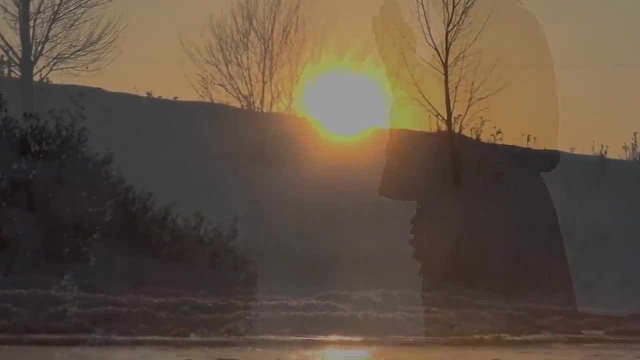 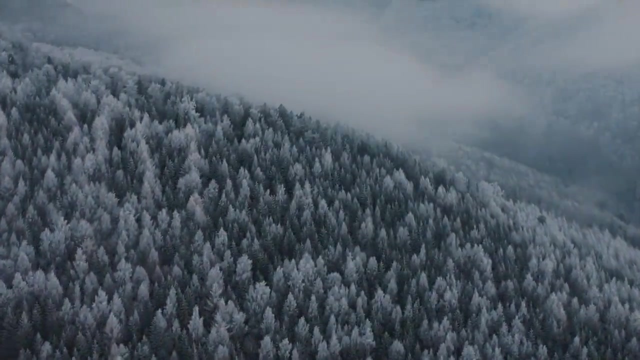 record Weighed down with objects to celebrate them, but also maybe to contain their dangerous powers after death. Just maybe they are evidence of some of the earliest shamans in human history, Turning back to the mammoth hunters of the Moravian Hills. a number of burials were also. 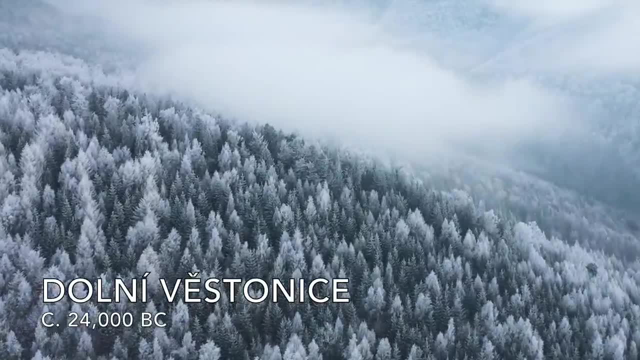 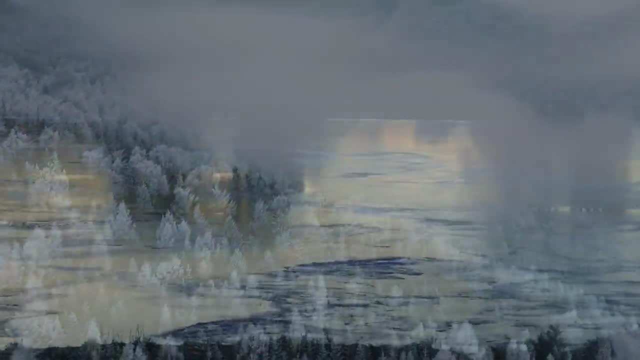 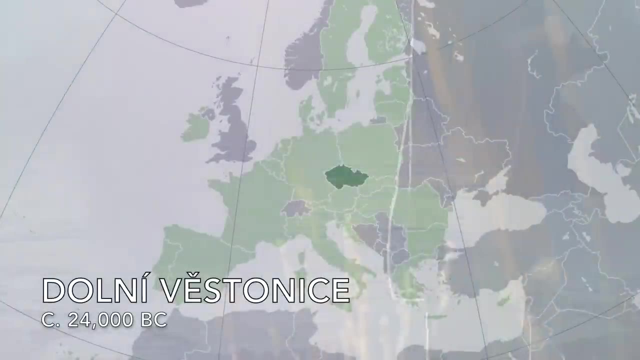 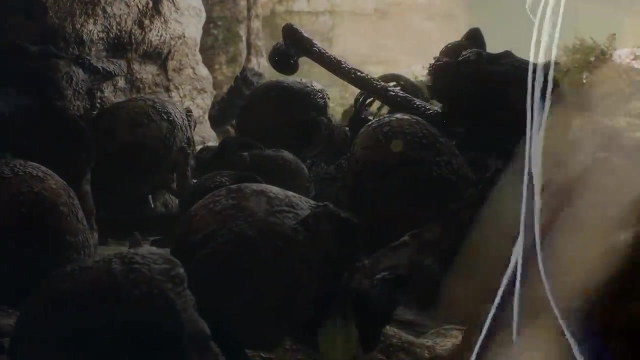 found at the site of Dolni Vesta, Nice, one in particular deserving special mention. Absolutely coated in ochre, laid to rest beside a mighty mammoth bone and with a hand resting on a fox, the remarkably complete skeleton of a woman around 40 years old was 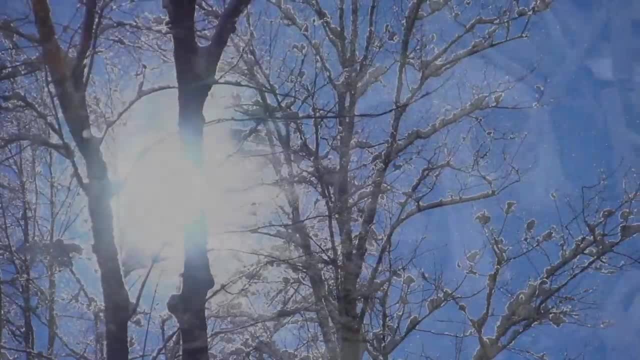 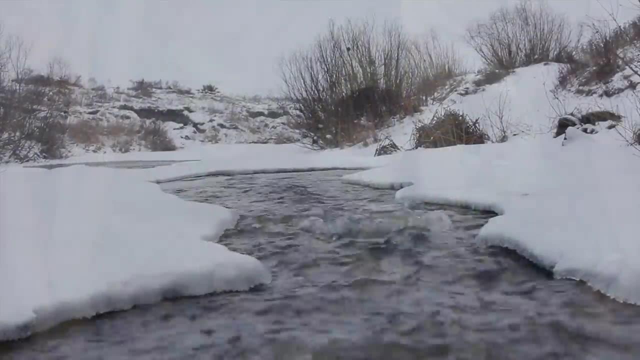 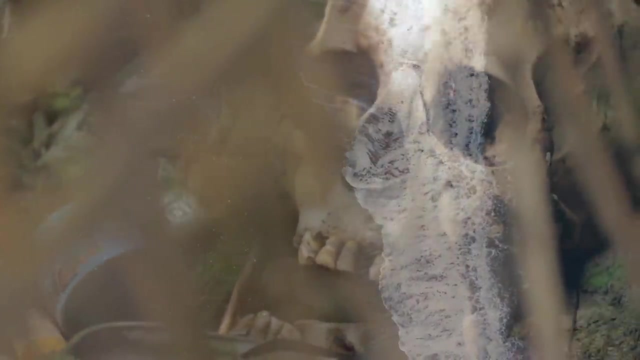 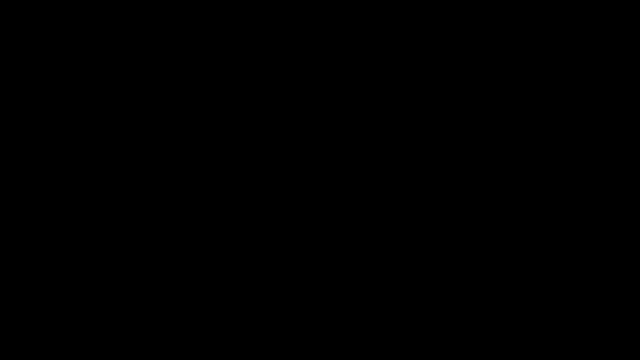 found And, like the other Ice Age burials of the Paleolithic, she had several striking features In addition to her relatively advanced age, old enough to have been a grandparent from birth. the left side of her face had very visible deformities. 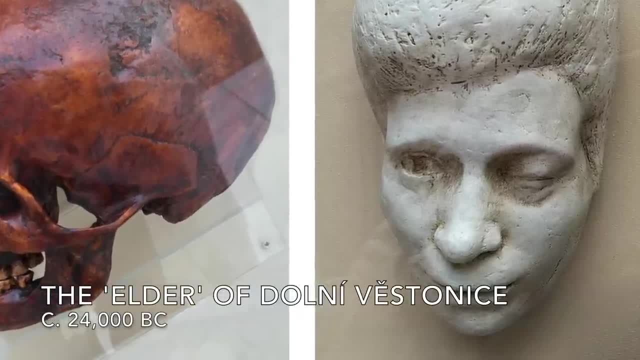 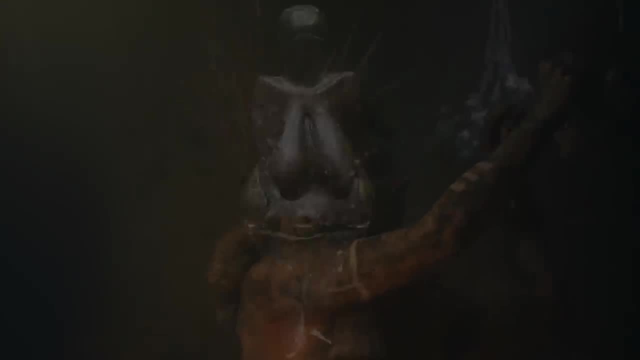 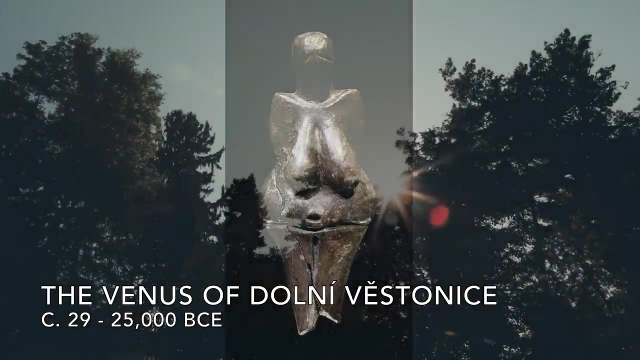 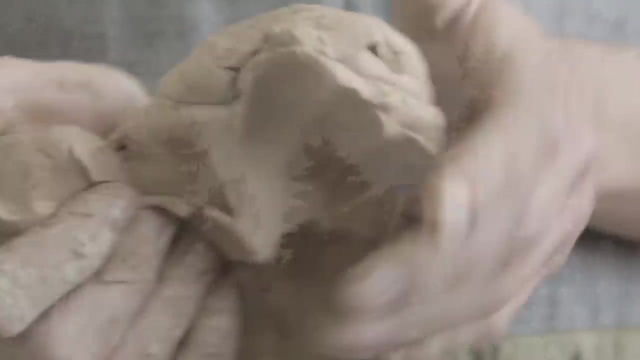 Was this so-called elder of Dolni Vesta Nice considered to be touched by the gods? As we have seen in the video, the figure of Dolni Vesta Nice was also found around the site, including an isolated spot around 80 metres upstream containing well over 2,000 clay figurines of various animals, Most of them in fragments. The figure of Dolni Vesta Nice was found in the late 18th century. As we have seen, a number of Venus figurines were found at the site, including an isolated spot around 80 metres upstream containing well over 2000 clay figurines of various animals, Most of them in fragments. 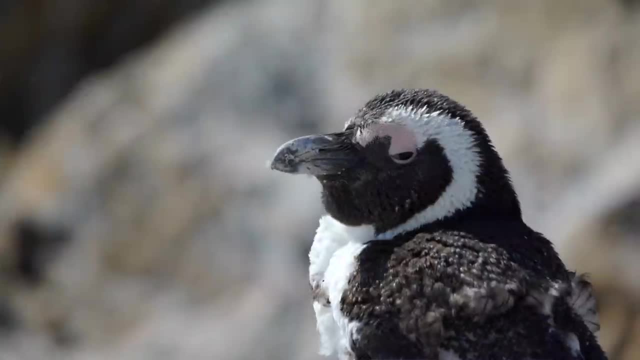 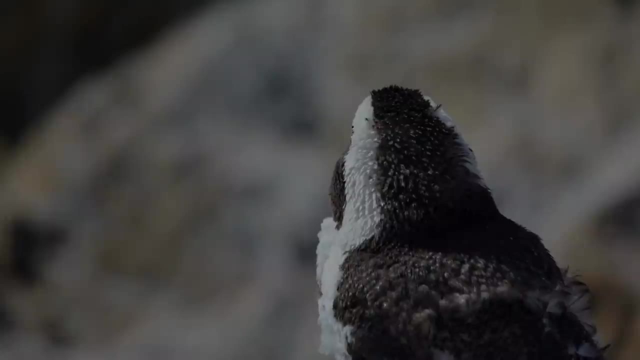 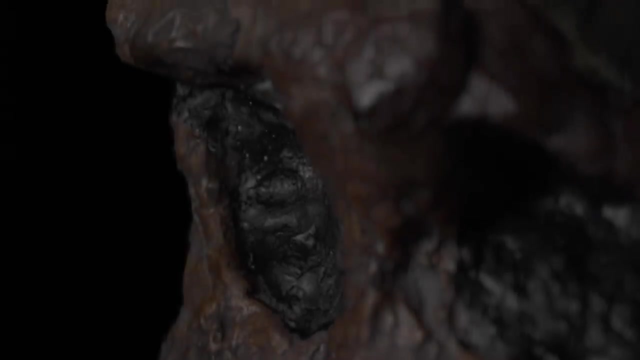 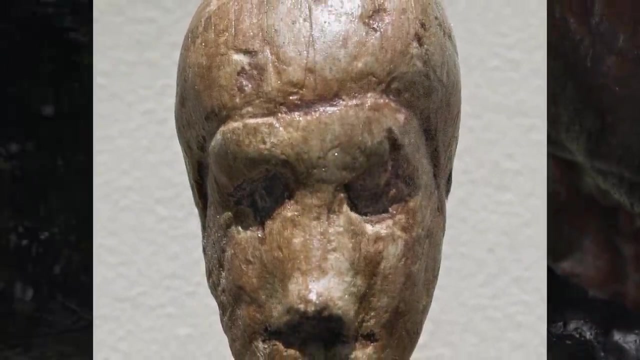 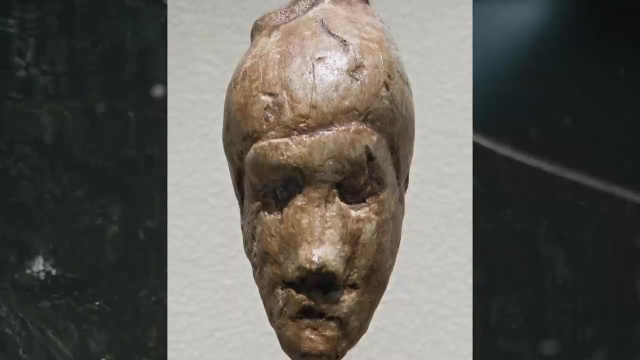 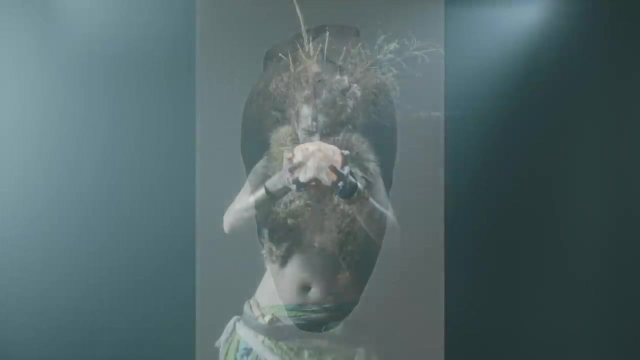 perhaps magical items created to be ritualistically broken. The most incredible of all, however, had exactly the same facial abnormalities as the elder, making it very likely to have been a model or representation, perhaps to remember her in future generations. It begs the question: do all the Venus figurines represent actual individuals who lived so many millennia ago? 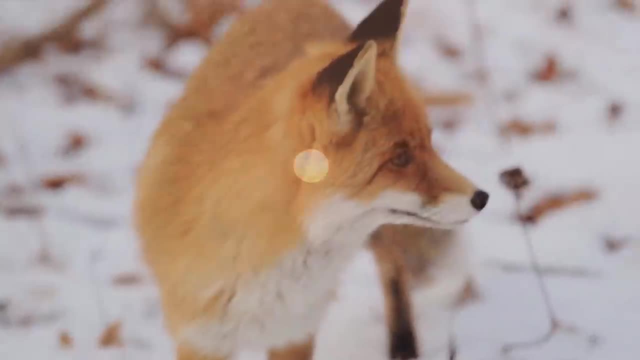 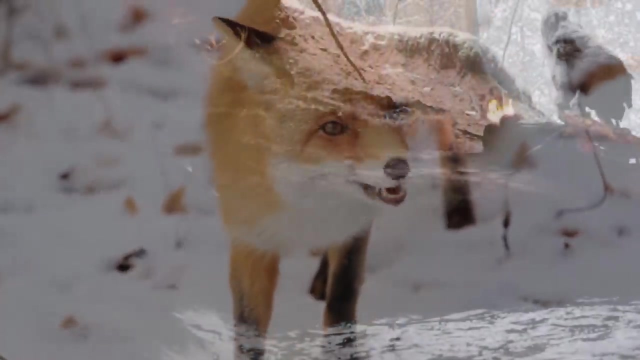 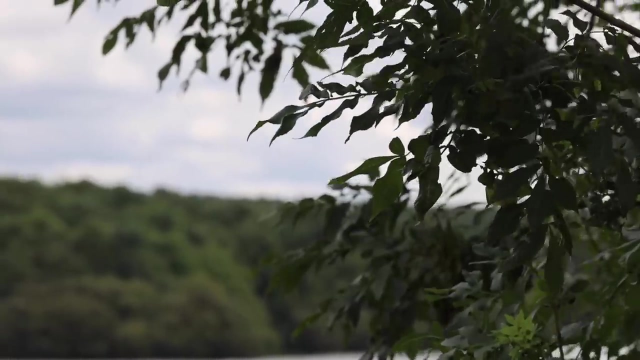 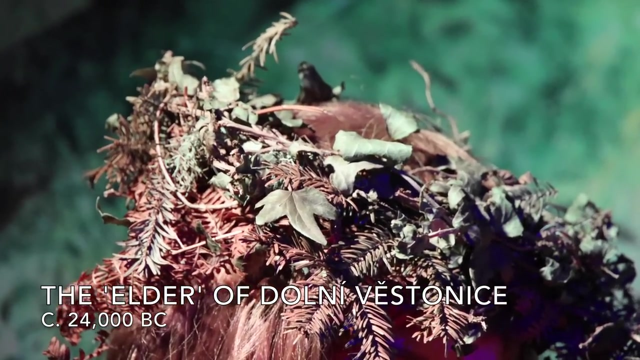 Given the discovery of the elder alongside a fox, an animal often associated with ritualistic shape-shifting trances, she is often thought to have been a shaman. Perhaps the dugout was her proto-temple, Whether she was an early oracle or ice age prophet, 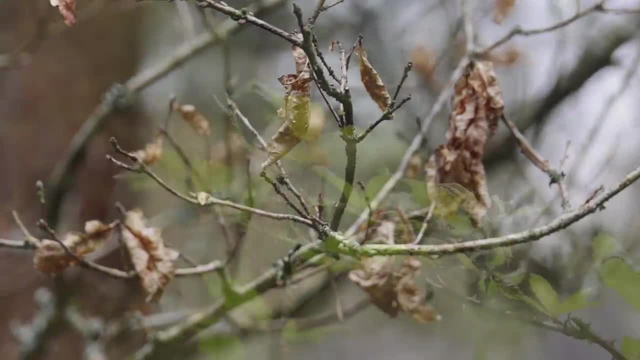 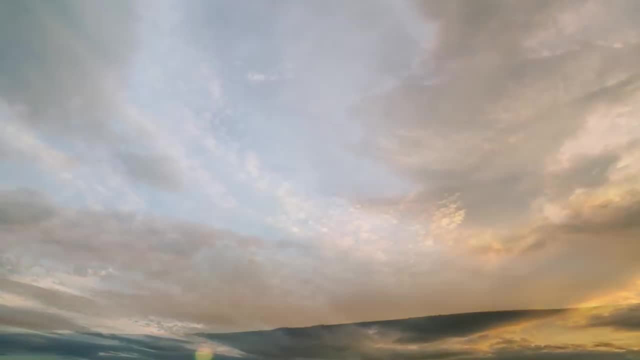 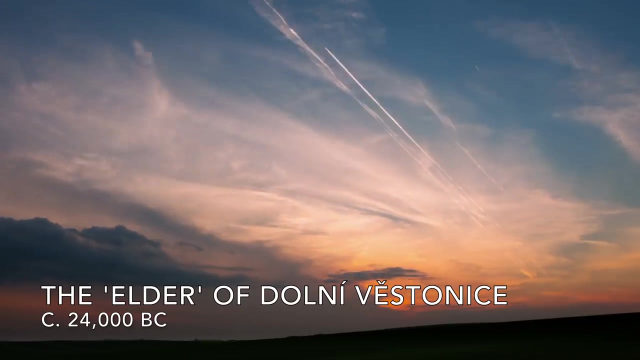 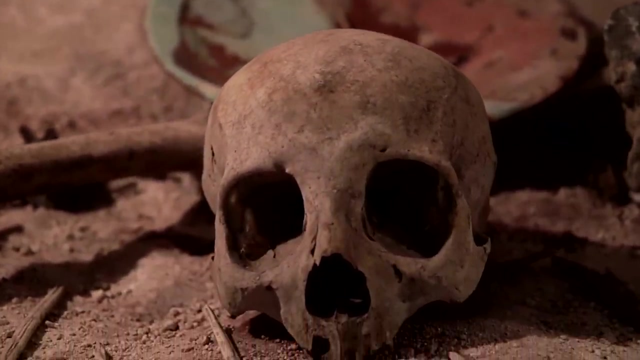 clearly, she was someone who had a lot of experience, Someone to be commemorated, remembered And, perhaps most importantly, not to be brought back to bring her wrath upon the living. And there is much more evidence of shamanic activity in the ice age. 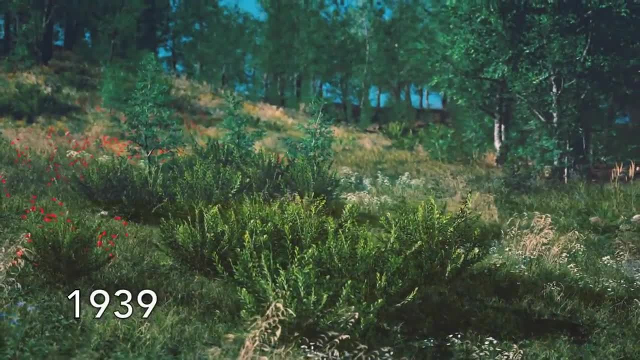 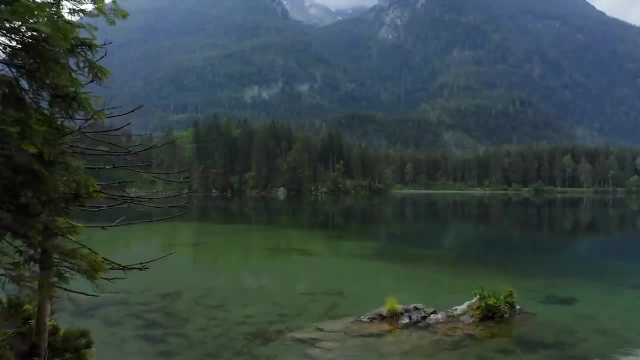 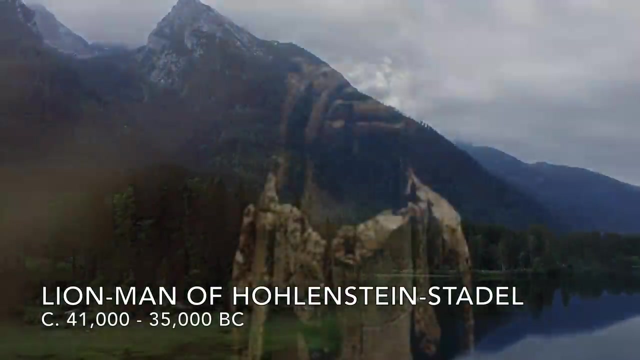 In 1939, an astonishing ivory statue was found in a German cave. When carbon dated, the Lion Man of Holenstein-Stadel was found to be as much as 41,000 years old, Although in terms of age it is not known how old he was. 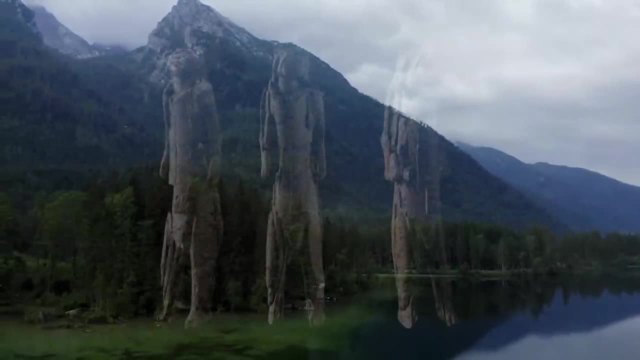 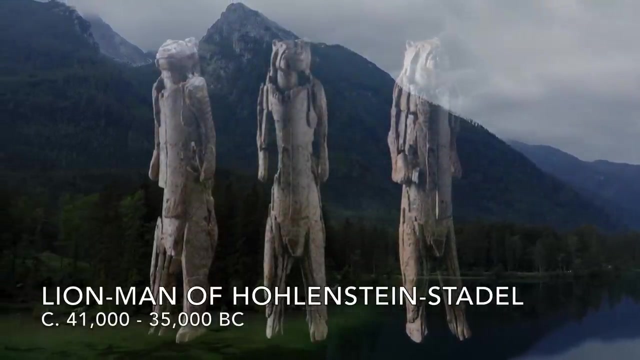 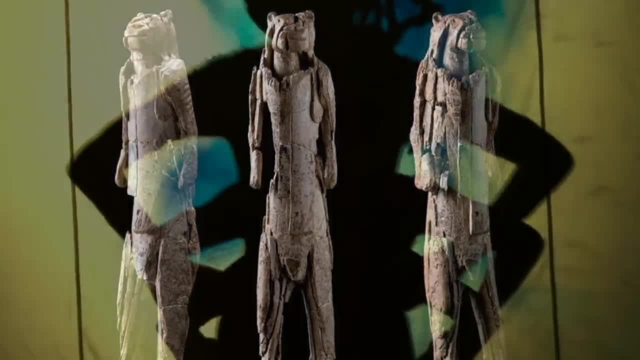 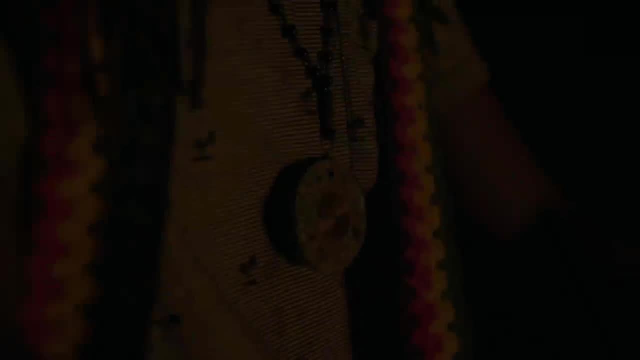 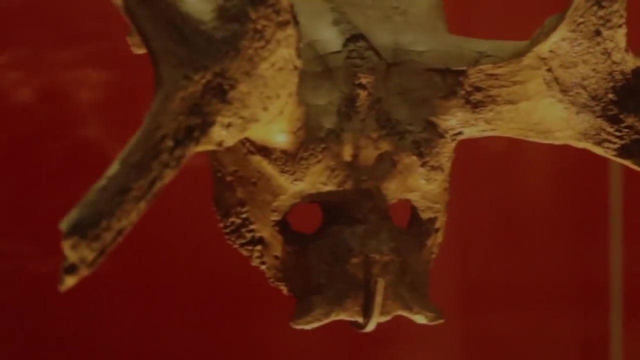 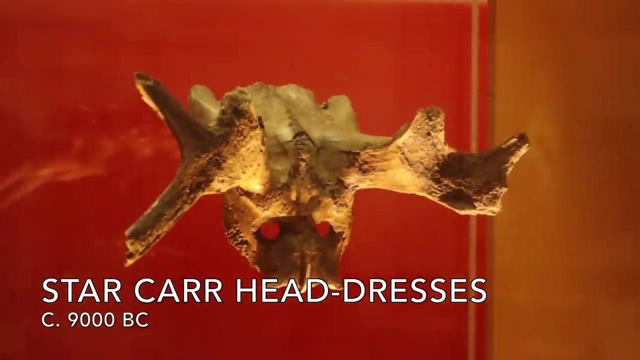 Just maybe in the midst of a shamanistic trance, With shape-shifting often considered to be an integral part, With shape-shifting often considered to be an integral part. These deer antler headdresses from Star Carr in Northumbria dating to roughly the same time as Gobekli Tepe. 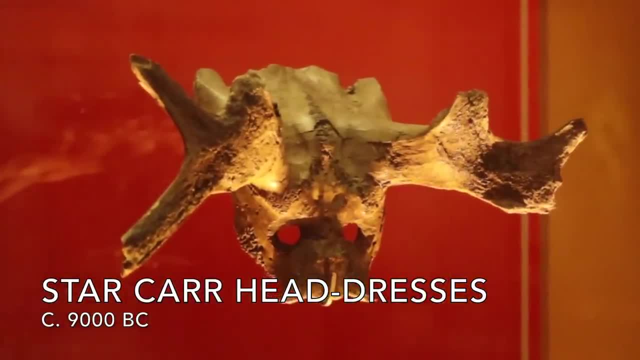 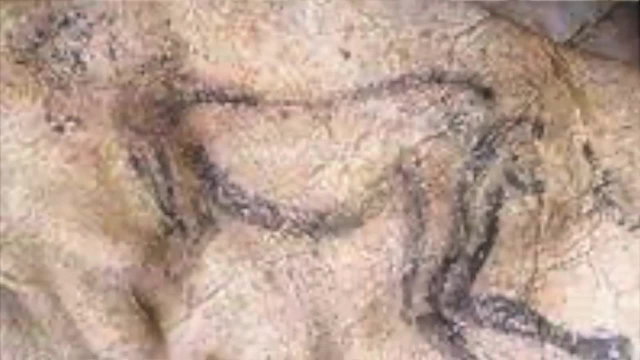 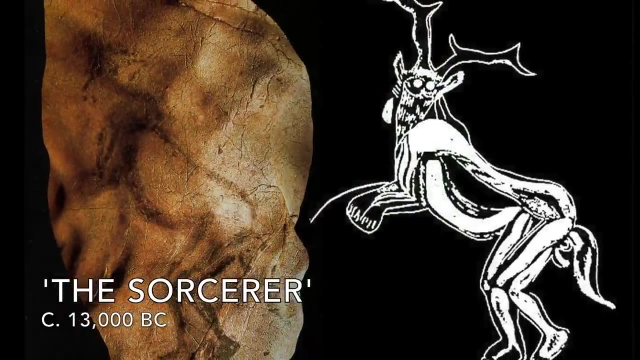 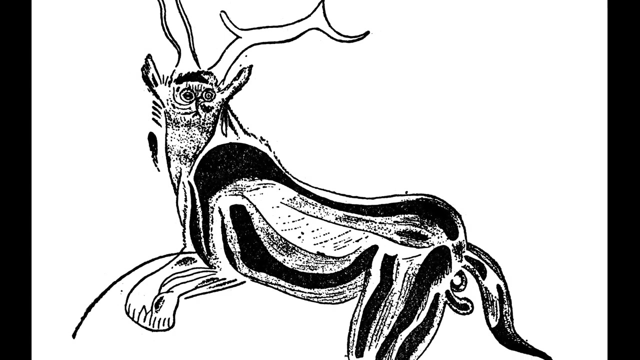 are also often seen as evidence for shamanic activity, As is this roughly contemporary cave painting from southern France known as the Sorcerer- known as the Sorcerer- Which may well depict a shamanistic ritual in process, Given the shreds of evidence we've seen. 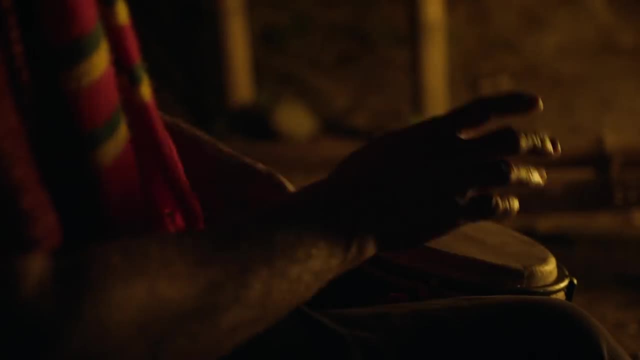 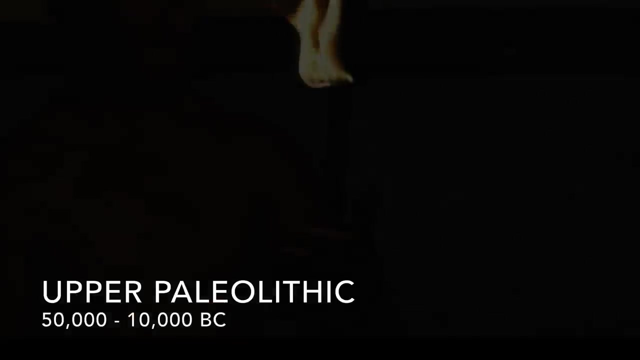 from the very beginnings of humanity's journey in Eurasia to the ends of the Ice Age and beyond, for the last 50,000 years or so at least. for the last 50,000 years or so at least, it's likely that ritual and religious experience 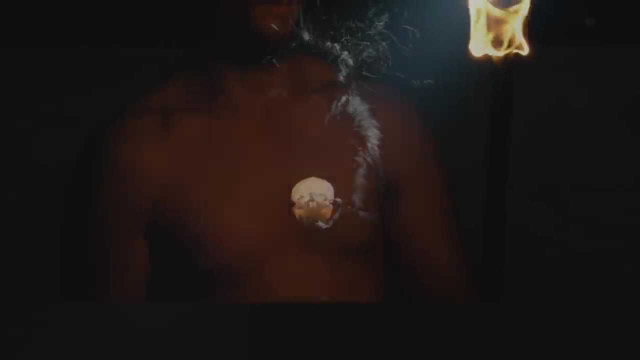 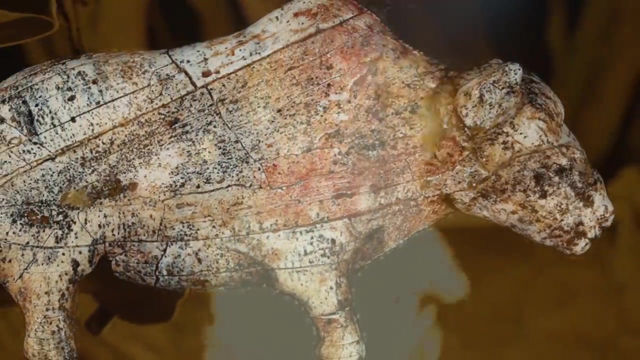 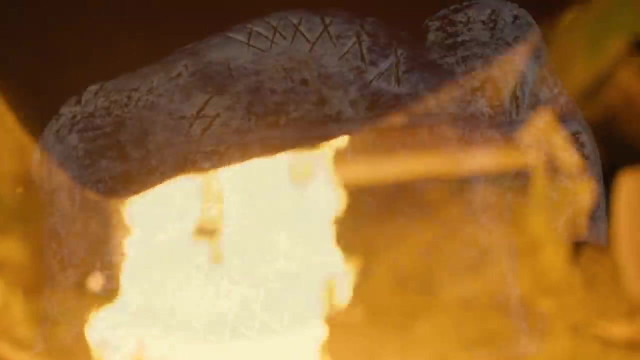 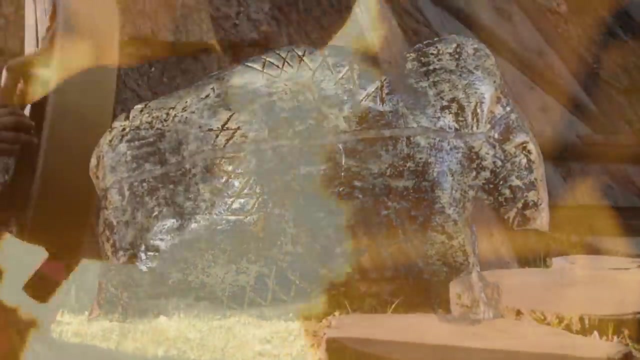 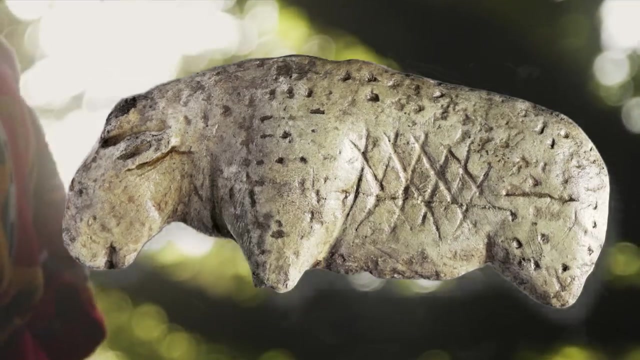 have always been a part of the social fabric, A hypothetical creative explosion linked with the need for social cohesion in the cold north. Maybe this was how smaller family units were able to congregate into larger clans and tribes at certain times of the year, Bound together by links to the ancestors. 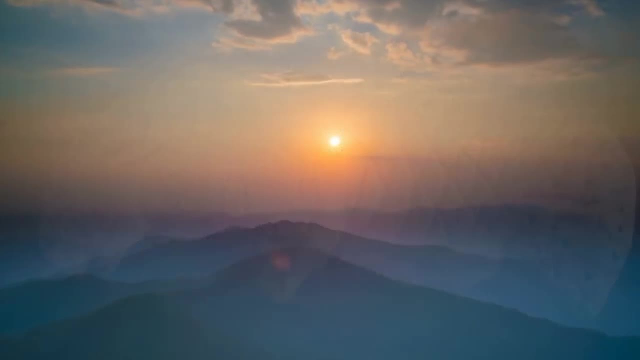 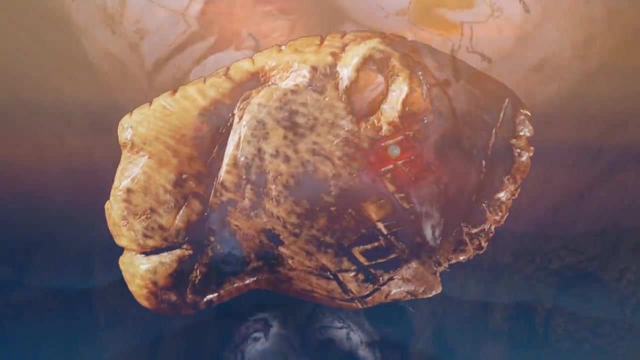 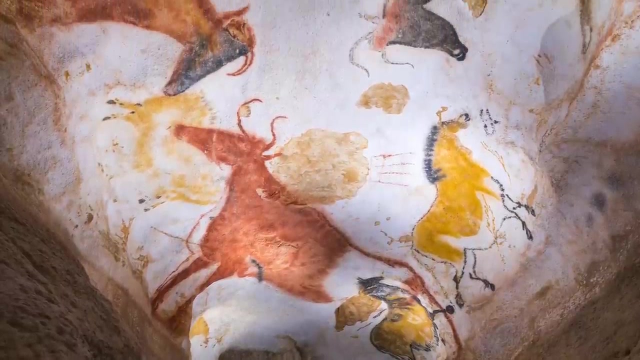 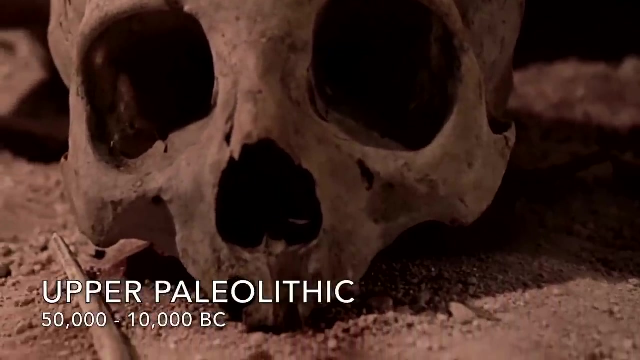 religious rites and perhaps even the worship of common deities, Culture by that time well and truly having outgrown biological evolution As far as the elaborate so-called princely burials of Ice Age Europe are concerned. hereditary systems of rank. 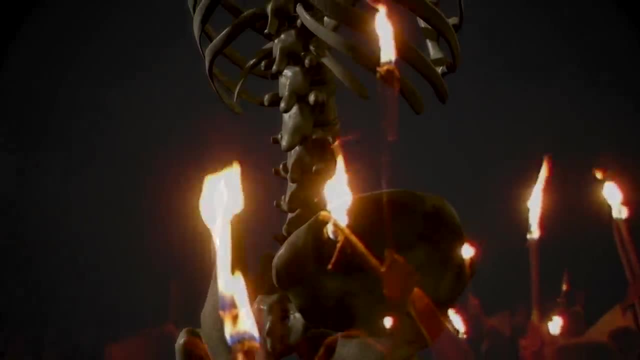 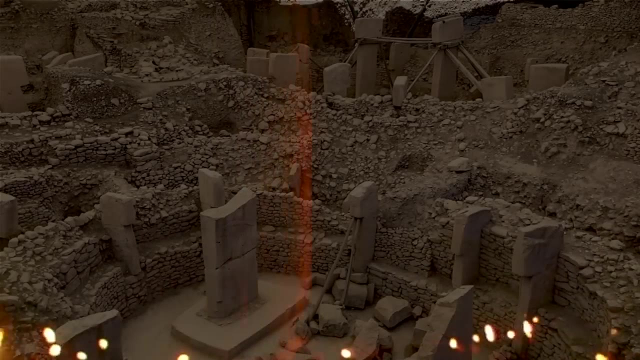 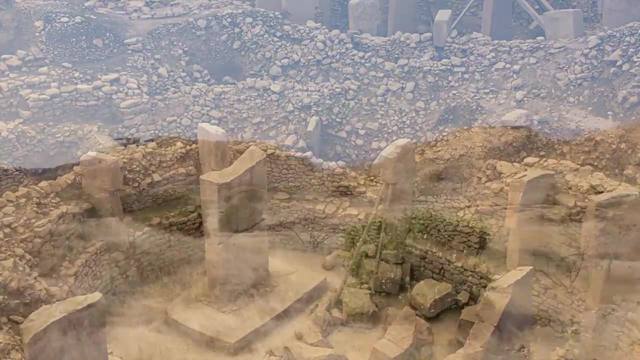 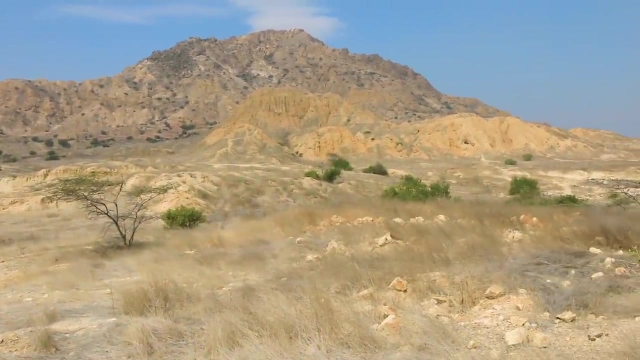 seem the most improbable interpretation of all. Again, this begs the question: is there a missing piece of the puzzle? at Gobekli Tepe, Like in ancient Peru and Egypt, where the erection of monuments was a holy task in itself, a form of worship dictated by a priesthood? 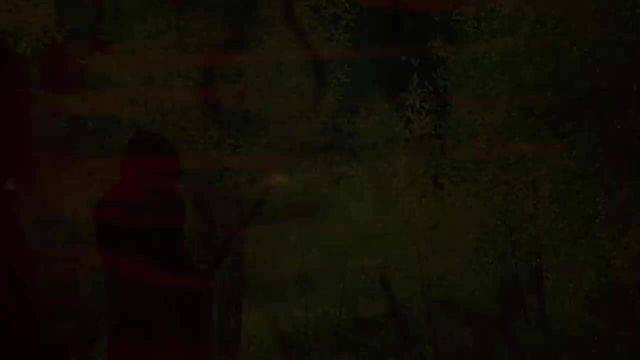 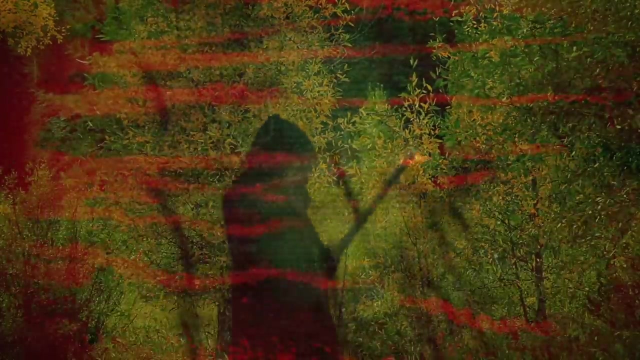 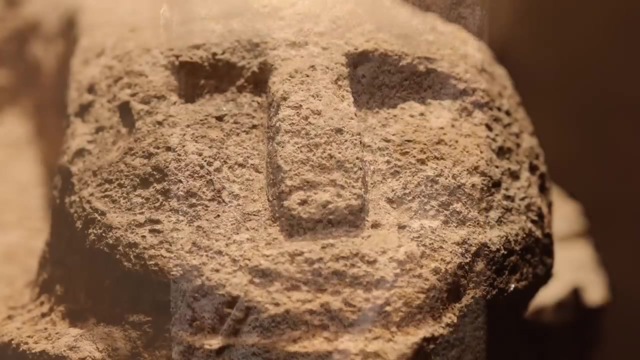 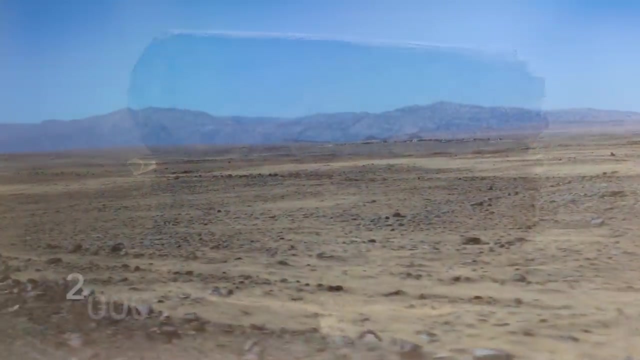 Was there a shadowy cabal pulling the strings in the foothills of the Urfa Plain? Not hereditary chiefs, but a meritocratic theocracy In the year 2000,. the translation into English of a relatively unknown French scholar's work. 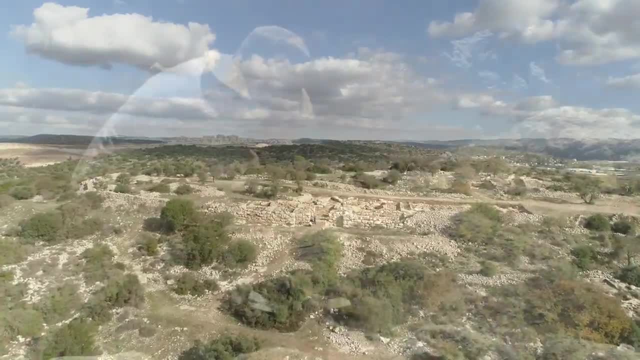 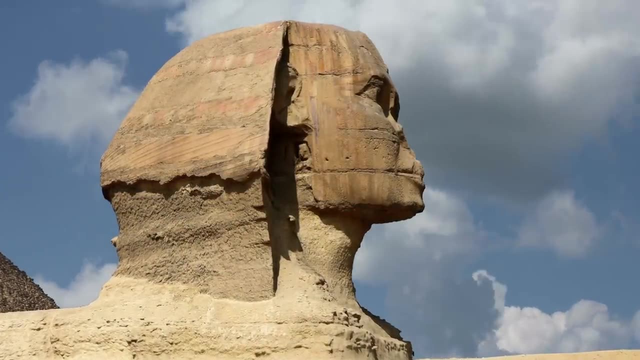 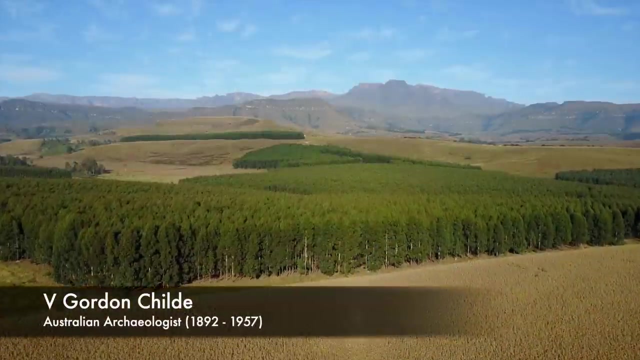 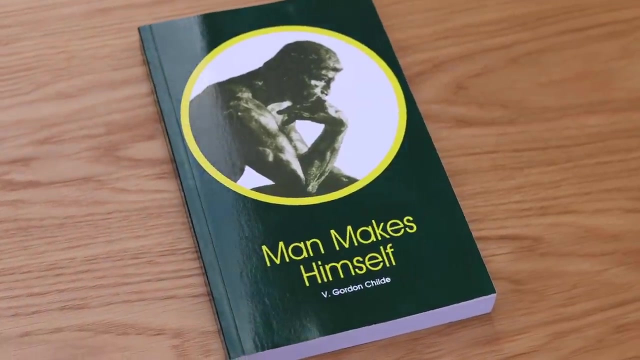 not only caused a stir in the archaeological community, but ever-elusive ripples into the realm of popular culture. Ever since Gordon Child's oasis theory and the like in the early 1900s, the majority of attempted explanations for the so-called Neolithic Revolution. 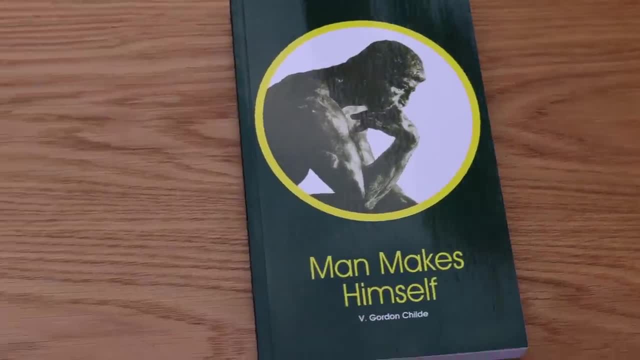 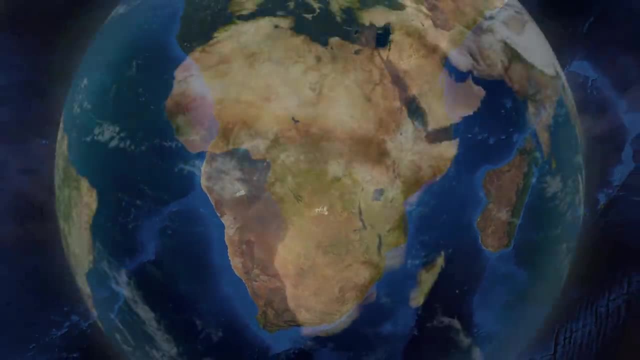 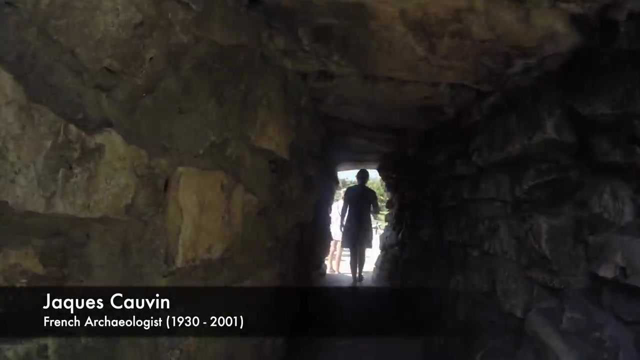 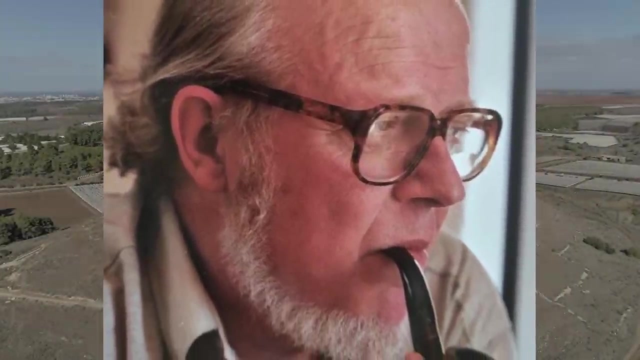 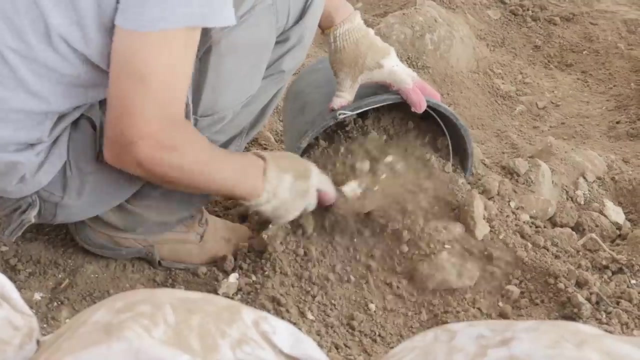 had focused on economic reasoning, geographical needs and material circumstances dictating growth into agricultural societies. Enter Jacques Covan In the early 1990s, after more than 50 years of research involving digs at some of the most important early Neolithic sites in the Near East. 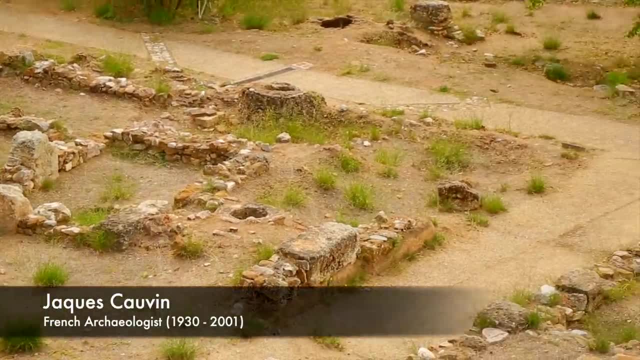 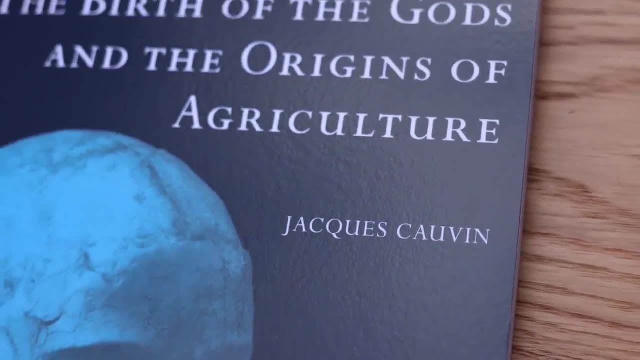 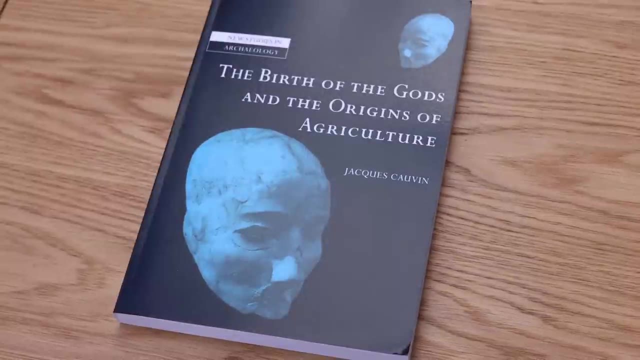 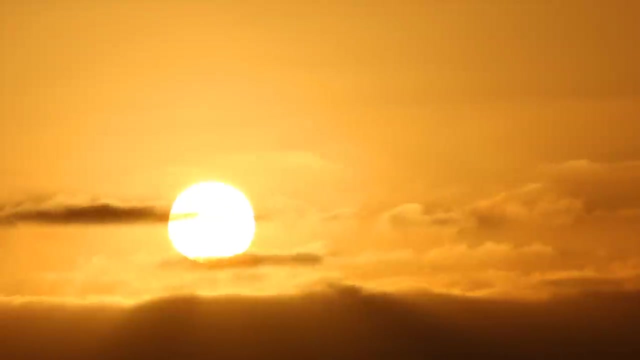 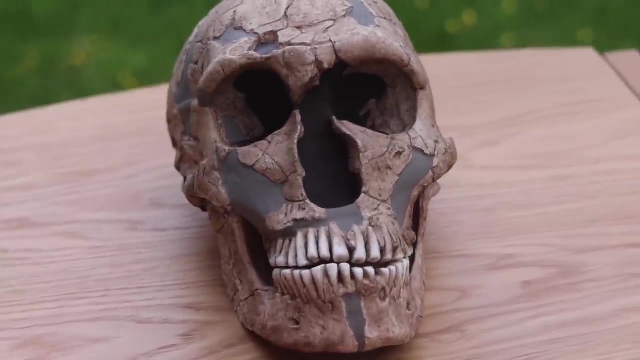 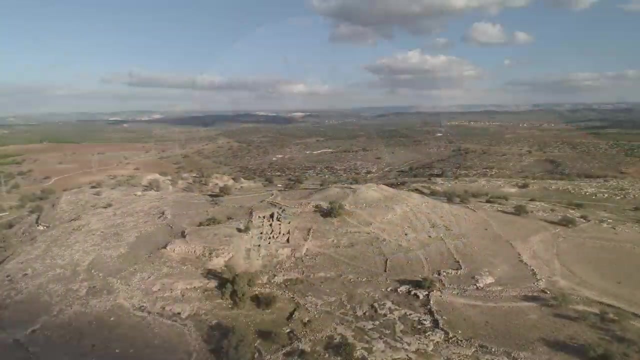 Covan went public with a completely different idea. In The Birth of the Gods and the Origins of Agriculture, Jacques Covan suggested not material reasons for the shift from hunter-gathering to agriculture, but a transformation that began in the mind, A profound cultural transformation. 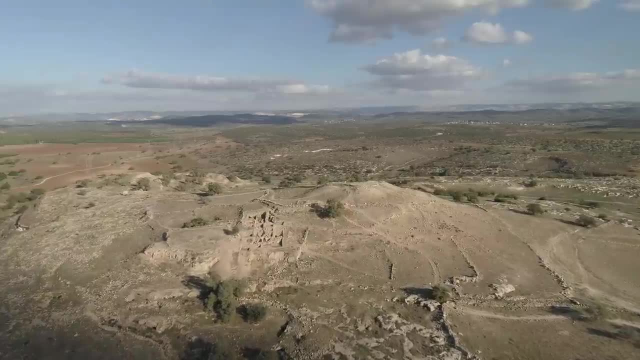 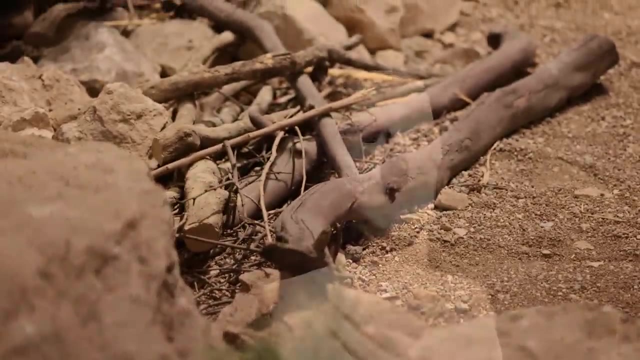 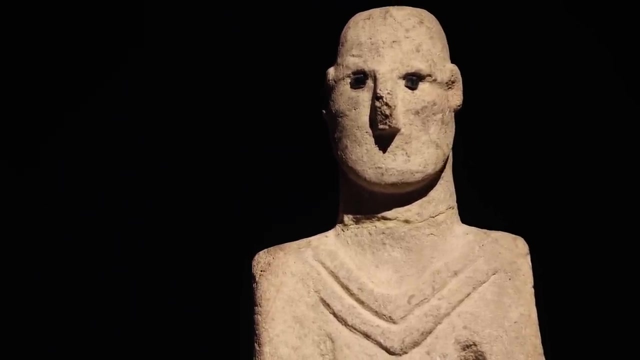 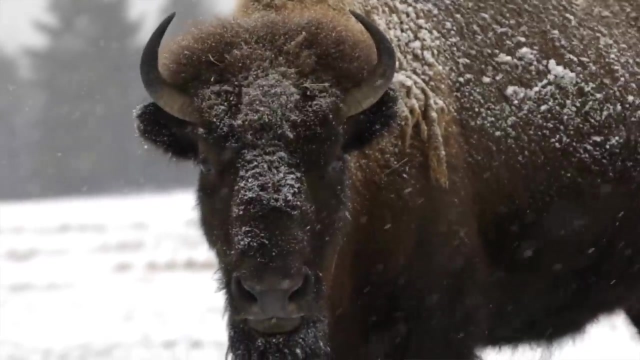 within the human psyche from around the 13th to the 10th millennia BC, primarily involving a shift in perspective from seeing humanity as a part of nature to being outside of it, Eventually with not only the potential to dominate the natural world. 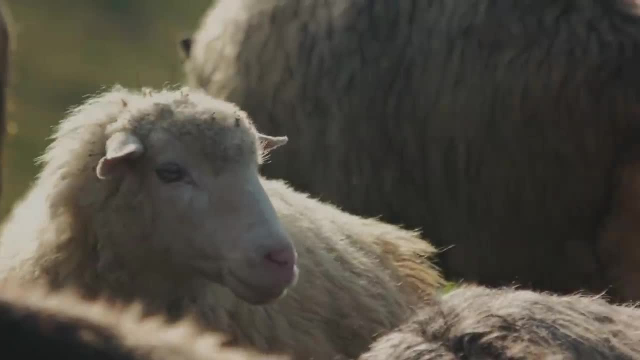 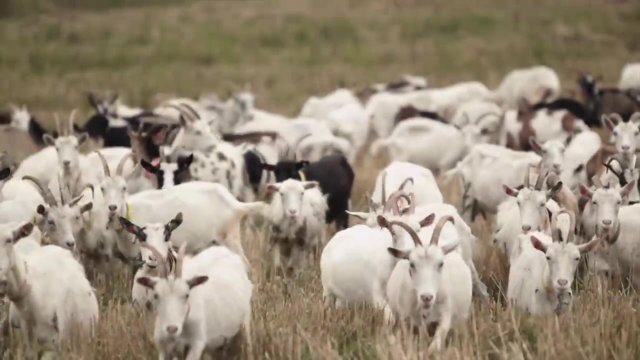 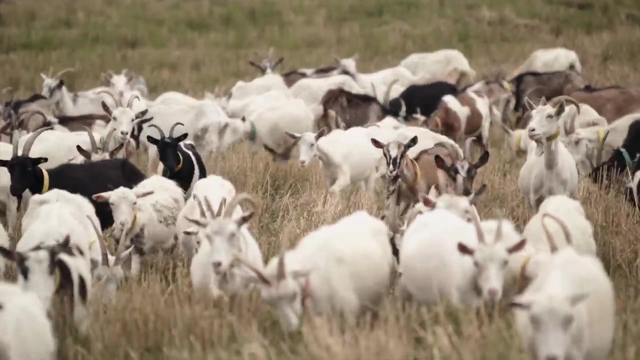 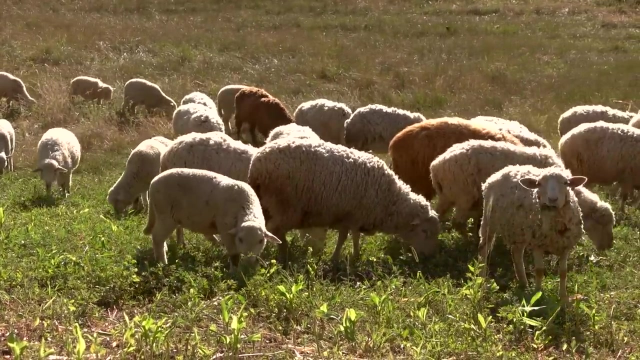 but the right. In other words, in order to become a farmer, you have to think like one first, Perhaps like all later religions, beginning as a single creative spark Rather than economic need, environmental shift or even individual social promotion. 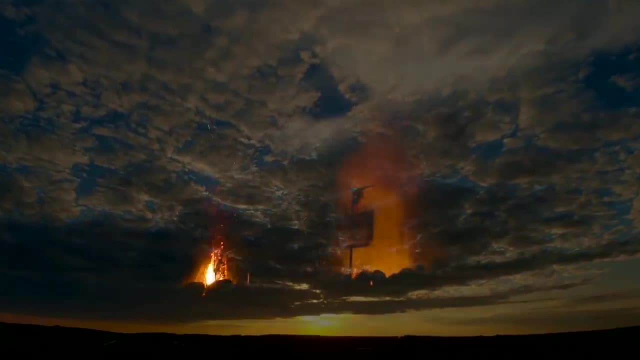 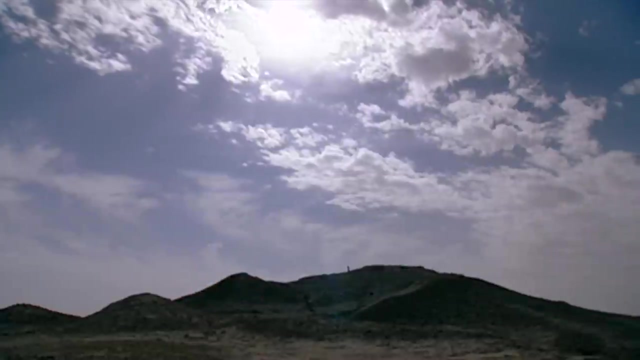 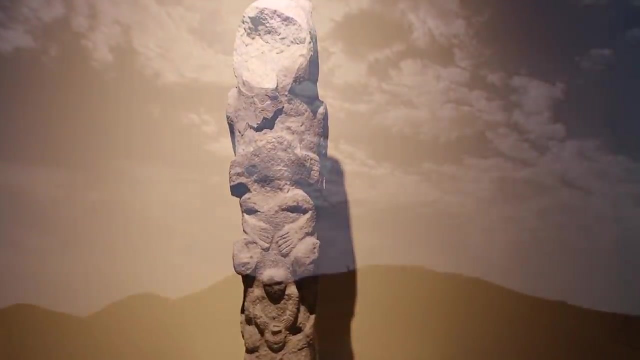 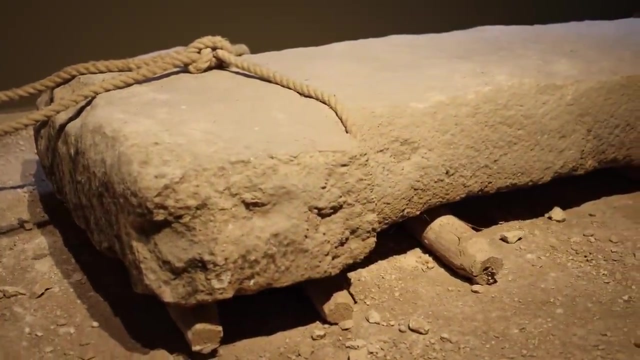 a collective epiphany expressed in new symbols and ideas At the very dawn of civilization, Though of course it remains completely untestable, If even at all true, and it could go alongside other theories to a certain extent: Jacques Covan's 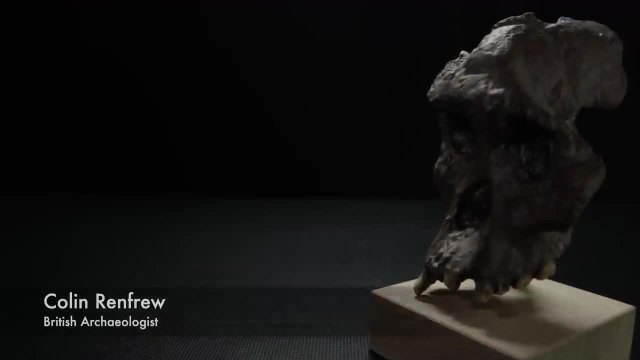 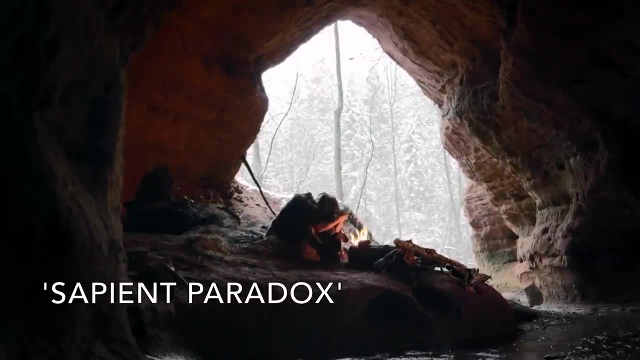 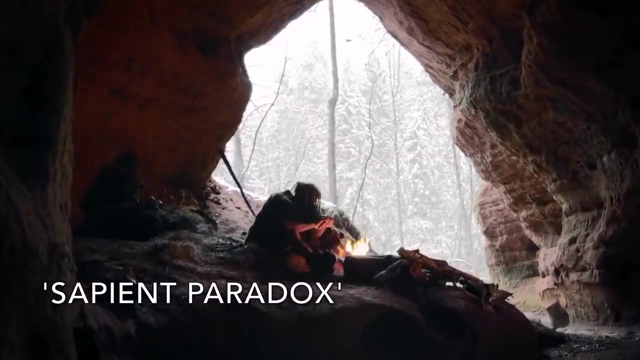 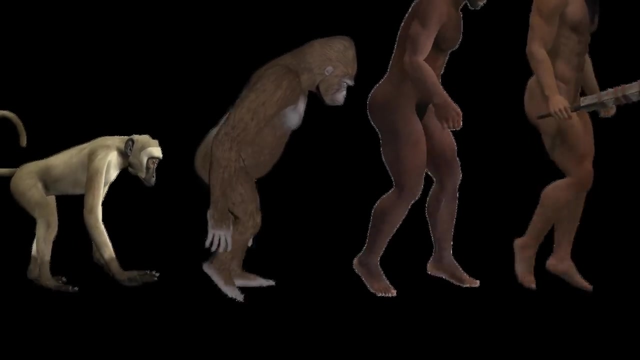 Birth of the Gods would solve Colin Renfrew's sapient paradox Of why humanity only began the road to true societal complexity by around 10,000 BC, After being anatomically modern for as much as three or four hundred thousand years. Covan's death. 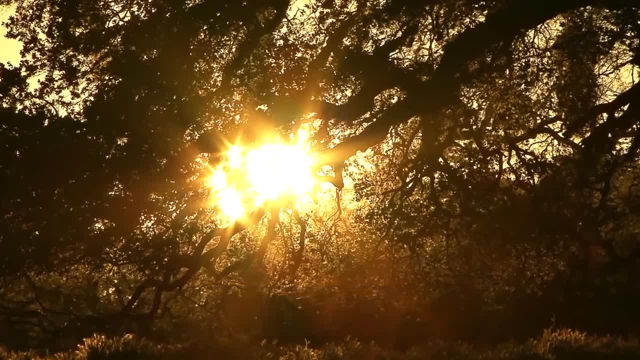 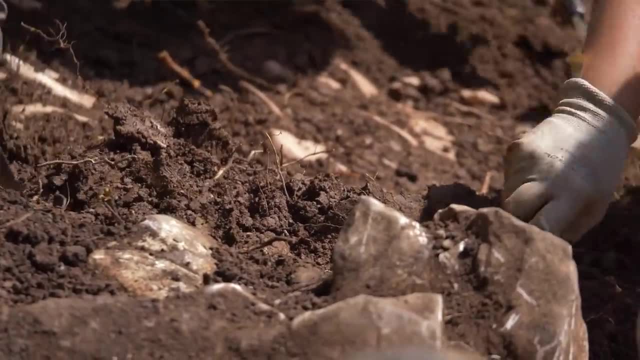 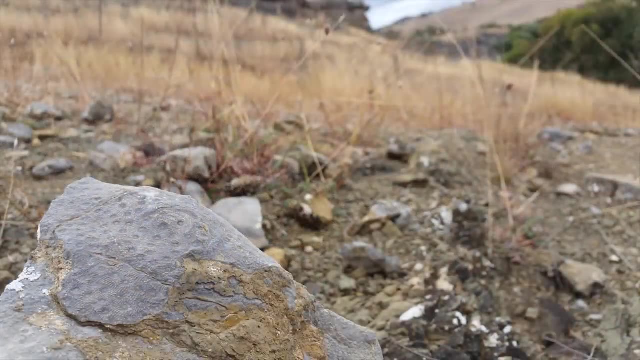 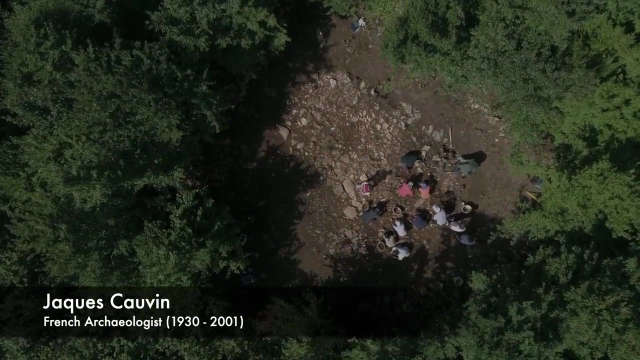 the very next year, in 2001, only added to the allure of the theory, Which remains immensely influential amongst archaeologists today. Far from the rigid economic reasoning of Braidwood and Childe, Jacques Covan evokes distant ancestral memories of ecstatic dance. 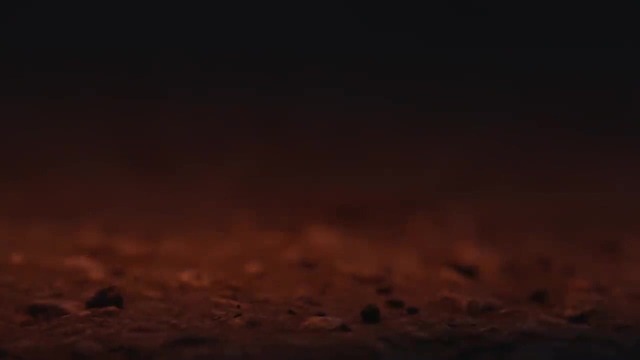 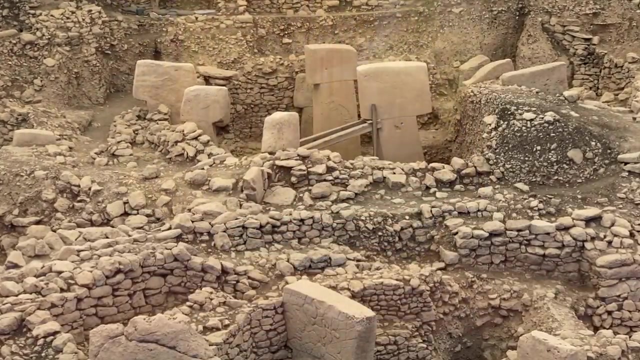 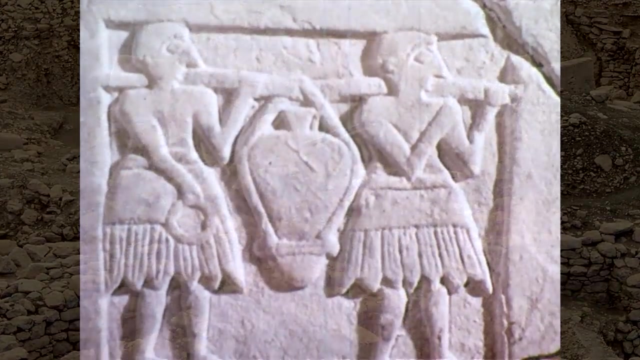 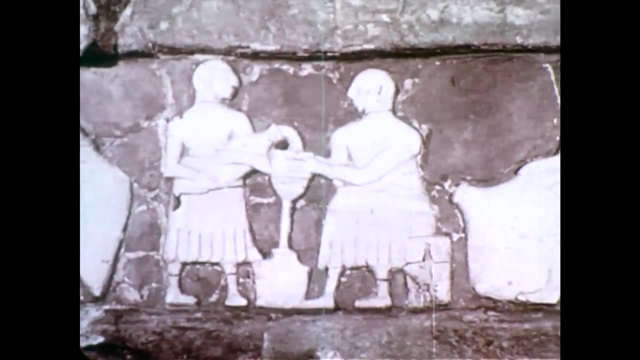 Beneath the colossal T-shaped pillars of elder days. From the early 20th century to today, a number of sociologists and anthropologists alike have studied the nature of religious ecstasy, Commonly observed all over the world and in all walks of life. 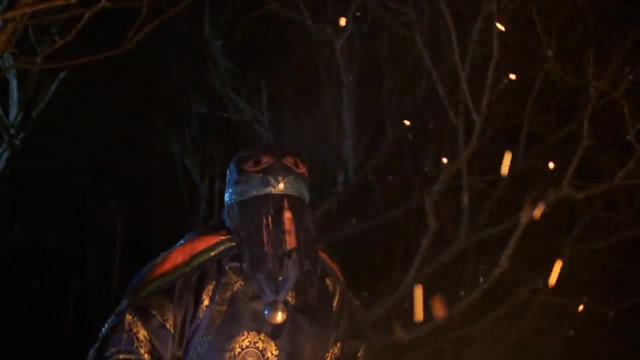 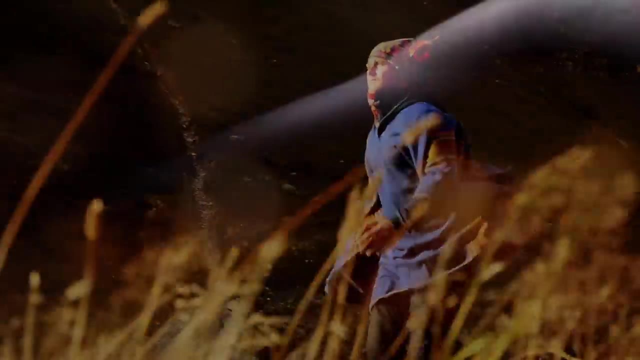 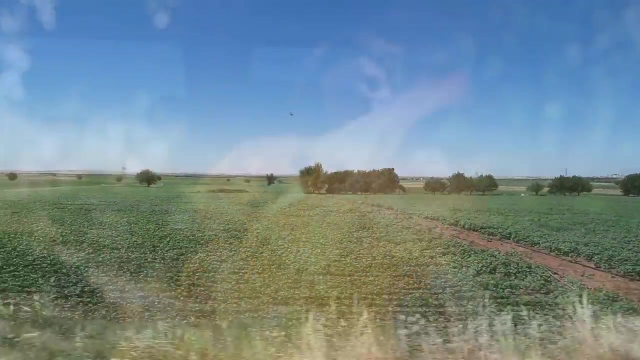 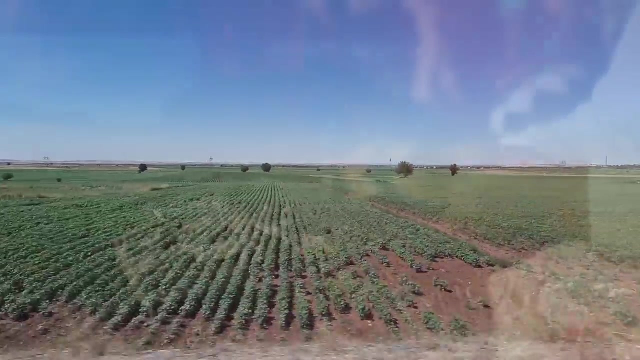 Perhaps most notable being the work of Messia Eliade and Emile Durkheim. For them, the effervescence and elation of religious ceremony has a tendency to ferment a sense of belonging and contentment in a community, Very possibly in prehistoric and historic times. 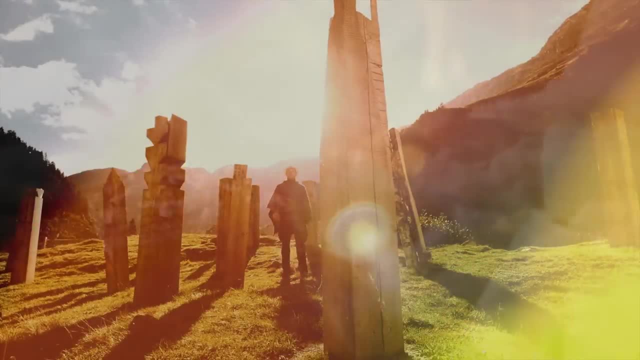 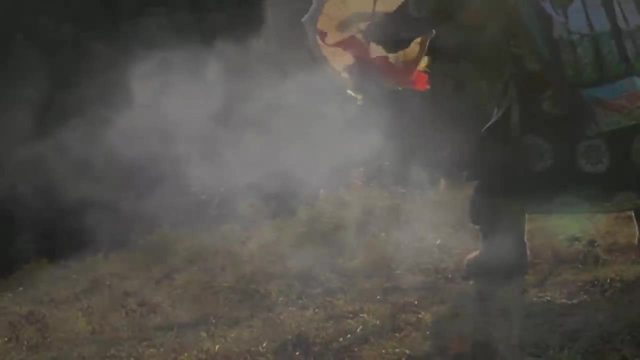 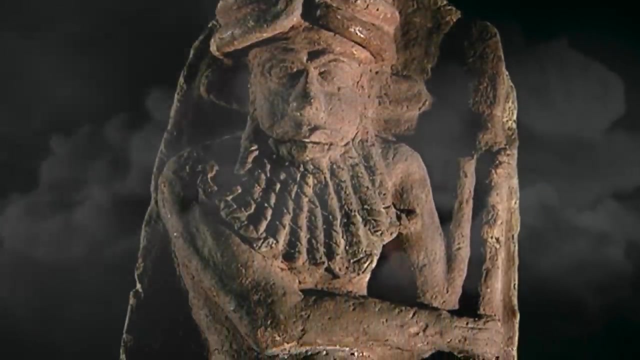 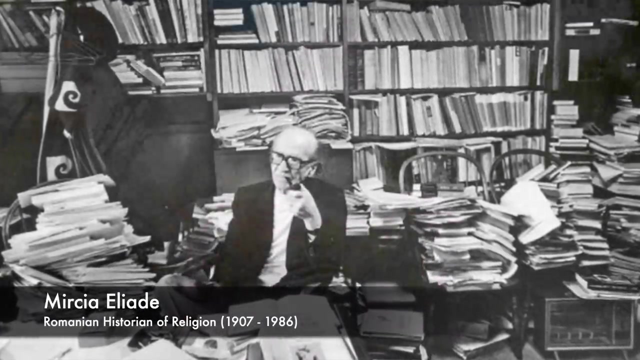 Allowing for ever larger conglomerations of people to coalesce than ever before, Sometimes ultimately resulting in asymmetrical power structures beginning to form An expert in world religions. Messia Eliade, in particular, talked of the pursuits of ecstasy being an integral part. 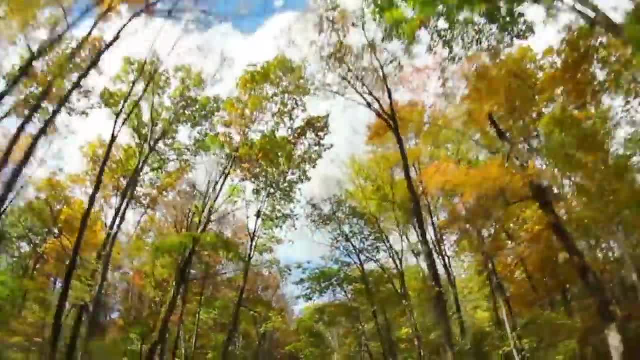 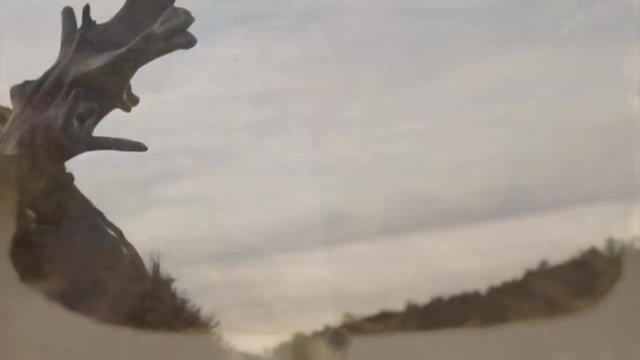 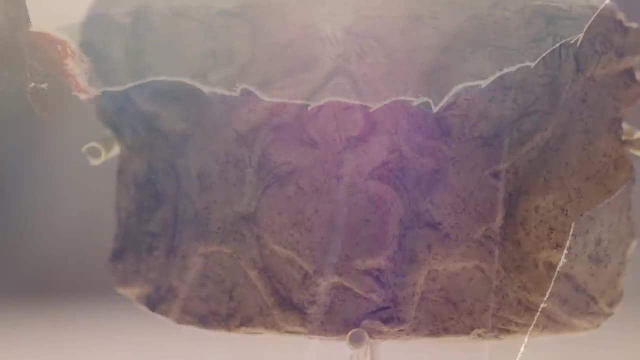 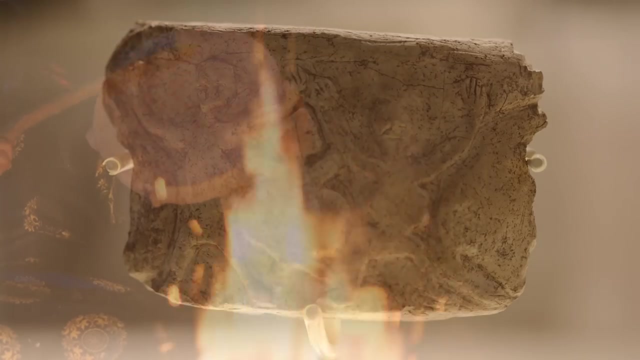 of the religious experience, The transformative feeling of awe, for example, being one that goes hand in hand with music, monuments, landscapes and nature, Music and dancing in particular, often inducing trance-like altered states and a sense of unity, All of which were present. 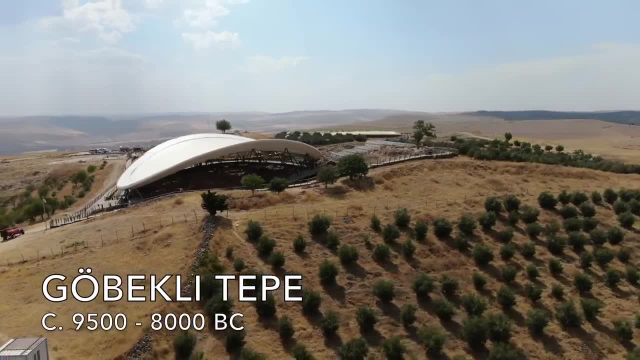 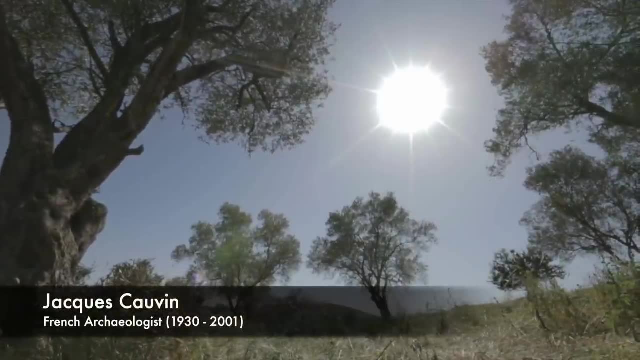 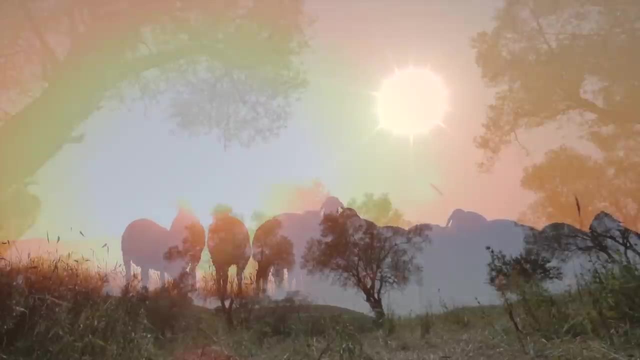 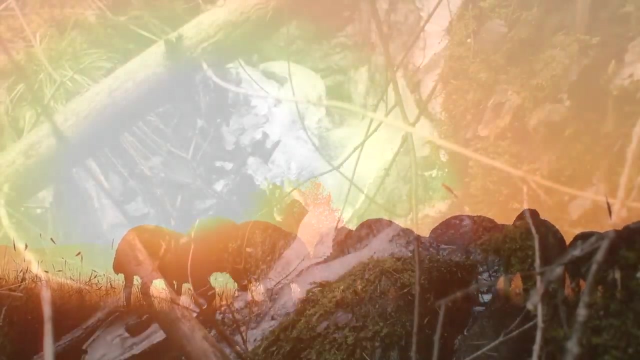 at Gobekli Tepe. Of course, by their very nature, Jacques Covan's ideas remain entirely untestable, Little more than hints of a shamanic council leading a societal revolution Awash with awe and ecstatic devotion, Building on time-honoured ideas. 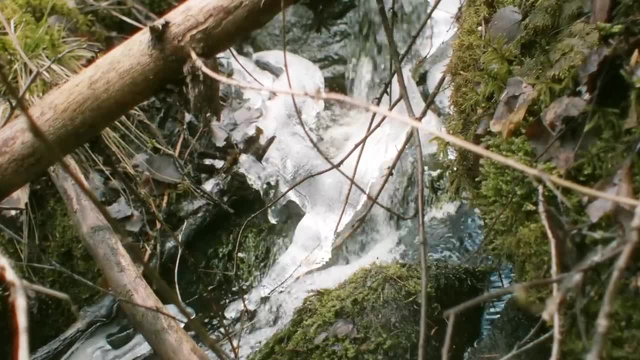 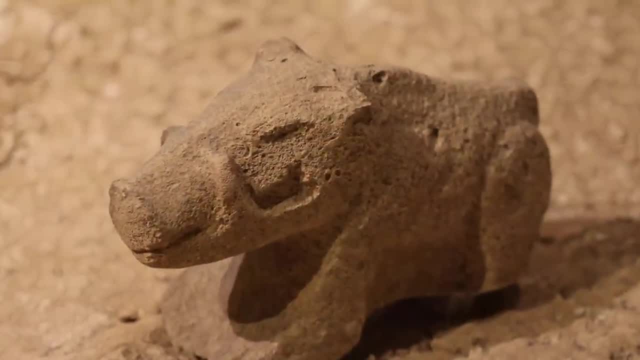 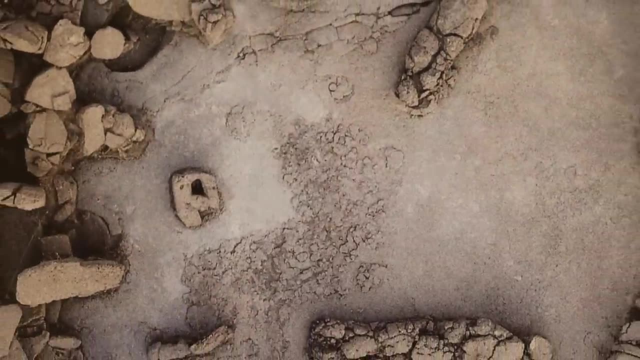 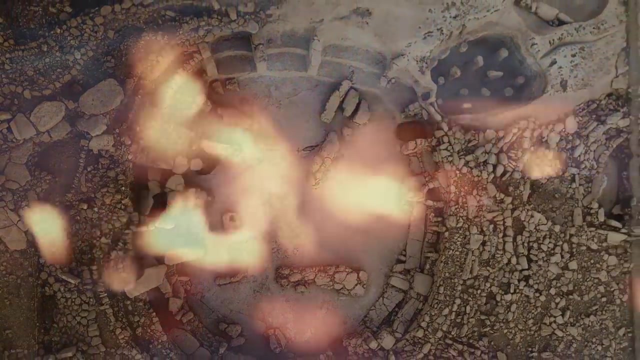 Stretching back tens of thousands of years into the Aurignacian, But imbued with newfound insights and effervescent immediacy. Annual festival centres, apparently common in older hunting societies, for exchange and verbal communication, Ever growing and ever spreading the new word. 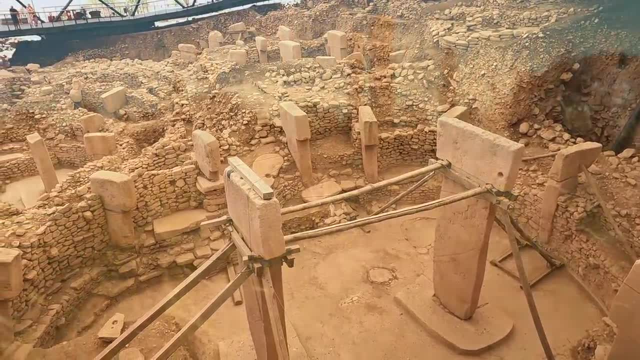 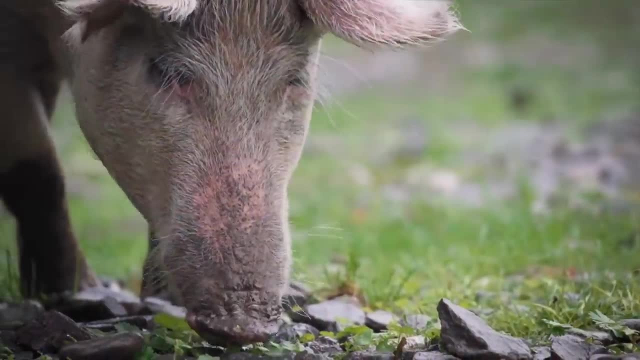 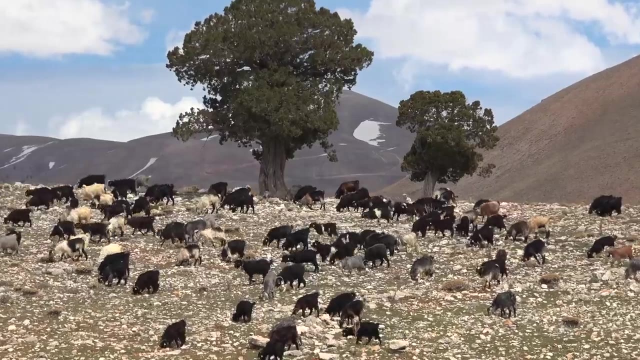 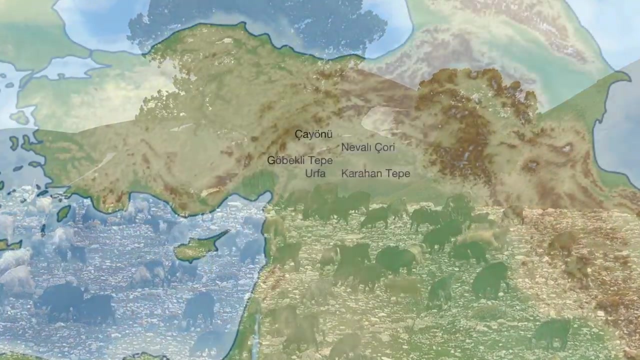 It's even possible that domestication of plants and animals ultimately came about in part as a means of feeding increasingly large groups of people drawn to holy sites to build and to worship Domesticated plants and animals showing up slightly later at sites like Nvali Chori and. 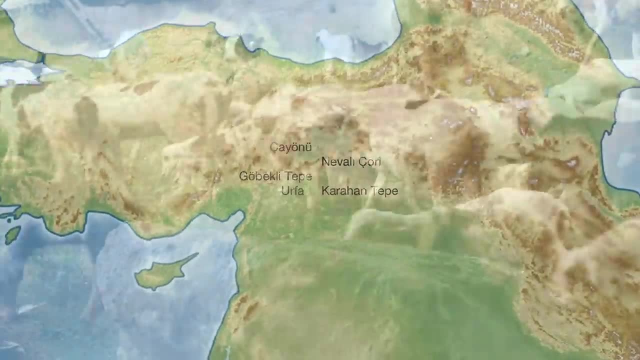 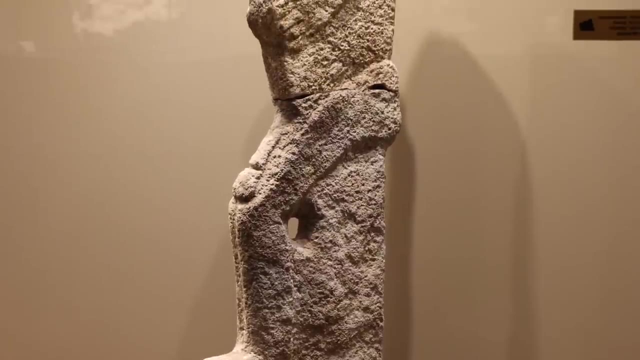 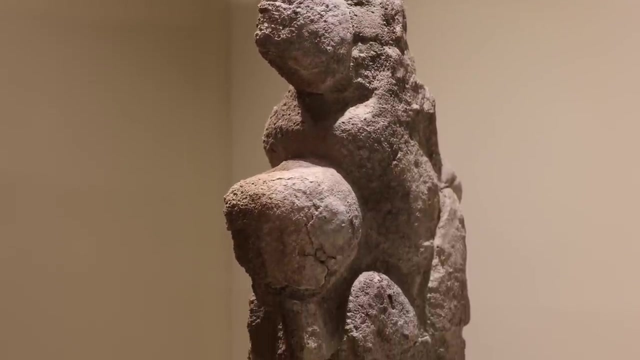 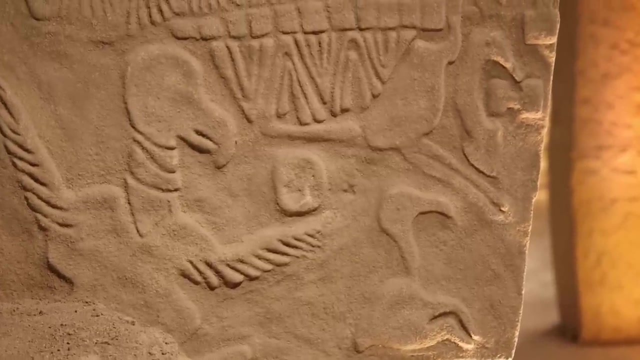 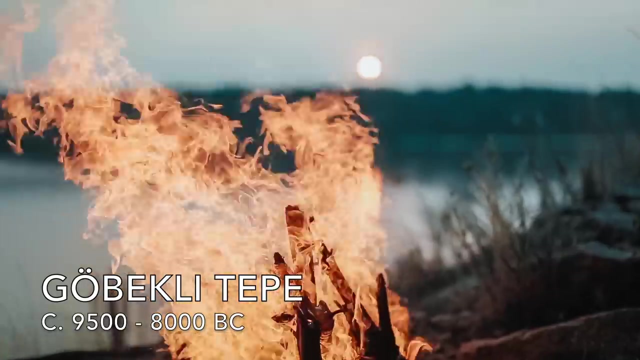 Chianu, The art of which still very much echoed that found at Gobekli and Karahan Tepe and their own older levels, Of course. another equally possible theory favoured by Klaus Schmidt holds that religion actually kept the hunters of Gobekli Tepe from pursuing agriculture where others to 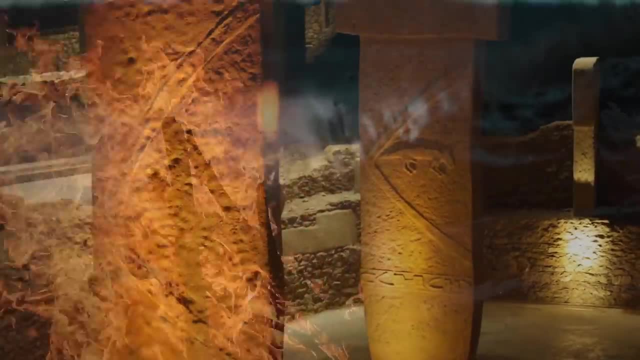 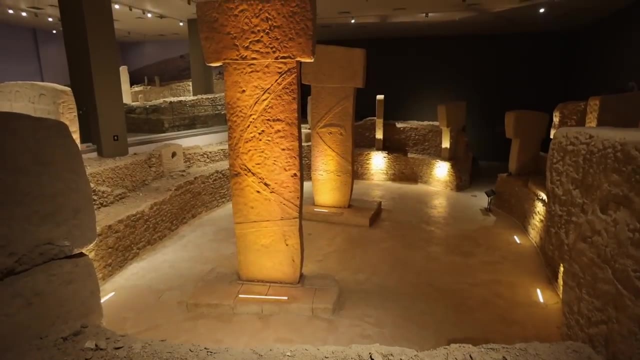 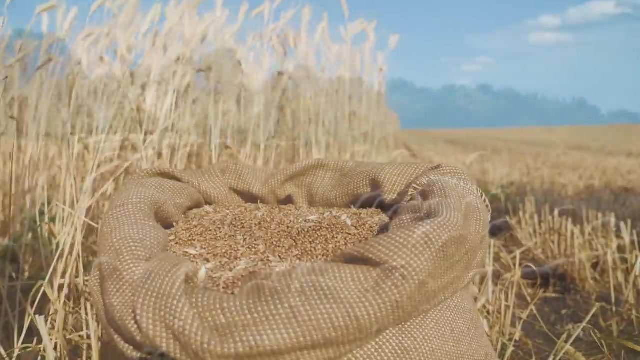 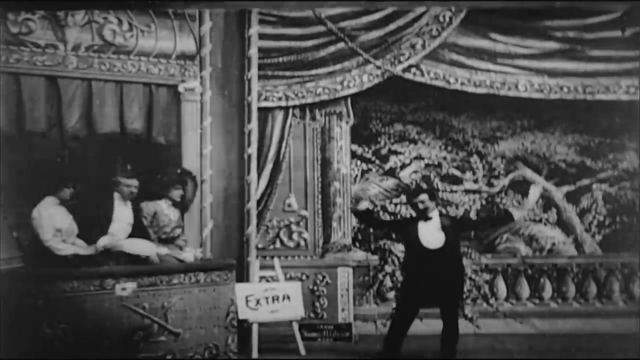 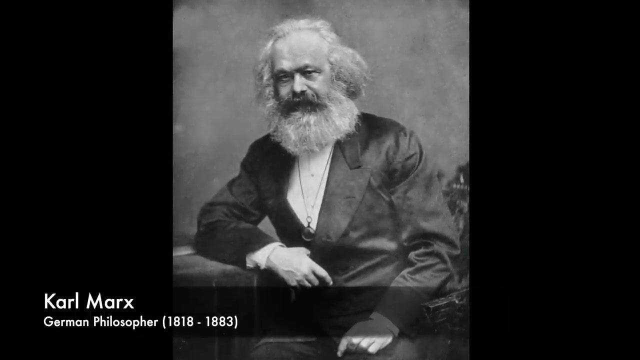 the south did so Being a last holdout of a resolute culture of hunting. In the late 1800s, German philosopher Karl Marx, one of the most influential thinkers ever to put pen to paper, implied religion to be a conscious invention of the elite, to 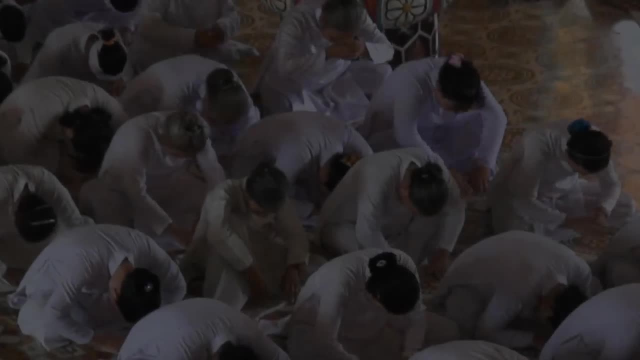 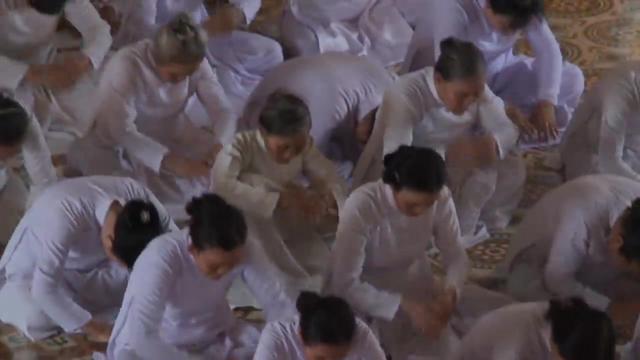 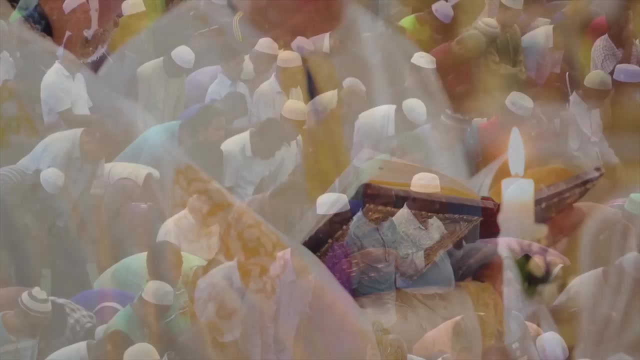 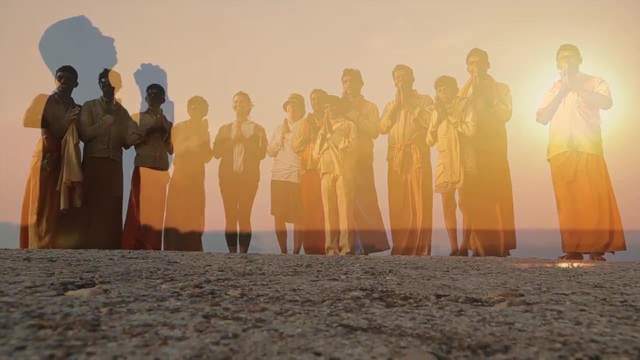 control the masses. The reality, as usually is the case, seems to be far more complex. Religious ideas conceived of until relatively recently as a form of science seem to have been utterly intertwined with humanity since the very beginning. The idea of religion as a form of science seems to be utterly intertwined with humanity. 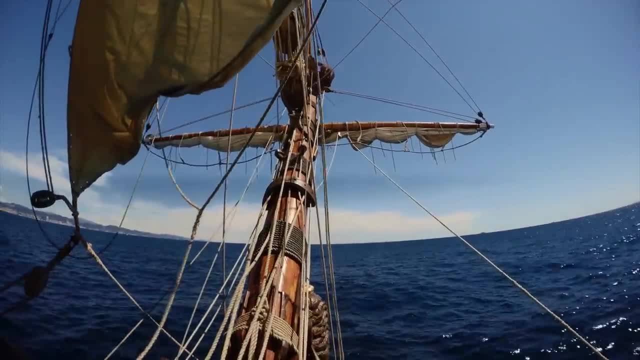 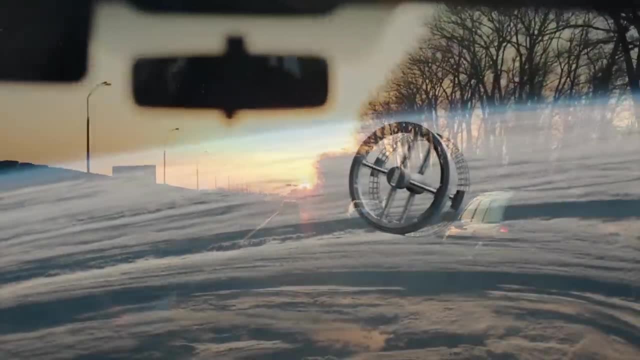 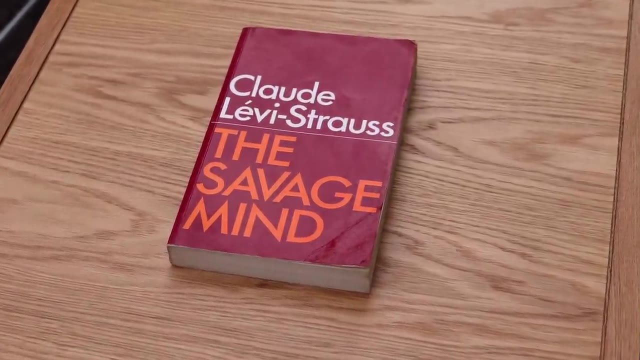 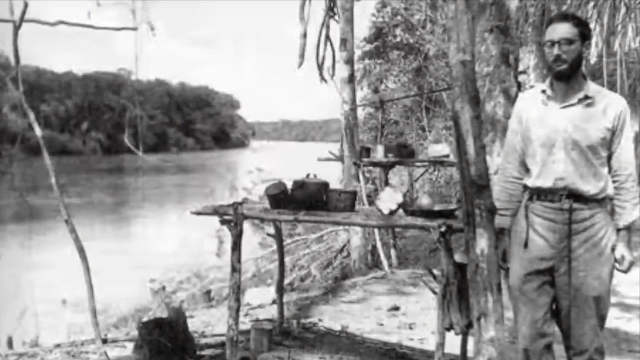 since the very beginning, Humans are a curious and immensely creative species And, as French anthropologist Claude-Levi Strauss first pointed out in the 1950s and 60s, in prehistoric societies, mythological thought and religion were the only ways of explaining. 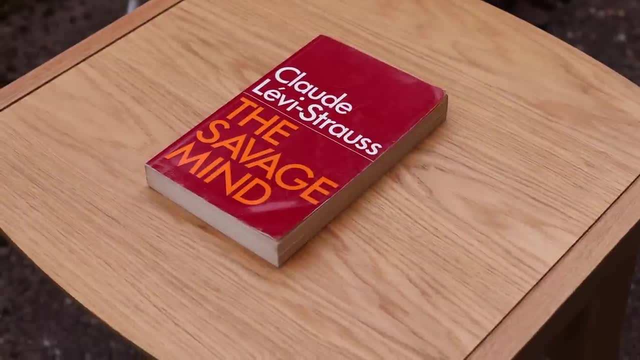 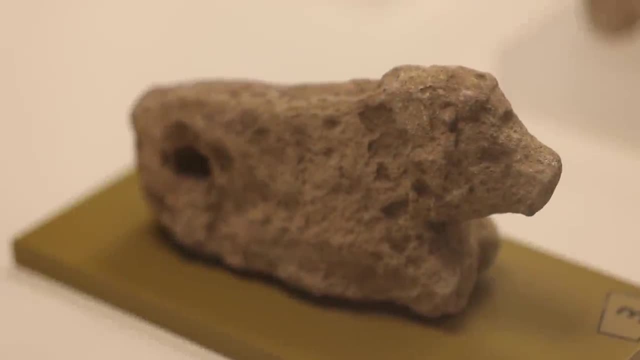 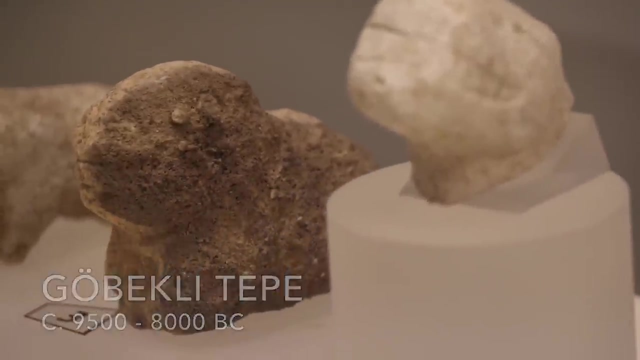 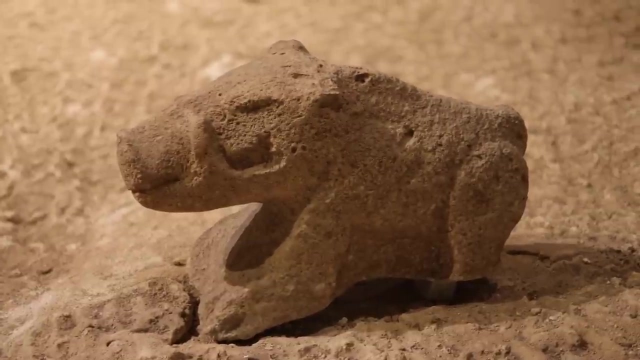 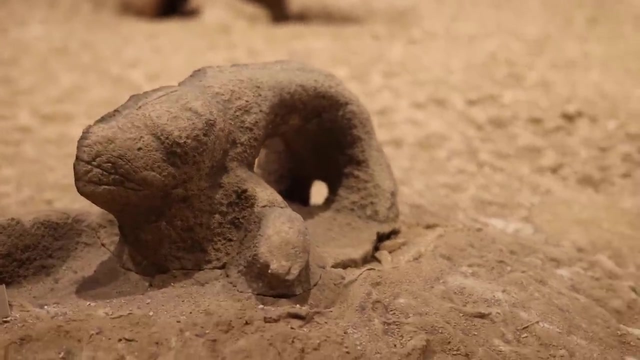 and exploring the world and the bigger questions within. Above all else, the individuals who built Gobekli Tepe were our intellectual equals – possessing exactly the same mental capacity that we have today, Just with a more basic cultural tradition and knowledge base, but no less colourful creativity to draw from. 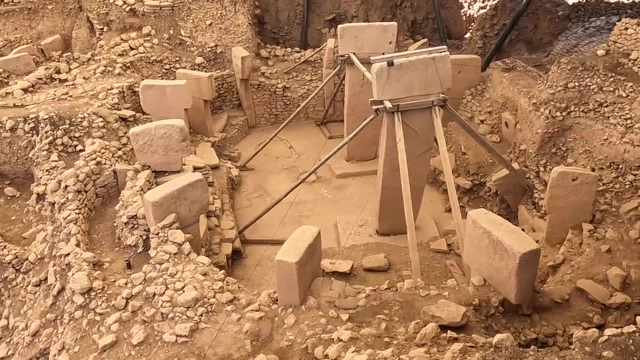 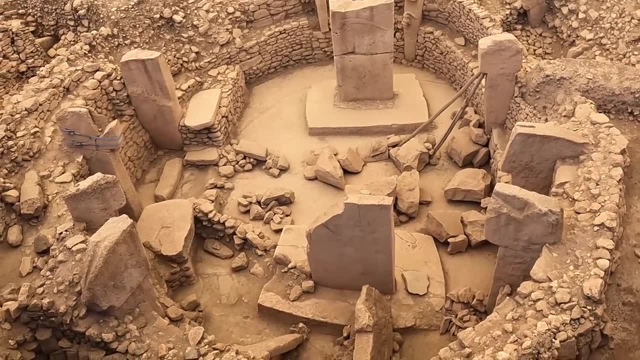 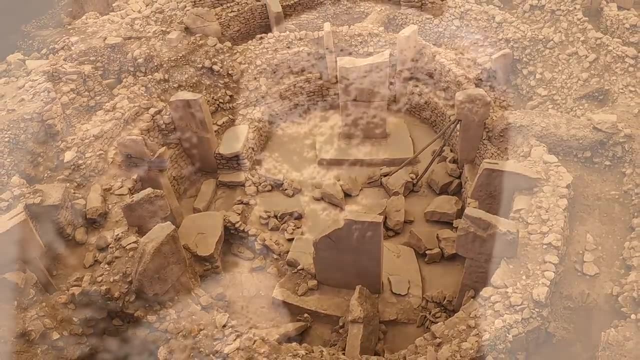 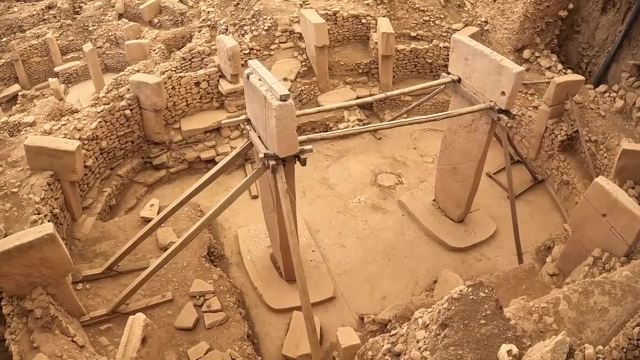 Far from a shadowy elite controlling the masses, like scientists and doctors today, early shamans or proto-priests would very likely have spent their days attempting to help their communities, to intervene with spirits, perhaps ancestors, and ultimately acting for the greater good. 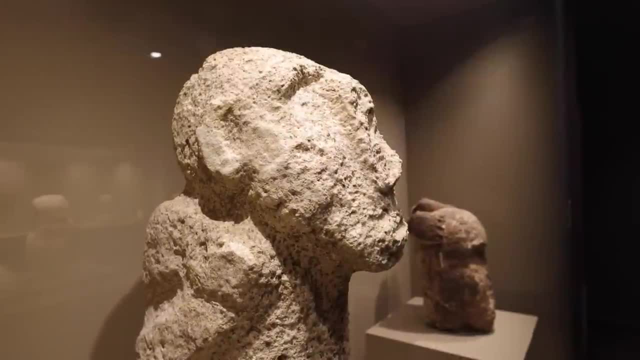 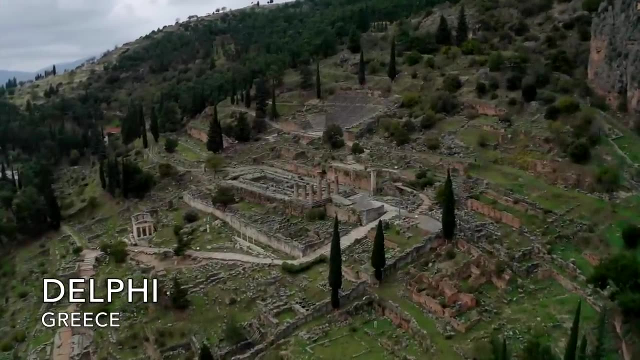 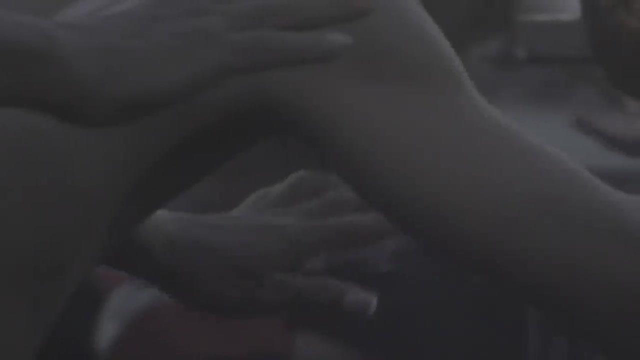 If they didn't, they probably wouldn't have been in their positions for much longer, Like the Vespers at Delphi in the Greek classical age, perhaps going into psychedelic trances To draw out near-impenetrable, yet nonetheless useful prophecies for those in need. 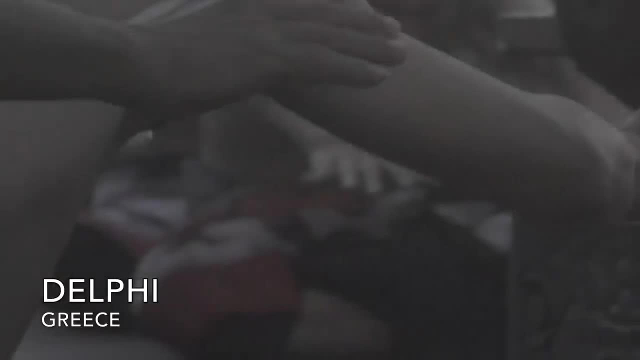 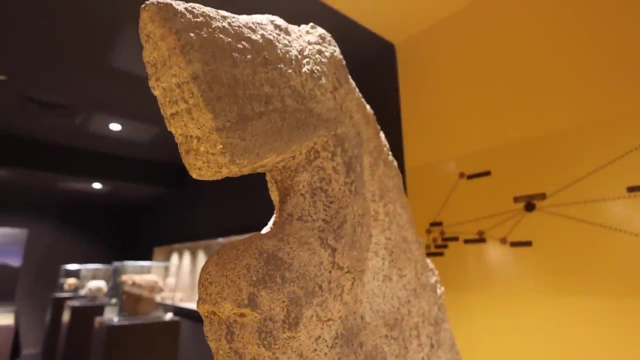 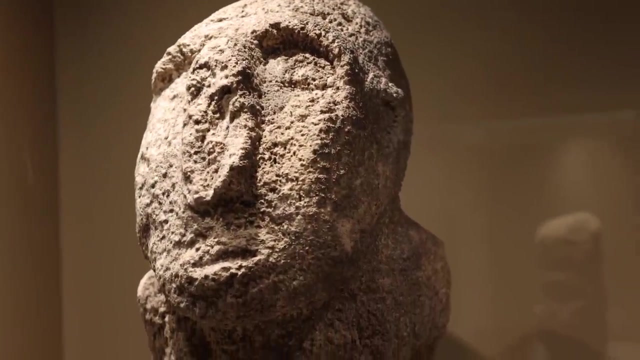 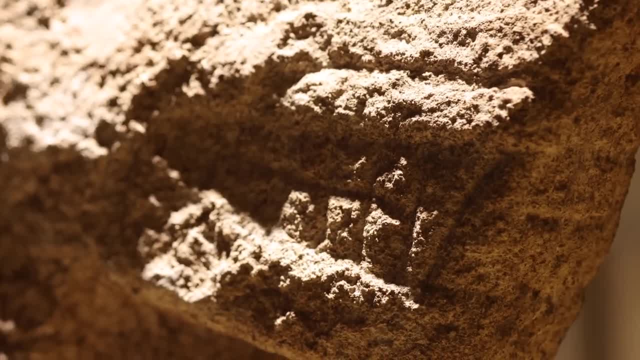 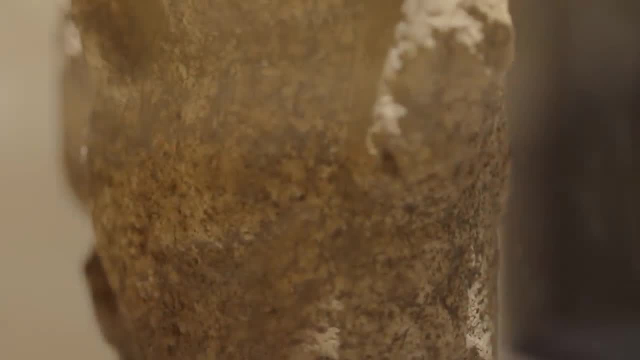 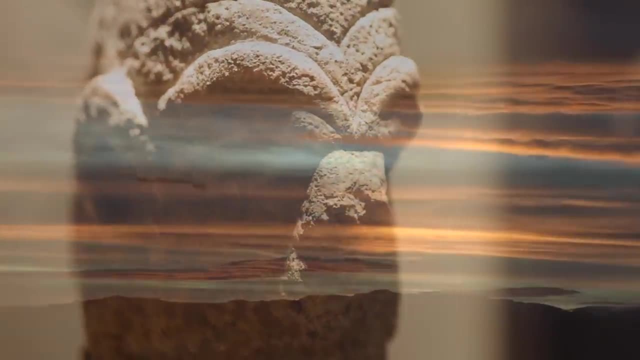 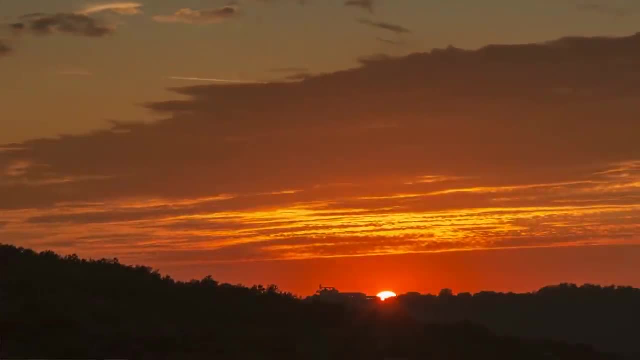 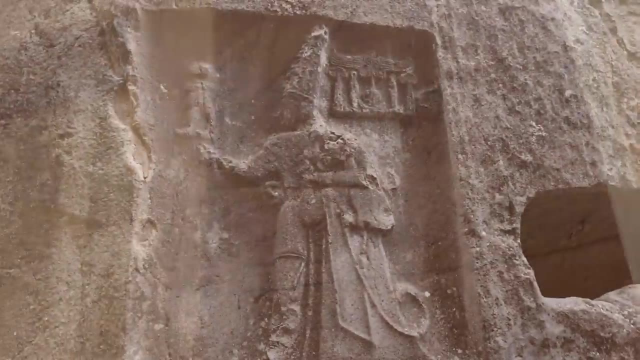 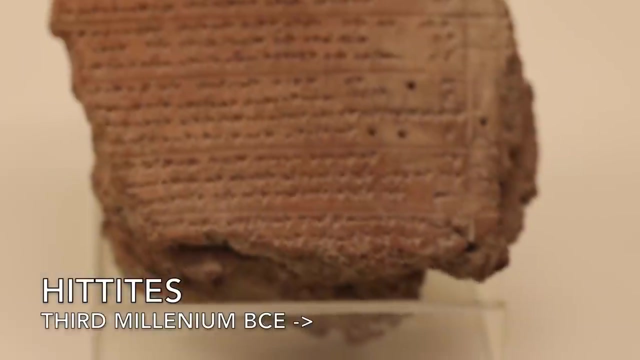 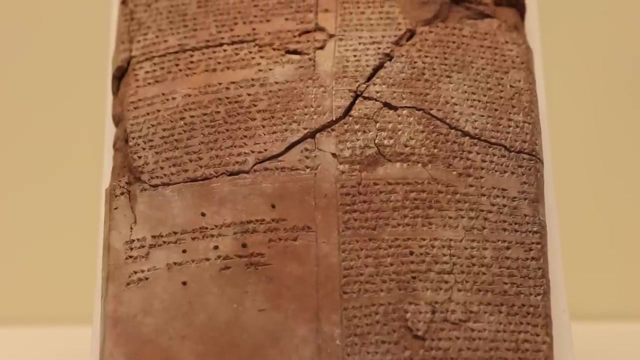 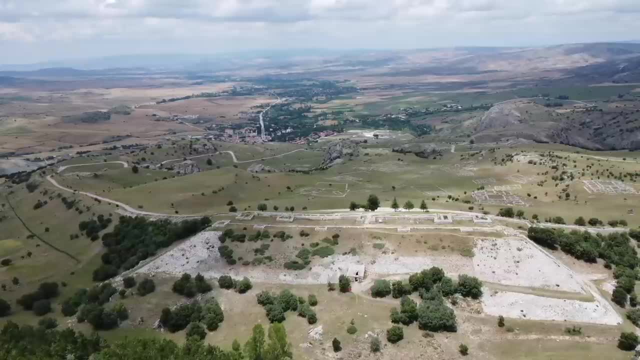 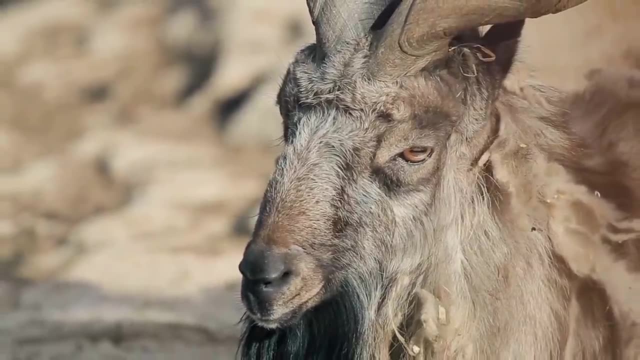 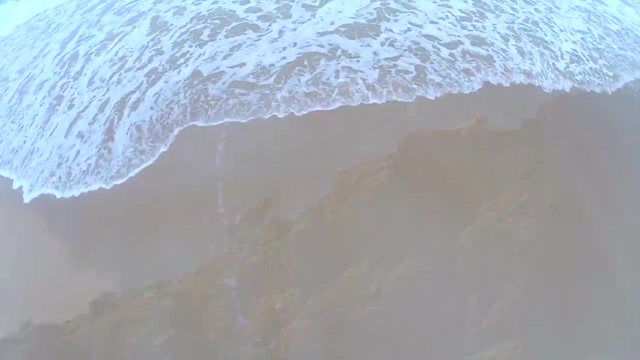 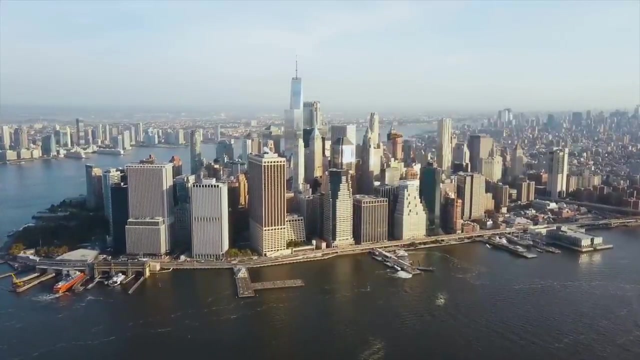 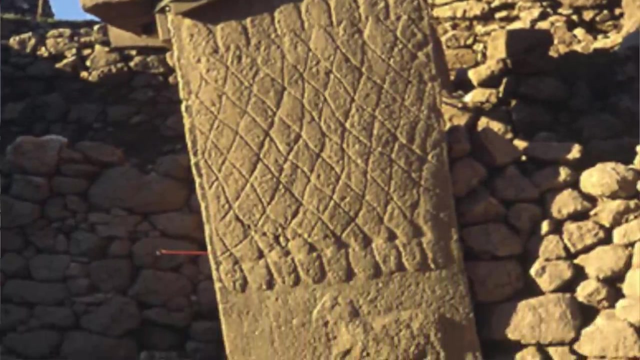 where members of a community would symbolically pile up sources of evil and anxiety onto a male goat. The sorry animal would then be chased out into the desert and left to its fate, thus relieving the society of its troubles. for a time, It's been argued that Pillar 1 at Gobekli Tepe could indicate a similar ritual. 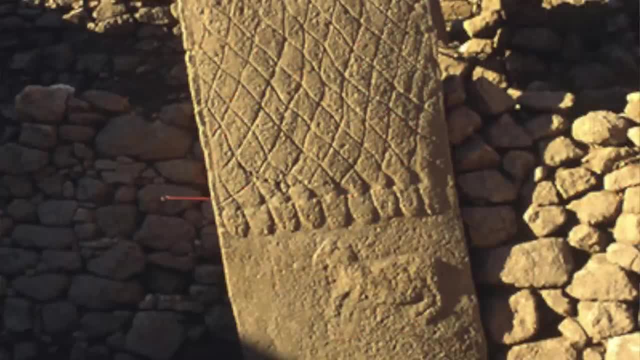 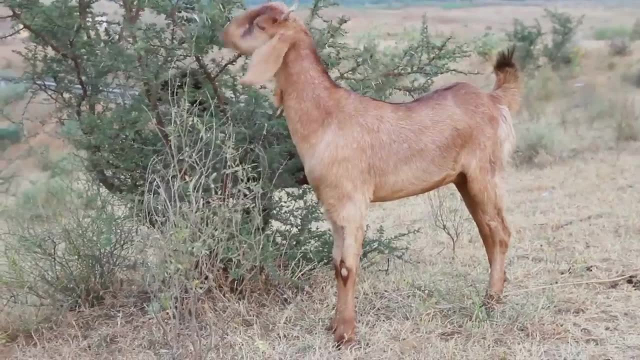 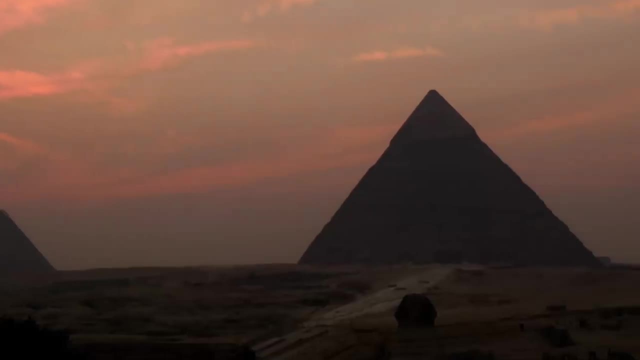 Of course, the origins of this ritual are unknown. The ritual itself websites the idea of a scapegoat, A ritual carried out unconsciously time and again throughout human history in almost every society on earth, And still very much in use today. 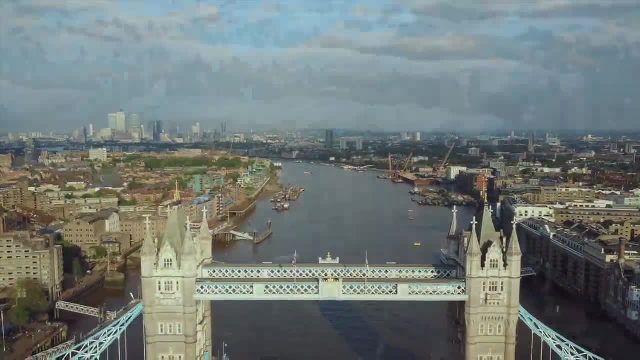 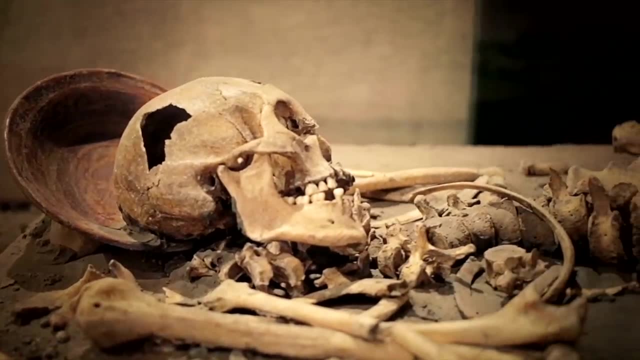 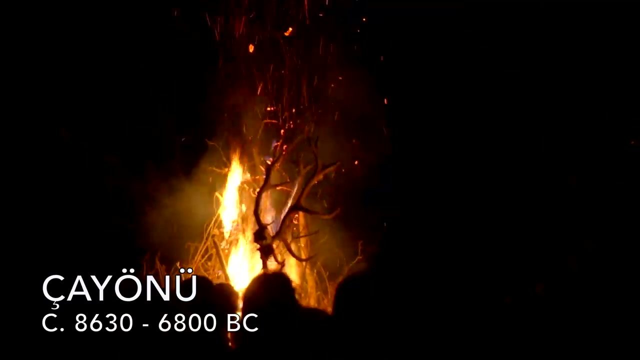 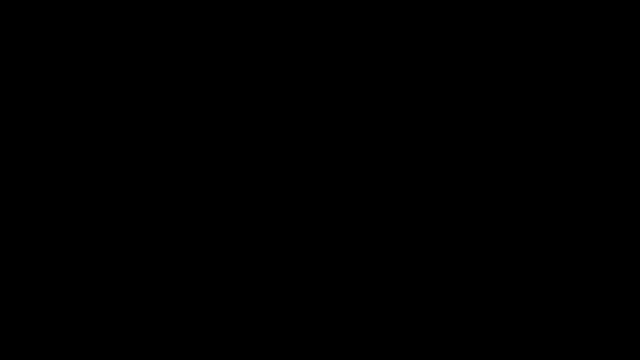 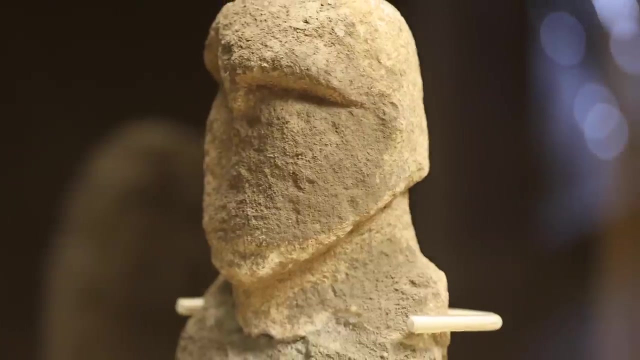 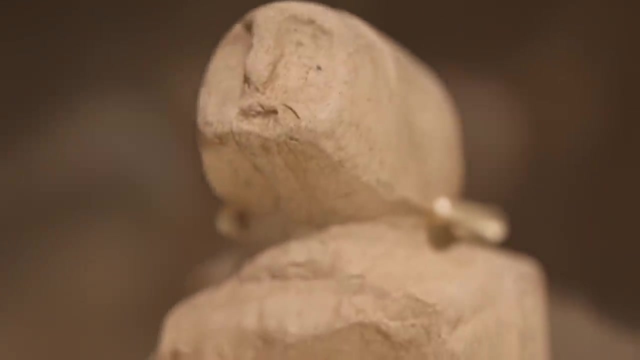 Of course, In many cases, much more than a goat is metaphorical, metaphorically forced out into the desert, As we have seen. at Chianu, a potential altar has been found which may well suggest human sacrifice, One argument being that sacrifice of animals, and sometimes people, became necessary to relieve. 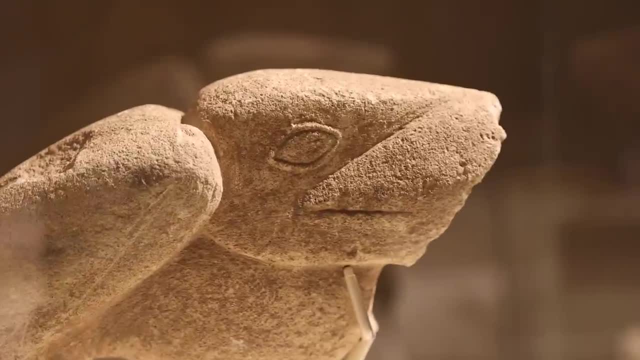 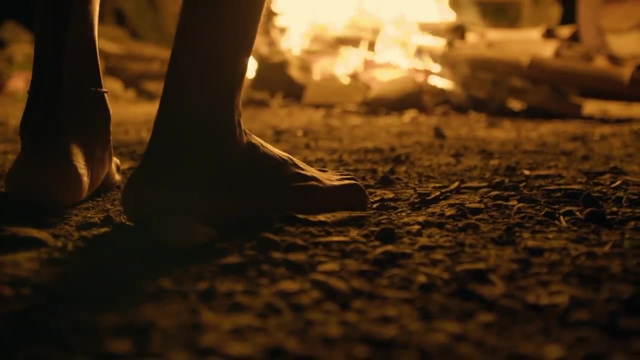 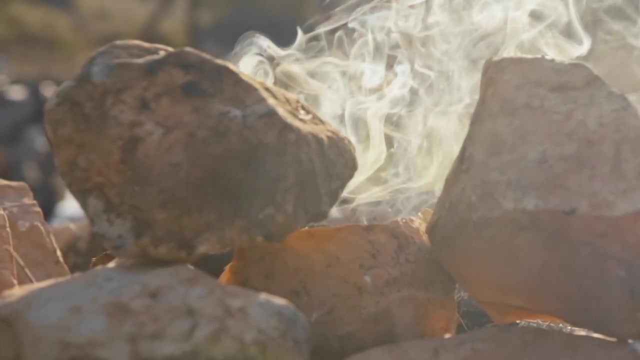 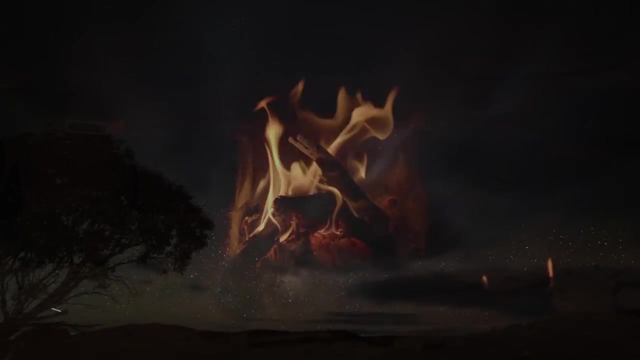 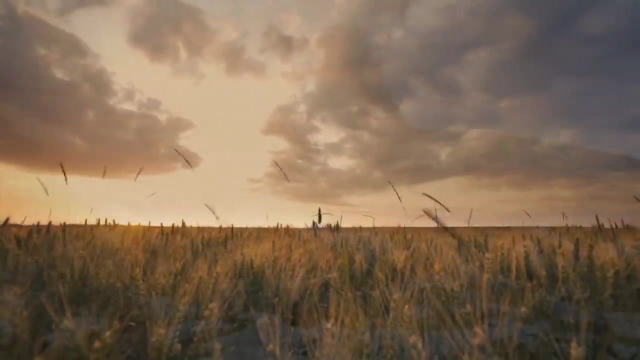 societal pressure during hard times, A placebo sometimes being effective as a morale boost or deliverer from stress. Indeed, from its very beginnings, the act of sacrifice does seem to have been an integral part of settled agricultural societies, Perhaps a means of psychologically being able to come to terms with the strange situation of delayed gratification. 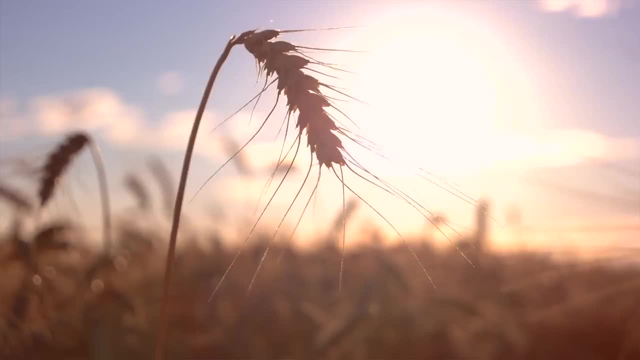 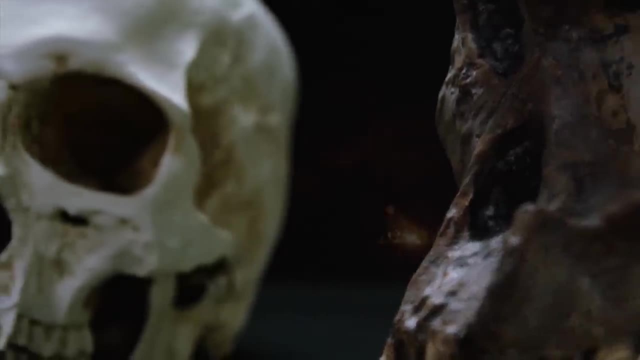 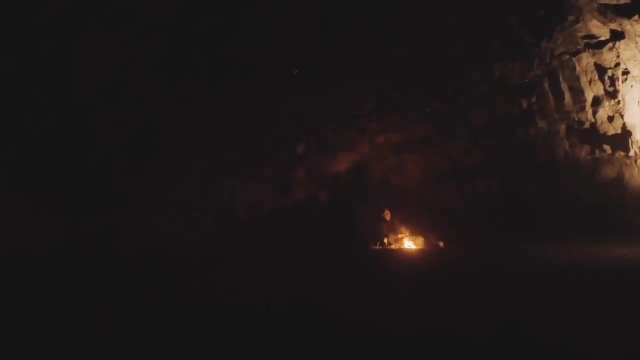 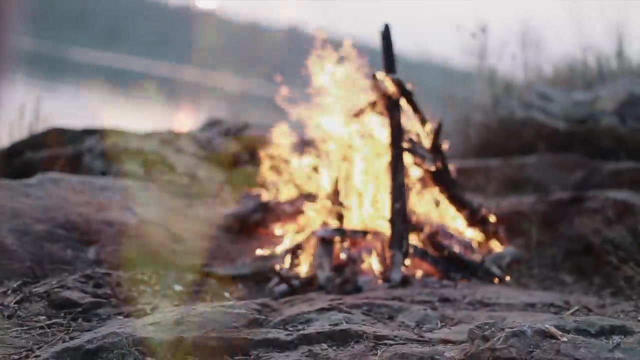 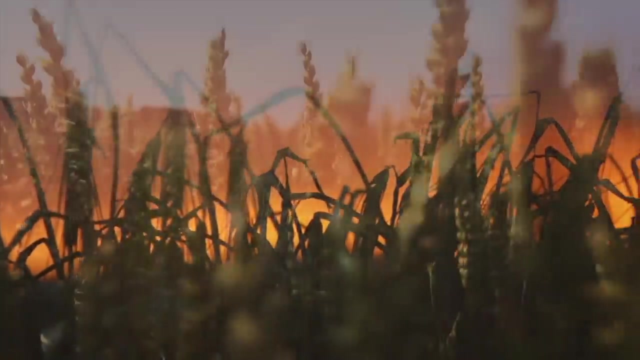 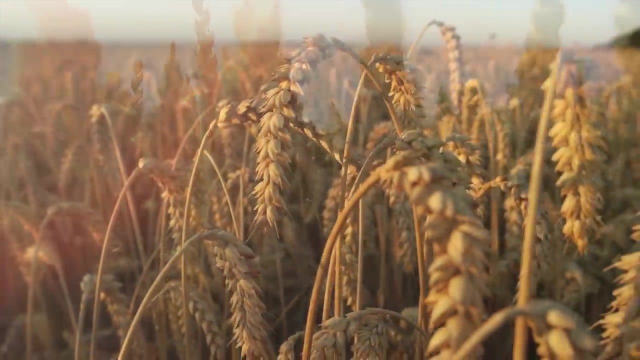 and occasional failure of harvests, An uneasy feeling that something has to be done to mediate with the divine And, in the aftermath, very often creating a sense of unity and community. Much more so if things do eventually turn around. Ultimately, as agriculture transformed their way of life, the newly sedentary Neolithic 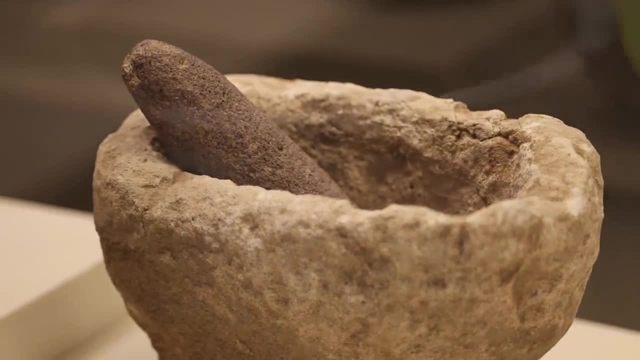 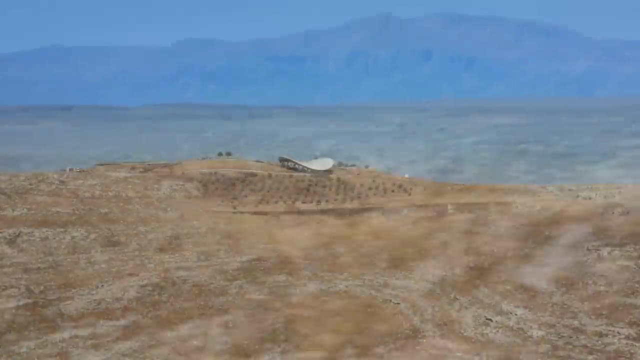 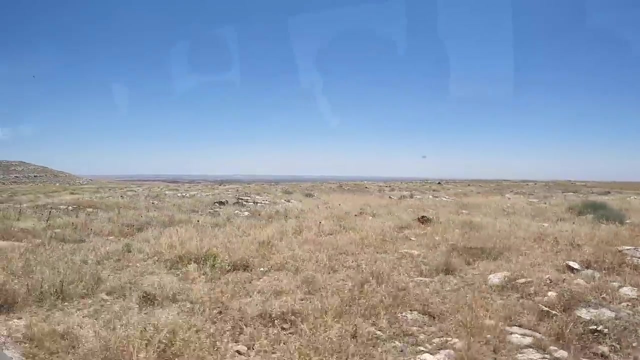 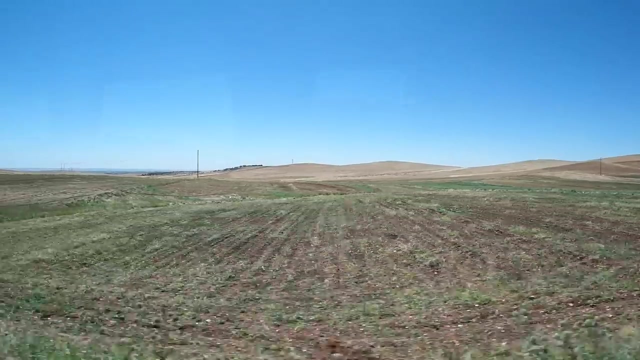 peoples of the southern Taurus Mountains ceased to make the pilgrimage. This was the only way to make it to the festival sites of the ancestors, Covering the circles in soil never to be seen again. Clearly, by around 8000 BC, the world had changed The T-shaped pillars, irrelevant in the face. 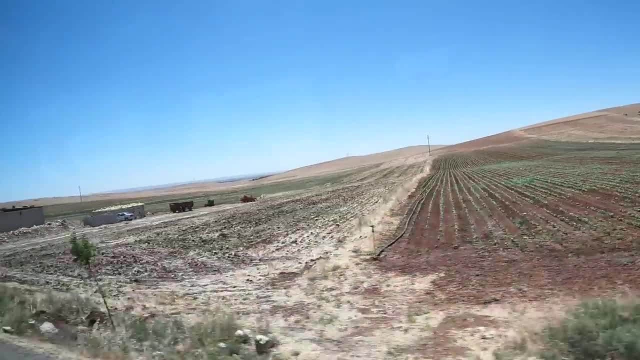 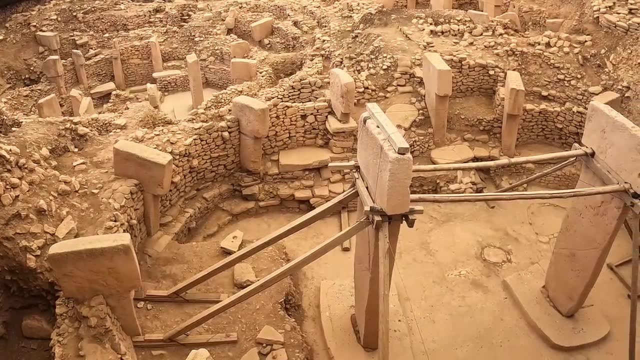 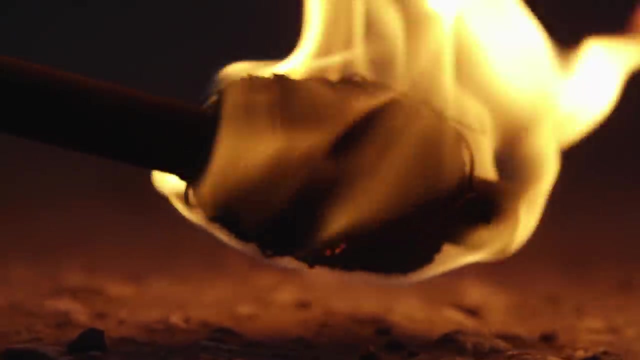 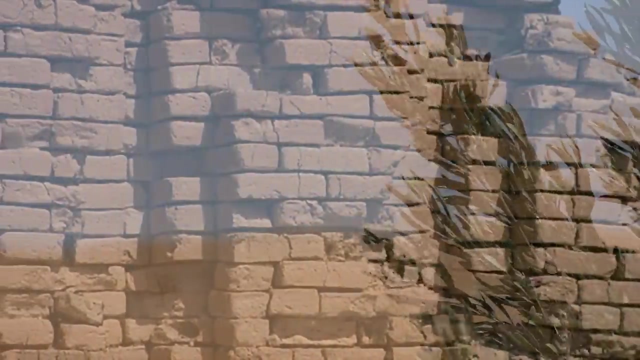 of new religious epiphanies, Whether any memory of their existence has ever been forgotten. it is unknown If any of their existence survived down the long millennia. we can only speculate. Somewhere along the line, many thousands of years later, by the 4th millennium BC, the 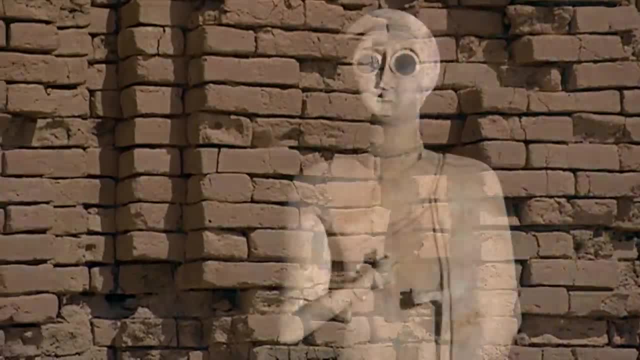 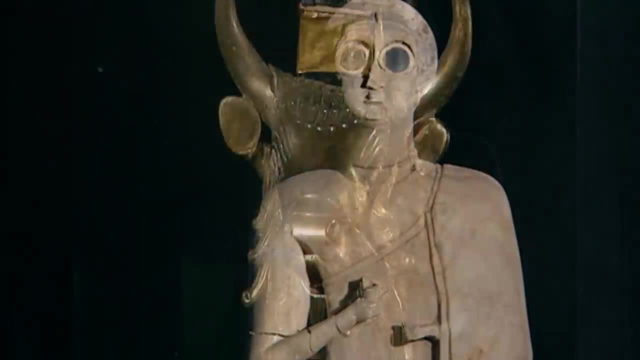 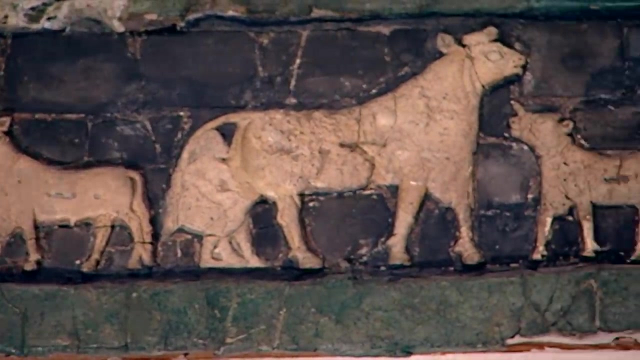 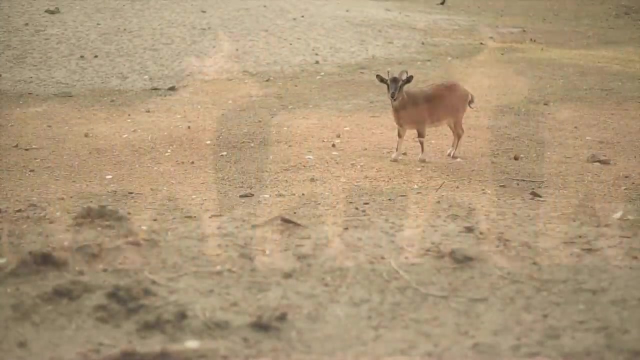 late Paleolithic shamans had become a priesthood. Whether any elements of deep-seated religion, religion, religion or religion have changed. it remains to be seen Whether any elements of deep-seated lore from the T-shaped pillars survived into those days, just as they had from the Upper Paleolithic. we will likely never know. 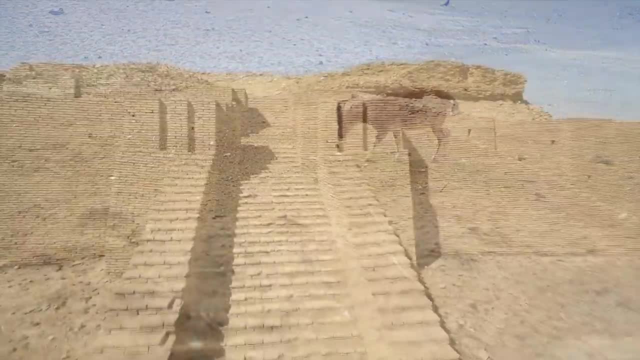 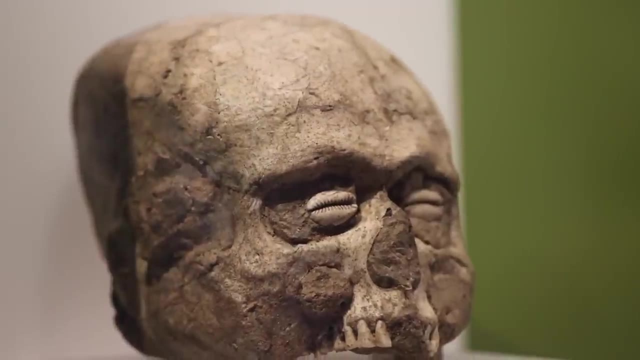 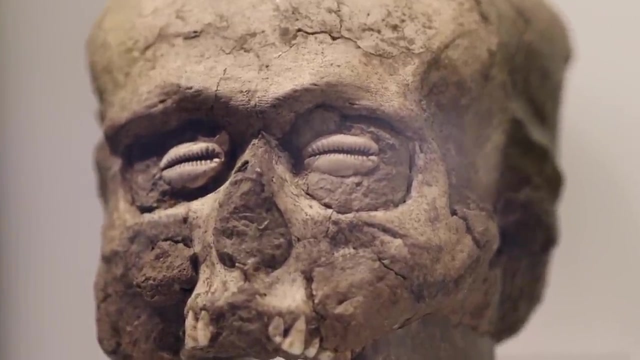 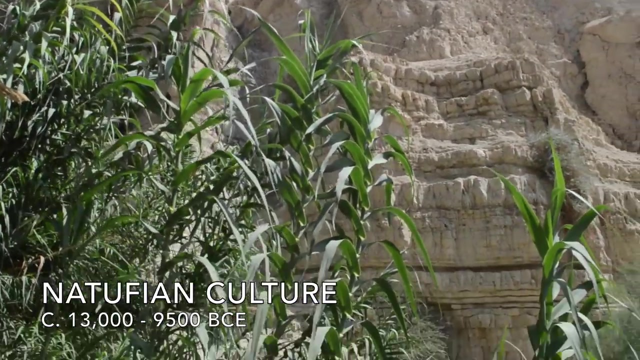 Though it remains at least possible. Skull removal and decoration, for example, continued in use for thousands of years after Stonehill's culture disappeared, Just as it had done before with the Natufians, And there are two-headed Janus figures at Gobekli Karahan and Gaziantep. 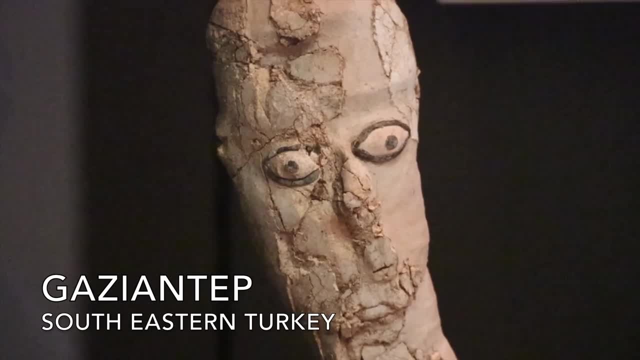 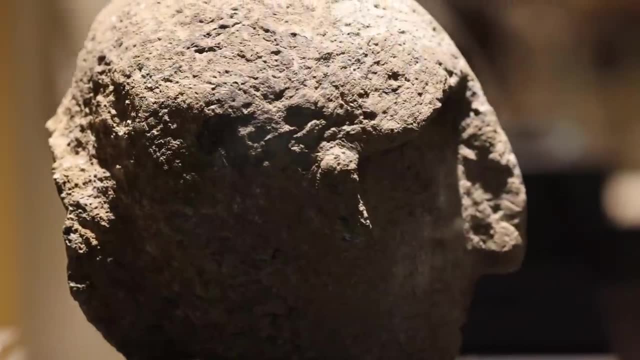 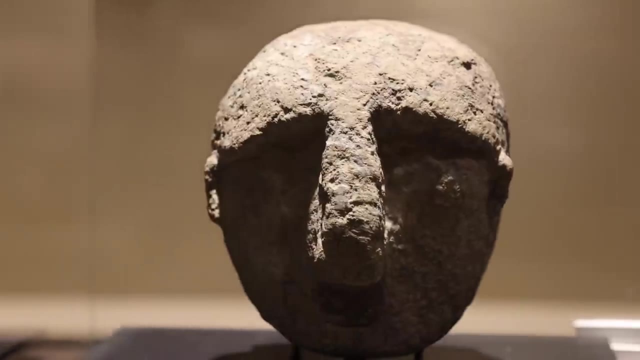 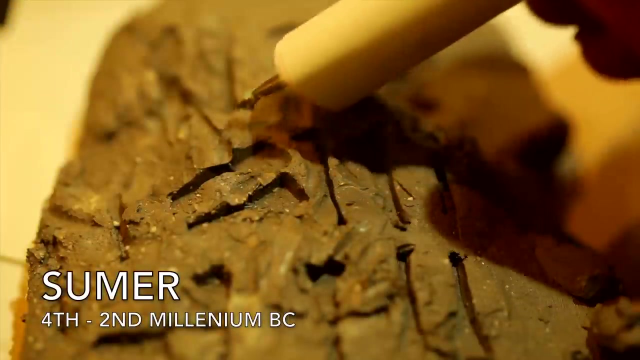 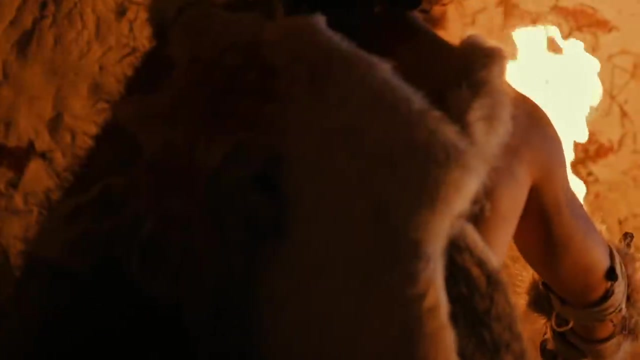 Just as there continued to be in much later millennia and today Perhaps, representations of the duality of existence. By the time of ancient Sumeria in the 3rd millennium BC, when stories began to be recorded in writing for the very first time, all manner of much older spoken tales managed to survive. 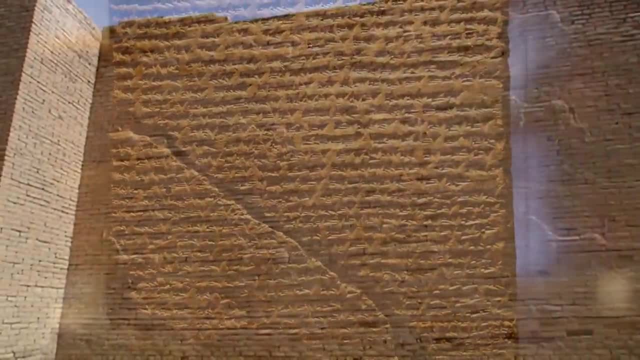 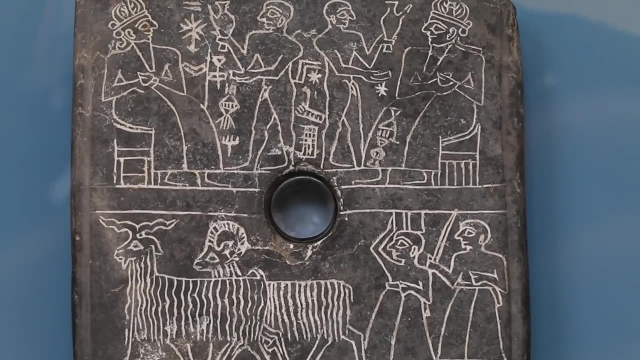 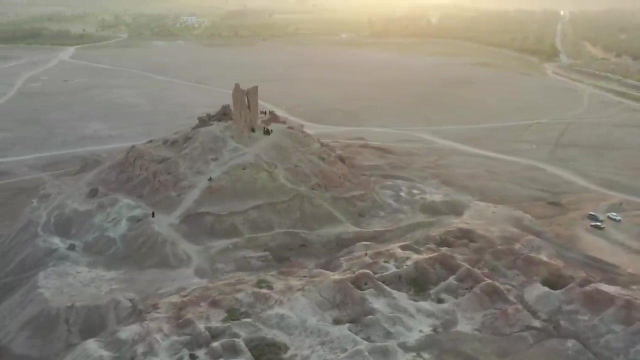 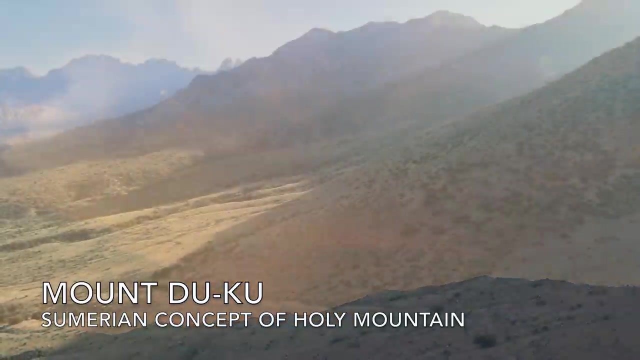 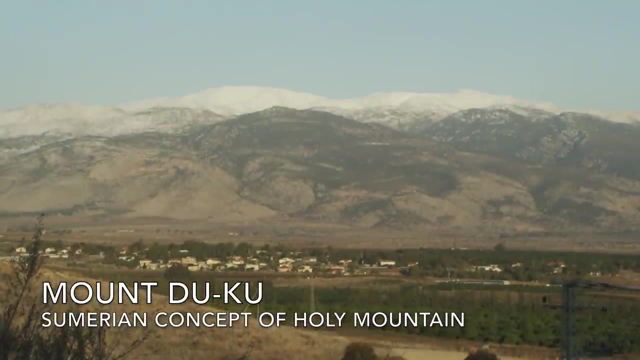 too, finding their way into the cuneiform archives of long-deceased city-states and forgotten kings. One of those tales speaks of a sacred mountain, Duku, Home of the ancient Honora gods, A sacred mountain sometimes associated with the hilly region around the Taurus and Zagros. 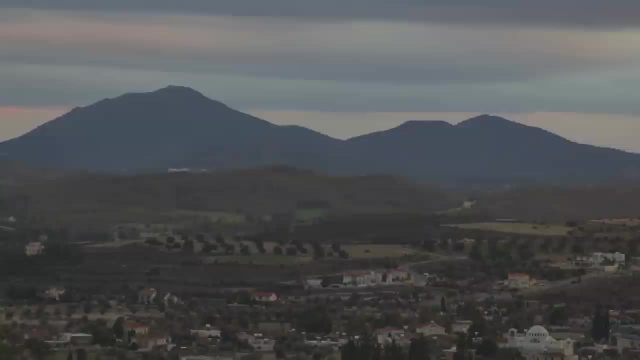 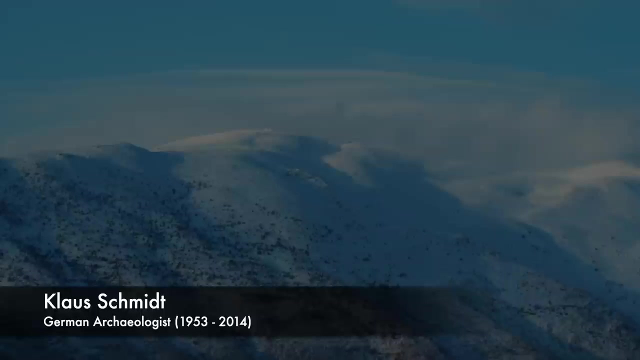 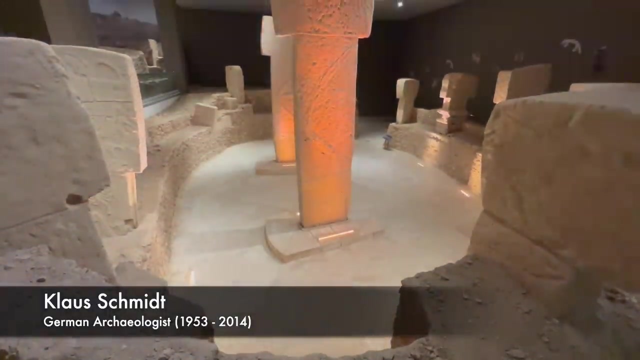 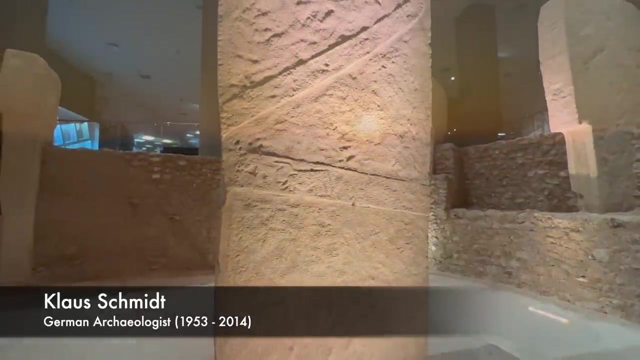 range on the very northern edge of the Mesopotamian world. It's a long shot, but Klaus Schmidt thought it at least possible that some shadow of the anthropomorphous pillars of Gobekli Tepe ultimately survived down the ages passed down by individuals. 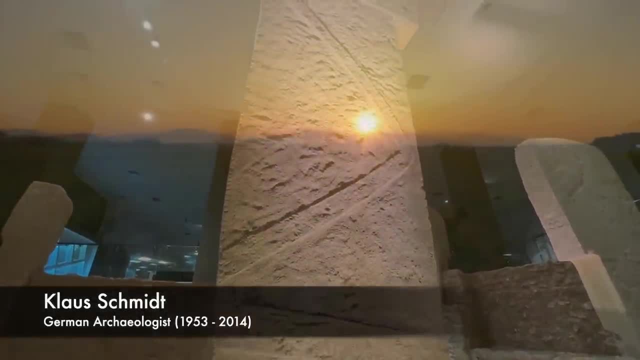 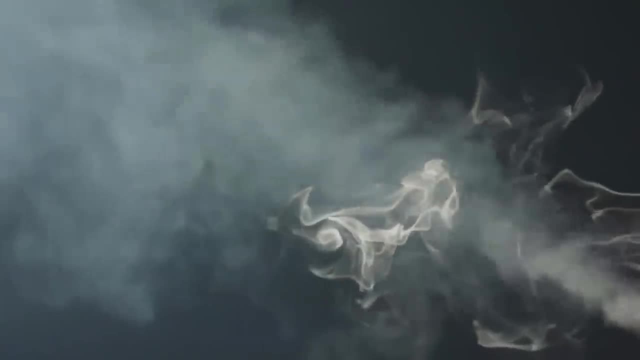 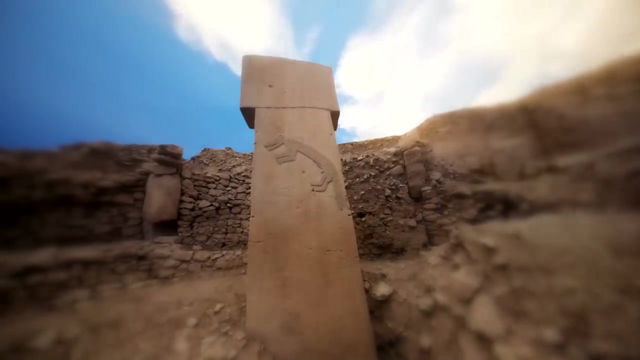 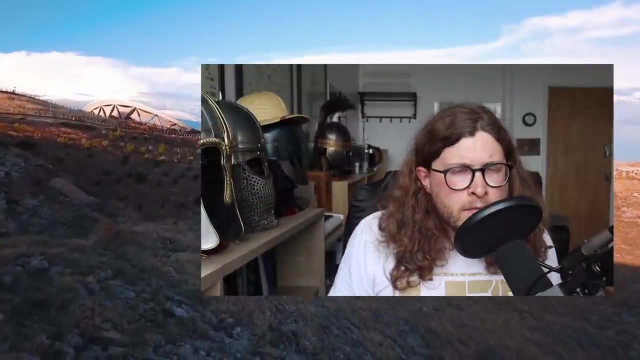 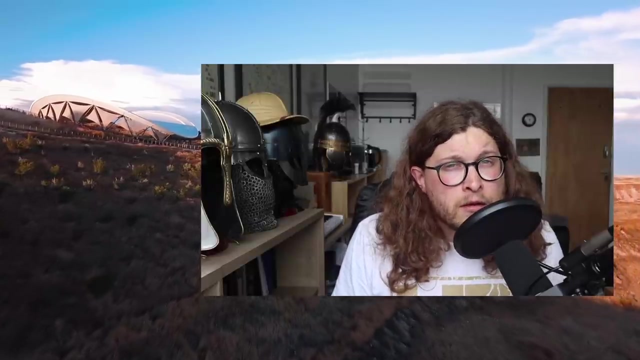 from one generation to the next to become myth and legend. After all, what else do we have but stories? Thanks for watching. As always, I'm your host, Pete Kelly. Another massive thank you to War Thunder for sponsoring this video.